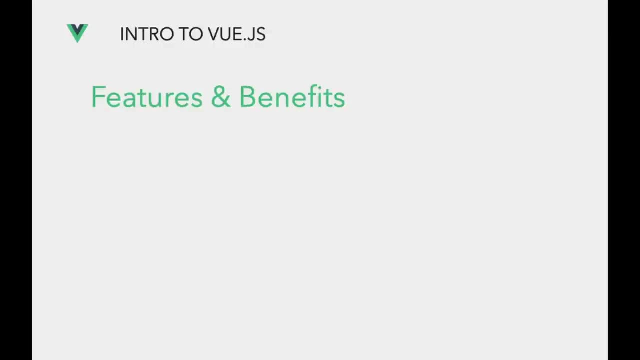 and teams that work in the same code base. If you have heard of the virtual DOM before, Vuejs is a virtual DOM framework. If you don't know what that is, it's okay, It's not important for understanding this course. The virtual DOM basically makes JavaScript web applications a little bit faster and more. 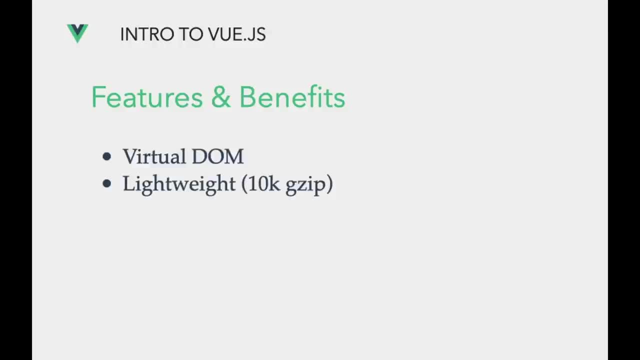 efficient. Vue by itself is extremely lightweight. You can get it down to about eight or 10 kilobytes. It's very easy to use. It's a very simple application. It's not as complex as JZipped, Although in a practical sense, your Vue and bundled JavaScript will probably never be. 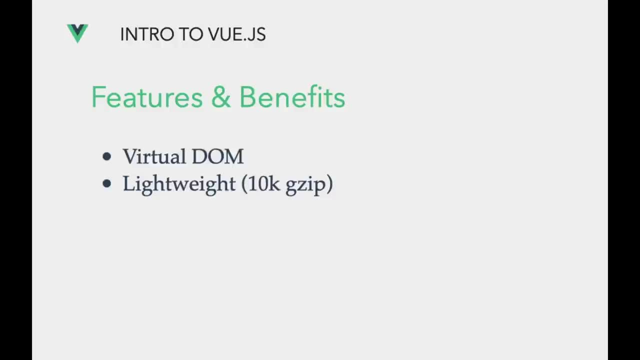 that small in an application anyway, Although it is good to know that Vue doesn't have a lot of extra code taking up more space in your application. Why does Vuejs call itself a progressive framework? They use the term progressive to mean that you can use it anywhere from small features. 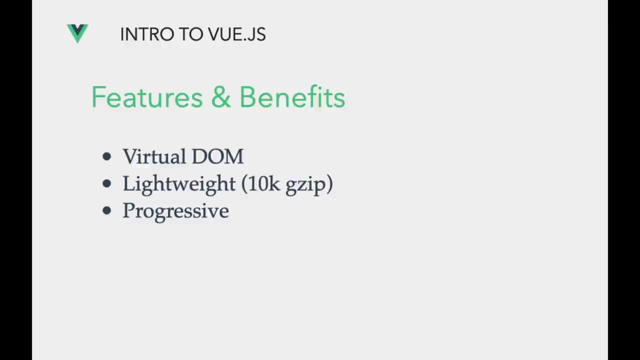 on websites Where you want to add something, Where you want to add some interactivity, And using it as kind of a drop-in replacement for jQuery and legacy applications, All the way up to using it as a more full-featured, batteries-included framework for large-scale. 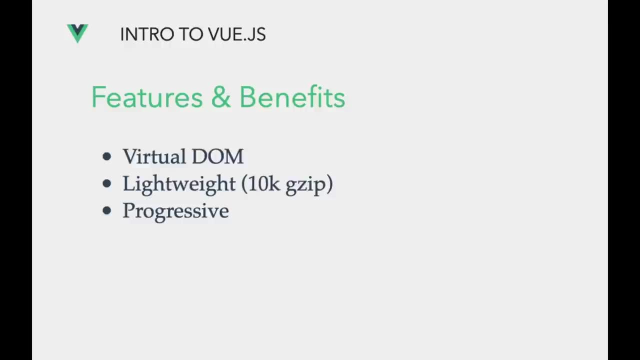 applications like Gmail or Twitter or something like that. You get to decide what features you want to add in from the Vue ecosystem beyond the core library, And it's extremely flexible to allow you to choose the tools and other libraries you want on your own. 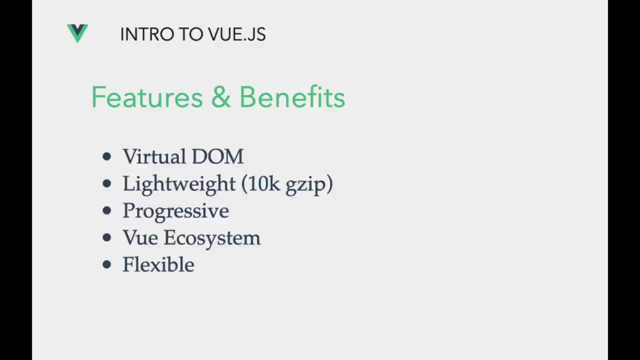 Or you can use the ones that Vue provides in its ecosystem by default. Many people and companies are using it for its incrementally adoptable nature. That means that if they have a legacy application, it's quite simple to update their application page by page. 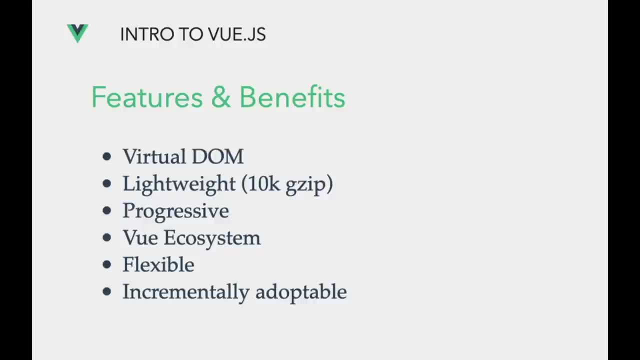 To turn it into a Vue application, To turn it into a more modern application, Instead of having to rewrite the whole app at once. That is one very convenient thing about Vuejs. Let's look at a really quick overview of the history of Vue. 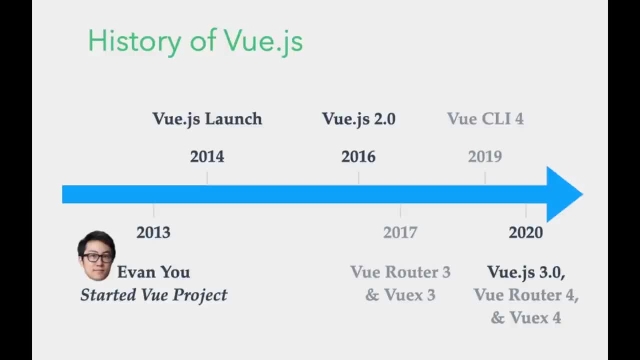 The Vue project was started in 2013 by its founder, Evan Yu. In 2014,, version 1 launched And it started to become popular in China, where Evan Yu is from. A few years later, Vue 2 was launched. 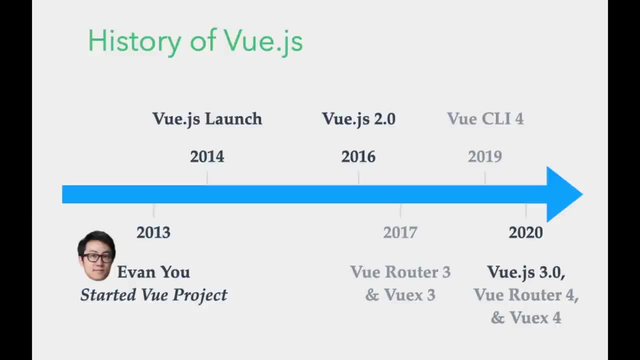 With many new updates and improvements over Vue version 1.. And with the release of version 2, is really where we start to see the massive growth of Vuejs in popularity in the rest of the world. So many developers had not heard of Vuejs before 2017.. 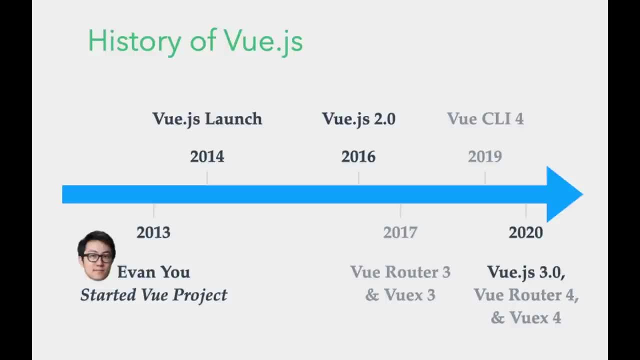 But from 2017, and especially in 2018 and 2019, Vue really solidified itself as one of the top three JavaScript frameworks. Many Vue conferences Started popping up. lots of content creation around the Vue ecosystem started to take place. 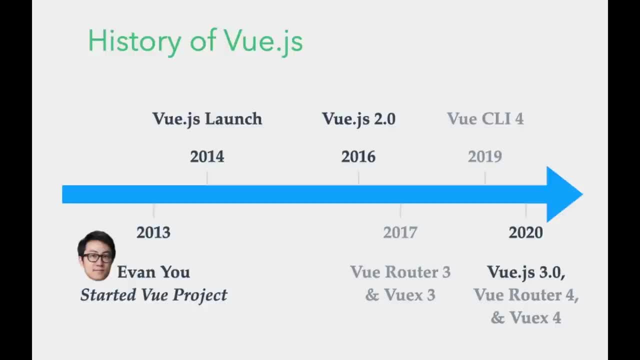 And many companies started to use Vue for their applications as well. In fact, many companies that you recognize, which are household names in the West, use Vuejs now, And now we can see that Vue version 3 has been released in fall of 2020.. 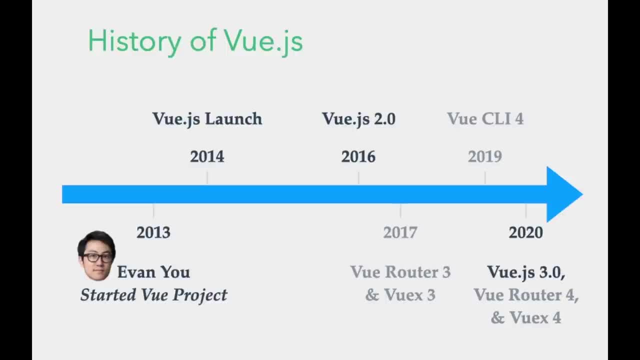 And along the way over these last six years, we see many different libraries that are also created and maintained by Evan Yu and the core team of Vue, Like the Vue CLI, Vue Router and Vue X, Also being regularly updated to match with the current version of Vue. 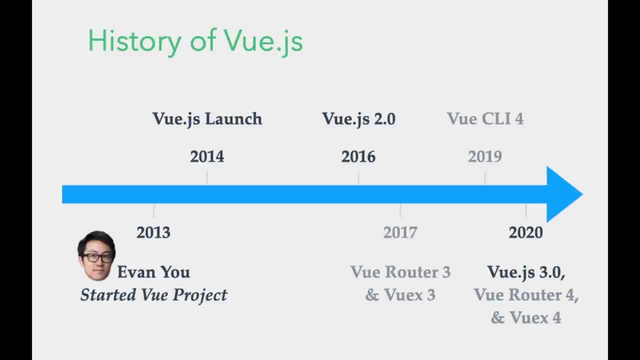 Even now, with Vue 3 just released, we see that a new version of Vue Router and Vue X have also been released to be compatible with Vue version 3.. In this course, we will be using the Vuejs core library as well as the Vue CLI. 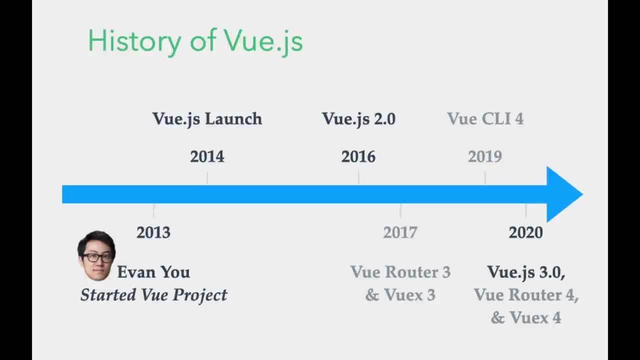 For more information about Vuejs and Vuejs core library. please visit the Vuejs core library For more information on VueX, Vue Router, Vue TestUtils and some of the other tools in the Vue ecosystem that I don't cover in depth in this course. I will be making future. 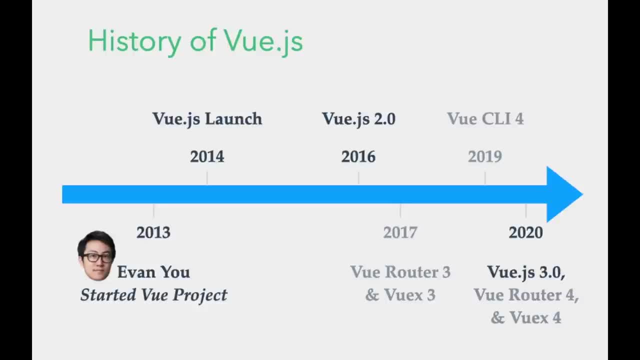 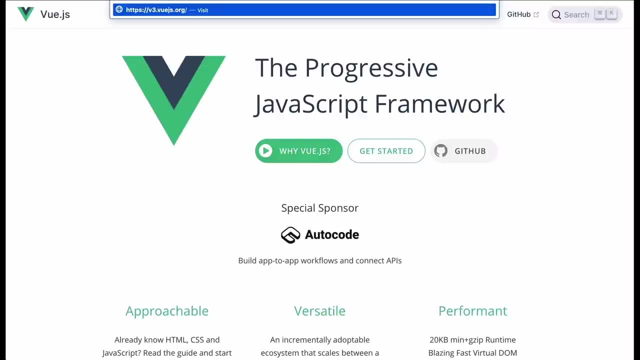 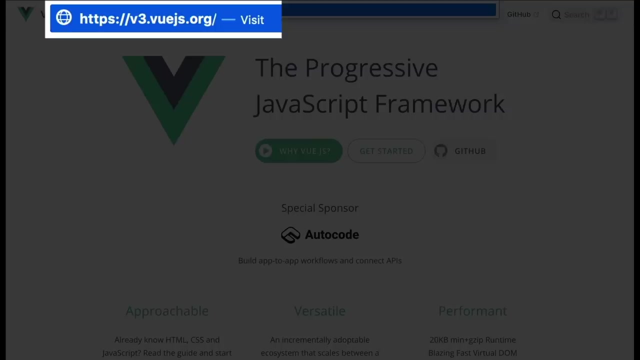 courses, about those on my Faraday Academy YouTube channel. So let's get started with learning Vuejs, And keep in mind I'm using Vue 3 here, so make sure you are at the correct website, which is v3.vuejscom. 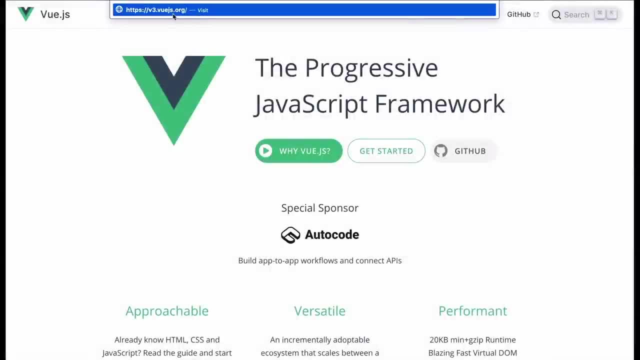 So let's get started with learning Vuejs. And keep in mind I'm using Vue 3 here, so make sure you are at the correct website, which is v3.vuejscom. So let's get started with learning Vuejs. 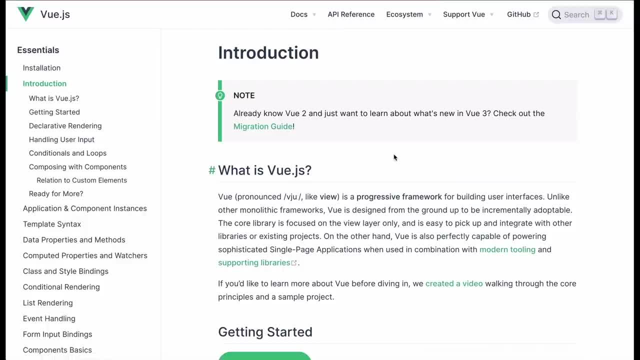 And keep in mind I'm using Vue 3 here, so make sure you are at the correct website, which is v3.vuejscom. So let's get started with learning Vuejs. And keep in mind I'm using Vue 3 here, so make sure you are at the correct website. 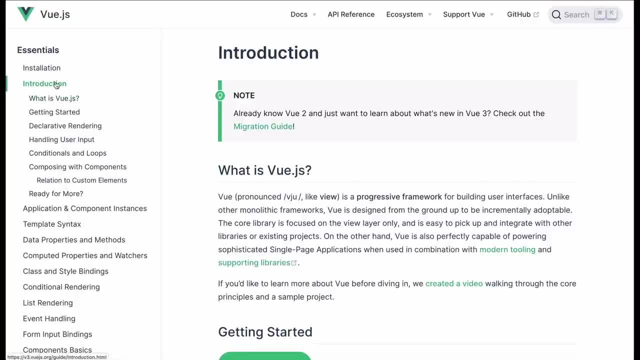 which is v3.vuejscom. So let's get started with learning Vuejs. And keep in mind I'm using Vue 3 here, so make sure you are at the correct website, which is v3.vuejscom. So let's get started with learning Vuejs. And keep in mind, I'm using Vue 3 here, so make sure you are at the correct website, which is v3.vuejscom. So let's get started with learning Vue 3 here, so make sure you are at the correct website. 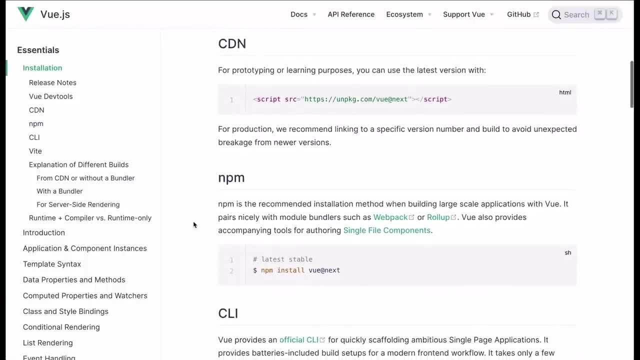 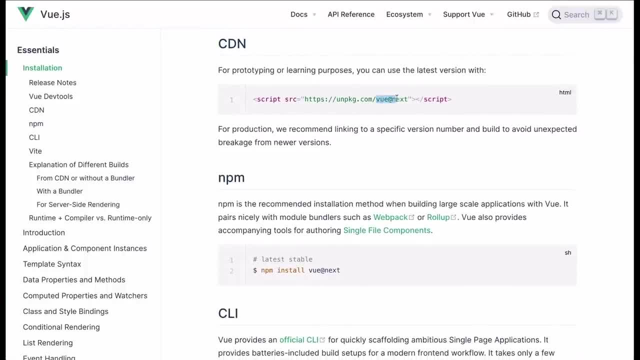 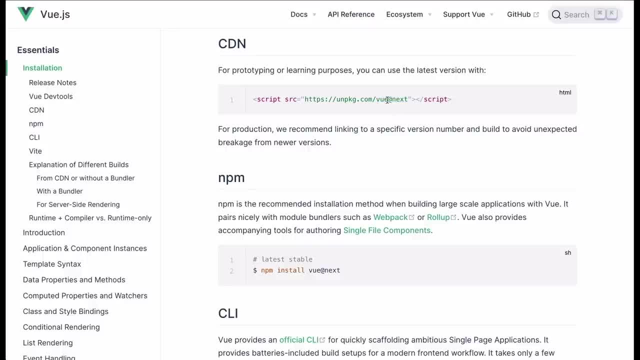 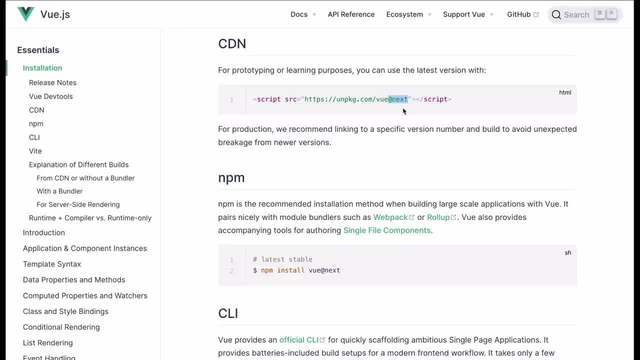 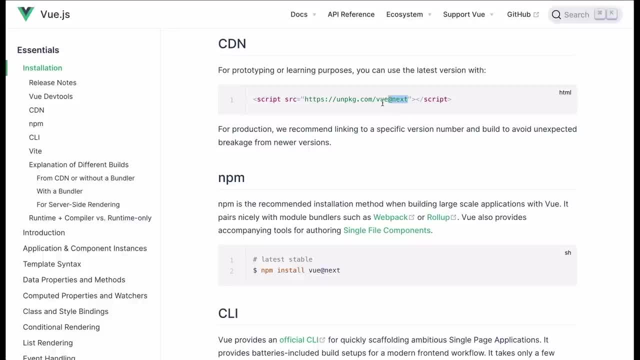 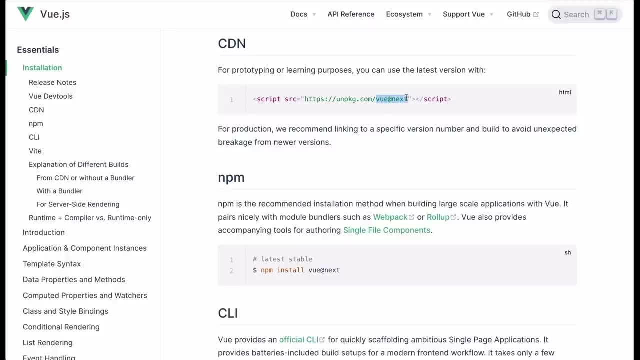 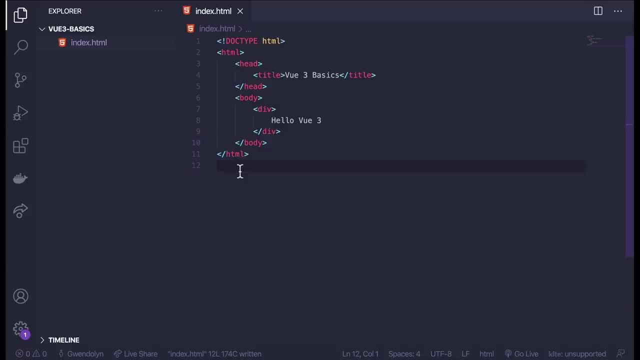 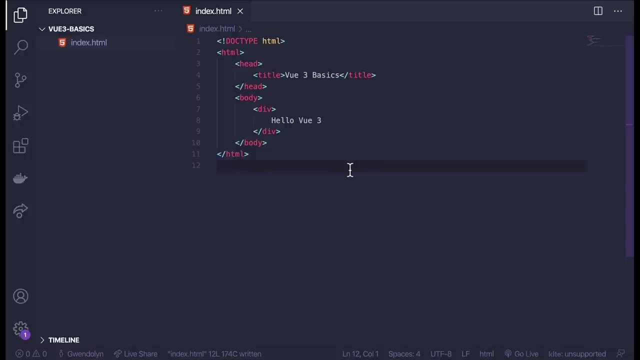 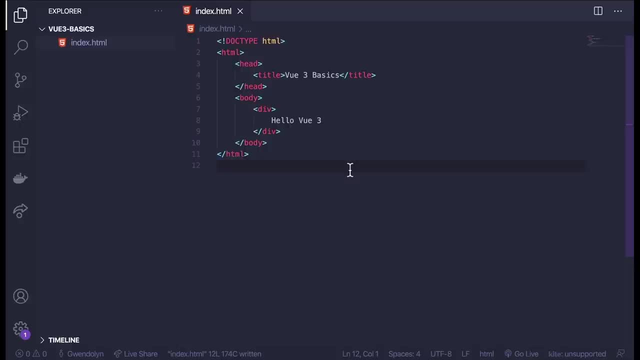 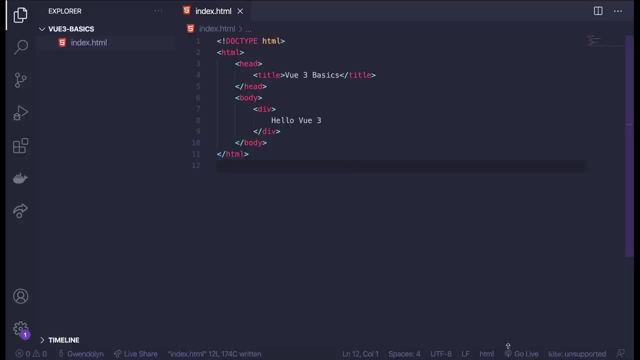 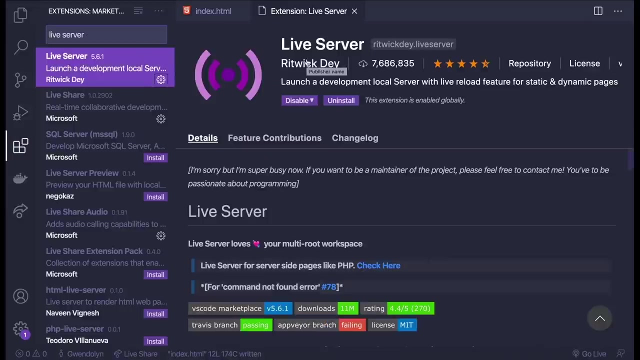 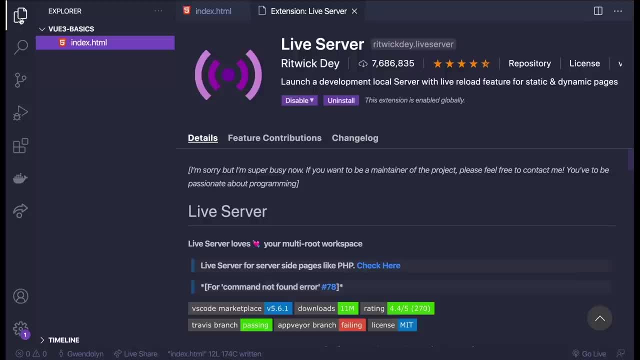 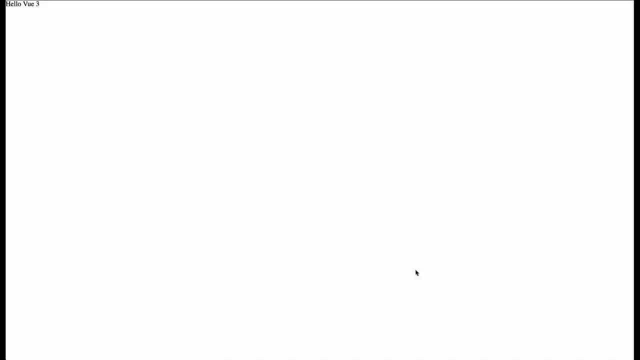 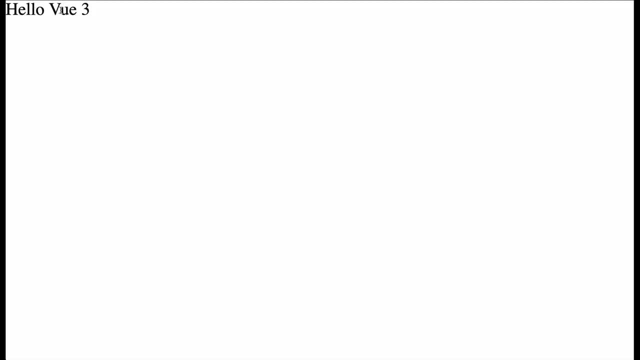 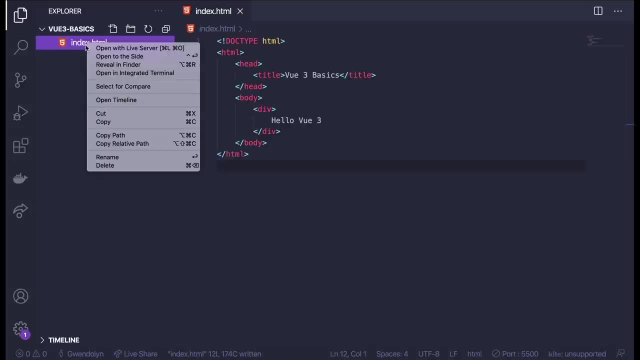 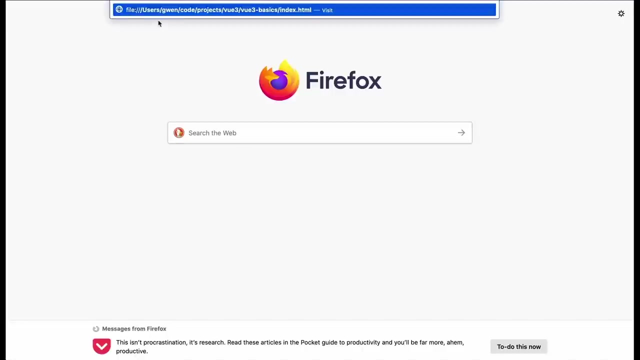 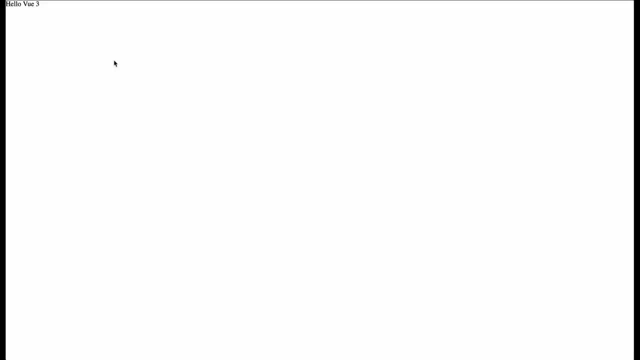 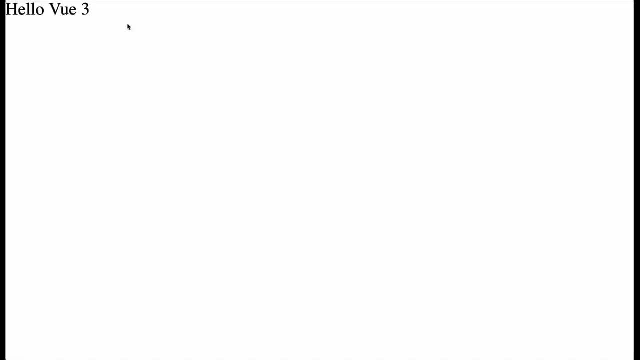 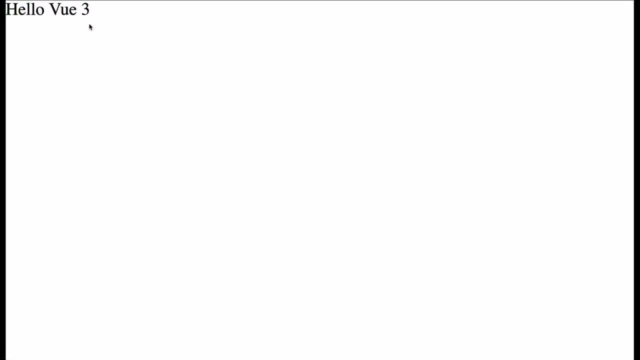 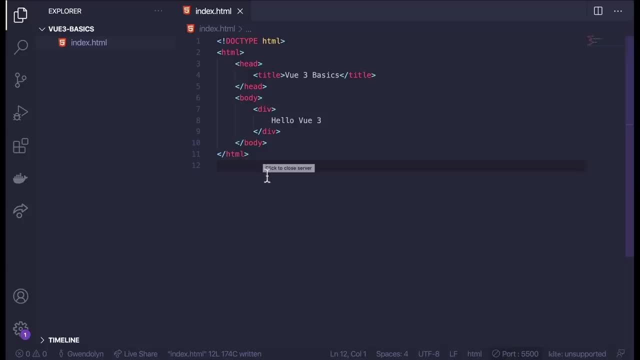 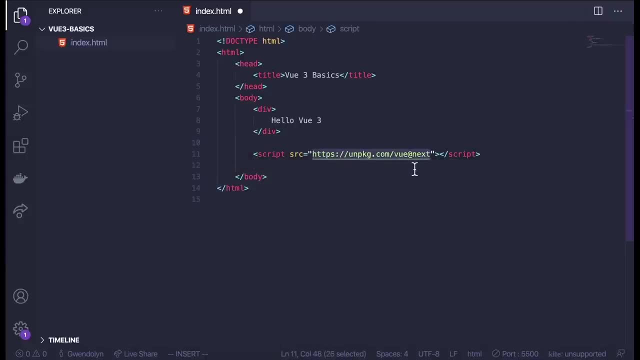 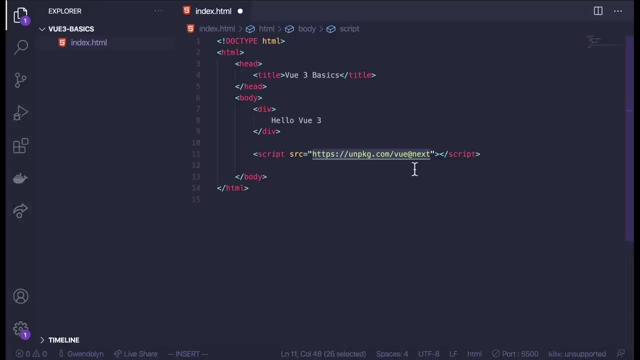 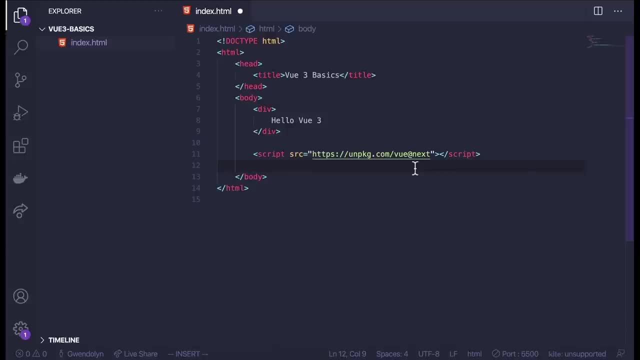 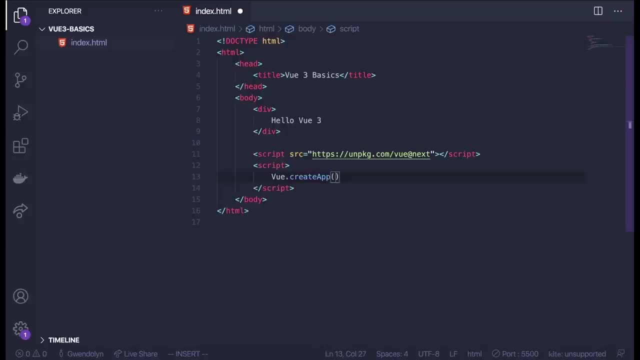 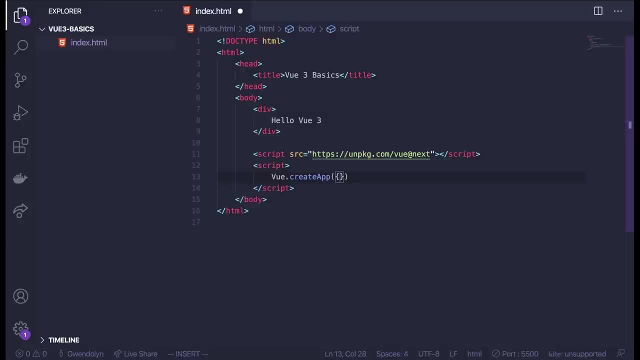 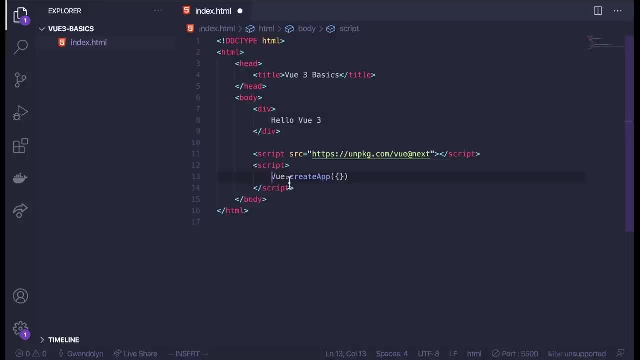 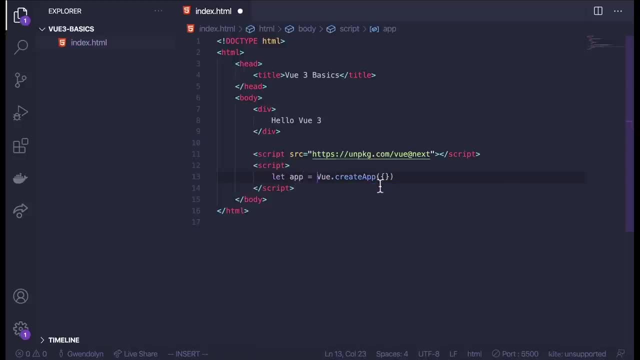 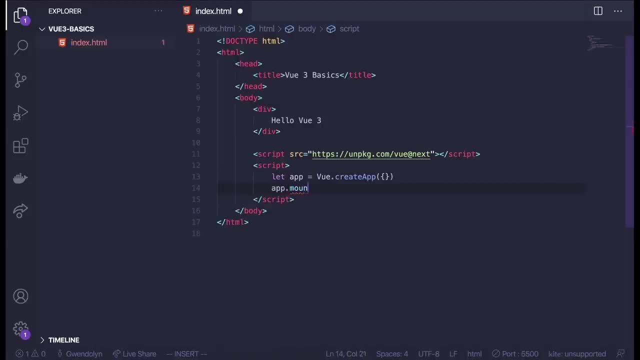 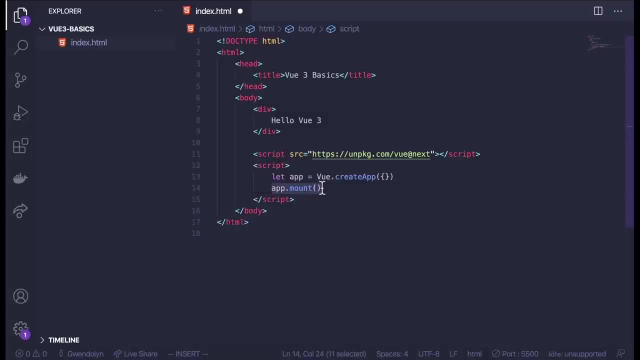 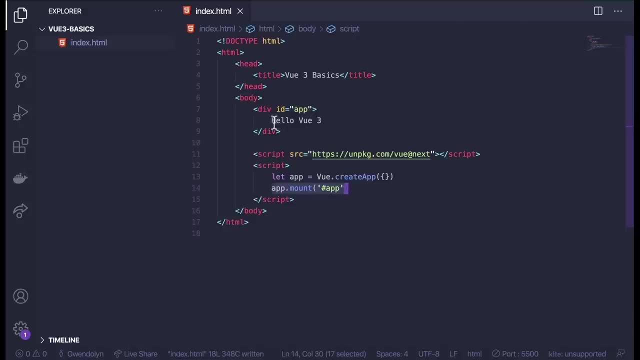 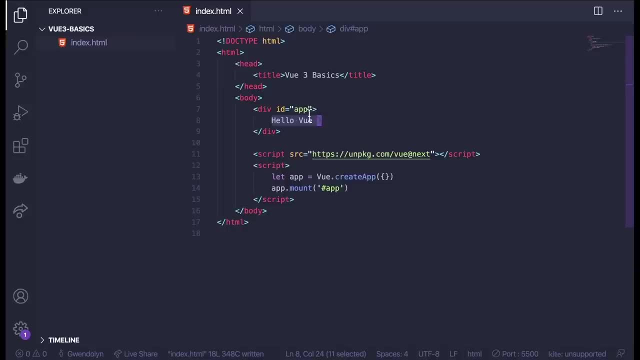 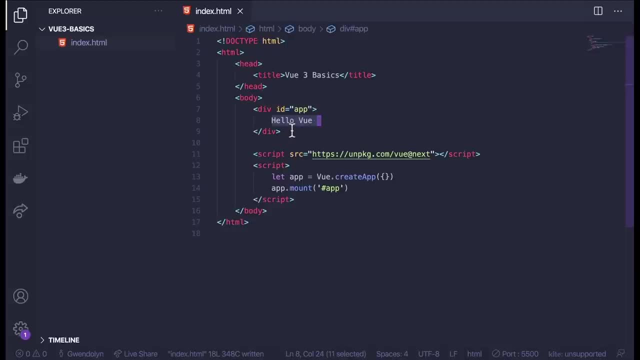 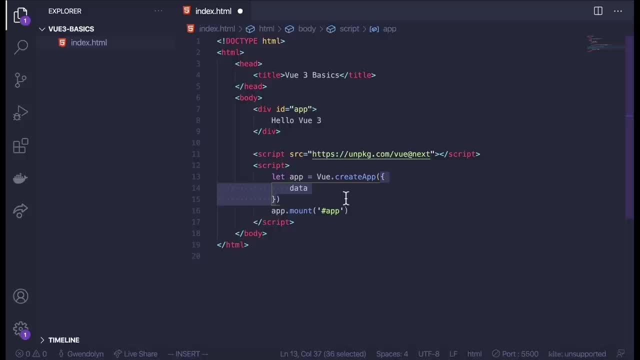 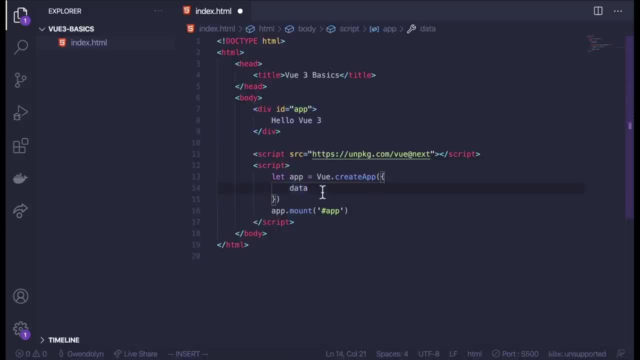 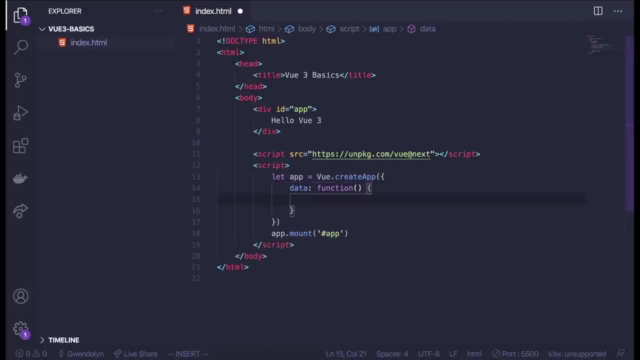 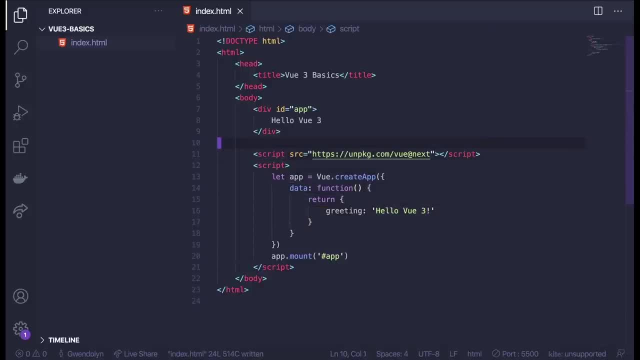 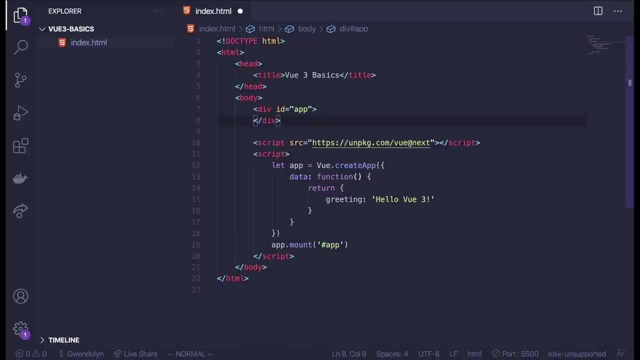 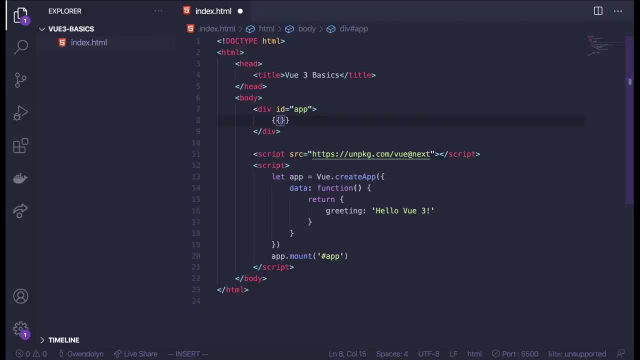 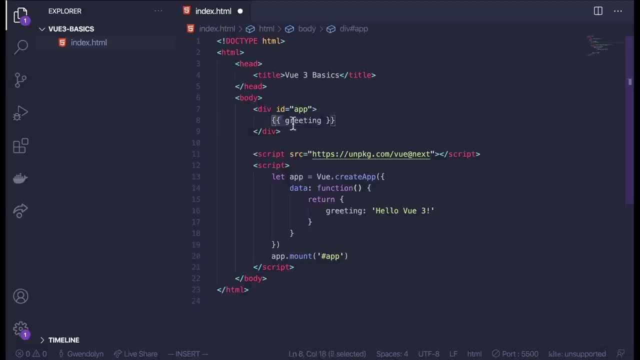 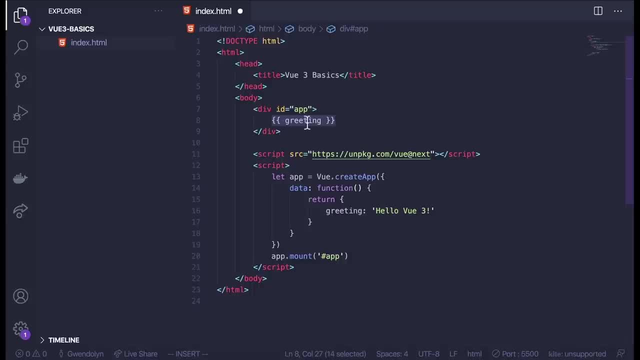 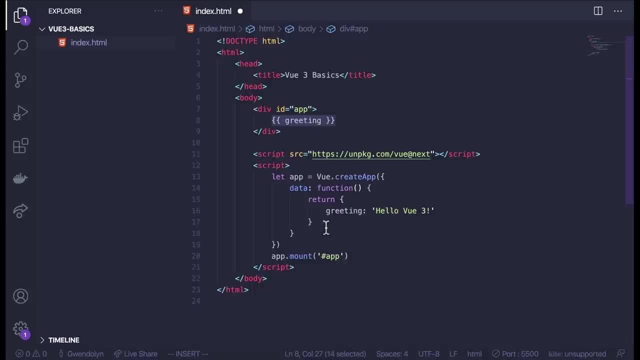 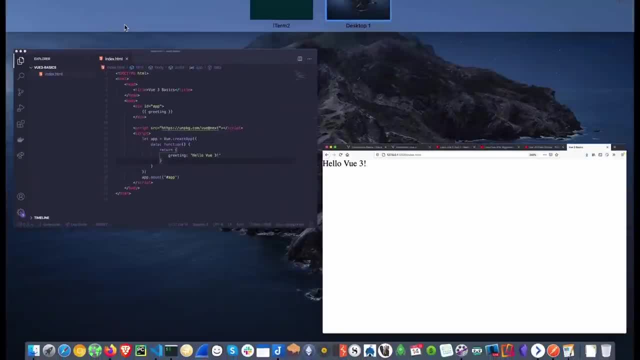 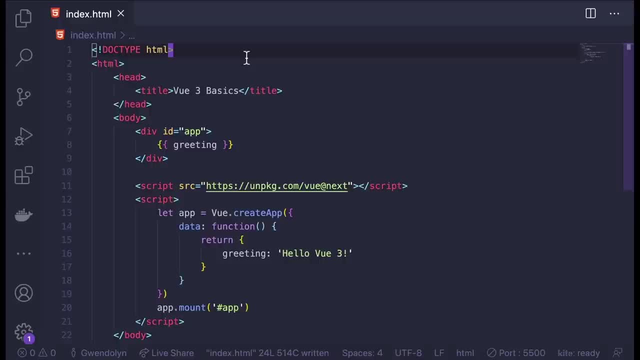 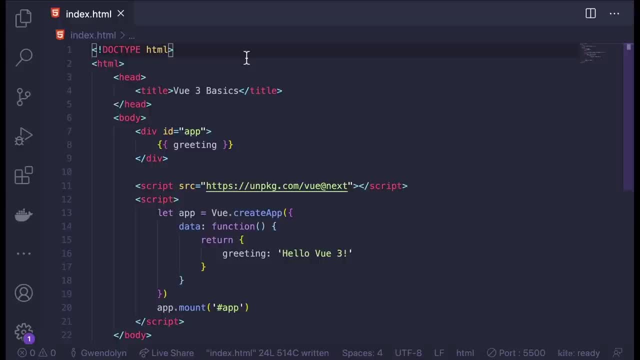 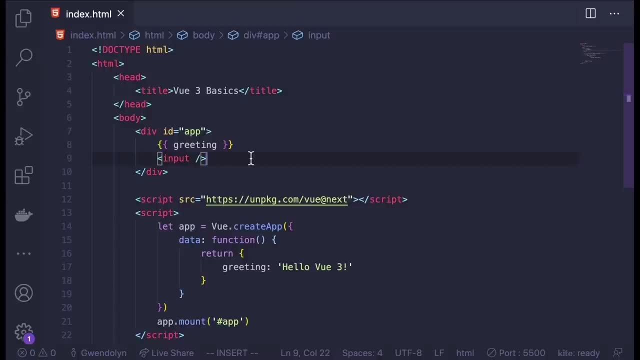 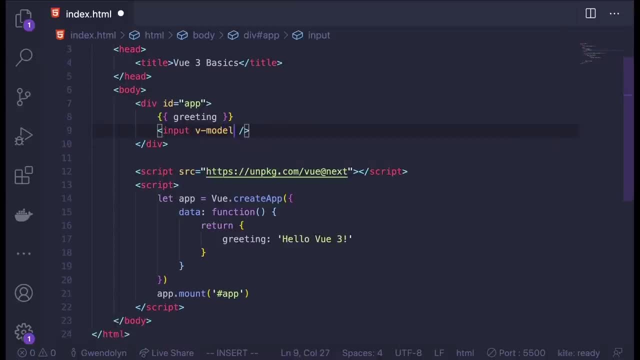 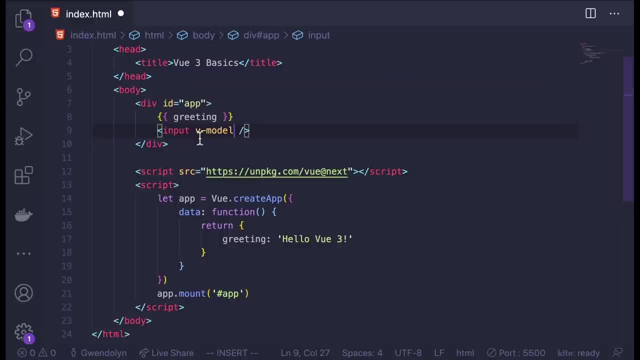 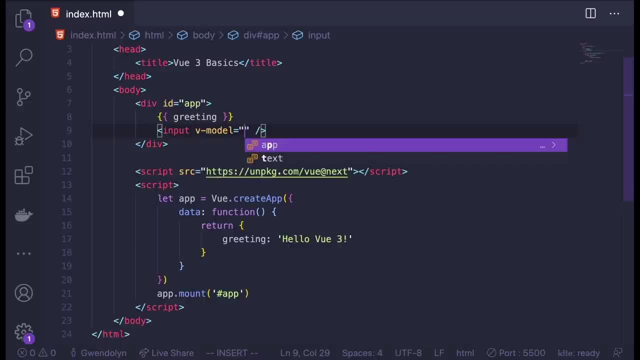 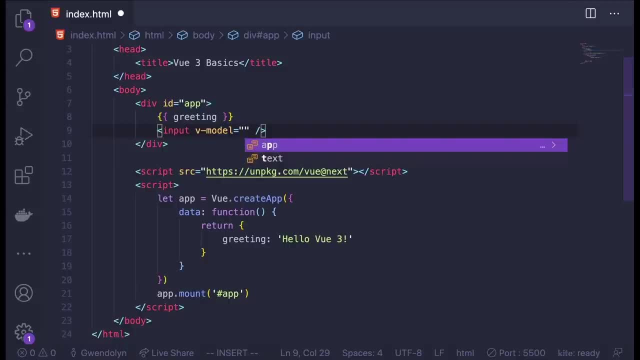 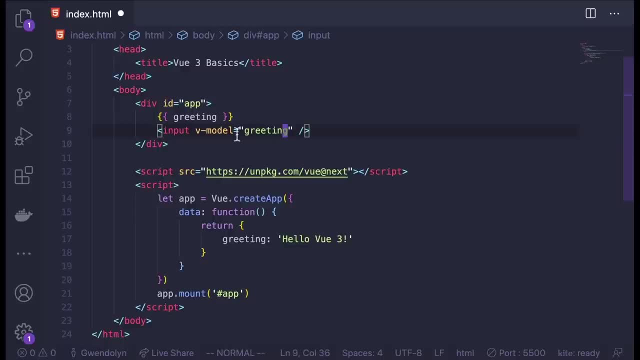 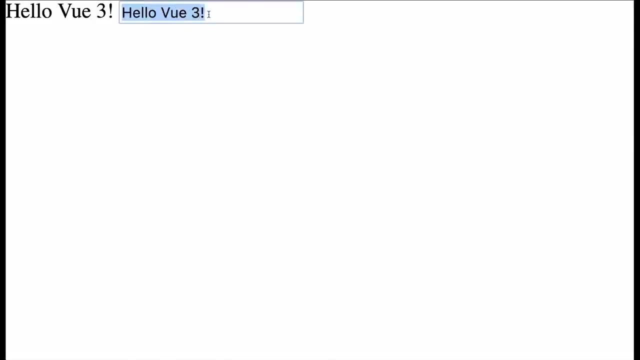 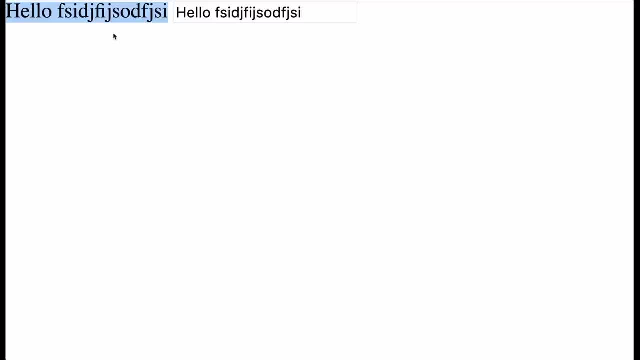 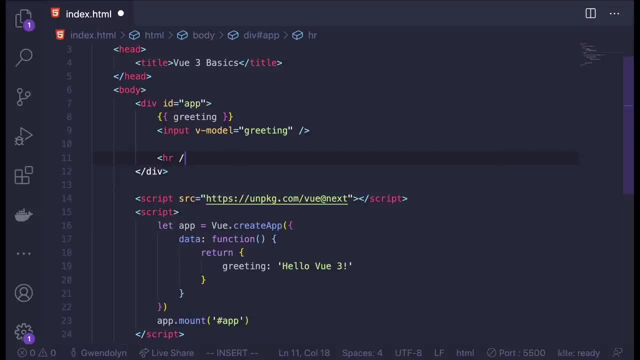 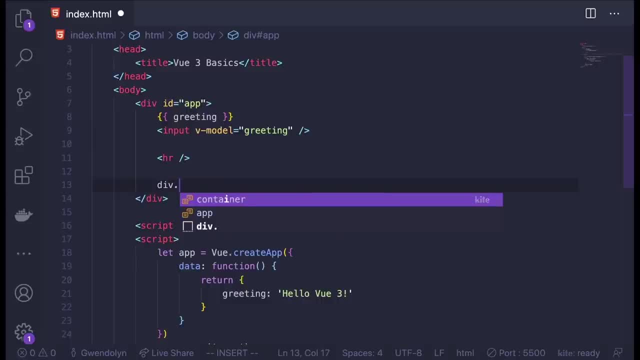 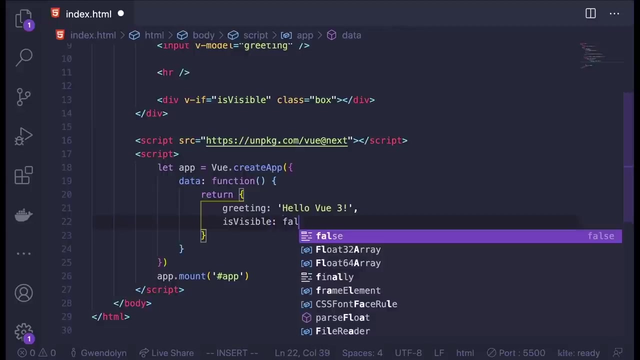 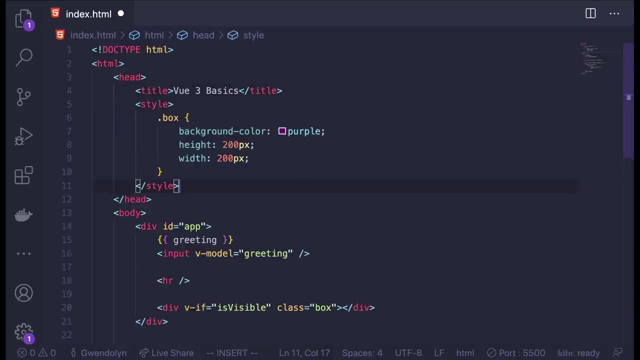 which is v3.vuejscom, So let's get started with learning Vue 3 here. so make sure you are at the correct website, which is v3.vuejscom, do is visible and set this to true. to start, I am going to paste in some styling that I made This: 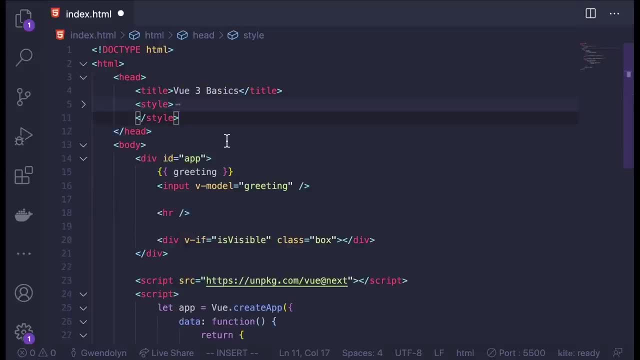 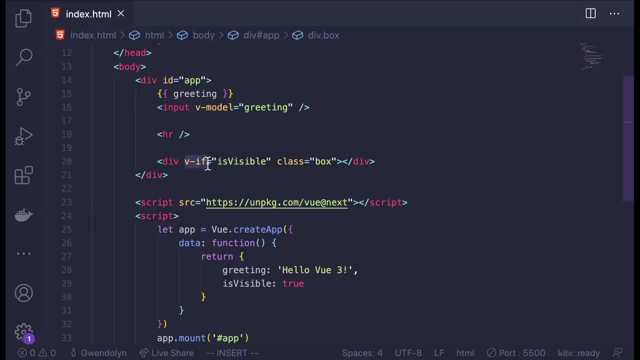 is just to style the box so you can see it on the page. I'll fold that. You can see that. I do see that box, because this V if directive is basically just like an if statement in JavaScript. So if this value is truthy, then this element will be displayed on the page, But if it's false, 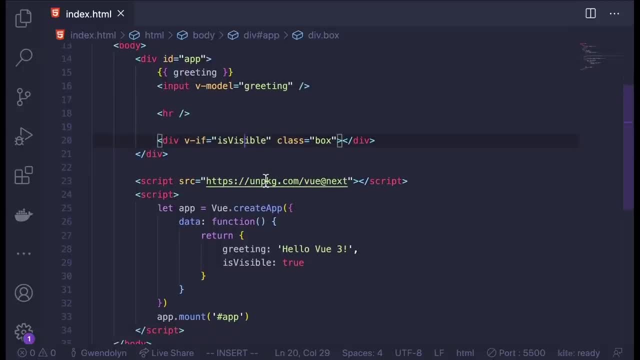 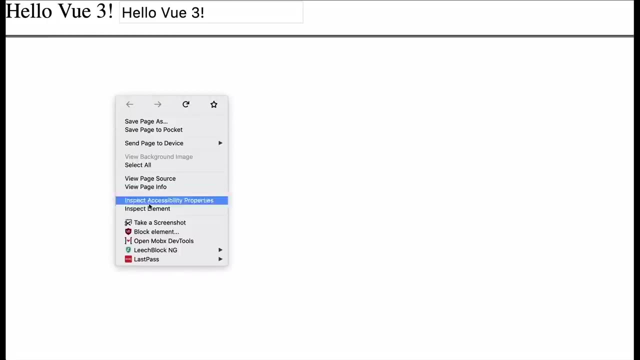 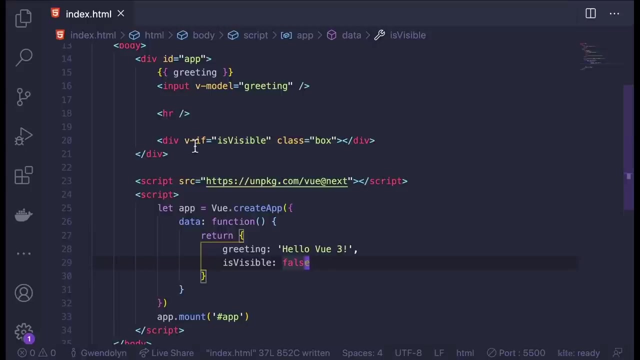 this div will not be rendered to the DOM at all. So let me change this variable to false And you can see the box disappears. And if I check, I can inspect element and there is no div found in the DOM. Now V, if is very similar to V, show. 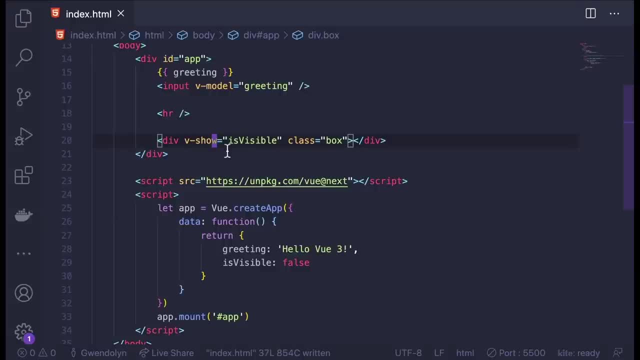 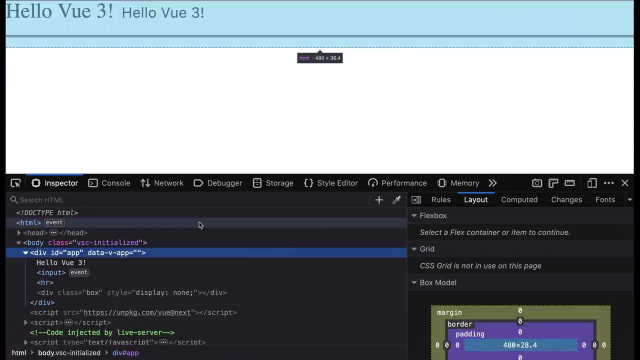 which is another Vuejs directive. It takes the same kind of argument, a Boolean expression, And let me set this to true again. You can see. if it's true, it shows on the page just like V. if, However, when it's false, you can see there's still a div rendered to the DOM, The only 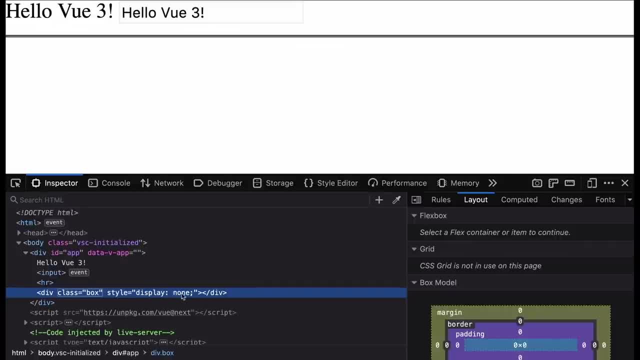 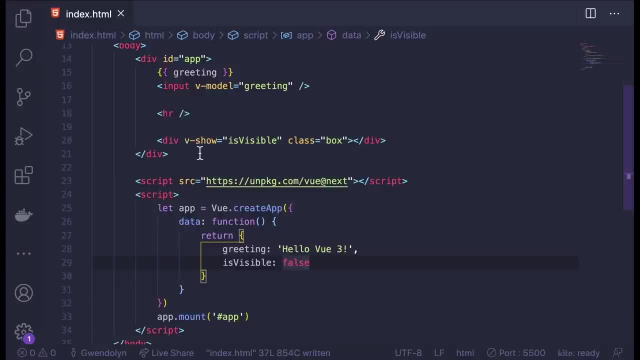 difference is the style is set to display none, So you won't actually see it, but it is there in the DOM. So when would you use V show? Well, in most cases you would just use V if, because you either want. 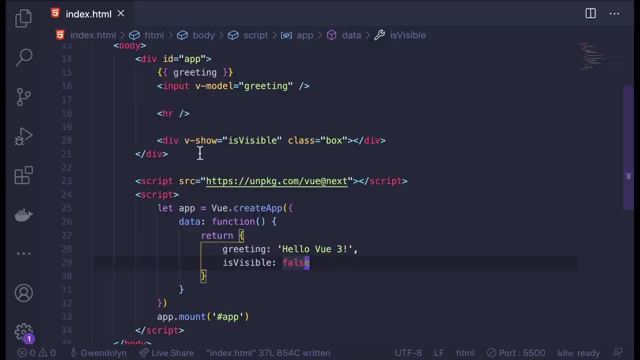 something to render or not. Like, if you have a loading spinner, you would use V if it's loading, show the spinner, And then when the page or whatever has loaded, you would set the variable to false and then V if would remove it from the DOM. Now, V show is useful for specific cases. 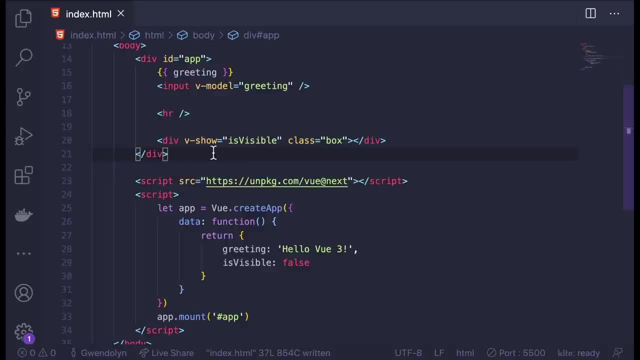 when you might need to toggle something more frequently And it would be more performant than adding and removing it to the DOM constantly. So it's already there. all you're doing is changing the CSS, So you're changing it from display none to display block, So changing this back to V. if 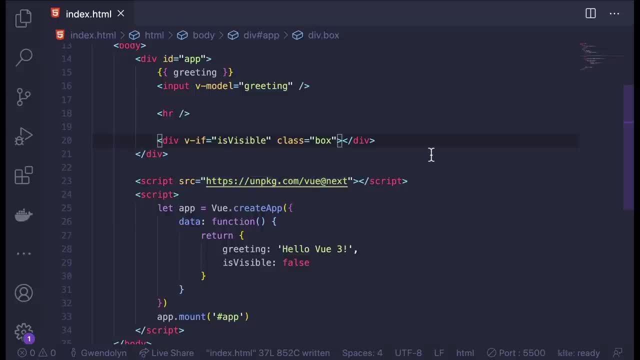 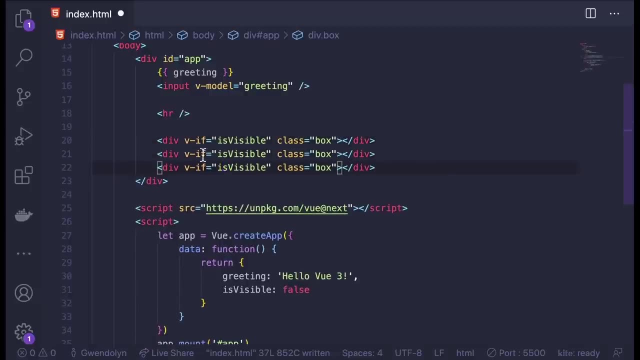 there are other directives that you can chain on to V if, there's V else if and V else, And you can already guess what these do. So I'm just going to show you the syntax here. So V else if and V else is the one that doesn't take any argument, And I'm just 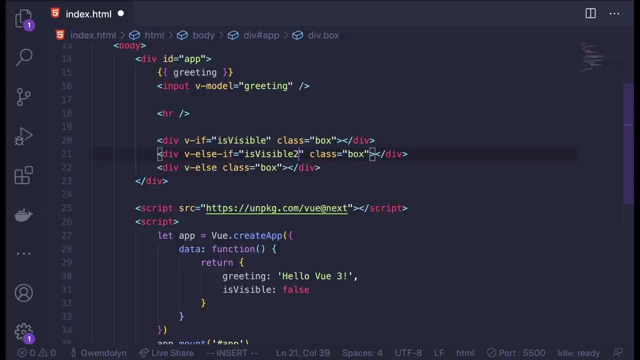 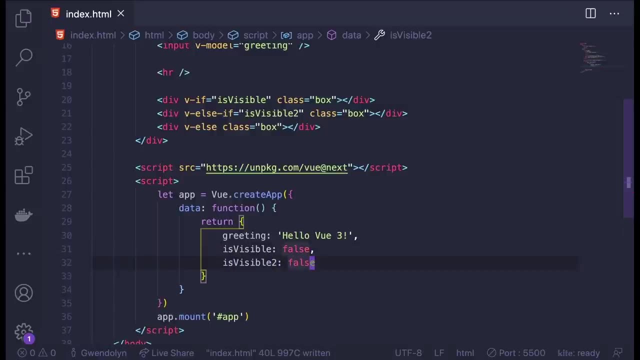 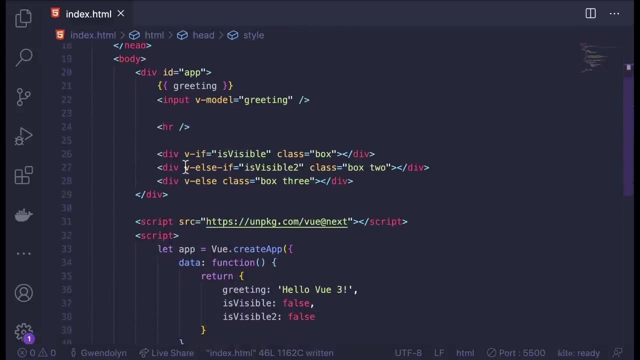 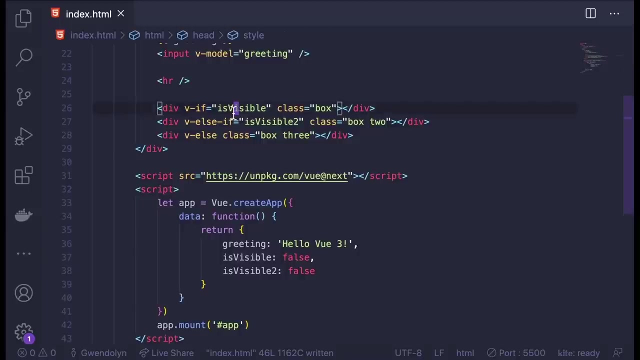 going to demonstrate these really quickly. I'll add another variable here. So is visible, is visible to. So I've added a little bit more CSS here to differentiate between the three boxes That I've created here, And this works as a regular if else statement. So if is visible is. 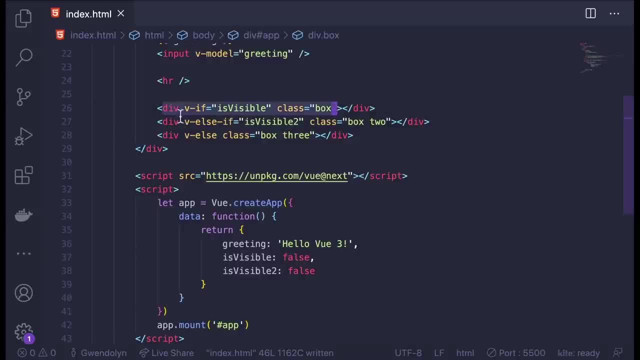 true, this div will be rendered. If it's not true, it's going to keep going down the chain. So it'll look at any V else. ifs you have here, you can have as many as you want. So then it will look at is visible to to see if that is true. If that's not true, 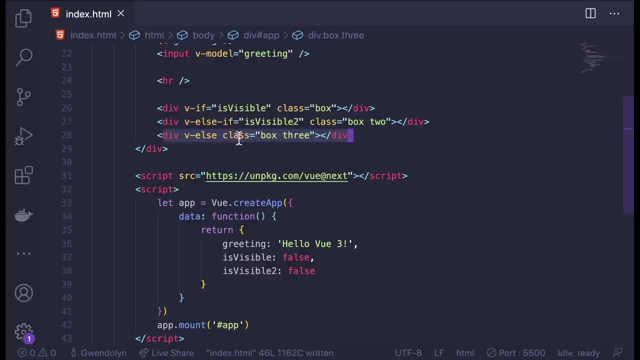 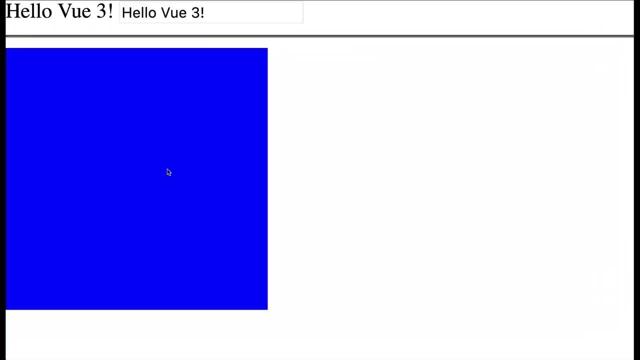 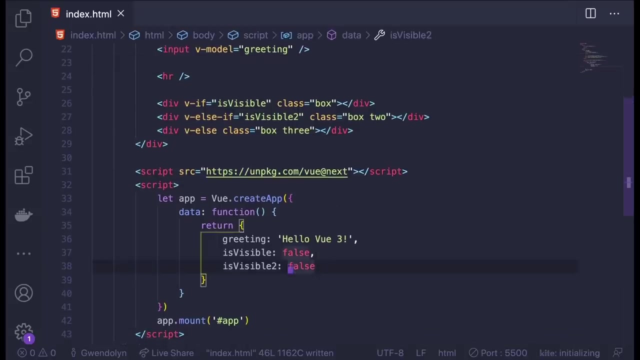 then it will automatically display this third box. Now the third box is blue, the second box is red and the first box is purple, So you can see the blue box displayed because the other two values were false. Likewise, I could change one of these variables to true. 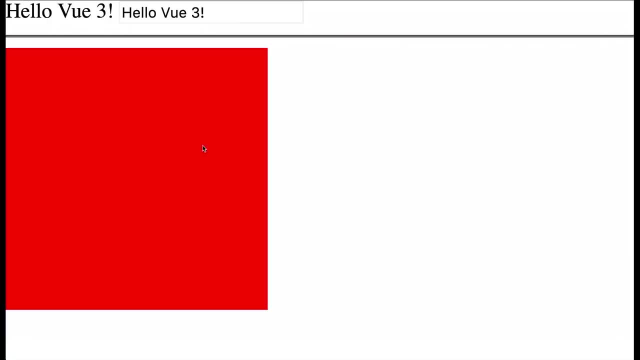 And then that box would be rendered in the DOM here. Now I want to point something out here. If I refresh the page you can see for a split second. you actually saw all of the boxes render, as well as the current box. So if I refresh the page you can see for a split second. you actually saw all of the boxes render, as well as the current box. But if I refresh the page you can see for a split second you actually saw all of the boxes render, okay. so now that we're done, we're going to disassemble. Let's go back to our slide. So I'm going to access the view editor And it's going to show up on the screen here. 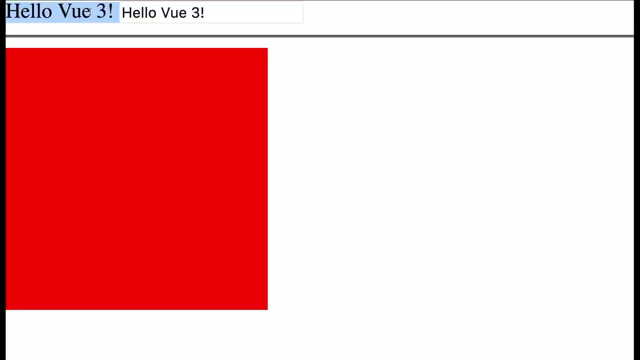 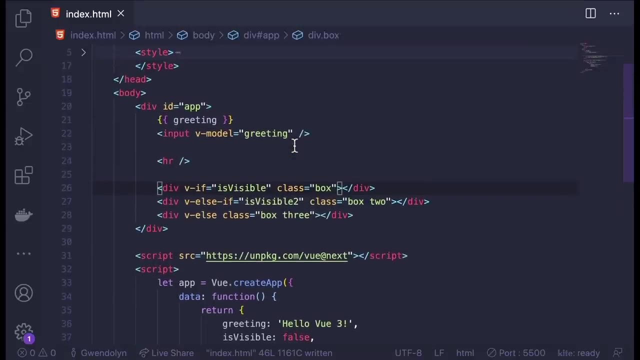 before it was parsed as a view variable. I'm going to refresh the page again and slow it down a little bit, just in case you couldn't see that. So how do I prevent that from happening? view has something called V cloak, which is a convenient utility that will hide anything. 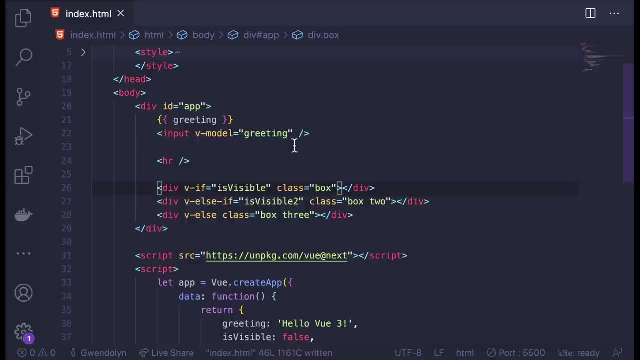 from rendering until the whole view application is ready. So I'm going to add a v cloak. you can see that that will hide anything from rendering until the whole view application is ready. So I'm going to add a V cloak here And then I'm just going to do the same thing. So I'm going to save this up here. 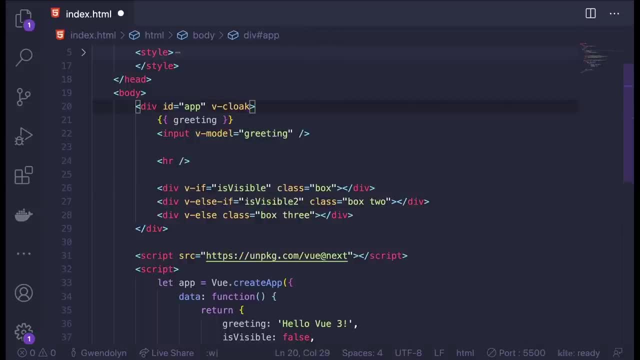 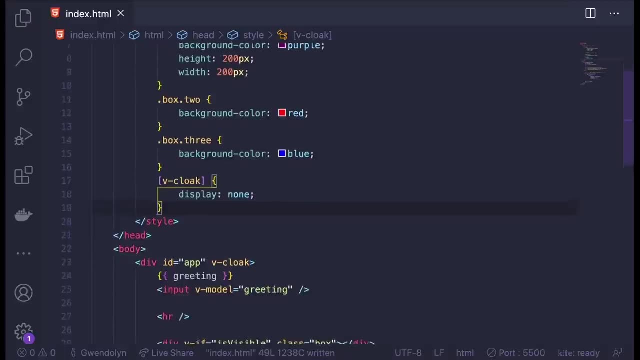 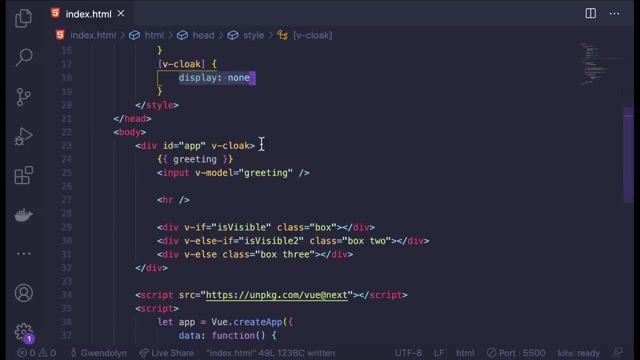 So I'm going to add a vCloak here and then I basically need to add a style for it. So you can see I'm setting vCloak or this vCloak attribute to display none. This is the recommended pattern in Vuejs. 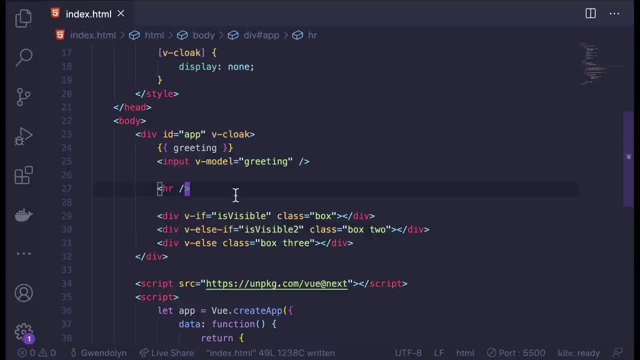 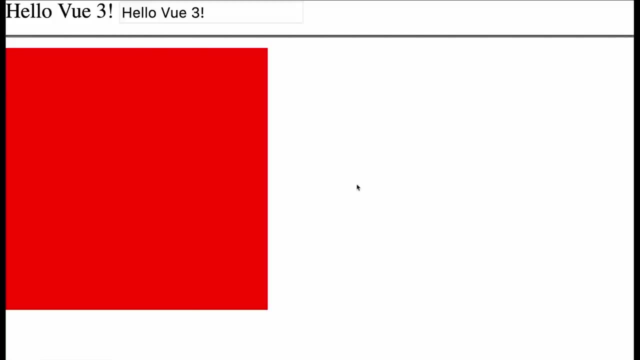 And then I just add a vCloak to my div with my app in it. Now, if I go back here and refresh, you no longer see the curly braces or the other boxes render. How does that happen? I'm going to go to inspect element. 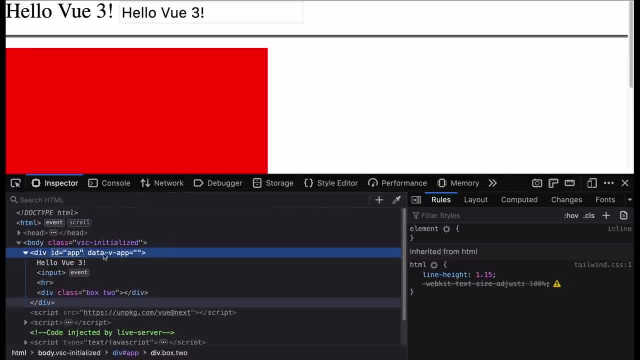 And you can see on the div with ID app here there is no vCloak attribute. But if I refresh the page you can't really see it because it's too fast. But basically that vCloak attribute remains on this div until the app is loaded. 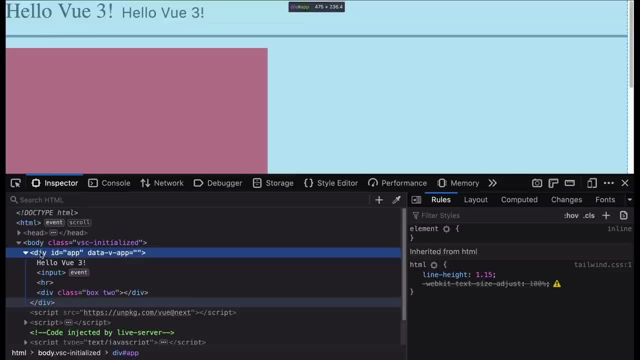 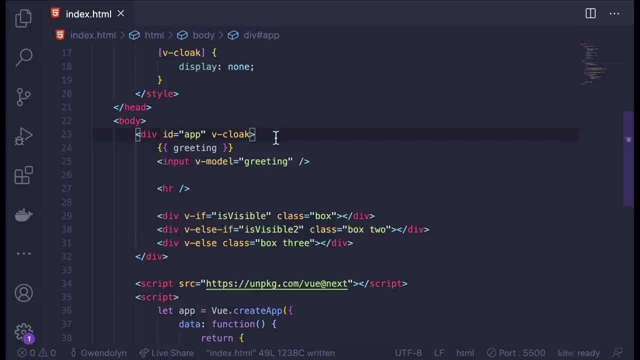 And then it's removed once everything is rendered to the DOM. I don't often run into cases where I have to manually use this, But it is a nice feature to know about if you run into that issue. These were just a few basic directives. 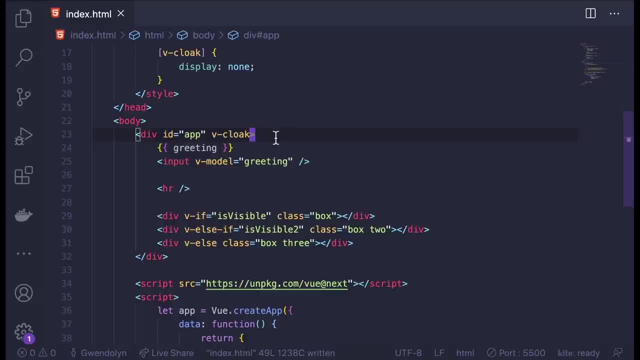 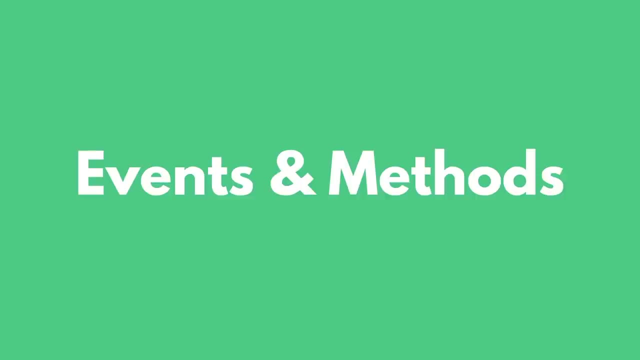 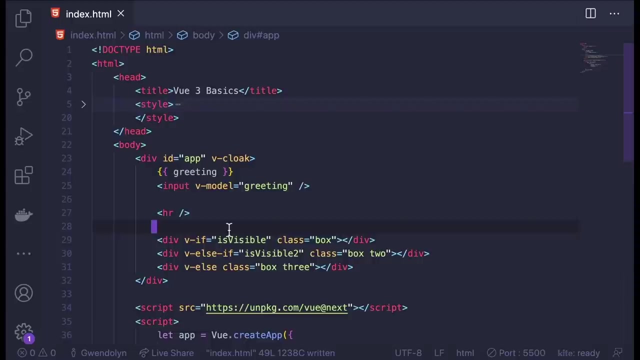 We will definitely be covering more directives as we go along in this course. In the next video, we will go over events and methods in Vuejs. Now that you've seen how to use variables and directives in Vuejs, let's make this code a little bit more interactive with events. 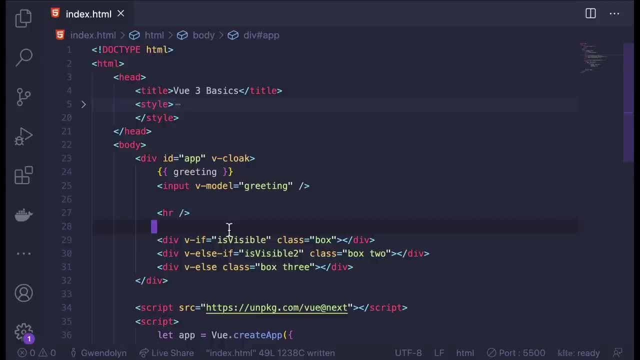 So you can see that I've added a vCloak here. You probably already know that there are many events that can be captured in the browser and used in our applications, For example, when the user clicks on an element on the screen like a button, or if the user 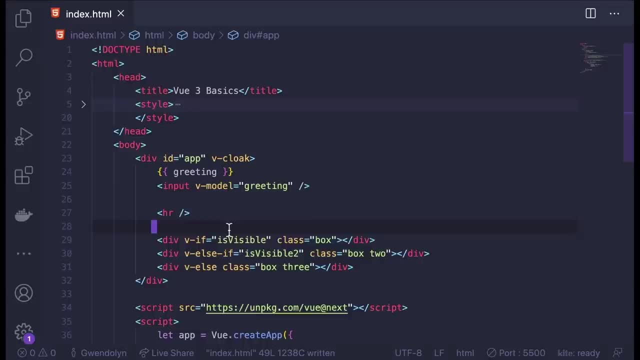 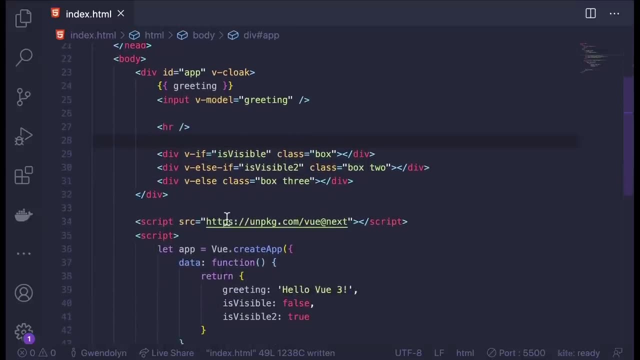 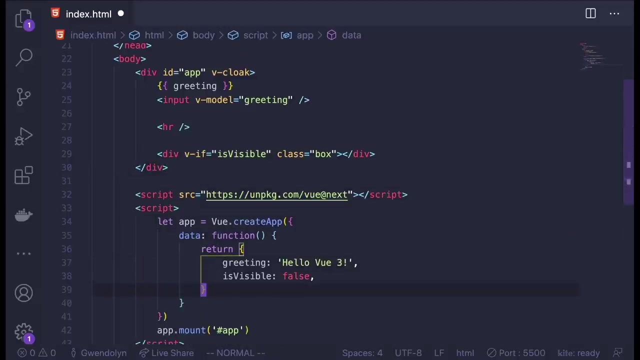 presses a certain key on the keyboard, like enter, to submit a form. Let's try out both of these cases in our little mini application here. First, going to get rid of the two extra boxes And I'm going to add a button here which, for right now, I will label as showbox. 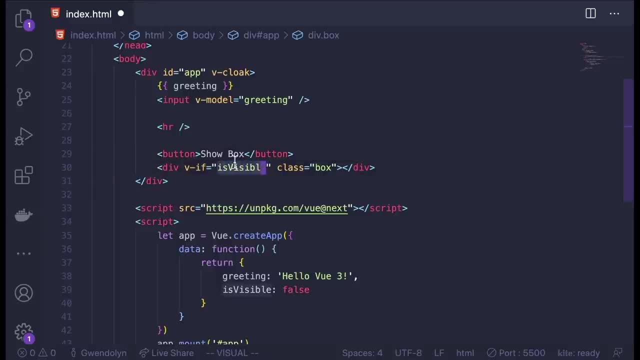 So right now this vif is set to false or the variable is visible is set to false, So this div will never be rendered on the page unless we somehow update that variable. Before we were hardcoding the variable value Here as true or false, but we can actually use this button to change the variable value. 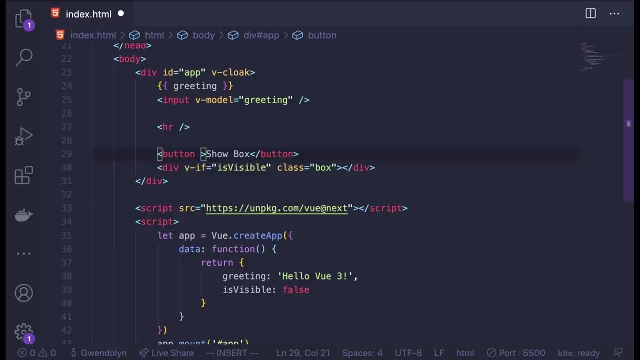 as well, And this is done with another directive called V dash on. Now, the V dash on directive is specific for events. you can use it for custom events that you create yourself, Or you can use it for any of the standard browser events, like, as I mentioned before. 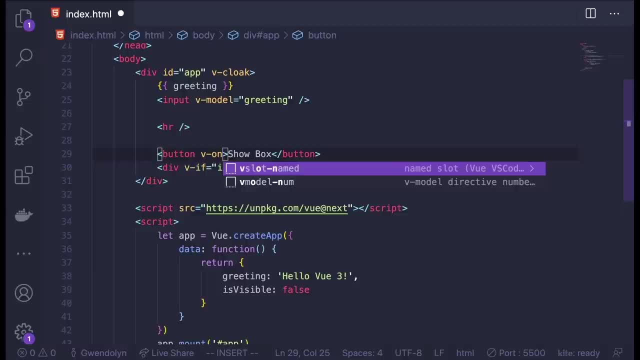 when a user clicks or presses a key on their keyboard And that's it. So here specifically, I'm going to do V on colon and then the type of event, which will be a click event. So I'm listening for a click event on this button right now. 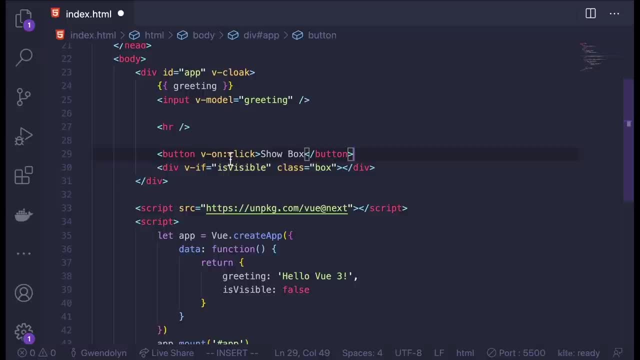 But now, when someone clicks on the button, I have to tell Vue what to do with that click event. So I need to pass in an argument of whatever JavaScript I want to run when this button is clicked. And for right now I will keep it simple. 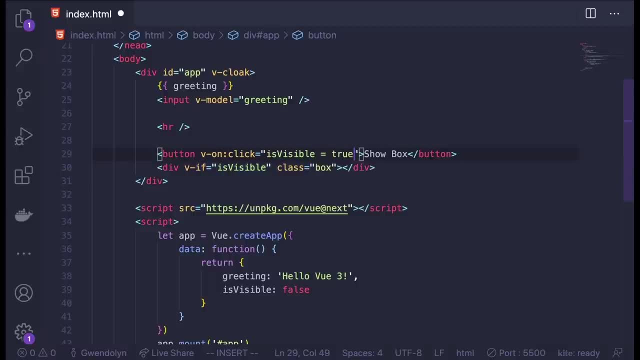 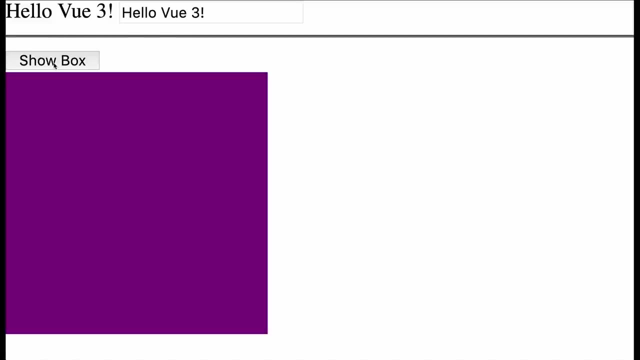 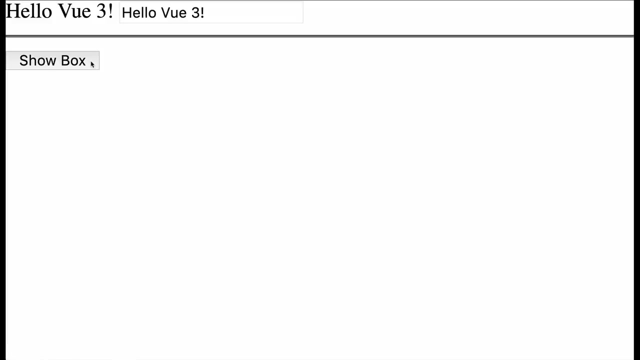 And I'm going to set the is visible variable variable to true When that button is clicked. Now you can see I have this button show box. When it's clicked, the box shows. What if I want to hide the box? right now this only shows the box. 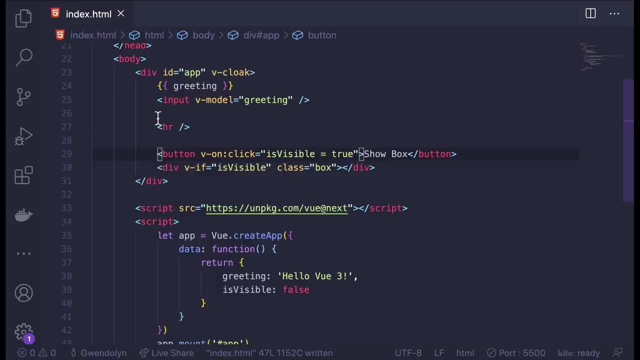 And the only way to get rid of it is by refreshing. I can set up a toggle for the box by simply saying: is visible equals the opposite of whatever it currently is. So is visible equals, not is visible. So if it's true, it will be set to false. if it's false, it will be set to true. 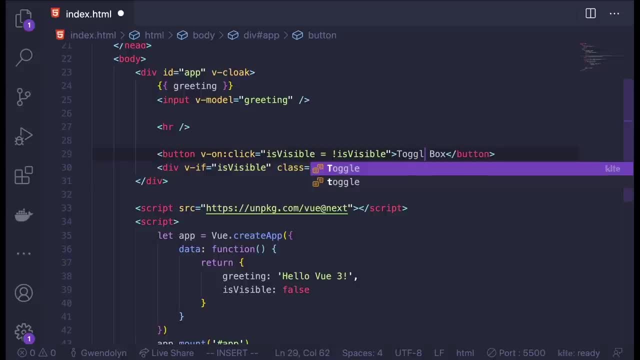 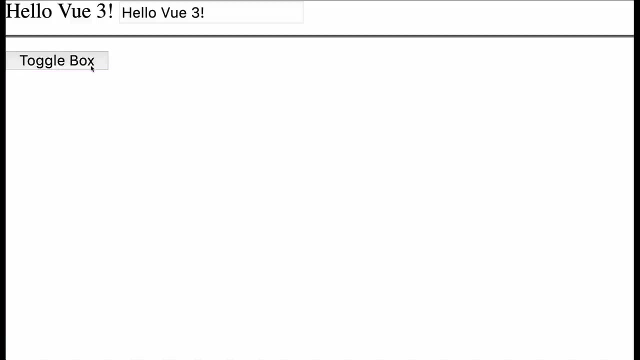 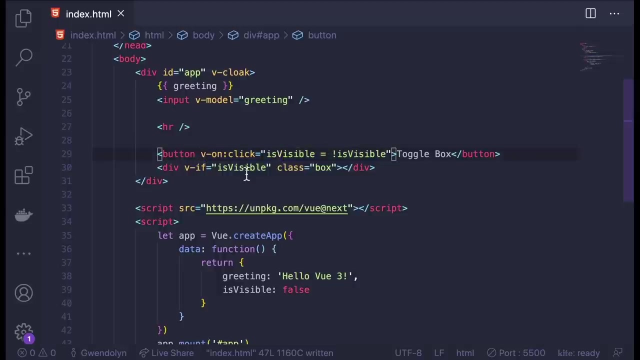 And this should toggle our box. I'll relabel this to toggle box. And now, if I keep clicking toggles on and off, that is basically how events work. There's also a shorthand for creating events, So you don't have to type out V dash on colon, you can just type the app. 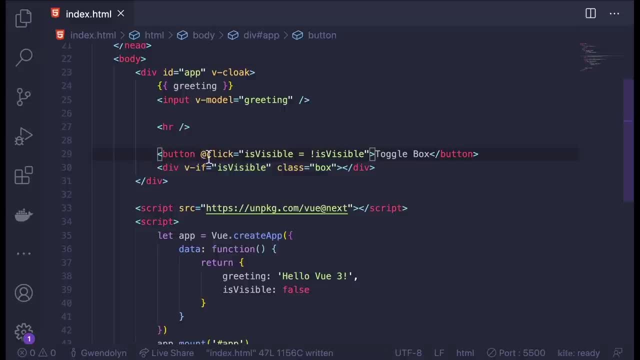 The app symbol and then the event name. And this is exactly the same thing as it was when I typed V dash on colon: the symbol just replaces all of that. So what if you wanted to do something more complex in here, not just setting a variable? 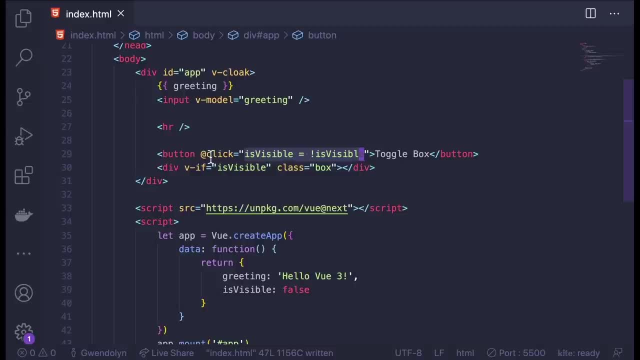 to true or false. Well, you can actually use this to pass in any kind of method on your VJS object. So I'm going to get rid of is visible here And I'm going to create a method. It's called toggle box. 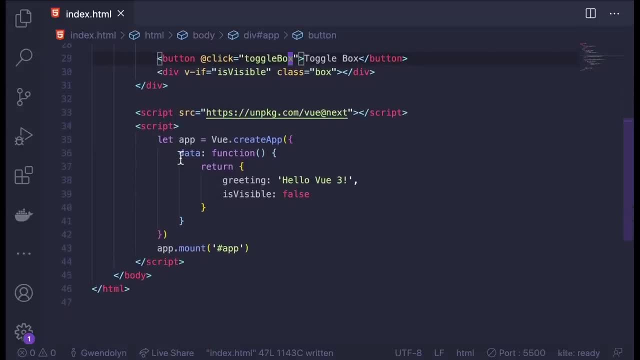 And now I have to create this toggle box method. You can see, I already have data on my VJS object, this data function. But now I need to make another key, which is called methods, And methods is an object of functions. I can put as many functions as I want on this methods. 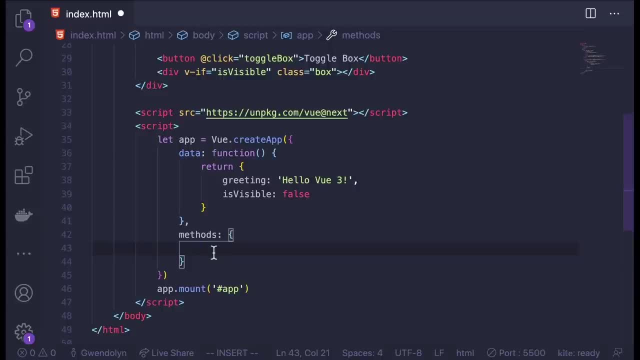 object to be able to use these in my VJS application. So let me create that toggle box function. I could do the same thing here as I did above, but I'm just going to use the function shorthand And I want the same logic again, but inside this function. 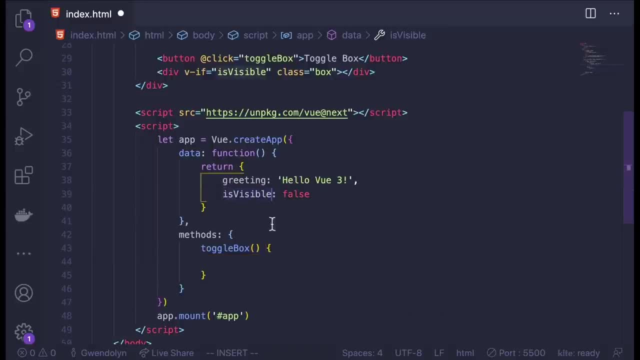 So in order to refer to this is visible variable here, I have to get it off of the this context and VJS handles putting all of my methods and variables on the this context So that they're available to me anywhere in my view application. 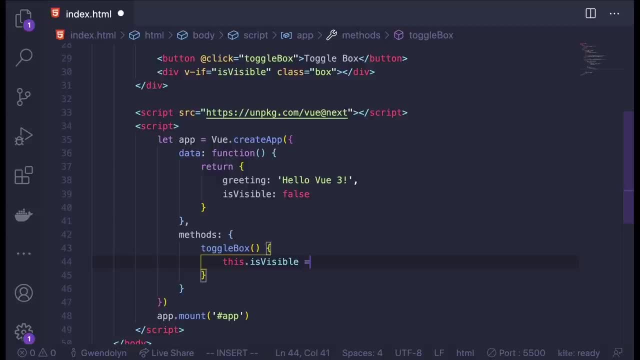 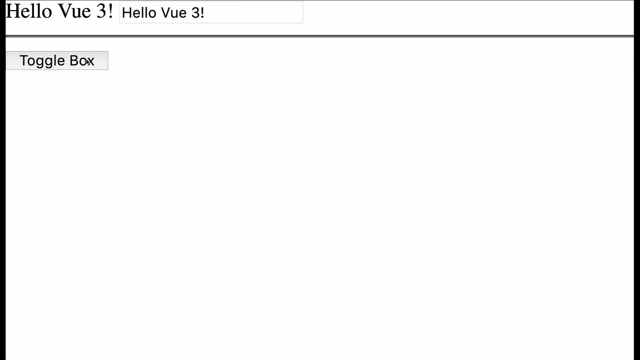 So I can do this dot is visible and then set it equal to not. this dot is visible. This is not a function there- And this should work the same way as it did before, So I can test it out and toggle the box once again. 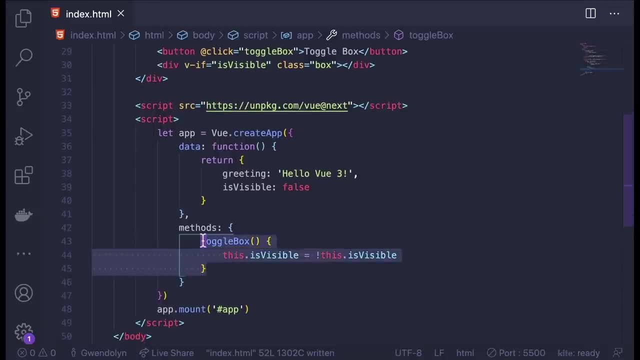 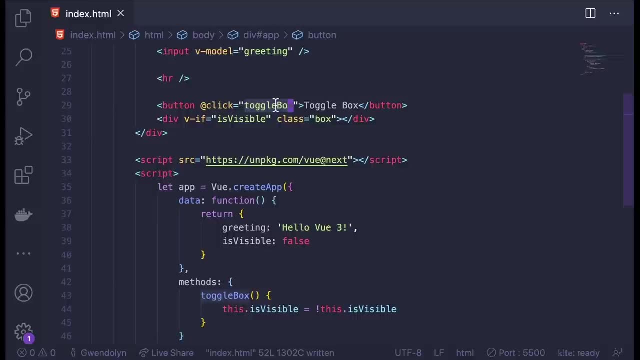 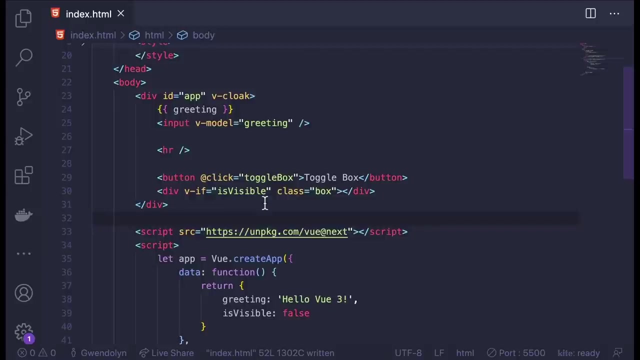 So that is the basics of how methods work, And you can see, because I have called my methods Toggle box, that it is also available to me anywhere inside my VJS template here. So let's look at one more type of event, And that will be an event listening for keyboard input. 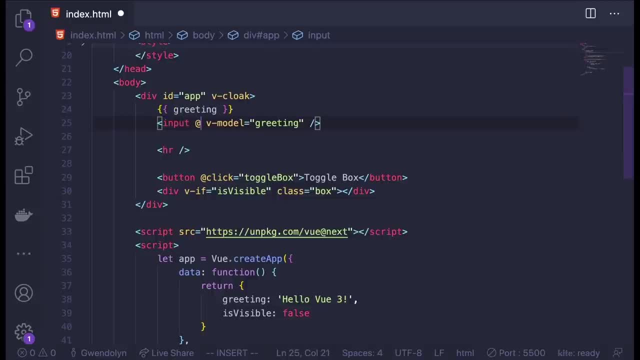 So here I want to listen for key presses. This is also an event, So I'm going to start with the at symbol and listen for a key up event. I could also use key down if I wanted to. So for keyboard events I need to add a modifier. 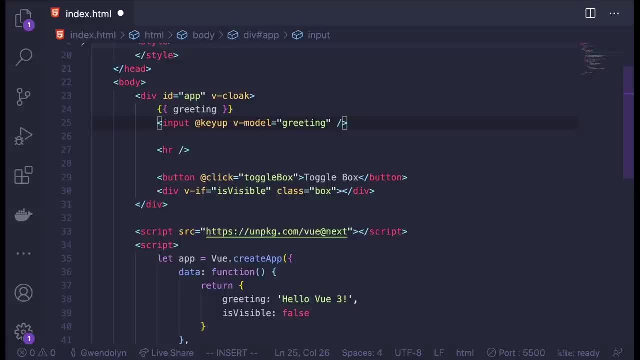 To say which keyboard input I am listening for. So for input here, I want to run a function or some JavaScript whenever I press the Enter key. So for enter, I actually have a shorthand because this is a common keyboard input. So I can say: listen for the key up event specifically with the Enter key. 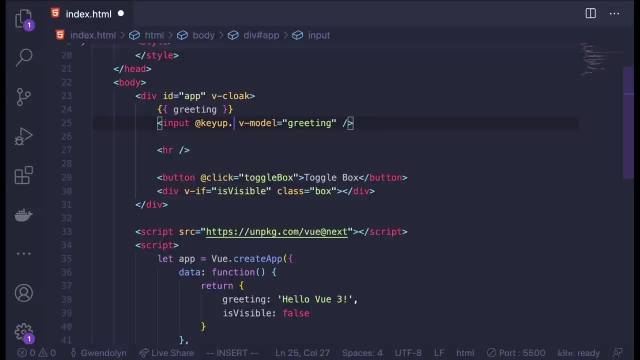 Or I can always use the key code associated with any key on the keyboard. So for enter that would be 13.. It doesn't matter, It doesn't matter which one I use. I'm just going to go ahead and use key up dot enter, because it's a bit more obvious. 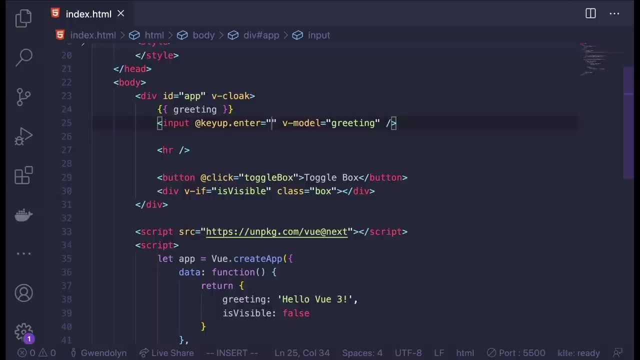 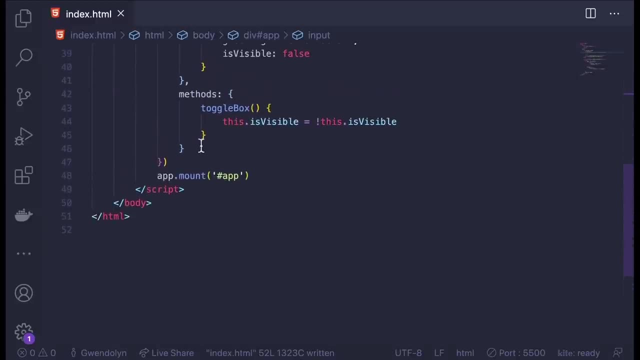 what it is. And then it's the same syntax here And I'm going to create a greet method for this key up event. So let me go down to my methods: create a method called greet, Use the method shorthand, And I'm actually just going to console dot log. 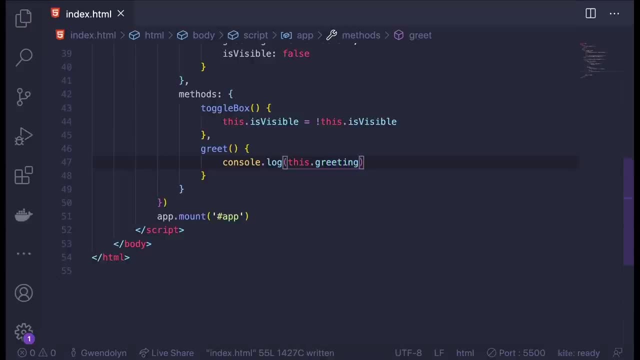 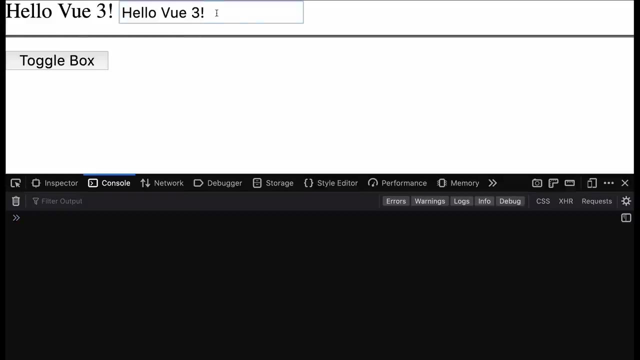 This dot Greeting And let's see how that works. So I can just focus this input anywhere and just hit enter. It doesn't matter what's already in the input And you can see. it logs out the greeting. If I change the input, it logs out whatever the greeting variable is currently set to. 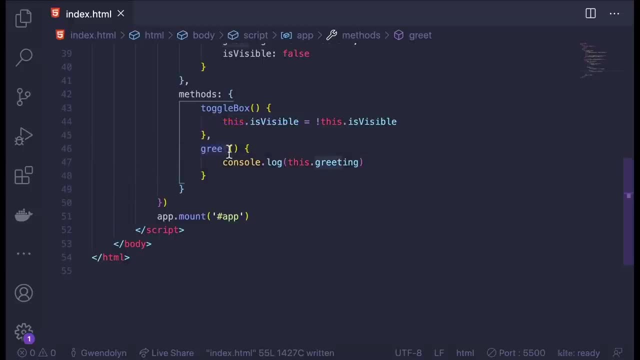 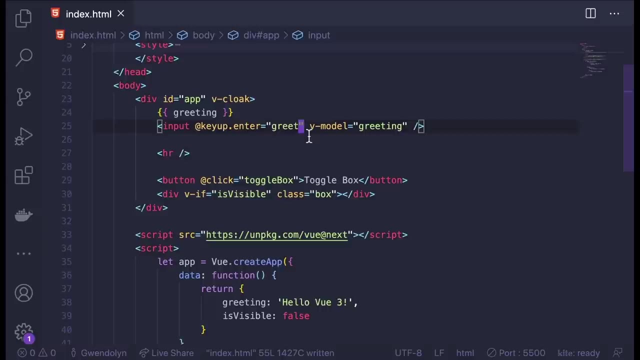 Now what if I want to pass something into a function, as I'm calling it into one of these methods, Then I could do that Just by Adding the parentheses to call the function. So for example: greet. here I can just pass something in. 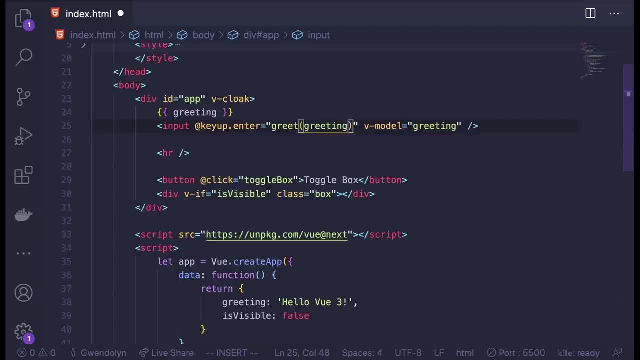 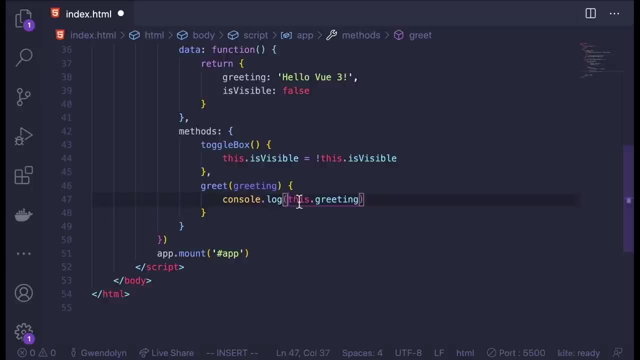 So, just for demonstration purposes, I'm going to pass in the greeting through the template here, I'm going to accept that here and I'll still call it greeting and then get rid of this, because I'm no longer looking for the greeting variable on the VJS instance here. 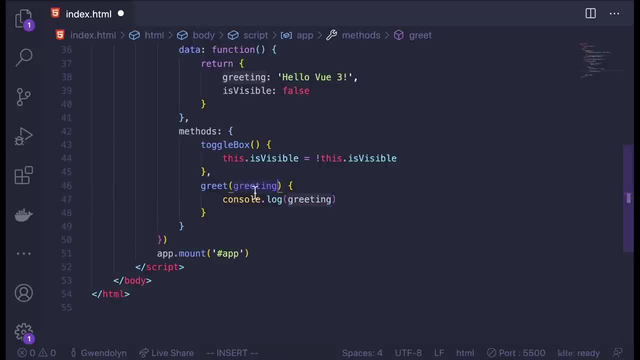 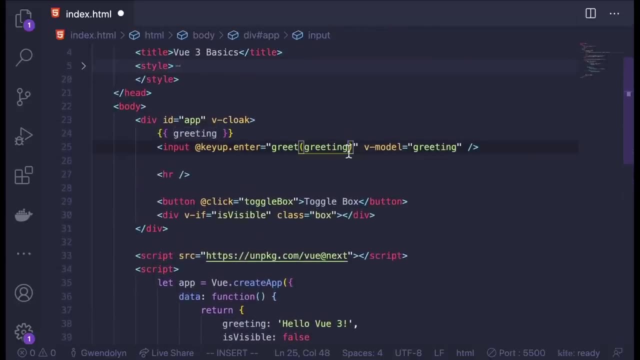 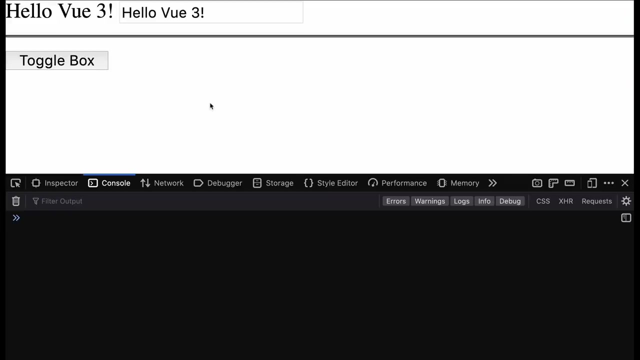 I am actually just going to be using the greeting variable that I am Passing in here And just to show you that it's different, I can use the greeting variable and then pass it in with some exclamation points appended to it, And now when I go here and I click enter again, you can see that it is the greeting variable. 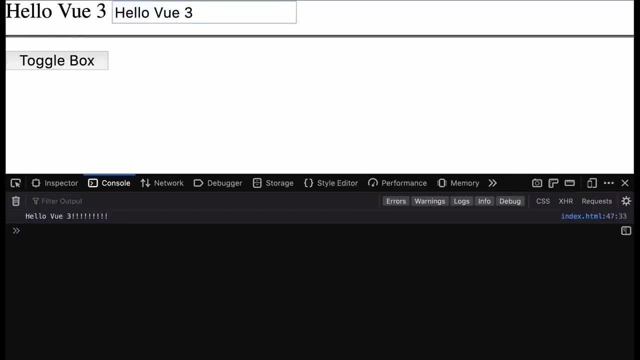 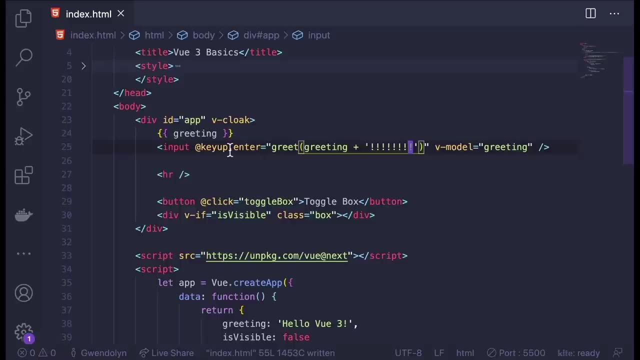 that I passed in through the template. If I erase a few characters here, hit enter again, You can see It's the same variable set to the new value. Those are the basics of how to use events and methods in VJS. I do want to point out here: you see this dot enter. that is an event modifier in VJS. 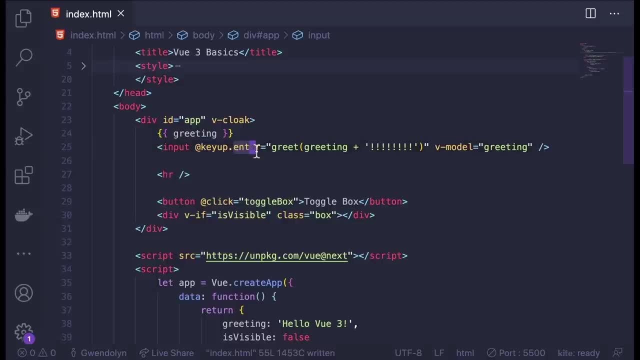 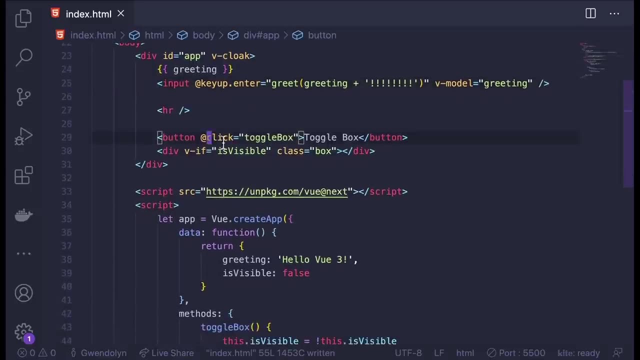 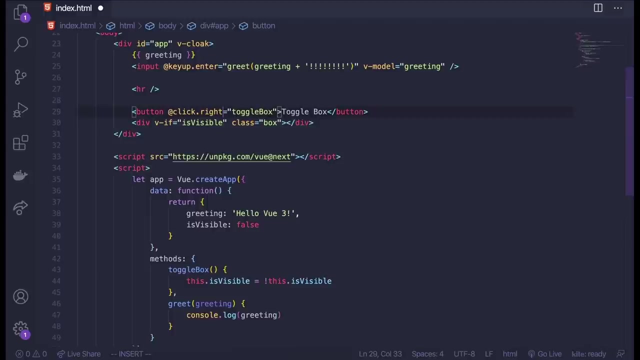 So you're not only listening to the key up event, you're listening to specifically the enter key. Now there are many modifiers that you can use, For example, at this click event here. for example, I could add a modifier here that says I'm only listening for right clicks. 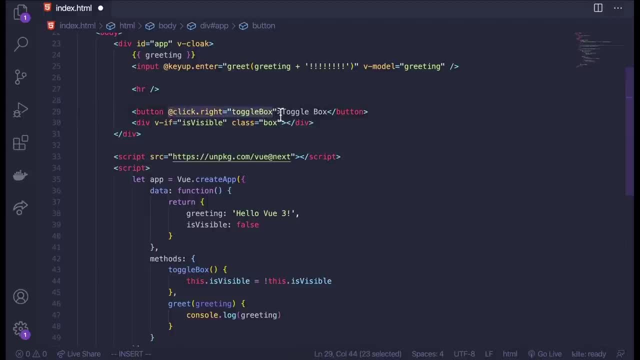 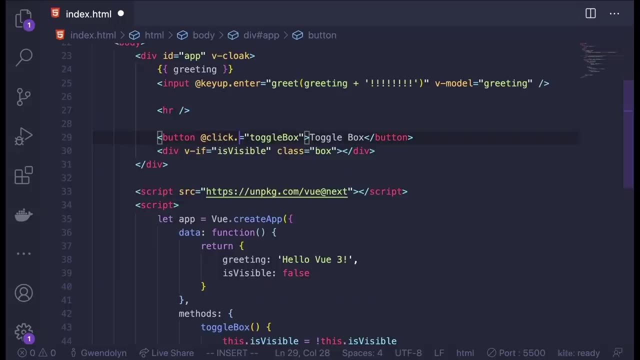 So a normal left click on a mouse will not trigger this toggle box, but only if you make a right click. I can also use some handy modifiers like prevent. So if I don't want a form to submit instead of using the regular event dot, prevent default. 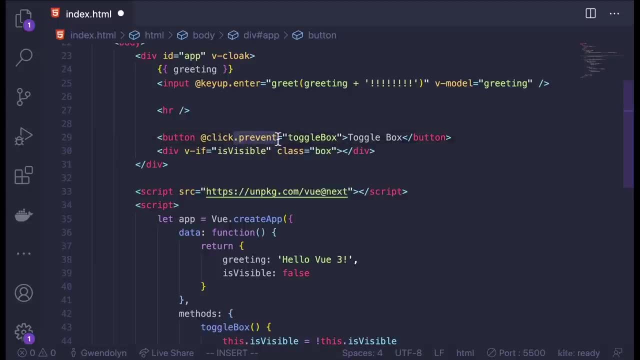 in my method. I can just add this modifier here, dot prevent, and I can do that for stop propagation as well, So I could addstop. You can chain as many of these modifiers as you want in VJS. They're definitely a handy thing to know about when you're building Vue applications. 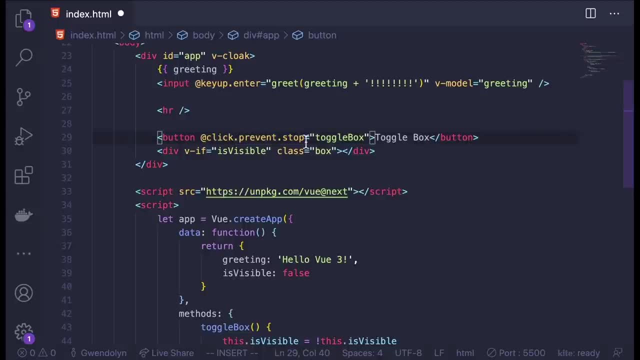 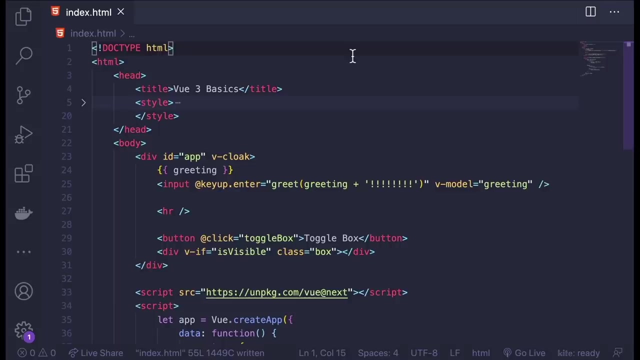 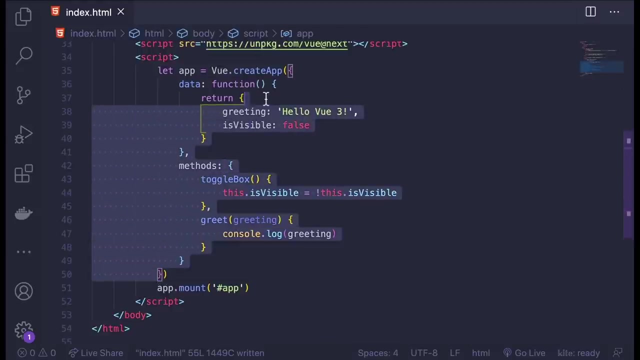 That's all for this video. We will be diving deeper into events and methods later on in this course and in future courses. In the next video, we're going to talk about custom components in VJS. Let's talk about Vue components Now. when we created our Vue application here we are basically just using one standard component. 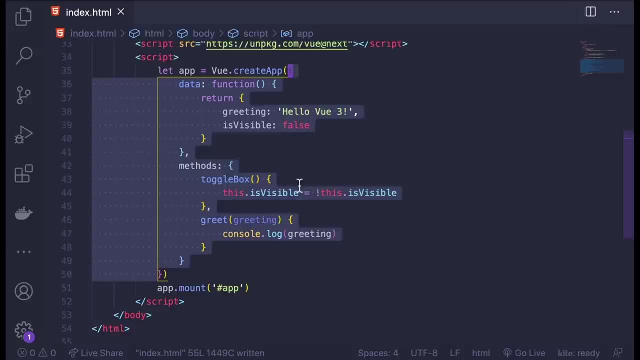 you could call it just a default options object for use in our template. So now we're going to work on breaking up parts of our application into separate components in order to prepare for learning how to build larger applications and work on applications with the Vue CLI outside of a single HTML file. 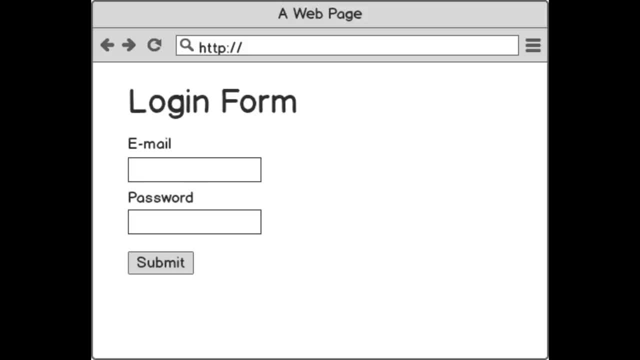 So let's get started. All right, Let's take a break from the code for a second and take a look at what we are going to be building with Vue components. We're going to use a simple example of a form to work on breaking up an application into. 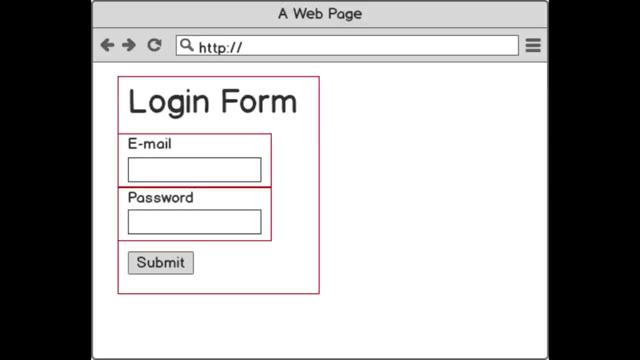 separate components. Now where you see the red outline, those are each going to be a separate component. So the outer red outline around the whole login form will be its own login form And then each input with its label will be a custom input component that we are going. 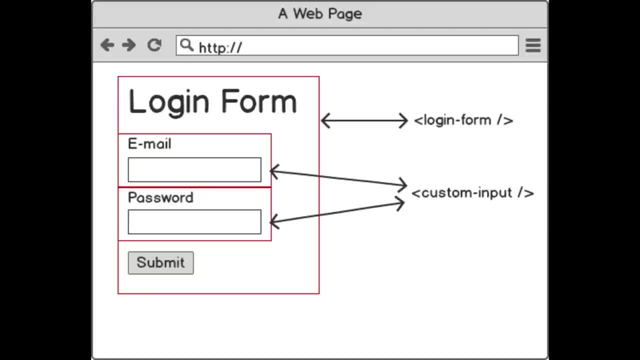 to create and be able to reuse for as many inputs as we have. So we're going to start off with this outer component and then break out the inner components into their own components after that, And then we are going to look at how you can pass data around between components in your 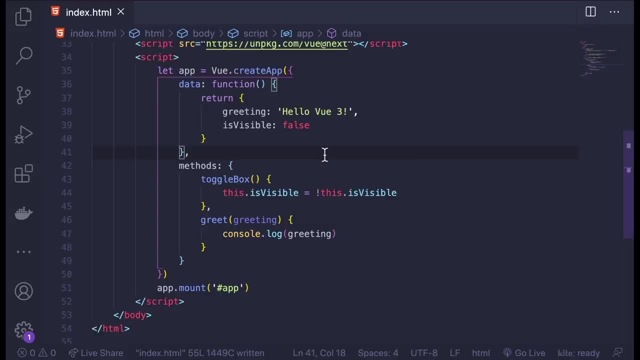 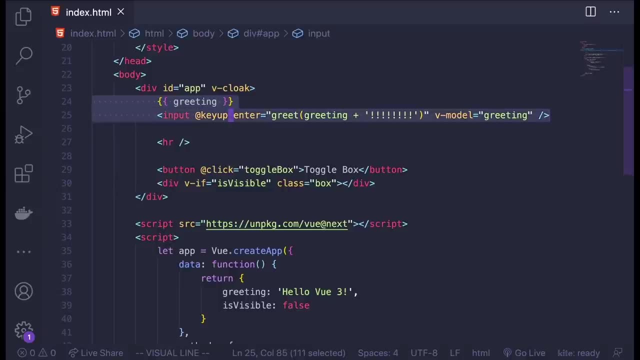 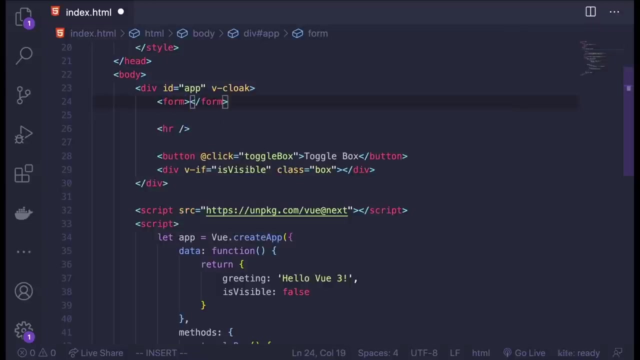 application. So what would a Vue component look like? Let's say we wanted to have a form in here- and I'm going to get rid of this greeting really quick and put a form here. So I could do this directly in the HTML and create a form tag, or I can create a custom. 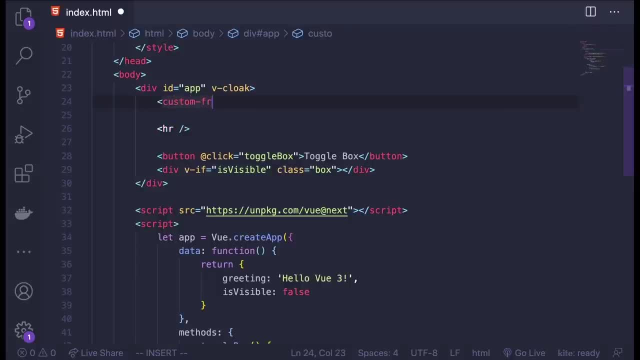 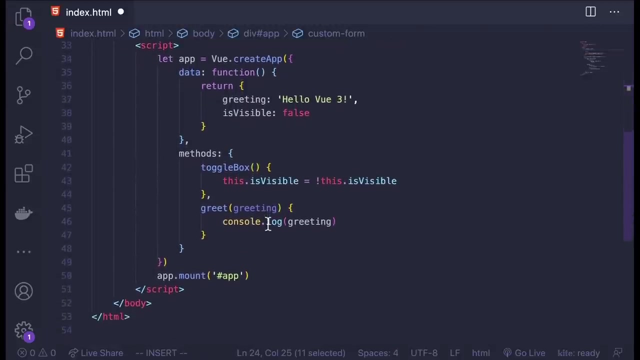 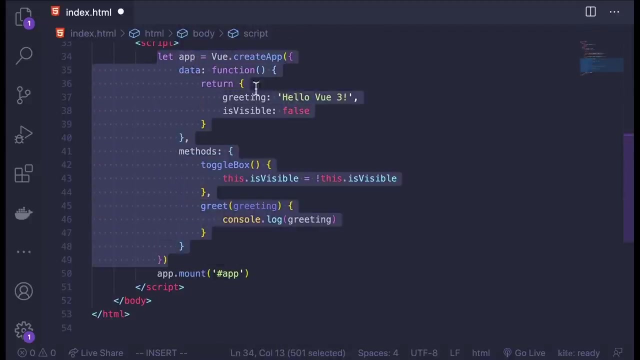 tag as a Vue component called custom form. Now this is the same syntax As if it were an HTML tag, except of course it is not a standard HTML tag. So I have to define it as a Vue component down here And I need to define it after I define my app variable, which is my Vue instance, and 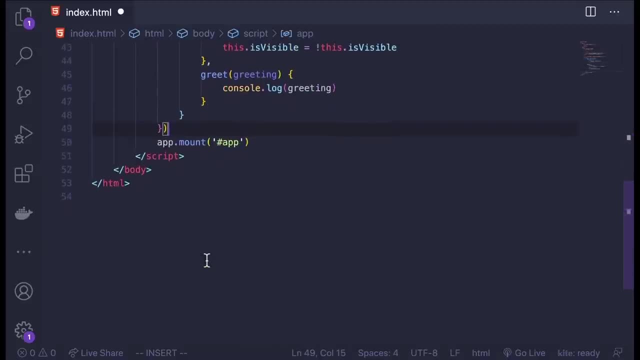 before I actually mount it to the DOM, So I can chain this here as appcomponent. This is a function And it takes two arguments. It takes two arguments here that I'm going to pass in. So the first one is the name of the component that I'm going to use. 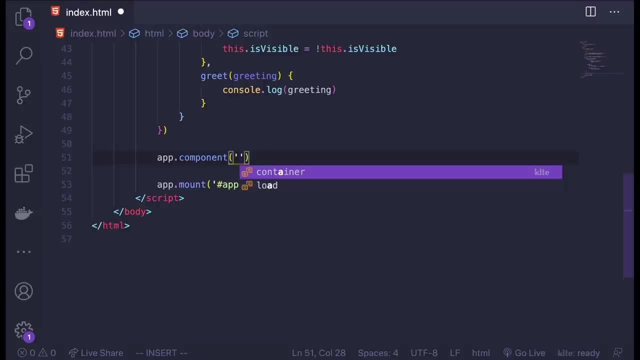 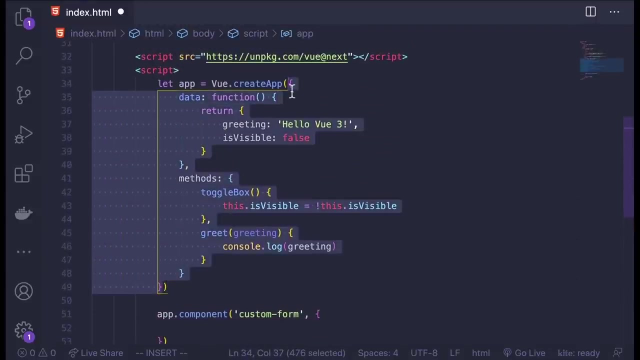 And that is the name that I'm going to be using in my HTML up there, So I'll give it the same name: custom form. And the second is an options object, And since this is its own self-contained component, I can actually use any of the same options. 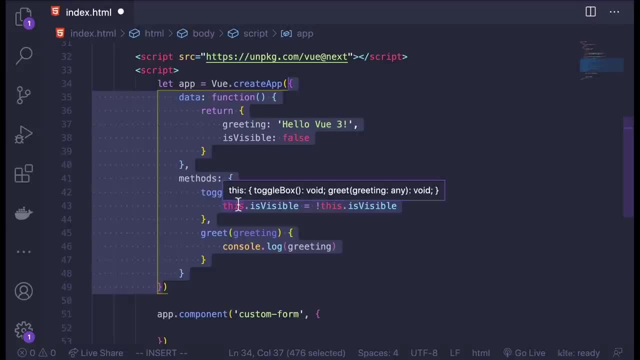 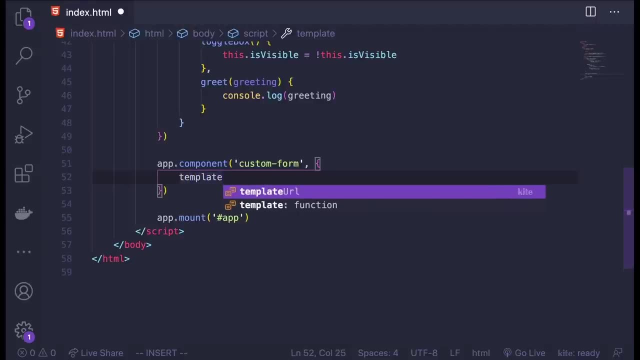 that I've been using here, such as data and methods, et cetera. The only extra thing that I need right now is I have to define a template for this component, And the easiest way to define a template is by using Graves, so I can make this multi-line. 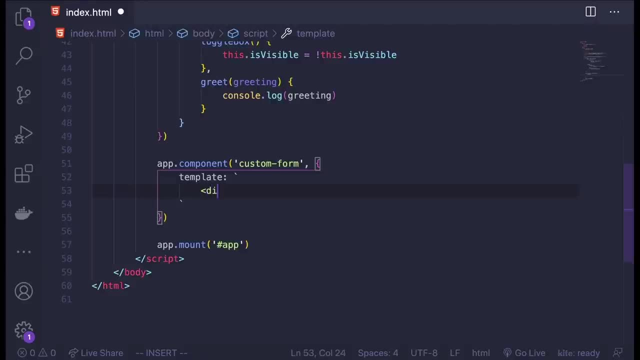 and pass in the HTML here. So, real quick, I'm going to create a div And I'm just going to put, let's say, two inputs in here. for right now I'll put a type of email, Okay, And then an input type of password. 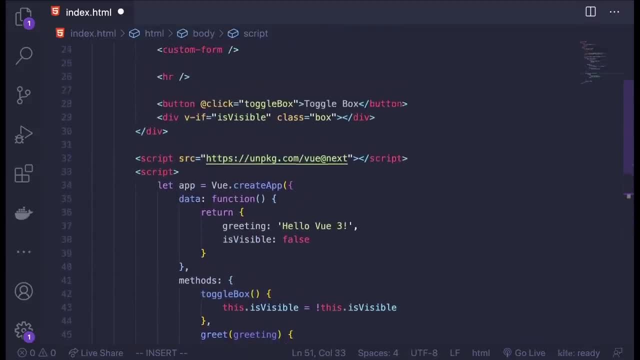 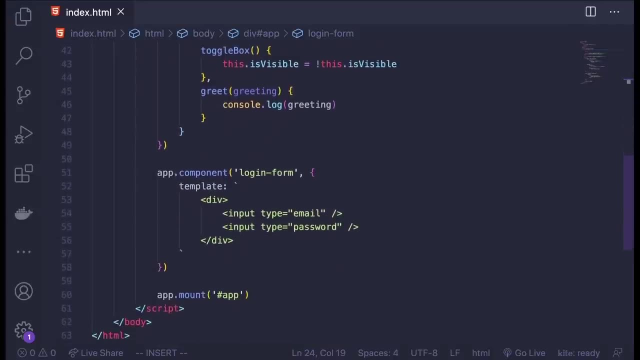 And let's call this a login form. Since we're doing email and password, I'll change that up here to login form. And since template is the only required option that I need to pass in on this object, it should run like it is right now. 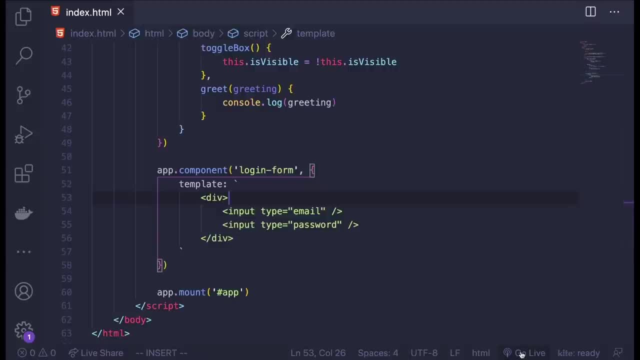 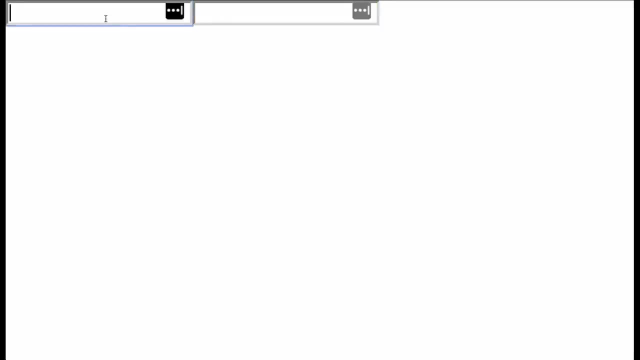 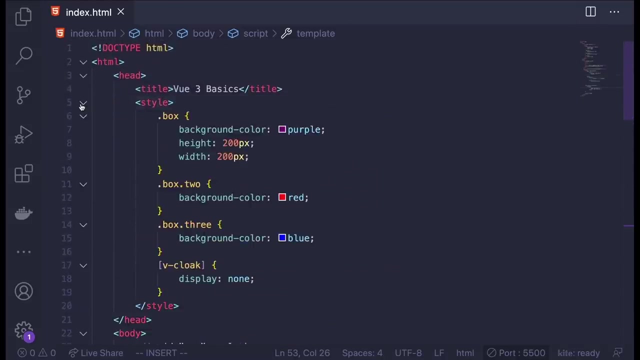 So let me see if this works. I'm going to go to go live And you can see these two form inputs up at the top here, completely unstyled, just basic browser inputs. So I'm going to style these inputs really quickly so they're easier to see. 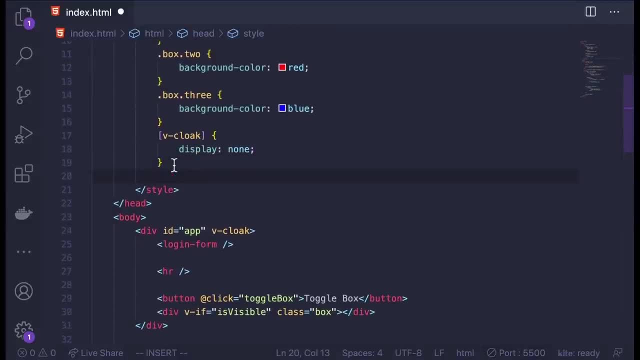 After all of these boxes, I'm going to add a reference to input. here I'm going to say margin of 10 pixels, just on all sides, And a display of 10 pixels. Okay, And then a reference to the default block. 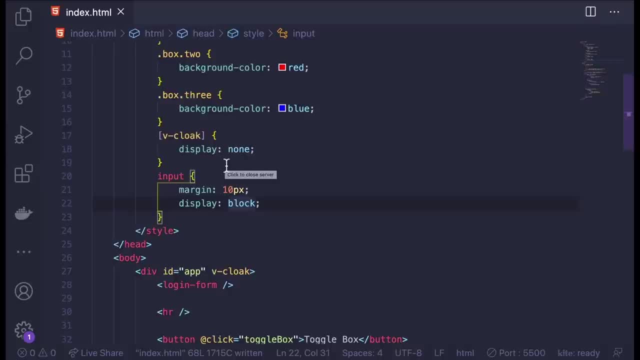 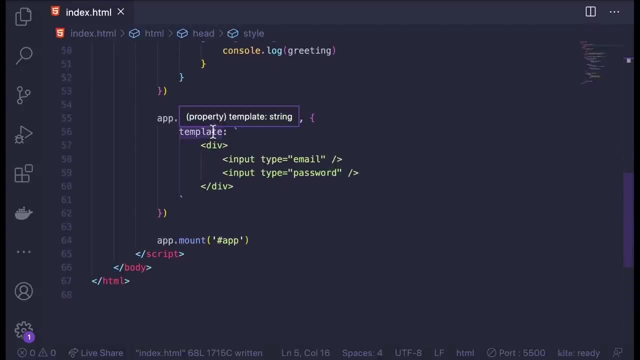 So they don't go in line, And now they are a bit easier to see here. All right, Let me code fold these styles again. And now let me add a data method to this component so you can see what that looks like. So after this template key I have here, I'm going to do the same thing I did above with data. 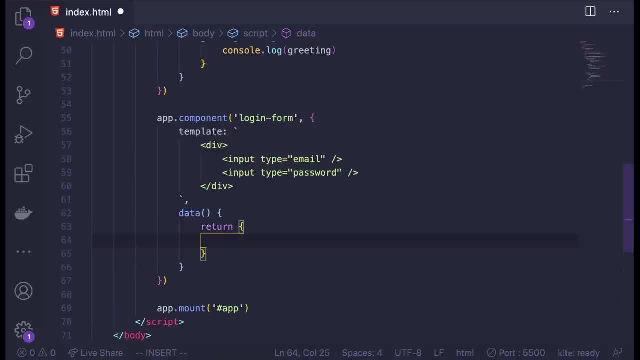 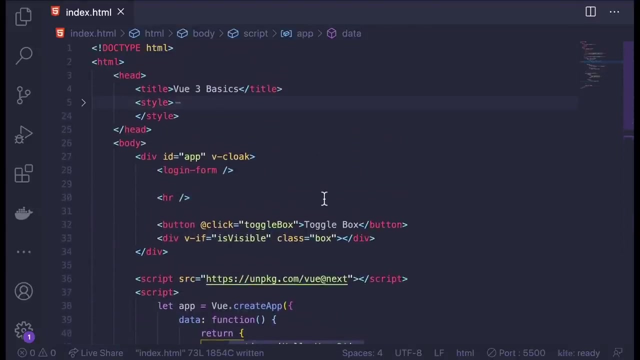 I'll just use the function shorthand here and here I'm going to give it a title And the title will be login form. And now I need to do something with this title. So up here, when I defined variables, I use them inside of my app. 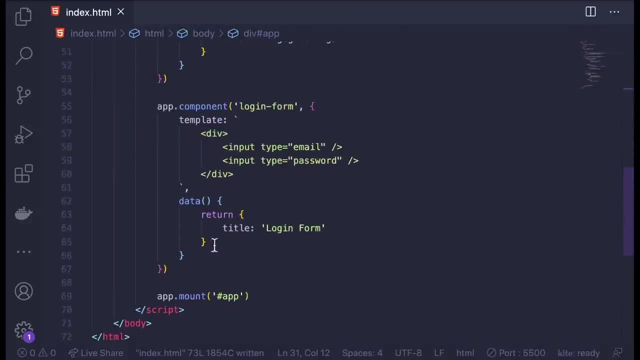 template here. But since my login form is a self contained component, any variables I define on data here I'm going to have to use them inside its own template. So I'll just add another line here and give it an h1.. And, by the way, this doesn't have syntax highlighting and isn't kind. 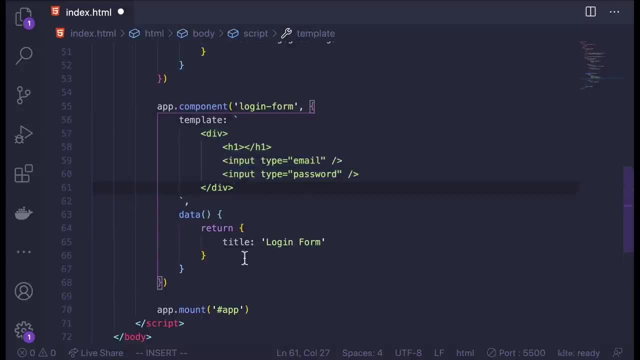 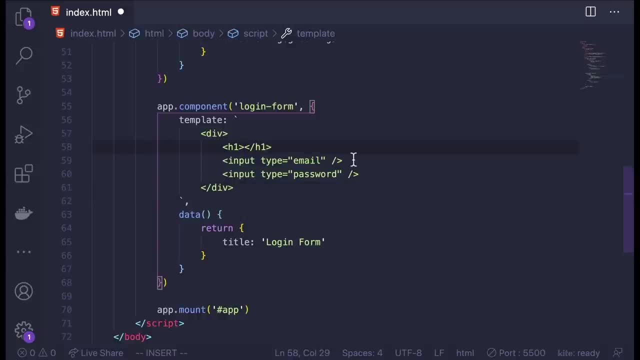 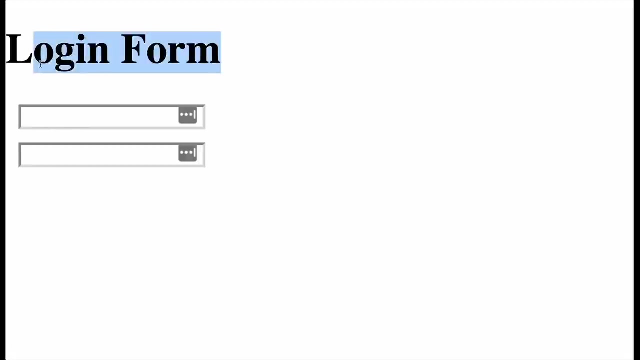 auto completion and all of those other great features. So here I need to use that variable title. So I'll use that the same way I did before, by referencing it, And now I should see the title on top of those two input boxes, And indeed I do. here I am zoomed in quite a bit. So that is the. 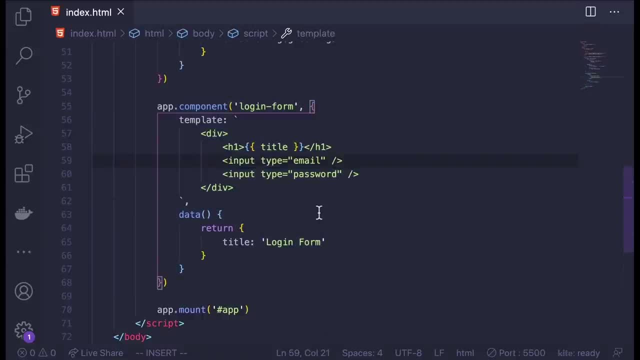 basics of how you can create a component here. I'm going to go ahead and keep building out this form and then also show you how to compose components now. so I'm just going to change this really quickly to form and then I'm going to add some submit. 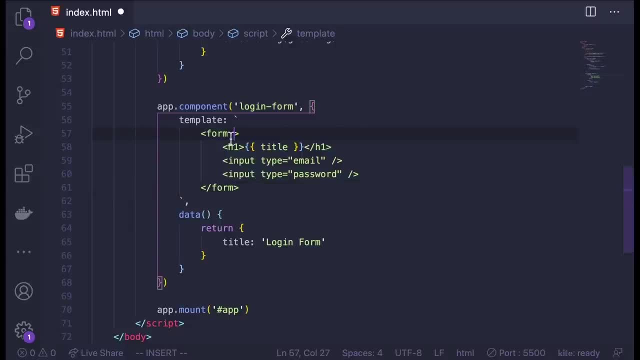 functionality here. so I'm going to add event for submit, submit and then pass in an argument with the method I want to run or the function I want to run when I submit a form. so I'm just going to call my function, I suppose, handle, submit and. 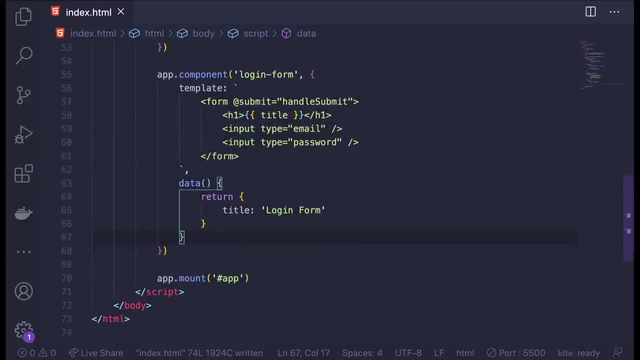 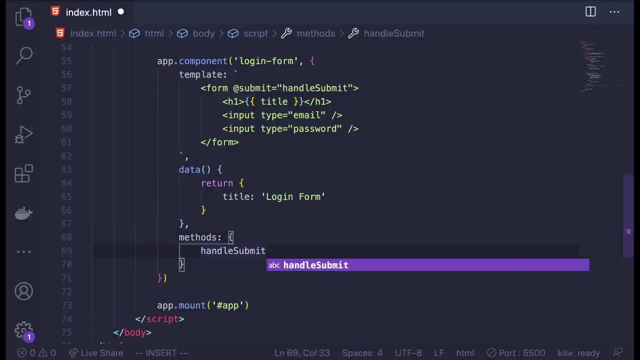 then I need to make methods object down here with that function. I'll call it a handle submit and I will just consolelog submitted. so now when the form submits, it will run this function. there's a few more things that I need to do. I need to add a button here that will actually submit the form. 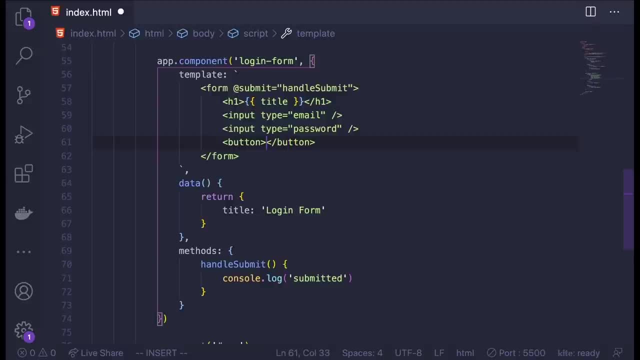 and then I'm going to add a function here that will actually submit the form, and then I'm going to add a function here that will actually submit the form. so by default, buttons are type submit. so I don't need to add that here, but I am. 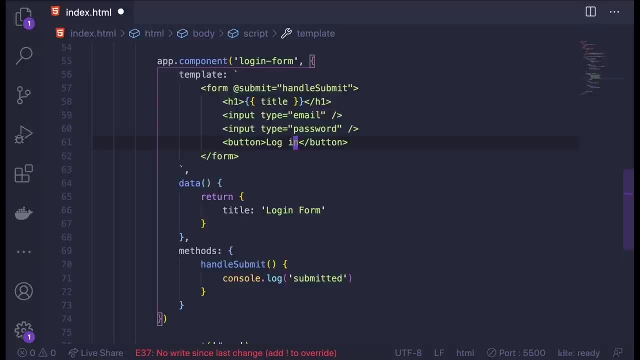 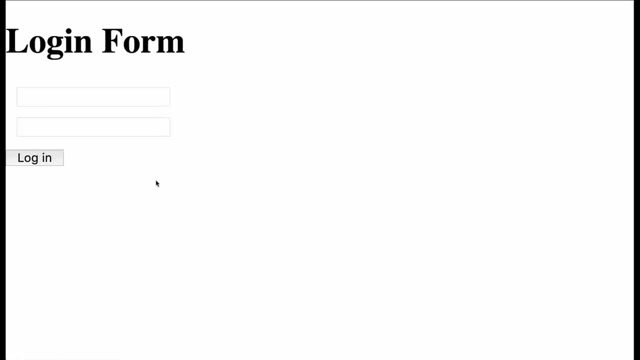 going to add some text to the button now. when the form submits, it refreshes the whole page. of course, this is the default behavior in browsers, so you can just automatically click and send data from the forum to your back end. but since we are going to be handling the form submission from our handle, submit. 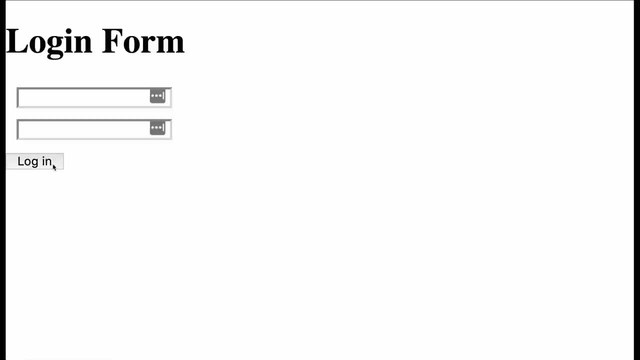 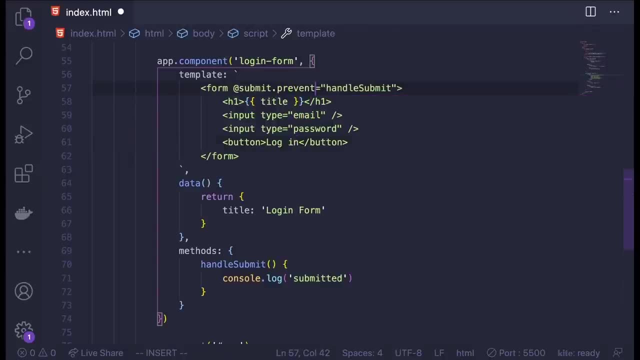 function. we don't want this default behavior to be in the form submission function. we don't want this default behavior to be in the form submission behavior with the page refresh. so, like we saw earlier, we have event modifiers so we can do prevent to prevent default. this would be the same thing as passing. 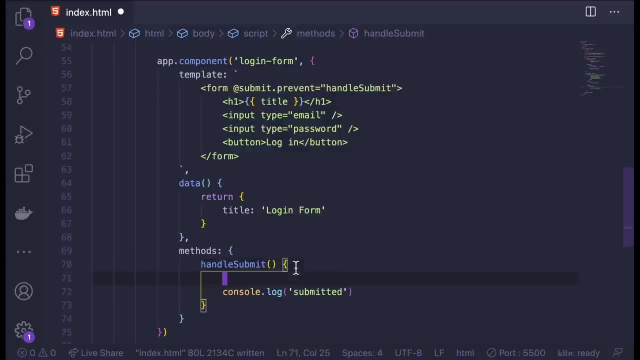 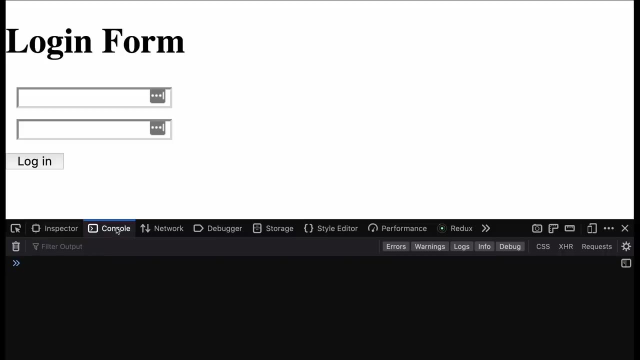 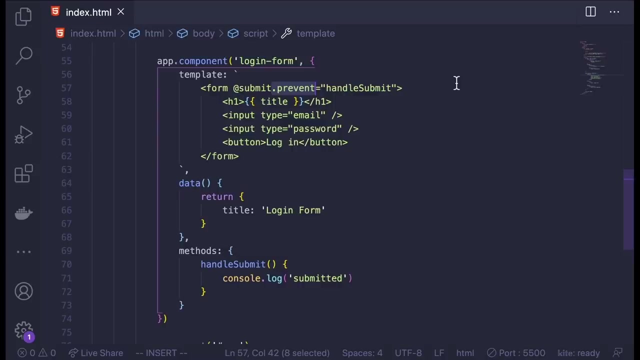 in an event object to our handle submit function and then doing e dot prevent default again. this is just a shorthand. so now, if we look at our console here, we see that it logs the form submission and then we can see that it logs the form submission when we submit the form. so now we probably want to be capturing these inputs so we can. 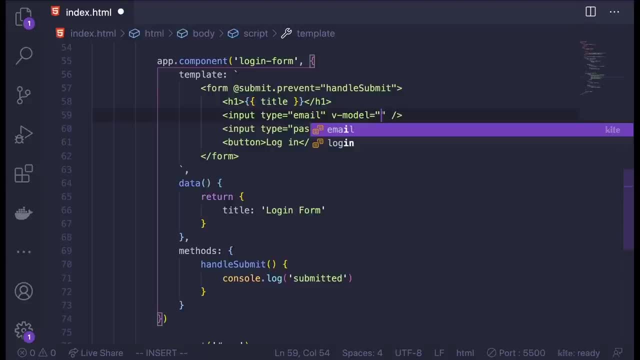 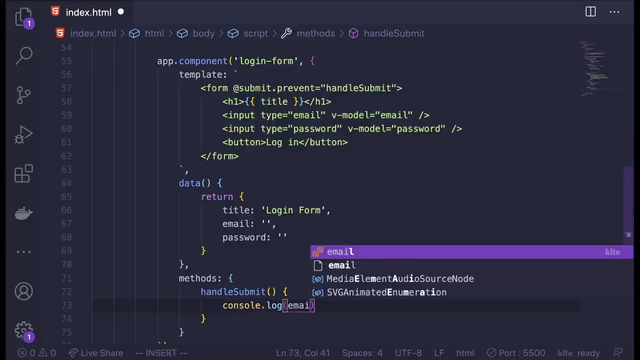 do that again by using the directive V model to bind the value of the form input to a variable. we'll call this one email and we'll V model this one as password and then add these into data. and now let's log those out. so let's log out email and password, of course, if you. 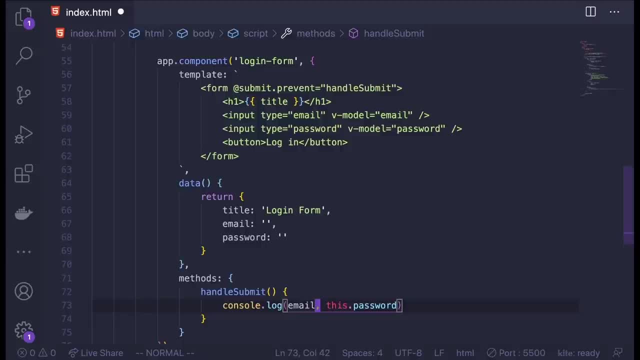 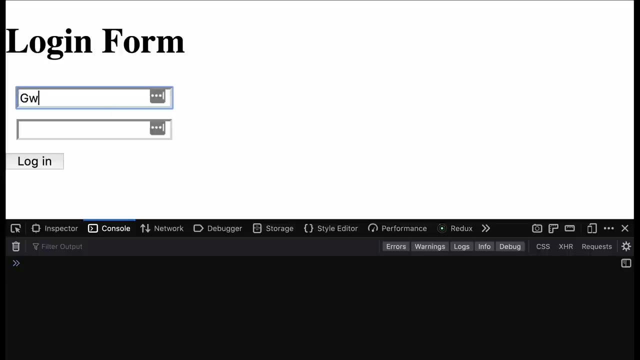 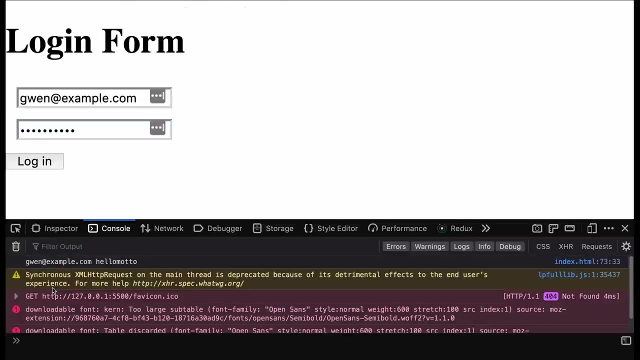 remember. I have to get it off of the this context, since I'm referencing it inside of JavaScript here and now. I should be able to type in something here. this has to be an email, so I'll say Gwen, at example, calm just any password and I'll click login and you can see it did log out my credentials here, okay, so. 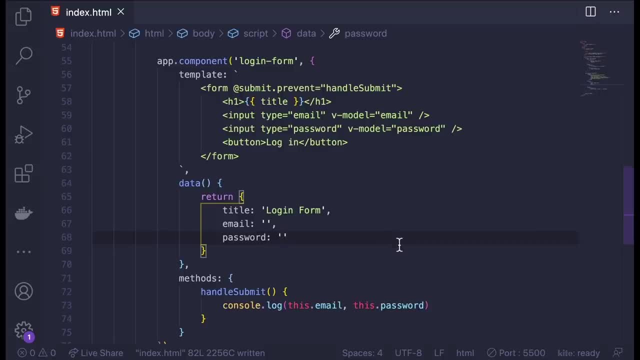 that's one component. in the next video let's look at how to break up this component and take out the inputs to put them in separate components, as you saw in the mock-ups earlier in this video, and we'll also look at how to pass data between components, so from a parent component to a child and then also from. 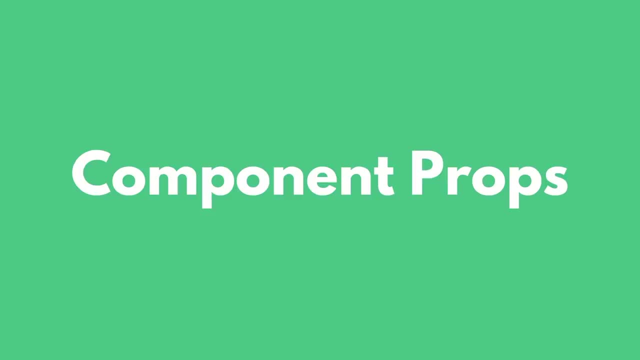 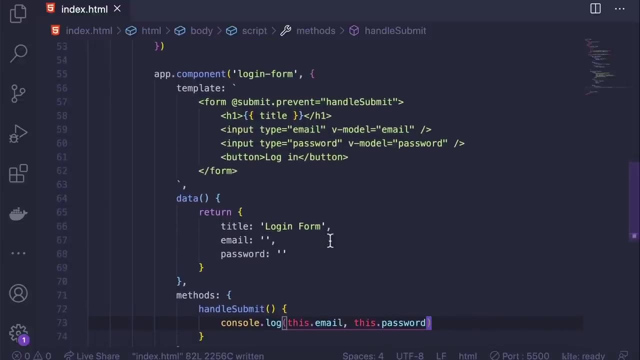 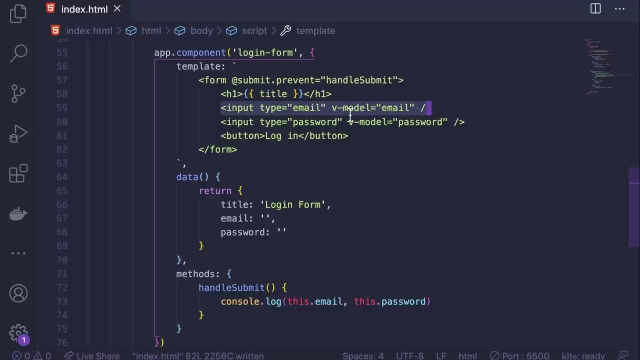 a child back up to the parent. so what if we want to compose multiple components together? let's demonstrate this by removing the inputs and creating a custom component just for our form inputs. let's say we want something like this and I've got some logic just contained within a special input component. so let 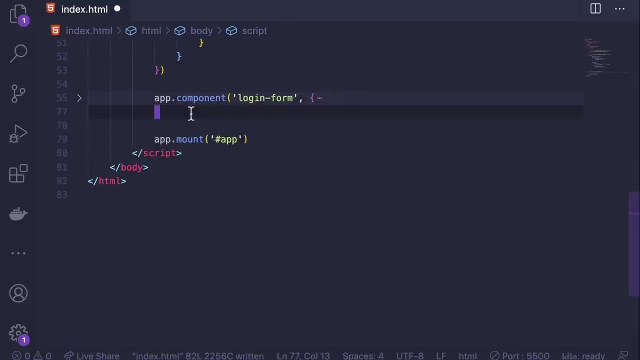 me fold this real quick and I'm going to create another component here. I'll do appcomponent again and I'm going to call this custom input pass in an options object. again, I need to have a template here and in this one I'm just gonna have. 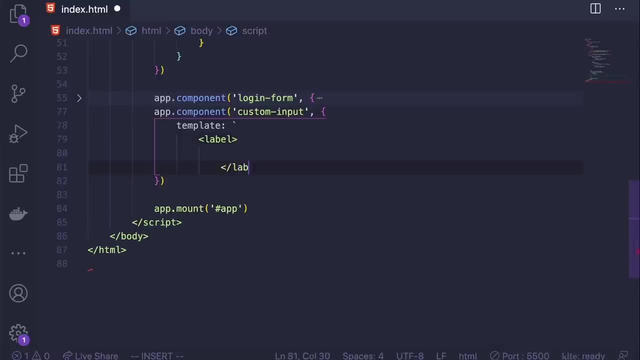 label label. I'm going to display a label variable here and then I'll have that wrap around the input And I'll use a type, just the default text, for right now. I'll change that in a second And that is a default input. 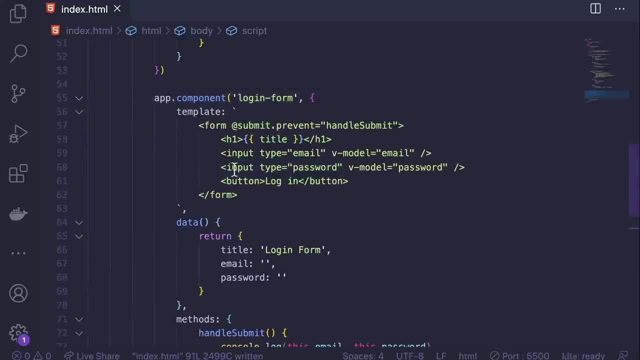 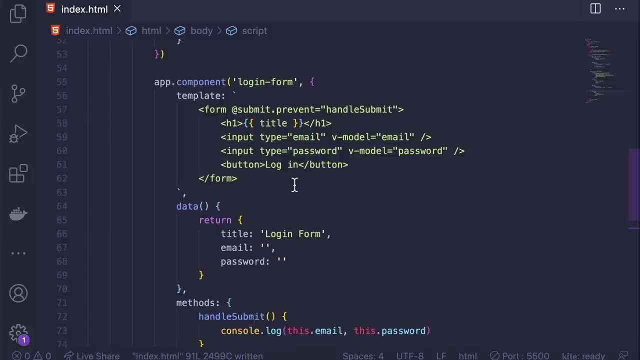 So now, where am I going to use this component? So I'm actually going to replace my input fields in this component with this new one that I created. So what I can do here is call this custom input and custom input and I can use my. 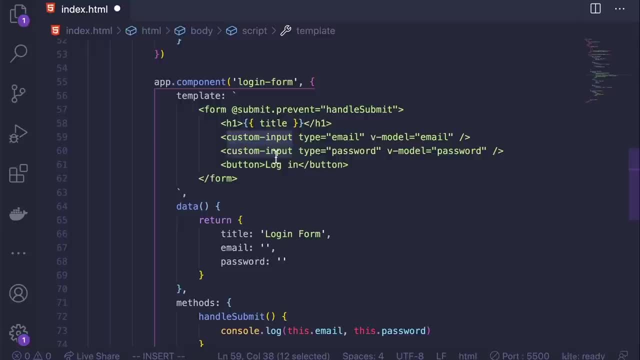 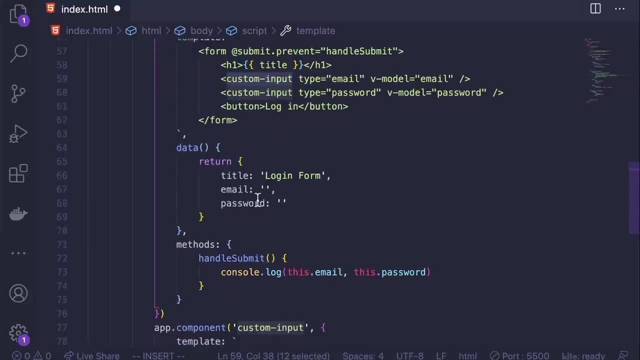 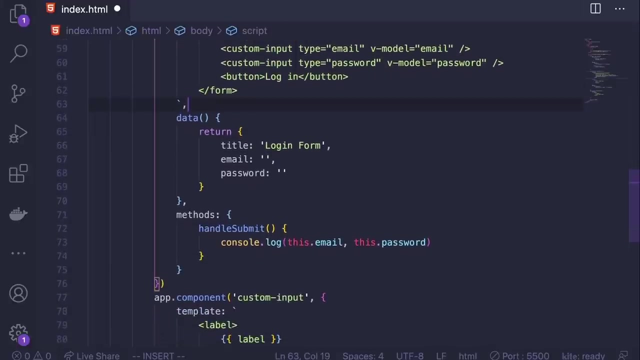 components inside of this other component. Now there's one more step that I have to take here, And that is registering the component. So I have to let my login form component- And I can do that here by creating a components array- And then just give it the string of the component that I want to be using, which is custom input. 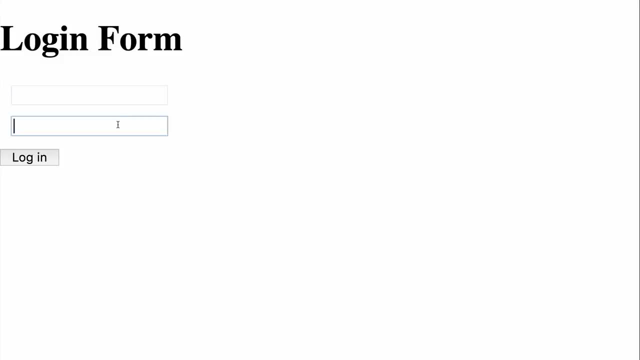 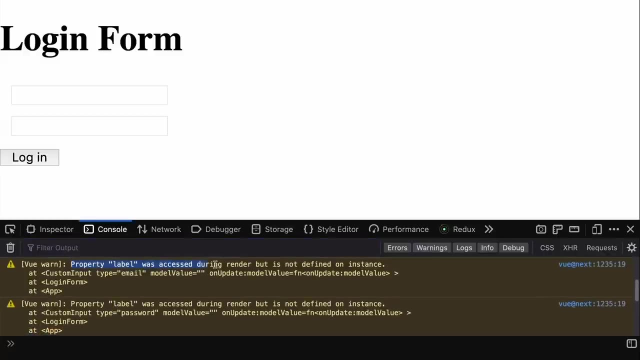 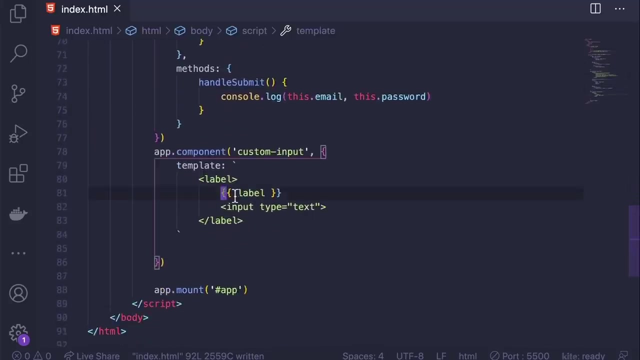 Now let's see how this works. Okay, so I have these two inputs. Now it is giving me this warning: that property label was accessed during render, But it's not defined on the instance. This is happening because here I'm referencing this variable label, but it is not defined. 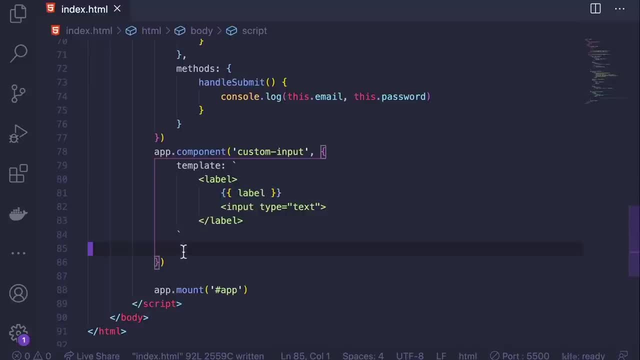 anywhere. So it's giving me that warning. Now I could define a data function here and create the variable on this component, But I want to demonstrate passing data from one component to another. So instead of defining it on this component, I'm actually going to define label on this. 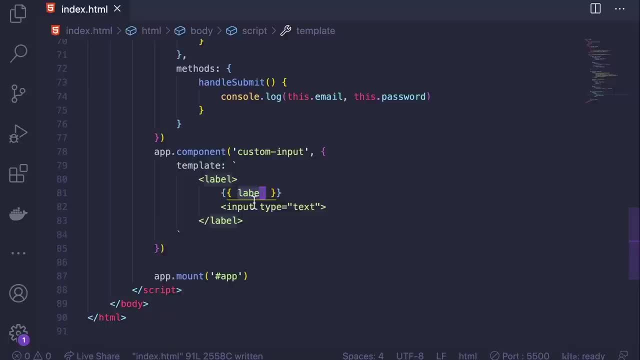 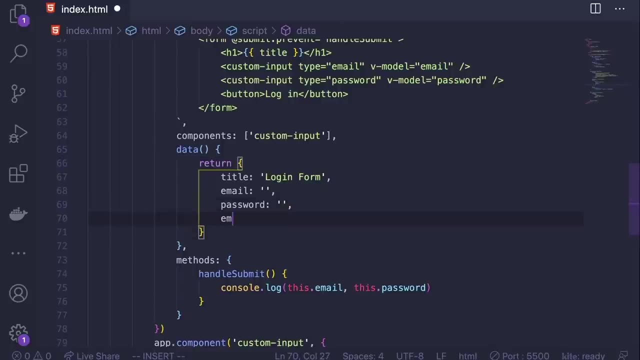 component And I'm going to pass it to the custom input component. To do that, I'm going to come here and add just a label. Let me add in, let me call it email label for right now, And I'm going to call it email. 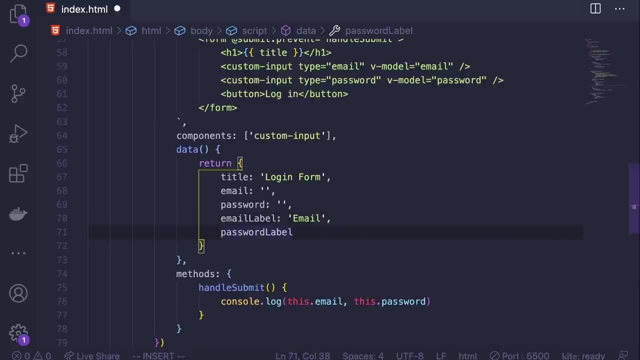 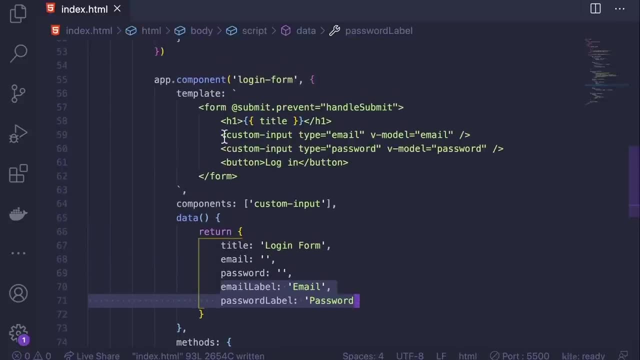 And I'll also have a password label and call this password. Now I have to get these two variables Passed into these custom components here, And so what I'm going to do here? I can go ahead and get rid of the V model for just. 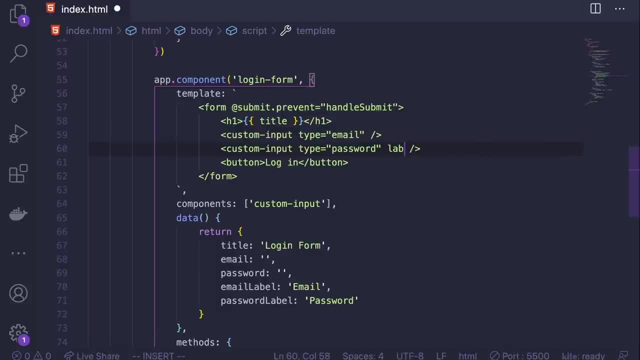 a second And I'm going to add a label here that I'm going to pass in, And I'm going to pass in the email label. Now, this looks just like an HTML attribute, but I'm actually going to add a modifier on here. 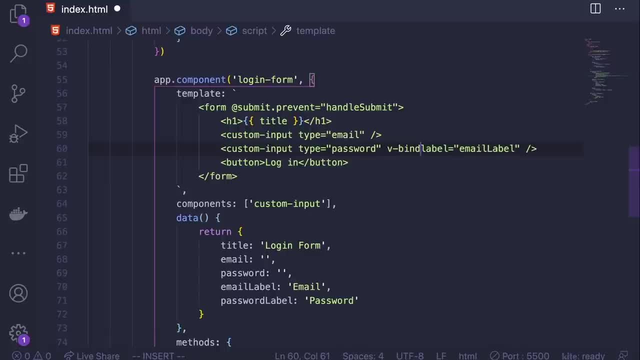 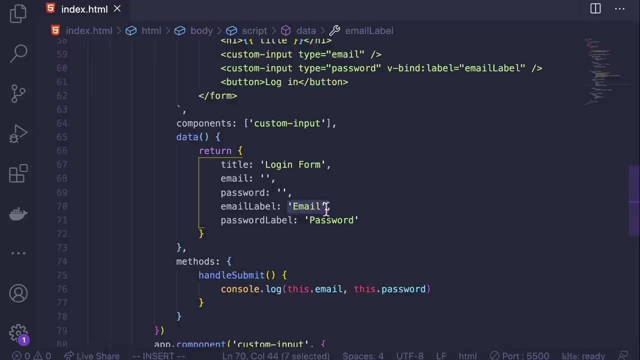 That is a view directive called V bind. What V bind does is basically turn this regular HTML attribute into something that can be parsed as JavaScript so that I can pass down a variable to the child component. So I'm V binding this label, which is email label, which refers to this string here, which: 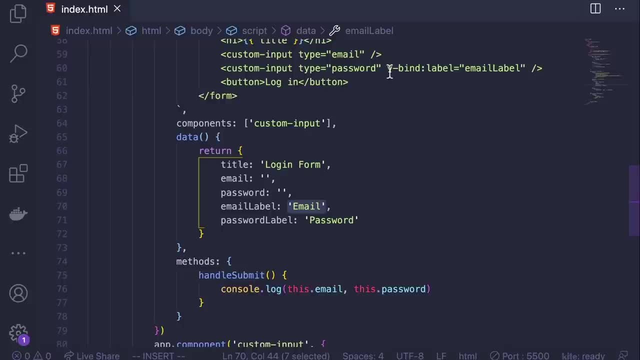 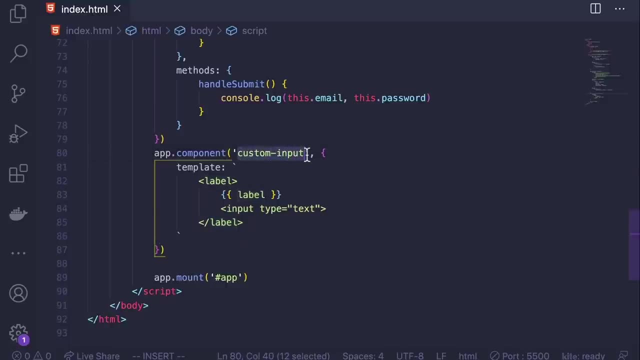 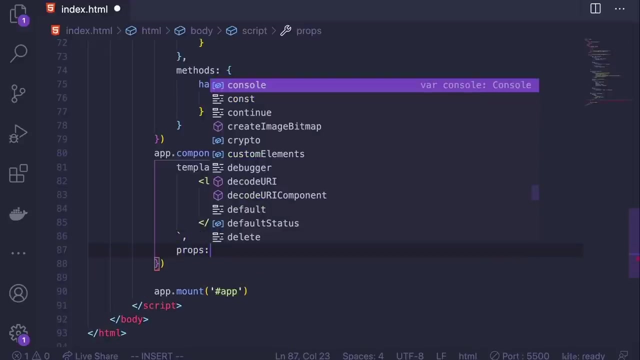 is email, This will get passed down as a property to the child component. So I'm going to call this child component called label. And now in this custom input child component I need to receive that property to accept it here with a props object. 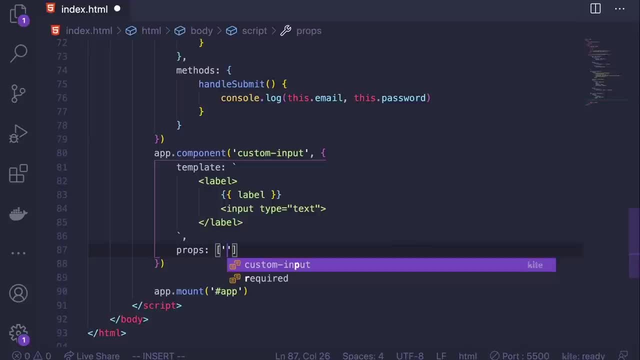 And the simplest way to write props is to make an array of strings, just like I did for custom components, And these props are basically just a list of all of the names of the information that I'm passing down, And I'm going to call this label label. 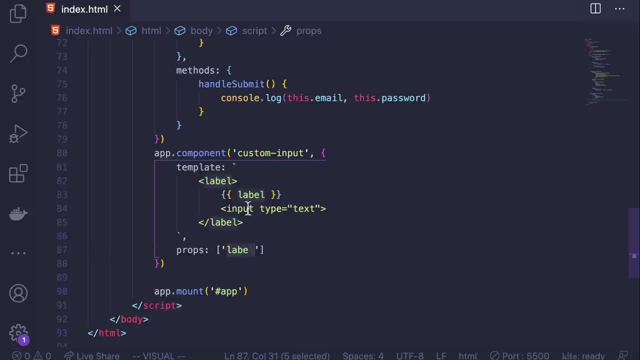 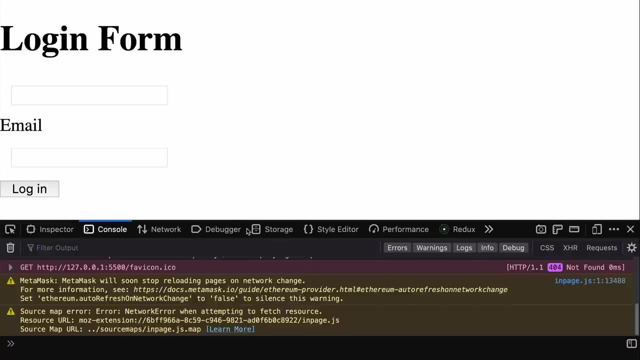 And now let's add a word in here And I'm going to say props to the child component. I'm going to say props to the child component because it's one of the most shopping tools out there and I'm going to type props to come down here. 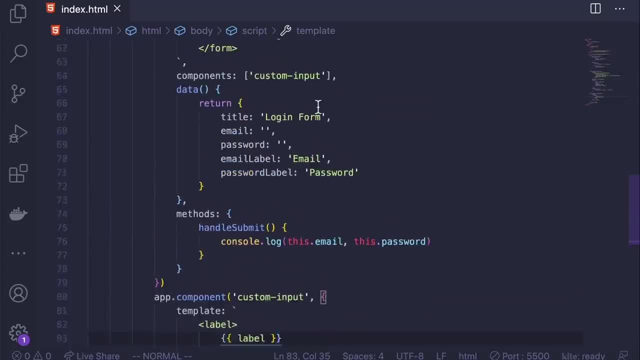 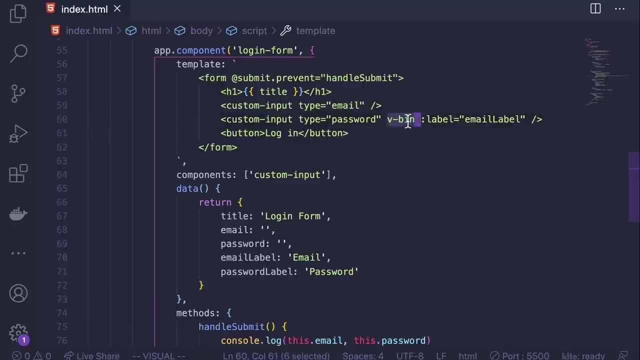 And I can also add some content here as well. So call this boss. I'm going to add something in password here. By the way, vbind. there is also a shortcut for vbind. This is one of the most common directives. 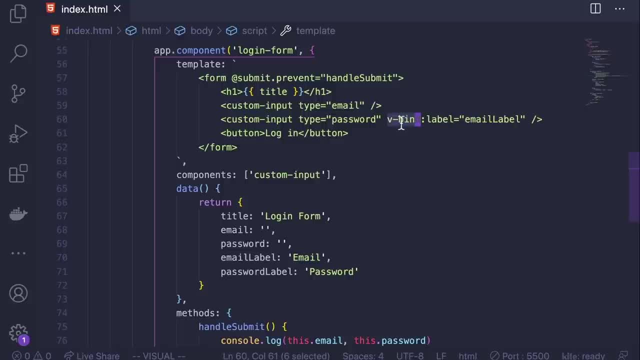 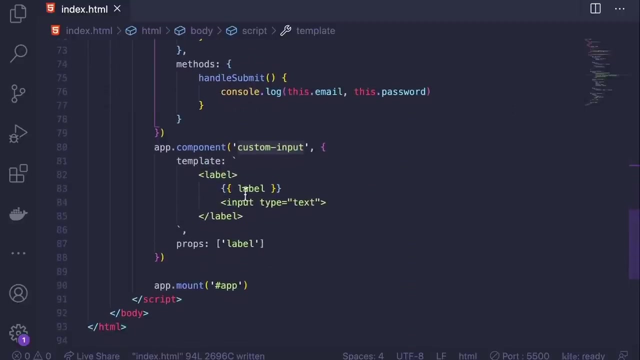 in all Vue applications. So the shortcut is: instead of using vbind colon, you just use colon and then label. So let me pass a label in here as well. So I'll pass a label in as password label, Since we're using this reusable component. 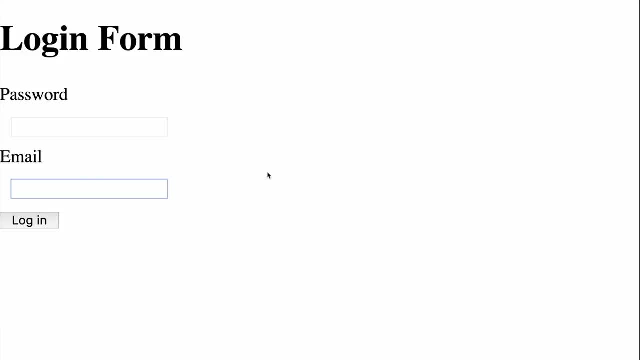 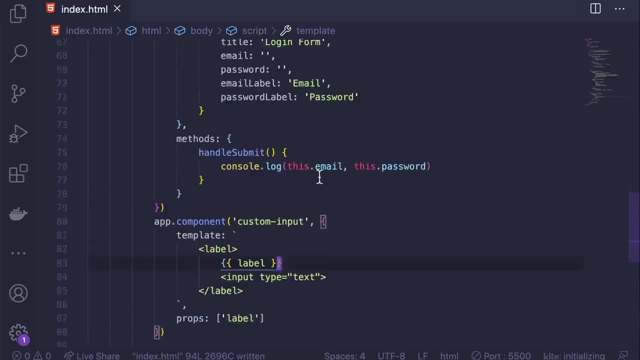 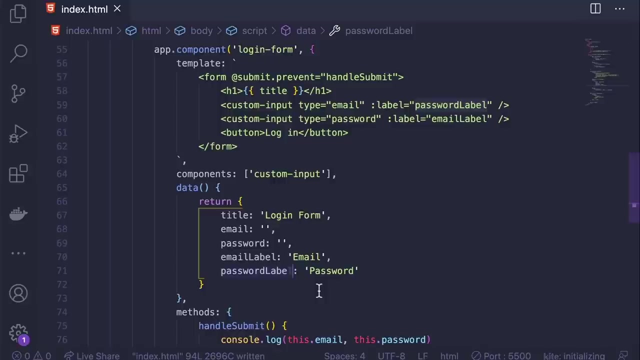 the label will always display as the label that we pass in, And now you can see that both form fields are properly labeled here. Now I want to point one thing out really quickly, and that is for email and these password labels. you could not make variables for these. 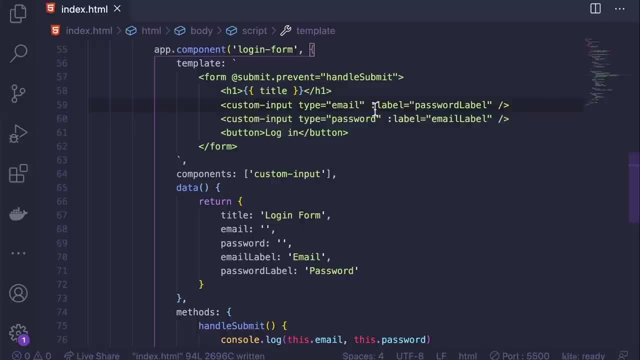 and just pass them in as strings here. So, for example, if I get rid of vbind, of the colon shortcut there, then I could just pass in, let's say password and let me put enter email here. so it's different. 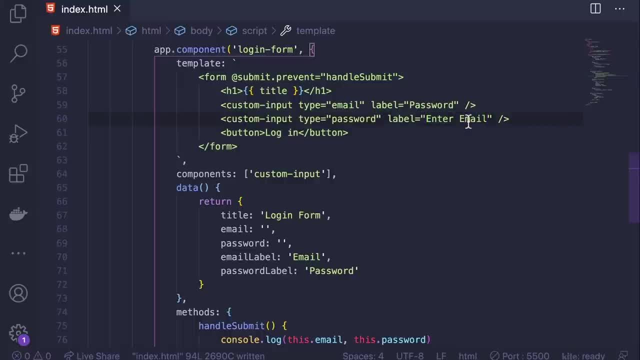 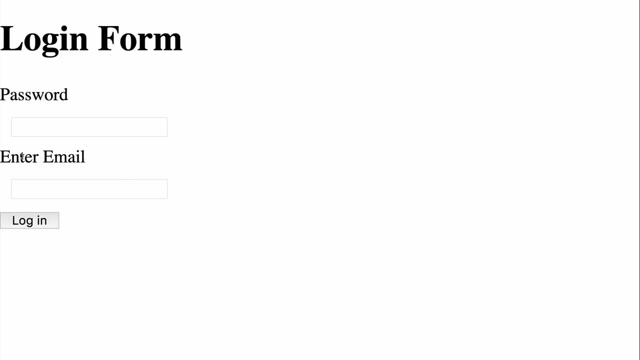 And now I can just pass in this text as a string, because there's no more vbind here. Vue is no longer looking for a variable, So now in the application you can see that it's just passing the string down as a label to the child component. 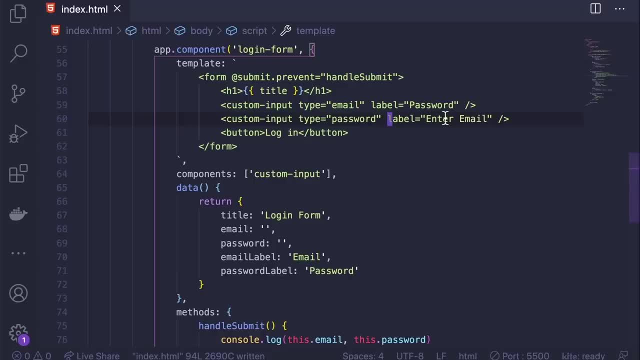 and displaying that string. I'm going to undo those changes. When you're working in actual Vue applications, you will see that 95% of the time you want to pass a variable in when you're passing a prop down to a child component. 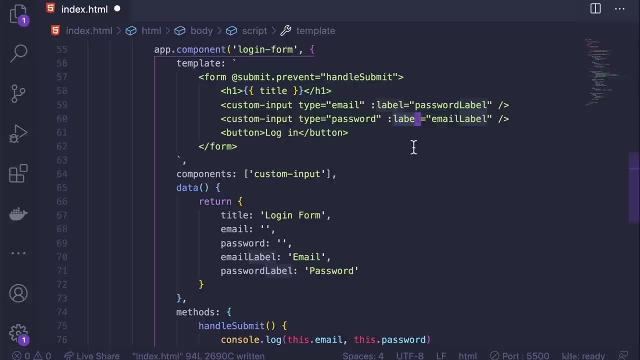 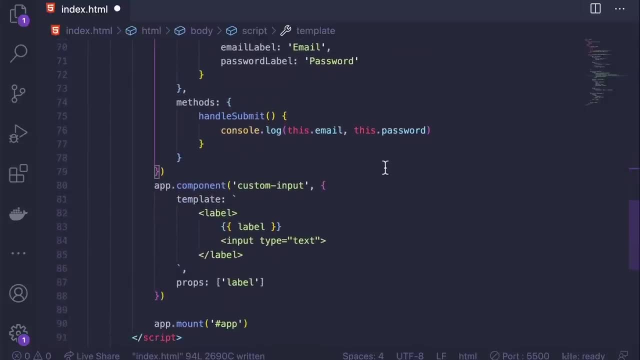 either a data variable or some kind of a function. So you'll almost always be using this vbind syntax here. Now there's one issue, because in the child component we have the input down. here We're not actually listening for changes to the text in the input. 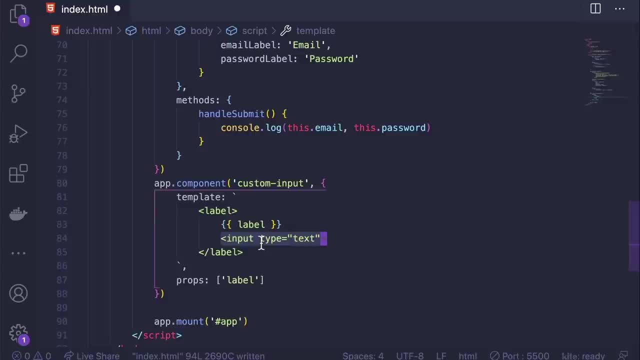 We're not vmodeling that to any variable, So we don't have access to whatever's inside the input. So we actually need to create a vmodel here in the child. I'm going to say vmodel And just temporarily here. 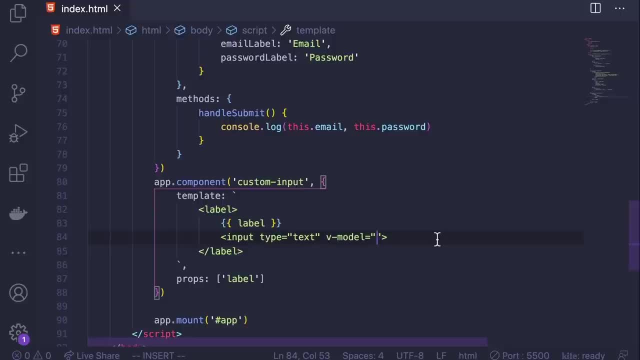 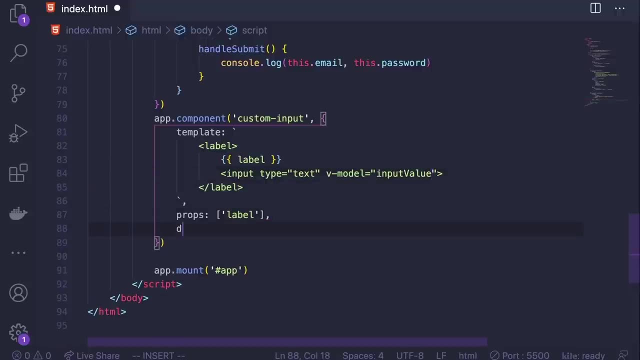 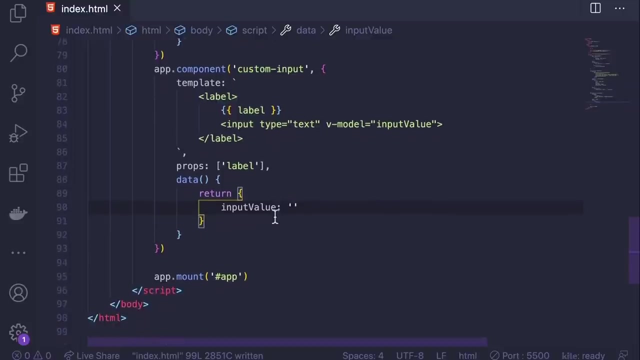 I want to map this to a variable in the child And I'm going to just call this input value And I need to create a data function here. Return an object with input value as an empty string. So now, in this case, you're already familiar with vmodel. 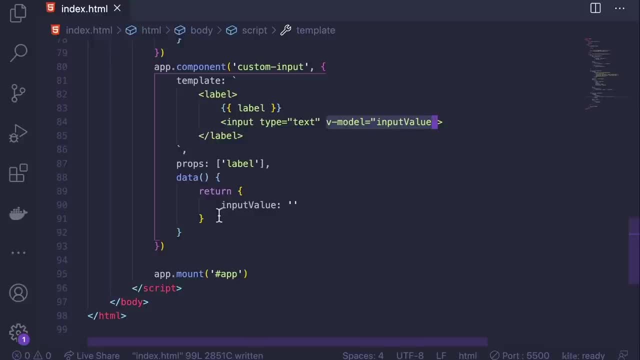 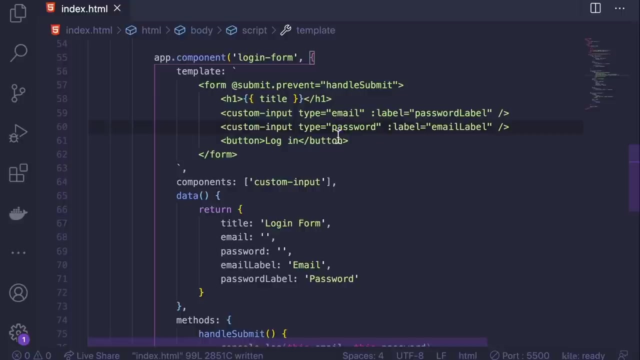 And you know that anytime we type a character into this input, it's going to update this variable And this variable and the input will stay in sync. But now how can I get the value of this variable up to the parent component here, Because I actually want it to stay in sync. 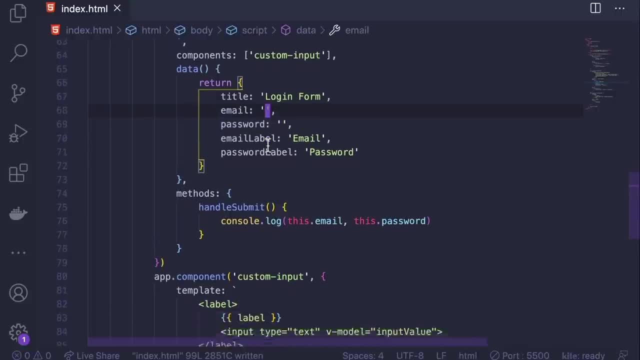 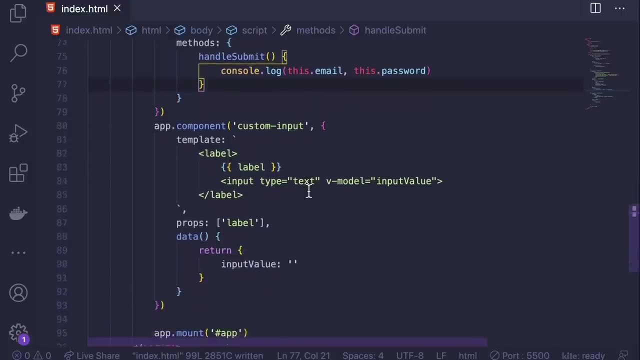 with these two variables on the parent component. So that way when I submit my form, I can have access to it in this handle submit function. So there are actually a couple different ways of doing this. I'm going to show you the most straight way. 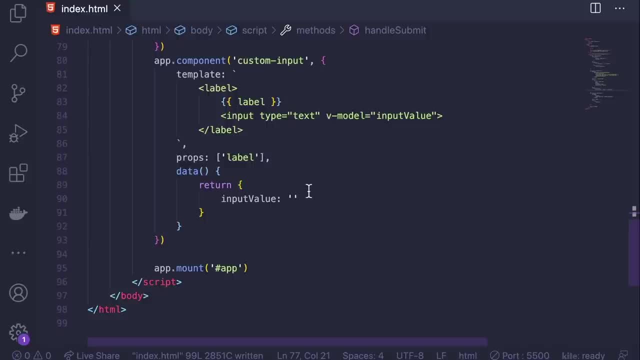 And then I'm going to show you the most straightforward approach for getting started with this, And then, in future courses, I'm going to explain a little bit more in depth about how you can use custom events and other methods of capturing the value of a variable. 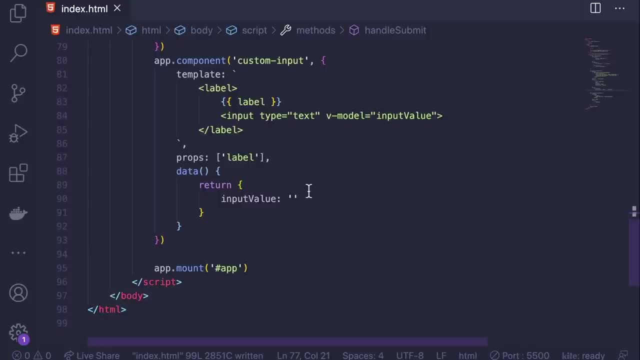 from the child to the parent. So to get started here, I'm going to use my same input variable, But I'm going to use a new object here, And this object is called computed, And this object is called computed. And this object is called computed. 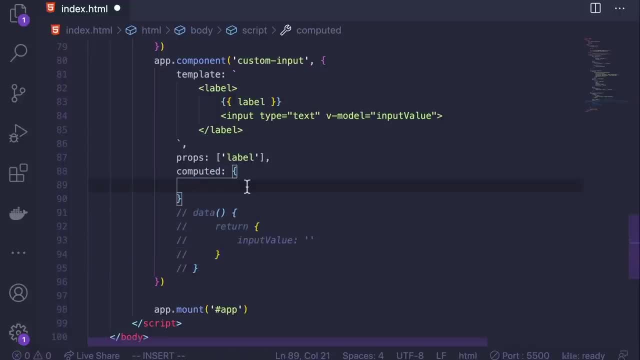 So I'm going to comment out data for a second. So computed is an object where you can put variable names in here as keys. So, for example, this input value variable that I want to create, I can put it in here as a key. 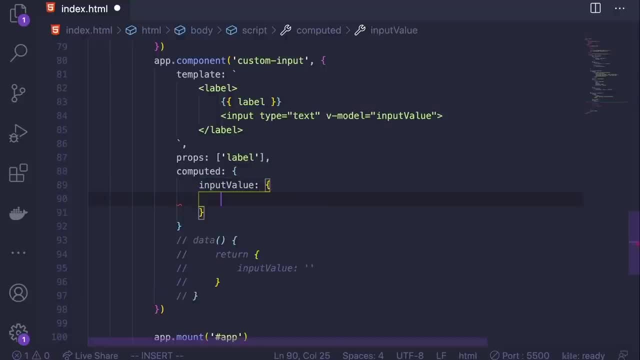 And whenever this value changes, I can actually get it to run getter and setter functions. So I can create a getter function and then a setter. So when I get the variable value here, it will run this function. And then when I go to set the variable value, 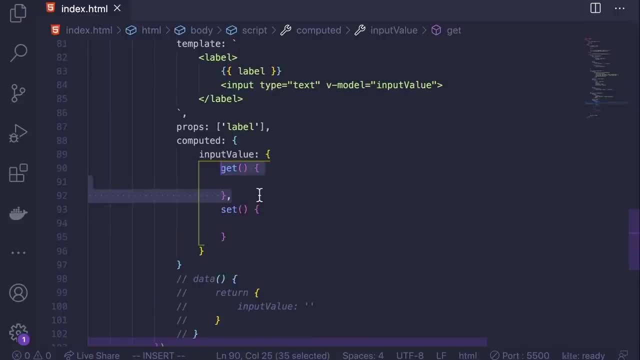 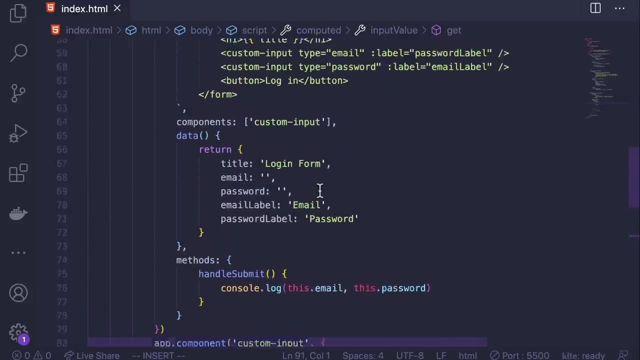 it will run the set function. So now, what value do I want to put in my getter here? I want to get that value from the parent component. So I'm actually going to use these two variables that I already have here, And I'm just going to get rid of. 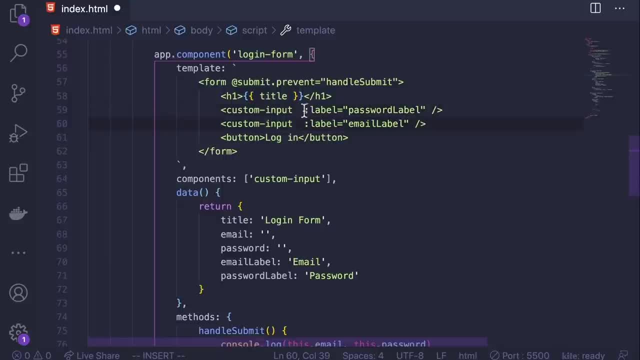 these types. I'm not using them yet, So get rid of those. And I'm actually going to do something different. I'm going to create a V model directly on my custom component here, And I'll show you why in a second. 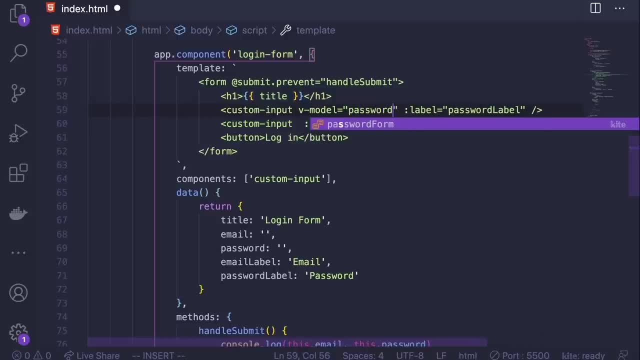 And I want to model this to the variable that I'm going to be using. So for this one, that is the password variable And for this one, that's email, And these got out of order, so I'll switch them around. 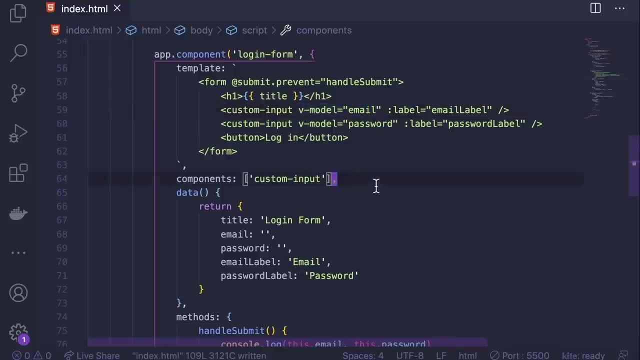 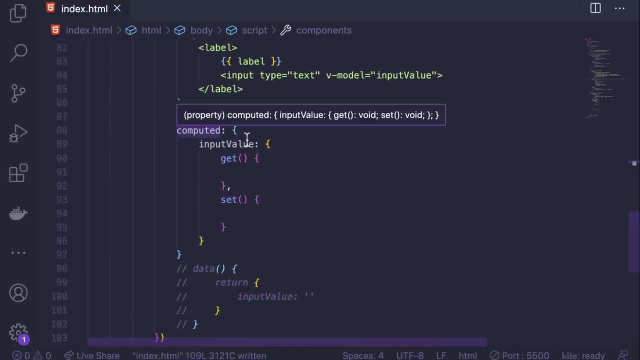 Okay, so now I'm V modeling the email and password, And now I want to get these variables in my child component here. Now how do I do that? So in props I can actually accept a prop called model value, And this comes from the parent. 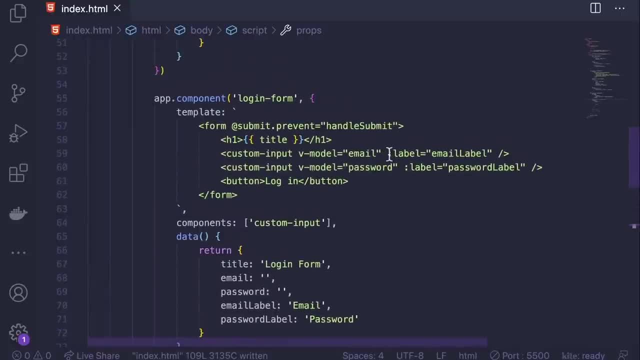 Now it doesn't really look like we are passing in another prop because we're not V binding any variable and passing it to the child. But actually what V modeling does on a child component is actually under the hood. it's giving us another prop called model value. 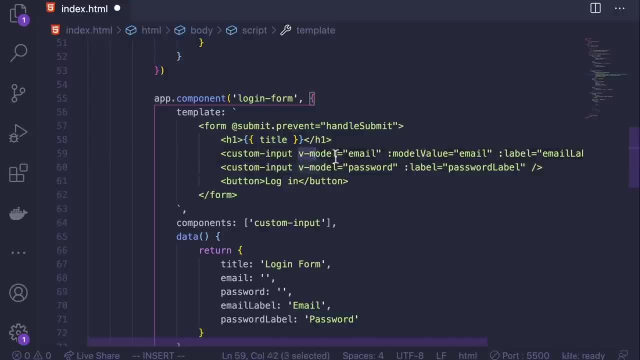 which is mapped to email. So V model does a few steps all at once. It's kind of a shorthand here. So I have access to this model value prop because I'm using V model, So I can accept that prop in the child here. 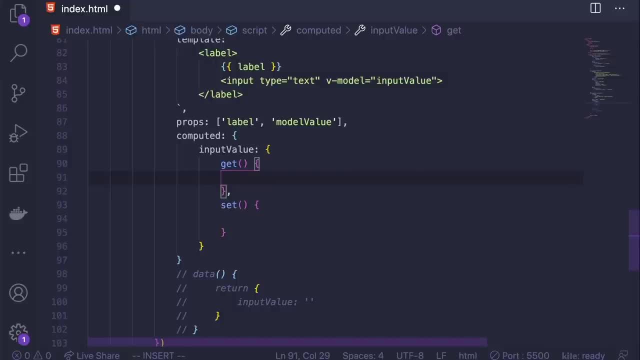 V model And then in my getter function I can do this dot model value and I can return that. So now, whenever I get the value for this input, it should be the same as the value in the parent component, And I can check that by just. 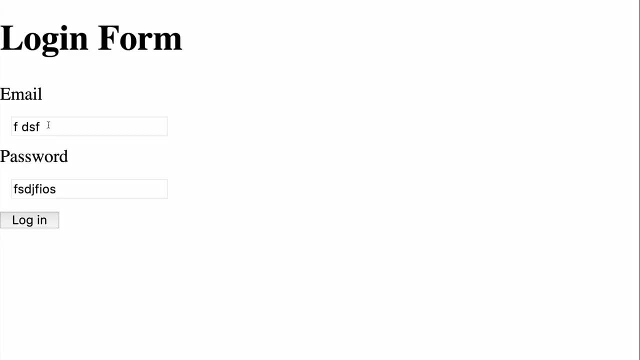 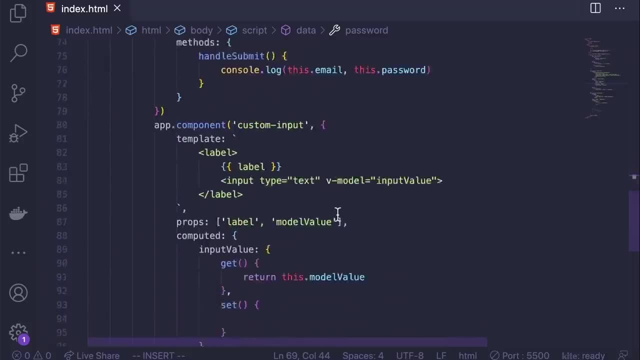 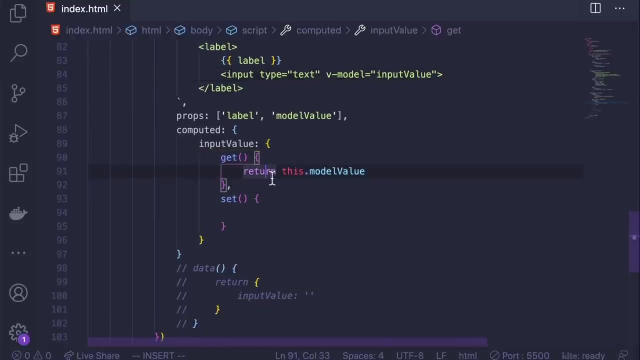 typing in some values here And you can see that the inputs are pre-populated with the value from the parent component, because I am V modeling this input to a getter function that I'm setting here and saying that the value will be this dot model value. 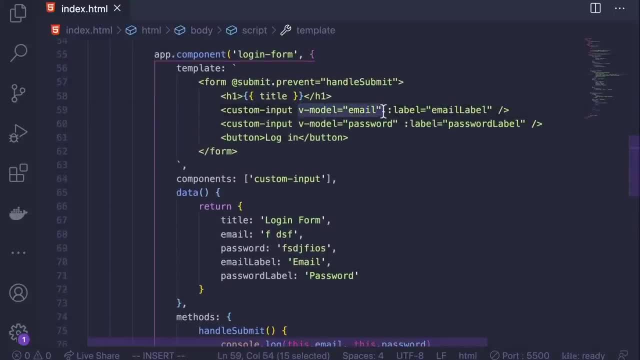 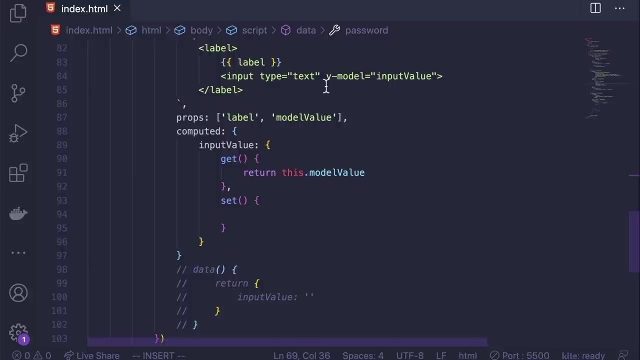 which comes from the V modeled variable in the parent component. which are these variables? So now, how do we handle setting the value if we type text into this input here? So we need to capture the value first and Vue passes this in via a parameter so we can give this parameter. 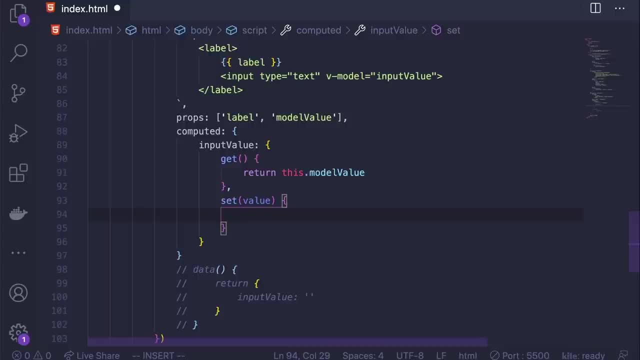 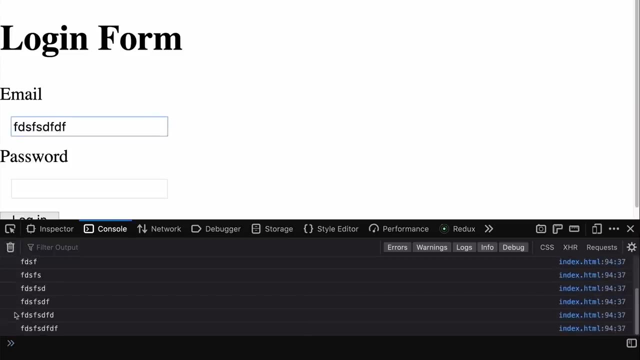 any name that we want. I'm just going to call it value and I'm just going to first log out this value. And so here I can try typing in and you can see it's logging out the value of the input from that log in the setter function. 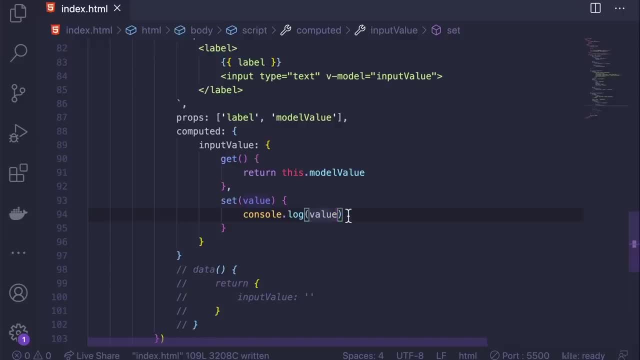 But now it's not setting a variable anywhere. So let me go ahead and set the variable Now. to do that, I'm going to use a new method that you haven't seen yet, and that is this dot dollar sign: emit. What emit does is allow me to emit events. 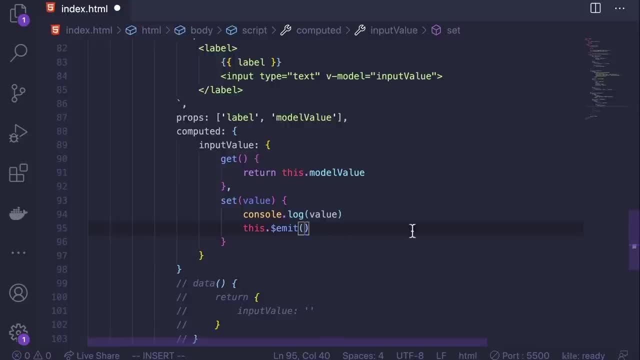 that other components can listen to And I can pass data around my Vue application like that. I can emit events that are built in, like I could emit some kind of click event or something like that. Or I can emit a custom event that I create. 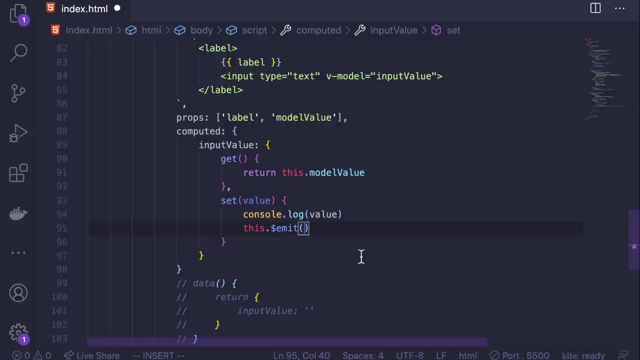 For right now I'm going to use an event that Vue gives me, and this is called an update event. This syntax is actually new, slightly updated in Vue 3.. So if you see older tutorials that might not be using this exact same syntax, it will probably be using. 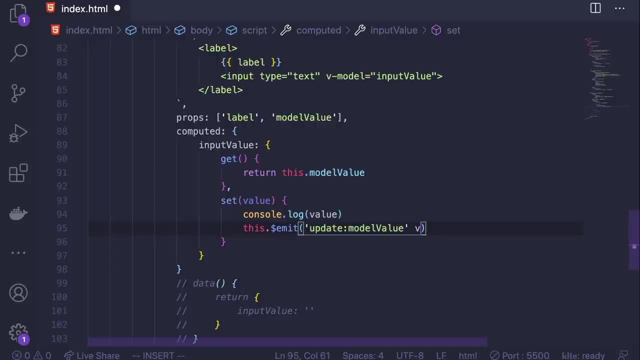 an input event here instead, But I'm going to pass in a value here. Oops, I need a comma. So this first argument is the type of event that I'm emitting And the second argument is the value that I'm passing through that event. 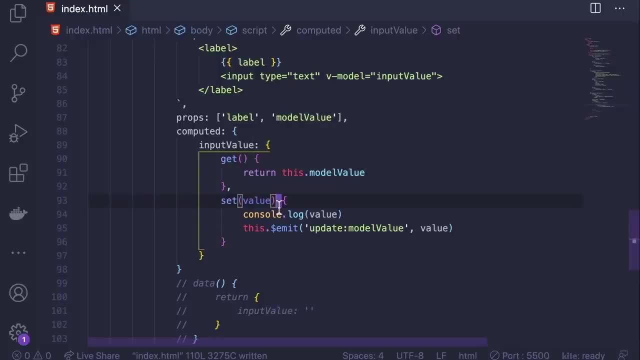 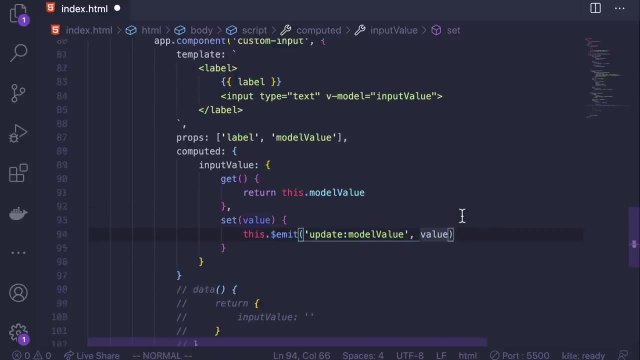 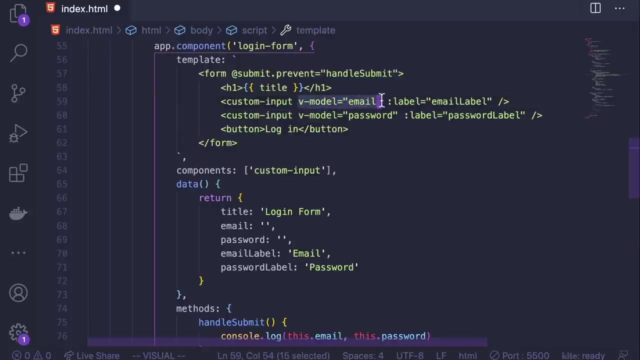 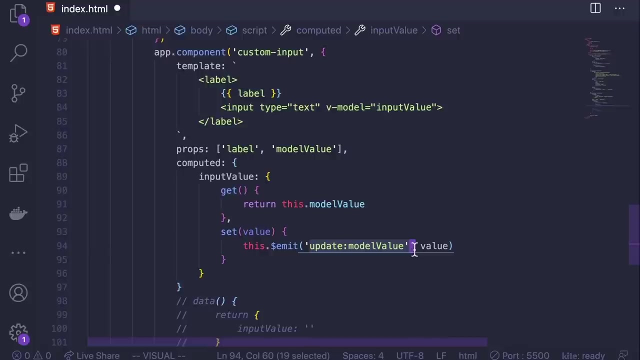 Which is this value that I'm getting from the input via the set function. Now, how can I listen for an event in another component? I could set this manually but, like I said before, Vue model is a shorthand, So Vue model is actually listening for this update event from my child. 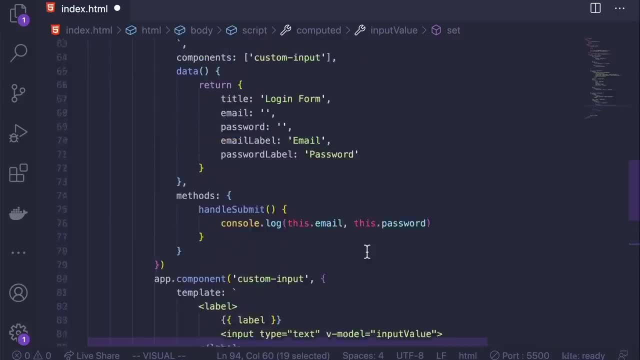 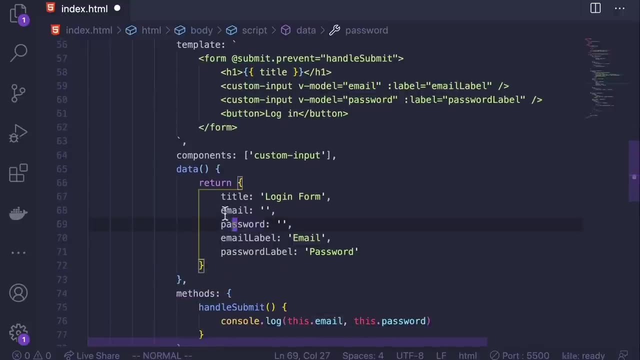 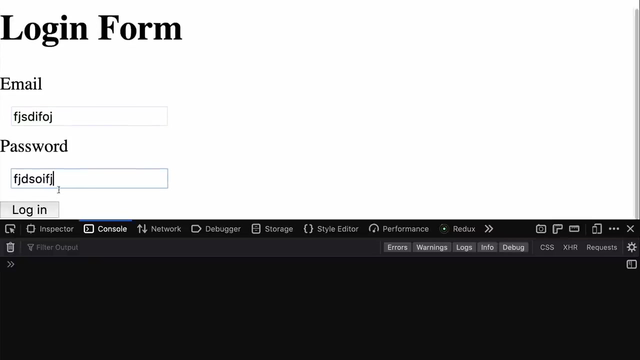 And whenever this update event emits this Vue model from the parent component is updating the value of the variable for us. Let's test this out. I'm going to start typing here, Typing here, And I'm going to press login And you can see that. 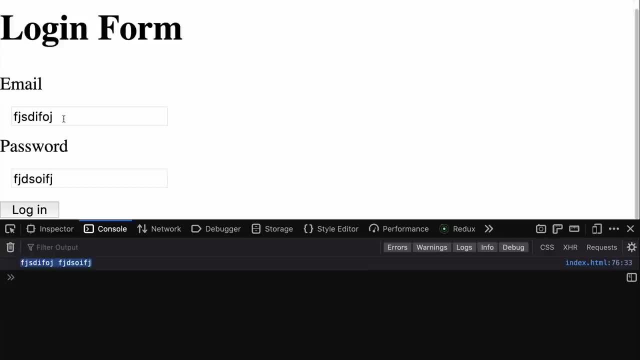 it logs out the values of the email and password. So this isn't that clear. so let me put a real email here- A real fake email anyway- And you can see there's the email and there's the password Which are coming from this log statement. 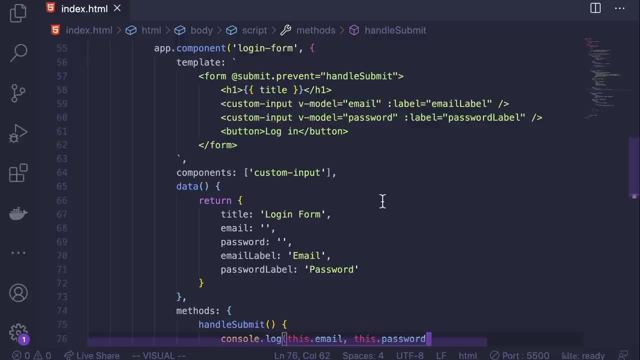 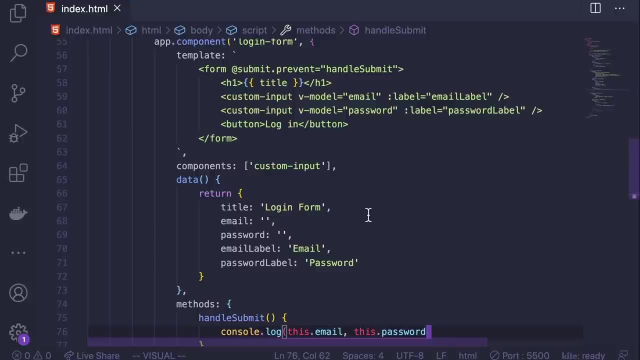 in handle submit. Now you might be wondering why do we have to go through all that trouble to model a variable from a child to a parent? And the reason why is because the props that we pass to children, they are immutable. We cannot change them in the child. 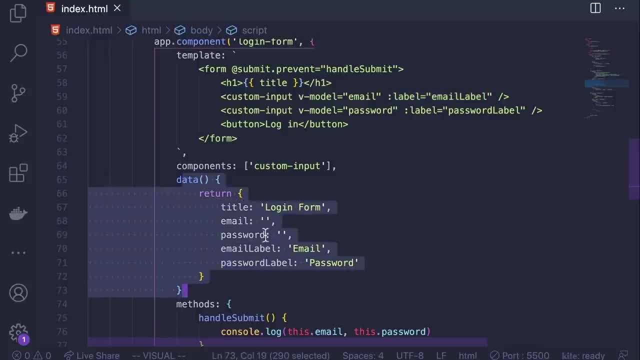 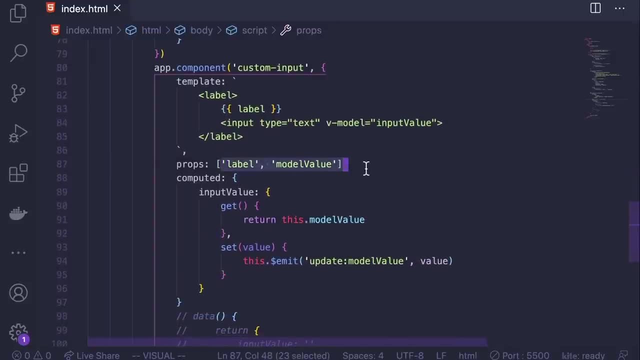 These variables on data here can only be changed in the same component, So my custom input can't change anything we pass in via props here. So, for example, if I tried to model this to label here, I'm getting all of these warnings to mutate prop label. 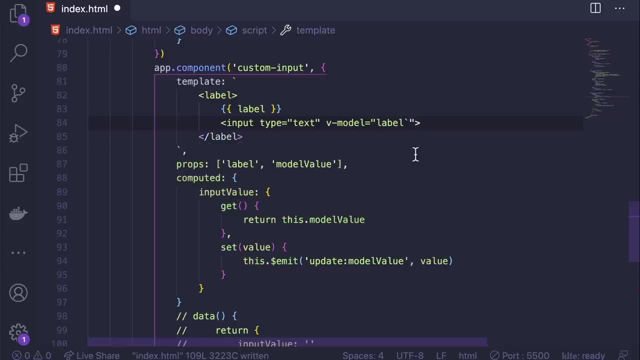 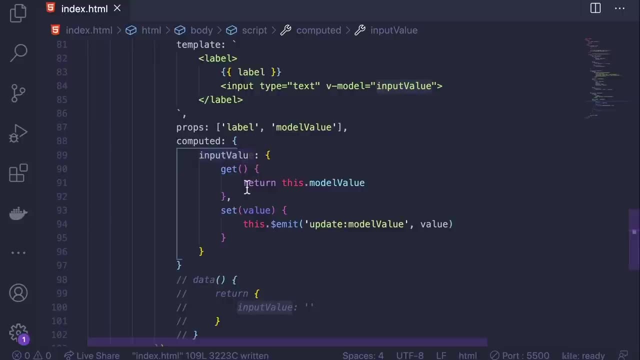 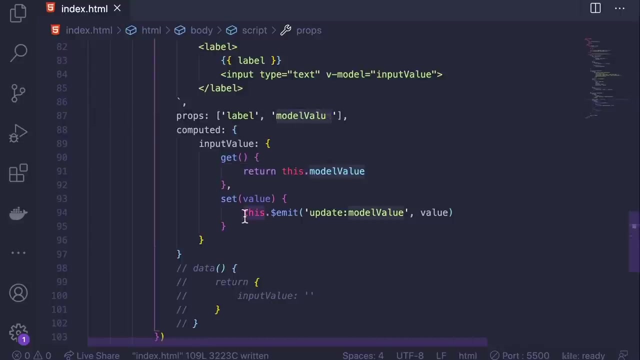 Props are read only. So I'm going to undo that. So that's why I had to create this extra variable in the child And create a getter. So I'm getting this read only model value prop from the parent And then what I'm doing to update. 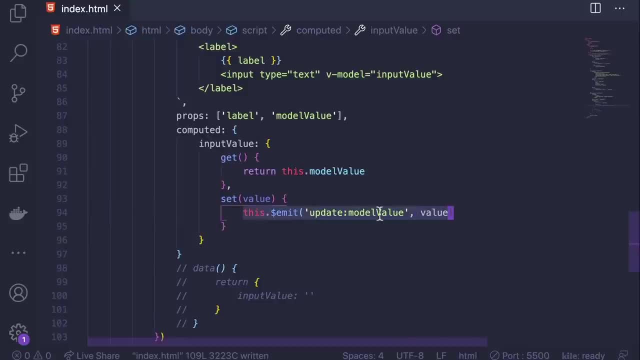 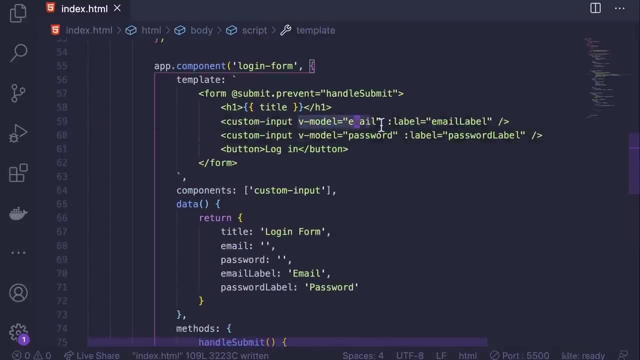 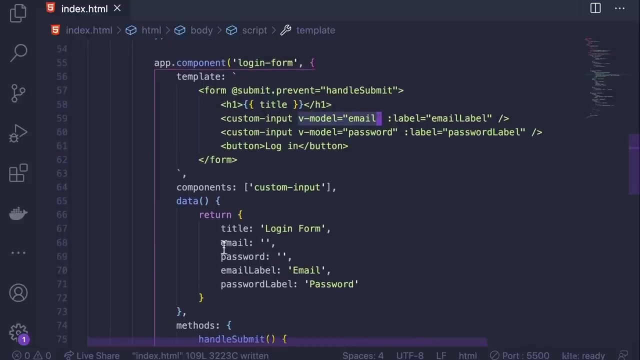 the value of that prop is: I'm emitting an event to the parent, This update model value event. So the parent, because I have this vmodel shorthand, is listening for that event And this component, this login form component, is actually updating these variables itself. 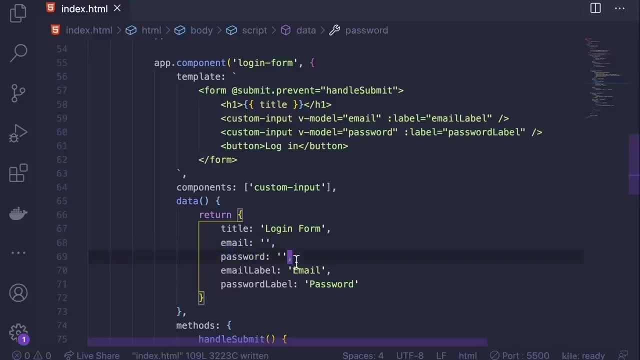 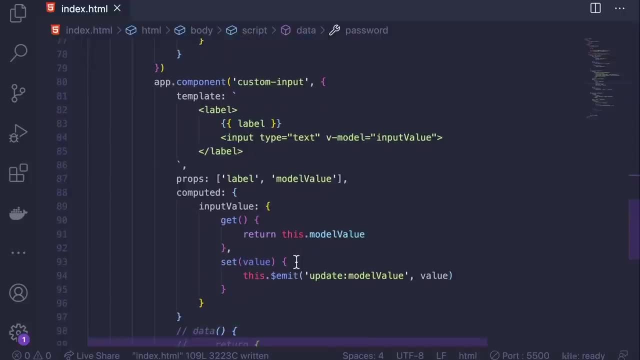 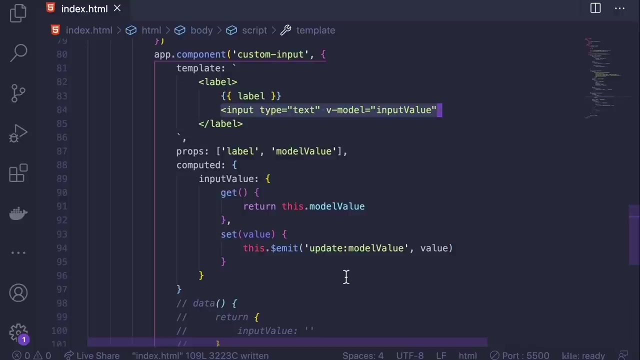 So I'm not actually mutating props from the child Now. there are definitely other ways of handling changing props In the child component. I could listen for changes on this input and I could call a method on a methods object which could do this same thing and either emit an event. 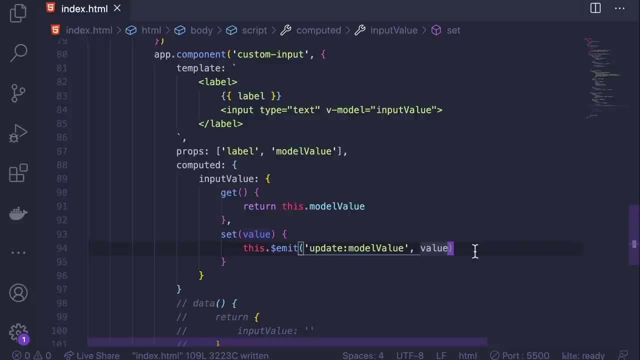 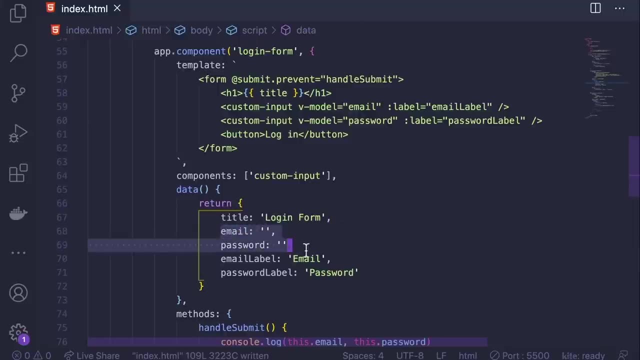 I could also pass a function from the parent to the child And the child can call functions in the parent, And then I could update variables in that way too. There are also other state management solutions, And we will explore all of these different options later. 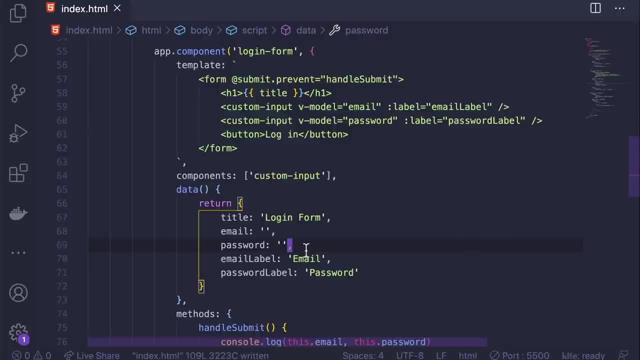 I just wanted to give you an initial taste of how this can be done in Vuejs, and specifically in Vue version 3.. The syntax has changed a little bit, So in this video we've gone over custom components, composing components together, importing them into each other. 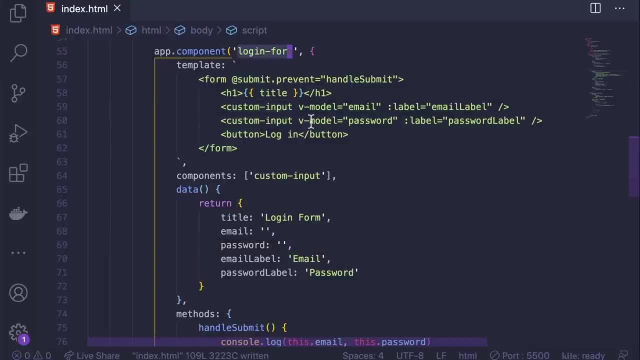 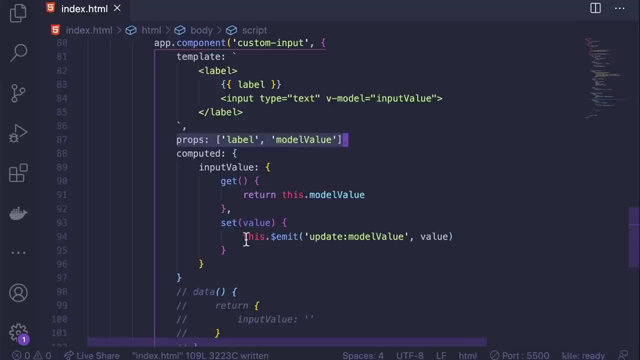 like we are with this custom input into the login form component. We also talked about using props, passing data from the parent to the child and then being able to set data by emitting an event that the parent can listen to and passing it a value. 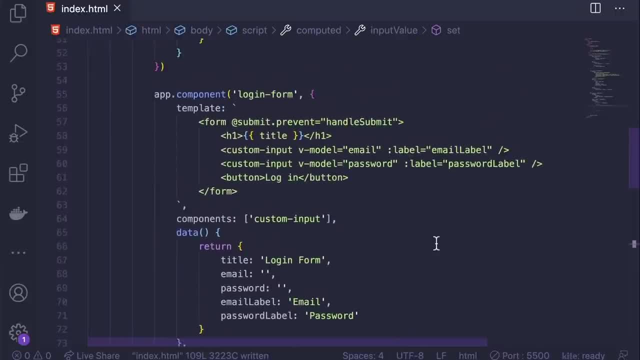 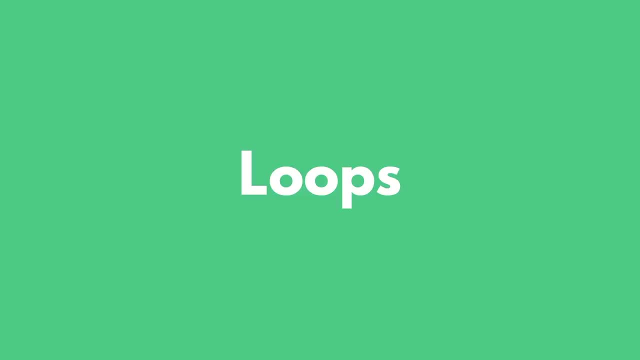 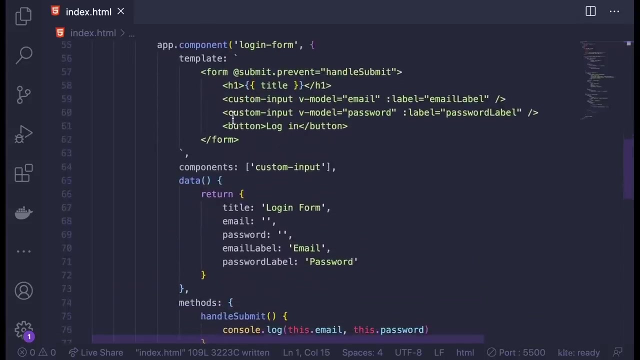 In the next video we're going to talk about loops in Vue. to simplify our syntax here with having multiple of the same component. Now let's talk about loops. here We have two of the same component, these custom input components, and I would like to just 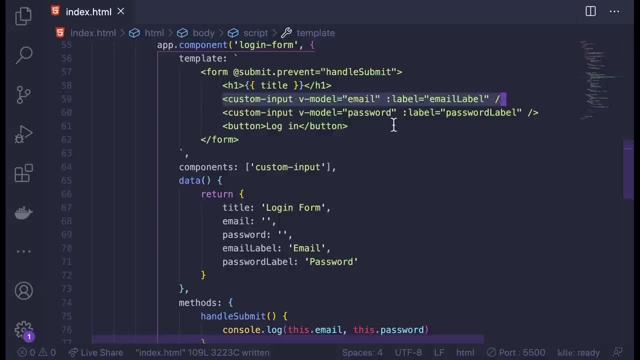 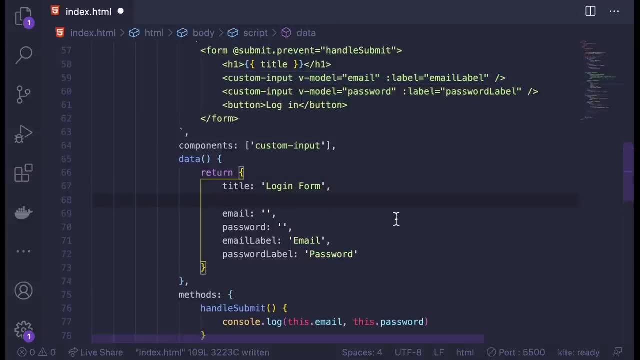 be able to loop through as many of these components as I want. To do this, I need to add an array in data here. This array will have all of the information for each input here, including the variable that I want to model to the label name. 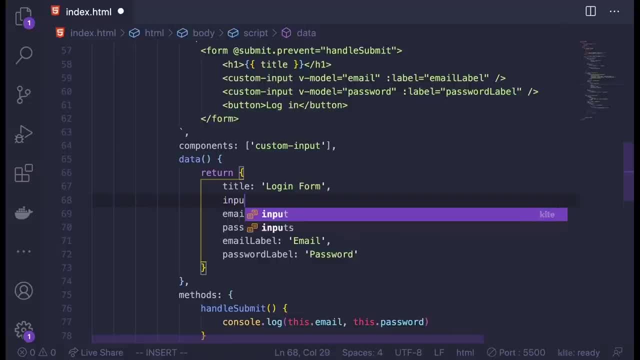 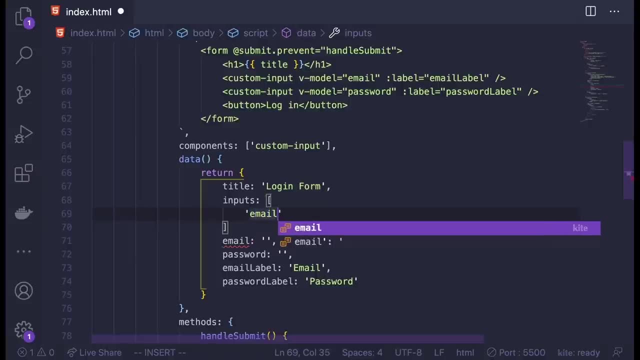 and I'm also going to add a type. So I'm going to create an array here called inputs and, just to demonstrate really quickly, I'm going to add just some strings here, like email password and, let's say, name. So if I wanted to display, 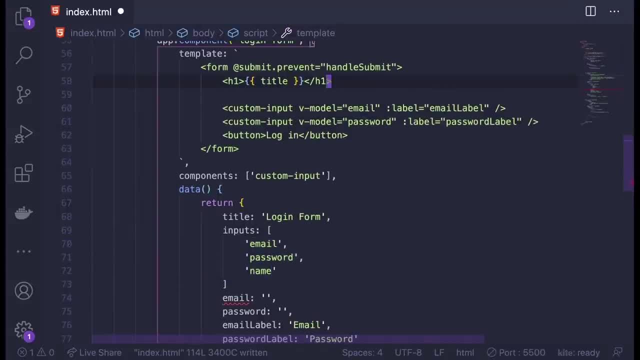 all three of these strings inside the template here. I'm going to come back to looping over the form in a second, but for right now I'm just going to create a p tag here and I want to show each one of these strings inside its own paragraph tag. 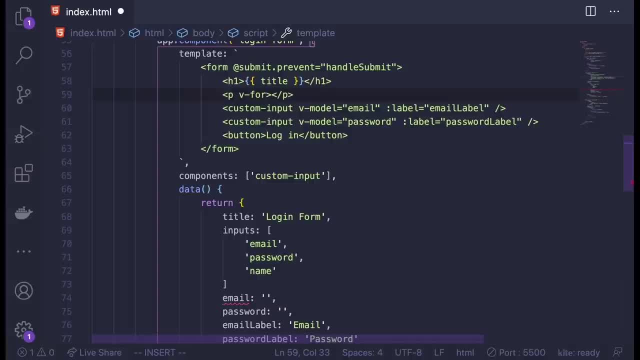 so I'm going to create a loop for these. I'm going to say: v4 equals, and then I need to pass in the array here which is called inputs. so I'm going to start the inputs array. now this is a for in loop, so I'm going to have to create a variable. 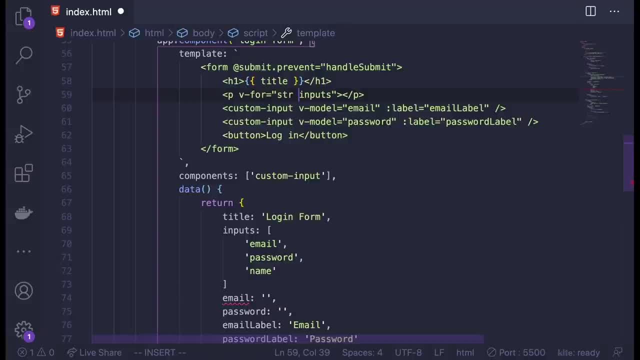 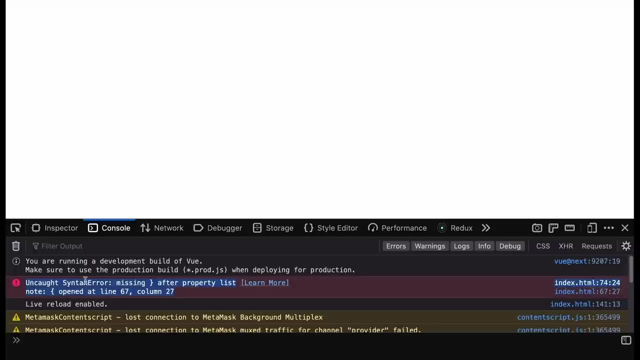 that I can use in the iterations. so I'm going to say for str, short for string, in inputs, and now I have access to this string variable each time through the loop and I can basically just display it in a variable. now, right, so it is complaining that I made a mistake in my syntax. 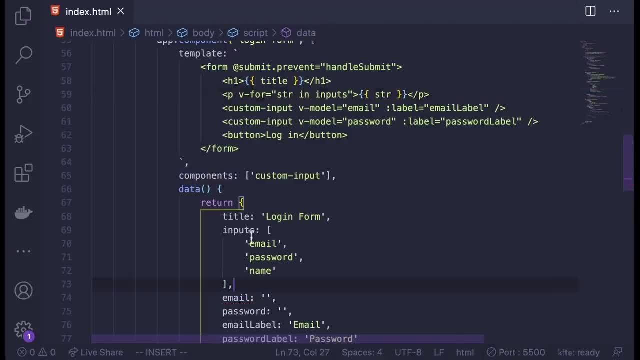 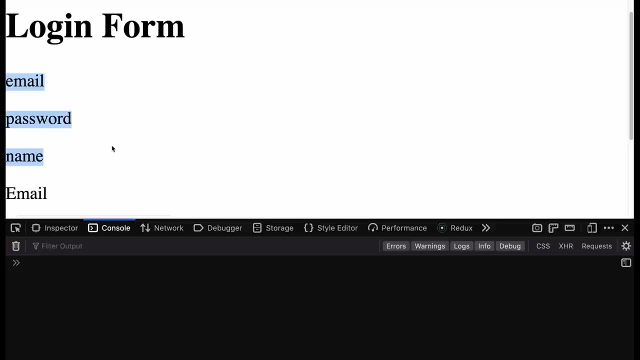 and of course that is because I didn't put a comma after my array, and now you can see that these top three here are strings that are displayed in a paragraph tag. of course they are so big because I am zoomed in so far, but they are displaying properly. 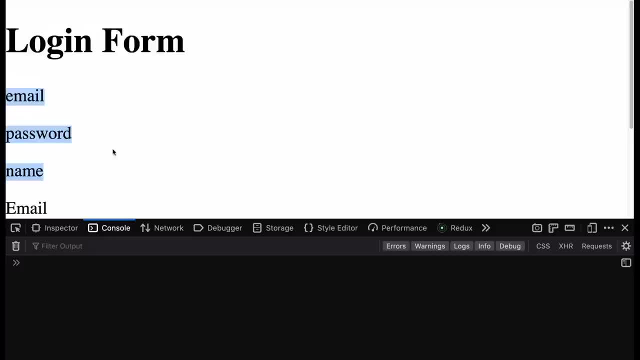 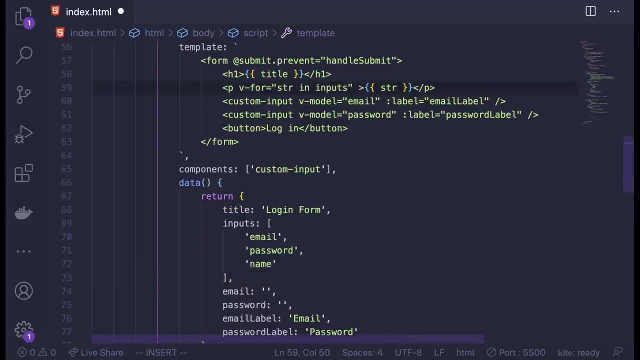 and that is basically how you use a loop in Vuejs. I am missing a prop here that I need to add. whenever you do a loop, you have to add a key prop here, and this key has to be unique on each iteration of the loop. now the reasons for using this. 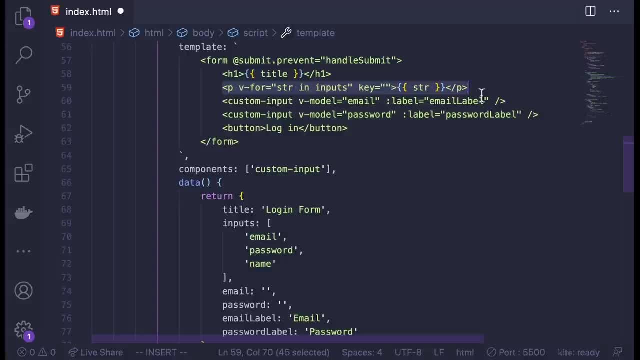 key prop are a little bit more advanced, so I am not going to go in depth on it in this video, but I just want you to understand that it is good practice for you to use a key that will uniquely identify any elements that you loop through in your Vuejs. 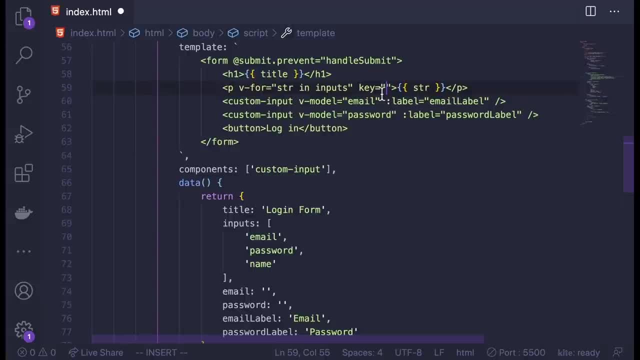 templates. this can help with performance and preventing bugs in your applications. and when you move into programming a more structured Vue application with Vue components in their own files, you will see that your linterer and code editor will pick up on it if you don't have a key. 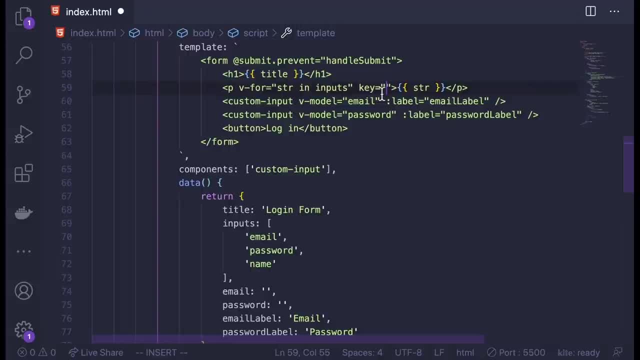 value here and it will give you a warning and ask you to add one. so we have to have a key to give a unique reference to each one of these paragraph tags. we are adding into the template. now what I can do, since the names are unique here, each string. 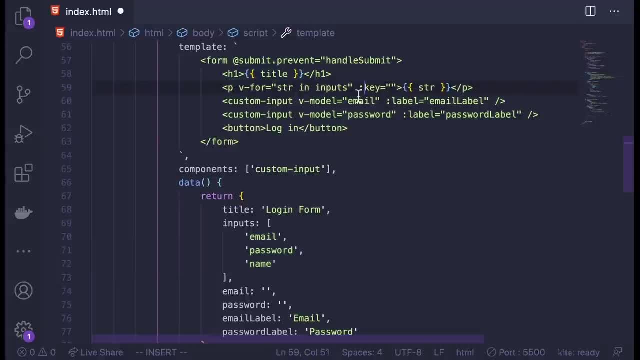 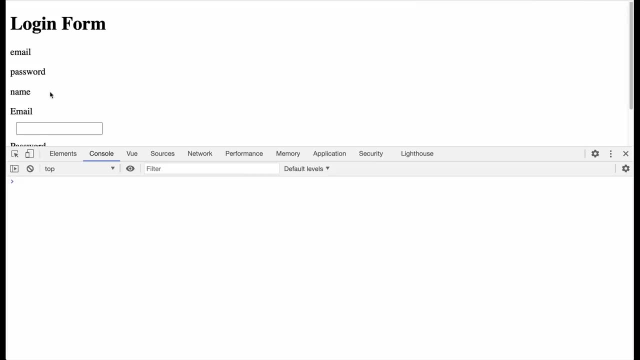 is different, so I can vbind to key the string variable str. this is a really simple Vue application, so you basically don't notice a difference in the browser, but Vue can see that there are keys attached to these elements. now I want to point out, though, that one more way that you can create: 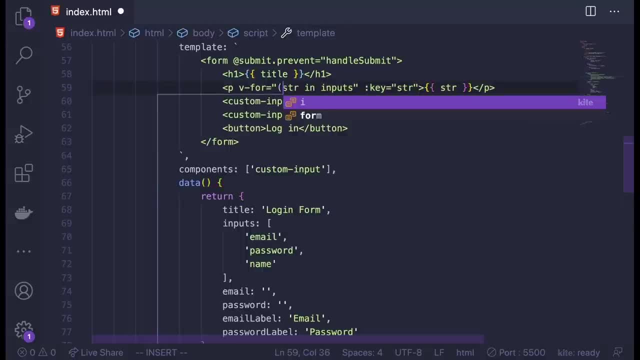 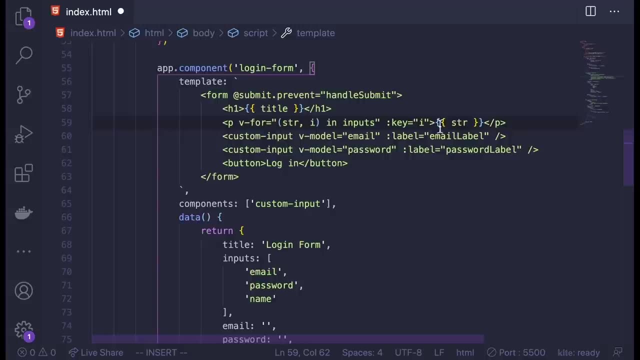 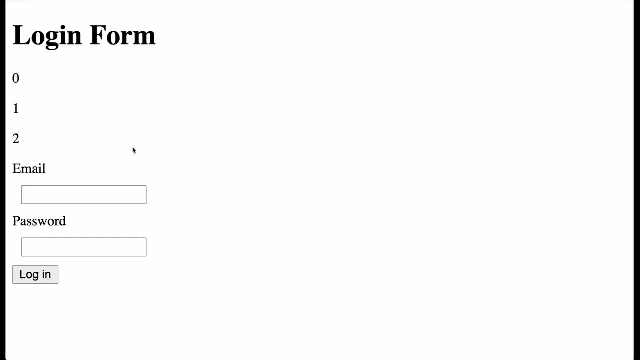 this unique key every time through the loop is you can actually get an index through each iteration of the loop. you can get i here and then use it as your key and if I print out i, you can see that i is the index of each iteration in the loop. 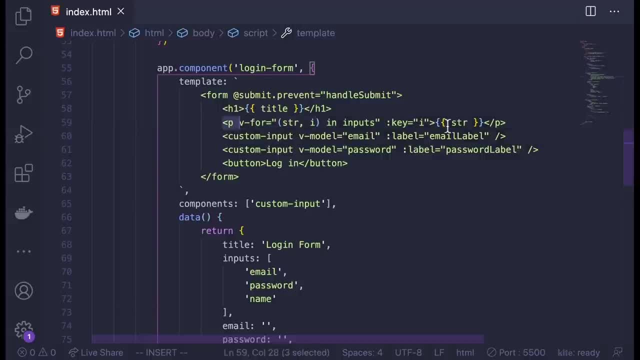 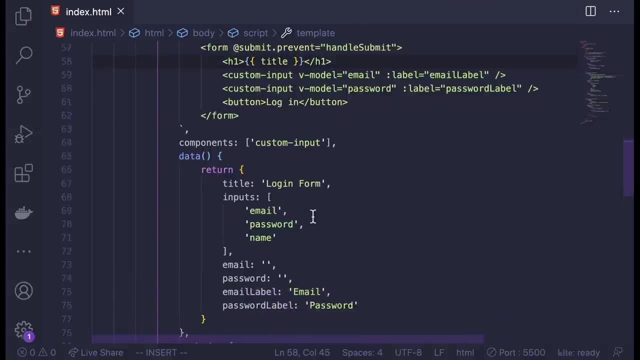 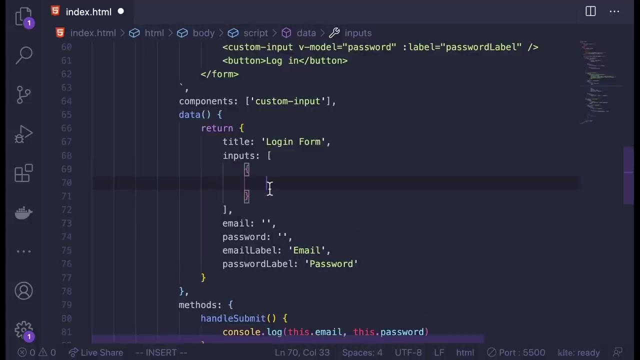 I'm going to put that back as string. so this was just a demonstration, of course. so I'm actually going to get rid of this whole p tag here, and what I really want to be putting in inputs here are objects, for the information that has to do with each input that I want. 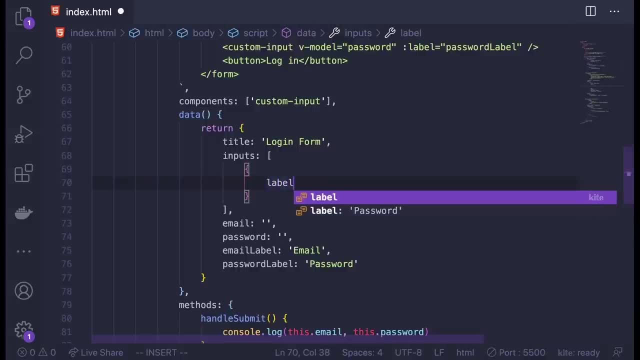 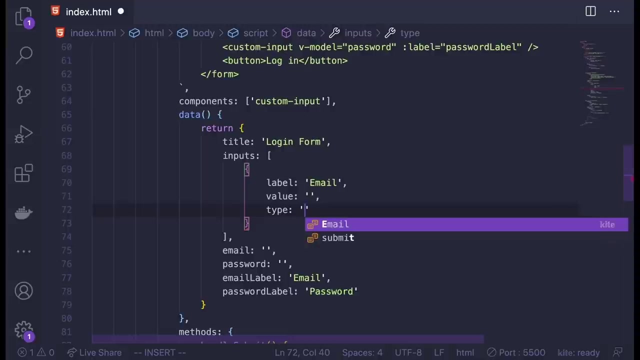 so the first one: let me put a label here and I'm going to say the label is email. I'm going to create a value here and this was what I'm going to vmodel to, and then I'll go ahead and add a type. so let's say type. 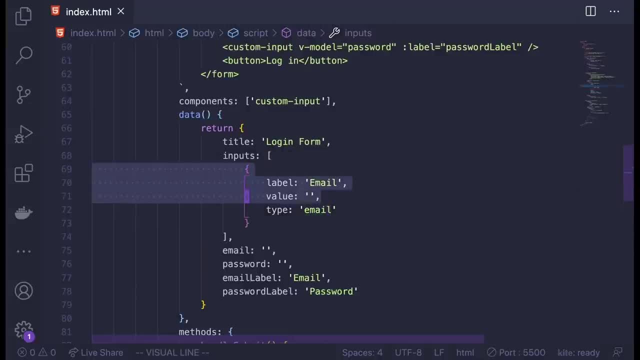 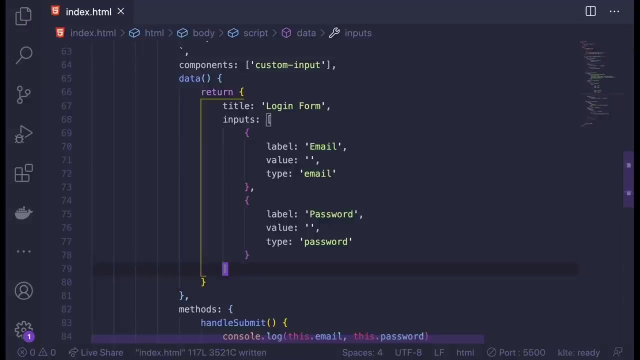 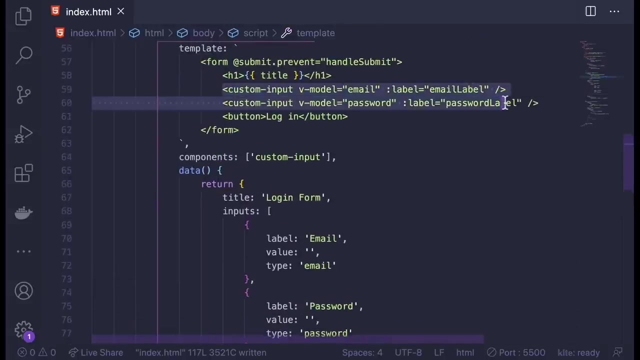 is email, and I'll do the same thing for password, and I can get rid of those now. alright, so now my application is broken because I got rid of all the data that I had been passing into these custom inputs and actually I'm going to get rid of one of these custom inputs. 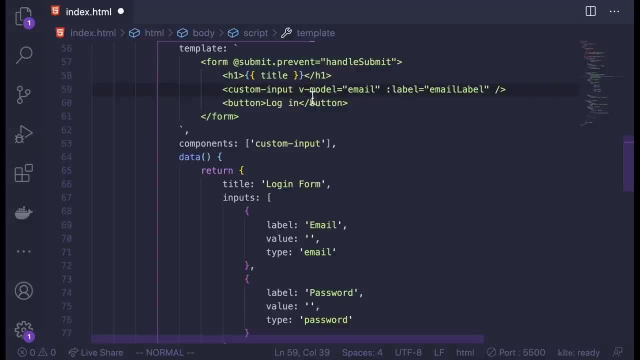 because now I'm going to be looping over just one, and it will create one for each iteration of the loop. let me clean this up a little bit. put these on separate lines, and so the first thing I want to do is create a v4 here and this: 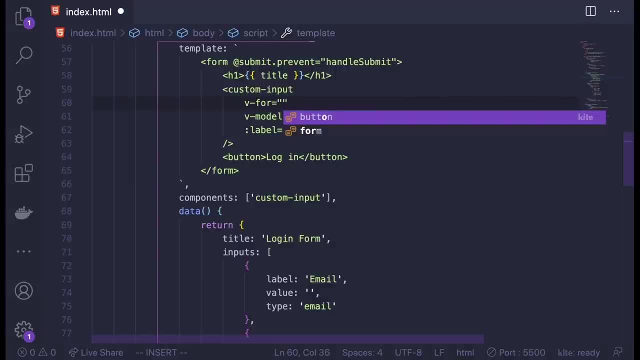 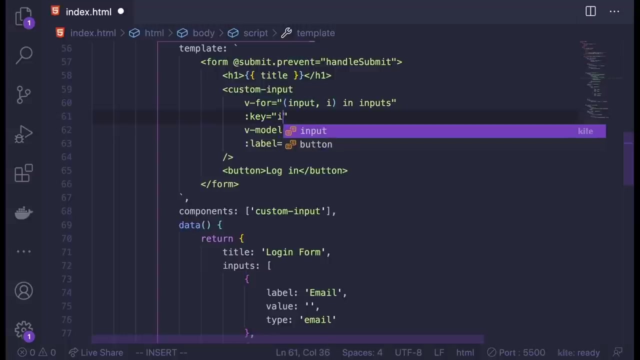 v4 will loop through inputs, just as I did before. I'm going to say for inputs in inputs, and I'm actually going to get the index here really quick as well- and then use a key: I'll vbind the input index. so now I can't. 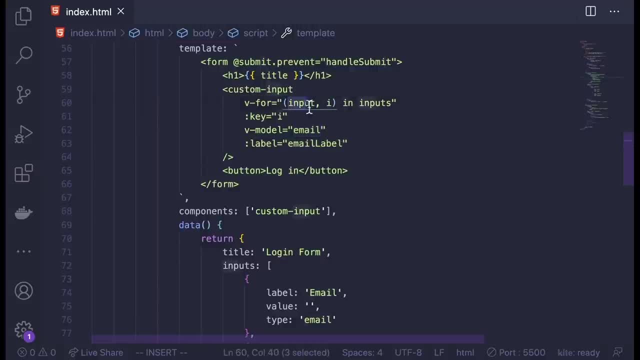 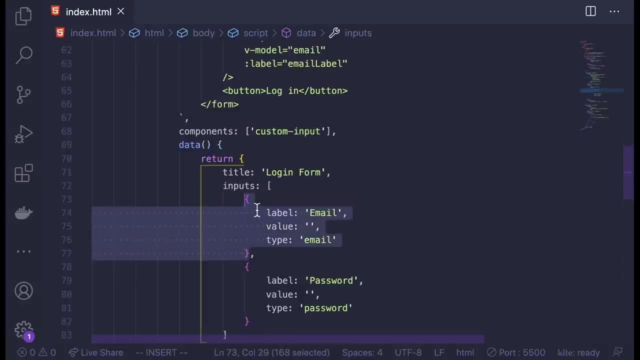 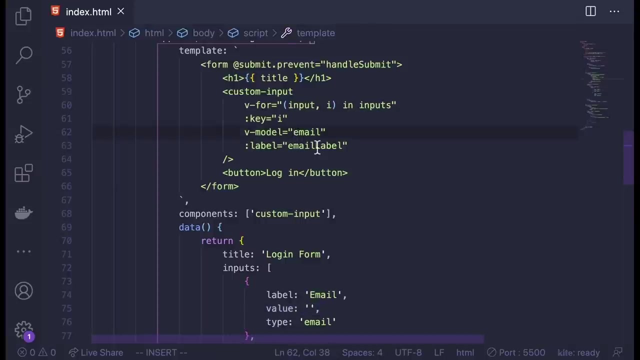 vmodel email. I need to vmodel based off of this input object, which is each object in this inputs array. so I'm going to have to vmodel input dot value here to model it to the value. so I'll do input dot value the label also. I'm going to have 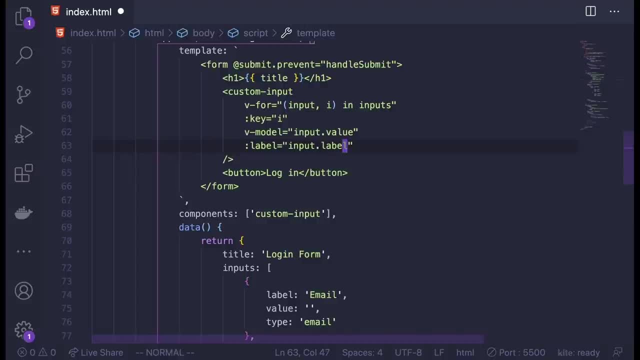 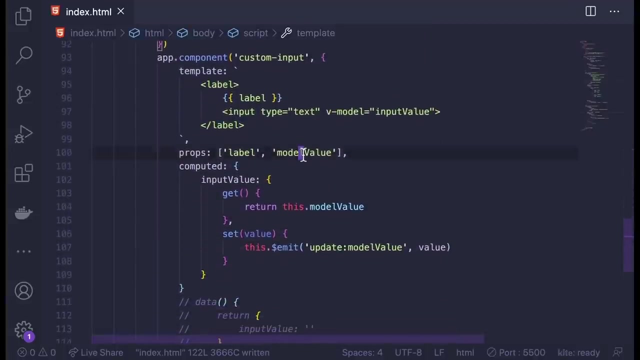 to do input dot label and now I do have a type, so let me vbind a type as well, and I'm going to do input dot type. so that's one thing that I need to update in this child component. now I'm still accepting that model. 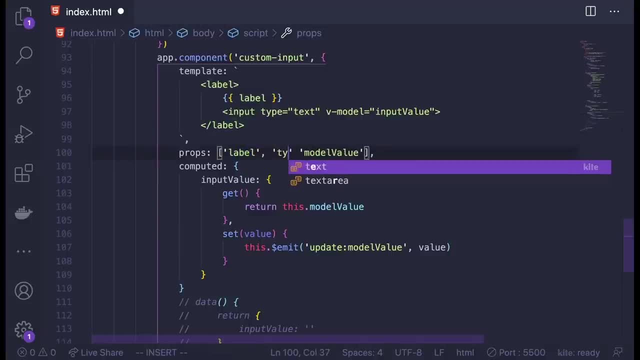 value prop and the label prop. but I also want to accept a type prop now and instead of doing type is text, now I have a prop from the parent based off of which component it is in the loop. so now I'm going to bind this so it can take a variable. 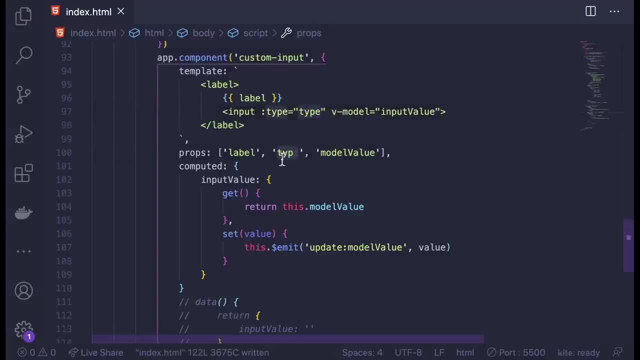 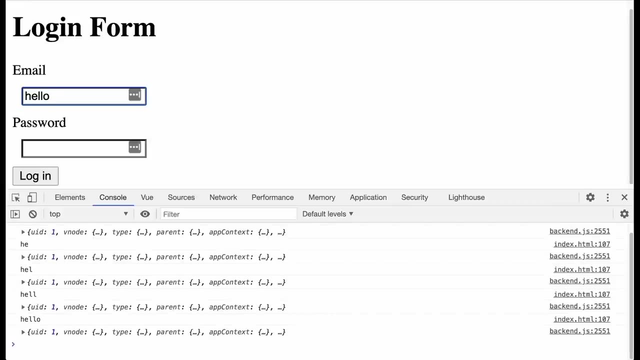 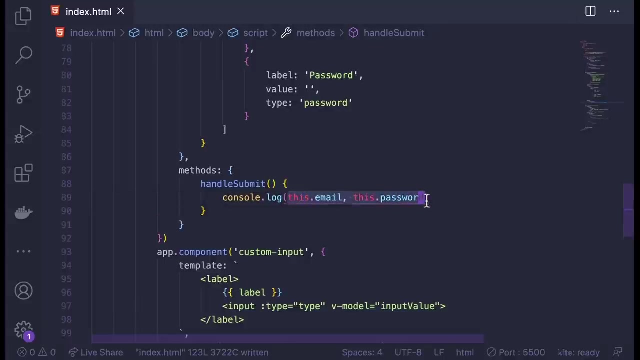 and I'm going to say type, which will refer to whatever prop I've passed in. so I'm going to come to my form here and I'm going to type in: and I actually forgot to change the logging here for handle submit. so I don't want to over complicate. 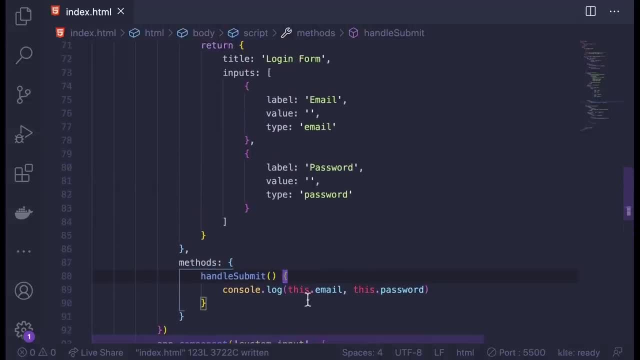 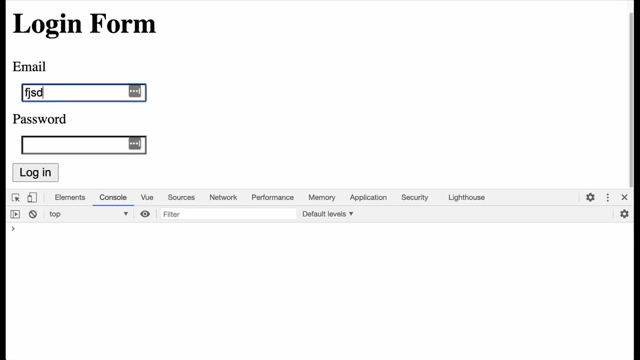 things for this example. so what I'm going to do is just delete this and log out this dot inputs of zero and that value, and then this dot inputs of one and then that value, and this should fix my problem here. let me just type something in. and it's complaining that I don't have an 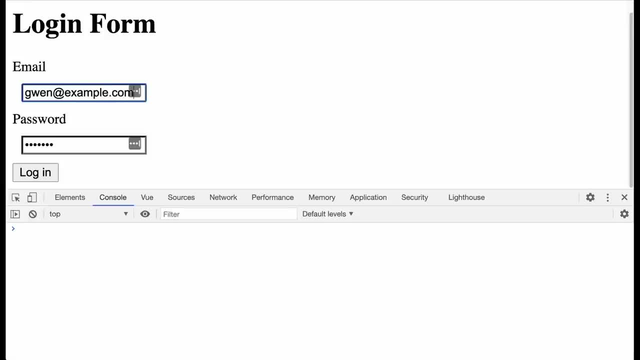 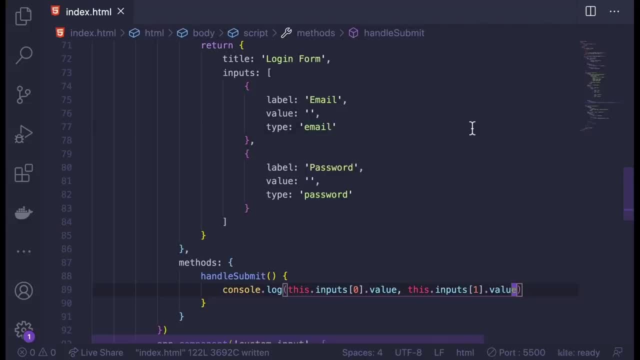 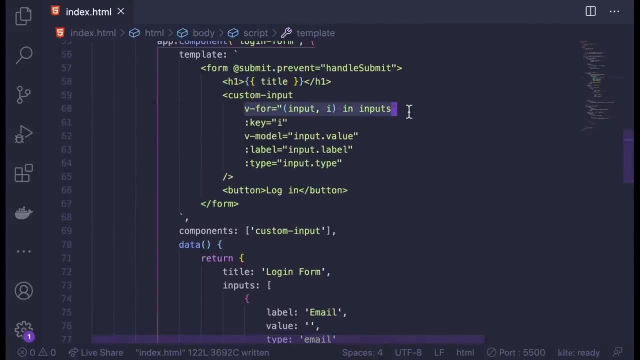 email address. so I'm just going to type in a fake email log in and you can see that it has my correct log in information. so this is the basics of how to handle loops in Vuejs is you can use V4 either on regular HTML elements. 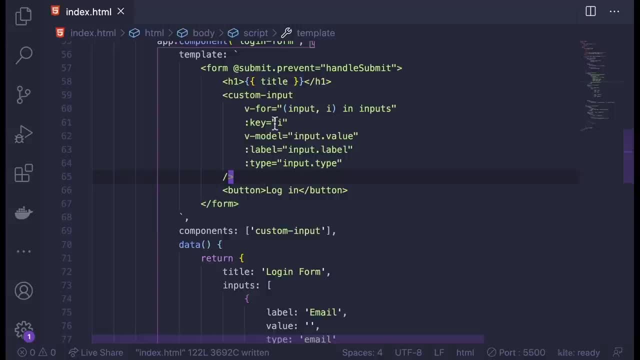 like an H1 or any custom components that you make as well. this is very commonly done with card components. if you see a website like Pinterest, how it shows all those different little boxes with pretty photos in them- if that was built in Vuejs it would be doing. 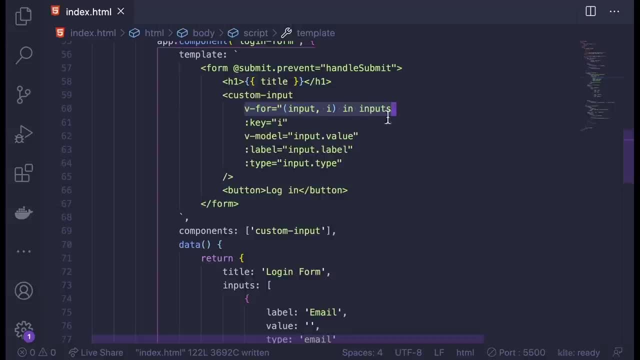 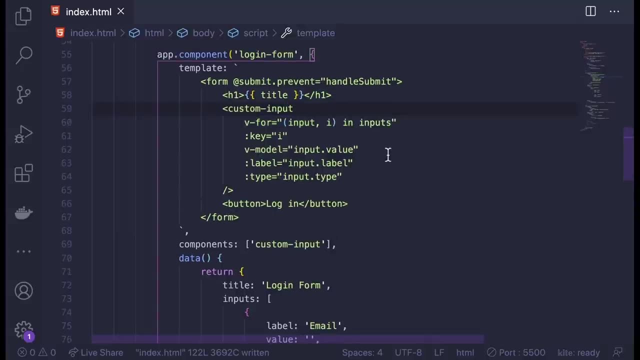 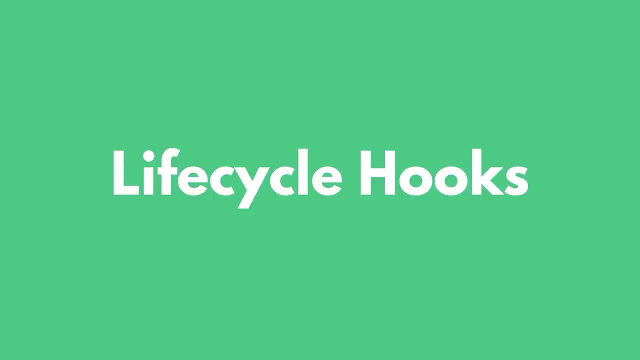 a nice V4 loop over all of those data objects that make up all of those Pinterest cards on your Pinterest wall. the last thing we need to look at before we get into the demo application is lifecycle hooks, so we will cover those in the next video, another important concept. 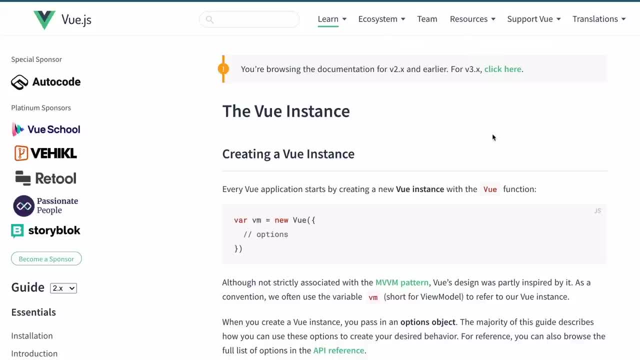 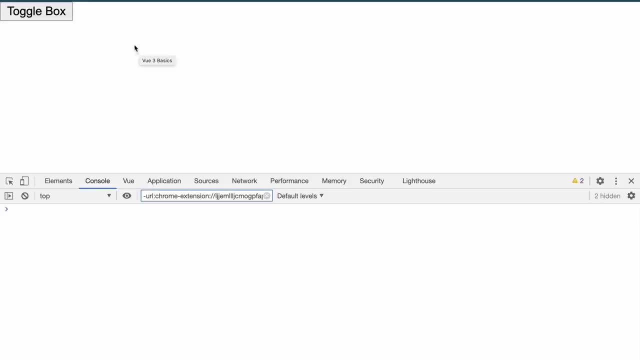 in Vuejs is lifecycle hooks, also called component lifecycle hooks. so what is a hook and what are component life cycles? to understand this, I made a quick demo similar to the demo that we started off with in this course. I can click the toggle box button and a box appears. 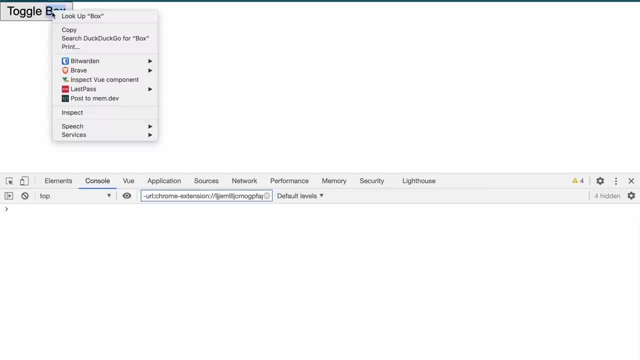 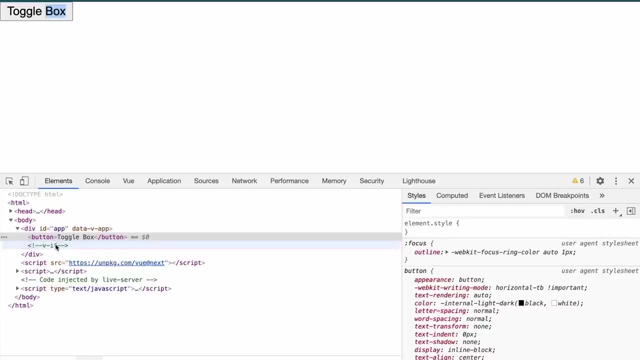 now I'm using a VIF to take this box, add it. you can see it was added to the DOM and if I click again, it was completely removed from the DOM. here, that whole process of going into the DOM and then finally leaving the DOM, that is the lifecycle. 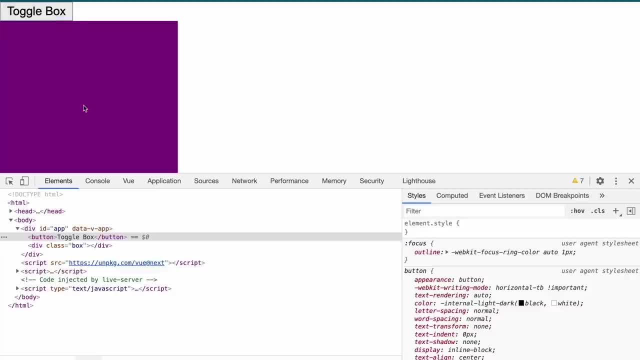 of this box component that I have now. sometimes things might leave the DOM because you navigate to another page, or because something is coming into Vuejs via scrolling, or because you are hiding and showing something like this example. in any case, you can use something called lifecycle hooks. 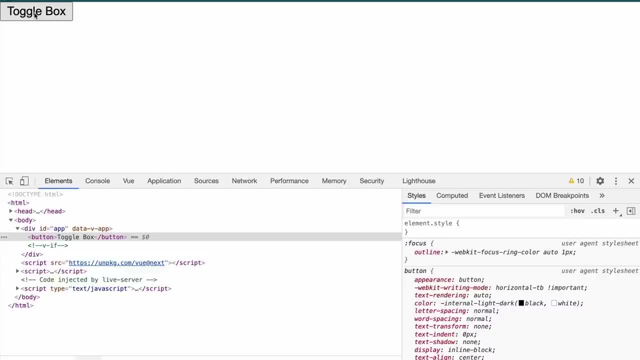 a hook is just a function that will be triggered to run at a specific point in the lifecycle of a component. for example, it's a function that will be called right when this purple box appears on the screen or right before it leaves the screen. if you look at the Vuejs, 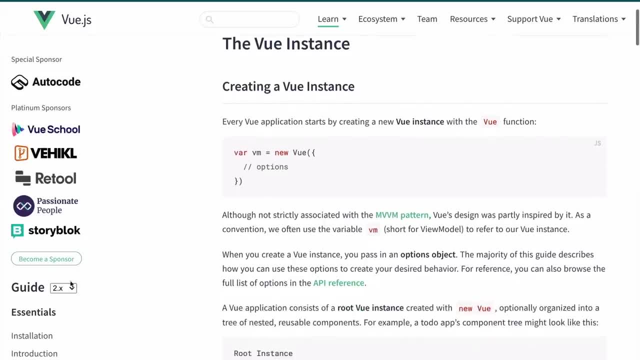 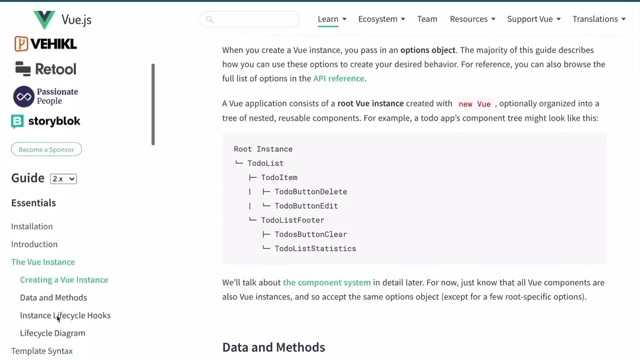 documentation. now, this is the version 2 documentation here, because they don't have what I'm going to show you yet in the version 3 docs, but it is the same thing. so I'm under learn guide and then, if I scroll down on the sidebar, I'm at the Vue instance. 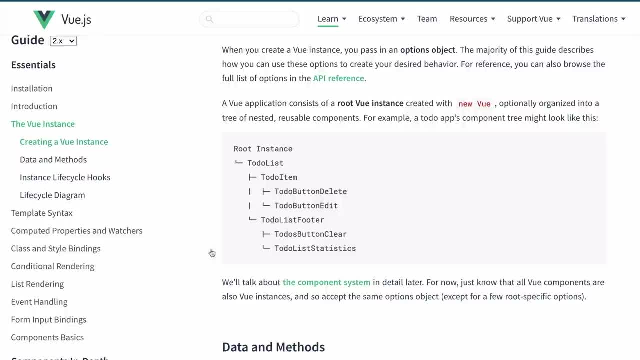 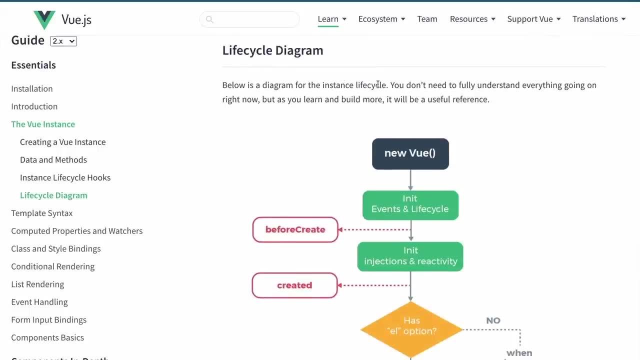 and creating a Vue instance, and I can actually click on the lifecycle diagram here. so this is a diagram, like it says, of the instance lifecycle of your Vue instance and, like it says, you don't need to fully understand everything that goes on right now, but it is a useful reference. 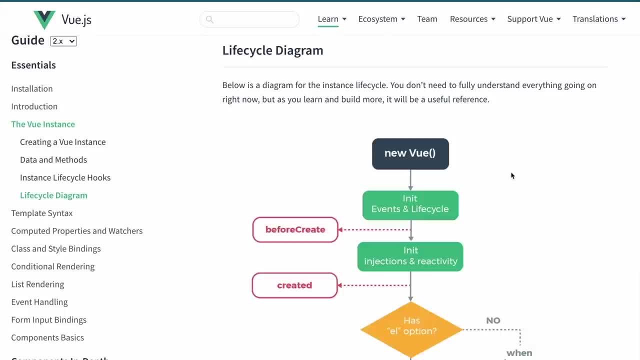 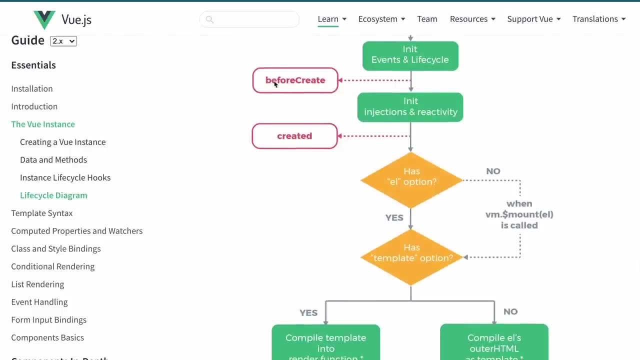 and this chart isn't just useful for your Vue instance, but every single Vue component will have access to these lifecycle hooks. so you can see these two up top in the red. all of the boxes in the red are the lifecycle hooks you can see before create and 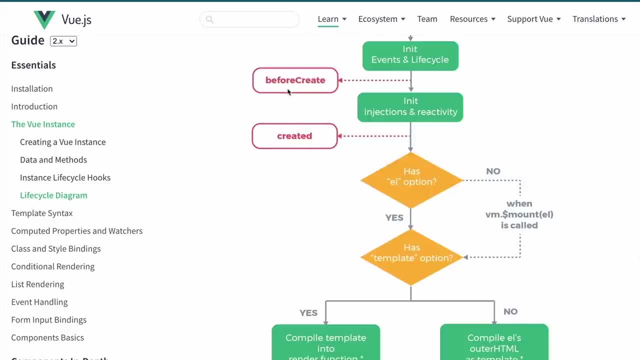 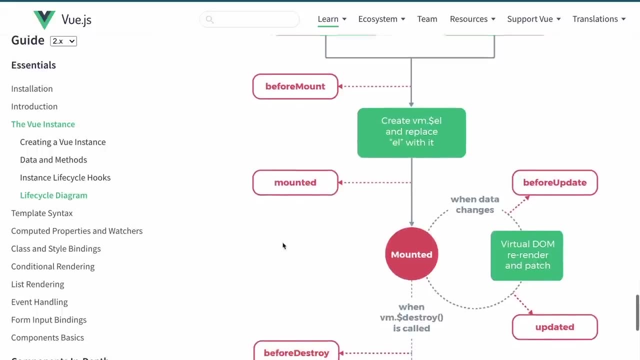 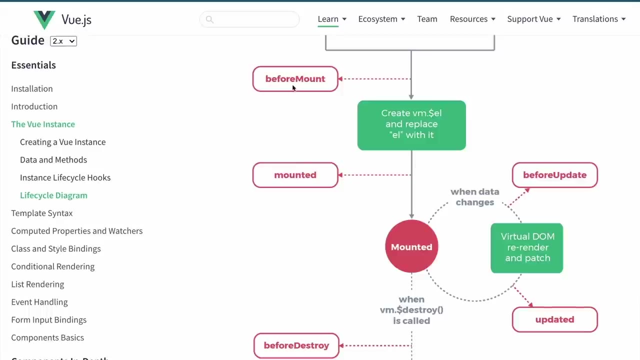 created. these hooks will be run right before and right after Vuejs has initialized your component. now the next two before mount and mounted: before mount is run: right before your component is mounted to the DOM, and mounted is run as soon as your component is mounted to the DOM. 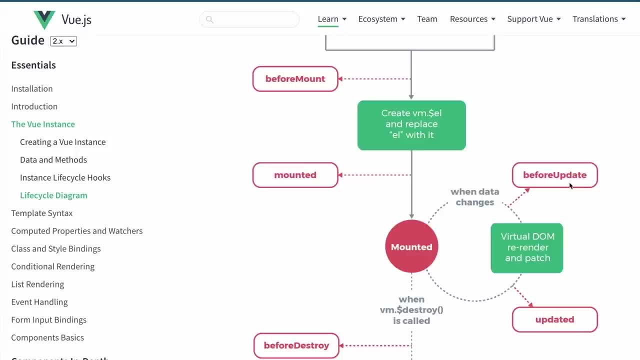 components can also go through updates. so before update and updated, like it says here, this will happen or these updates will be triggered when data changes on your component. so any of those data variables that you create, if you're incrementing a number or changing some kind of value, then 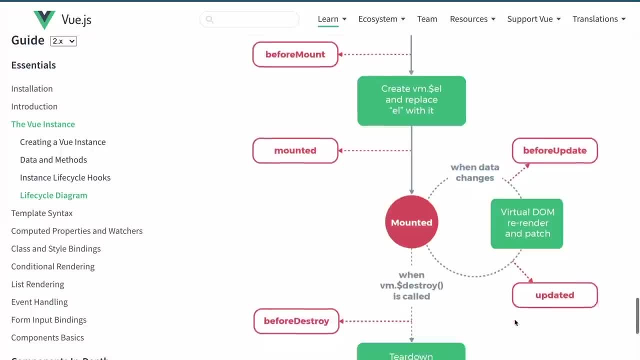 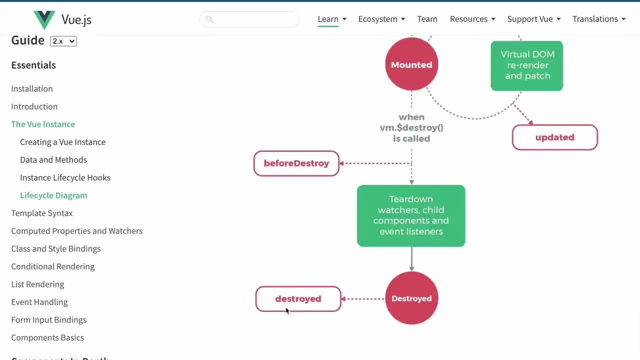 created and before update will run. and then when your component is going to leave the DOM now here it says: before destroy and destroyed. now this terminology has been updated for Vue 3 for these two lifecycle hooks. so if we go to the Vue 3 documentation now and we're on. 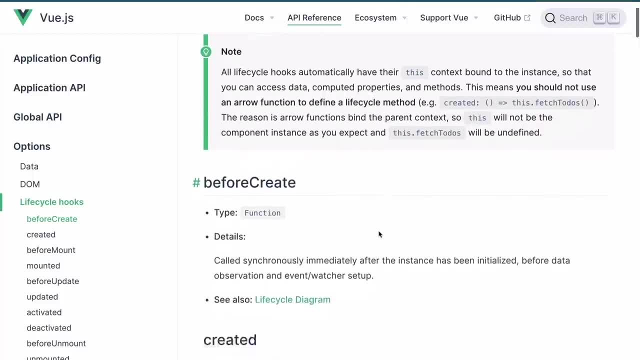 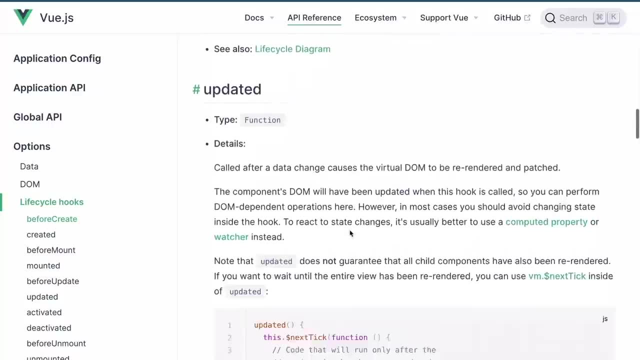 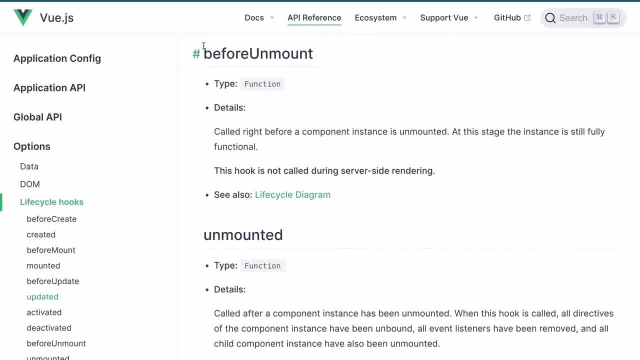 lifecycle hooks. here I'm going to scroll down so you can see: before create, created, before mount, mounted, before update and updated. I'm going to skip over some of these and now you can see it's before unmount and unmounted which is in place of before destroy and destroyed. 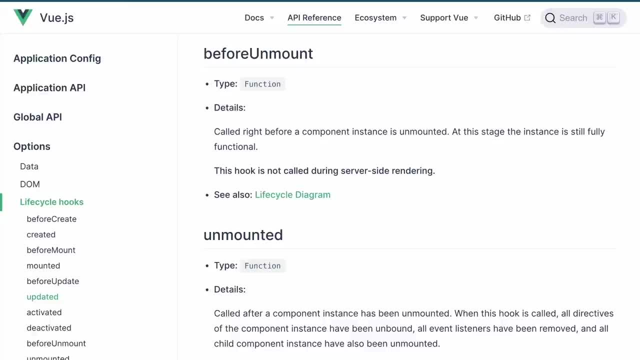 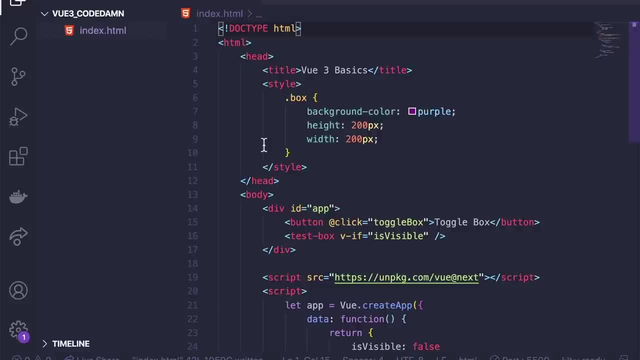 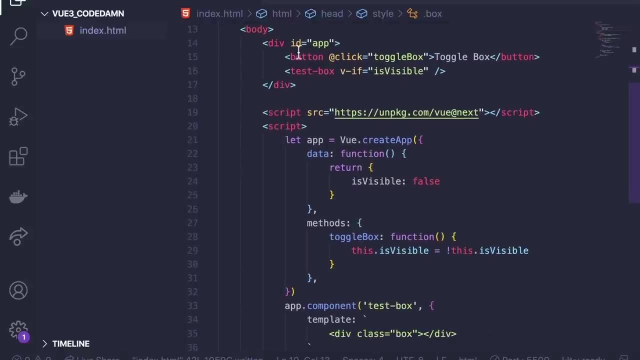 the lifecycle hooks function exactly the same way. they've just been renamed. I hope this will become a little bit more clear as we look at a demo. so in the code you can see I have the same box that we used before up here and here is the. 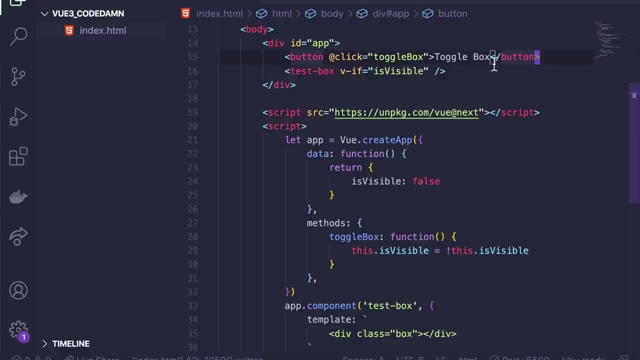 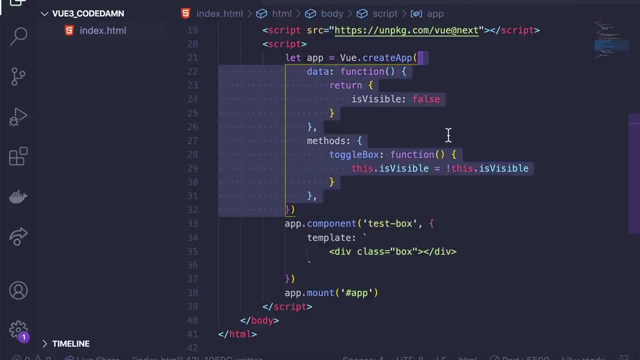 toggle box button inside of my Vue template. but this time I do have a special test box custom component that I made which is toggled based off of a vif. so this is my main application and the options object with my is visible variable for whether or not the box is visible. 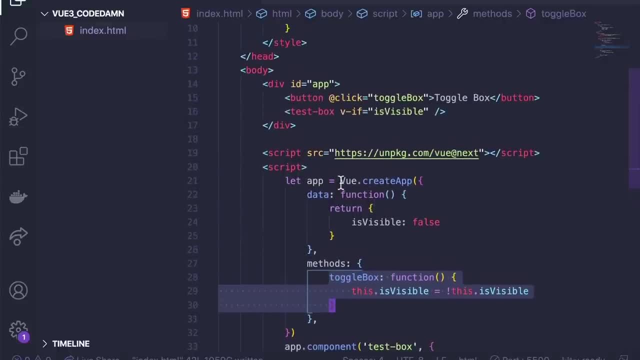 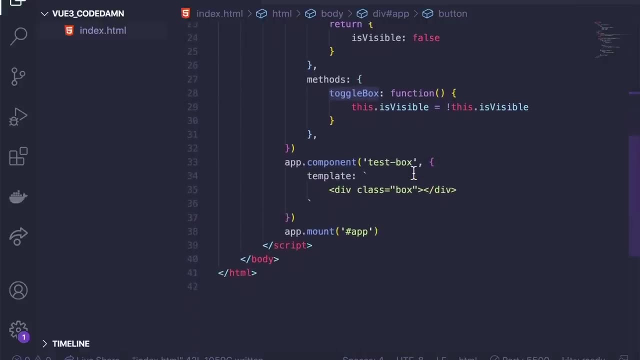 and then I just have a toggle box method which I call when I click this button. so again, this is pretty much the same thing that we did before, except for this new component. here I put the box in its own component now, now that we've learned about composing components, 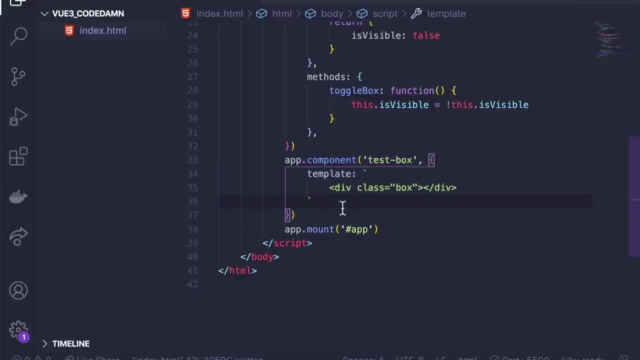 and I'm just going to add some lifecycle hooks here really quickly to illustrate when these are called on the component lifecycle. so I'm just going to add a couple of them here. I'm going to add created and then mounted and then unmounted, and in each of these 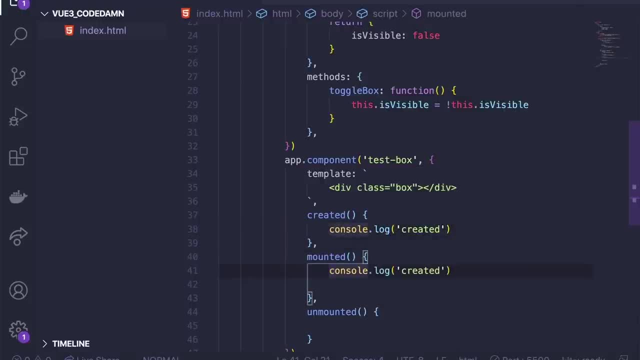 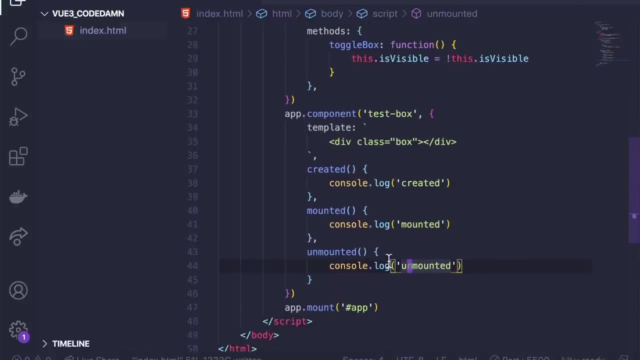 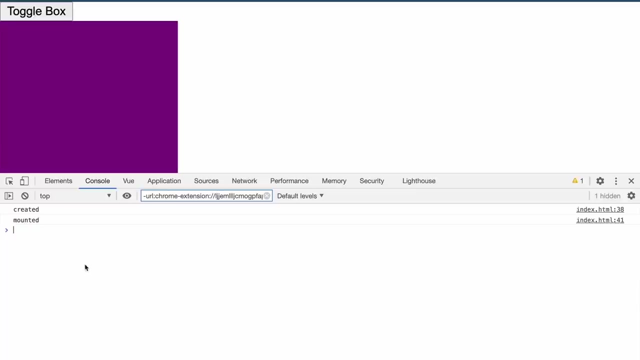 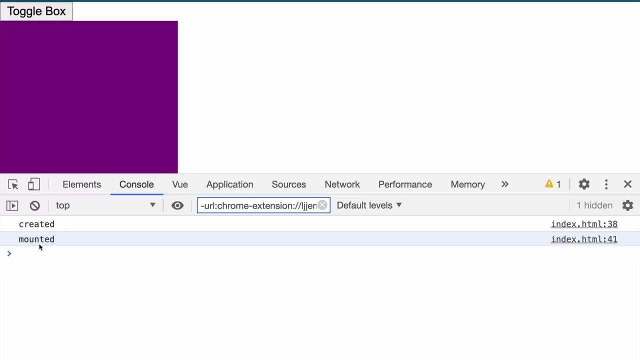 I'll put a consolelog and let's see when these consolelogs print out back in my browser I'm going to hit toggle box here and you can see in the terminal at the bottom: created, printed and then mounted. printed in the same order that we saw. 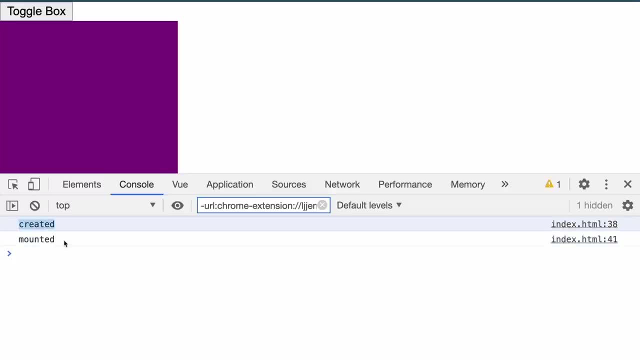 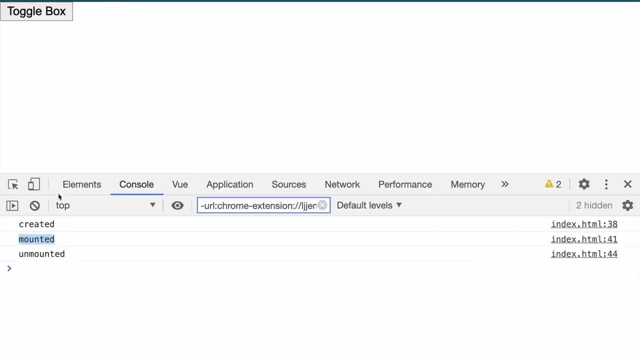 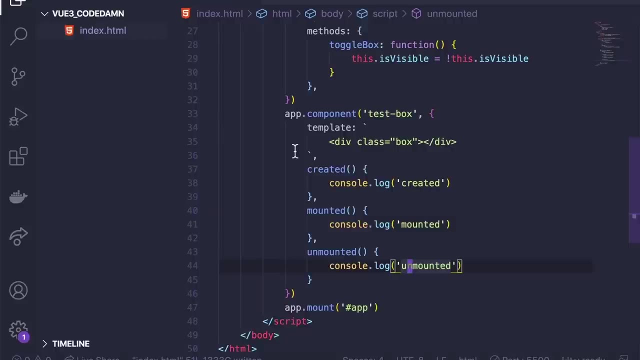 in the VJS documentation. so this one happened before and then this one happened after it was mounted to the screen, to the DOM here. now, if I hit toggle box again, we can see unmounted prints, because that is run after the box leaves the DOM. now let's look at another one. 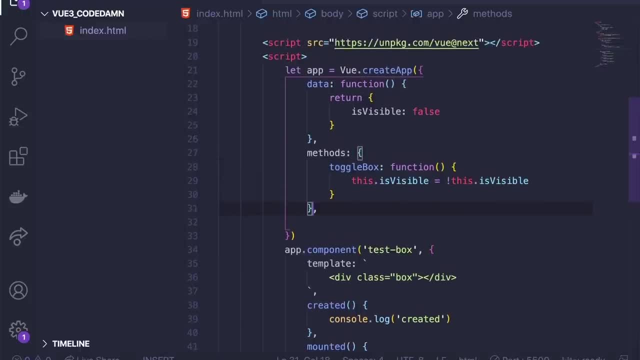 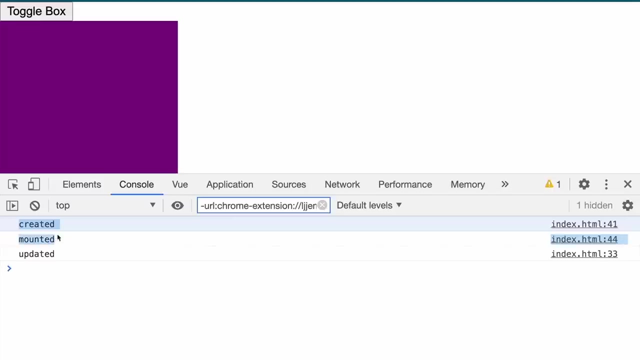 after methods here, I'm going to put a lifecycle hook on this component or on the main view instance that we have here and I'm going to try updated and I'll hit toggle box and you can see that we have created and mounted those. both print from the 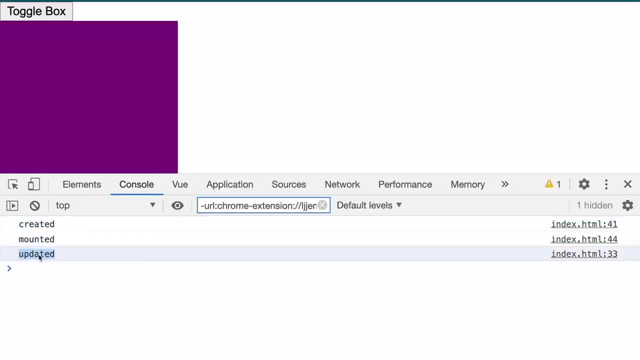 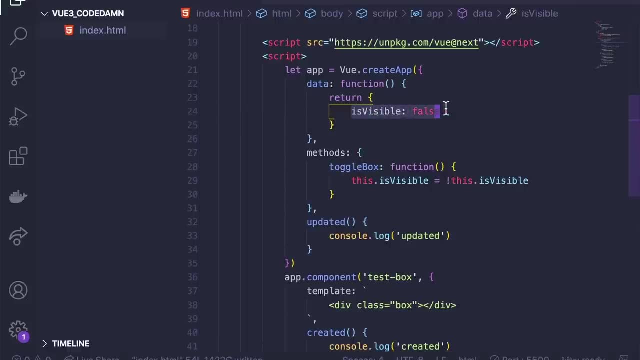 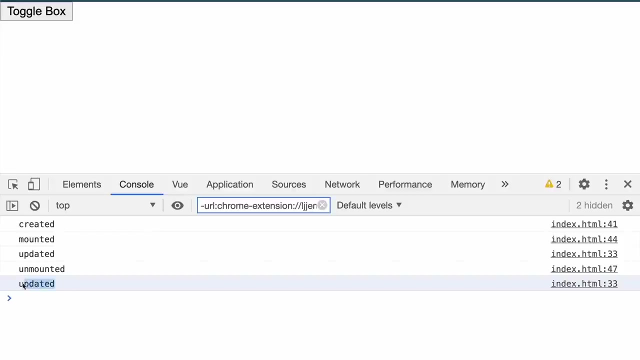 box component itself but from the main instance also updated prints. and that is because we are updating this data variable from isVisibleFalse to isVisibleTrue and so the update function is triggered on this component because our data updated for that component and if we toggle it again we can see updated is run again. 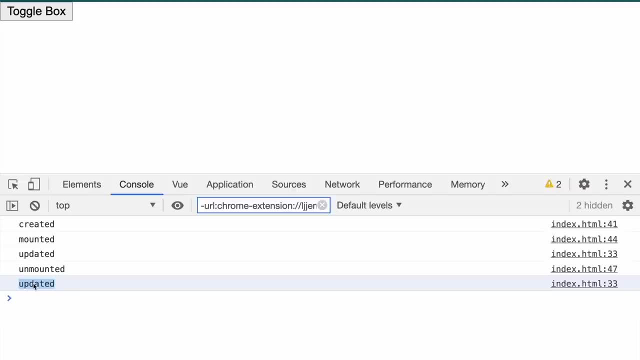 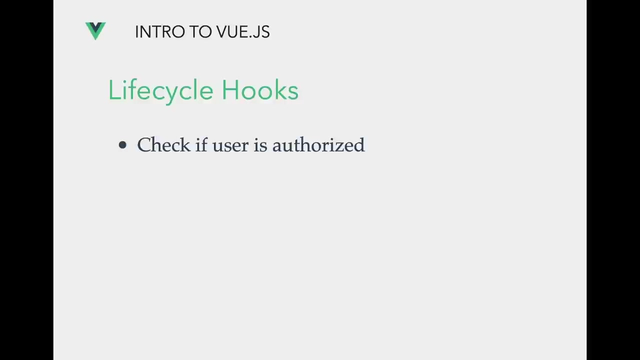 because that variable was changed to false again, so updated will run every single time the data changes. now why might you want to use a lifecycle hook? some of the most common use cases are checking whether someone is authorized to view a certain page or component. a lot of people use the created and mounted hooks. 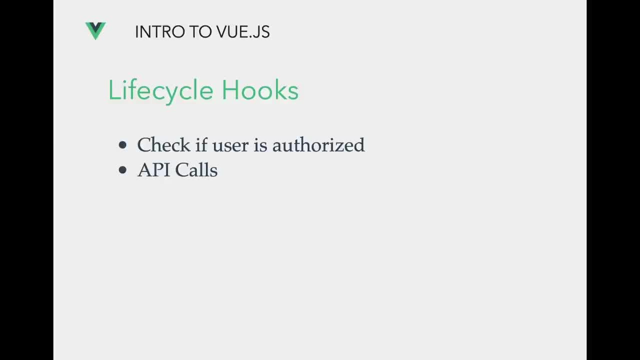 as well to pull data into their application from a backend or from in browser storage. sometimes they are also used to initialize events and then, when the component is about to unmount, you can clean up that event and you can save some data or run some kind of check. 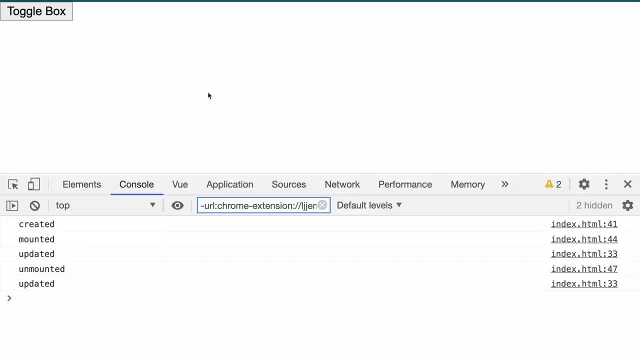 on before unmount or in the unmounted function. so those are the basics of lifecycle hooks. I encourage you to test out lifecycle hooks on your different components and see what happens when you use different lifecycle hooks. in a future course we can get into some more advanced examples. 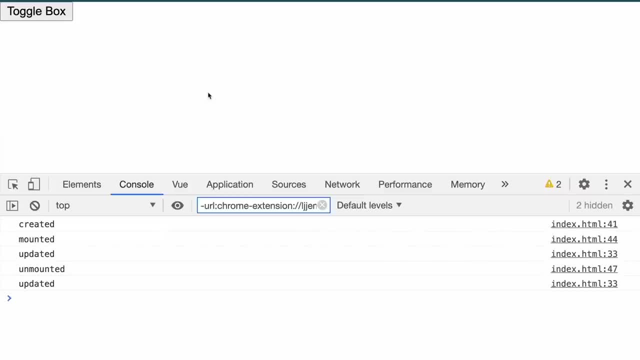 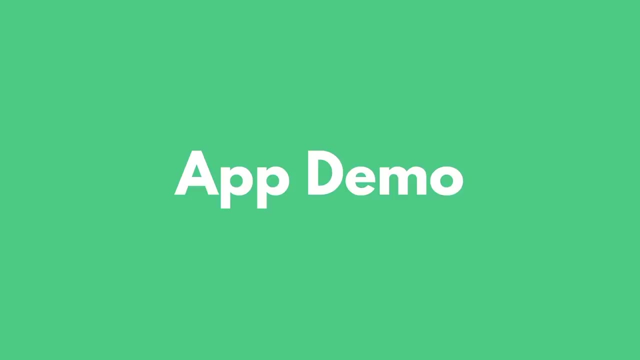 and a few of the more advanced lifecycle hooks as well that you won't see as often. so those are the basics of Vuejs. in the next video, we are going to build a Vue 3 application from scratch, starting with the Vue CLI. this time this is a demo of the application. 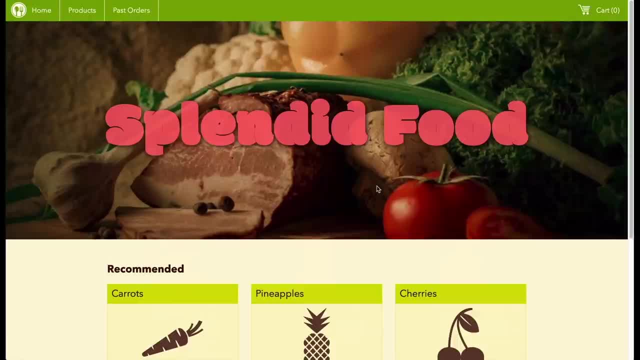 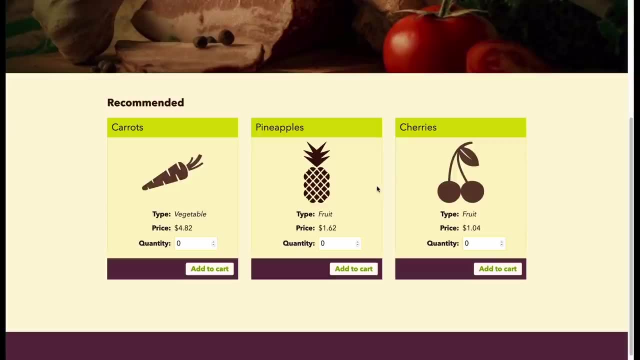 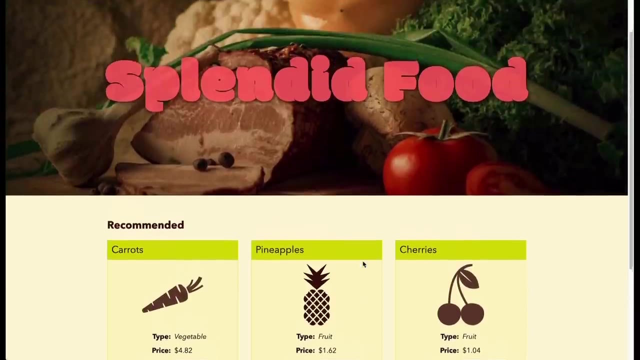 that we will be building. it's a simple shop application with a few items. now it looks like the webpage is already done, but actually it's just static HTML and CSS. so far as you can see, if I click the add to cart button, nothing happens, and if I scroll up, 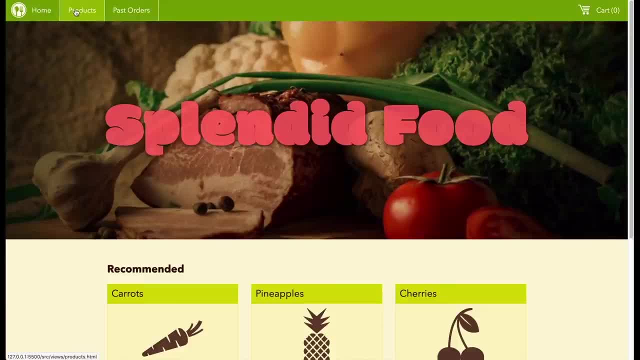 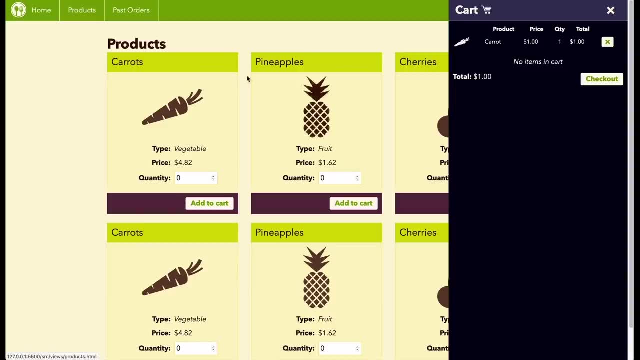 the only things that are actually functional on this site right now are these top nav links, which are just regular browser anchor tag links to bring you to another page. so this one goes to the products page and you can see I have this cart which is not functional. 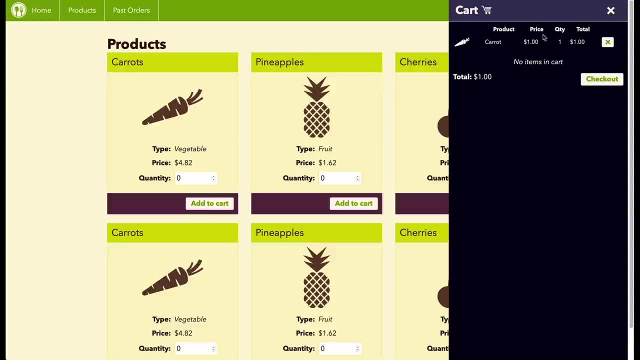 so if I click the X, nothing happens, it's just fully slid out here to demo how it will look. and if I click the X, it doesn't delete the item. I can't add items to the cart and on this page I have a past orders table. 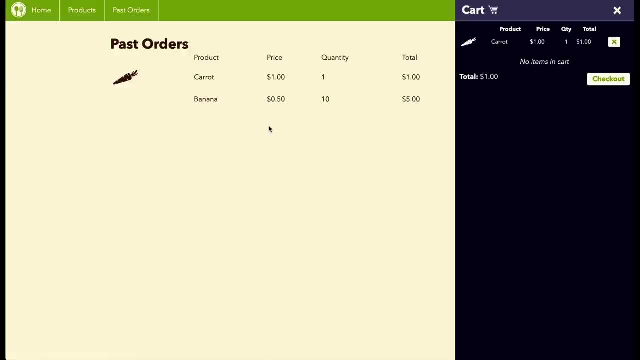 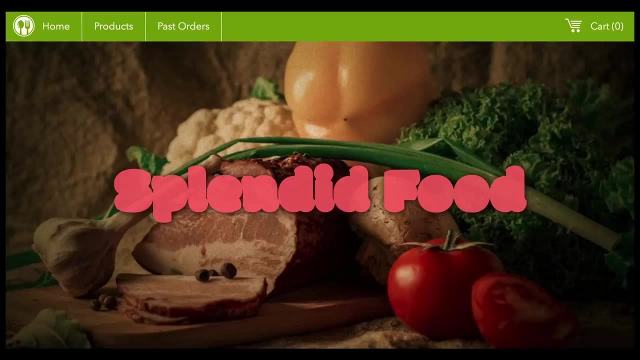 which is also just static content right now. this project is going to be a little bit different than tutorials that you are used to. we are not going to be starting from scratch with some mockups here. instead, we will be starting with a static application with HTML and CSS already coded. 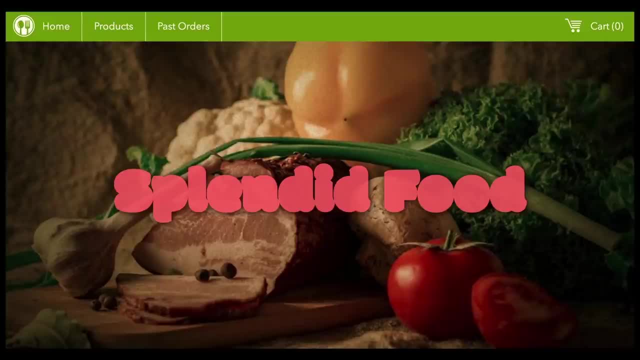 then we will figure out, step by step, how to add Vuejs into the application. this will help to give you a deeper understanding of how Vue works and how to build real world Vue applications. first I will give you an overview of the code base and then we are going to see how it looks in the browser. 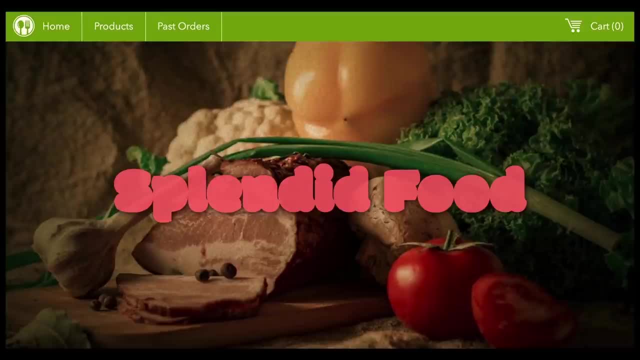 and then, finally, we will start with the Vuejs portion and implementing our own Vue code into each feature, one at a time. the goal is to eventually reach a point where it gets to be difficult to continue to code inside of HTML, and then we are going to move. 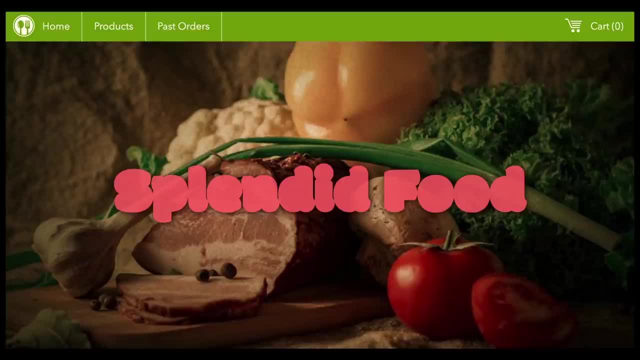 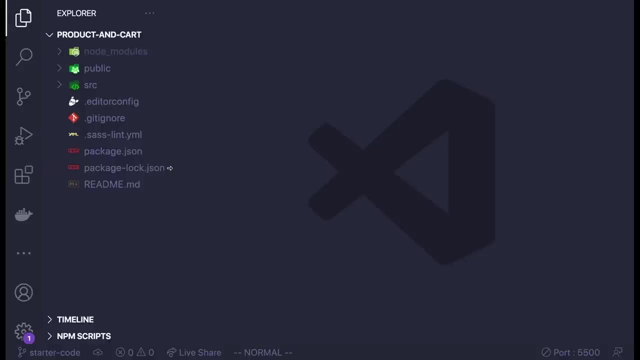 the project over to a Vuecli setup project where we will have Webpack and the full ecosystem of Vuejs tooling and libraries like Vuex and Vuerouter. so let's get started looking at the code. so I am going to start here with the packagejson. 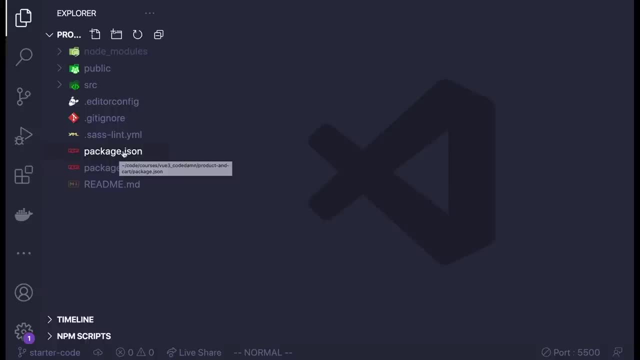 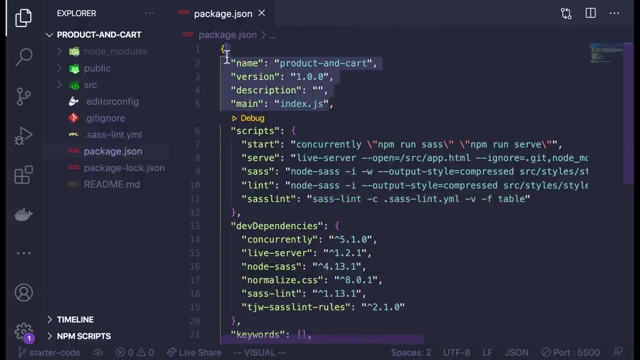 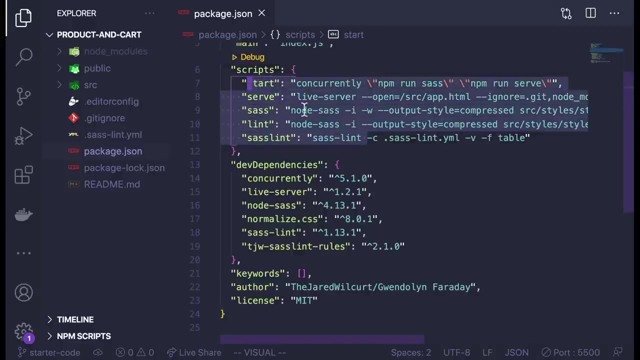 now, this is the file that is generated by NPM- you should have seen one of these before if you have worked with JavaScript- and it has some metadata about our project here, and then the scripts section, so you don't need to know what all of these scripts are doing. 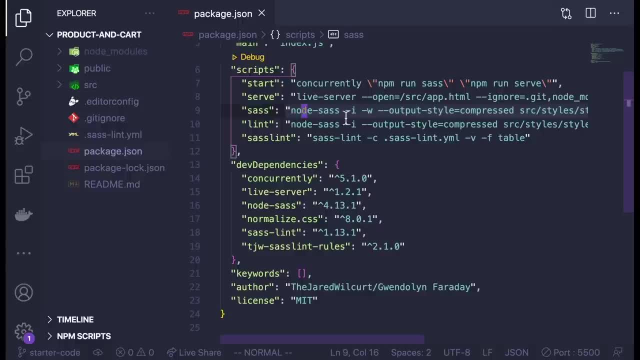 this code will be available for you. so if you want to dive deeper into each one of these, you can, but since we are focusing on Vue here, the important part is that we have this start server that compiles our styles and serves our application for us now, later on. 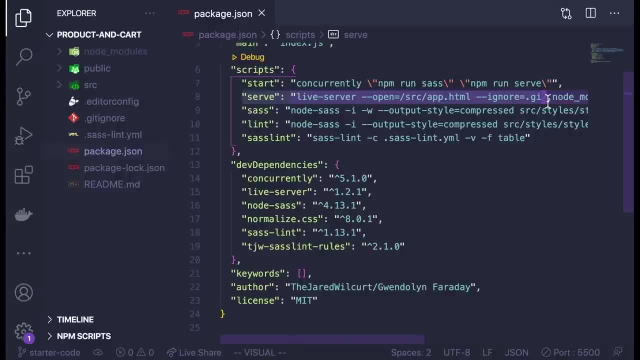 I will show you how to start an application with the Vuecli, but I had to use some kind of a temporary server here in the meantime. so that is what live server is doing for us. it will serve it on a port, similar to what we did with the live server plugin. 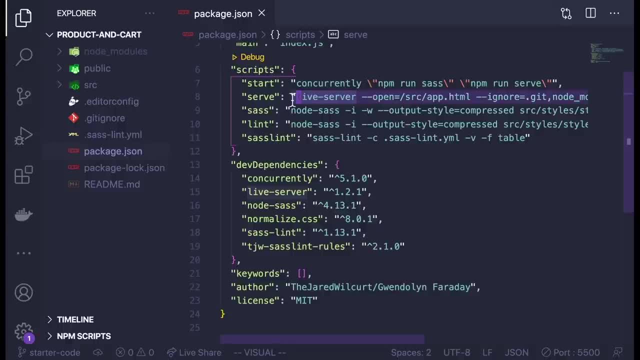 that we used in VS Code for the last demo application. so to start this application, I am going to go up to my terminal option here and I am going to choose new terminal and my terminal opens at the bottom here inside my current folder, and I am going to run the start command. 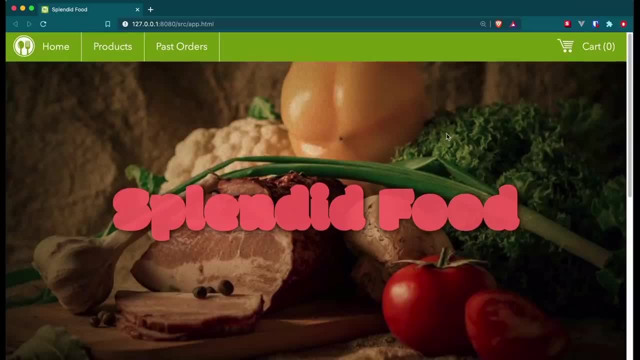 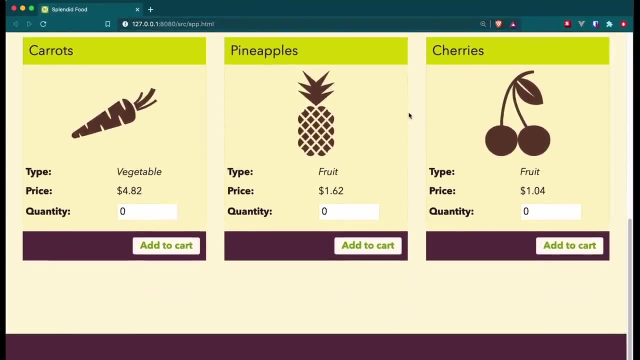 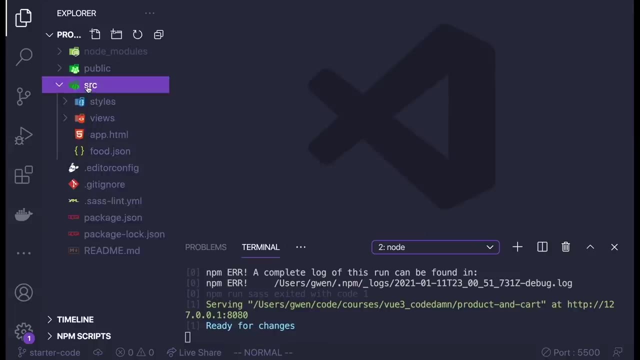 so npm start. you can see that automatically opens the application on the correct port here. and if I scroll down, I can see the same page that you already saw. now back in the code, let's look in the source directory. so the source directory is where all of our 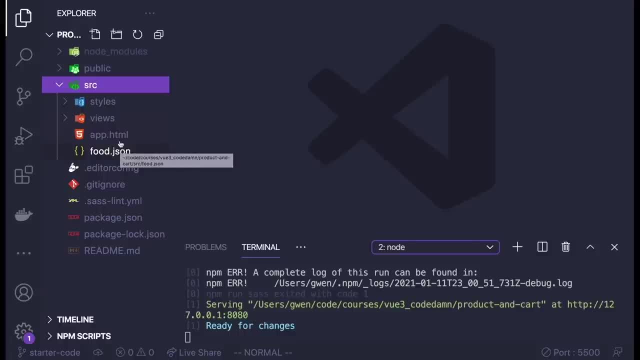 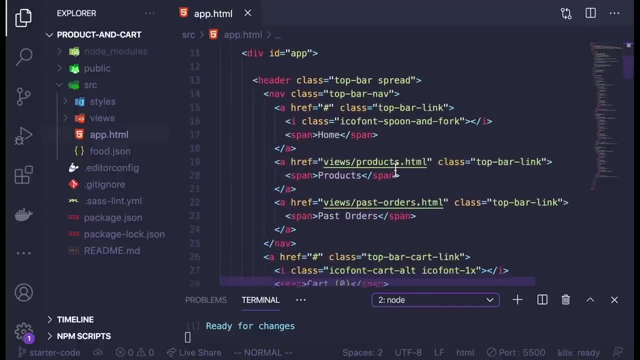 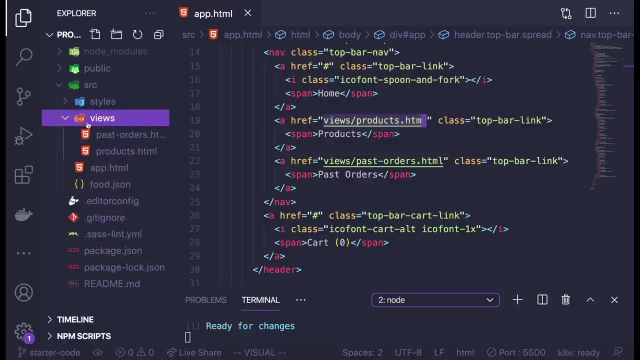 javascript and other code is going to live and this is where we will also be adding Vuejs. this is our main html file for the application, which is the home page, and you can see. the links here go to Vue's pages inside of this Vue's directory. 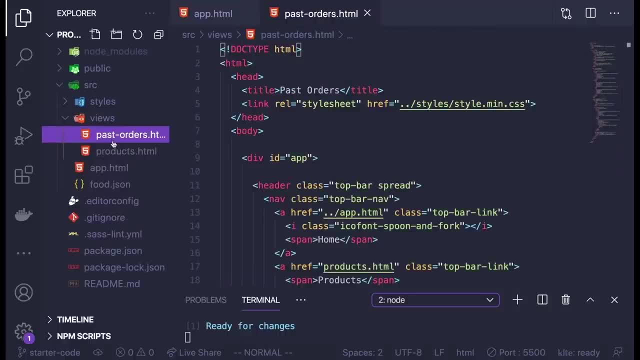 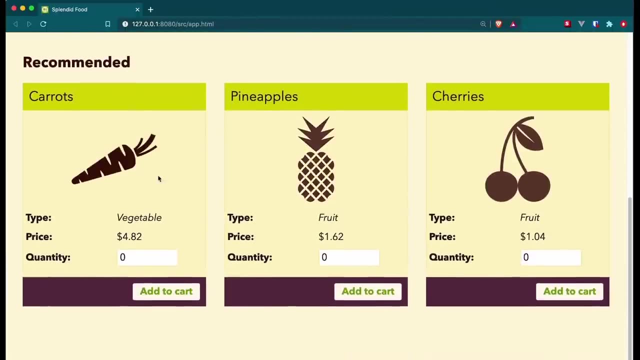 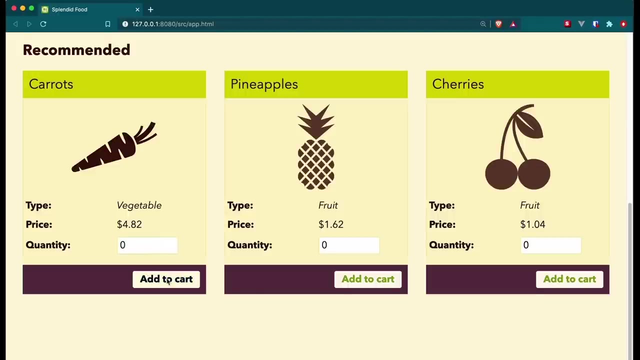 over here, so the links will take you to the past orders page and also the products page. now to start working with Vuejs, I am going to start with these cards here right now. I want to be able to update and save the quantities and be able to add them to the cart. 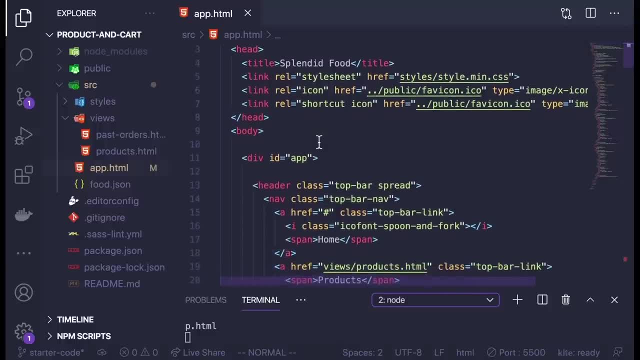 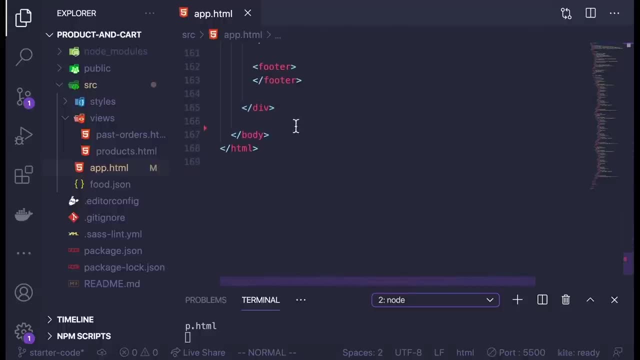 so in this apphtml file I am going to go ahead and add my link to Vuejs, just like I had in the last demo application. so I am going to go to the bottom here and paste the script tag. so I am importing Vuejs and now I need to. 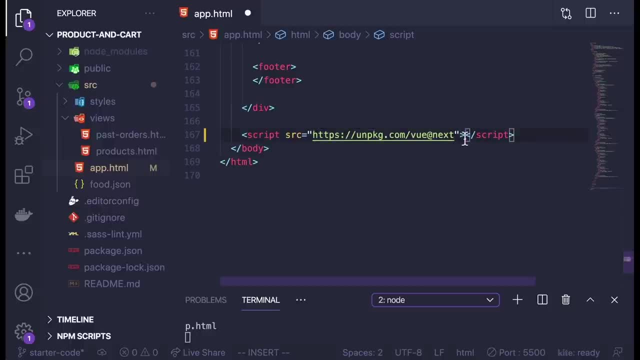 write some custom Vuejs code to hook up my application. so I will create another script tag and here I am going to do: let app equal Vuecreate app. I will pass it an empty object for right now, and then here I am going to do: appmount. 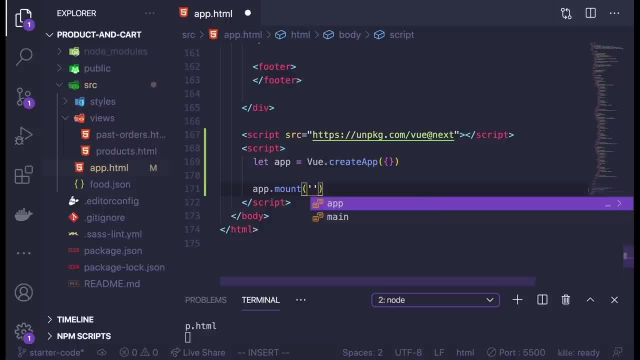 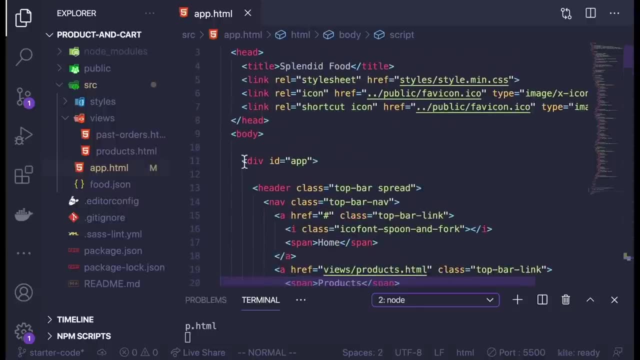 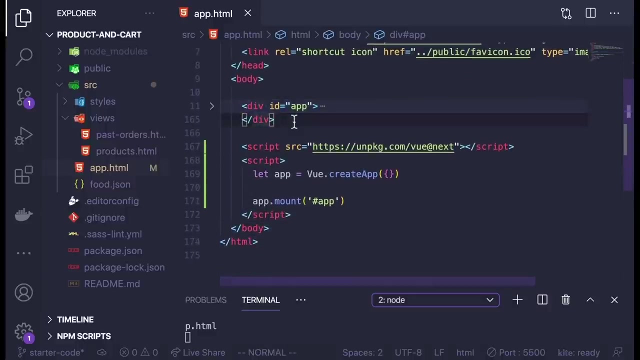 and then mount it in the same DOM element as before with the id of app. and let me just check here. yes, the wrapper. if I fold it, you can see all of the content is created inside of app. so to get started here, I definitely want to create a data. 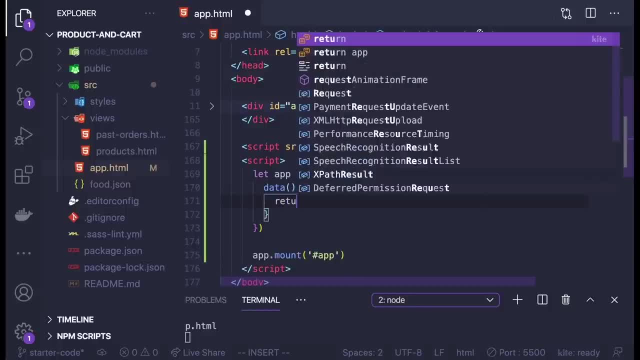 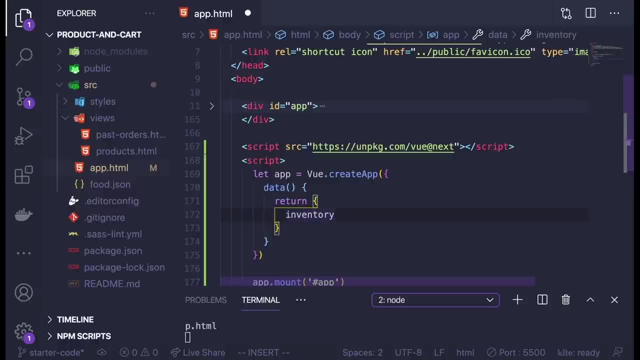 method and I need to return an object and on this object I want to track my inventory. so when someone clicks the add to cart button I want to increment or change the amount of inventory that I have. so inventory itself will be an object and you can see the different. 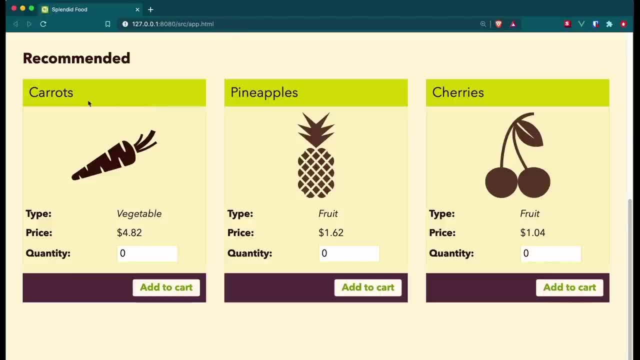 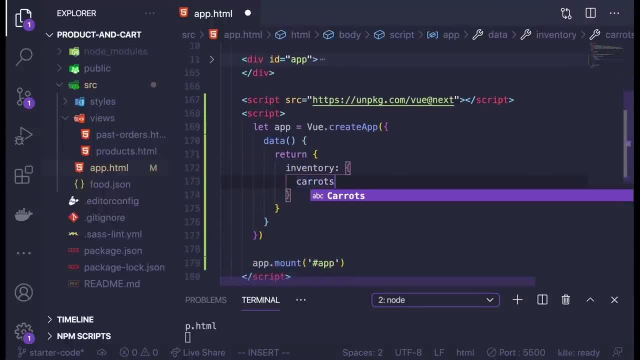 types of produce that I have here, so carrots, pineapples and cherries- and so I am going to add these three items to my inventory carrots and I am going to initialize all of these with zero. that looks good. now I need to find these elements inside my application. 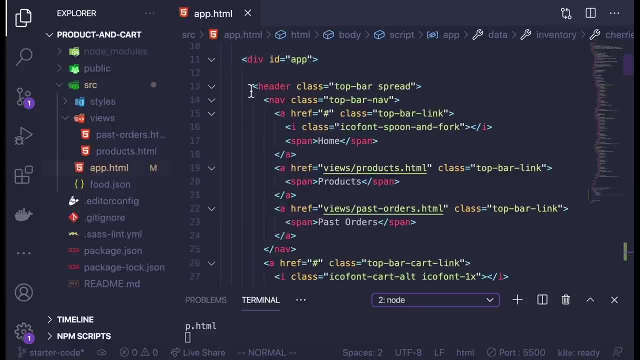 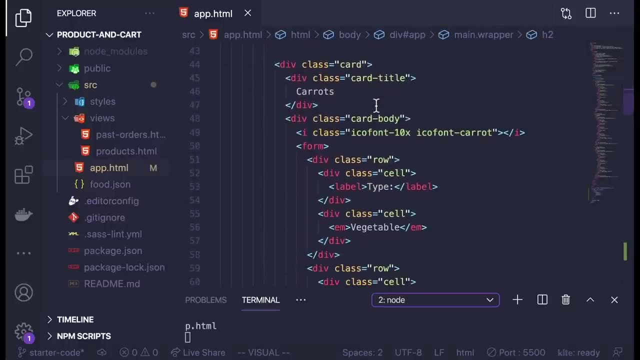 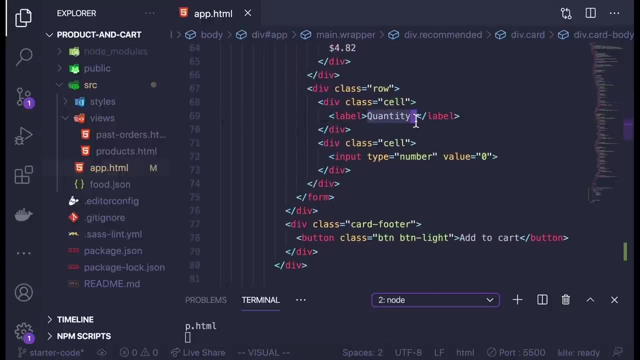 and put the variables there. so if I look down at these cards you can see here is the recommended product section, so I have carrots here and I have the price. here is the quantity with the input field, and what I want to do here instead of setting the value. 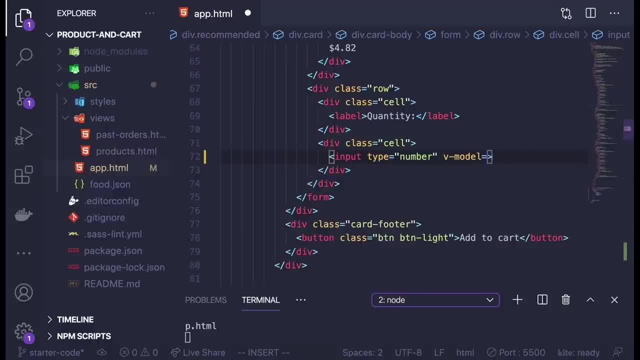 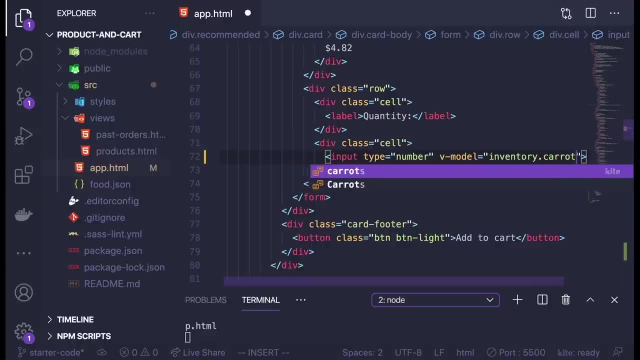 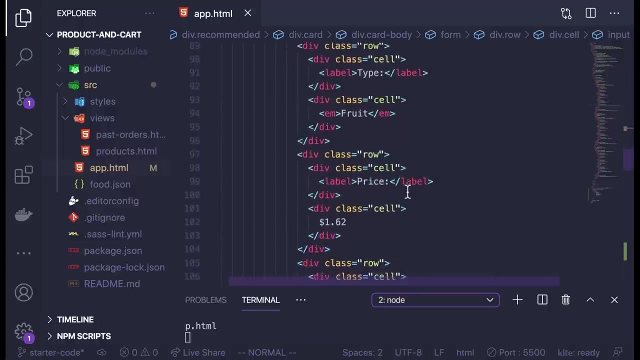 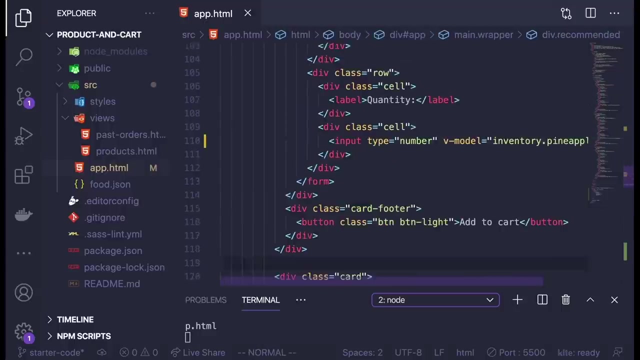 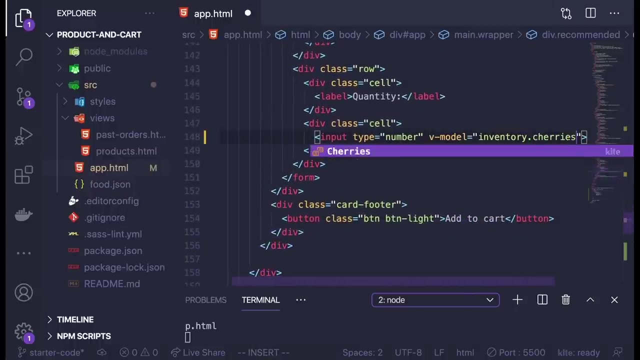 I want to do v model and this should be inventory dot carrots, and then I am going to copy the same thing for the other fields. so I will come down here to pineapples and paste this, and then cherries as well. ok, now let me take a look at that. 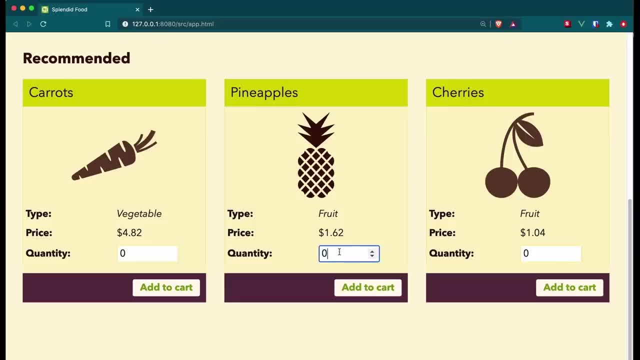 and you can see it still shows zero here. just like before, I can update the number. let me do three carrots and now the number starts at three. so now we want to do something. when someone clicks add to cart, if they have a certain quantity in here, we want to add it. 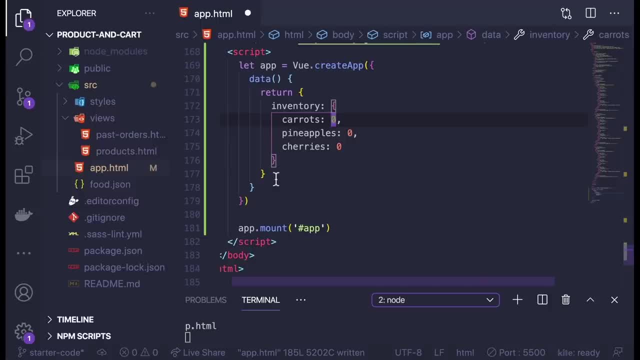 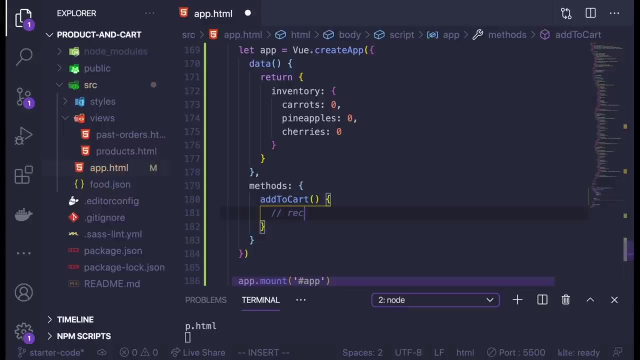 to a cart total. let me change this back to zero. so to do that, I need to create a method. let me create my methods object. I will create an add to cart method and in this method I need to take in the number of items that someone wants to. 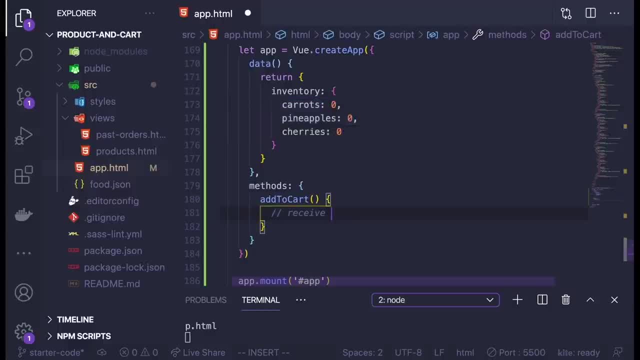 add to their cart and also the type of item. so to do this, I am going to need another place to store what items are actually in the cart. so I am going to create a cart here and for right now I am just going to copy the same items over. 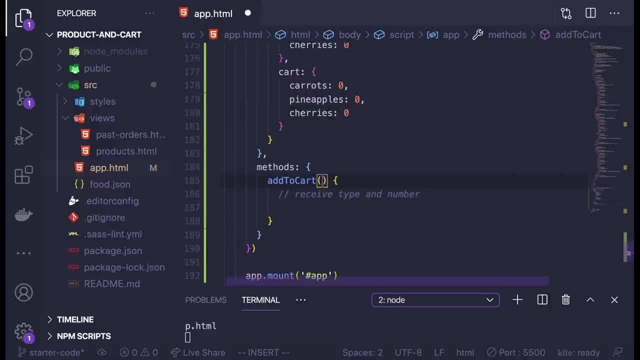 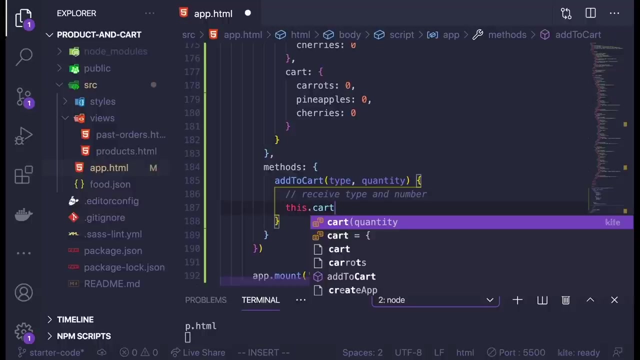 and then when I call the add to cart method, I need to pass in the type of item and the quantity. then I can access my cart variables by doing this dot cart, and to pass in a variable that I want to access on my cart object I need to use the square. 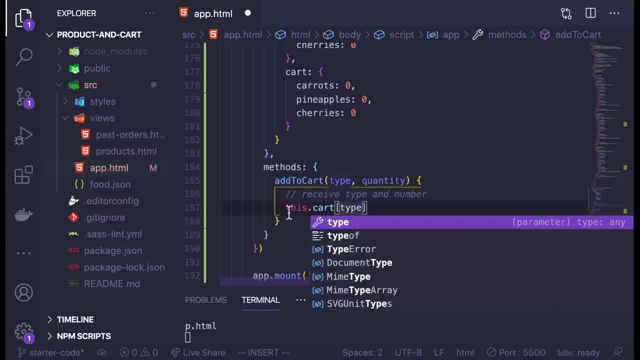 brackets, and then I can pass in type, so it would be the same as this dot cart dot carrots or this dot cart dot pineapples or whichever item we want to access. and then I am going to increment by the quantity, so plus equals quantity. now I don't have. 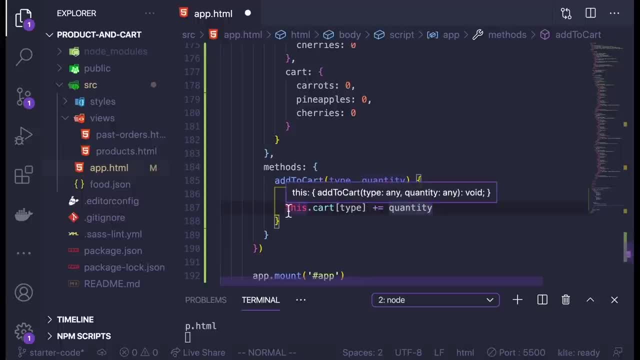 to return anything from this function, because this is really the action that I want to take by calling this function is to update whatever I have in my cart right now and to show this. I am just going to log this out in the console in the browser so you can see it. 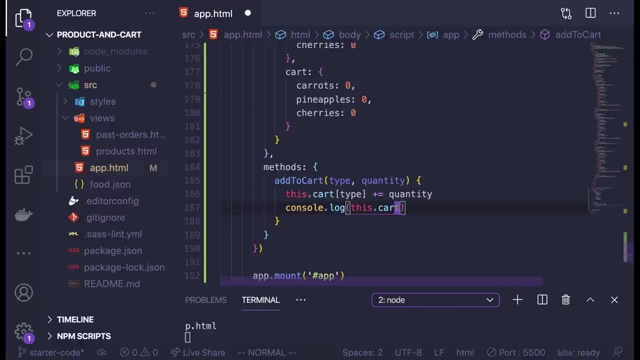 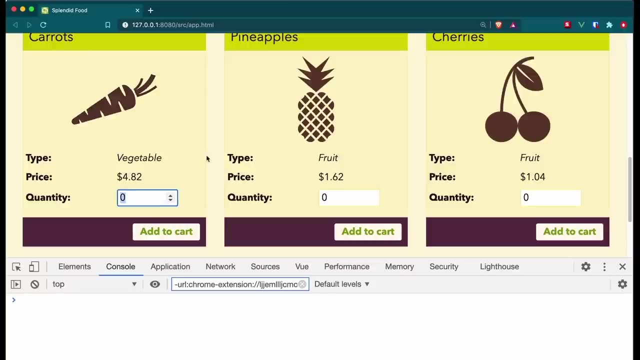 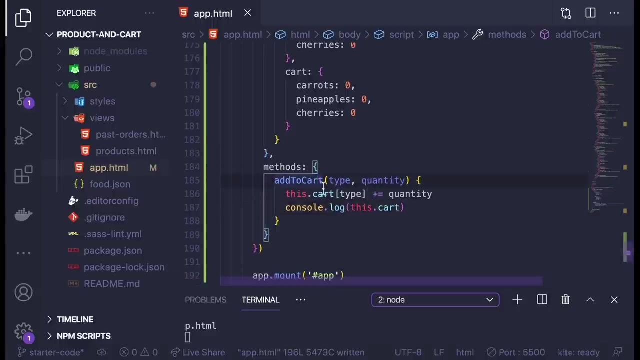 I am going to log out this dot cart and I am going to open my console here. so for carrots, I am going to add three. you can see nothing happened. that is because I forgot to connect this method to that button. so let me go up here and add. 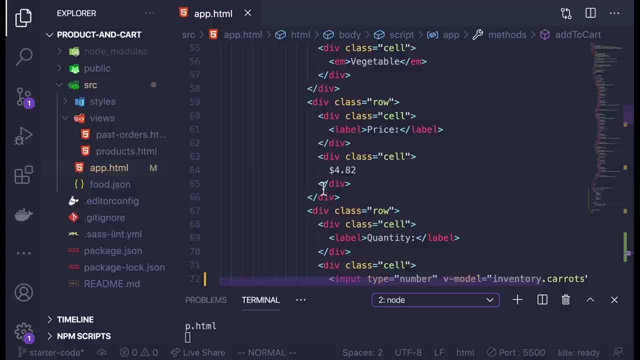 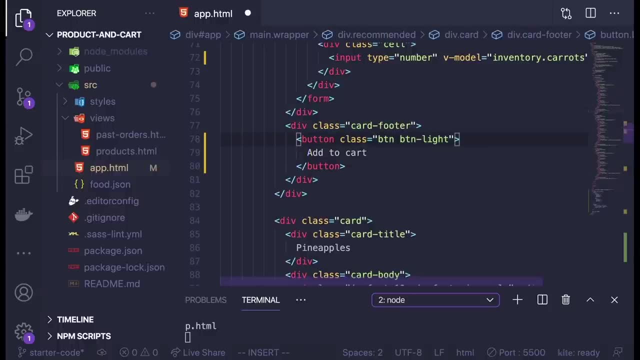 that button. so I am just going to add it to carrots right now here. so when someone clicks on the add to cart button, I am going to call the add to cart method. now I need to call it passing in a few arguments here. so the first one is going to: 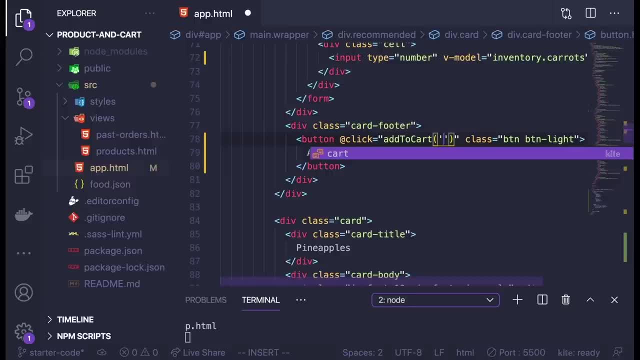 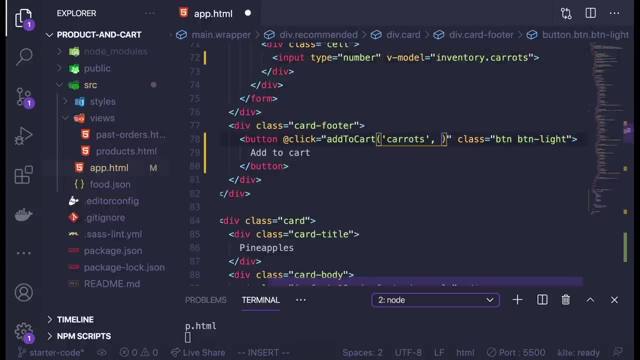 be the type of item that I want to add to the cart. so this one will be carrots and I also need to pass in the quantity. to pass in the quantity I need to use the inventory dot carrots variable so I can just pass that in here. I could also just call it from inside. 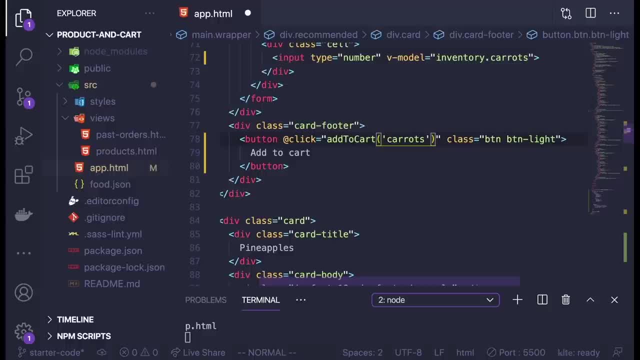 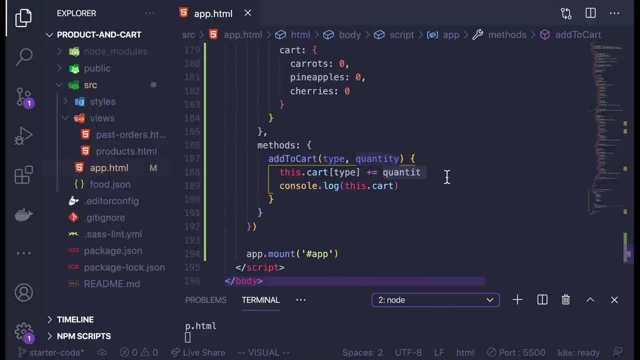 of my function, which is actually what I am going to do. so let me scroll down to see my function again, and instead of quantity here, instead of passing in this extra variable, I am going to just update this to this dot, this dot inventory, and then get the type from. 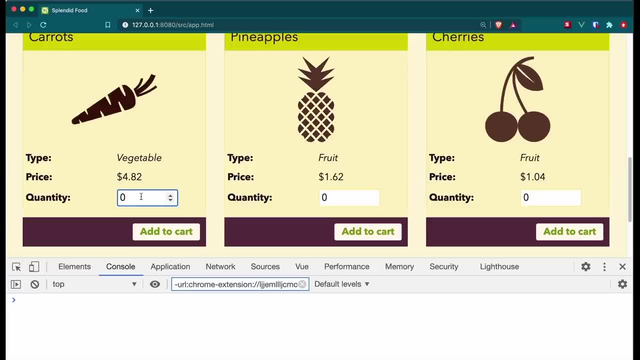 there. so let's see if this is working. let me add to cart and you can see there is definitely a problem, because the input value is a string and it is trying to add it to the number zero, so then it turns the expression into a string. now Vue has a very easy way. 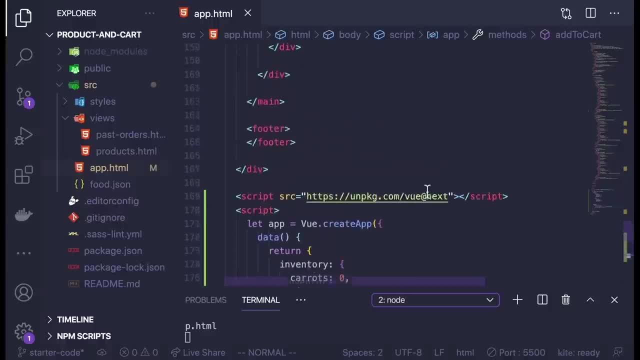 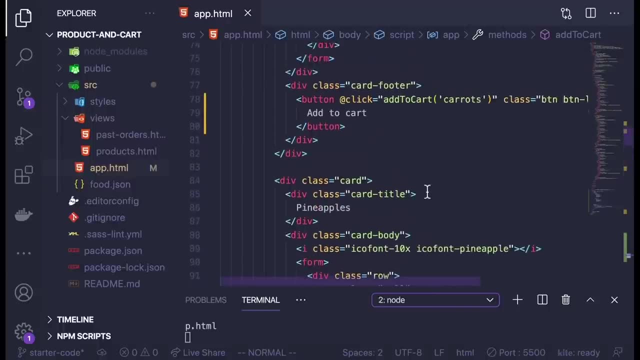 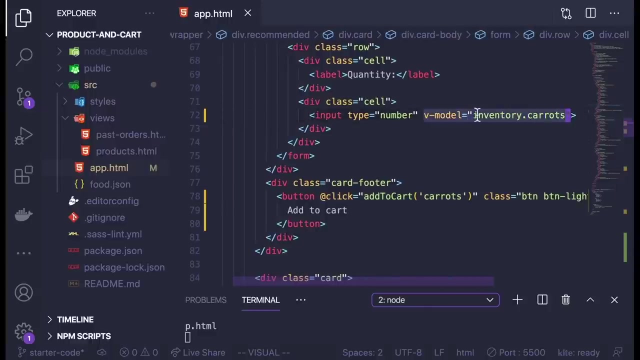 of fixing this, and this is through a modifier, just like we learned about a little bit in the last demo that we did. so let me go up here to the V model. and we don't want this V model to be considered as a string. we want to. 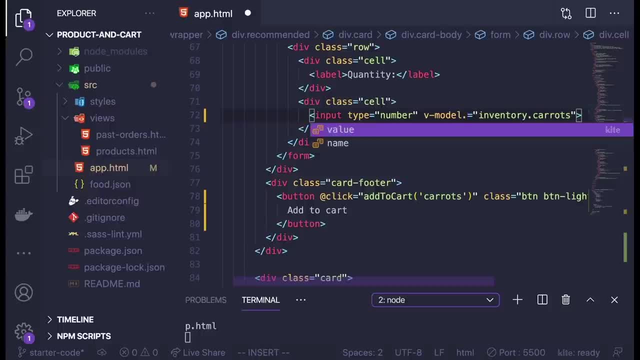 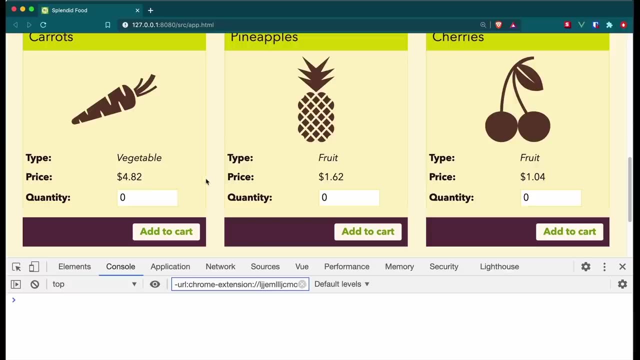 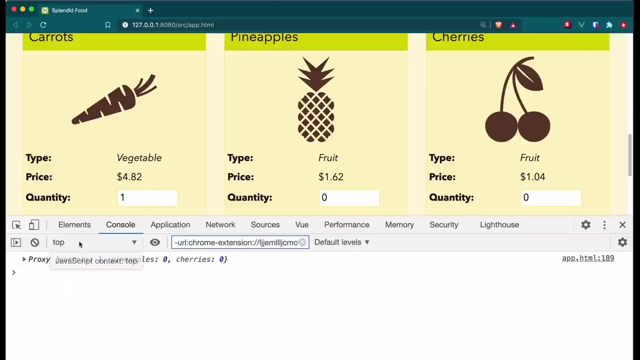 go ahead and cast it as a number. so Vue gives us this modifier as a shortcut. so V model dot number. so now, if we look in our application, let me add to cart, and I can see down here that my carrots have one item in it which is a number. so I can. 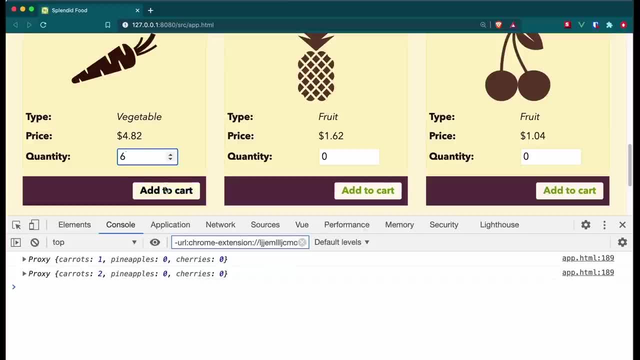 add to cart again, and now it's two and I can add multiples, and now there's eight carrots in the cart. let's stop here for this video and don't forget to download the related code and try out these features for yourself. in the next video we will. 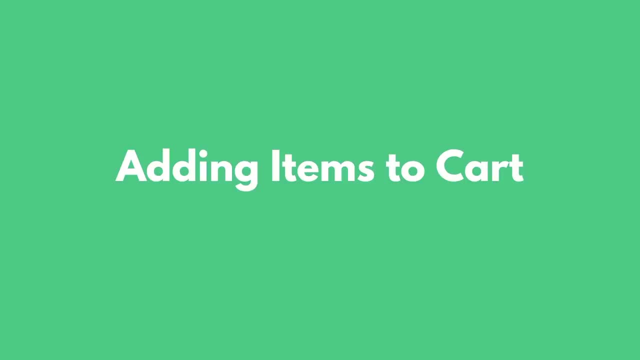 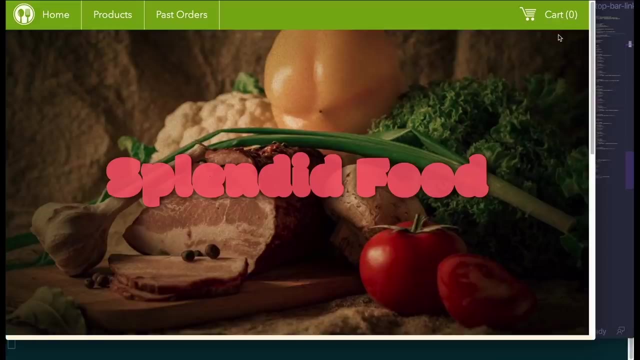 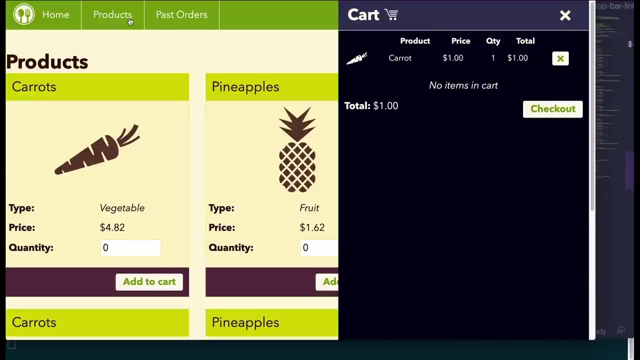 work on displaying the items in the cart. so now we want to hook up this cart menu or cart slide out, and right now it's just static content, so we can only see it from the products page and if you look at the code, we go to the products dot html. 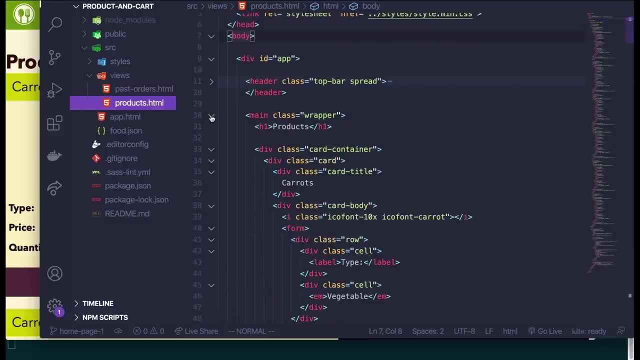 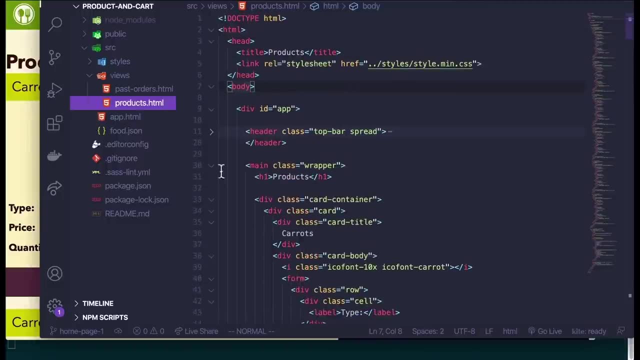 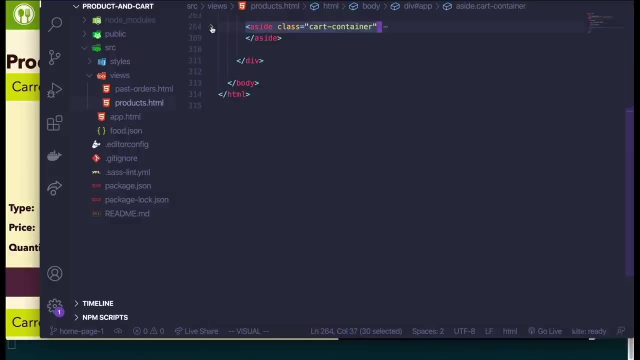 I'm going to fold this header and also the main container, which is this main part of the page, right here and now. I can just see this aside, which is that cart section on the side. so I basically want to get all of this html and make it available on my other. 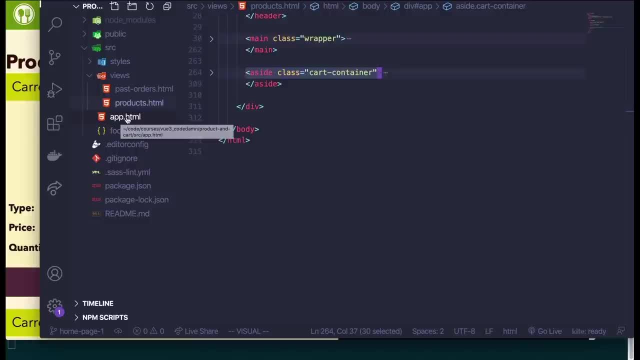 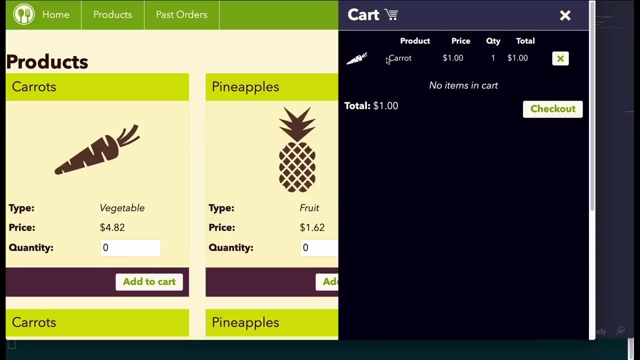 pages, like my app page, which is the home page, so that I can use Vuejs to trigger opening or closing the menu. and I also want to make these cart items dynamic so when I add more items to the cart it can update the quantity and the price. 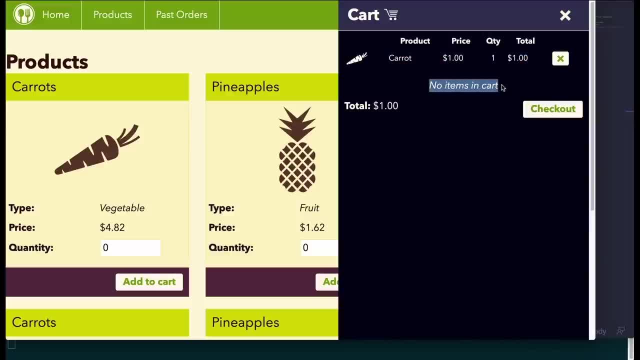 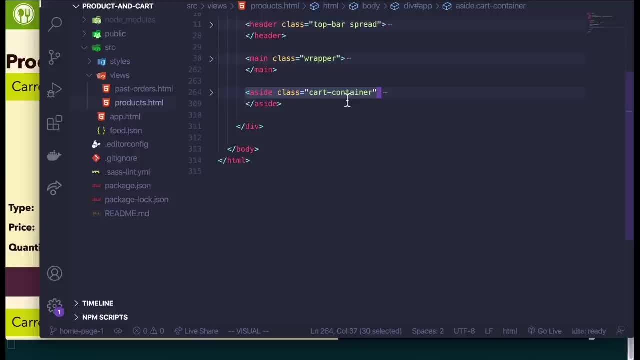 and I can also set a variable. so if there are no items in the cart, this will display. now, html itself doesn't have something like an import to import a block of html into another html file. a lot of people use php or some other backend tool for that. 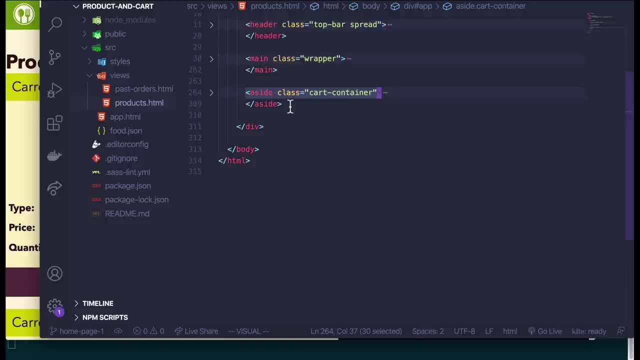 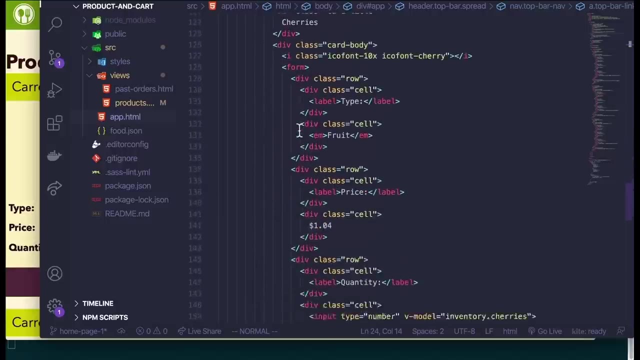 but we can also easily do this in javascript, so we're going to do this in Vuejs, actually. so I'm going to remove this sidebar from the page that it is on right now and move it into our Vue application. of course, our Vue application is nested. 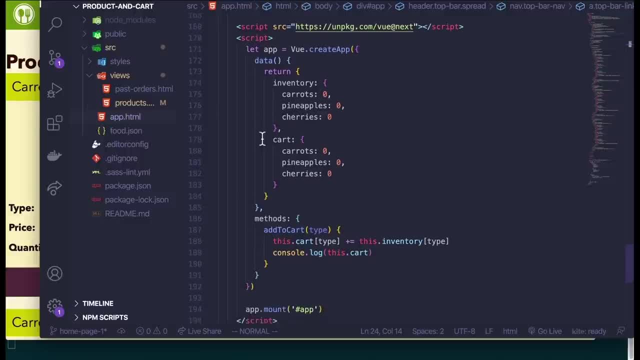 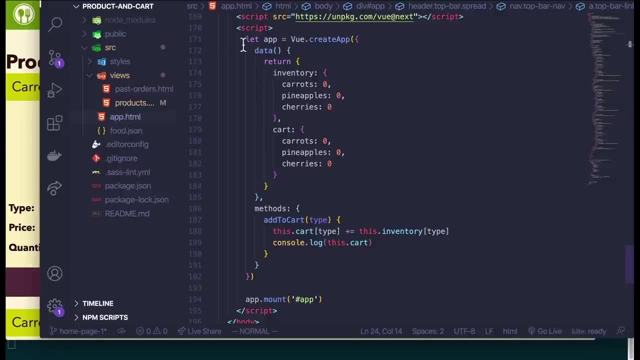 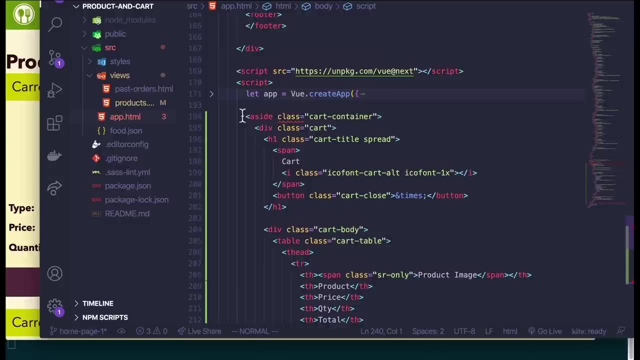 inside of the apphtml page, but we can move it outside later so that this menu will be accessible on all pages in the future. so I'm going to fold this Vuecreate app and now I will paste this html aside that I have. now it's giving me an error. 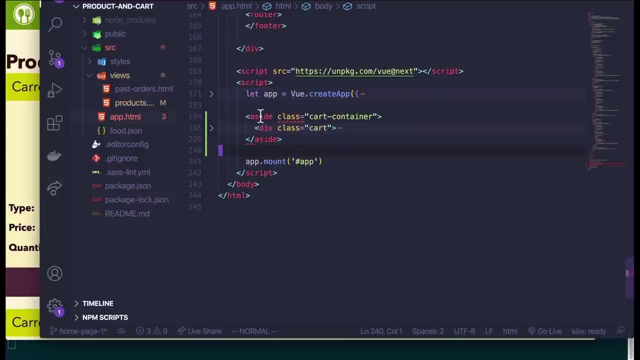 or a couple errors right now because it's inside of a script tag, but I'm going to fix that. so, if you recall, in the earlier lessons we defined different components inside of our Vue application. so this is a perfect use case for a component right now because it's this reusable. 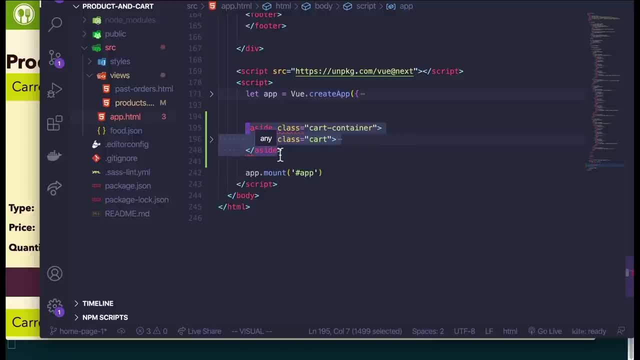 block of html or template that we want to use on multiple different pages and also interact with. so I'm going to register this as a component and I'm just going to call it sidebar, and now I pass in the object just as before, and on this options object. 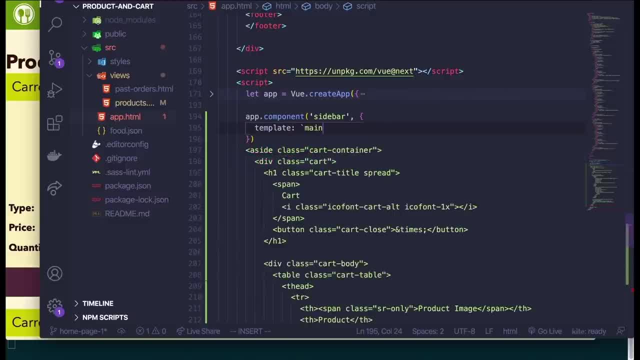 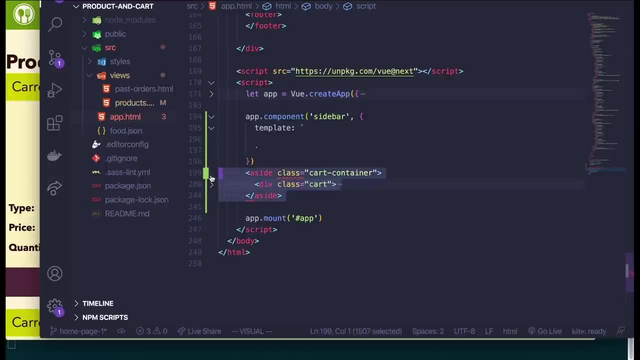 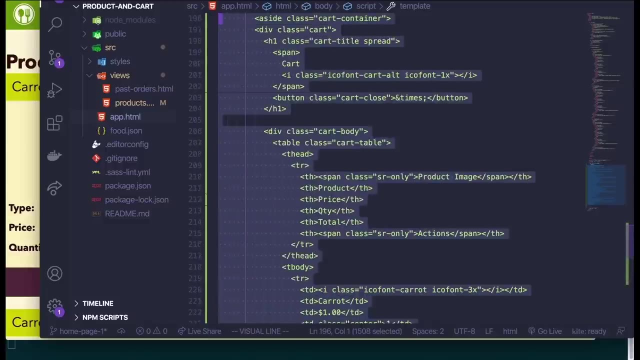 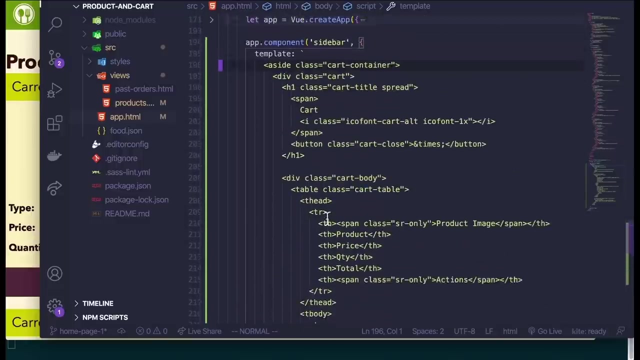 I can set the template and then use graves, and now I want to grab this aside again and paste it inside of here. and so now I have this whole aside, all of the code inside of my template for this component, and now I can add this to the page. 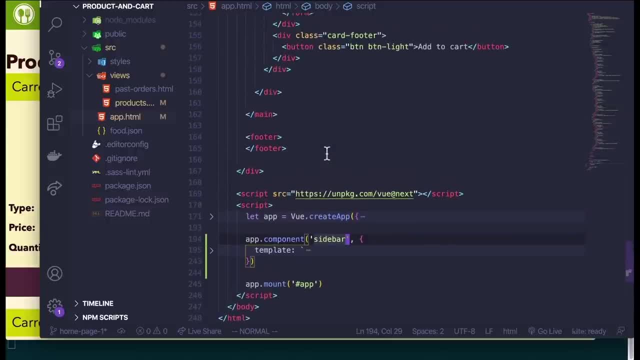 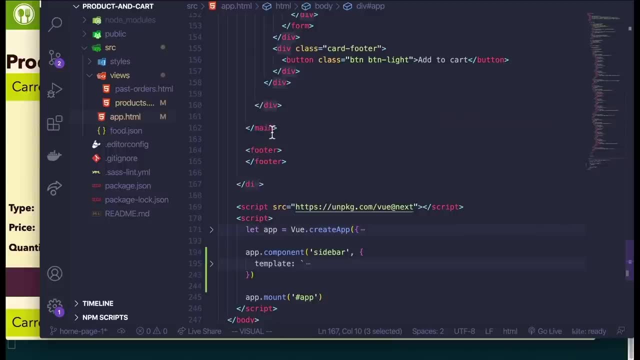 with the name sidebar, so I'm going to go ahead and add it here and remember that our div wraps the whole Vue application, so I can put this anywhere inside of that div. with id of app- I'm going to put it here. and the footer: I'm going to put the custom. 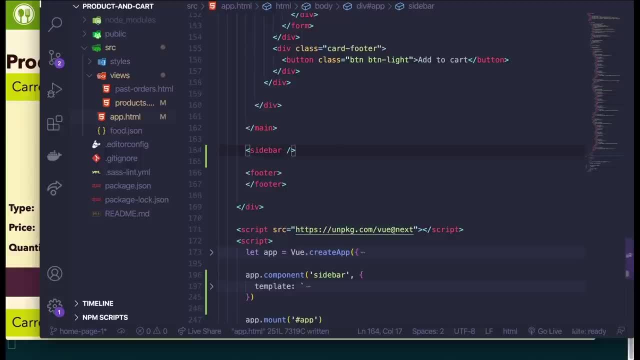 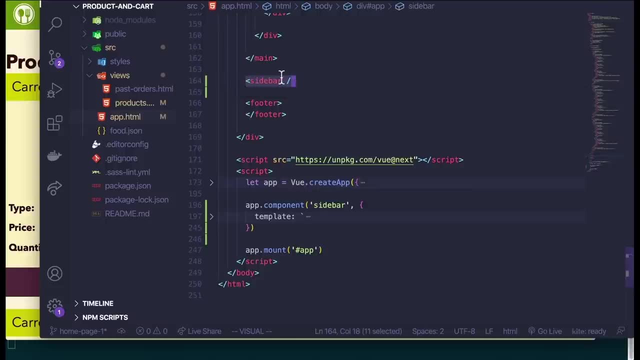 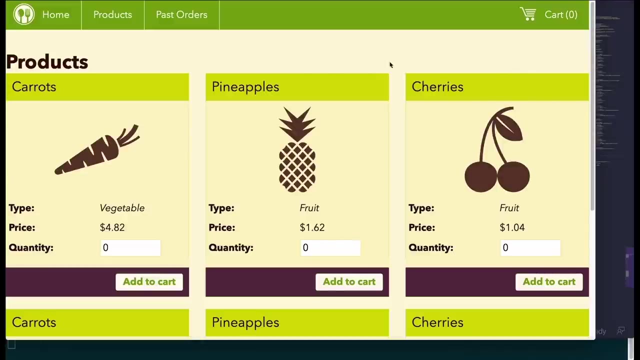 component sidebar and Vue will handle putting the template I have down here where this sidebar element is in the template. so let me go back to the html here. you can see the sidebar is no longer on the products page. but if I go to the home page now I have a sidebar here. 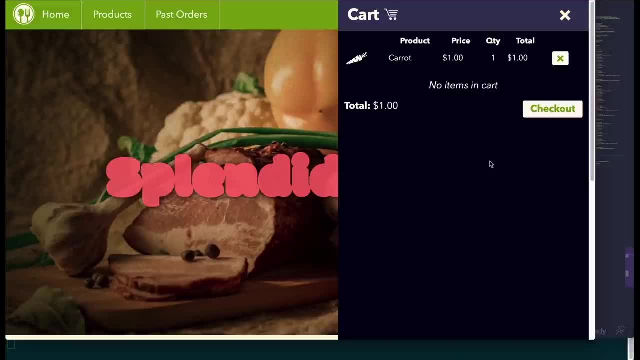 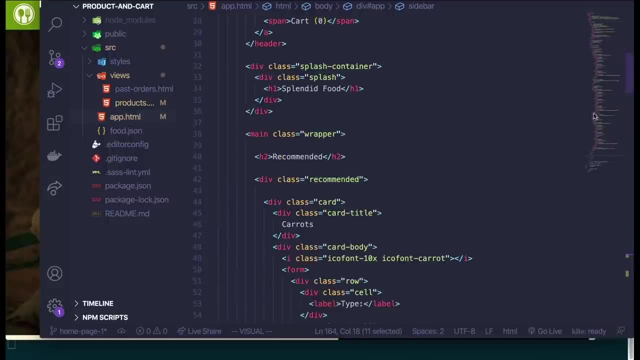 so now that the sidebar is in Vuejs, I can start making it interactive, and the first thing I want to do is be able to hide and show the sidebar. so basically, when this is clicked, I want to hide it, and then when another button is clicked, I want to show it. 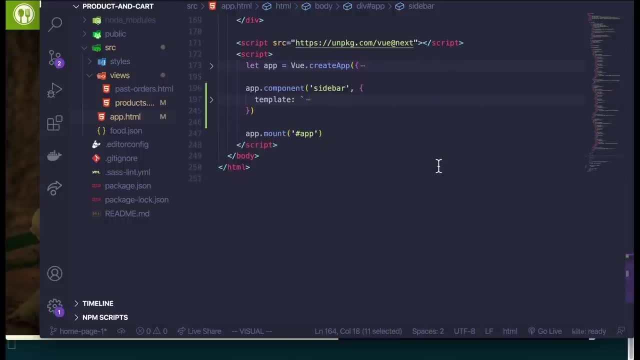 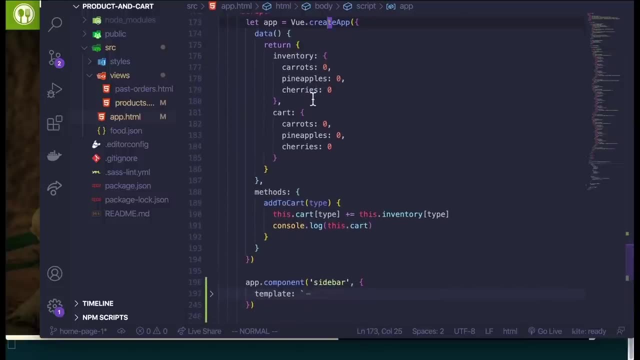 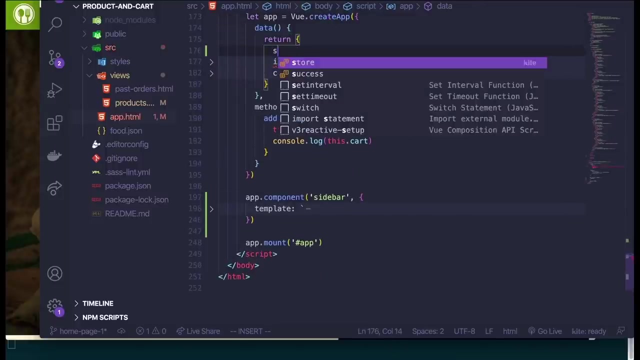 so I need to create a variable for this and let me go down to my javascript down here. so inside of my regular create app here and my main options object: I'm going to add an element data here and I'm going to call it: show sidebar false. 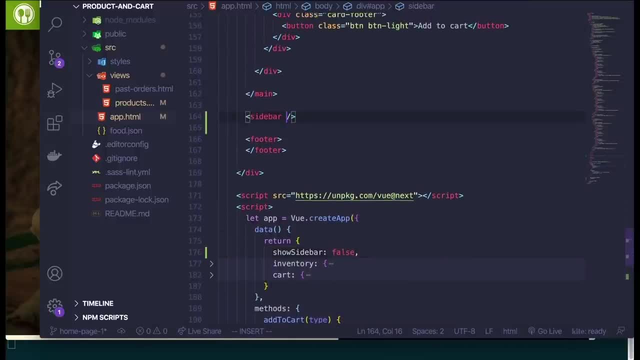 and now I can come to my sidebar and simply use a vif and point it to the variable show sidebar. so if show sidebar is true, then my custom component will show up on the page. if it's false, then I shouldn't see the sidebar at all. 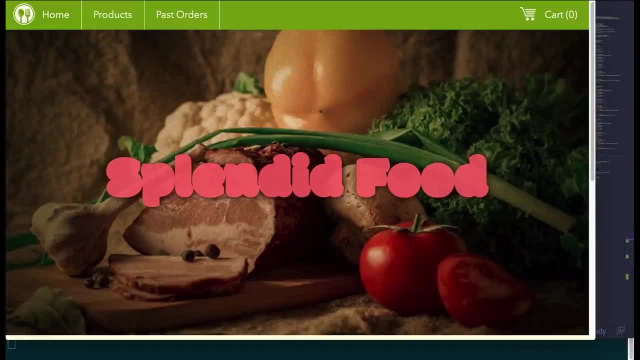 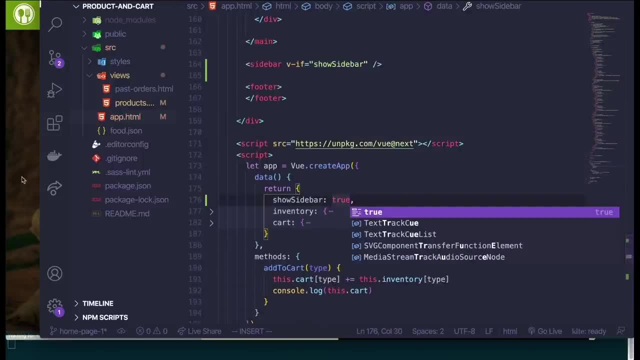 and you can see it's false. I don't see any sidebar, and when I change this to true, I see the sidebar. now I just need to add a toggle for this sidebar. let me change it back to false by default and now I can create a method. 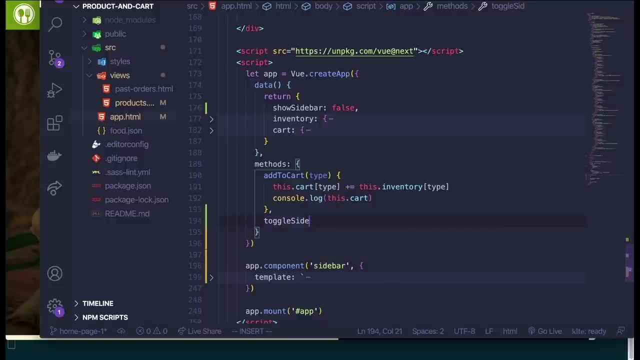 called toggle sidebar and I'm going to say this dot show sidebar equals the opposite of whatever it is, because it will toggle true or false every time this function is run. so I'm going to say it equals not this dot show sidebar. so if it's currently false, 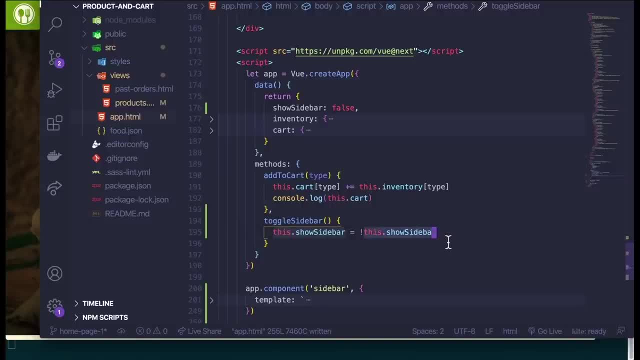 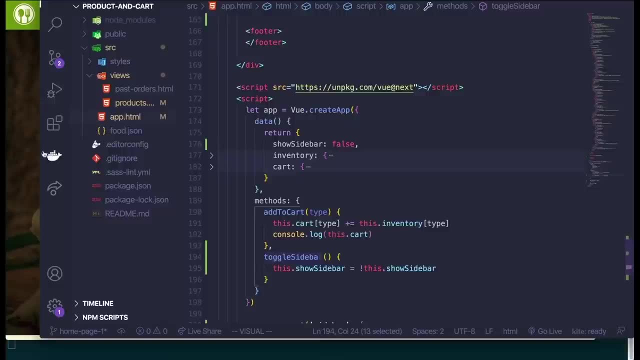 that means it will be set equal to true, and if it's true, it will be then set equal to false. now I just have to call this method, so the first place that I'm going to put it is on the this button here, this cart button should. 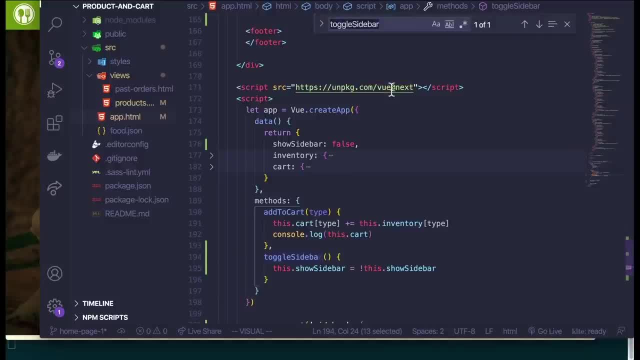 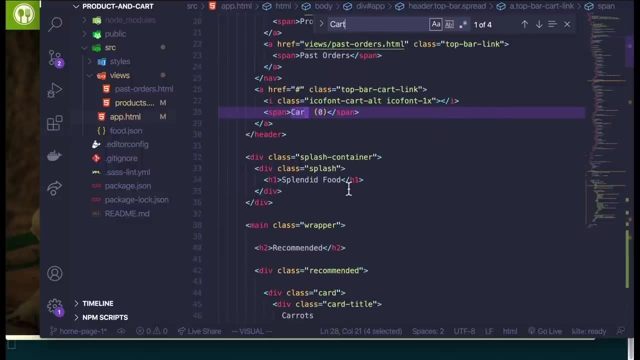 open that cart sidebar. I'm going to find that on the page. here is that cart button and I'm just going to add an at click here. at click equals toggle sidebar. I don't need to pass anything in, so I can just leave it as this and view will automatically look through. 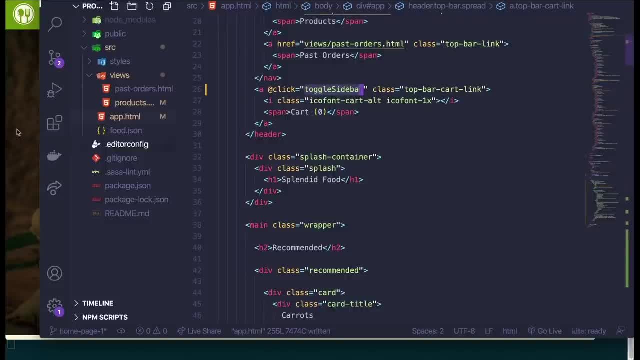 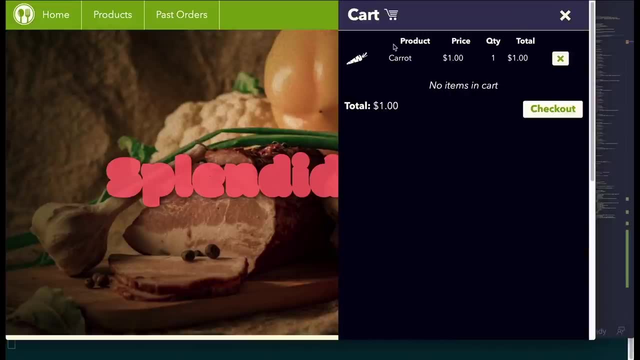 my methods and find that method, so let me see if that works. go back to the page. should be able to click on this now, and yes, it does toggle now. the next thing I need to be able to do is close it, and I need to close it using this x here. 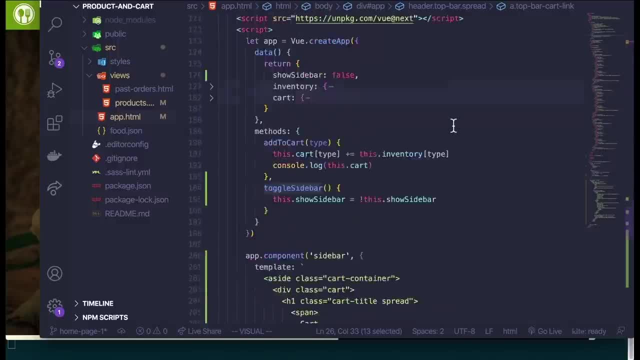 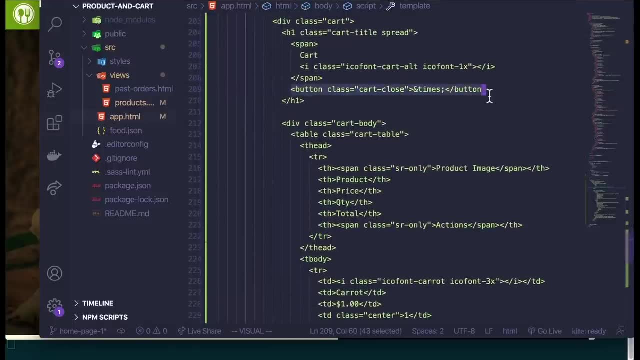 so I'll have to go down to my template here, and here is the button, that's that x, that's in the corner of the header for the sidebar. so I need to add an at click on this and I'll have to do at click. now I want to use the function. 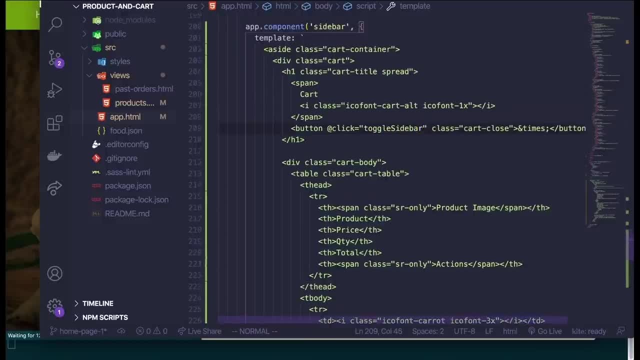 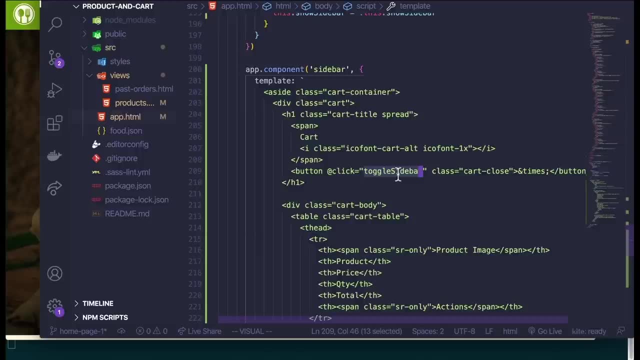 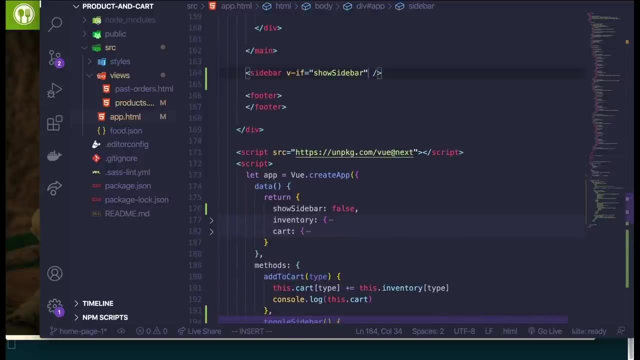 toggle sidebar, but because this is wrapped in its own component, I actually don't have access to the toggle sidebar function from here. I actually have to pass it into this component to be able to access it, and I can do that here. so I'll pass it in as. 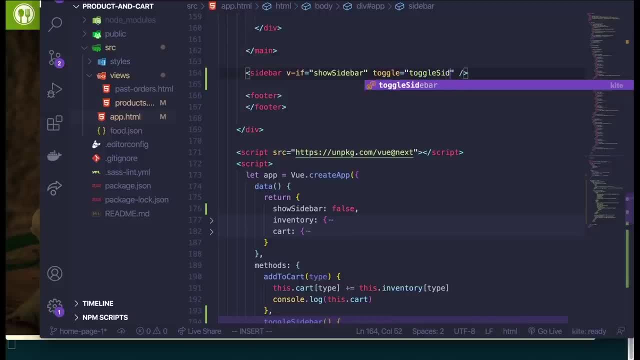 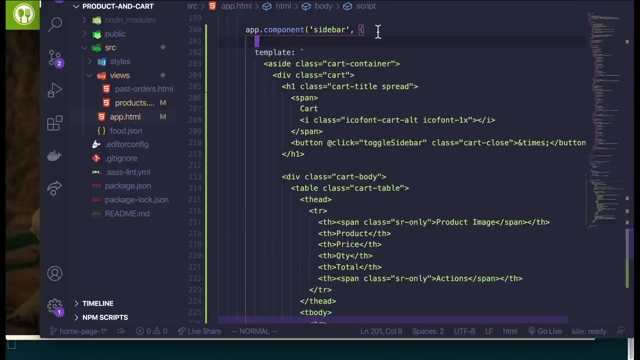 toggle equals toggle sidebar. I'm using my method on the vjs object called toggle sidebar, passing it into the sidebar component with the name toggle. so inside my component here it's going to be called toggle. so I'm going to have to accept it as a prop and 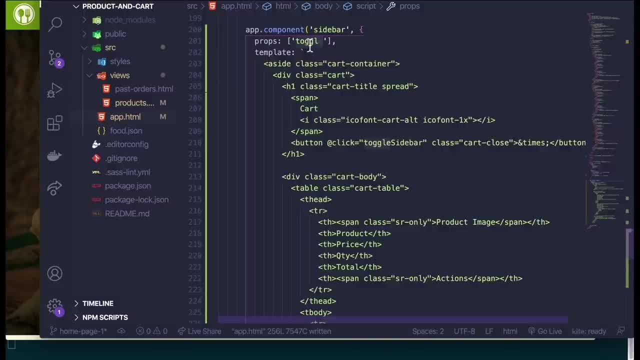 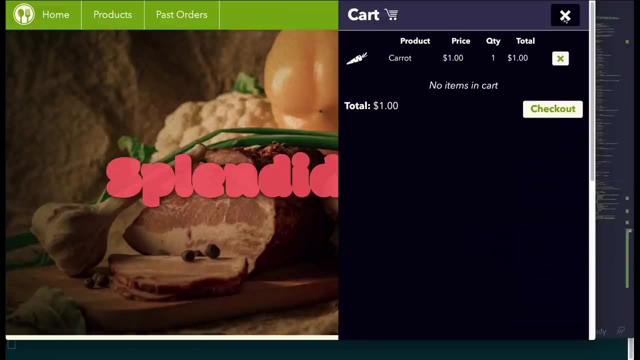 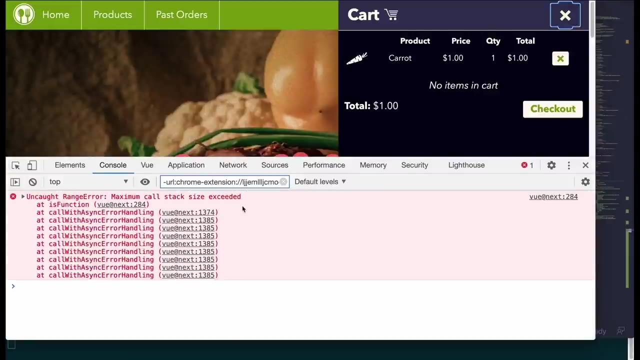 I'll accept it as toggle and that will be my function name. so now I have to rename this function and call it toggle. let me see if this works. go to cart, click x. and it is not working. so I do have an error here. maximum call stack size exceeded. 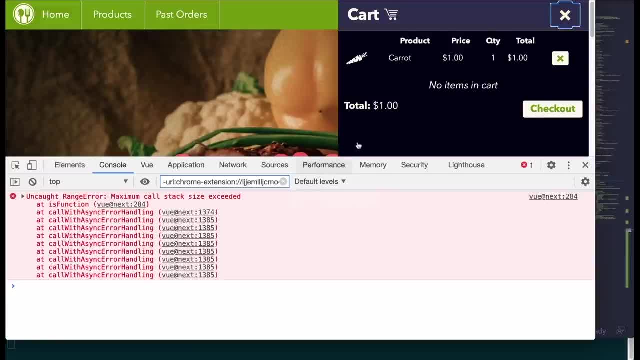 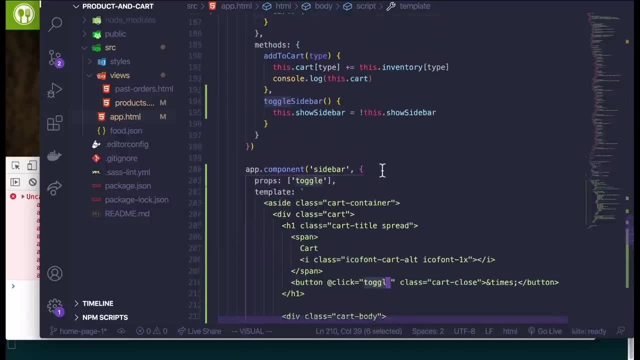 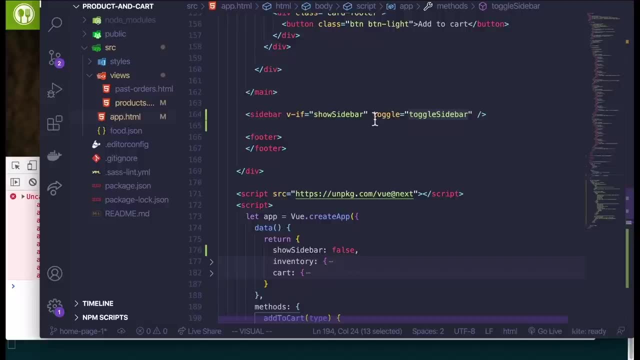 so let me see what I did wrong in the code. so I'm importing the prop toggle. the function should be called from here. I have toggle sidebar. that is pointing to toggle sidebar here and oh, I forgot to make this point to a view variable instead. it was just trying to use. 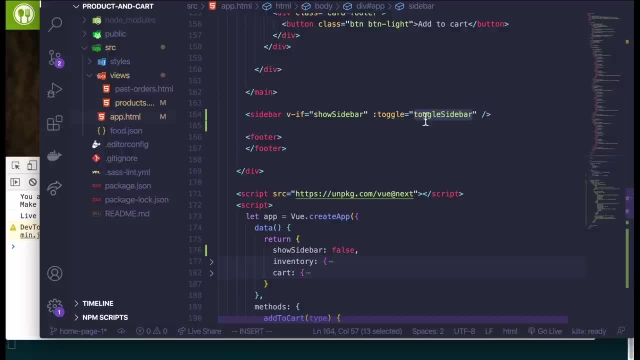 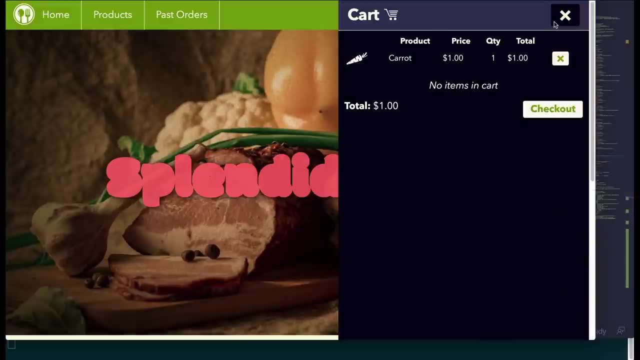 it as a string before, which was causing an error. so now it should be calling the actual toggle sidebar function and let me see that in the code. ok, it works just as intended now. so now on the sidebar, I want to be displaying actually dynamic items here for right now. 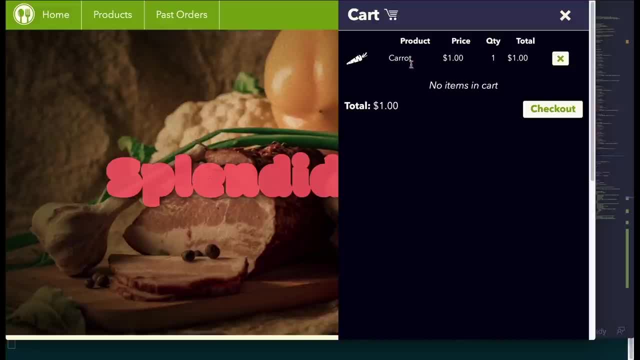 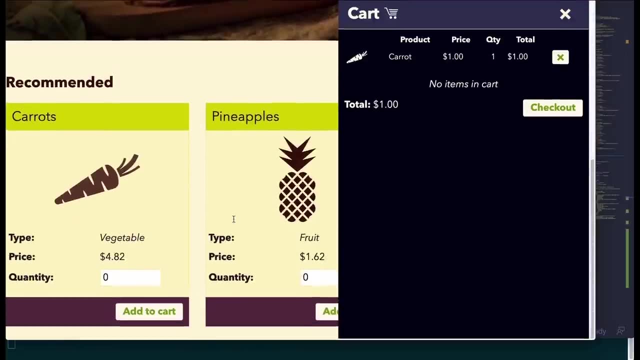 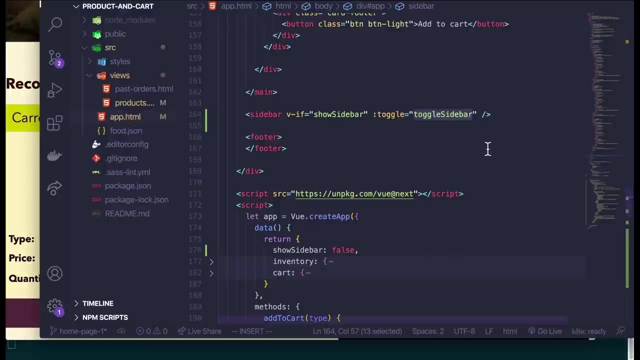 I only have one item hooked up- carrots- and so I'm only going to be working with this one item until the next video. so let's hook this item up. when I add items to the cart here, it should update in the cart over here now to do that. 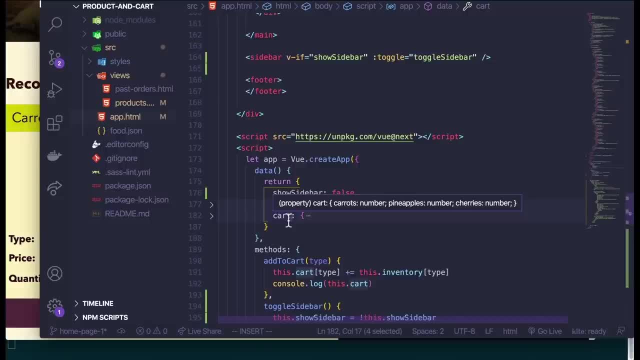 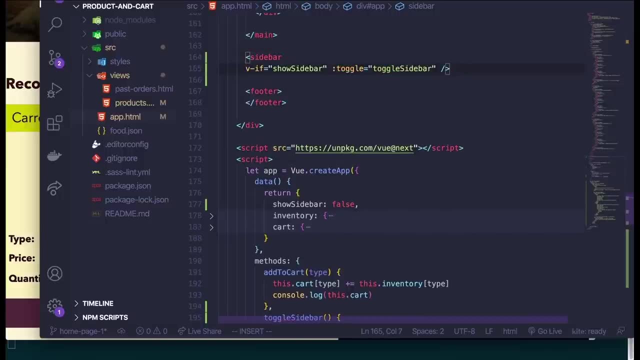 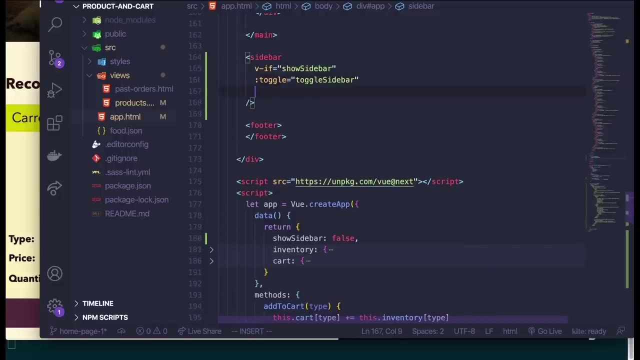 I need to take this cart object and pass it in to my sidebar so my sidebar has access to it. first, let me do some cleanup here, but I'll do this on multiple lines to make it a little bit cleaner and I'm going to pass in cart. 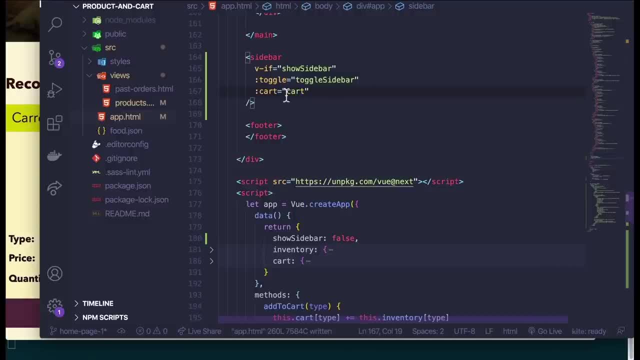 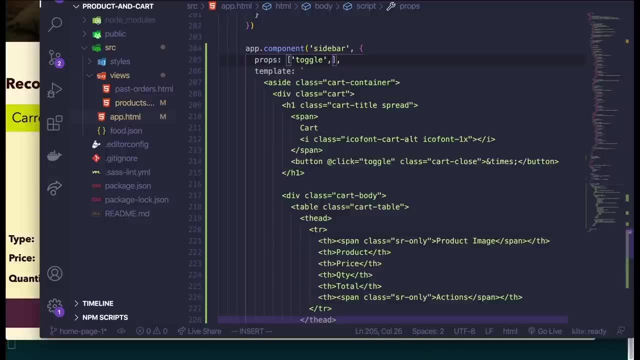 as just cart. and now I have to receive this prop in my component here, so I'm going to do it here and call it cart. and now cart that I'm getting in my component is actually that cart object. so since I'm only working with carrots for right now, 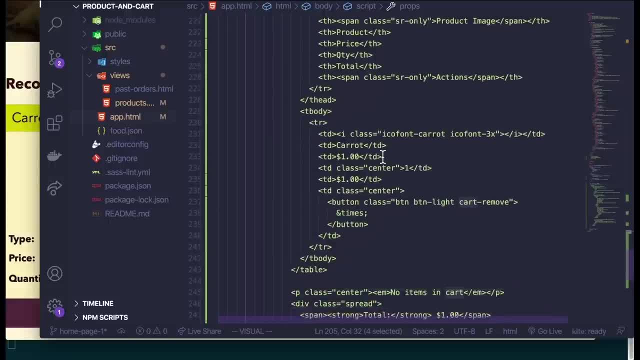 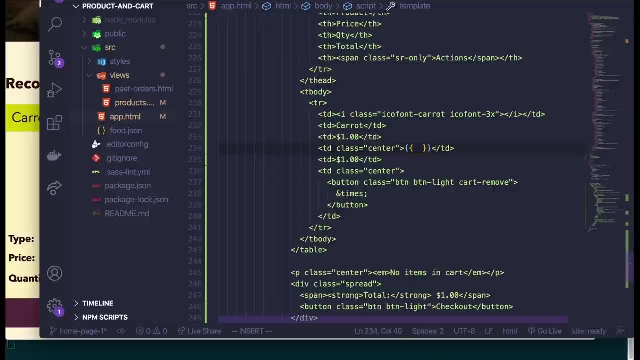 I'm going to just assume that and only add the number here for carrots. so I'll use my double mustache syntax and I have that cart variable. so I'll do cart dot carrots and that will be the number of carrots that I have. so let me go back to here. 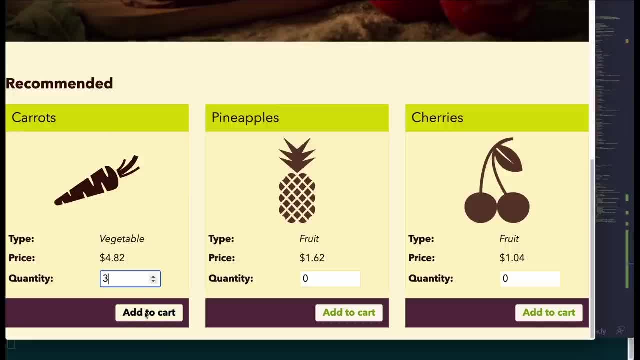 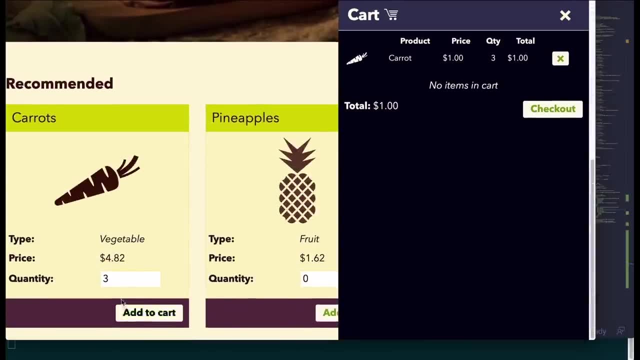 and it automatically updated. let me add three, and my cart now has quantity three. so if I add, let's add five more. now there's quantity eight in my cart, so now my cart is dynamic. of course, the total should also be updated based off of the quantity. 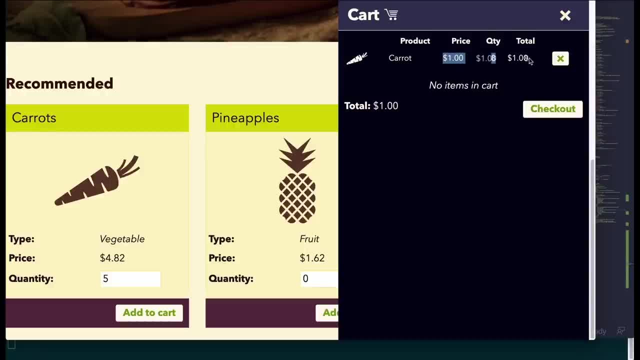 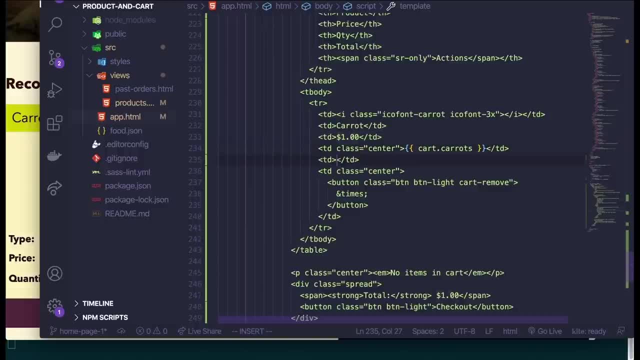 it should be: price times quantity equals the total for that item. so let me do that really quickly. this is the total number, so I'm just going to have to do this. and let's say cart dot carrots times the price which it says, it's one dollar. 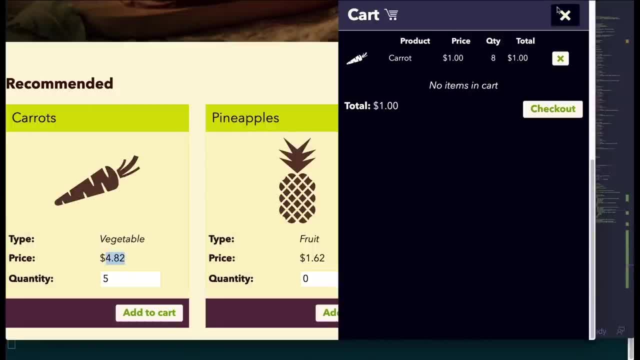 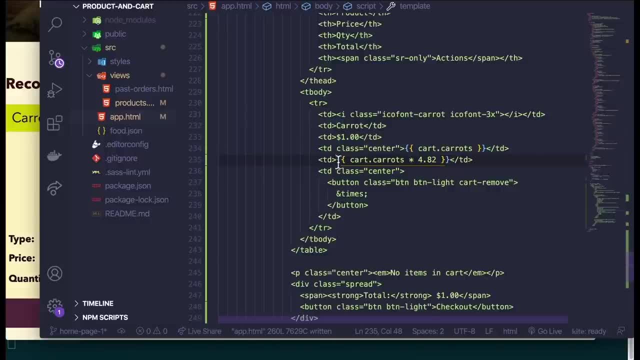 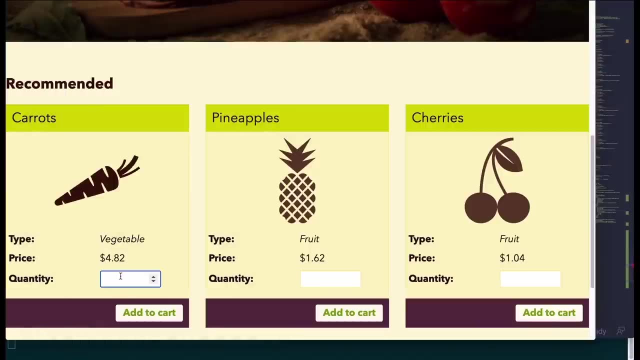 but here it says four eighty two. so I'm going to use this price because one dollar isn't that interesting. so I'll do times four, eighty two and then before that I need to put in dollars and let's see if that works. two add to cart. 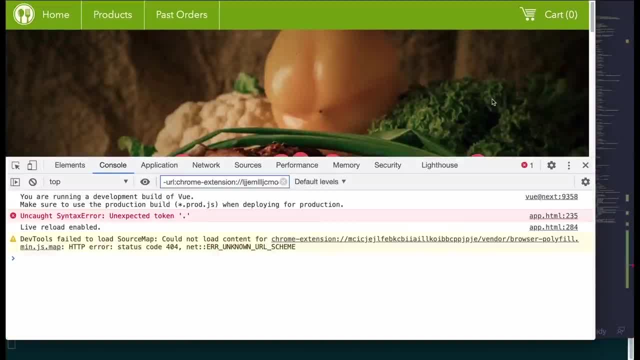 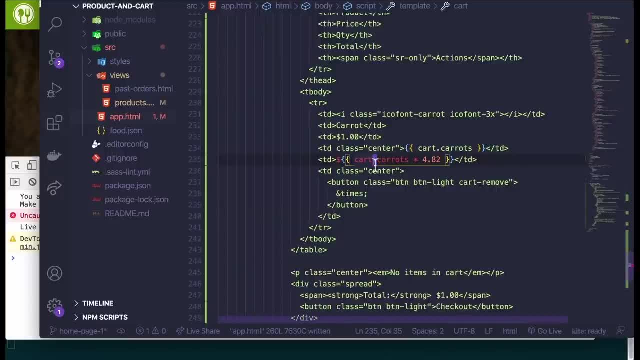 now there is an error. let's see what the error is: unexpected token with a dot. the reason why it's complaining is because a dollar sign followed by curly braces in javascript whenever you put that syntax inside of the backticks that we have around this template here. 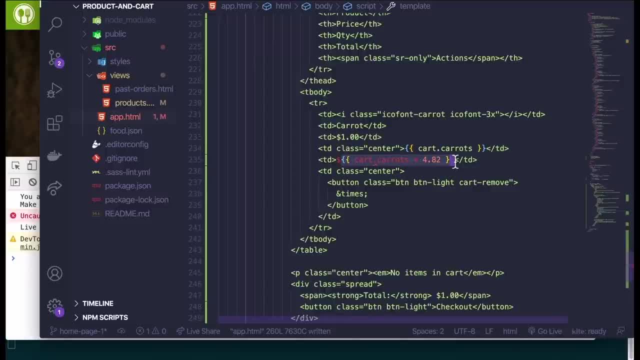 it's called a template string and it will parse whatever is inside those outer curly braces as javascript. so it thinks we're trying to pass in a javascript object and it's complaining because cart dot carrots is not a valid key. so the only thing we have to do here 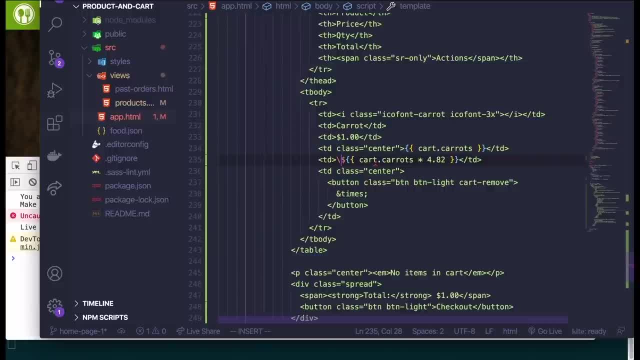 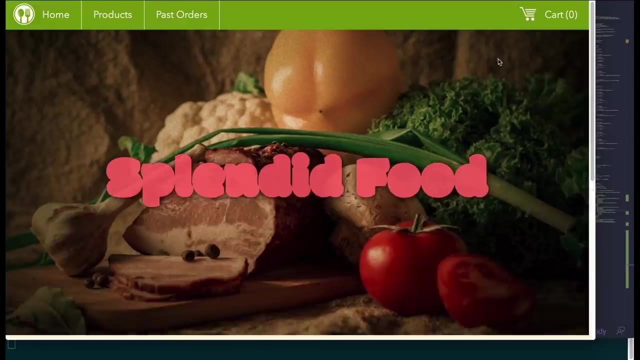 is actually escape the dollar sign. so javascript doesn't think we're trying to use a template string and pass in a variable, and then Vue can just parse the double curly brace syntax. on its own this should work, so let me go to cart. now. my cart opens. 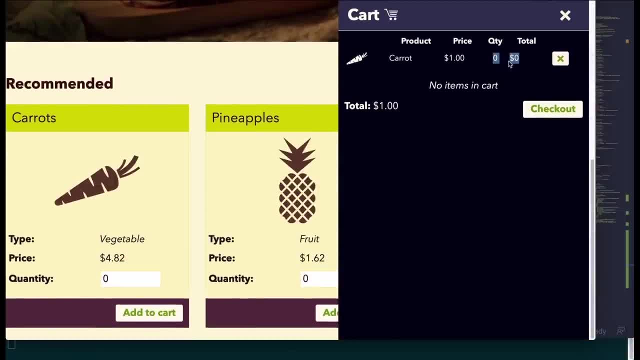 as normal. you can see there's zero carrots, and now, if I add two carrots to the cart, it now gives me the correct total of nine sixty four. now I also want to have a total of all the items in the cart. I only have one item now, but I will have more items. 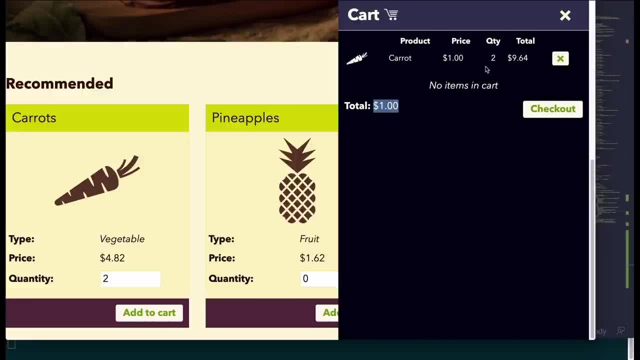 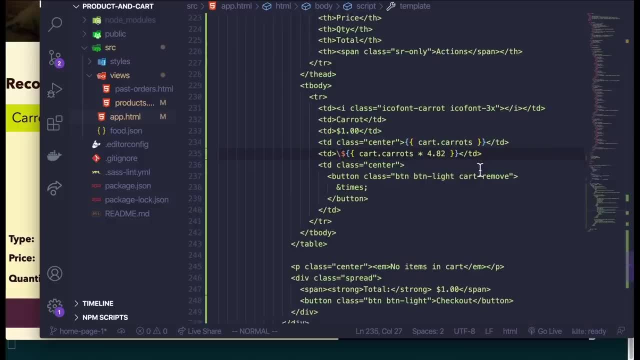 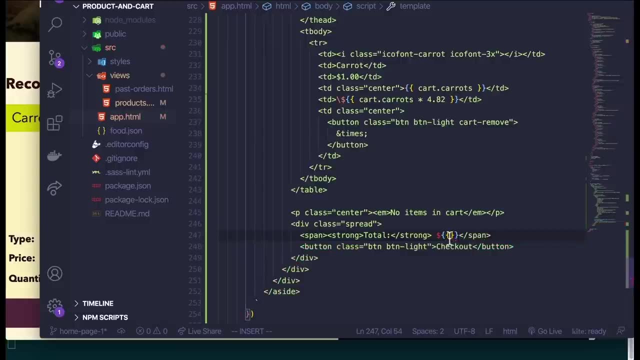 soon. so I'm going to go ahead and add a function for that, and then we will hook up the rest of the items in the next video. so back in the code here. this is the total that I want to update, so I'm going to add this and escape. 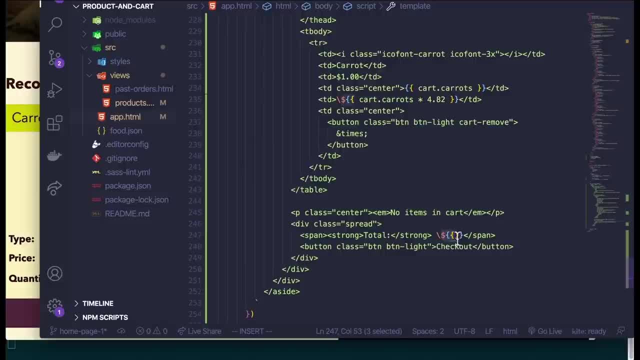 that dollar sign that comes before the double curly braces. now I could create a formula just in line here and say: cart dot carrots times the carrot price plus the second item times that price, and so on and so on. but that's not going to make a lot of sense. 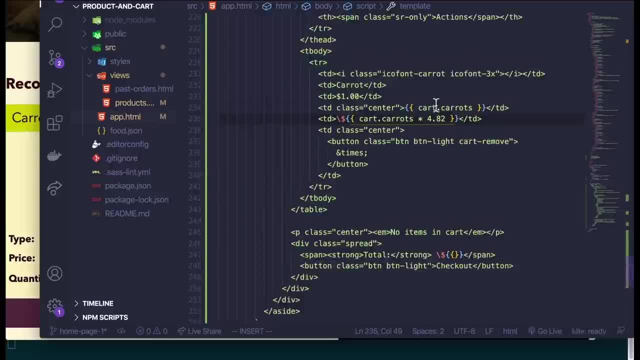 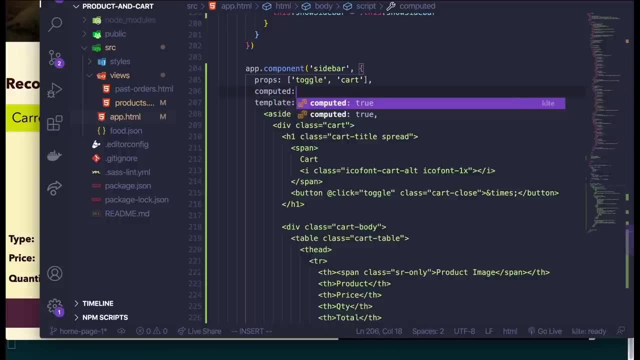 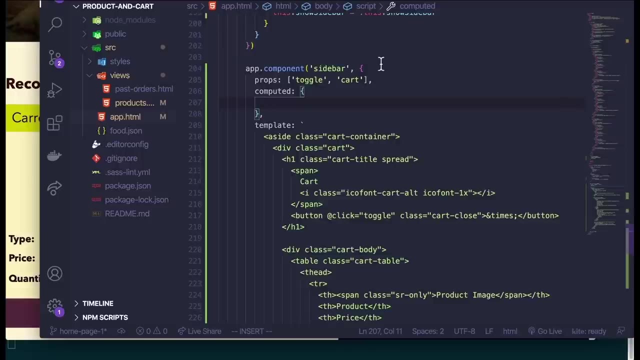 and that doesn't scale for multiple items. so what I'm going to do here is actually add a computed object and if you remember, computed watches the changes in variables and will update the result. so I'll call this computed function, cart total and on my cart up here: 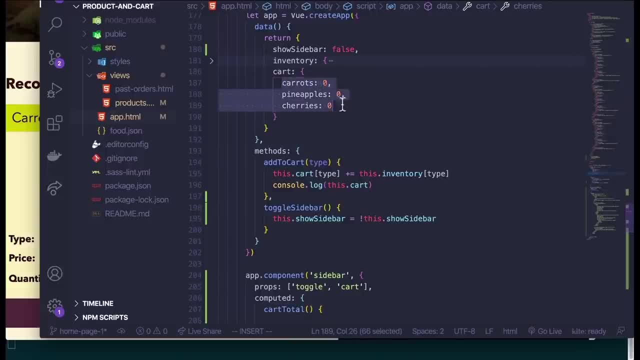 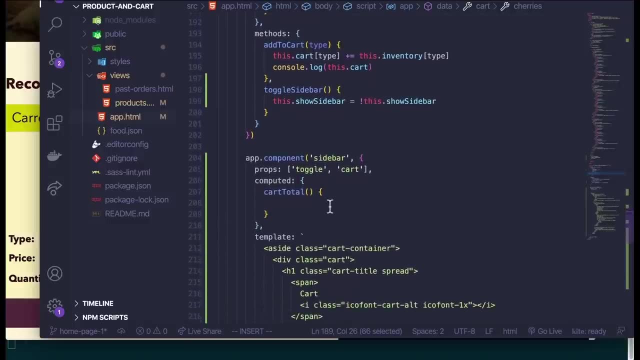 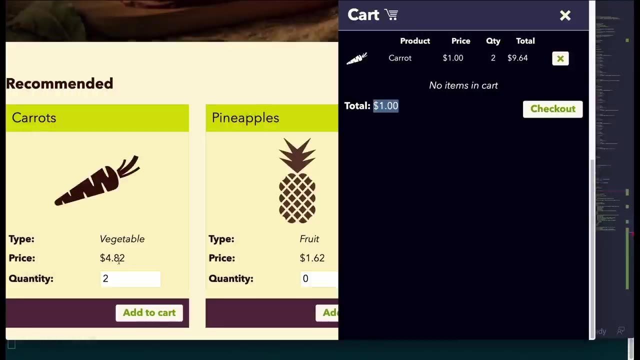 right now I have just the number of each item. so for right now I'm just going to hard code the price down here. so I'm going to return cart dot carrots times the price, which is 482, and now I can take this computed variable that I created. 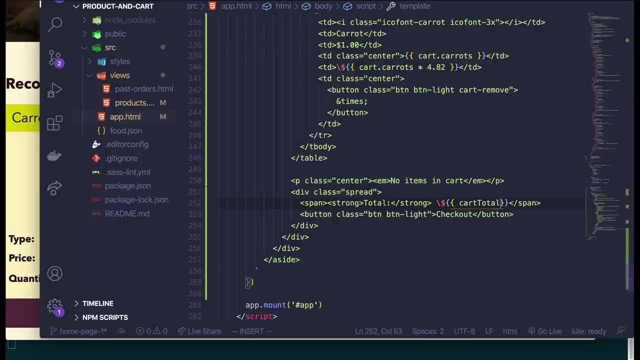 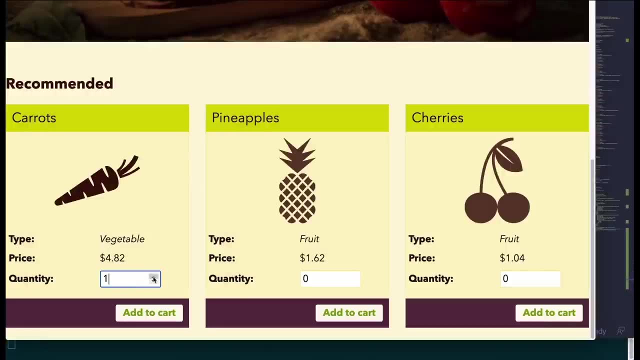 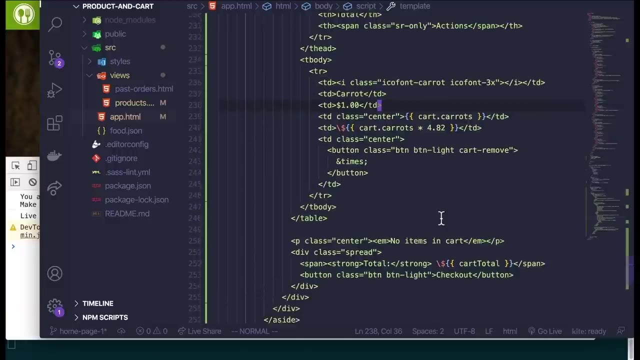 and put it in here and now. the cart total that I created should be updated every single time. let's see if this works. add to cart. open my cart and there is a bug because it's not opening. I'm stepping through, trying to figure out why the cart total isn't. 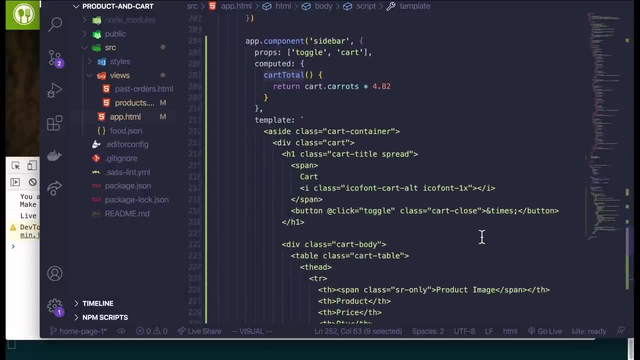 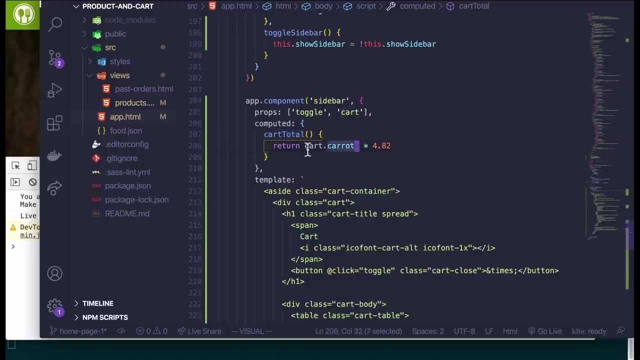 working and it is because I have accessed it incorrectly. so cart dot carrots has to be accessed. this is inside of javascript, so I need to access it on the this context in my component. so I have to access it on this dot cart dot carrots and that should come up with my number. 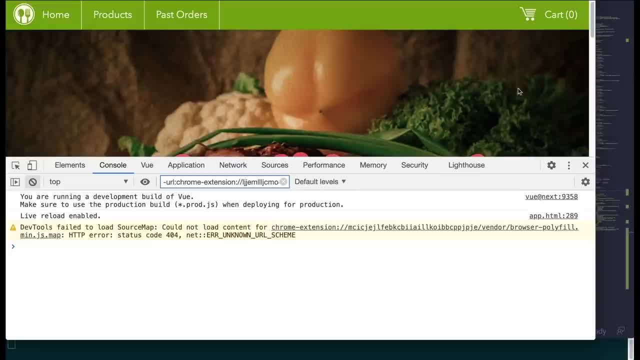 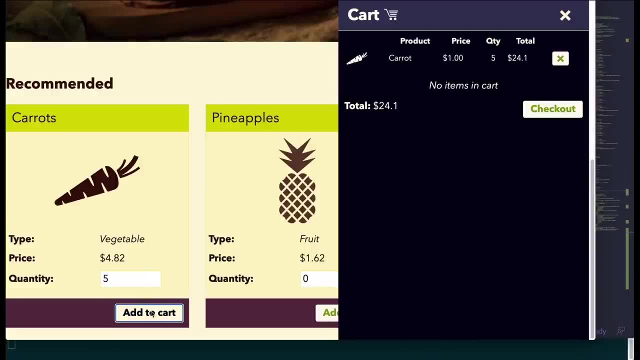 times that number. so let me go back to my page. and now it opens and if I add items I can see it's 24 dollars and 10 cents. of course this isn't that pretty. sometimes it rounds it to one, or sometimes there's only one decimal. 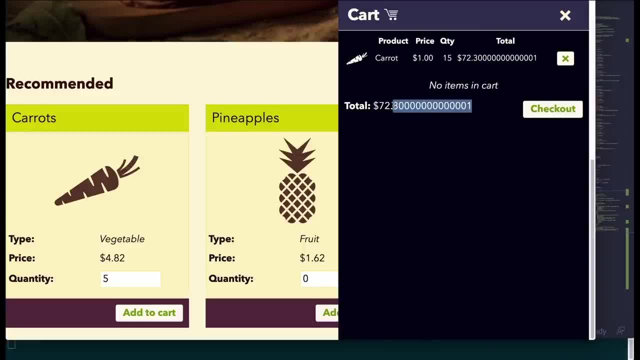 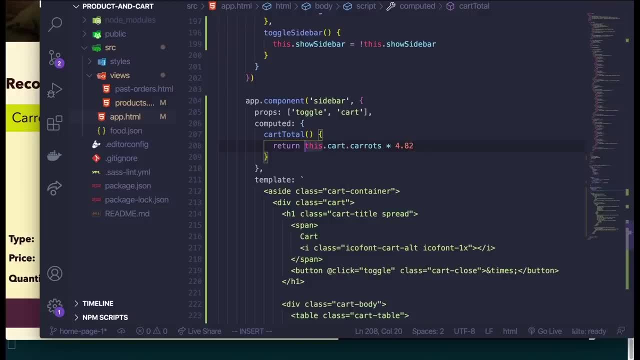 and sometimes there's like 10 here. so let's just round this really quick using something built in in javascript, so we just get two decimals. I'm going to wrap this here: dot two fixed and then the number two and let's go back to the browser. 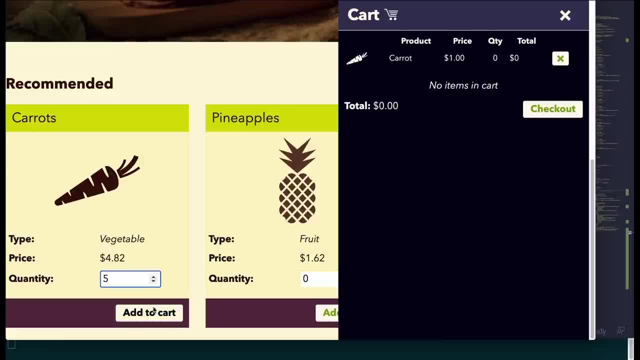 I'm going to open up the cart, add a few items and now it's at two decimals exactly, always two. okay, I'm going to leave it there in this video again, please try out implementing these features on your own from the example code you should be able to check out. 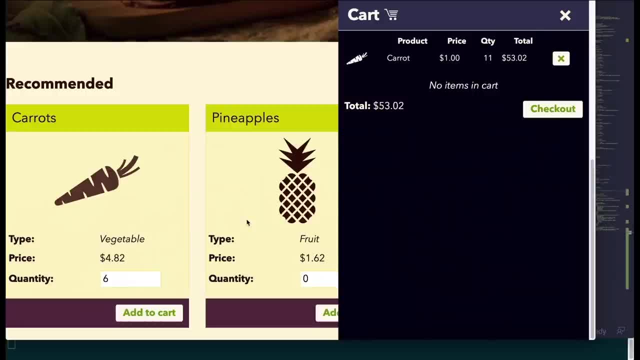 the starter branch, called home page, one from the repository and start exactly where I did at the beginning of this video. in the next video we will cover adding all of the rest of the items to the cart by importing them into our javascript, so we can use loops to make our code more efficient. 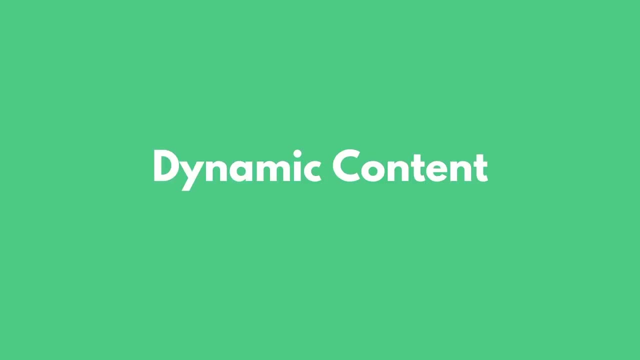 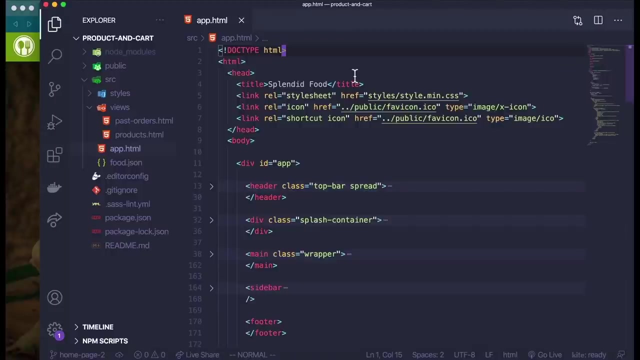 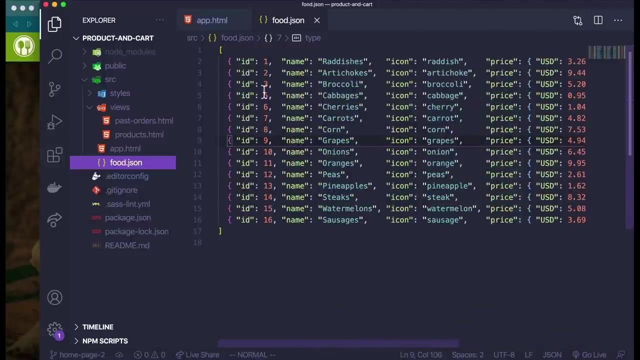 and not have to hard code everything in this video. we are going to pull in dynamic content to populate our page and that will be from this foodjson file, so this actually has a list of objects, of all different kinds of groceries that we are going to display. 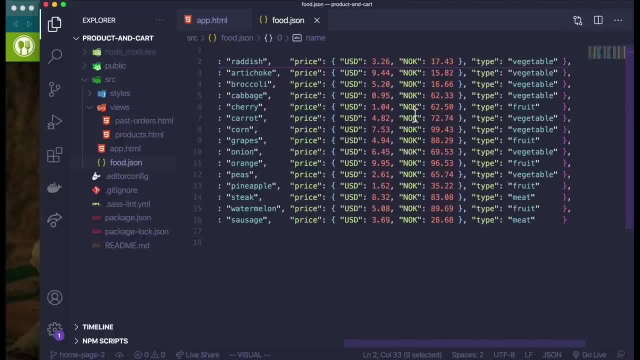 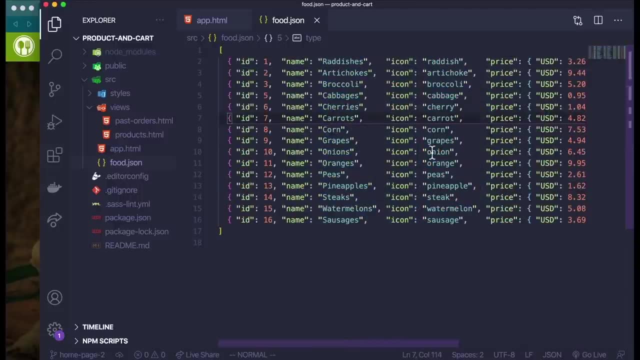 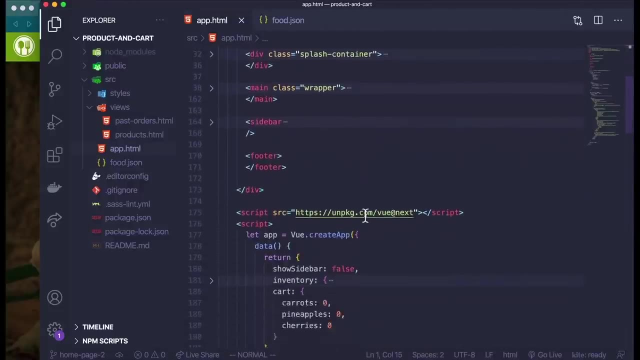 in our app. it has some information like the names, as well as the price, and then even if we want to add a filter to sort by the type. so how can we pull this into our application? actually, we are going to use lifecycle hooks in Vuejs for this, if we come. 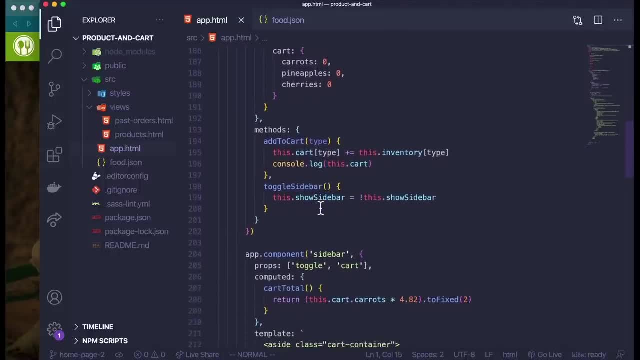 to our main Vue application. here below methods, I am going to add a mounted hook, just like we had before, and inside of here I am going to fetch this json data and that is going to be an asynchronous call, so I first need to fetch this from the file name, which is: 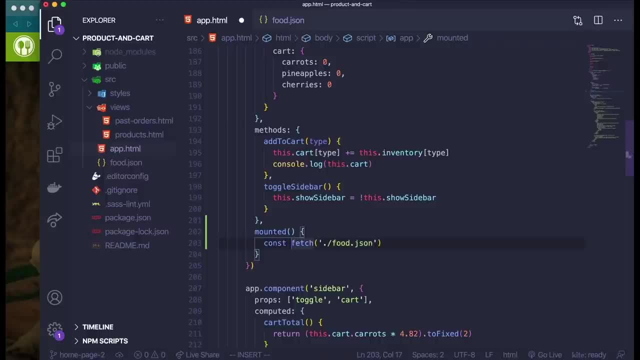 foodjson and I am going to call this the response, and then I need to call the json method on that response, which I will put on this line and that will be data and actually I need to add a weight to these calls. so, resjson, I can call that method. 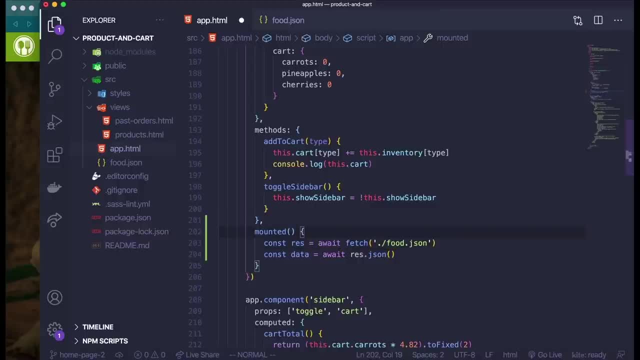 I am going to await this as well, and then, because I am using await, I need to add async to this mounted method. so now I have created the mounted lifecycle hook, I get my data, which is the array of all of the food objects, and now that I have 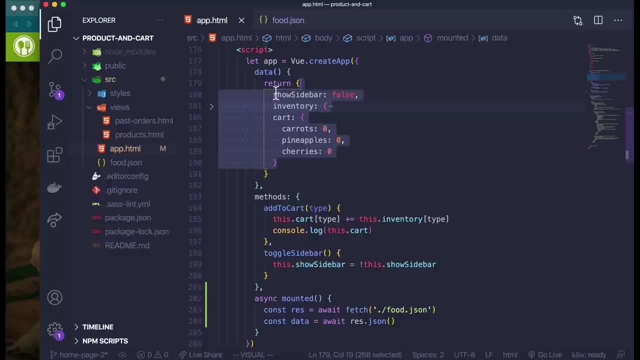 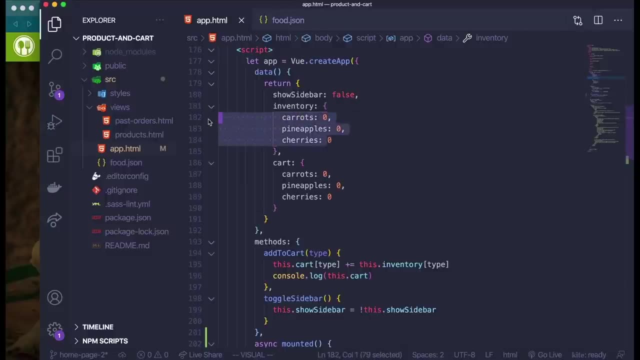 my data. I am going to set it on state here. so instead of inventory here, I am going to replace inventory. just get rid of all this dummy data that I have right now set it as an empty array. this will definitely break my application right now, but it is okay. 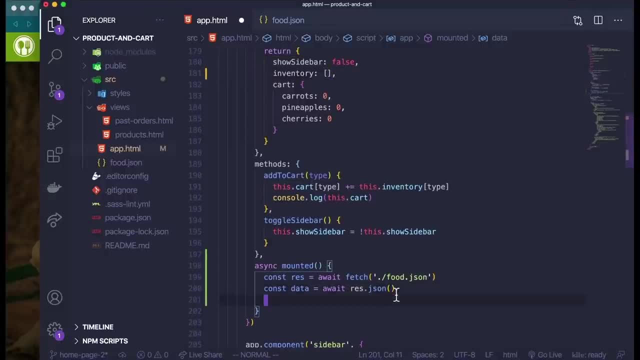 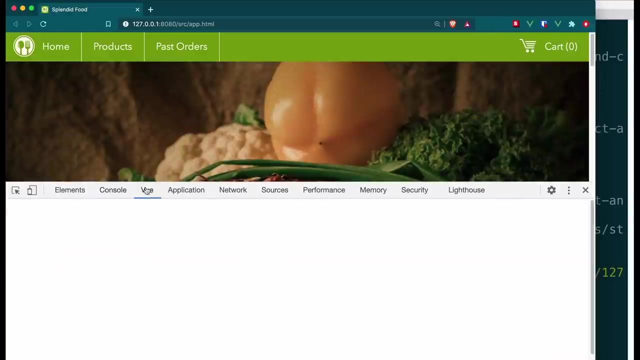 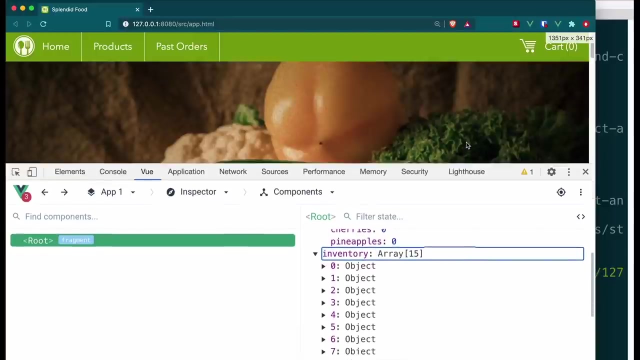 because it is a step toward fixing it. so now I am going to set this dot inventory equal to data. let's see if that even works. and I am going to come to my view. here I can see my root and I can see that the inventory in my 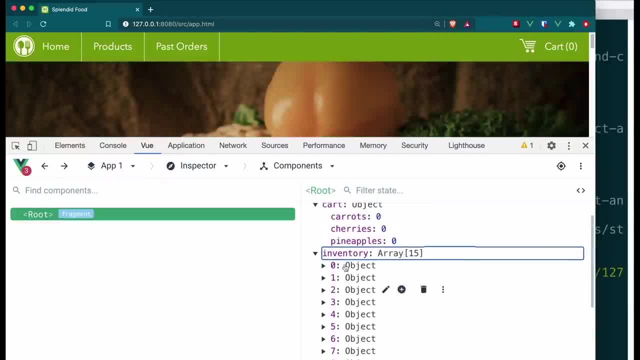 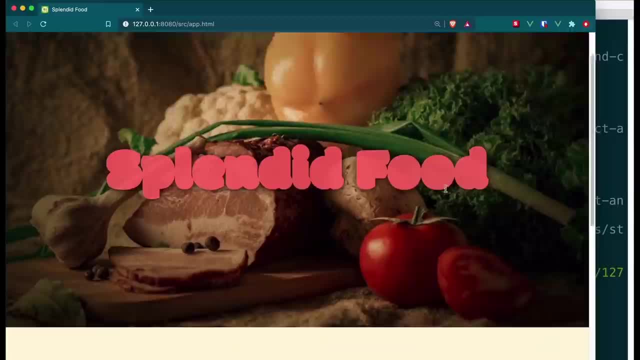 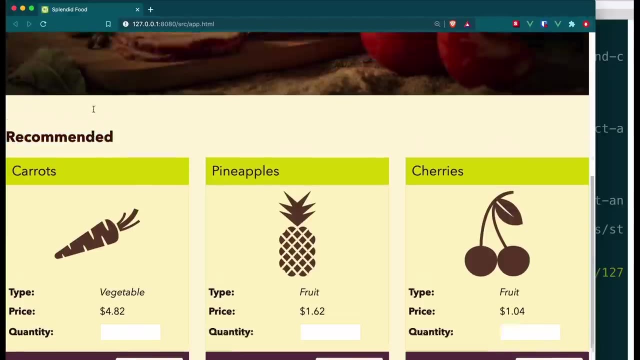 root element here that I have all 15 items. good, so I know my data is working. now the next two things I need to do are display that data on this page here, and so these are just three recommended items. actually, all of the products will display on this page. 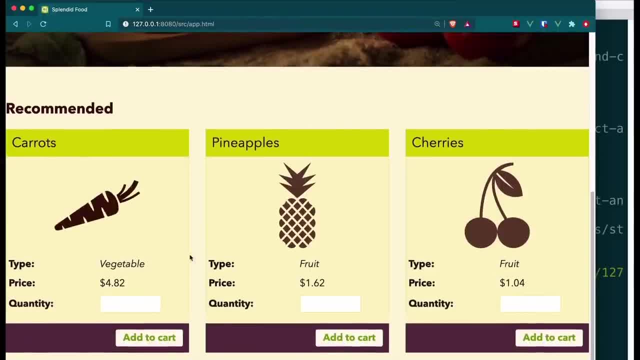 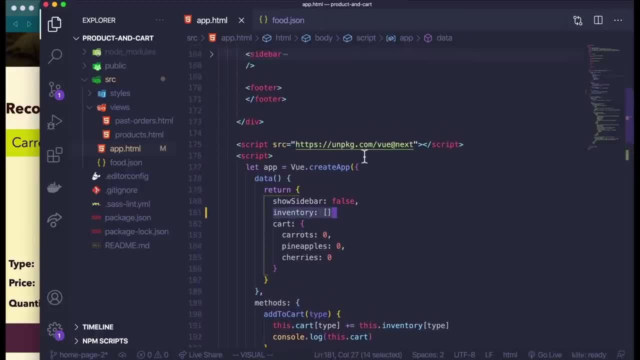 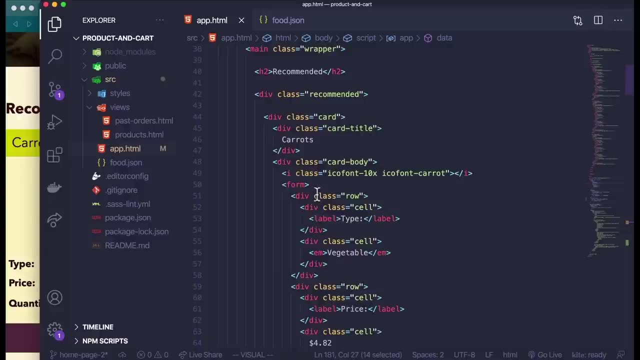 so for the home page, I am just going to display the first three and slice that list as I loop over it. so now that I have inventory, I am actually going to come up here to my main container and I am going to come to the recommended section. 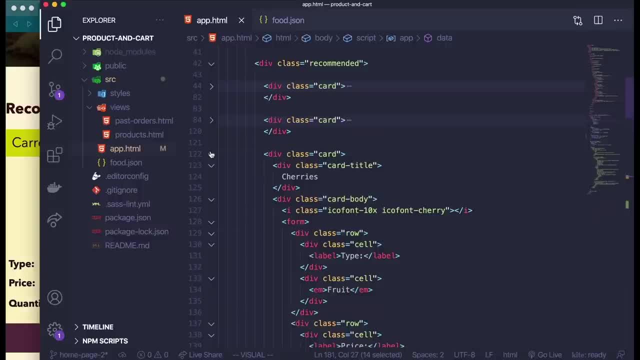 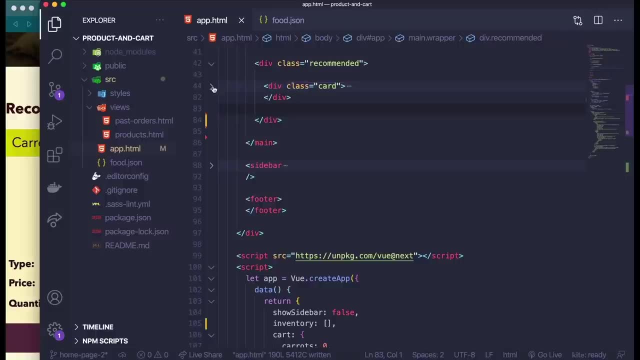 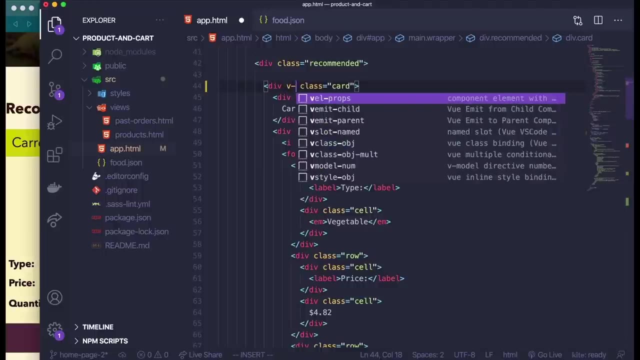 and fold all of these cards and get rid of the last two, because I am only going to need one for my loop. and now, with this initial card, I am going to turn it into a v4 loop and loop over each item in that inventory array. so equals. 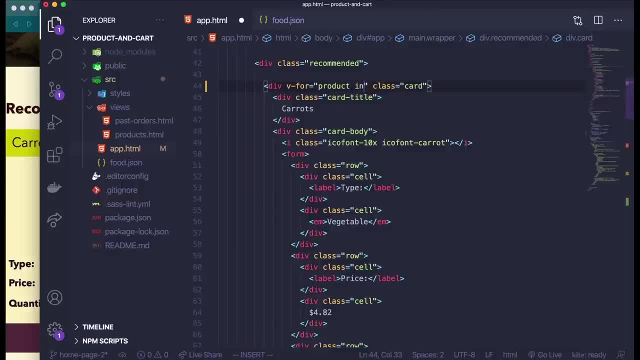 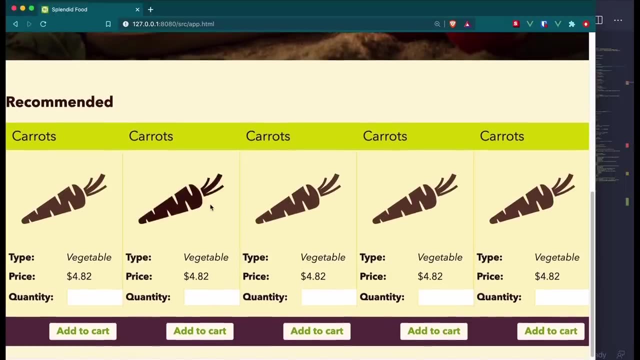 product in inventory. let me just see what this looks like really quick, and yes, it tries to loop through every single item in the whole inventory. so I am going to slice it at three items now and I can do this because inside of my view directive I can. 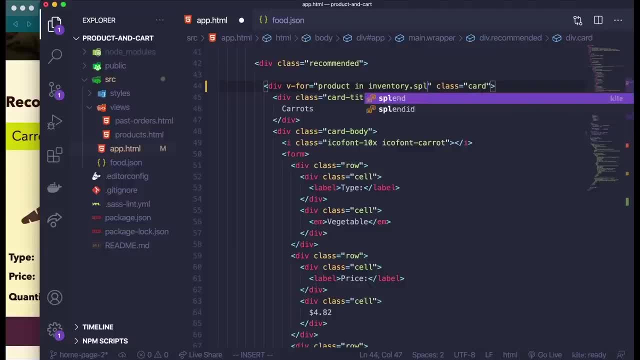 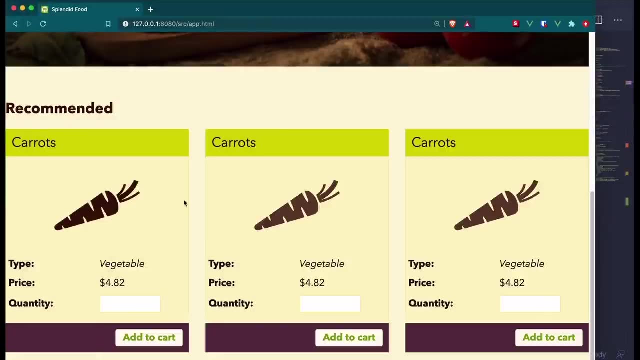 put valid javascript. so I am going to do slice from 0 to 3, and now I will go back to my page and you can see I only have three items now. of course it is only displaying because that is all still hard coded, so let me put some dynamic. 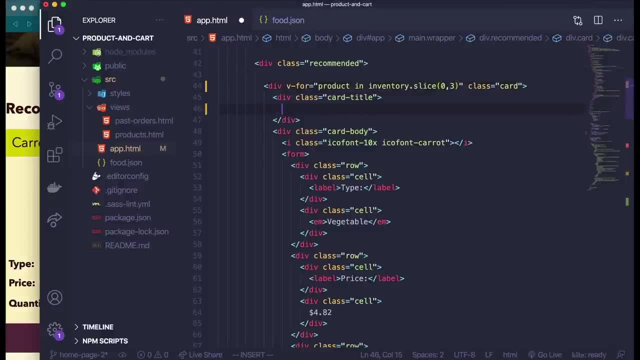 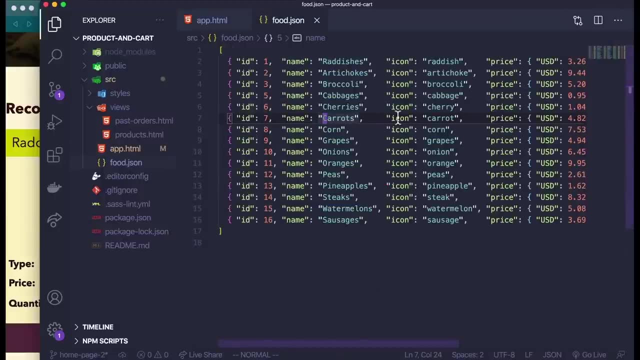 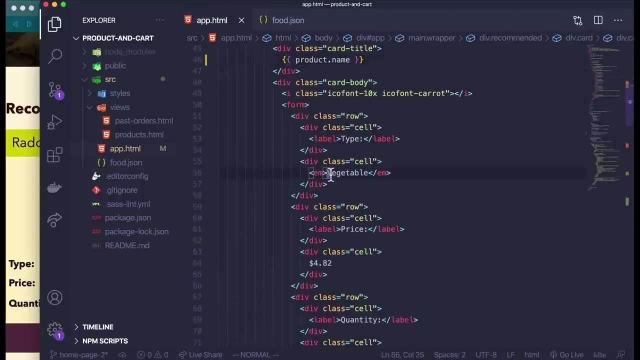 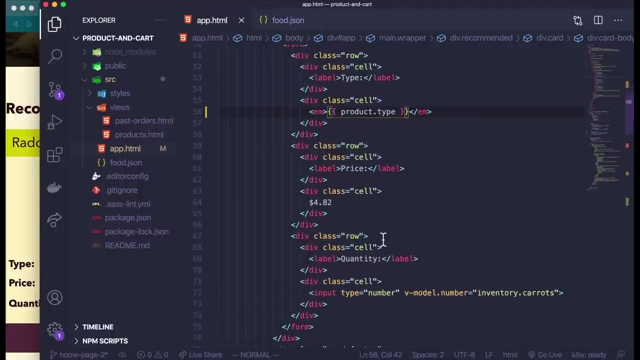 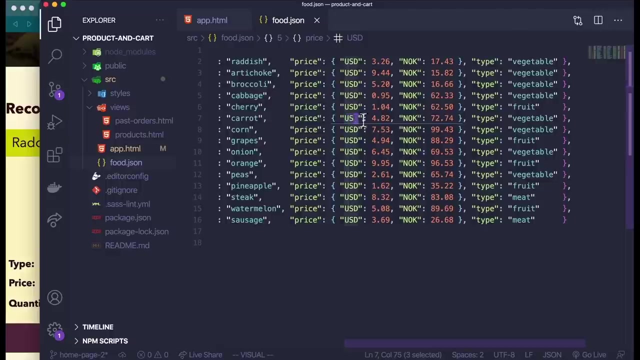 content in here, and first with the name. I am going to put productname and then I believe it is producttype. yes, so here I will put producttype and for the price. now I do have prices in two different currencies. I am just going to use US dollars. 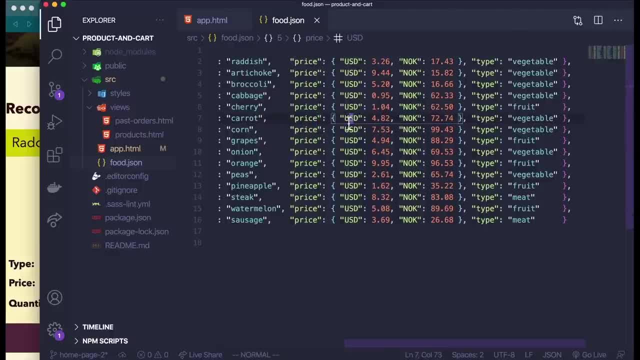 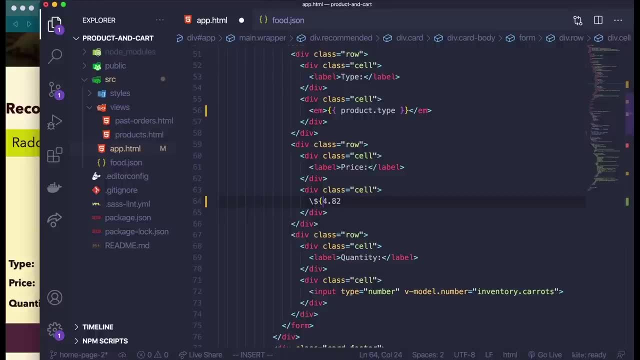 for right now. so I need to access priceusd, and so here I am going to go ahead and escape this and then do productprice usd, usd. and actually this is just an html template. this isn't inside of a javascript template string, so I don't need to escape. 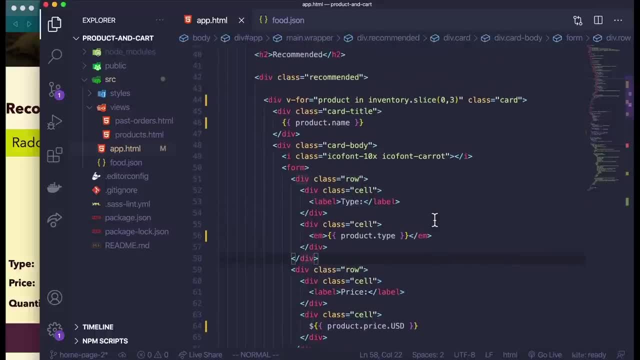 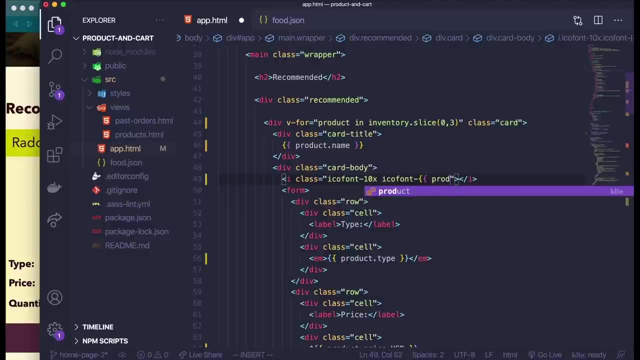 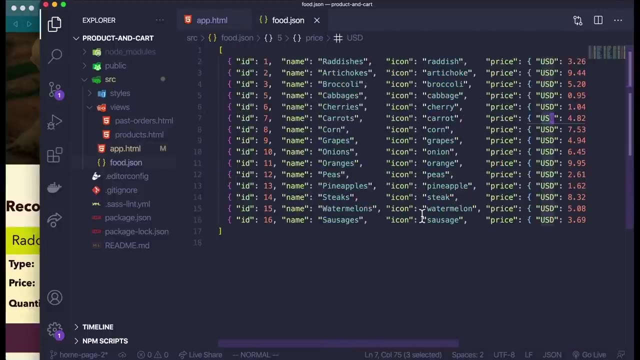 that at all, and that should be all of the dynamic content that we need for right now. let's actually go ahead and update the icon as well, so that would be producticon icon. let me make sure that is the right one, yes, icon. icon. 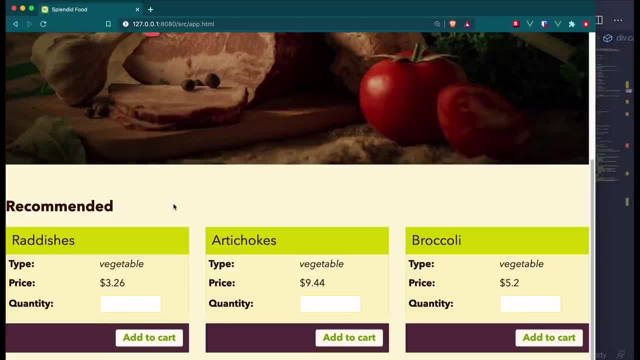 ok, so let me go to the page. ok, so the icon is not working, but all the other data is displaying quite nicely. so now we want to add functionality so that the quantity properly updates and we can add it to the cart. of course, right now, all of these. 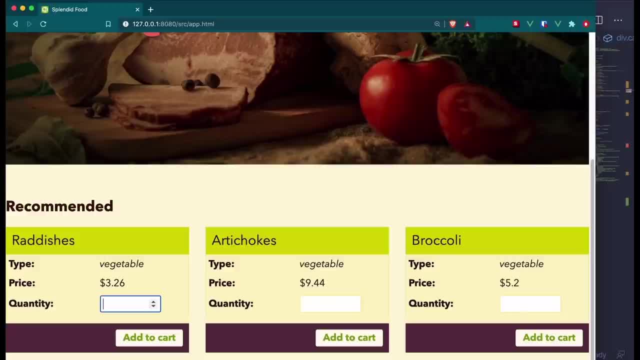 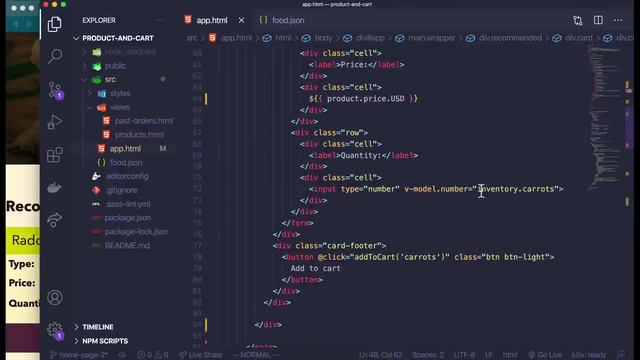 elements have the same vmodel, so that is why they are mirroring each other. so let's change that. now I am going to go to the vmodel here, which is inventorycarrots. but I need the inventory of the correct item instead of just hardcoding carrots here. 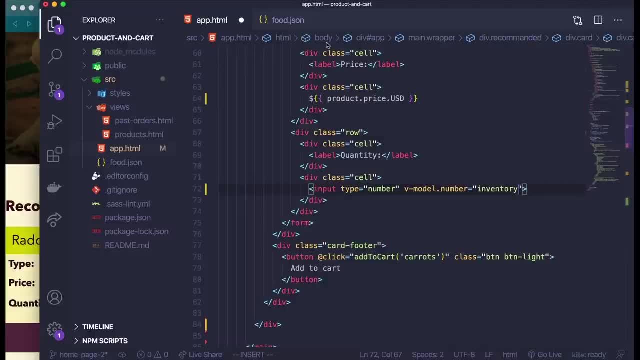 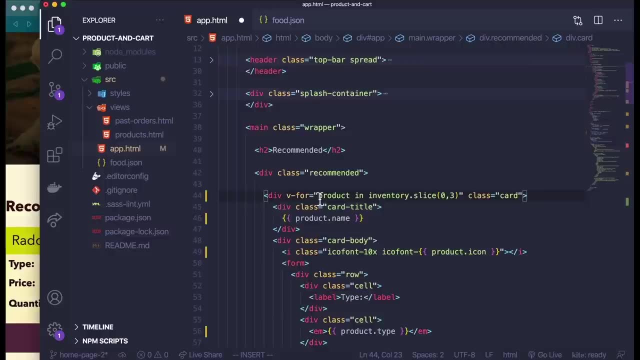 so because these numbers are in order or because this is an ordered list, I am going to come to my loop and get the index. of course I could use the id as well, but I will just use the index in the loop here. and actually I almost forgot I also need 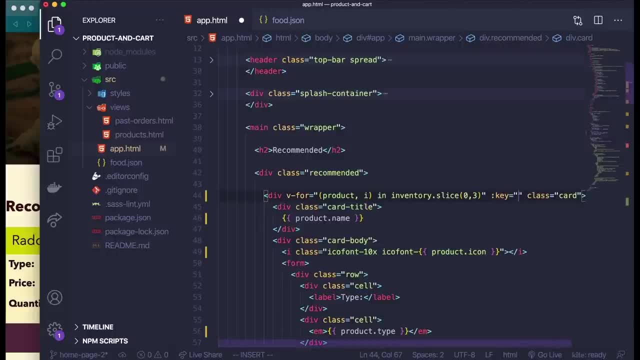 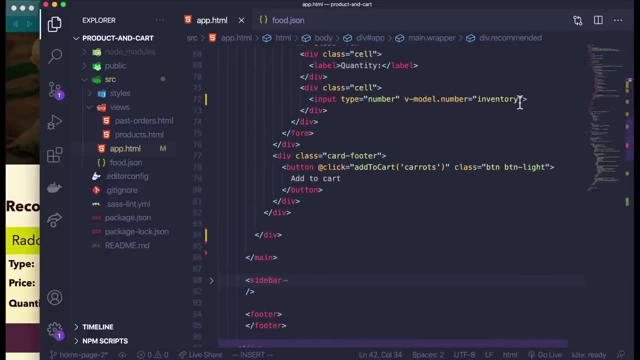 to add a key here, since I am looping, so let me add that key and I am going to come down here and in inventory I am going to pass in that index and then I am going to add a new attribute called quantity, and so this should model to an attribute called 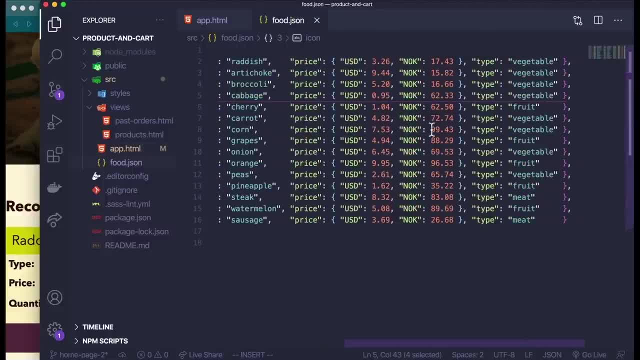 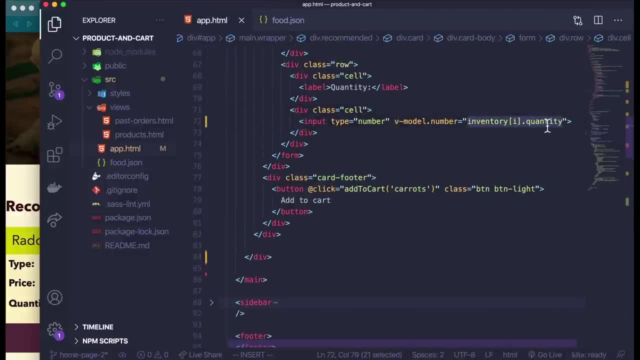 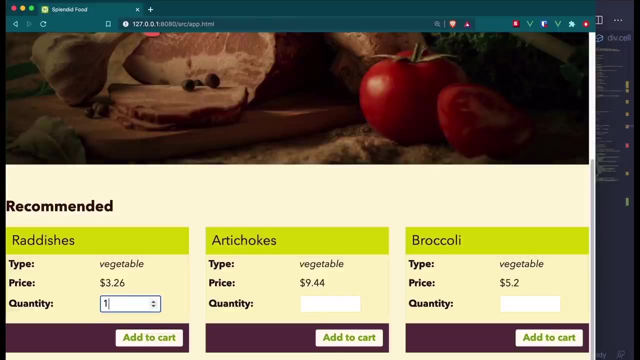 quantity, which is not currently on the objects, but that is ok, I will just leave it off, and this should just add the quantity key to the object as needed. so let's see if this works. let me go back over here. I am going to add one here. 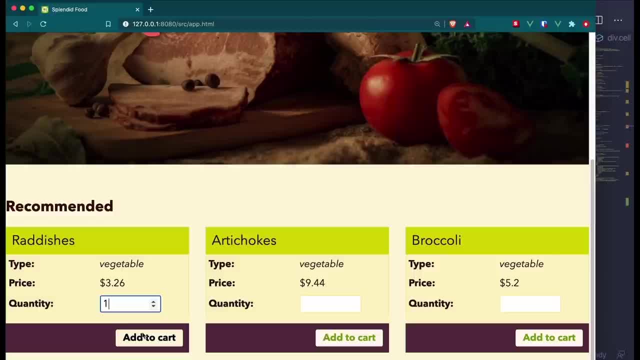 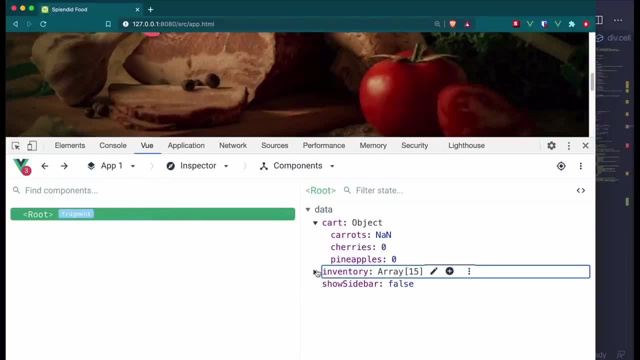 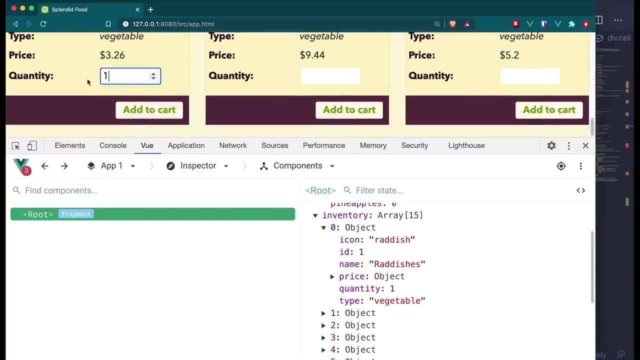 you can see they are not all mirrored for each other anymore. I am going to add it to cart and let me see how this represents, in my view, data. here I can come to inventory and I can see quantity of one. whatever number I put mirrors it. but now I need a way. 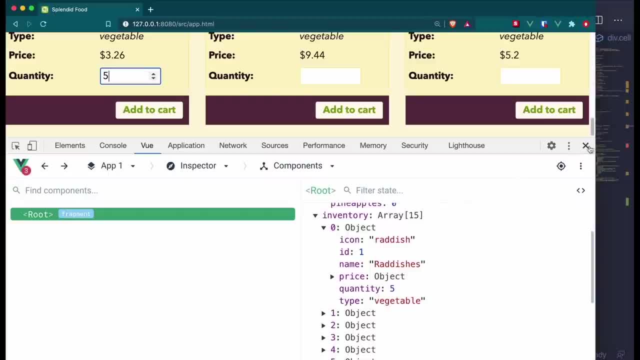 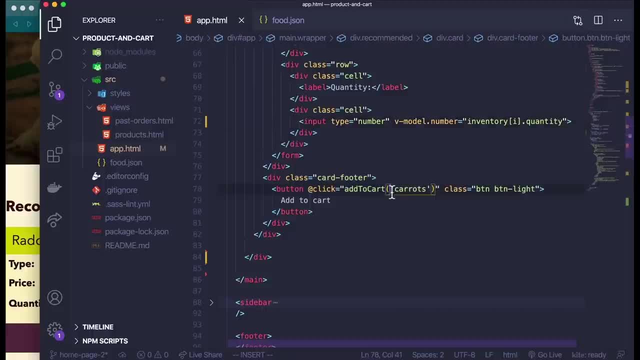 to add this to the cart. so let me set up the cart then, and here at this add to cart function. I do need to change it because I need to pass in, instead of a string, the dynamic name of the item, so I can do product dot name. 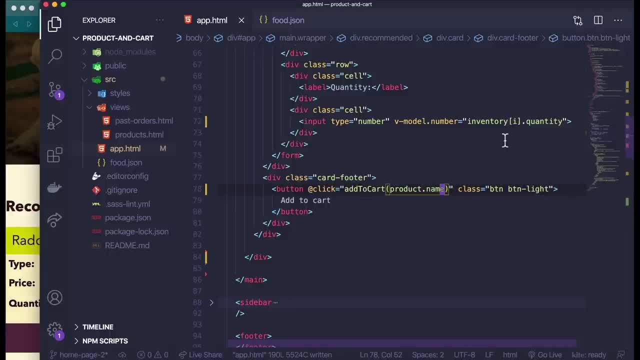 and actually here I didn't think of this, but instead of inventory and getting the inventory at index I, I already really have that in this loop. that's what the product variable is, so I am just going to replace that, and that should work just fine. now, of course, 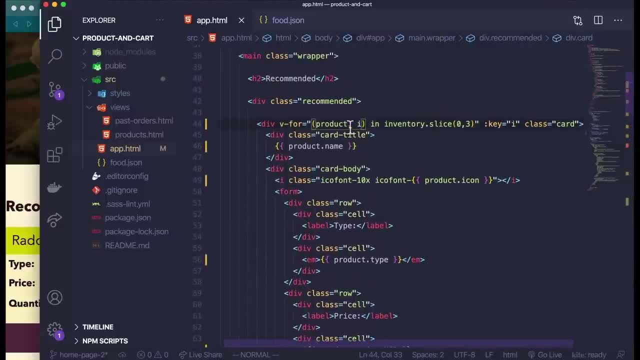 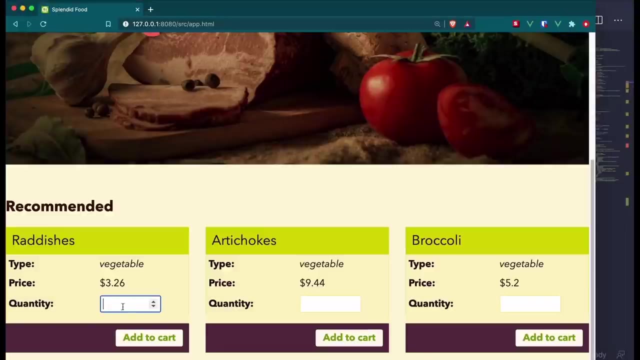 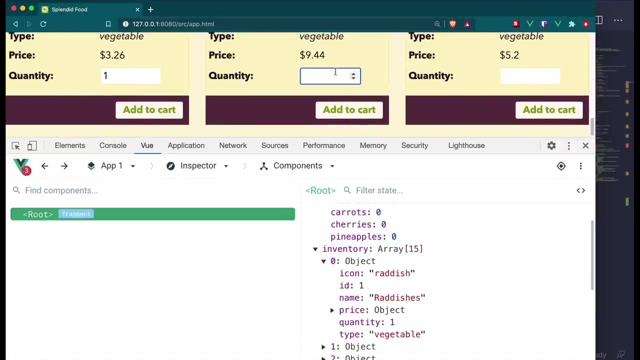 I don't really need this index anymore because for the key I can use the id of the product. so let me just use that product dot id and that should work okay. and then this should also mirror for object two. let me see if that does. yes, and the. 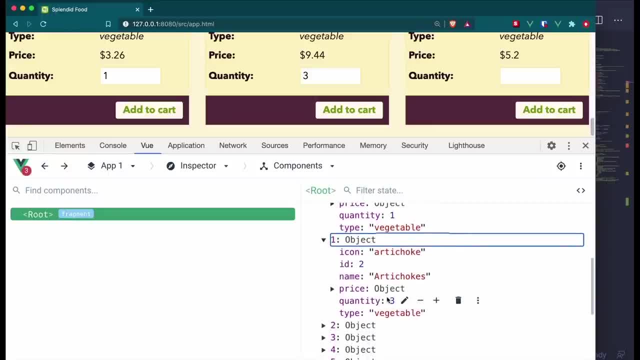 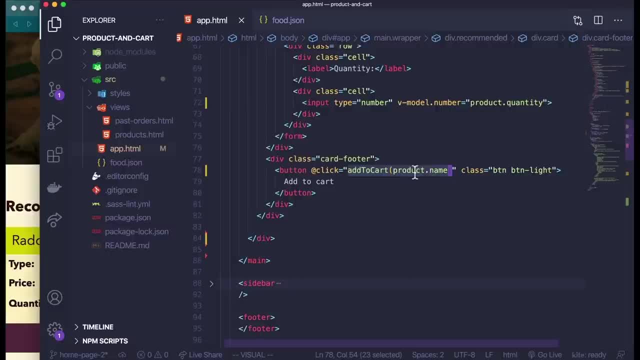 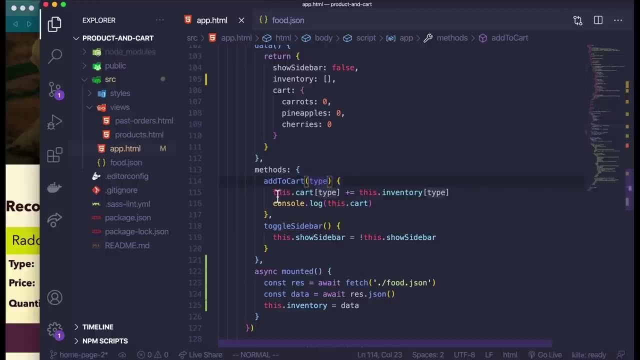 quantity is mirrored. okay, now for the cart. I'm passing in the product name as add to cart. let's take a look at the add to cart function. we are passing in the type here and then saying this: dot cart, dot type. so it will be like this: dot cart, dot radishes. 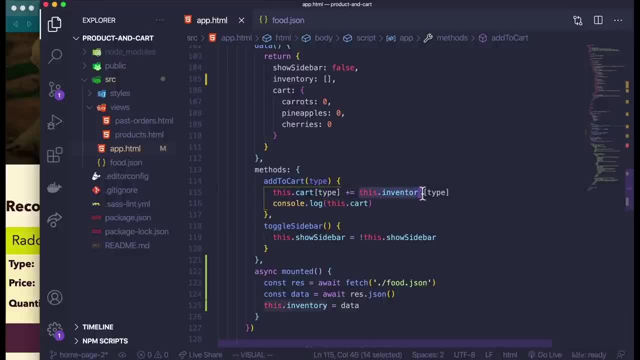 plus equals whatever the amount is at this dot inventory. so we do need to do one more thing here. we could either search and find the item by name in the inventory, or the easier thing to do would be to pass in the index of that item. so that's what we are going to do. 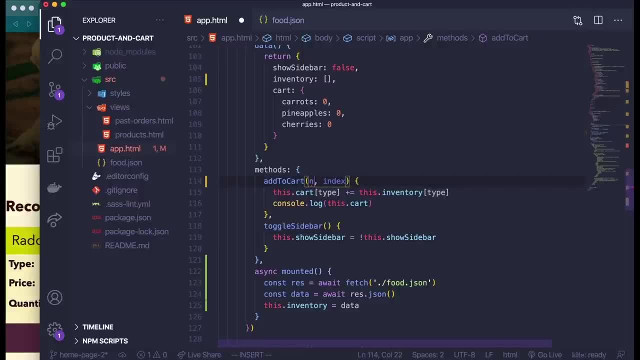 and while I am changing this instead of type now, I think it makes more sense to call it name, because it is the name of the item and we are using type for the type of item, like vegetable or fruit, not the name anymore. so now to access it. 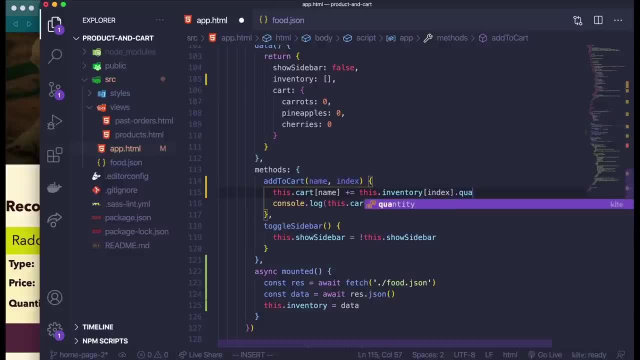 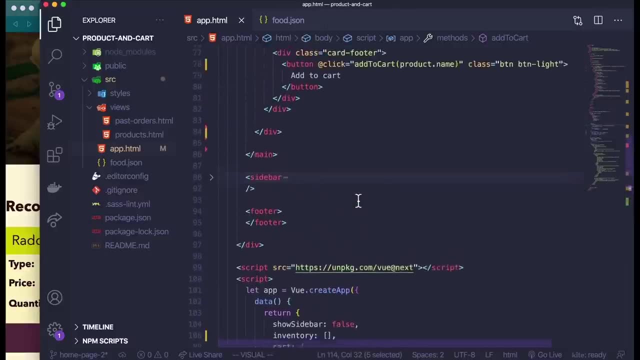 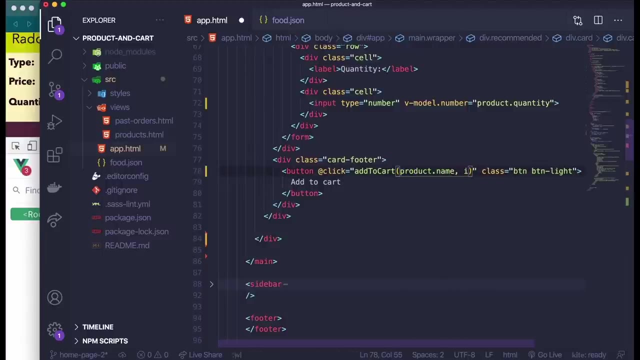 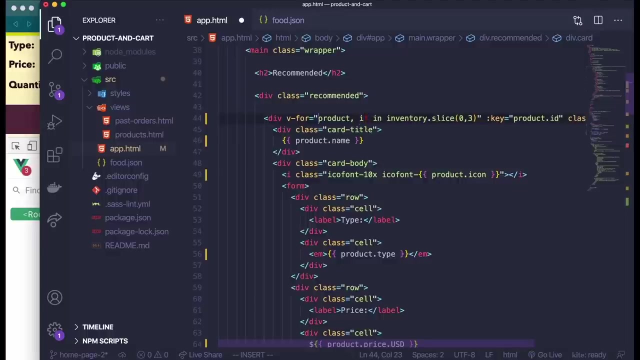 in inventory I want to do index and then dot quantity and that should work. but we have to actually pass in the index here and up here we are actually going to be passing in the index actually. so I am going to take the index here and now add to cart. 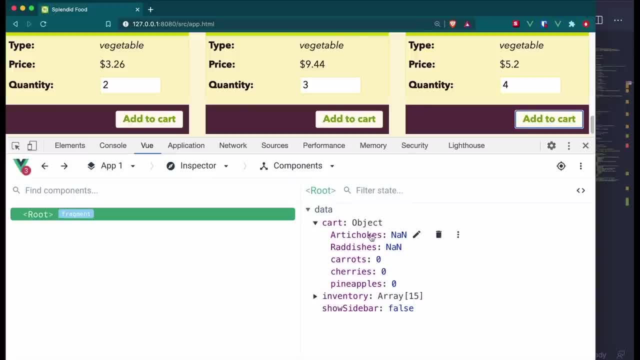 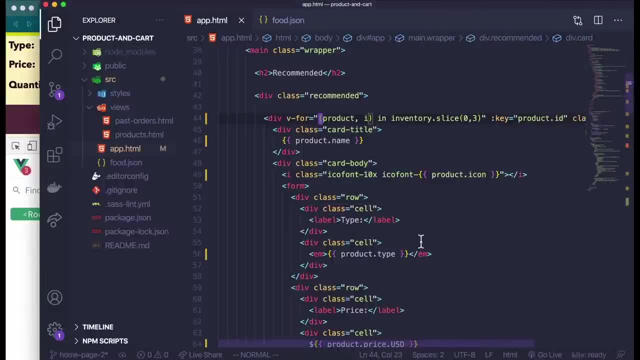 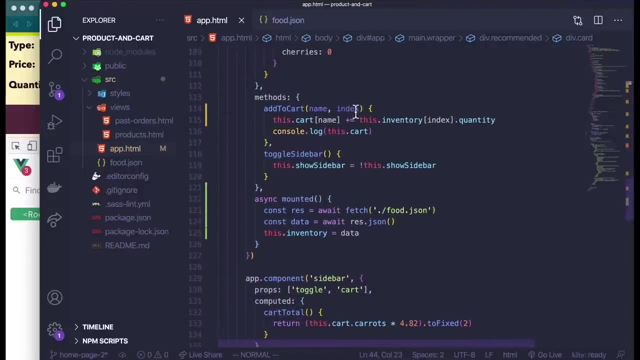 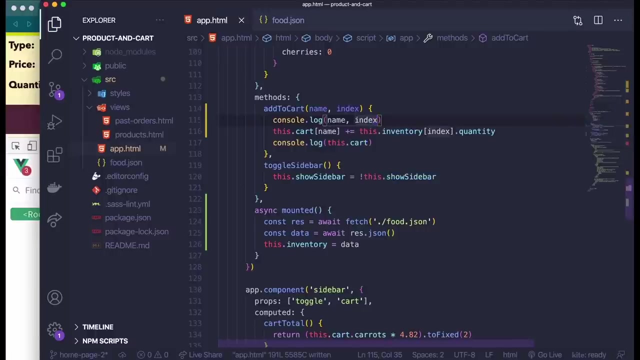 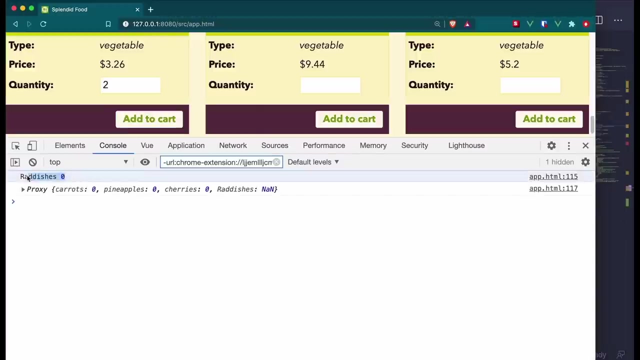 ok, so we are getting not a number for these values. so I actually want to see what we are passing in, or what gets passed in to the function, and so to debug the function quickly, I am just going to now back in the code so the arguments are getting passed into the function just. 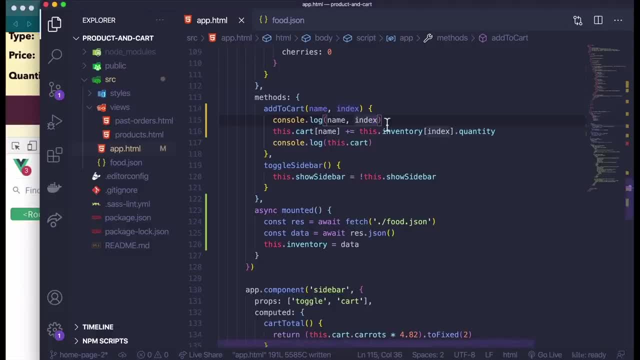 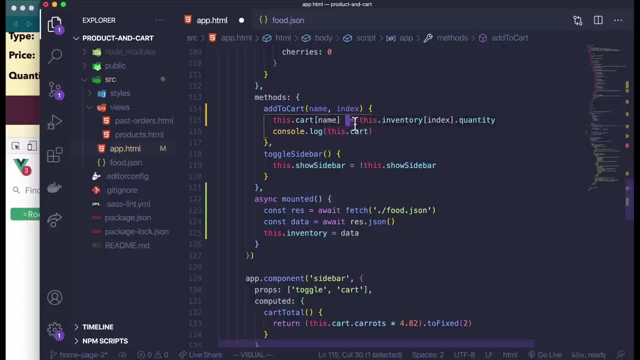 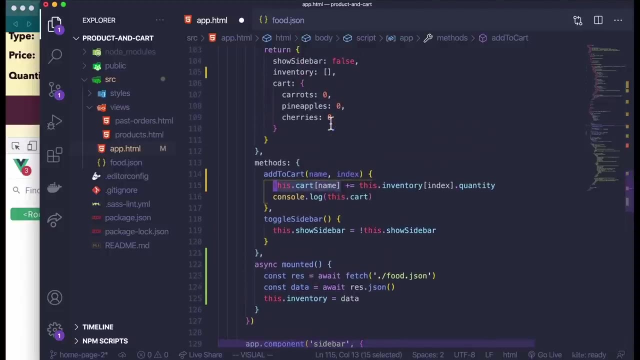 fine. so stepping back through this, I can see that my problem here is that I am doing a plus equals on cart or this dot, cart, dot name, when there is no value for that name in the cart yet. and, by the way, I am going to go ahead. 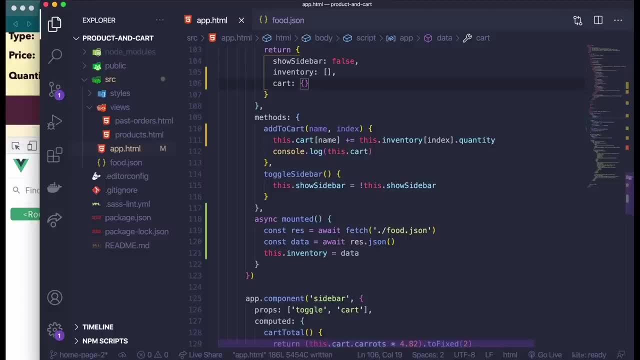 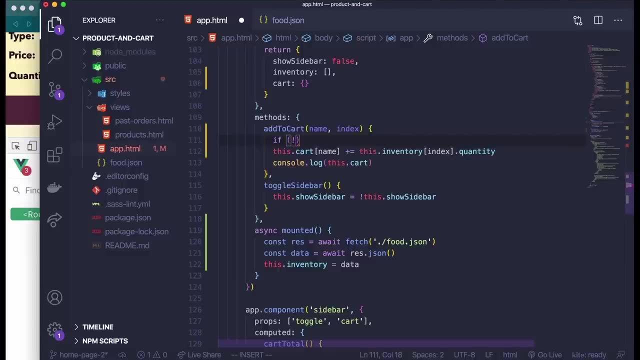 and get rid of my dummy data in the cart, and here I am just going to put a simple check. so if not this dot cart name, then I am going to set this dot cart name and equal to zero, and now this statement should work. ok, let me try again. so, 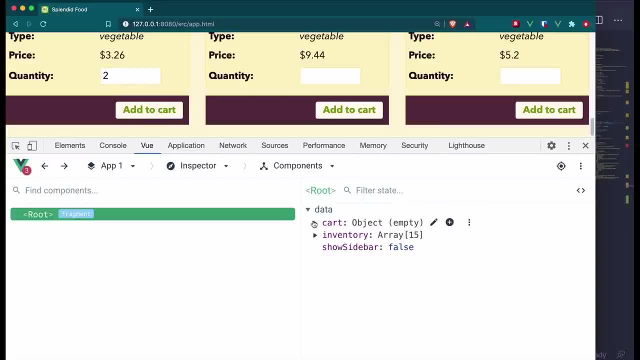 here. I am going to do two and this should update. let's see. ok, yes, it is just taking a minute for some reason, but it shows the correct number of each in the cart, no more, not a number. now that it shows it on the cart over here, I want to show it. 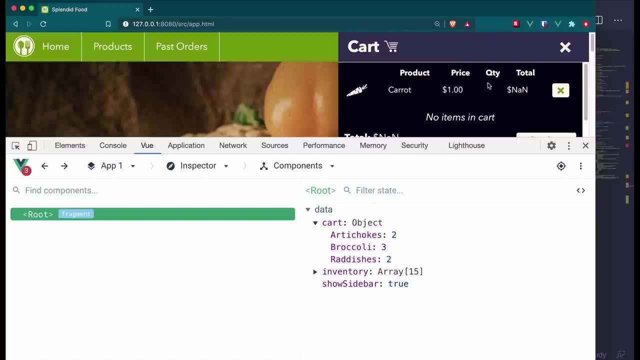 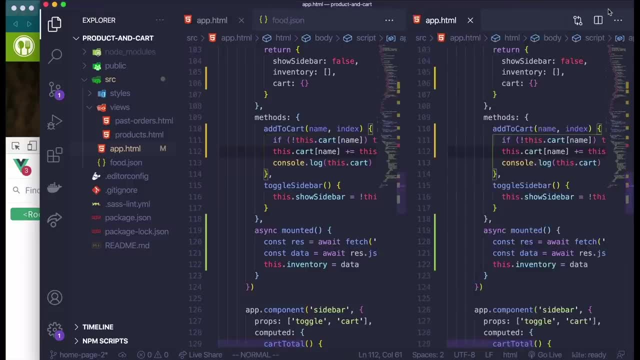 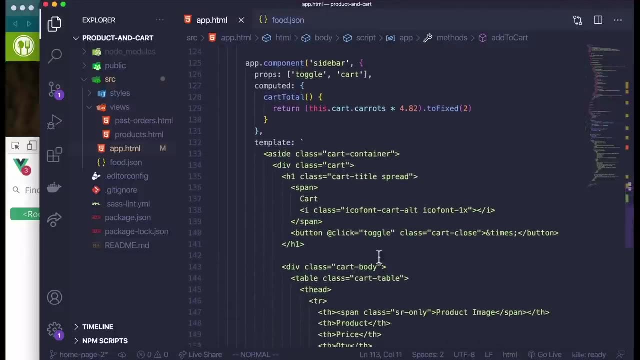 in the side bar. right now the side bar is hooked up to only look for carrots, so let's make the side bar dynamic now. so, if you remember, the side bar here is in this template, so it is part of the custom side bar component that we made. 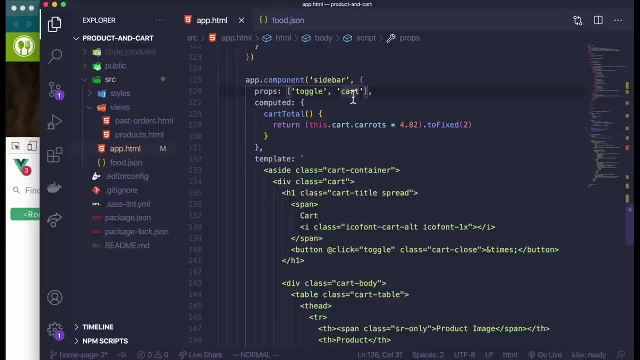 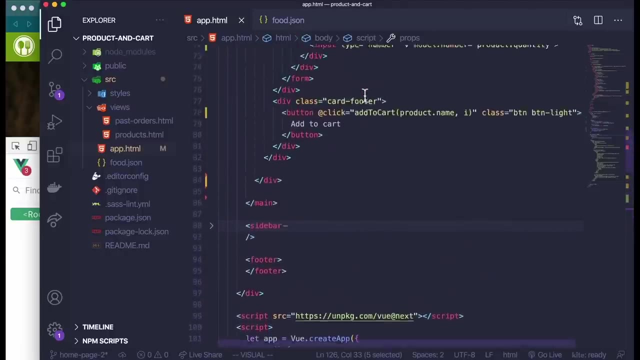 and we are already passing the cart in here. now we actually need more information, because the cart is only showing us the number of items in the cart. but we also want more information from those items, such as the price. so I am going to come up here to my side bar. 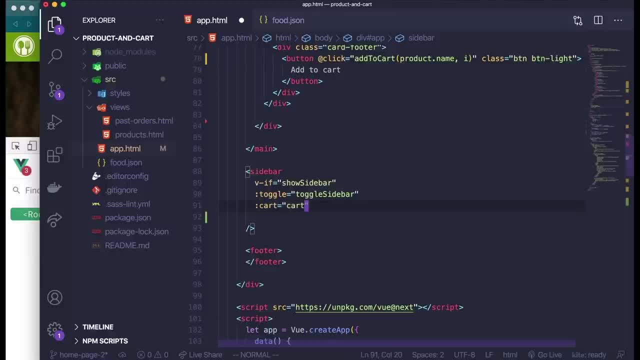 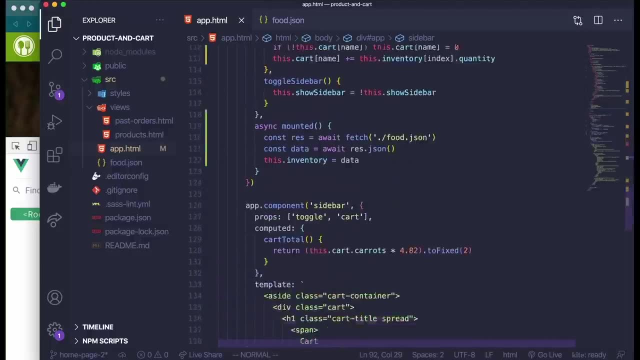 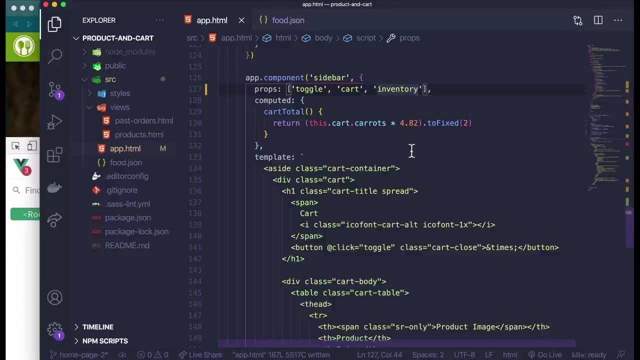 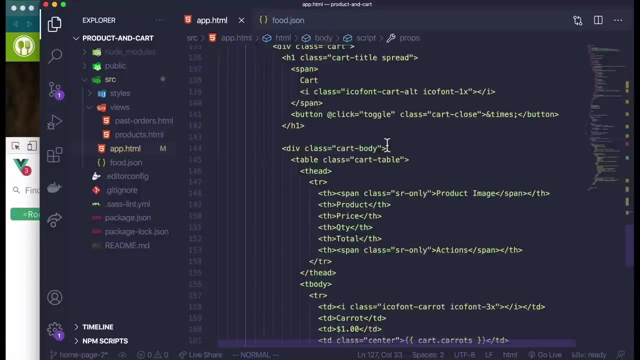 and after cart. I am going to be passing in the inventory as well as inventory, and now I can receive that as a prop in my component. so basically, we have to loop through all of the items in the cart and display their information now, and we have a table here, so we have 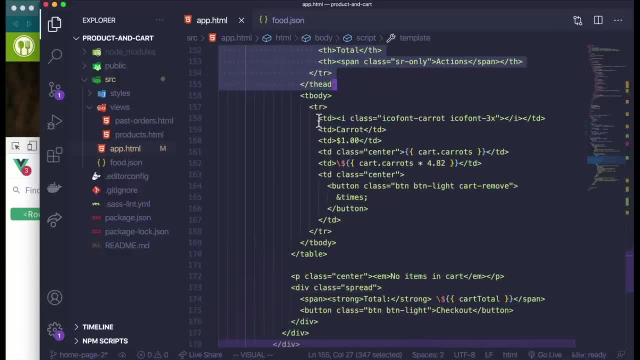 all of the headers for the table and then we can loop through these rows and basically make as many rows as we want. so I am going to go ahead and add a v4 here to loop through each item in the cart, and here I do need to. 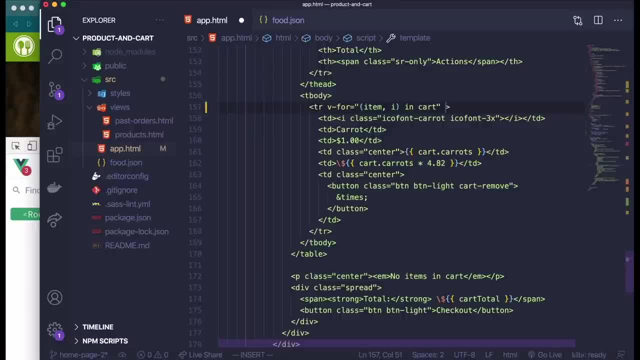 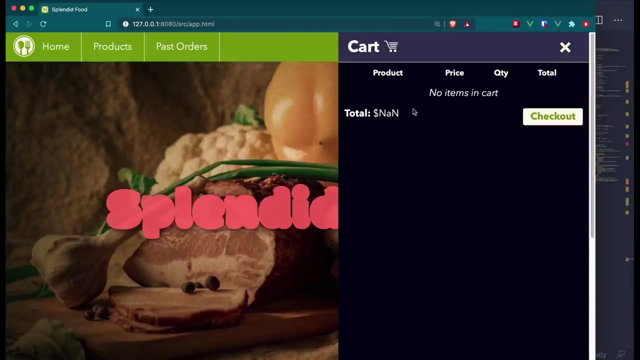 use the index. I will be using that as a key here. ok, and now these are being looped through in the side bar, so if I come to the side bar, I should see no items right now. of course, the total needs to be fixed, and now I can see I have. 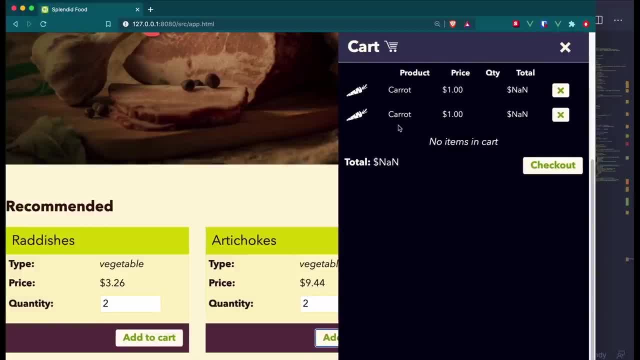 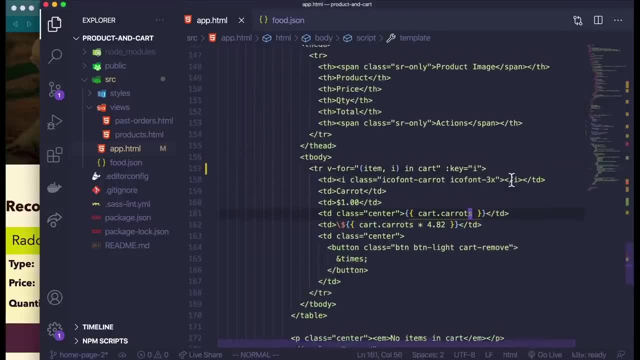 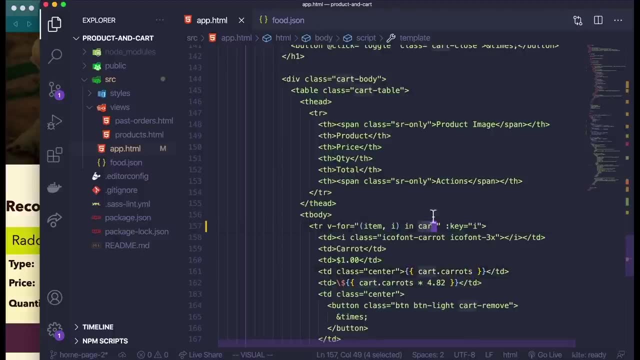 this item and now I have another item. so now I need to get rid of these hard coded names. now, to do that, I am going to go ahead and grab the key for these items in the cart and actually, because cart is an object, this index is actually going to be a key. 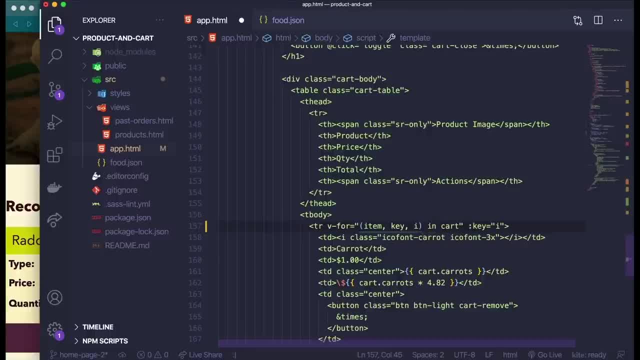 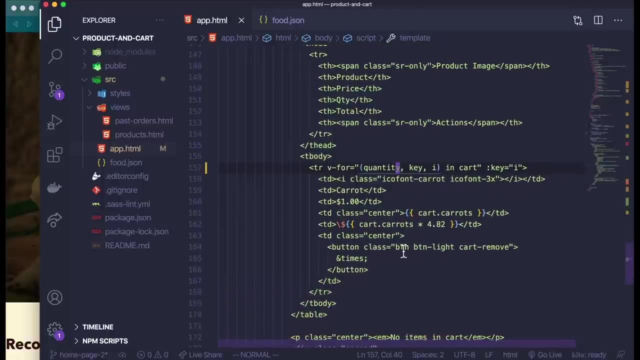 and then the third one is index, or just i. so now I have access to the item name, which is the key, the item quantity, which I will change this to the name quantity, and here I can change this to that key, and we should see the names of all of the items in our cart. 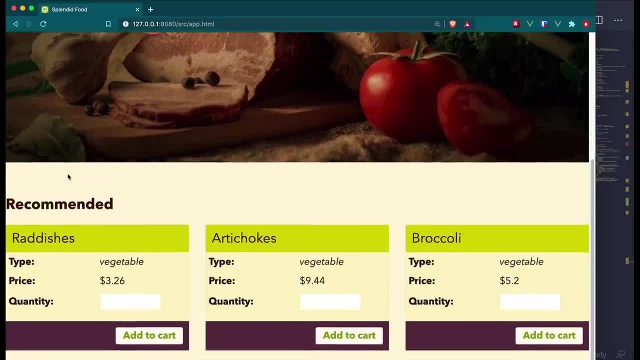 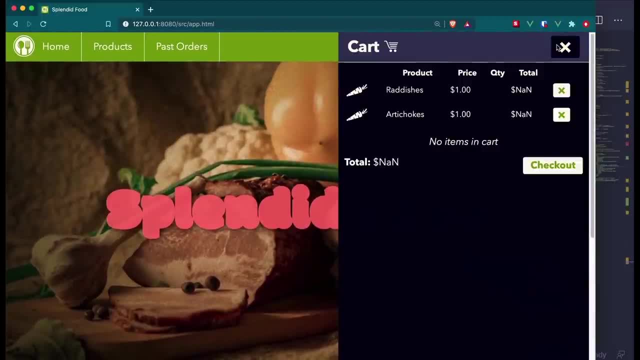 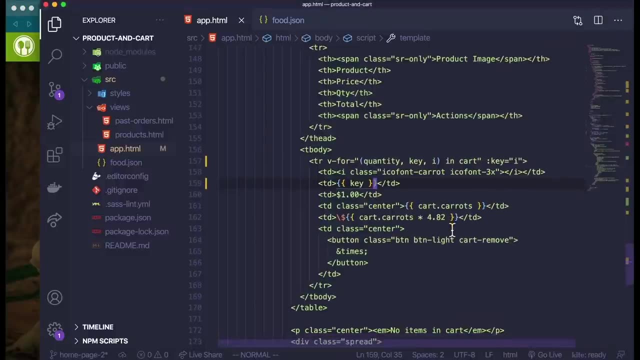 let's test this out. let me add different items to the cart. we should see radishes and artichokes, and in the cart we do indeed see radishes and artichokes. now let's display the quantity. so here we can get rid of this and say: 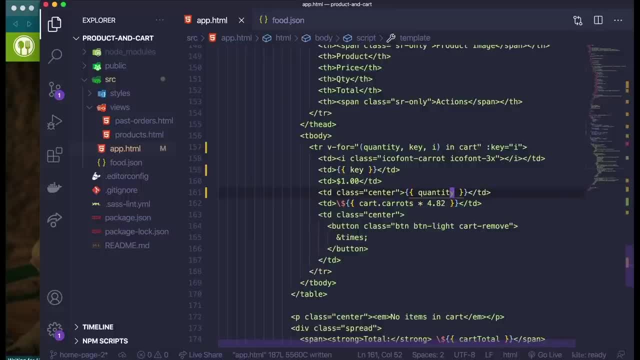 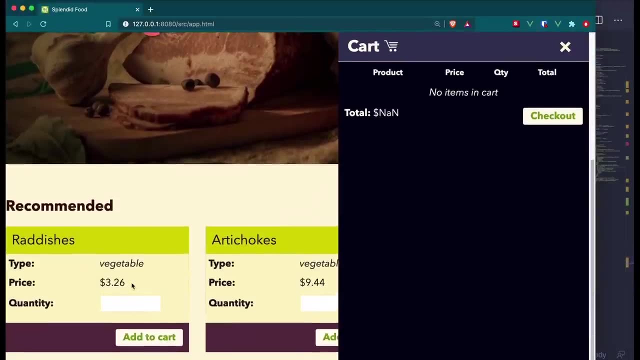 just quantity, which we are pulling off of the object in the cart. of course we already know that should work. let me add an item here, and quantity works. now price is a little bit trickier because we don't have the price stored on the cart. we actually have to search through. 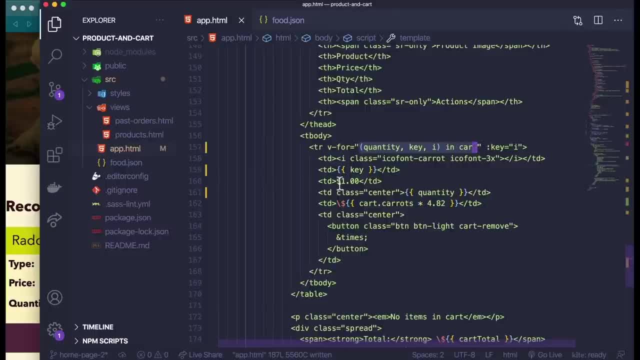 the inventory for the price. so we are going to make a helper method for that. first let me escape this- and then we are going to call get price pass in the name of the item, which is the key, and we will find the price and return it based off of the name. 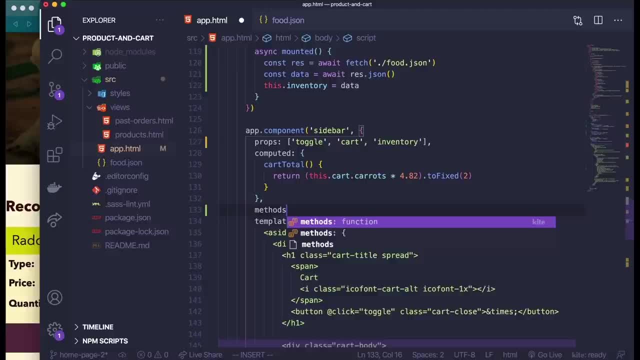 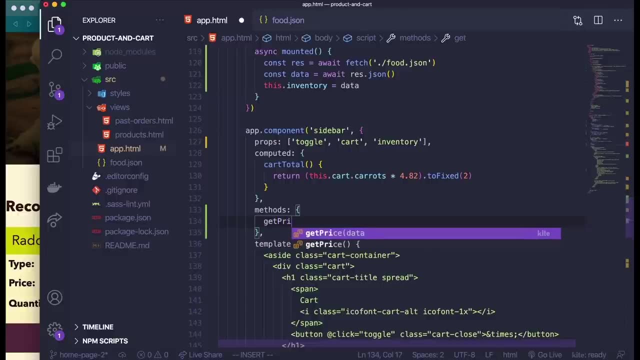 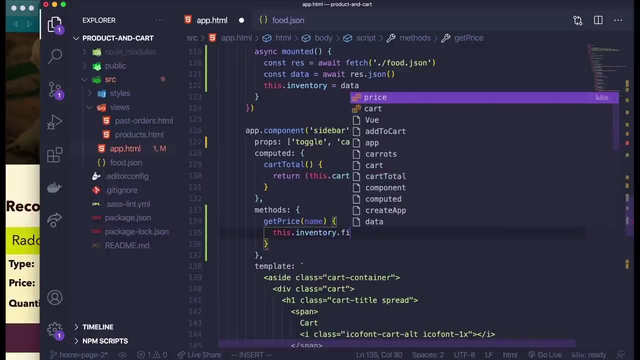 so after computed here I am going to add methods for this, just a regular methods object and add that get price and basically we can access this dot inventory and do a dot find. so we want to find one of the inventory items, so I will call each item product. 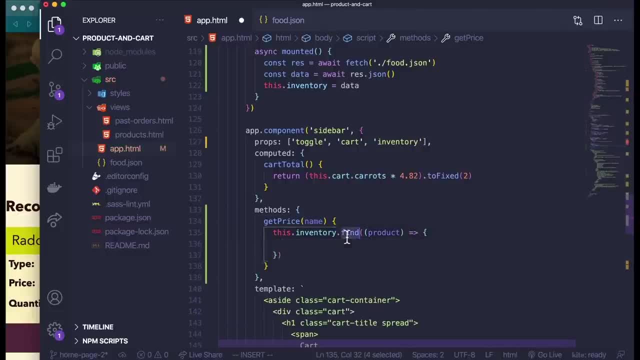 in the function that I pass in and dot find will loop through all products in the inventory and try to find whatever item I want. so I want the item where the product name is equal to the name that I am passing into the function, and when I find that product, 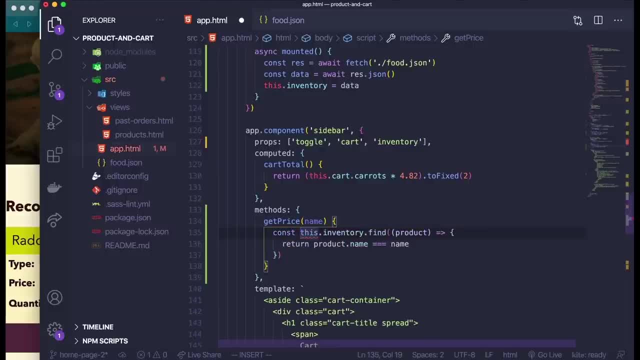 I am going to set it equal to a variable here. kind of confusing if I call it product again, so maybe I will just call this one p instead. there we go, and now for the return function. now that I have the product saved in this variable, I can do: 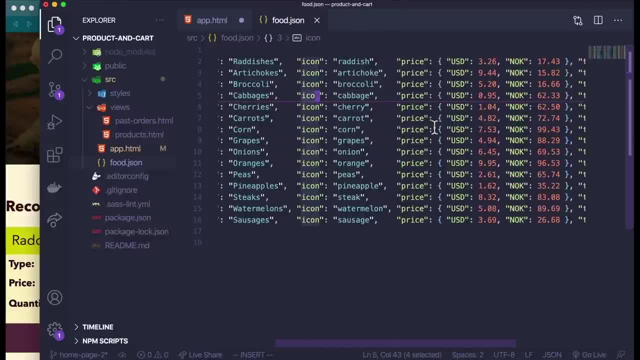 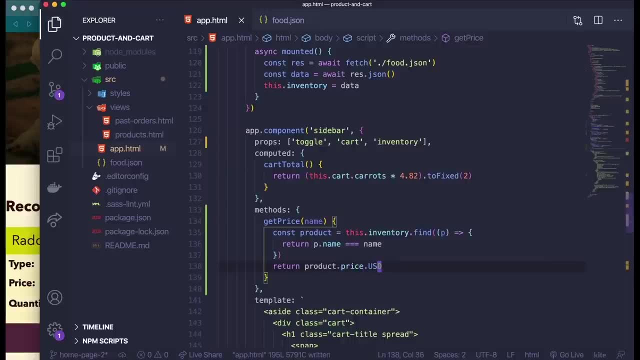 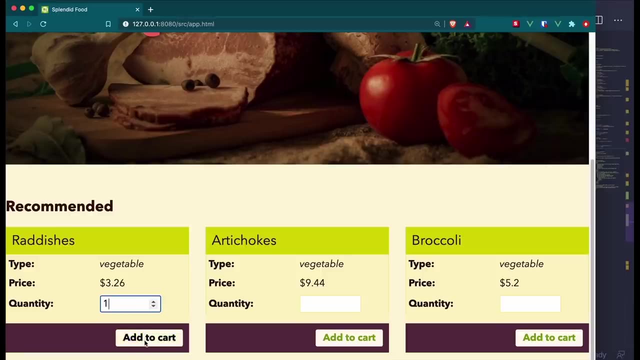 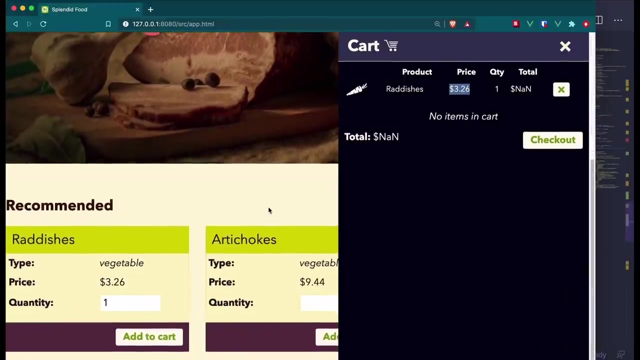 product and it should be dot price, dot usd again. so dot price, dot usd and that should return the price of the item and let's see if that works. so let me get one here and view the cart and I can indeed see the price. let me try that for. 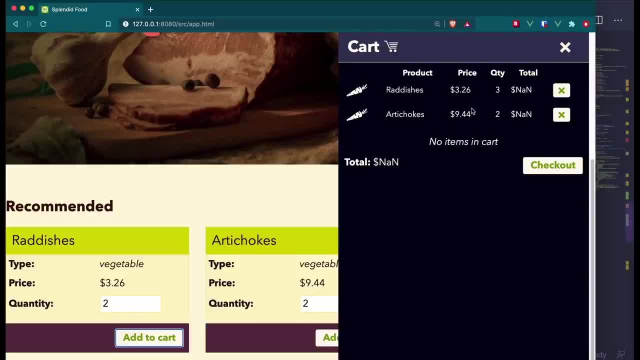 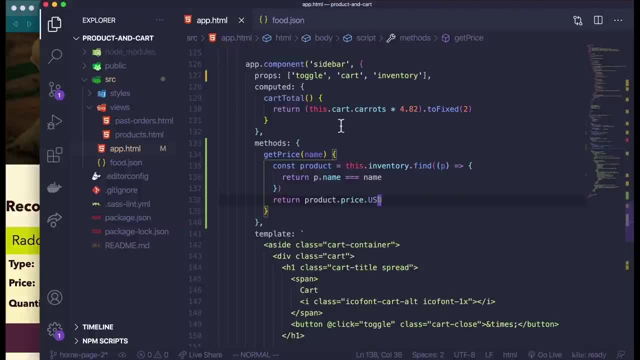 artichokes too, and see if I can get the price and quantities of the item correctly. now let me update the function for total, and so total here needs to be dynamic, based off of the whole cart really. so to do this I am actually going to use 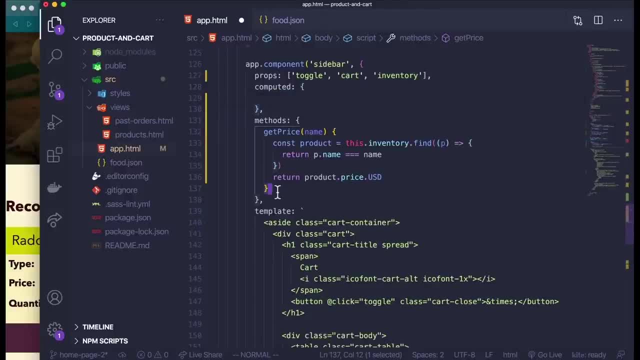 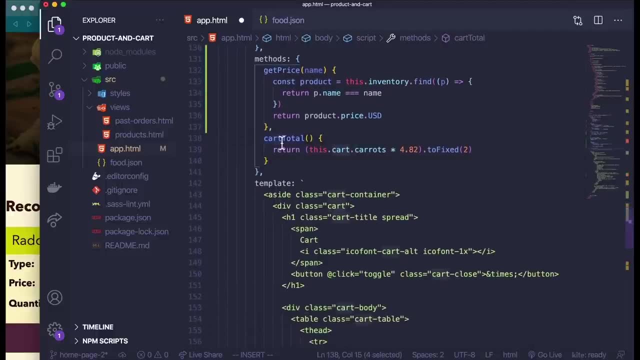 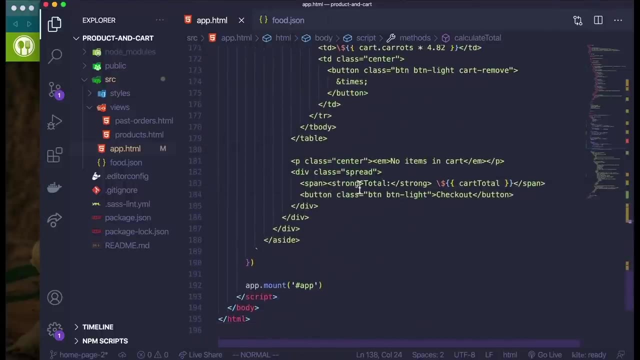 a helper method. so what I am going to do is take this out of computed and instead use it as a method. so, since it is not computed, it is a method. I am going to call it verb, so calculate total, and I am going to go ahead and 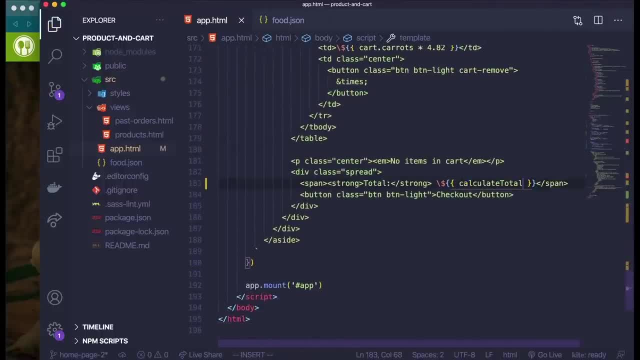 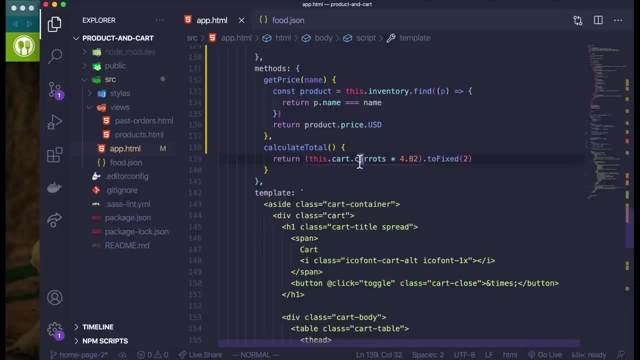 rename the method call down here. of course, I will actually be calling that as a function now and I won't be needing this line of code anymore. so now we basically need to calculate the total based off of the quantity in the cart, and then we have to look up the 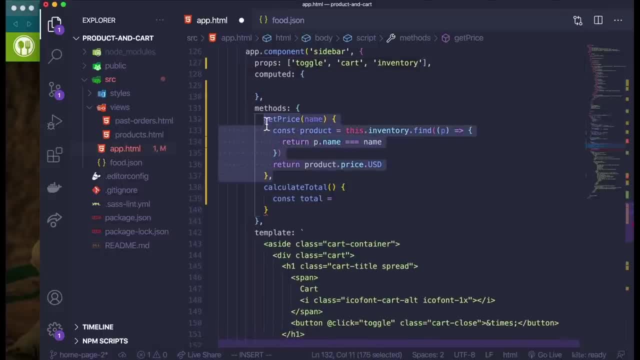 price in the inventory. fortunately, we already have a method to be able to look up the price, so we are going to just use that, and the easiest way to do this is actually to do objectvalues, and so objectvalues can give me an easy array of values out of an object. 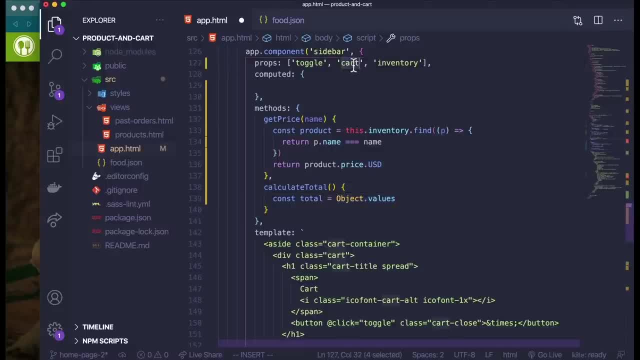 and because cart is an object, I am not going to loop through it directly. I am just going to grab all of the values out, so I will pass in cart, and now I have an array of all of the values here, which are the quantities that I want. 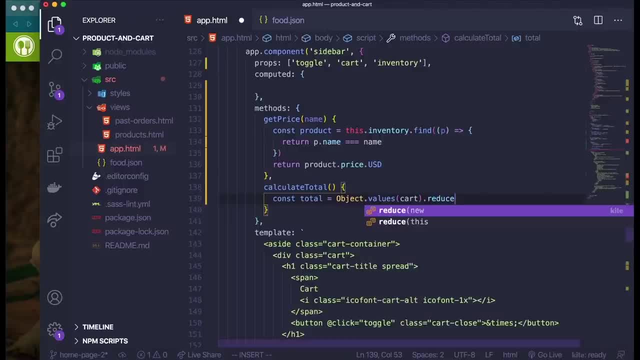 so out of that array I am going to reduce it. now the reduce function is just a built in javascript function where I save an accumulator. some people like to call it a sum. I will call it an accumulator because that is what it uses on MDN and basically I am. 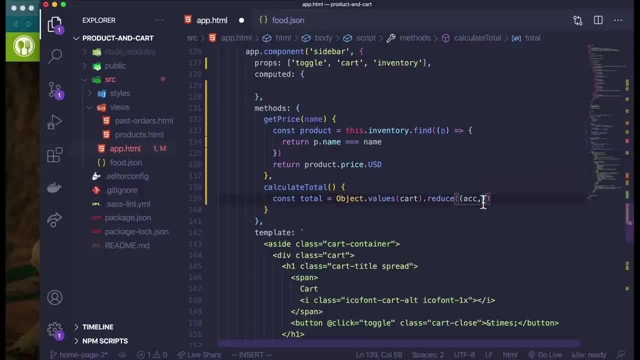 calculating a sum on each iteration through the loop. I also have my current item that is being looped through, and then I can also get the index of that item in the function and basically what I want to do is return the accumulator sum total, whatever you want to call it. 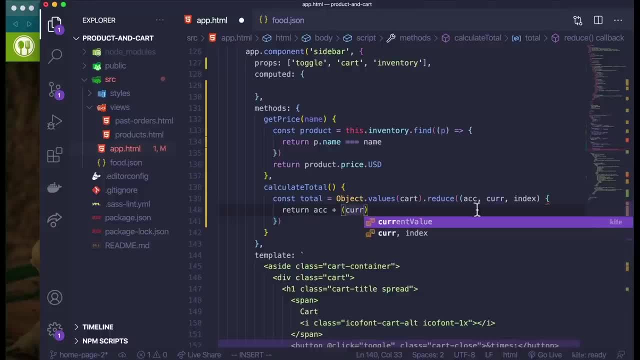 plus the current item or the current value, because I am looping through all of the values on the cart here and I need the value times the price. so I am going to have to call this dot get price and then I need to pass in the name of the item that I want to get the price for. 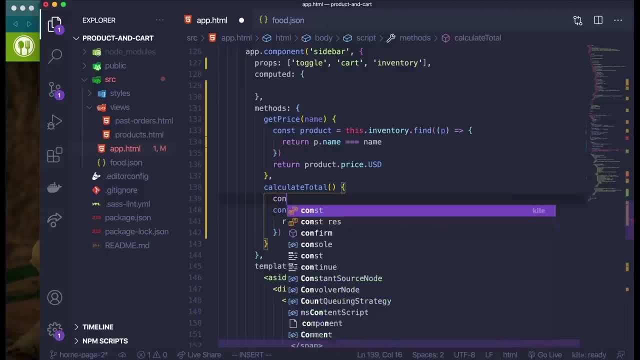 so the easiest way to do that is to also make an array of names. so I am going to do that by using this time. object: dot keys and I will do this. dot cart- get all of the keys this time off of cart. and actually I forgot to put this. 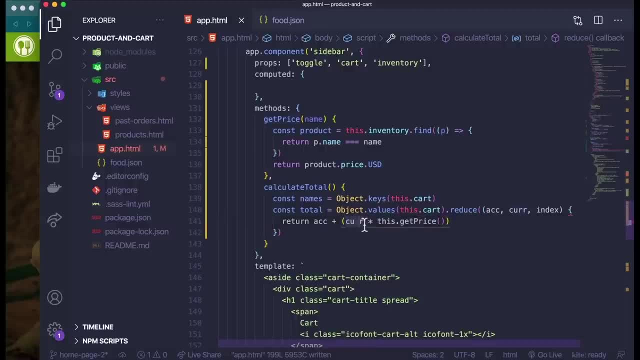 here and so I will do the current value times this dot get price. and now that I have the names here, I am just going to look up by the index so I can pass in names index to the this dot get price function. and that should work for the function I forgot to. 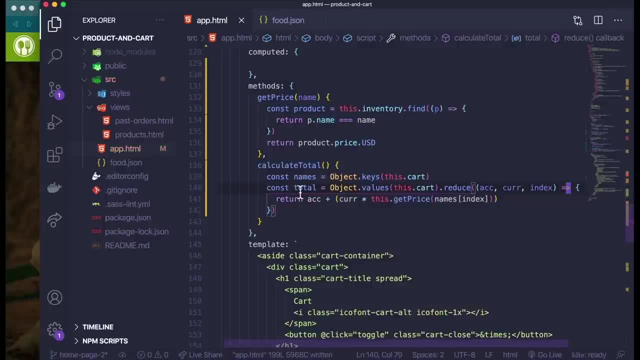 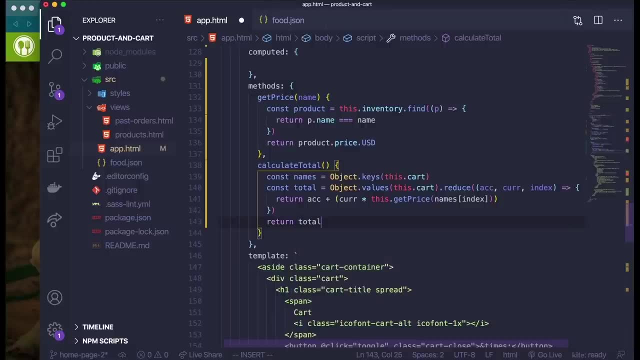 put in arrow here and now for the total variable. I just stored it in a variable to explicitly name it. all I need to do now is return the total. now this function works. there might be a more optimized way to do this. this is just to demonstrate how to calculate a total using 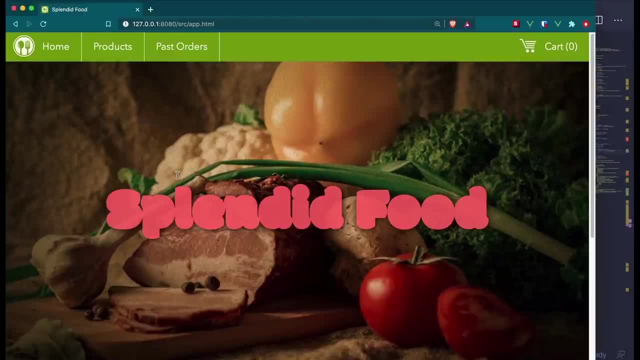 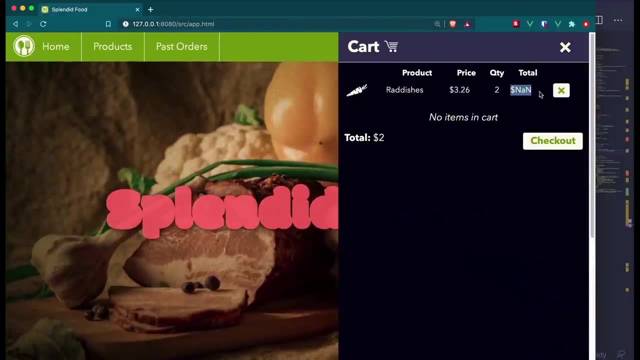 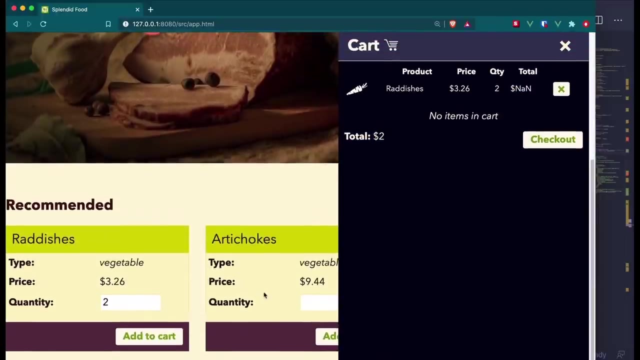 a vjs method for this application and it is basically just using regular javascript. so let me add the names to the cart here and, of course, this total. we haven't done yet, but we do have two radishes and the total says two dollars, so let's add some artichokes. 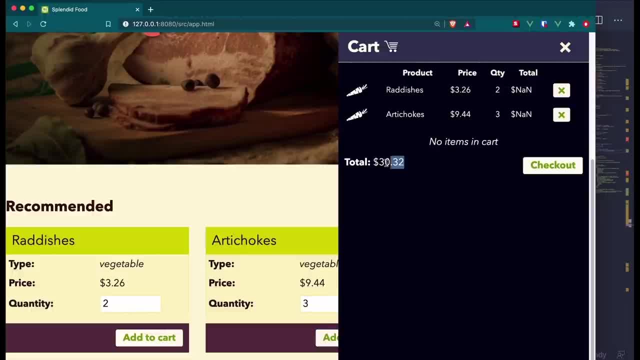 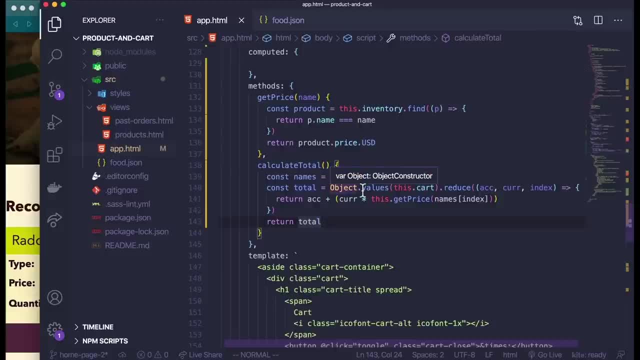 and now we have a total of thirty dollars and thirty two cents. as you can see, those aren't the correct values. what I believe is happening is, because objects are unordered and arrays are ordered, that the names and the object dot values. they aren't being listed in. 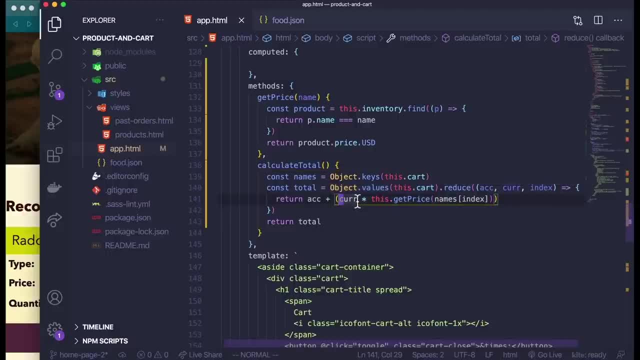 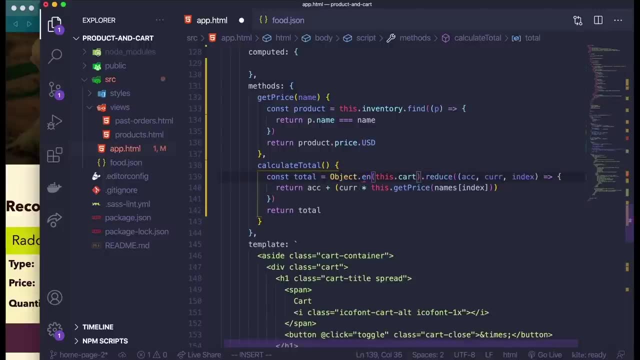 the array in the same order. so I'm going to have to, instead of making two separate arrays, here I'm going to get rid of this one and here I will just have to change this to entries, and now my current value here will basically be in array. that will. 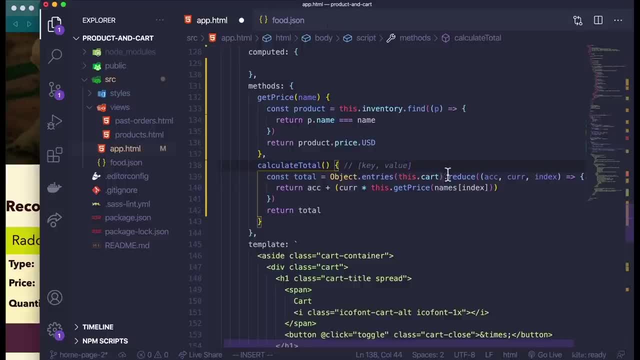 be the key and the value each time looping through this larger array. so for the value, now I will have to access it at the first index and instead of names here I can access the name at the current item at the zeroth index. that all looks good. the last thing. 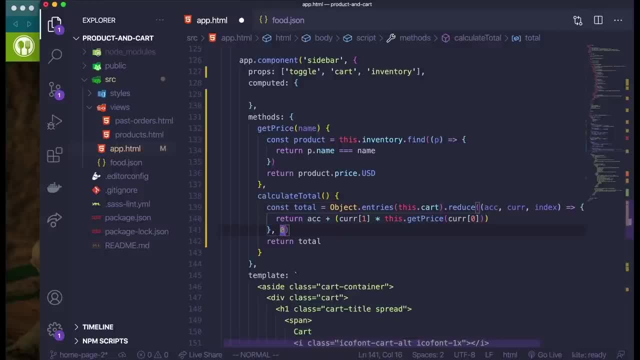 I'm going to do is add an initial value here, and this means that the accumulator will start at zero, and also, if there are no items in this array- which there aren't any- to start that means the number will just be zero, total. and for here, for the total actually I'm going to use 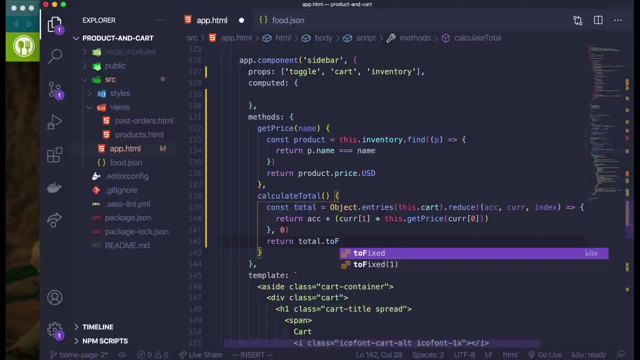 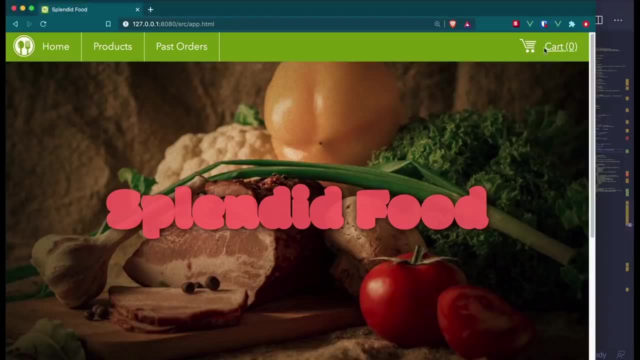 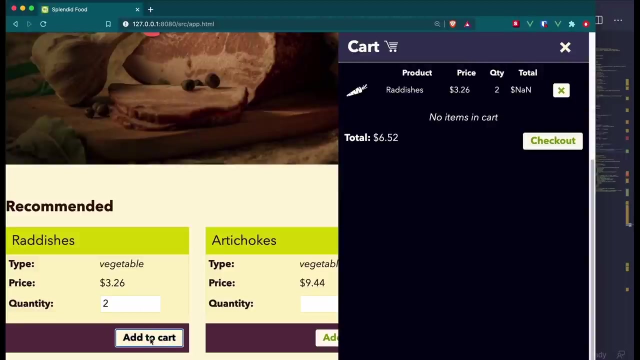 that method again that we used before, which was two fixed, so I could do it to two decimals, which is what I want in my cart. let me see if this works, and this is exactly what I want here, so let me add items. yes, and the price is: 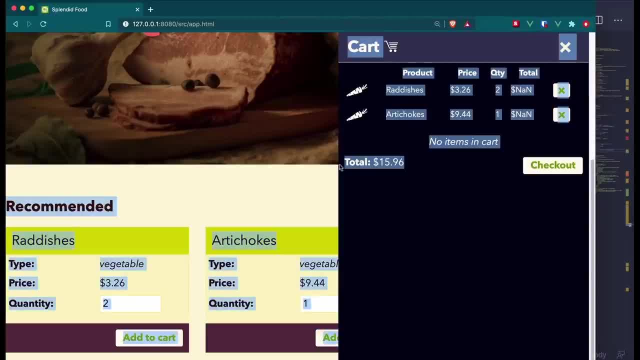 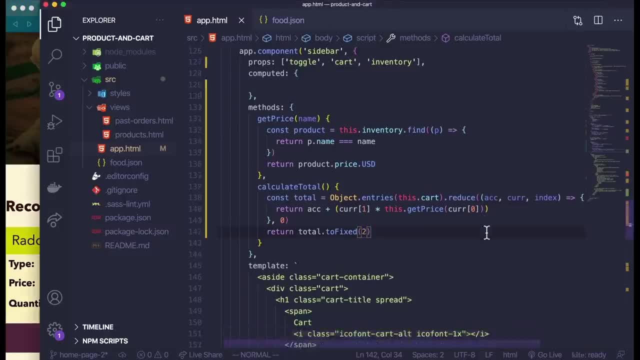 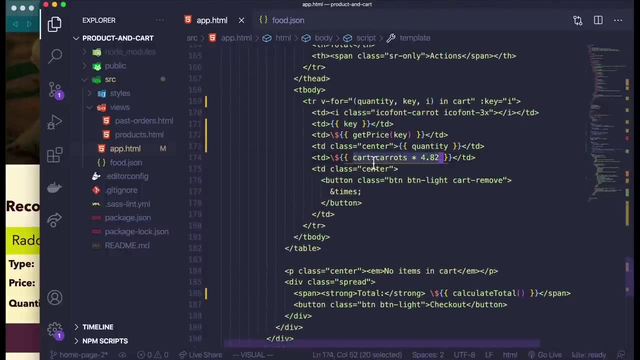 exactly right. one artichoke and the price still works there. now what about the total here? that should be easy enough to do with our get price method, so let's go down to the total. right now it's hard coded as carrots, which doesn't exist. so now I 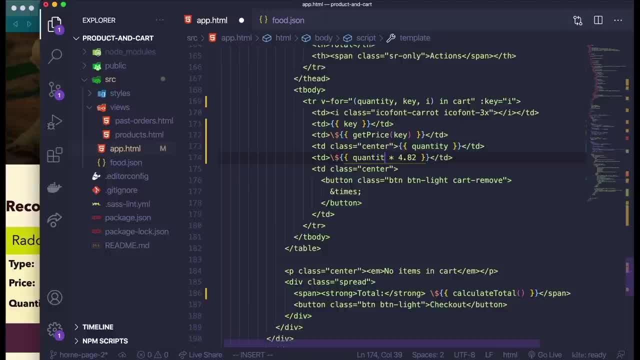 can do just the quantity, which is the quantity of the item in the cart, and then I'll call the get price method and I'm going to pass in the key, which is the name of the item, and so that should multiply by the total. let's see if that works. 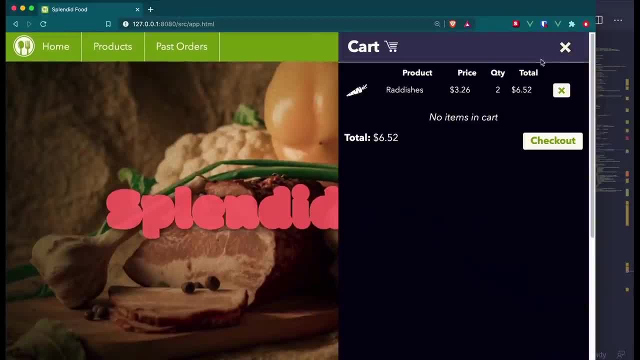 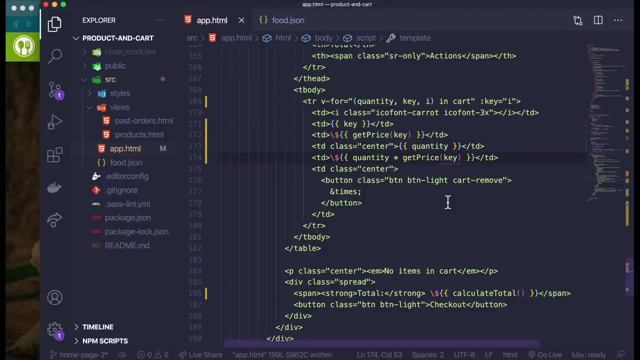 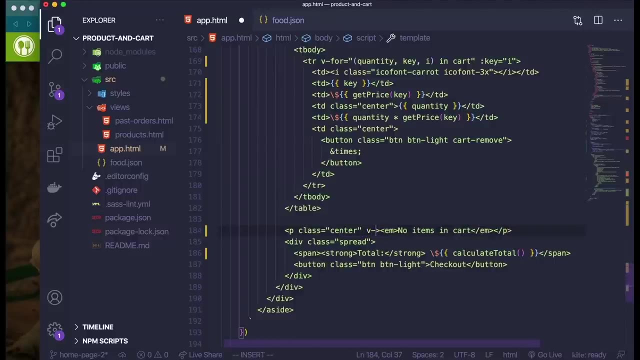 add an item and check out the cart, and we do indeed see the total here. now it still says no items in cart. let's go ahead and fix that. so this should only show if in fact there are no items, and so I'm going to add a vif. 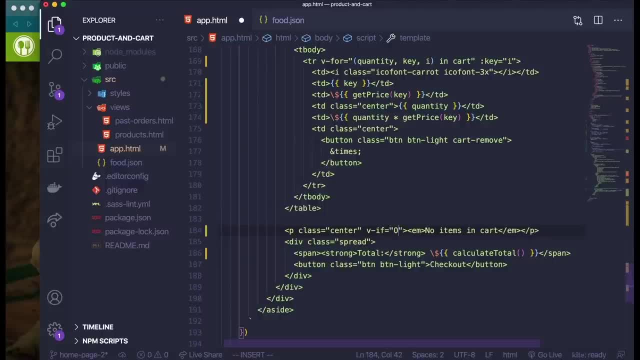 here and just to speed this up, we're going to do object dot keys and then check the cart object. so if there are no keys on the cart object, that will be zero, which is a false value, and let's see if that works. let's go down here. 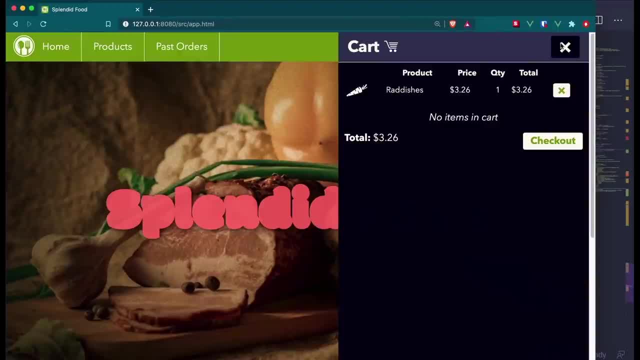 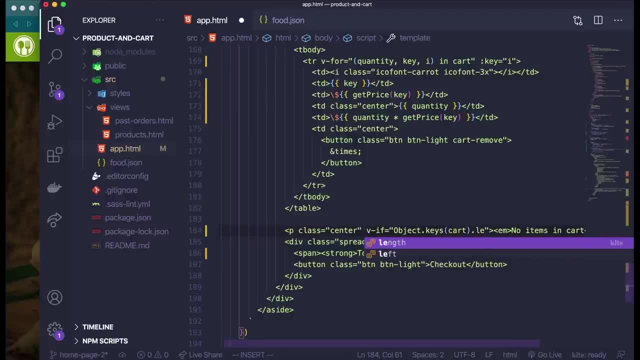 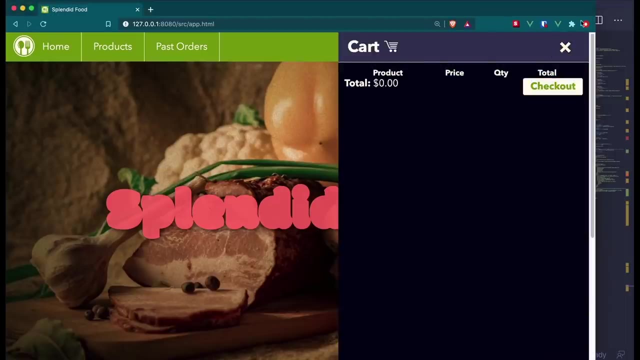 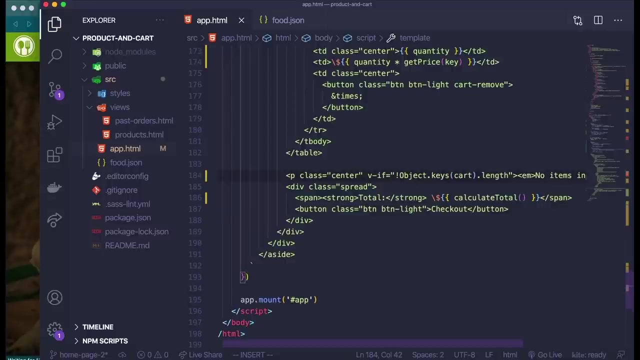 to radishes, add one in the cart. we are still seeing this: no items in cart. so I believe I have to do length here and let's see if that works. okay, that does work, but I have it backwards. so I basically need to do, if not, because 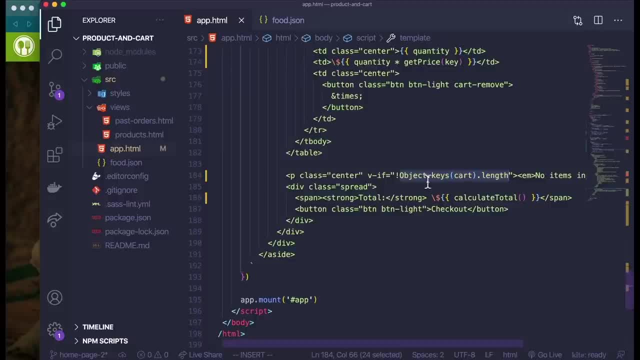 if the length is zero, I want to show this, and if it's not zero, then I don't want to show this. no items in cart? because there will be items in the cart, so let's see if that works. let's first go here. it does show no items in cart. 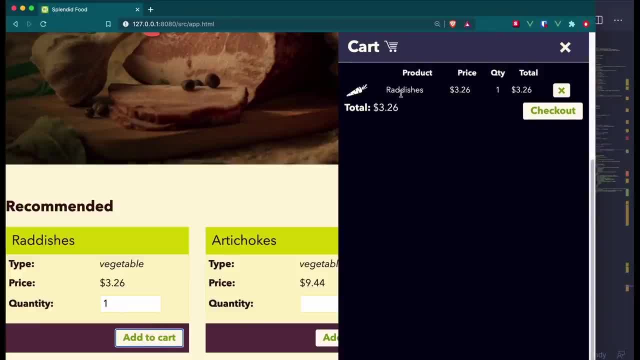 and now let me go here and now it changes to the item in the cart and all of the totals are shown correctly and the quantities updated, and all of that stuff. the only other thing I want to do is provide full crowd operations, and this delete does not work. so 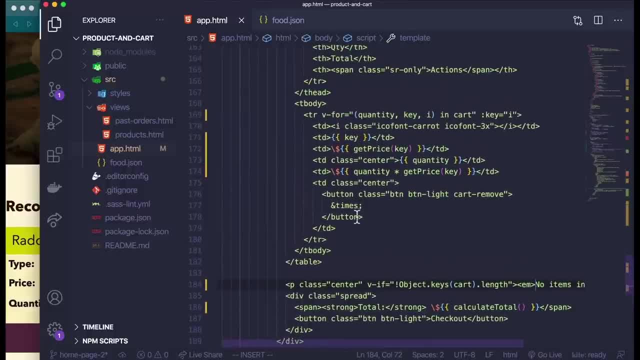 I'm going to hook up the delete now so you can see the delete is here on this button for remove, and so I'm going to add a function here, and actually this function will have to be not inside of this component but inside of the parent component, which is my. 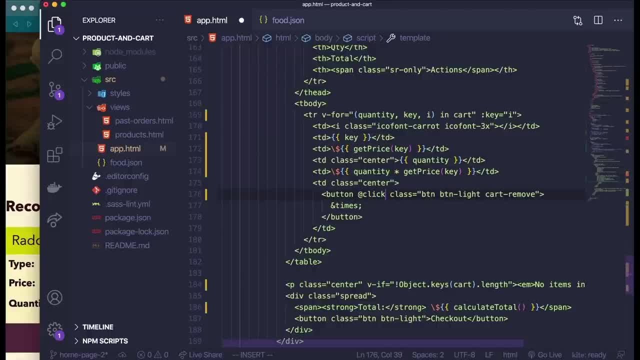 main view application in this case. so I'm going to do a click. so when this button is clicked, I'm going to say remove item, to remove the item from the cart. and then I need to pass in the name of the item, which is the key now, this: remove item. 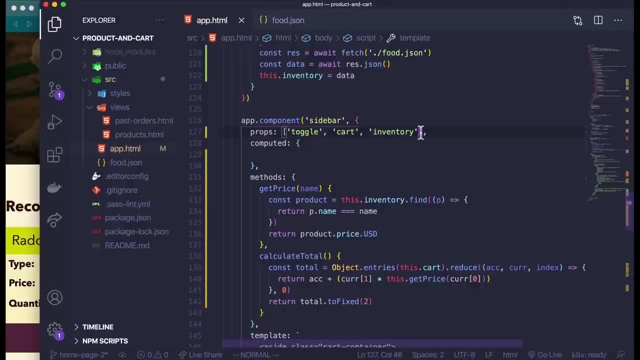 is going to have to be a function passed in as a prop here, because I can't mutate props, so I couldn't change the inventory or the cart actually directly from this component. I have to change it from the parent component where it originates. so I'll take a. 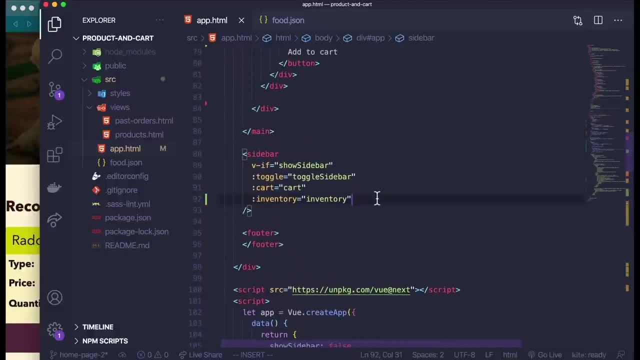 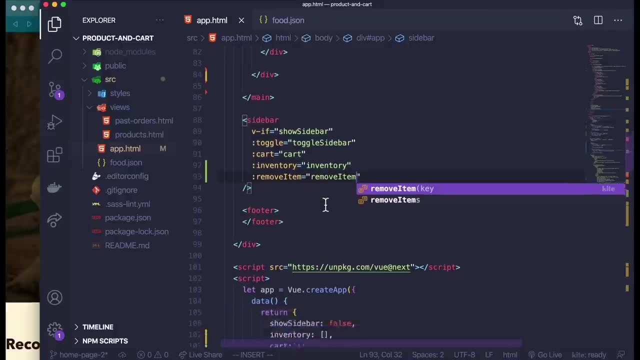 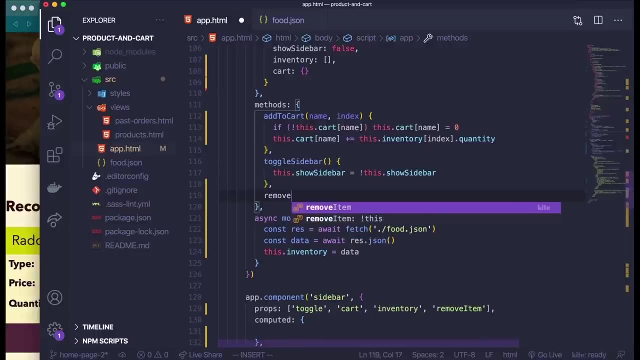 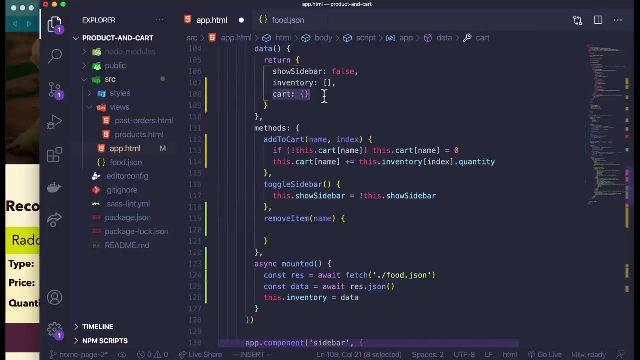 remove item function. let me go ahead and pass that in. remove item equals remove item, and now I have to create that function here as one of these methods, so let me add that remove item. this will take in the item name and I am going to remove it from the cart, basically. 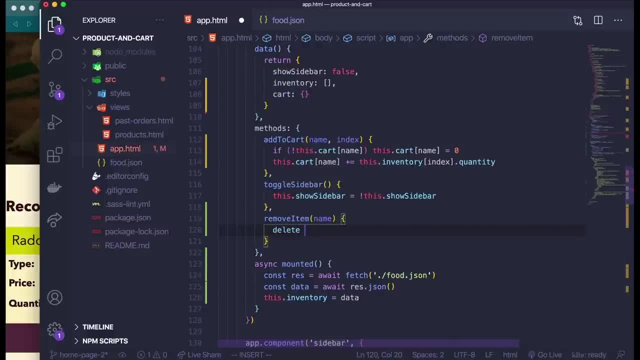 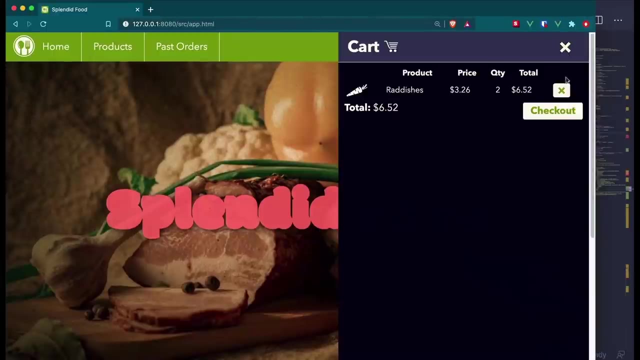 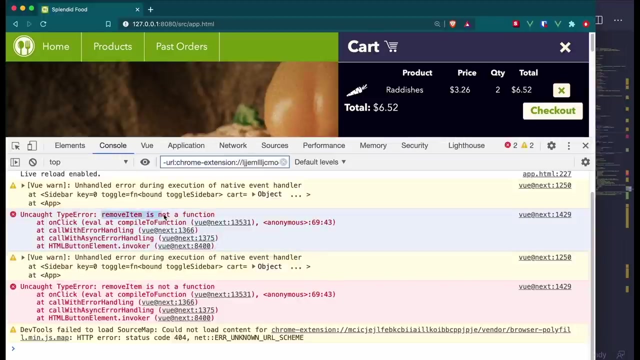 so I can just remove javascript. delete this dot cart name. let's see if that works. let me add some vegetables to my cart and now I will remove them. and it does not remove. let's see if I'm getting an error. remove item is not a function. 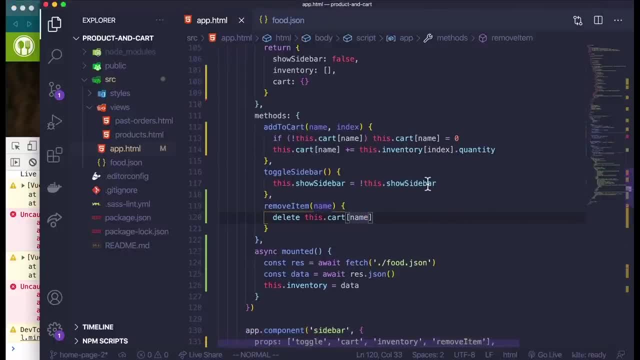 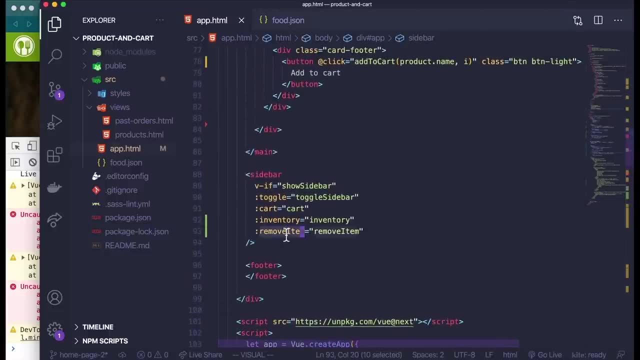 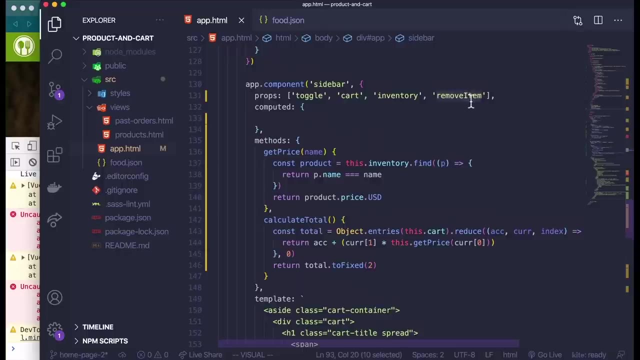 so let's see why it's not considered a function. I do have it in methods here: remove item. let's go here. this is remove item that I am passing into my sidebar. I am also accepting it as a prop in the sidebar here. let me get rid of computed. 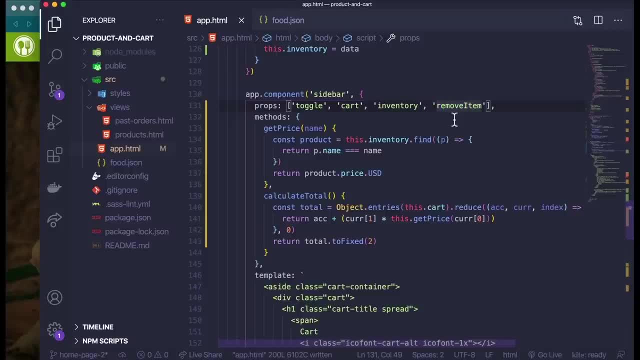 so it's not recognizing this as a function, so what I'm going to do is rename it in the child component. now, this is a work around only for the CDN. you won't have this problem if you were using VueJS from NPM, but I'm just renaming the function. 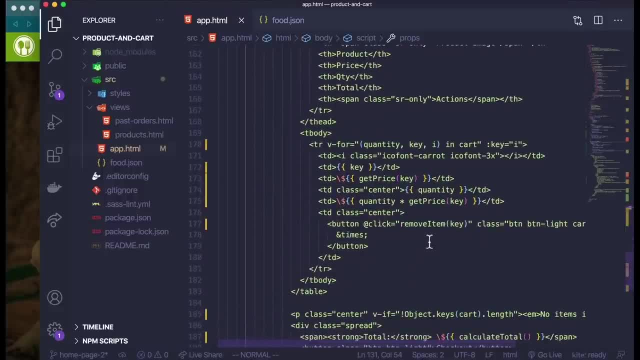 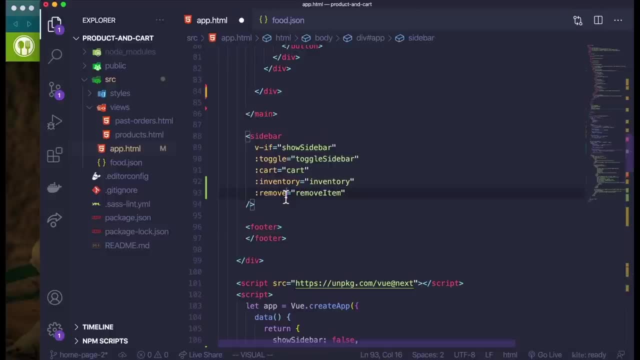 in appcomponent here. there we go, and of course I need to pass it in as the name remove. so I basically gave it a different name for the child component and for the parent component and let's see if it recognizes this as a function. now I will come here. 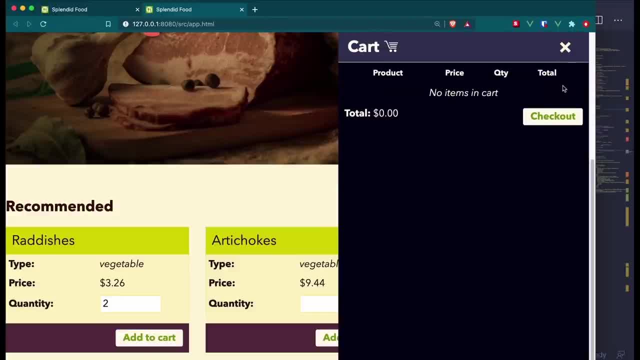 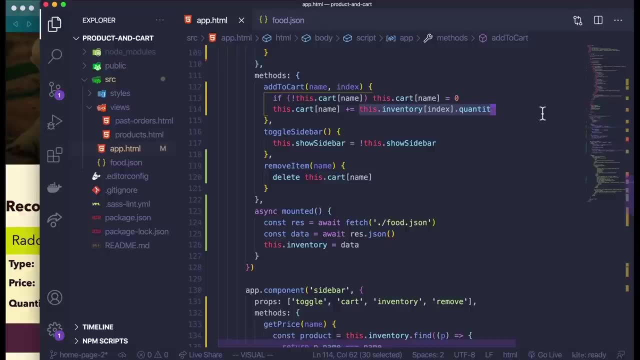 and I can remove it from the cart- awesome. of course, when I add things to the cart, I do want the number to clear here, so let me take care of that really quickly in add to cart here, just really quickly. I'm going to set this to zero. 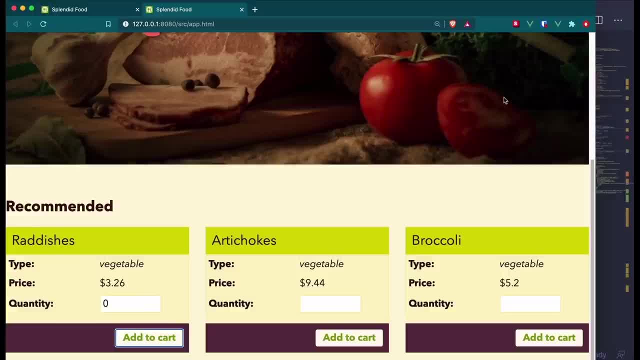 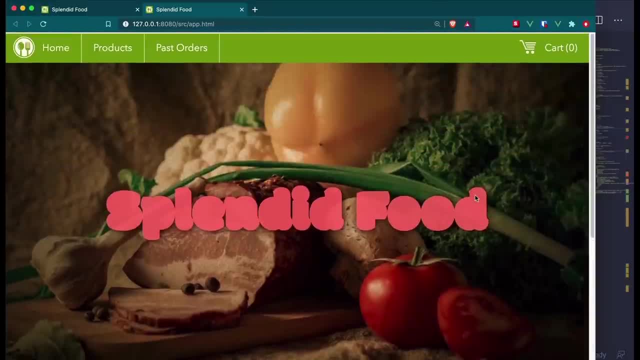 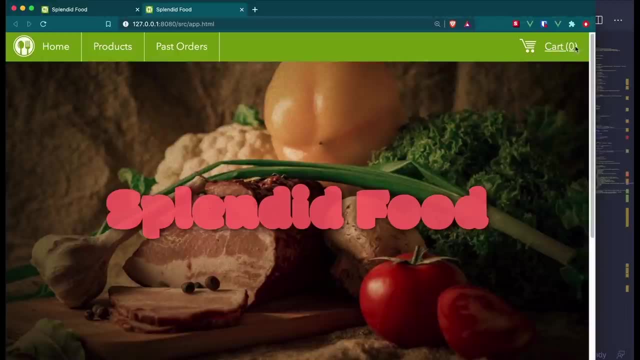 let's see if that works. and back to zero and it is in the cart now- awesome. the only other thing is that the cart does show zero items even when there are items in it. that's because the number is not dynamic, so let me change that really quickly. 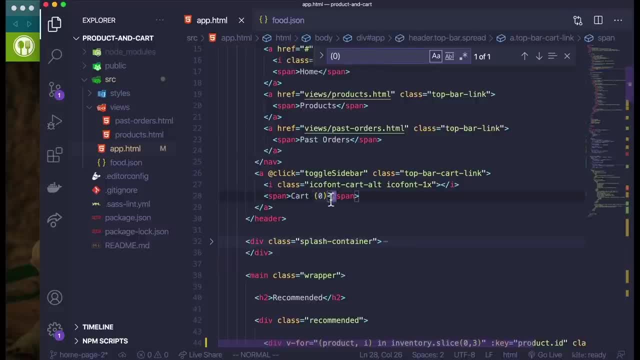 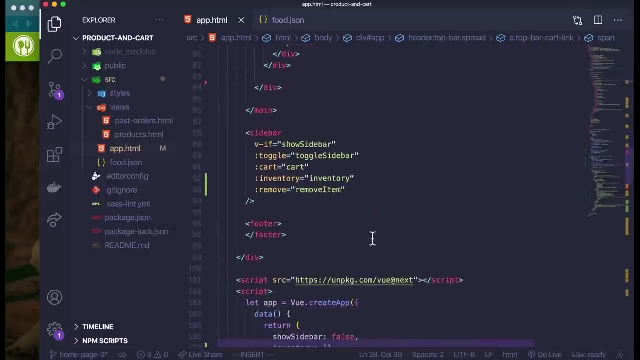 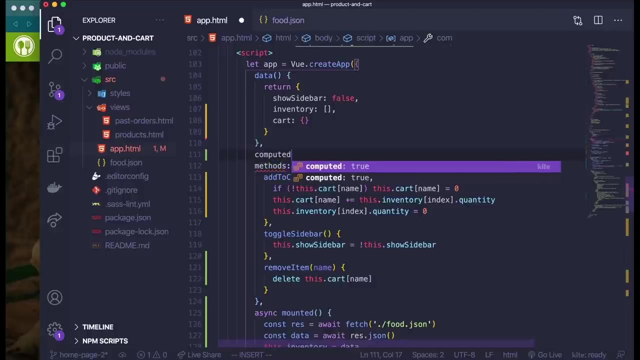 here inside of the parentheses. I'm going to change this to be dynamic and I'm just going to call the variable total quantity. okay, and now I need to make this variable. so what I'm going to do is create a computed object here and I'm going to say: 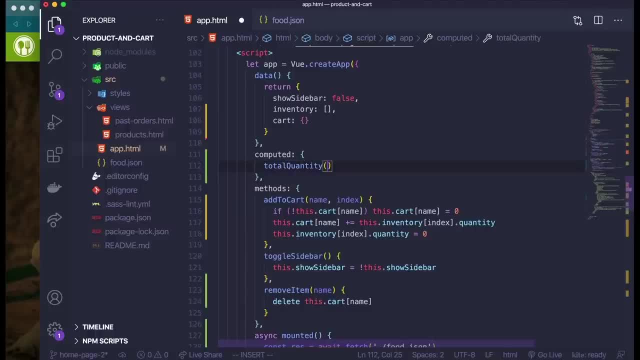 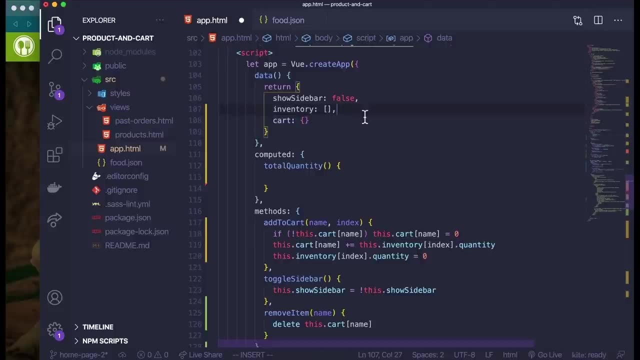 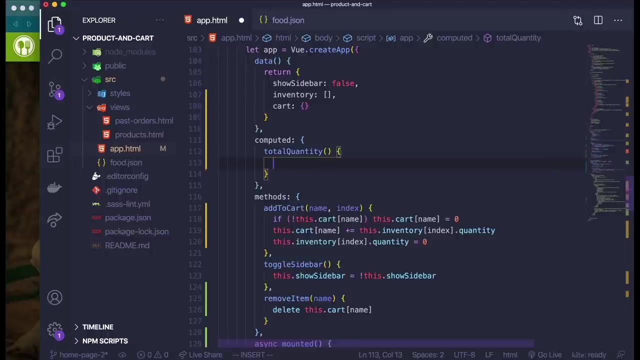 total quantity is basically the sum of all of the quantities in the cart. and to do this I'm going to use another reduce method. I'm going to say projectvalues, pass in thiscart and then I will reduce those to sum up all of the numbers. so I have my accumulator and my 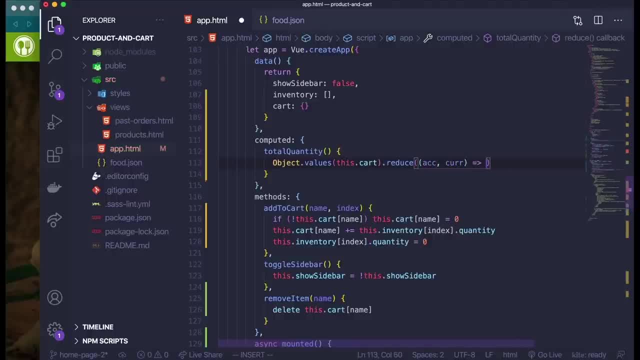 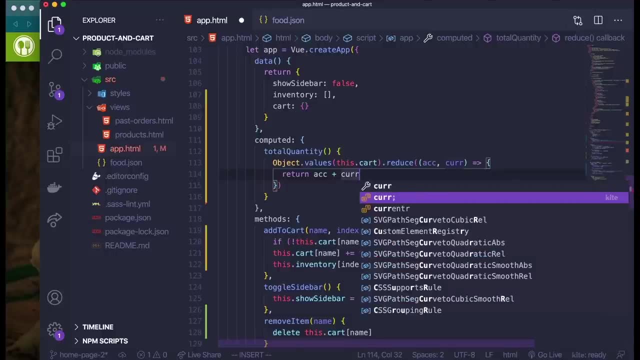 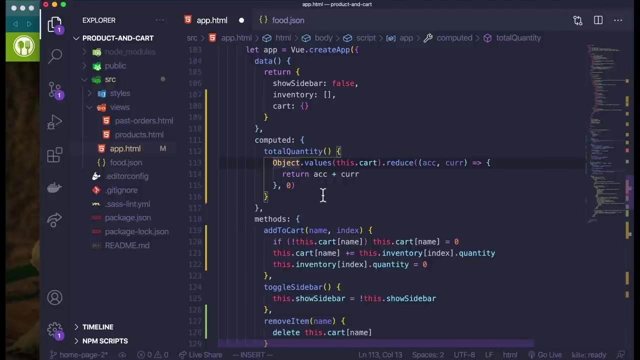 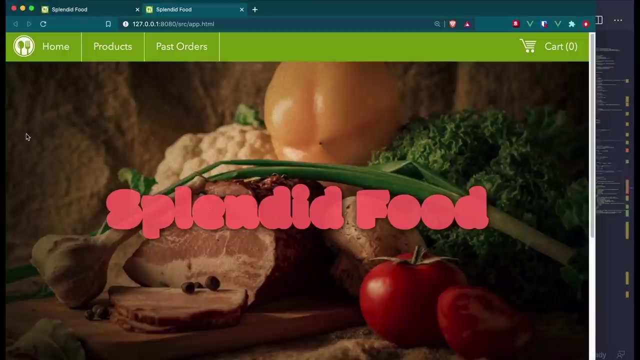 current value, and then all I need to do is add the accumulator and current value together. of course, I'll set a default of zero here- starting point or initial value- and I'm just going to return this directly this time. let me see if that worked. right now it says zero. 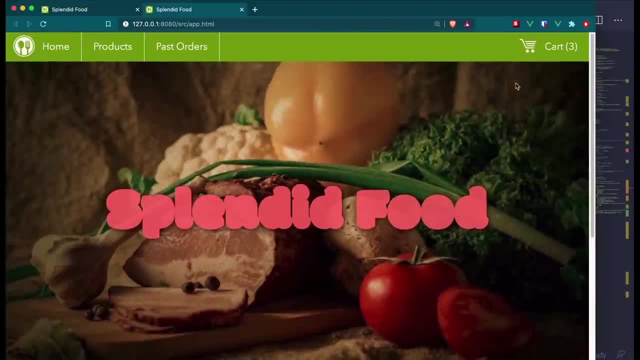 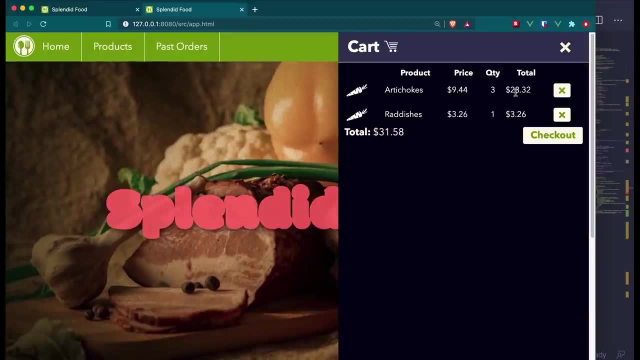 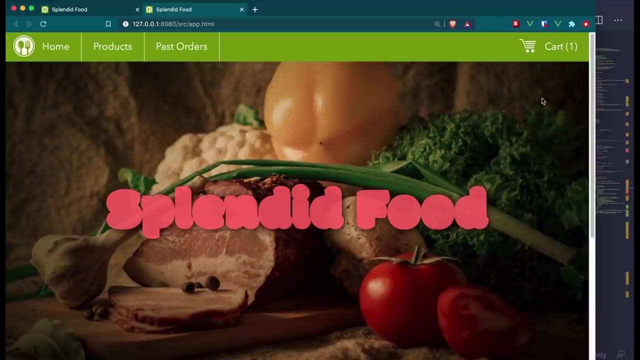 but let me add items. now it's three, let me add one more, and now it's four. so the quantity is working. if I remove one now, it's just one. so that is a dynamic value now, and that is basically it for the home page here. in the next video, 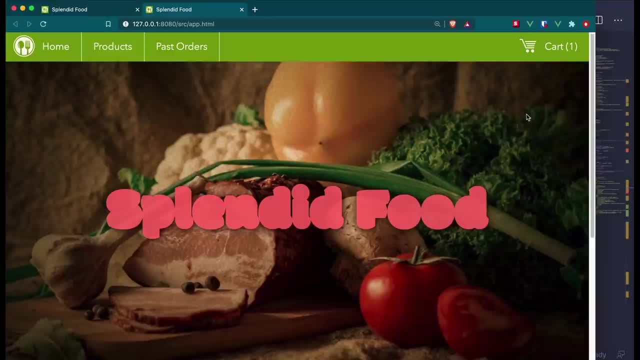 we are going to move the Vuejs code outside of the apphtml file so we can see how it can work in multiple different pages and also some of the struggles that we might run into trying to build a multi-page site via the Vuecdn and trying to do things. 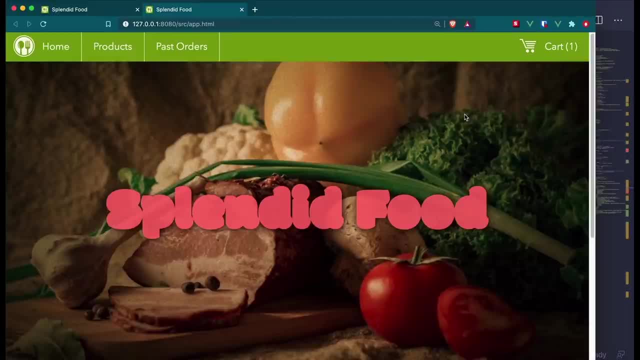 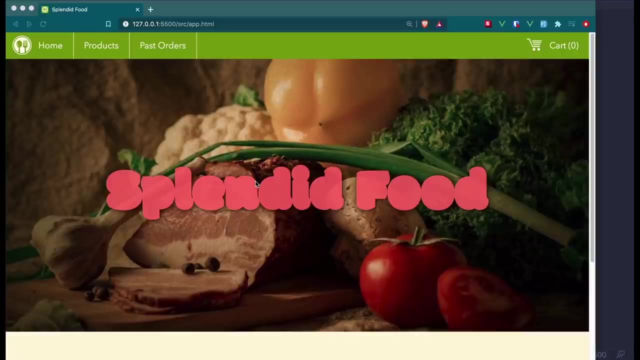 like share data across pages and stuff like that. if you want to see the starter code for this video, make sure you check out the branch in the repo called home page number two or home page two. hi, everyone, welcome back. first I want to review what we did. 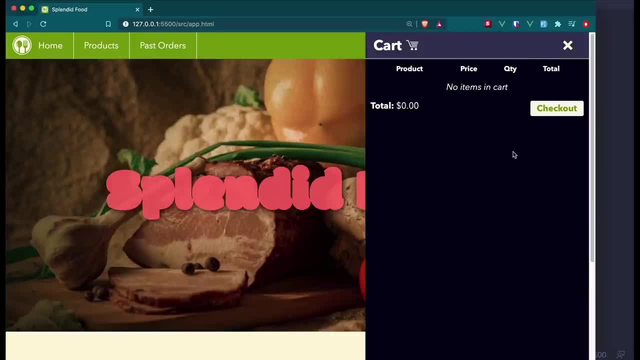 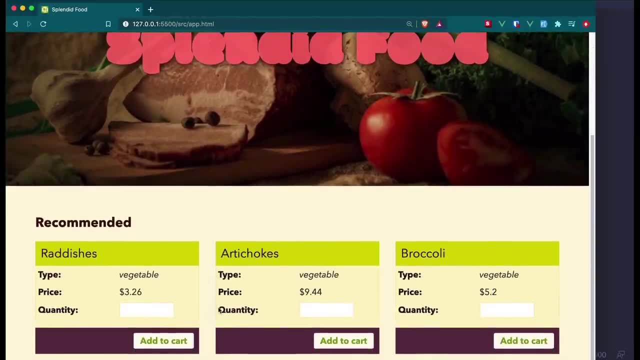 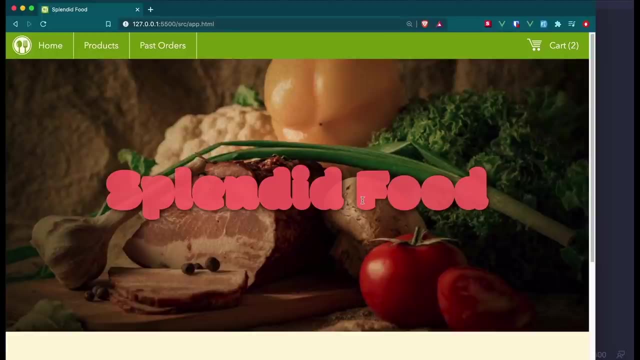 in the last video we connected the cart slide out draw menu on the right here and made that fully functional, and then we added an actual loop as well as functionality, to be able to add items to our cart here. now this is only one page, of course, so we also have 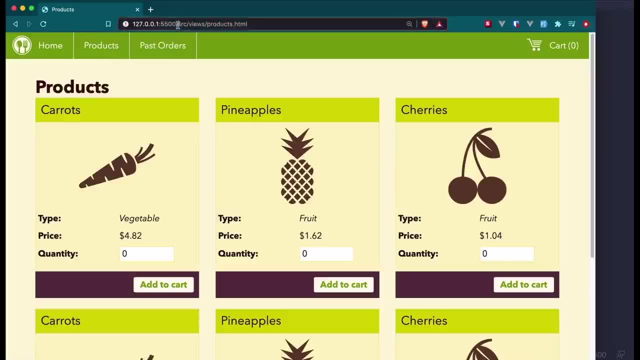 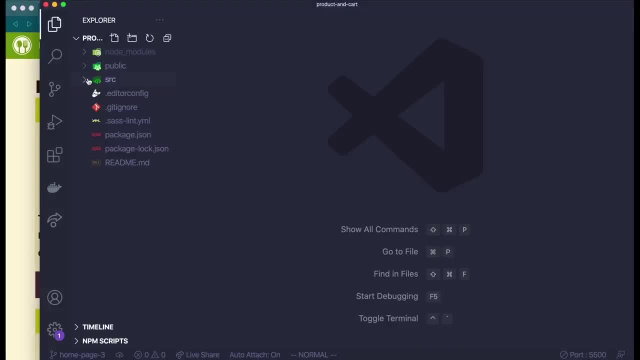 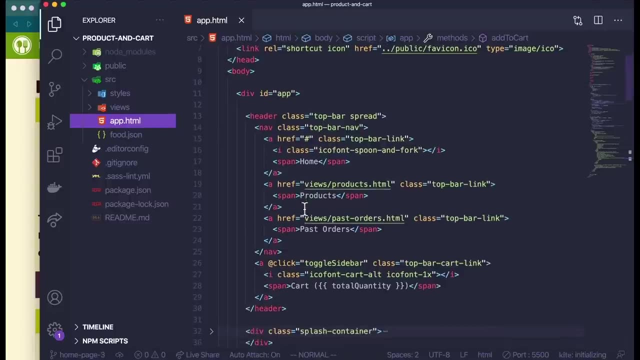 the products page here. so if I go to products page you can see the url changes to go to the productshtml page now if I look at this in my code. so let me open up the source and this apphtml file again you can see here is the. 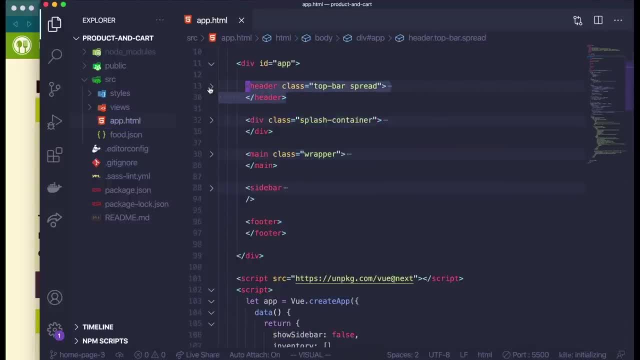 header with all of the links on it. I'm going to fold that real quick and then you can see the different sections of the page, including that side bar that slides out that we actually want on every page, but now it's kind of just hard coded into this. 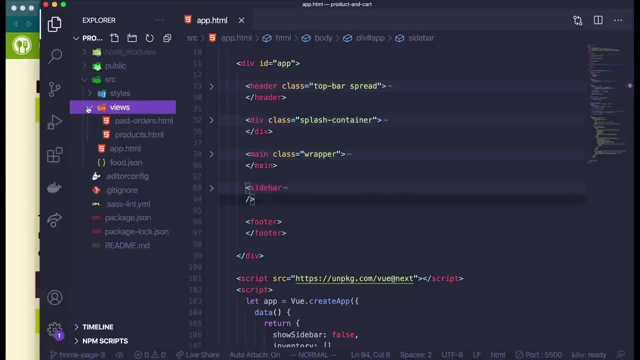 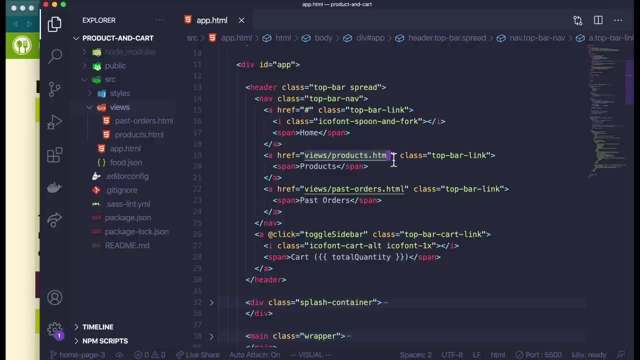 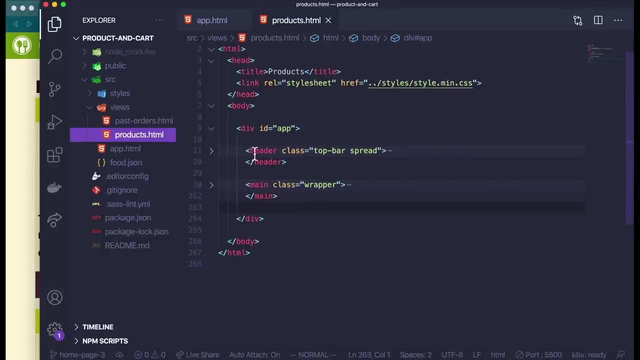 home page. I can also go to views here. so you can see in the header actually. so when I click on products it goes to views- slash productshtml. so it's actually navigating me to this productshtml page and if you look at the header here, here's the whole page. 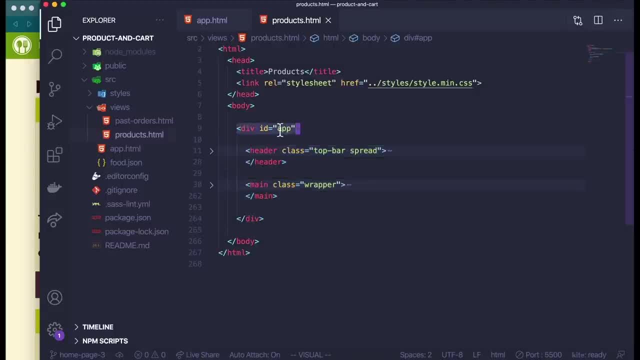 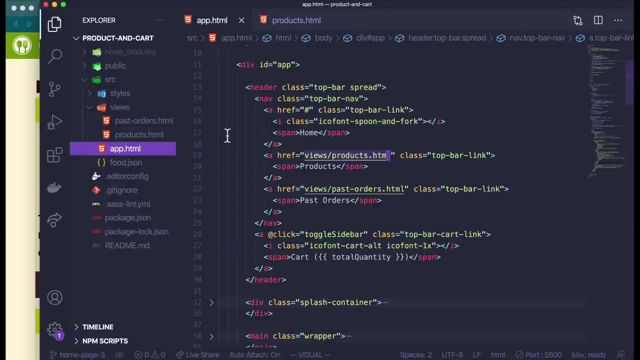 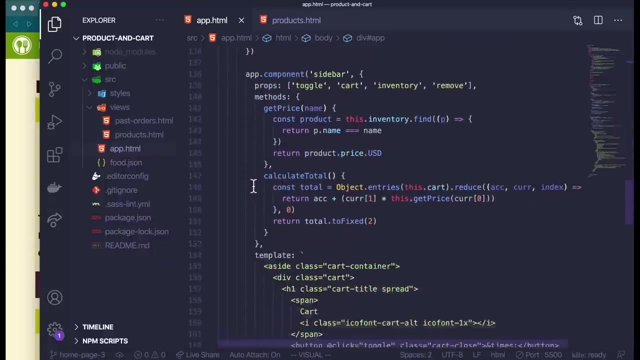 including a completely separate div with id of app where we would have to inject our vuejs code. you can see we already did that on this page, because our vuejs is in this script down here and we are rendering it or mounting it inside of that div. 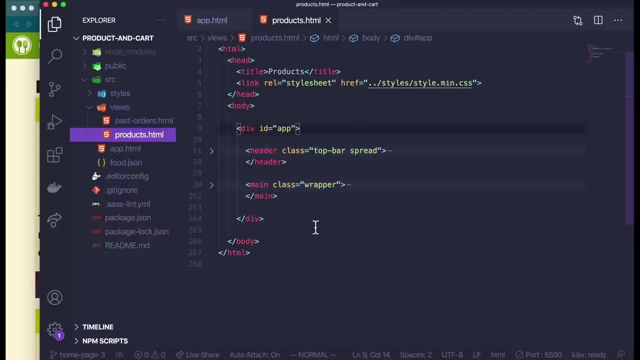 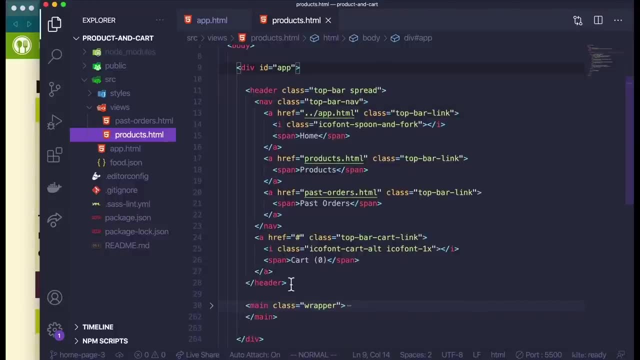 but if I go to products, we have no javascript, no interaction. everything is hard coded. we also have a duplicate header, so this is exactly the same thing as the header on this page. it's just copy pasted into the html on this page. of course we don't want to. 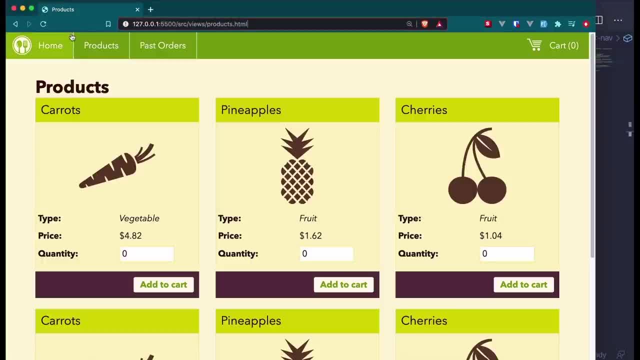 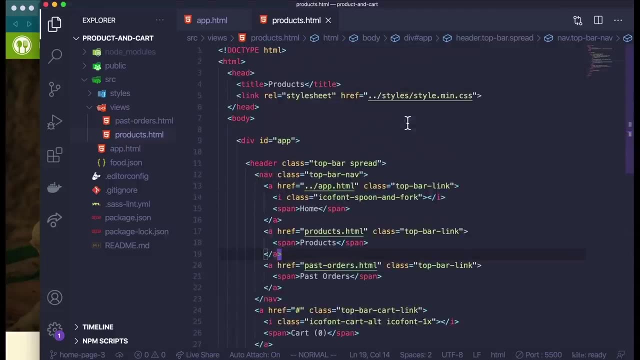 do that everywhere. we don't want to have a copy pasted header for all of our different pages. not only that, we would have to copy paste the whole cart side bar as well. so to make this code reusable here, we need to extract these things into other. 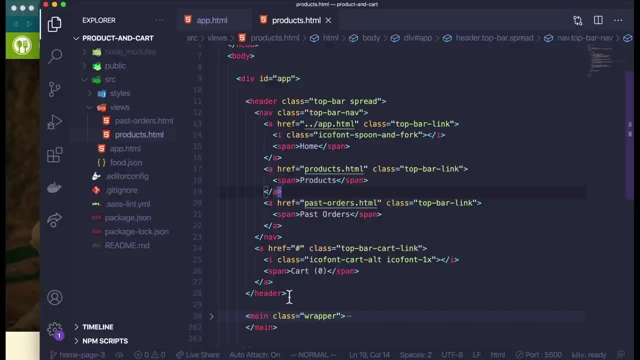 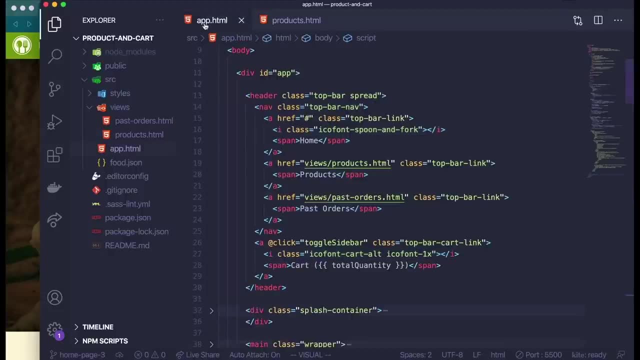 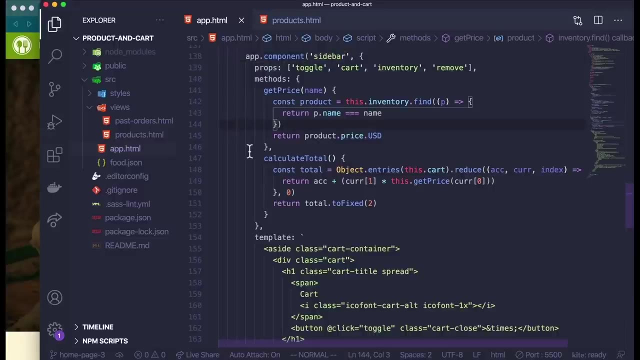 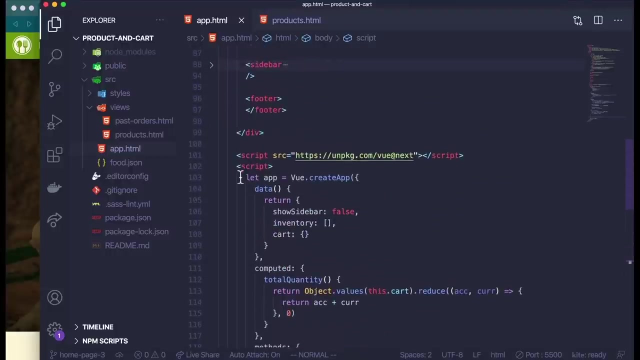 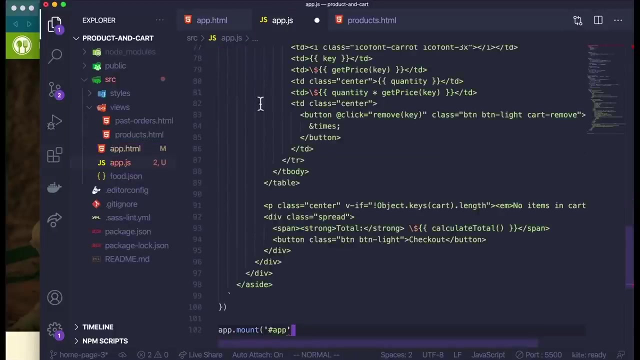 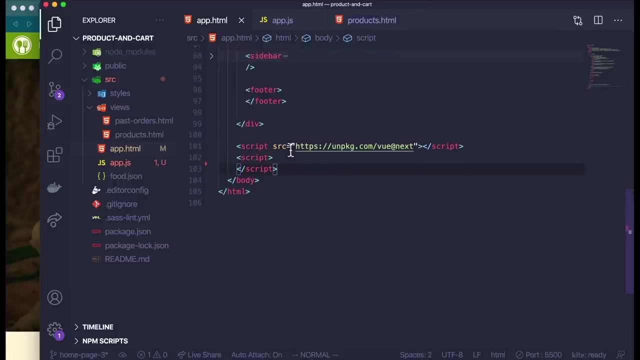 files. now, this is not easy to do for plain html, but we can use a vue component, like we did before with the side bar. so I'm actually going to extract all of this out into a separate javascript file and paste it into my html and now import this file. 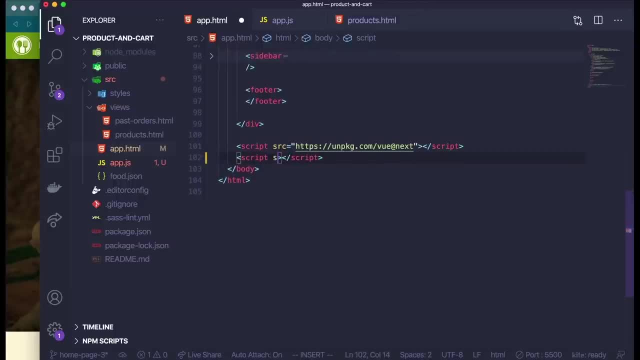 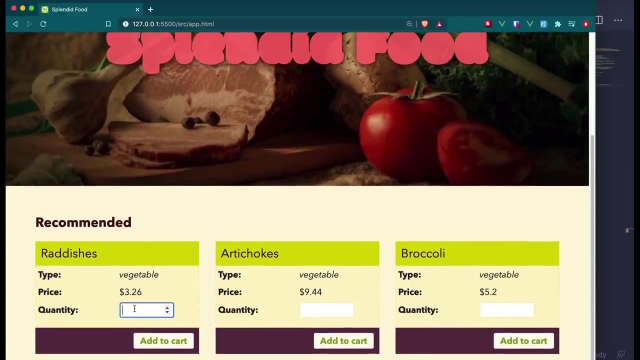 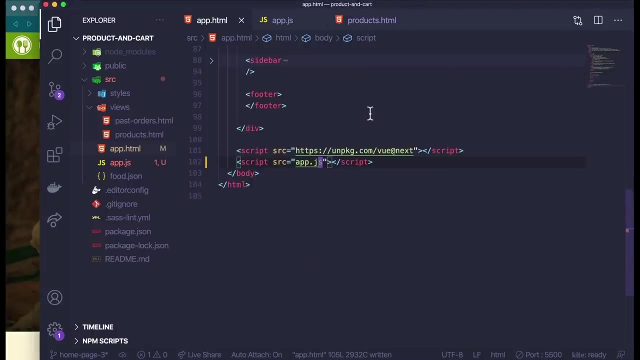 into my html and you can see: my page is still working, my cart is still fully functional, and what this allows me to do is now take this file, this javascript file that I have separated, and import it also into my productshtml file, and I'm actually going to grab. 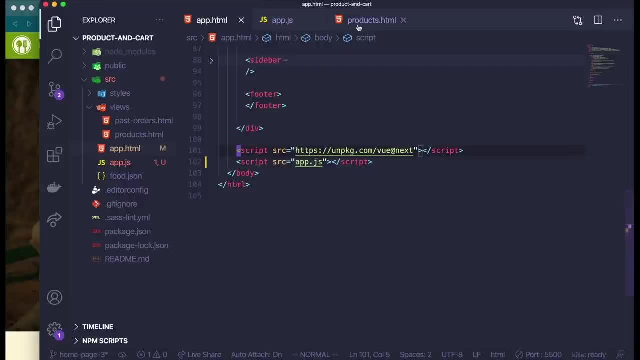 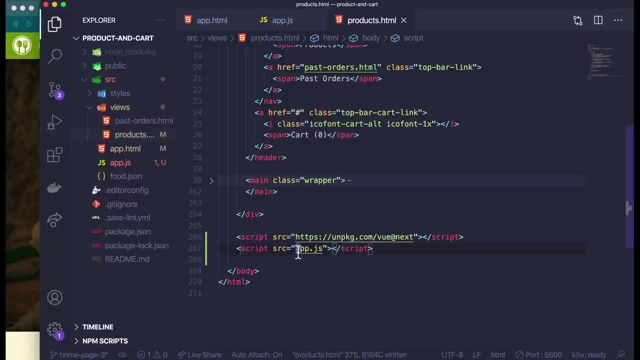 both of these script tags so I can also have my vue, and I'm going to put them at the bottom here. except I'm going to have to go up a directory here because my appjs file lives outside of my views. right here's products and I need to get. 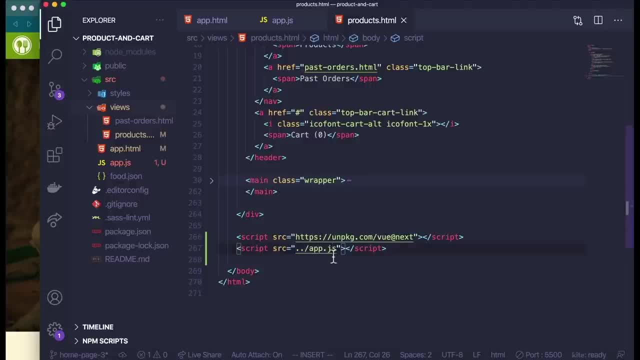 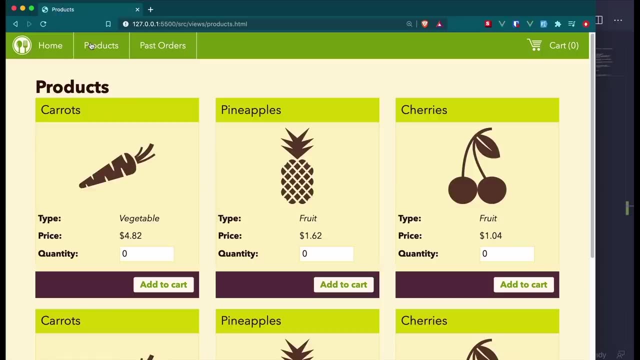 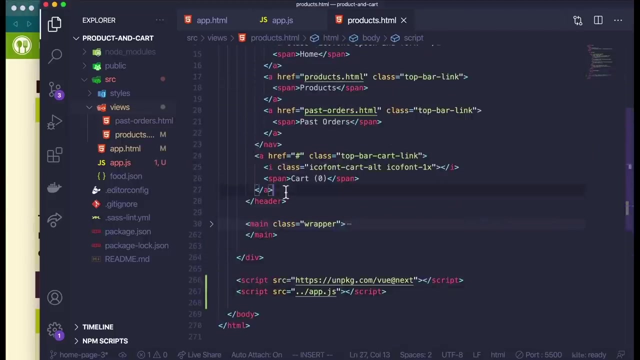 up one folder to app. so I have to do dot dot and that should reference the correct appjs file. let me see if that's working. if I go to products and you can see the cart page doesn't open. but that's because I have not hooked up the cart button yet. 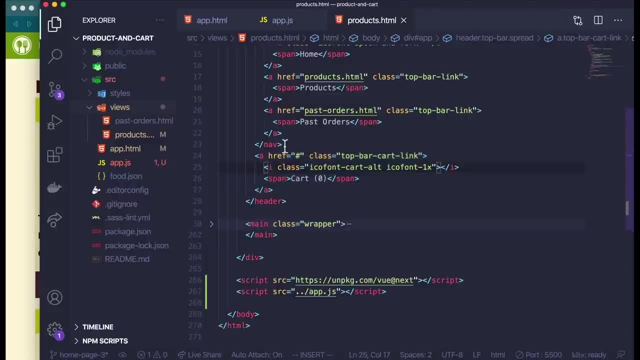 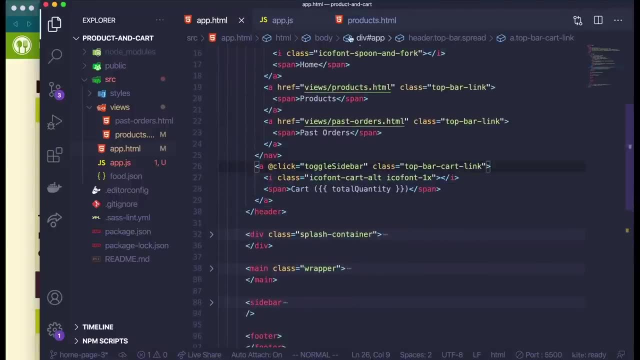 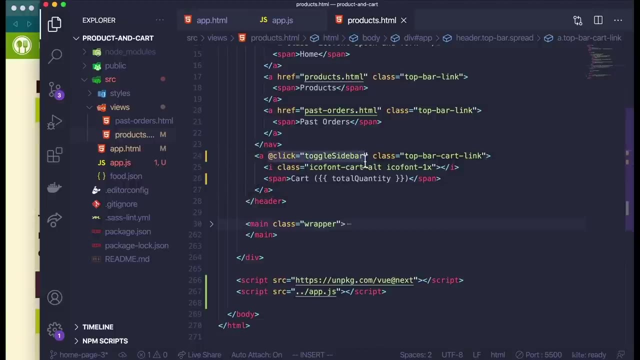 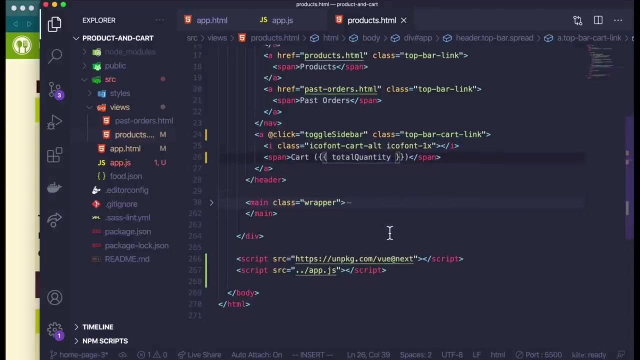 so I will have to copy this over from the apphtml file for right now. so if I go here I can just take the same code and now it should reference that same toggle sidebar function and also display the total quantity correctly as a well, because I am importing. 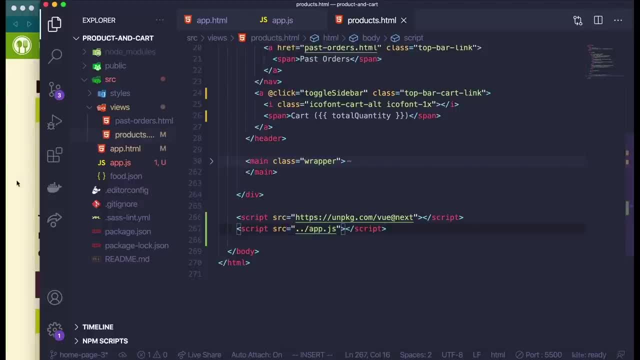 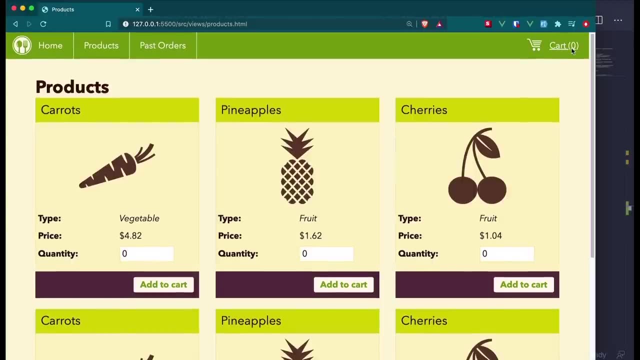 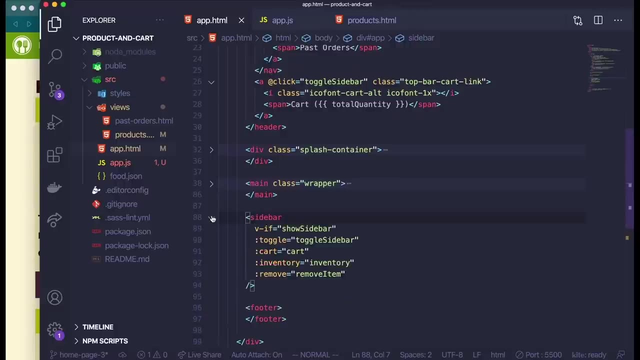 the same vuejs code in the script tag here. now you can see that the cart variable displays just fine on the products page. but if I click here, of course the cart doesn't open, because the cart is only available on this page. I only have the sidebar component here. 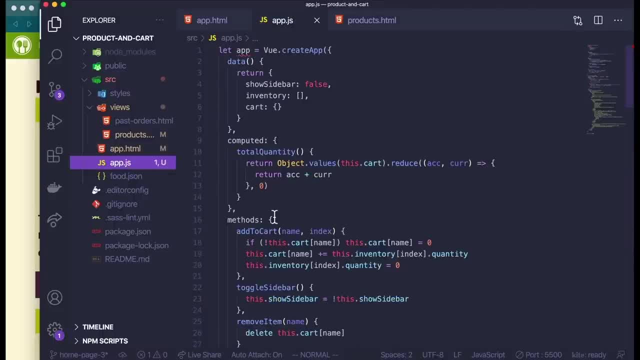 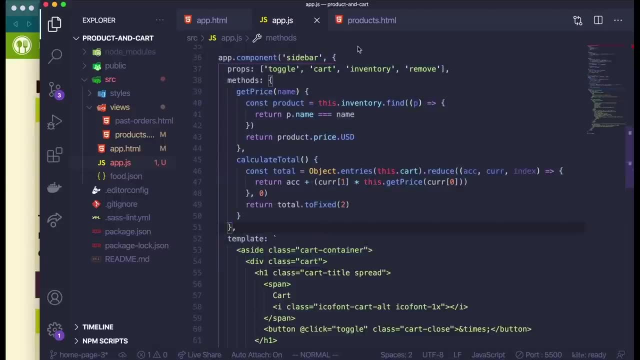 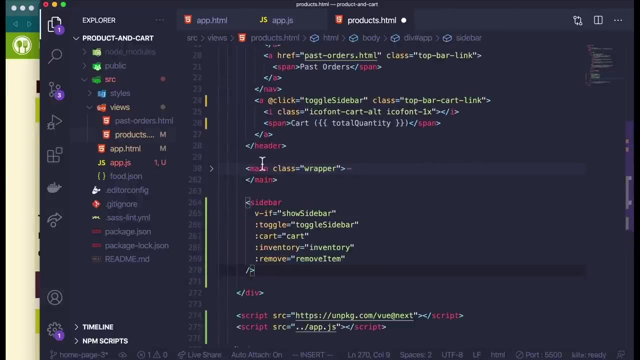 and the sidebar component, you know, is actually a custom component that we made in vuejs. so we can put that on any page where we import the vuejs. so I am just going to put it here, below this main tag and with all the same variables. those should be fine because we are sharing. 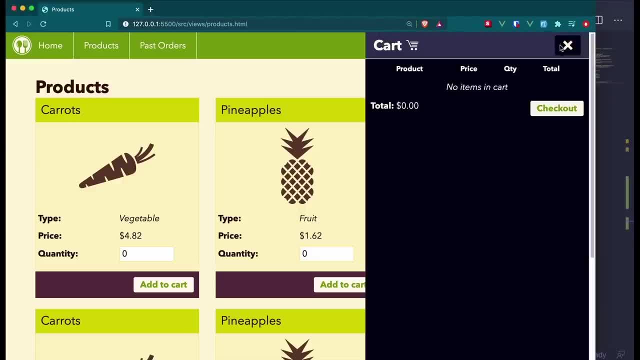 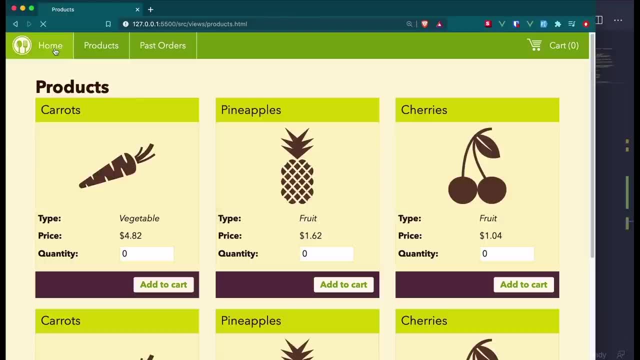 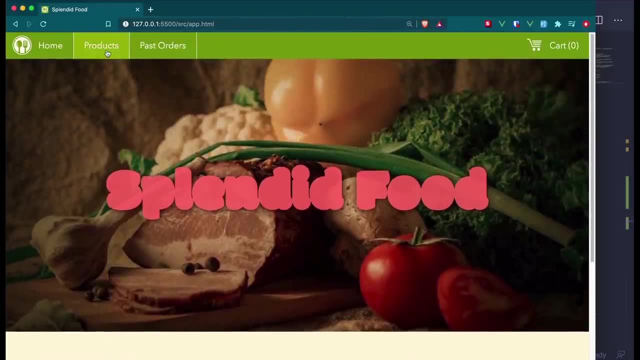 the same vuejs script. let me save that. now you can see I can toggle the cart here. and all of this is pretty much the same thing that we did on the home page down here, where we looped through the different types of foods. we would do the same. 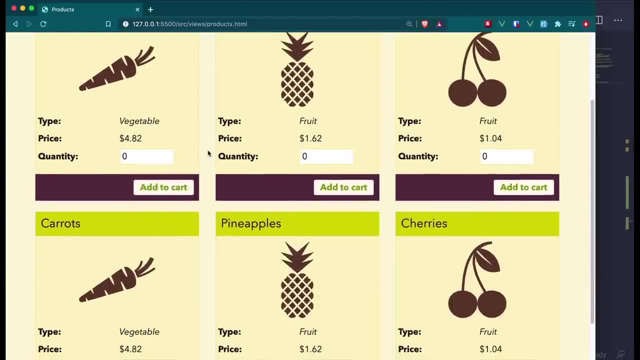 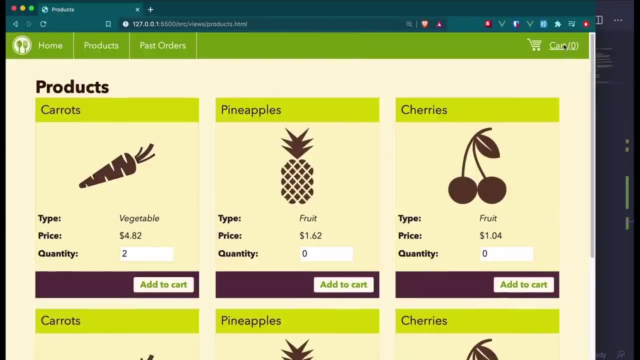 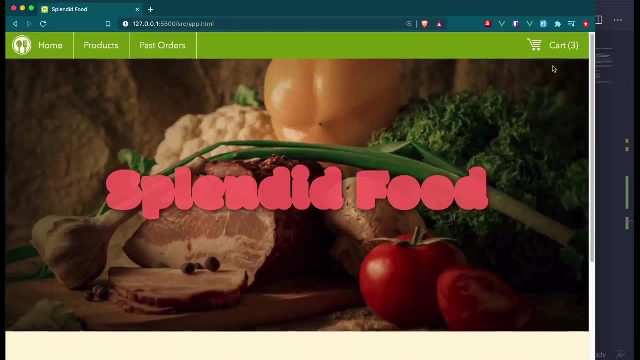 thing over here on the products page. loop through them, hook up each individual number, then hook up the add to cart button so that it would actually display in the cart over here. now if I add items here, let me add a couple to cart. you can see I have three in my cart here. 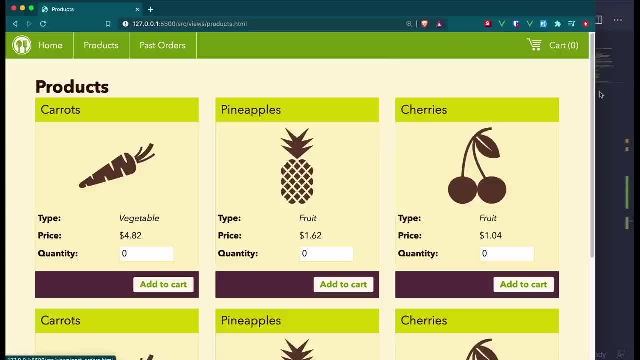 if I go to products, you can see the page refreshed, and now there are no items in my cart. so, though there is some functionality to this application, so far, there are a few problems that we have run into with just using a CDN to import vuejs, and that is. 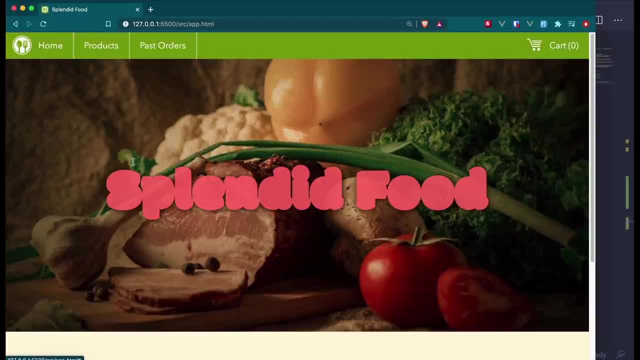 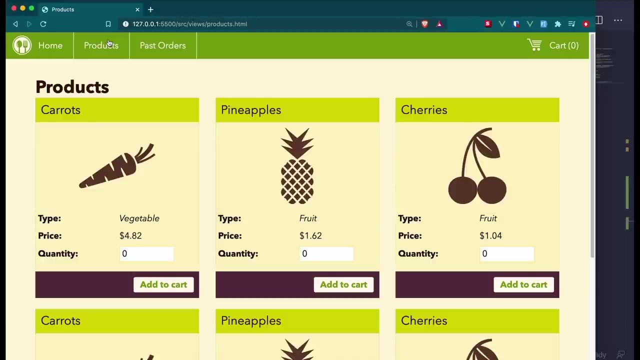 how do we share data across pages and across page refreshes? so here at the home page, when I add something to the cart here, it leaves the cart as soon as the page refreshes. so as soon as I navigate to another page it's gone. now how would I fix that problem? 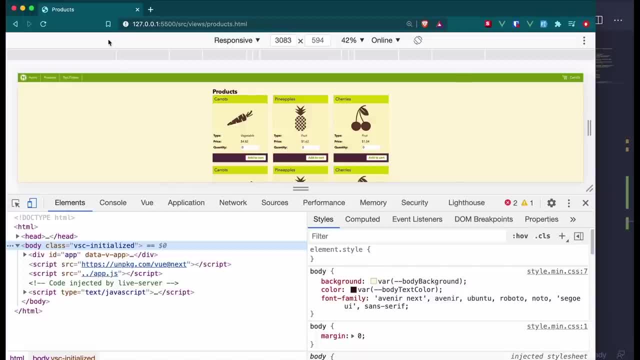 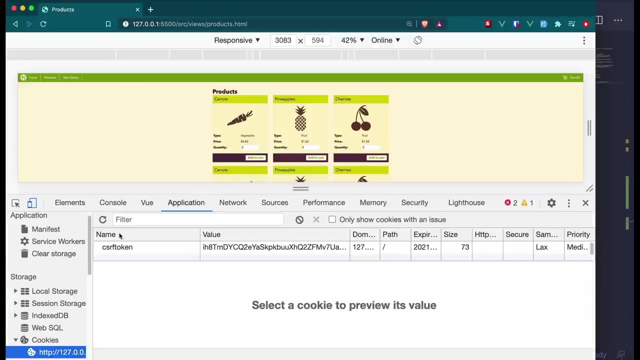 so generally in front end applications, we would want to do something like persist our data or save our data somewhere. one easy way to do that in the browser- one very common way- is to go here in application and you can see there's different types of storage. this is in browser storage. 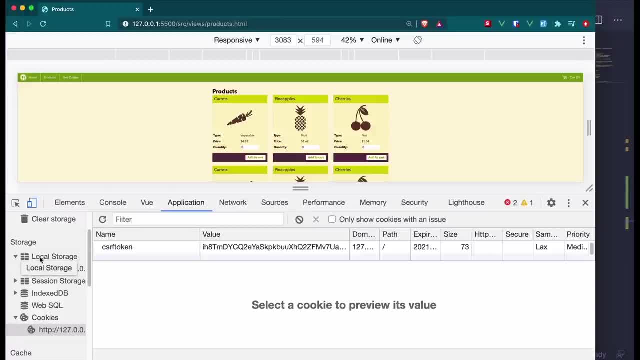 and local storage will persist even if the page is refreshed, so we can actually save the data, like our cart data, into local storage here and then, if we refresh or anything, we will just automatically try to pull anything that's saved from local storage for the way our application is set up right now. 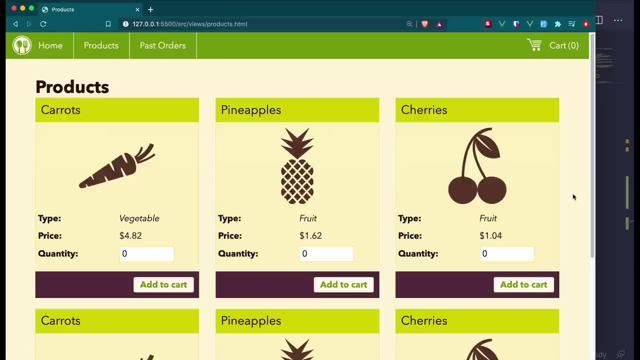 that would be. every time we navigate to a new page we would have to check local storage, see if there's anything in there and then pull it into our application. it's kind of a work around for our set up, so one way to fix this would actually 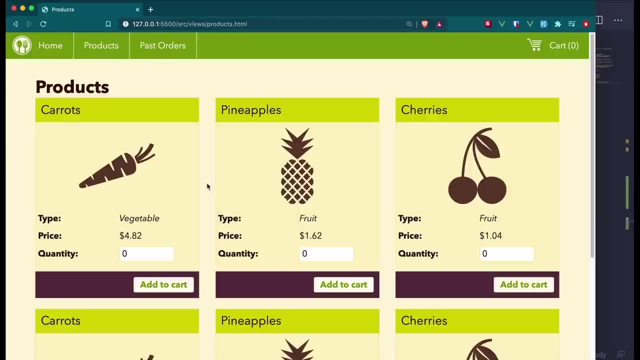 be to create a single page application with Vue, where the front end would actually do the routing instead of our server. in this case, we're just using a live server in VS Code, but our server is serving up pages every time we go to a new URL here. 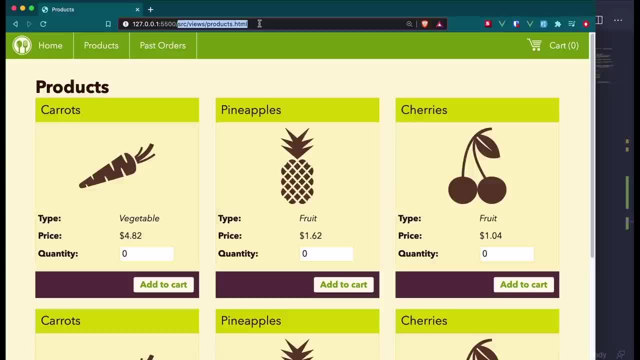 and that's why it has to refresh, because it's coming from the server, whereas if we make a single page application, there will be no page refreshes. we will go seamlessly from page to page because our front end, in other words Vuejs, will be routing us to different pages. 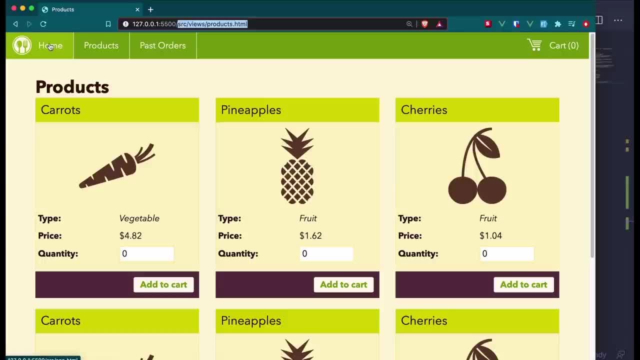 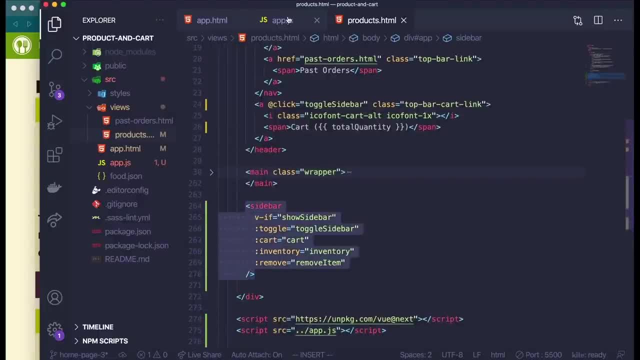 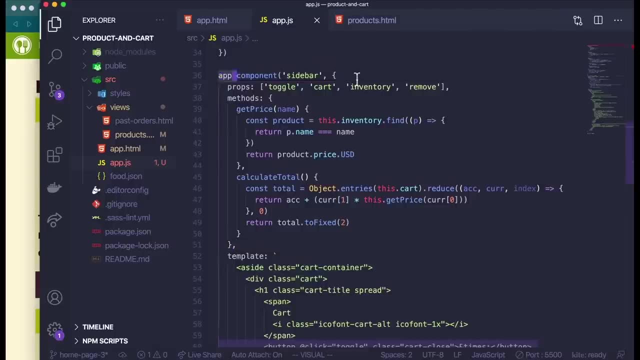 the second problem, as you can see, is sharing code. we do have some duplicate code across pages. of course, we are reusing the same sidebar template here. this sidebar template, we just registered it as a Vue template, a Vue component called sidebar, and we can use that on any page now. 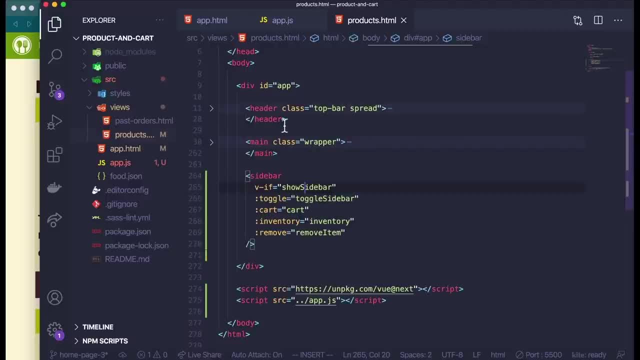 we could do the same thing with header as well, and we would probably do that if we were going to build an application using the CDN. we could extract this into a template as well, and then we would have to do the same thing for the past orders page. 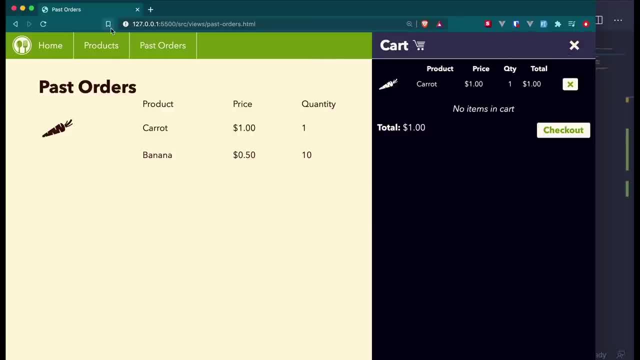 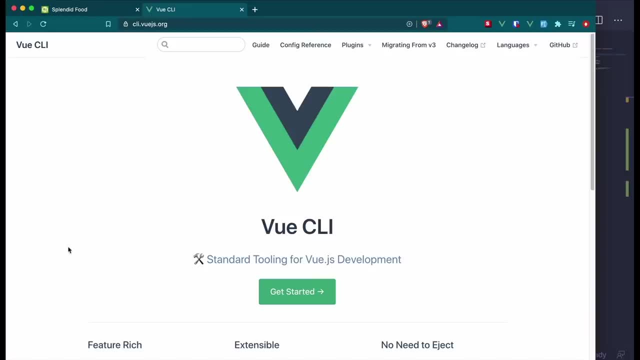 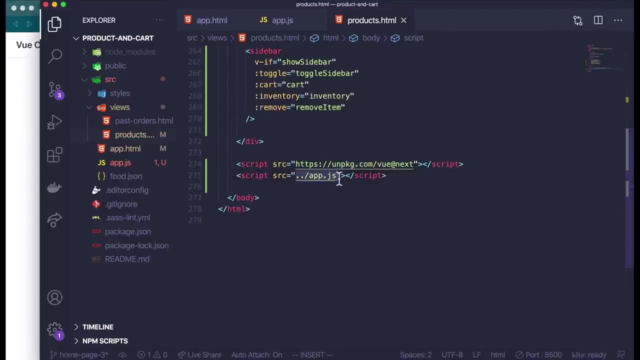 of course, none of this is dynamic or set up yet, but the easiest thing to do is actually to set up our project in something called the Vue CLI. as our codebase grows, it will be very difficult to manage many different components if we are managing them just importing. 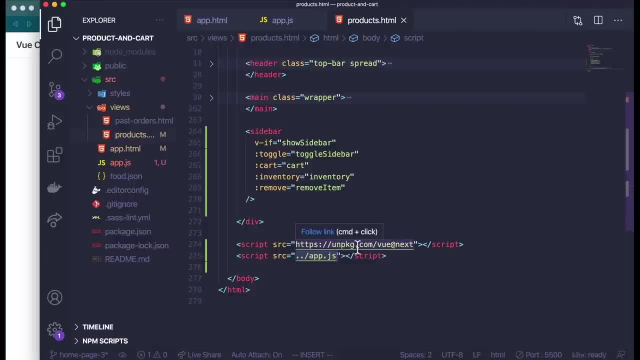 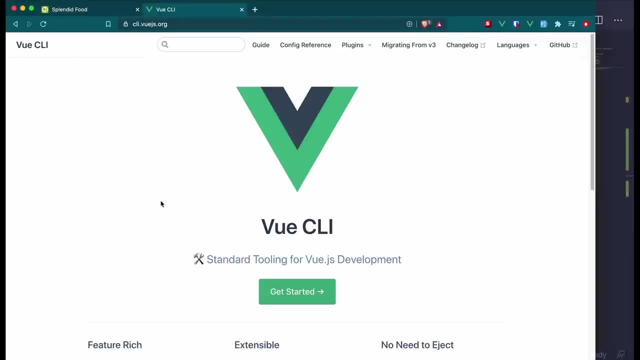 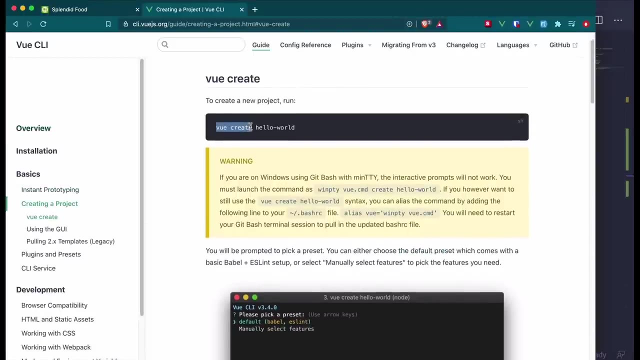 different files into all of our different HTML files. but there is a much easier way and that is with the Vue CLI. this is why it was created. the Vue CLI basically gives us one command, Vue create, and our project name. then it creates a whole project for us, it walks us through. 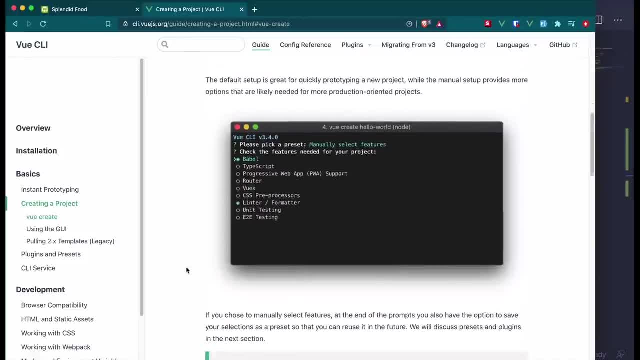 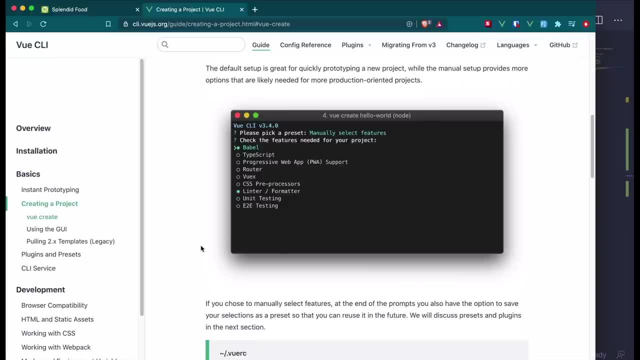 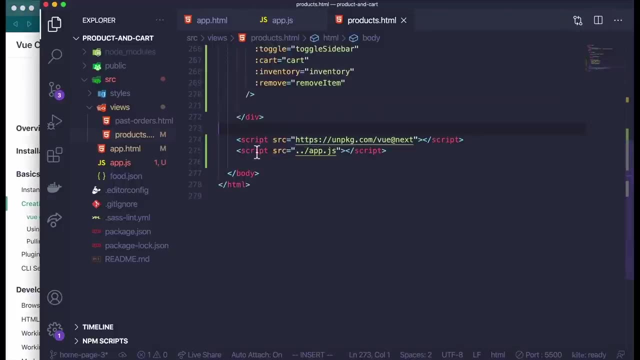 a setup wizard asks us what features we want and then we will create all of the files, folders and build tools necessary for a robust front end single page application. so in the next video we are going to take all of our code currently in HTML files and our JavaScript file. 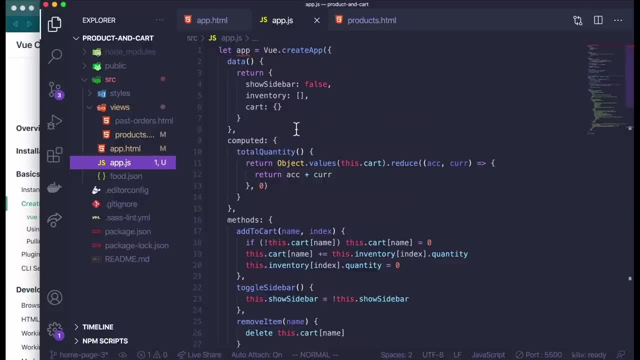 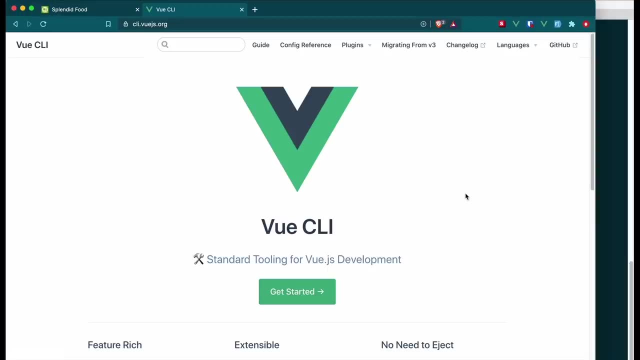 and convert it to a Vue CLI application. I'll see you in the next video. let's get started with the Vue CLI. I am at clivuejsorg and I'm just going to click getting started and if I go over to the side, click on installation. 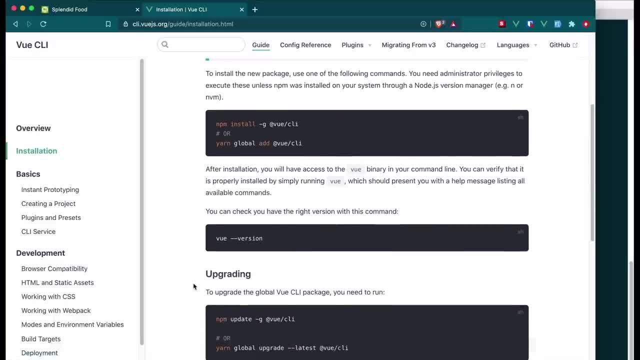 I can see that it is prompting me to globally install this Vue CLI package at Vue dash CLI so that from my command line or terminal I will be able to use a Vue command to create projects. now you might see some places on the internet that install a different package. 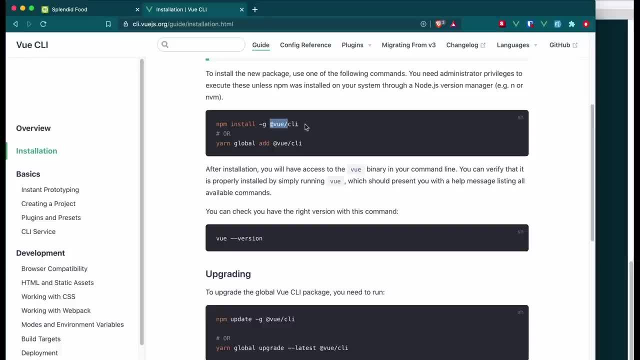 without the at sign and slash, just Vue dash CLI or something like that. that is an older version of the package. Vue basically has its own namespace and then each one of its packages are after the forward slash. so to install Vue CLI you can copy this command here: 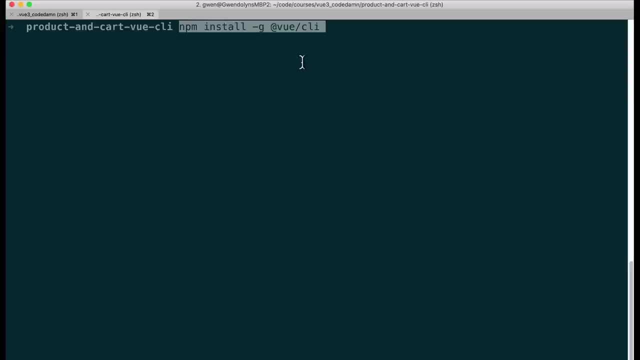 I'm going to go to my terminal and now I have the Vue CLI installed. I can check and make sure that it is installed by checking the version. right now I have version 4.5.11 and now I want to use it to create an actual Vue project. 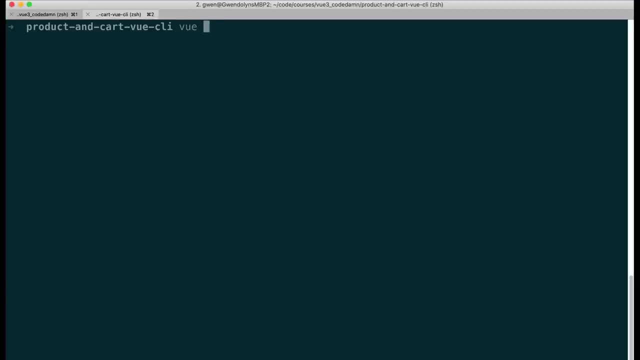 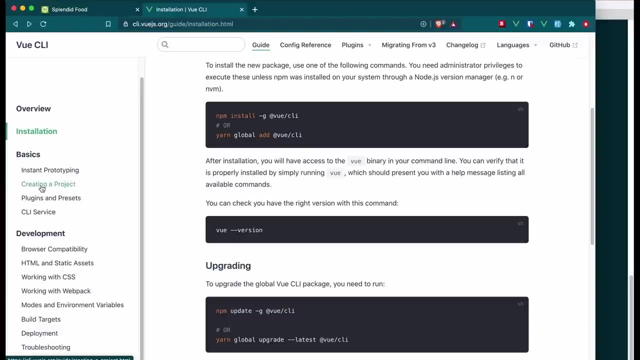 and I can do this through the Vue create command and then give it the name of the project that I'm going to create. if you want to see the documentation for this command, you can come over here under basics to creating a project and read about how Vue create. 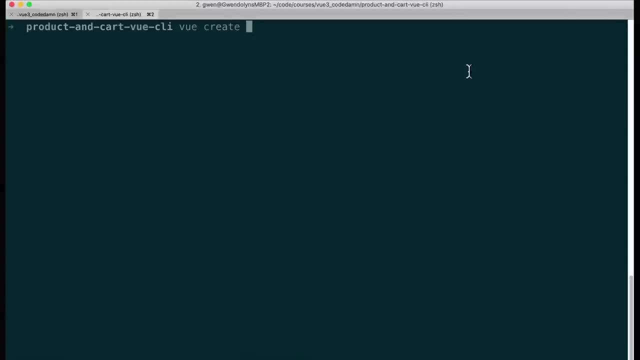 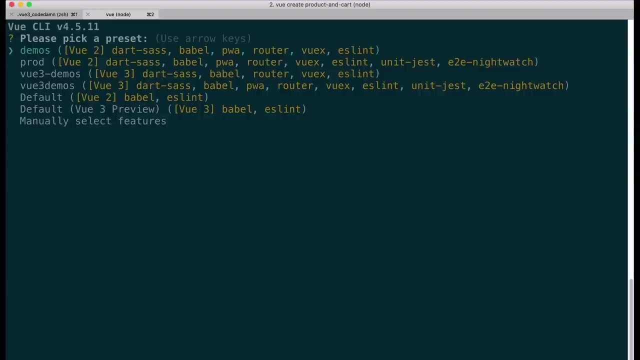 works. here I'm going to go ahead and say Vue, create product and cart as the name of my project and click enter. now if you've used some tools like create react app, you will notice that here it's a little bit different. it doesn't just bootstrap the whole project. 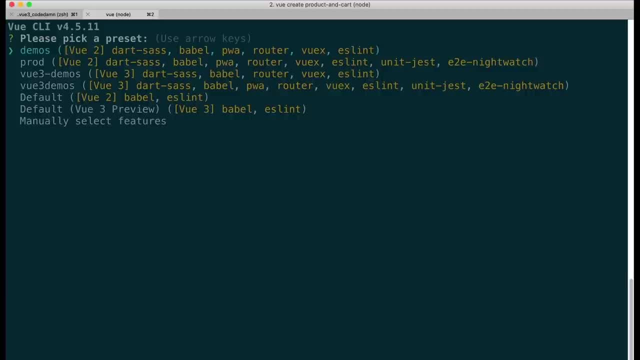 for you right away. you actually get to pick your own options and the packages that you want to install and use. these top four options here are actually custom options that I have created myself. Vue gives us these two defaults right now. one is for version 2 of Vue. 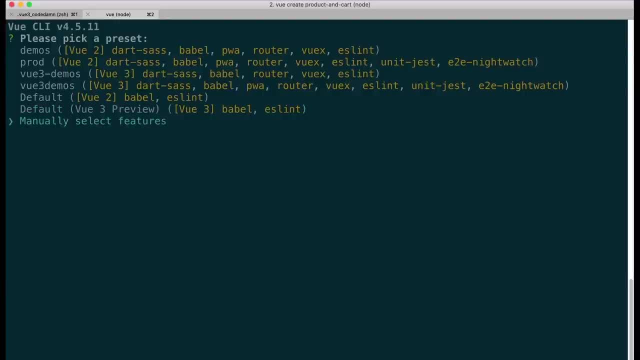 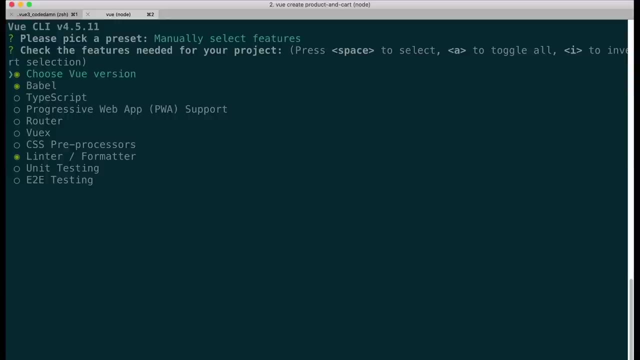 and one is for version 3, and then it also gives us the option at the bottom to manually select features. so I'm going to go ahead and do that, just to show you how it works. so I basically use the arrow keys and then I can click enter. 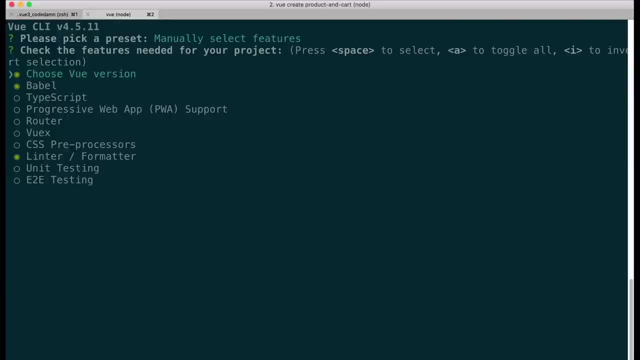 when I want to select something. now you'll notice that this list here is multi-select and if I press spacebar I can select or deselect an item. of course I want to choose my Vue version because I want to use version 3. I definitely need to have Babel. 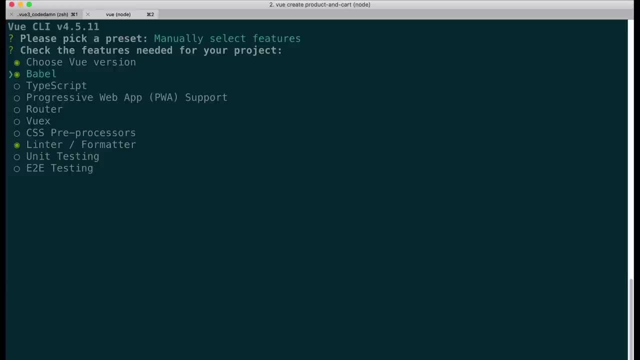 set up for me. for transpiling my Vue code, I'm going to need routing in this application. I'm also going to use state management, but I'm going to add that later to show you how to add a Vue CLI package after you've already set up. 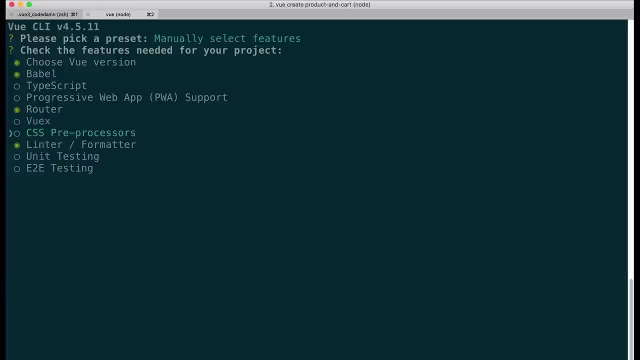 your application. CSS preprocessors are things like sass. if you think you will want to use sass in the future, it's a good idea to go ahead and set it up now. I believe this also works with LESS and Stylus as well, and then I definitely want linting. 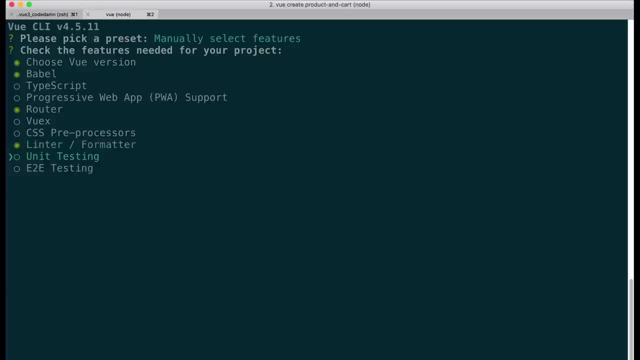 and formatting in this project, and I can optionally select testing if I want, but I'm not going to do that this time. so once I'm ready, I'm going to hit enter. it takes me to the next step. I can choose the version of Vuejs arrow down. 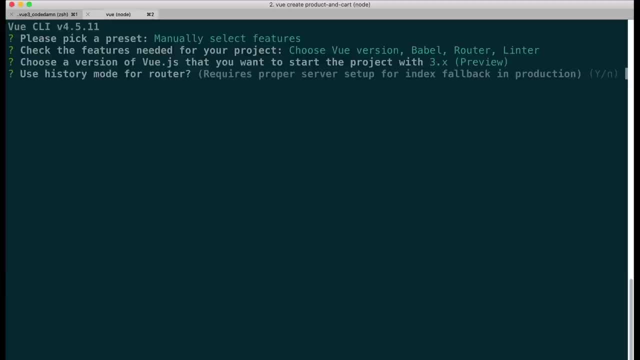 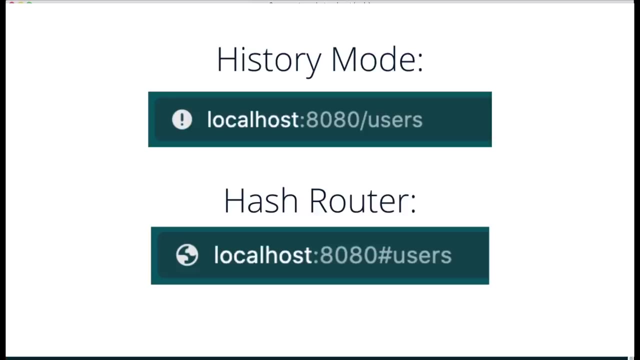 and I'm going to choose version 3 use history mode for the router. this is a pretty small coding change, but it's usually what you want in a project. this basically only affects the URL of your project from a user point of view. so if you want, 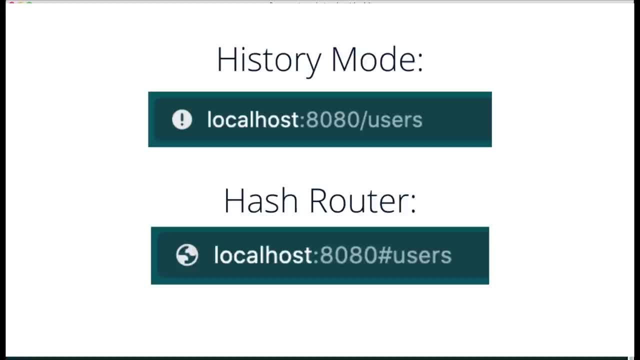 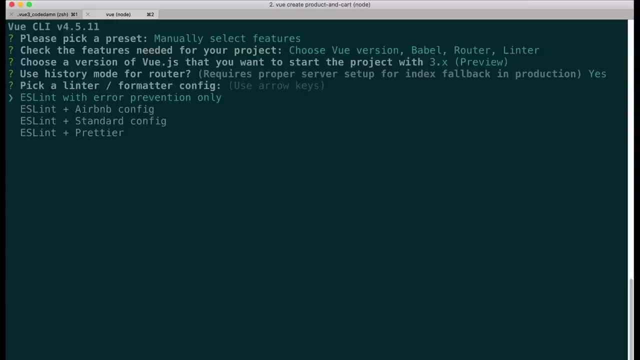 your routes to be after a hashtag, it will use hash router. if you want your routes to be after just a normal forward slash, like any website you would navigate to in your browser, then you can just go ahead and use history router, and I'm going to use history router. 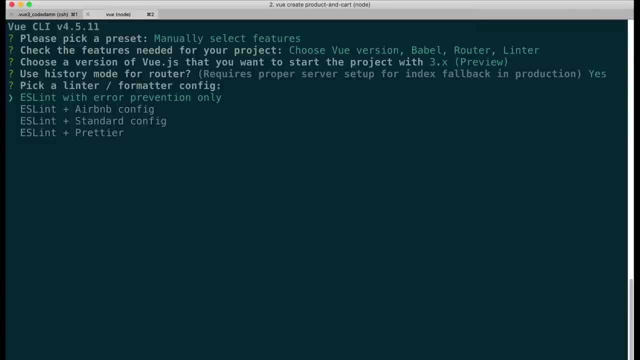 now it's asking me to pick linter and formatter, so I'm going to go ahead and pick eslint, plus the standard config that it has for Vuejs. click enter. I'm going to save the files. when they are saved, I'm going to choose to put my configuration. 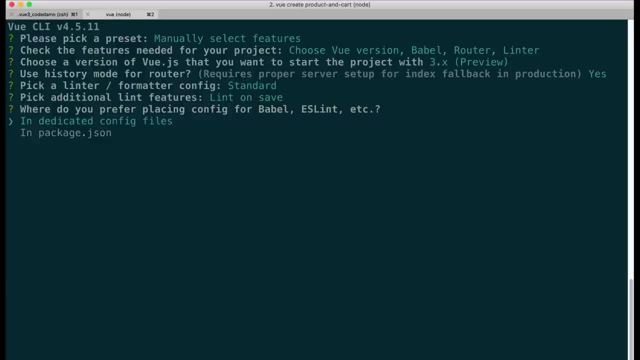 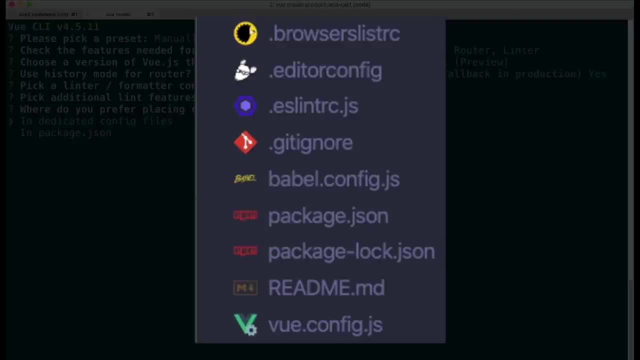 in the packagejson this time, just so I don't have a bunch of extra config files. usually when you have larger projects you want dedicated config files, so it's not cluttering up your packagejson. do I want to save this as a preset? no, I do not this time. 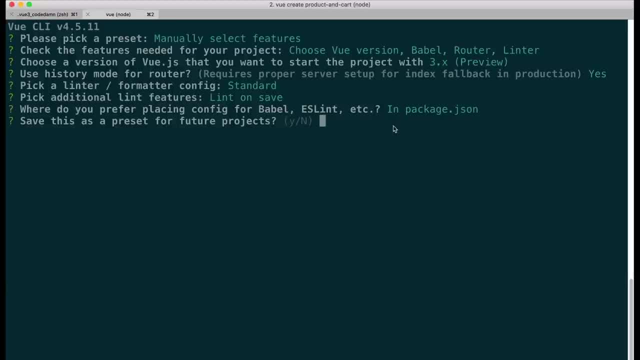 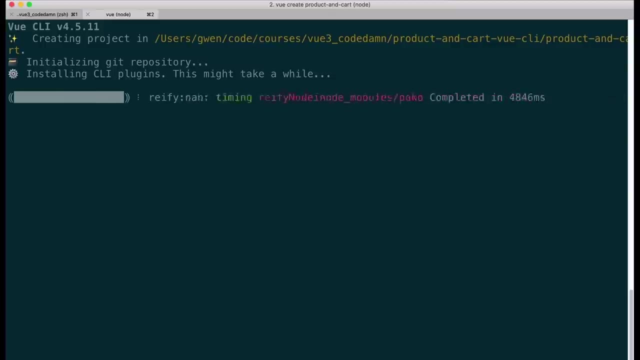 but if you remember at the beginning of this walkthrough, the four top options, those were presets that I had saved in the past. but here I'm just going to say no. here it's basically setting up my whole project with the file structure and everything, and it's also running. 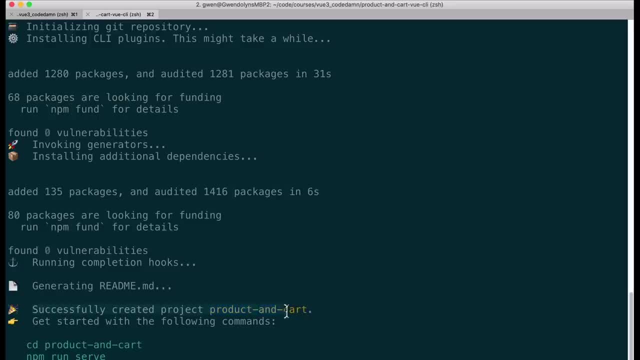 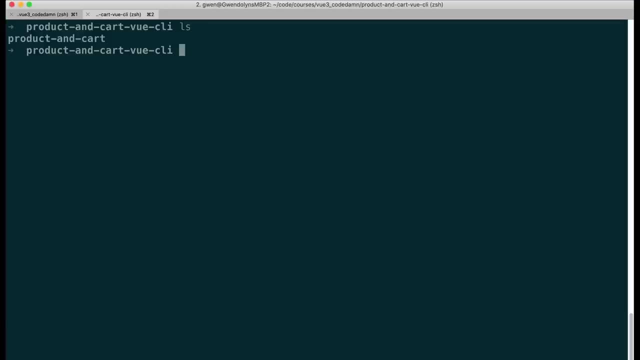 an npm install, you can see it successfully created my project. if I list the folders inside, now I have this new folder that was created for me by Vuejs called product and cart. I'm going to go into that folder and you can see when Vue spun up the project. 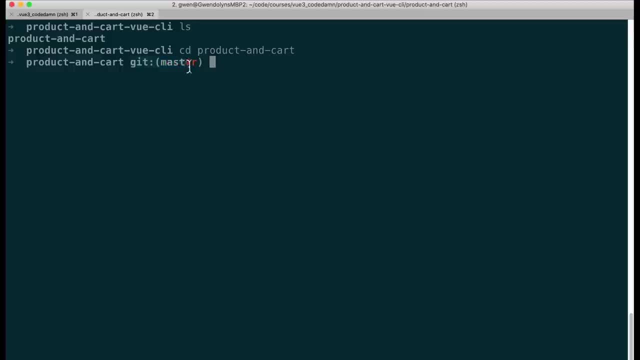 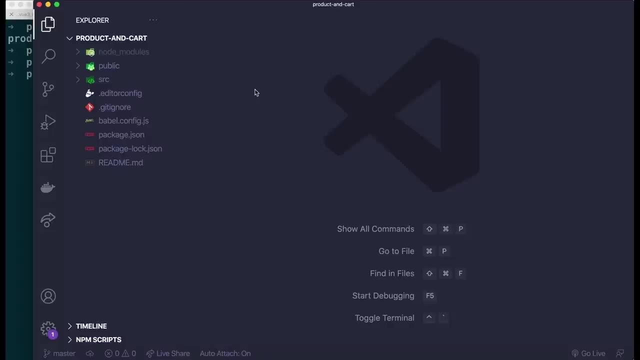 for me. it also initialized a git repository for me and saved all of the changes that it did initially as a commit. so let me open this up in VSCode and I have my complete project created for me by Vuejs. in the next video we will look through 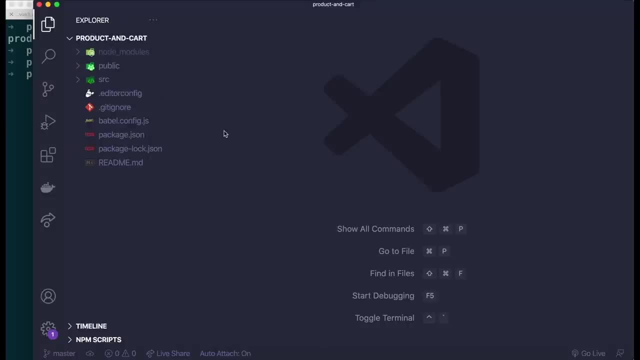 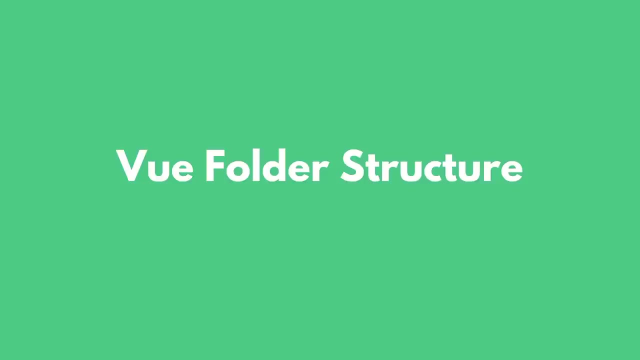 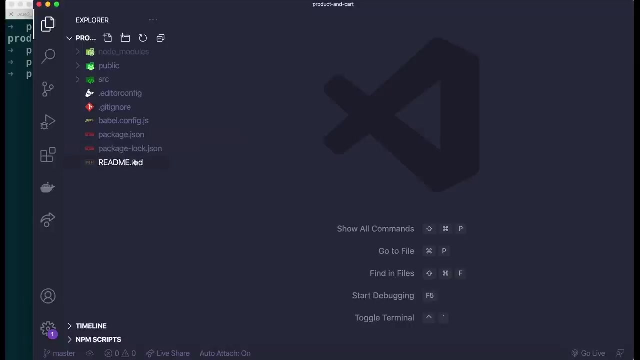 all of these folders and files and give you a little bit of a tour of how your Vue project is laid out. let's look at all of these files and folders that Vue spun up for us. now, looking at this, this looks pretty much like the last project. 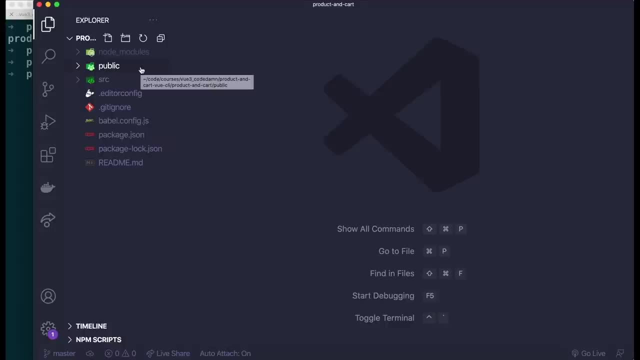 that we worked on with static html, css and javascript files, and that was by design, to give you the same style of coding and file structure that you would be using in a real Vue application. this, however, is much, much nicer. starting with the Vue, CLI gives us. 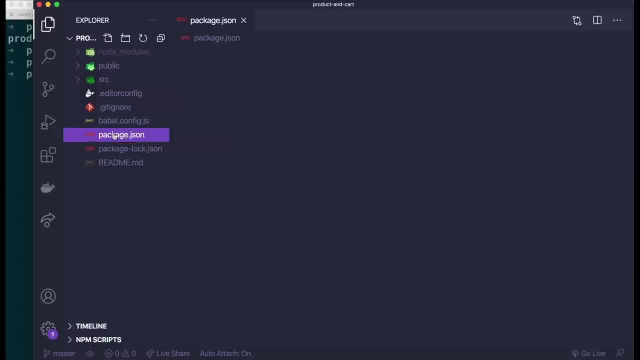 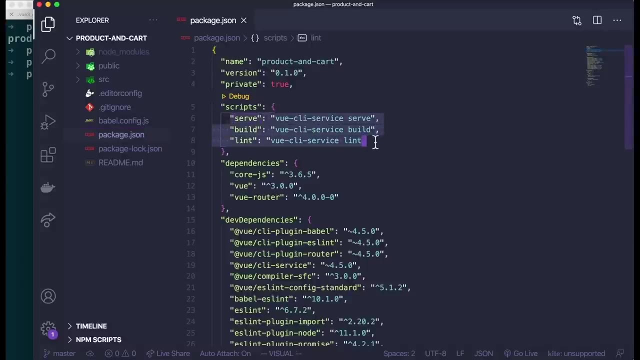 a lot more features out of the box, though we can see in the packagejson. we have three scripts here by default. there would be more if you choose to install the testing packages as well, because we installed a linter. the Vue CLI gives us this lint command. 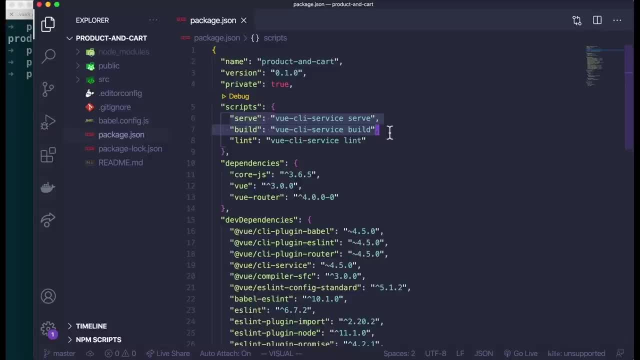 and then it also gives us our main two commands for the Vue application for development locally. it gives us this serve command which basically calls this package Vue CLI service. that's from Vuejs. gives it the serve command and it will run a development server for us. so there's. 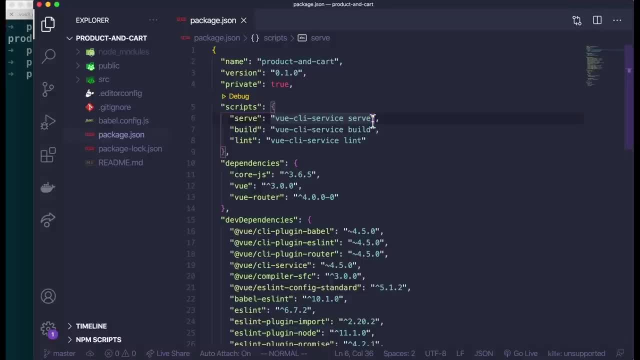 no more of the old complicated server setup that we had in the last version of this. in the last application, the build command is really for when we want to host our project live. this will generate production ready files for you, like your HTML, CSS and Javascript, so you can. 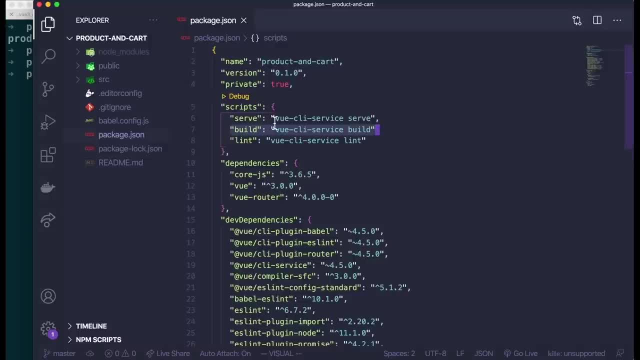 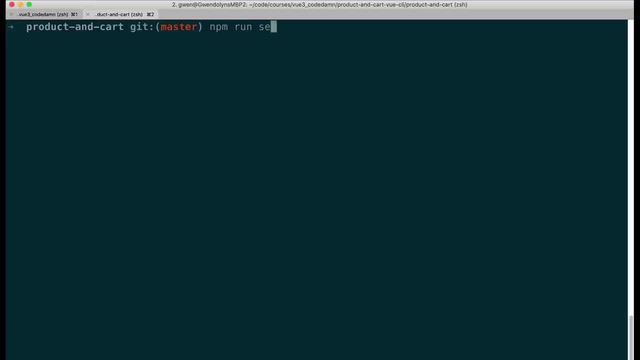 deploy them and have a live website somewhere. we're just going to be talking about this command in this video and to give you an idea of what it does, let's go ahead and run it. I can use npm to run the command, so npm, run, serve. and now my app. 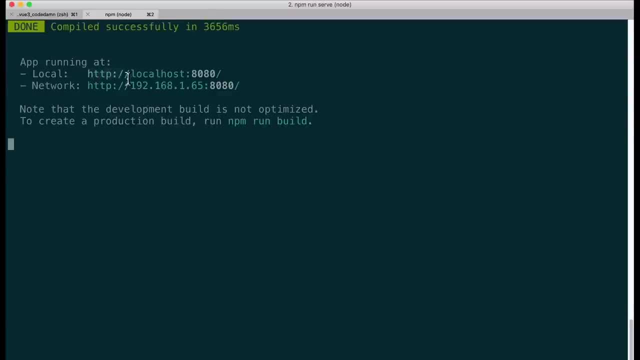 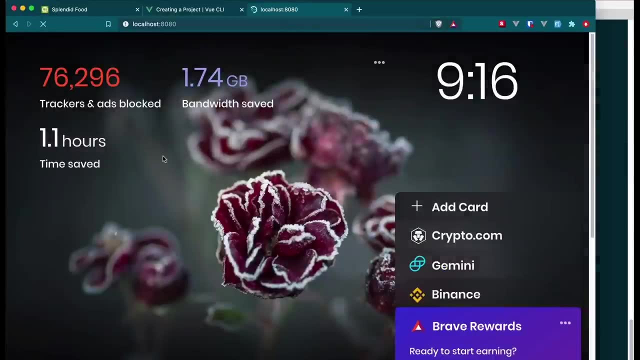 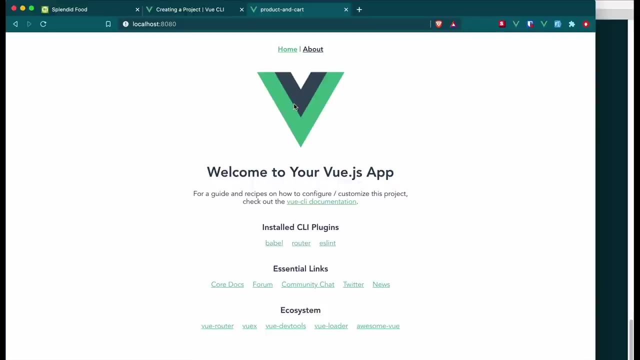 is running at port 8080. if I highlight something in the terminal, it automatically copies. I'm going to come to my browser, open a new tab and I can see it gives me an app already set up out of the box and because we chose to. 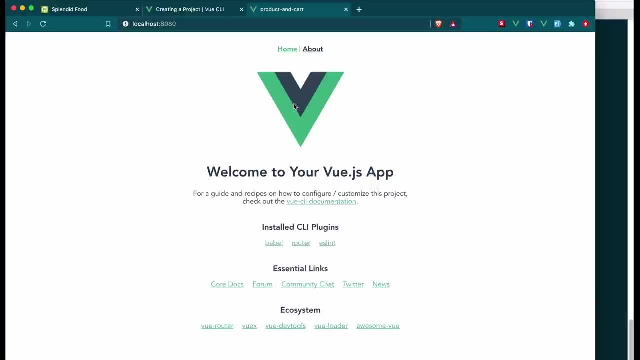 install a router as well. it installed the default Vue router, which is also called Vue router, and you can see I can go to different page routes. now this isn't the same as our last application, because there is no page refresh in between page routes. these are not HTML. 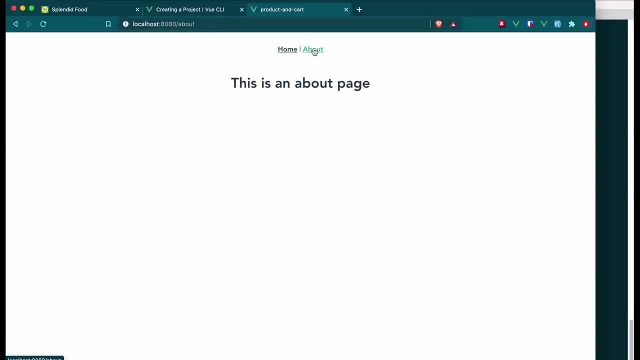 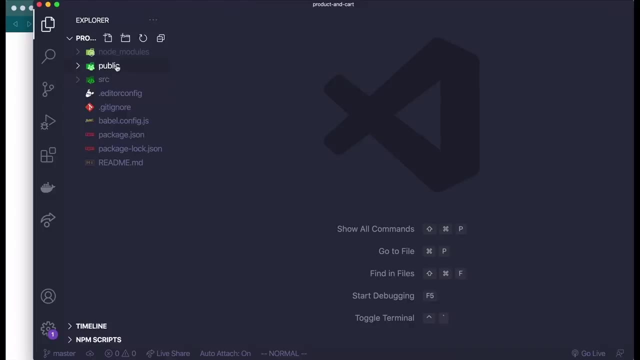 links. this is just a Javascript router rendering, hiding or showing different pages of this application. you'll also notice from the home page it's just port 8080. when you go to the about page it adds slash about. if we look in the public folder here, you can see. 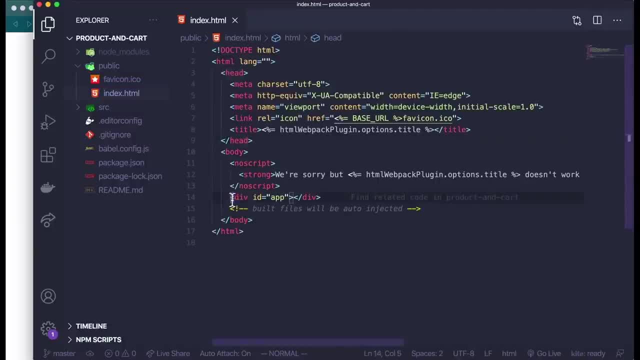 here's our HTML page and we have a div of id app and this is where our app will be injected, but also when our application is built under the hood. this Vue CLI service command is running webpack and bundling all of our files together and also handling running babel. 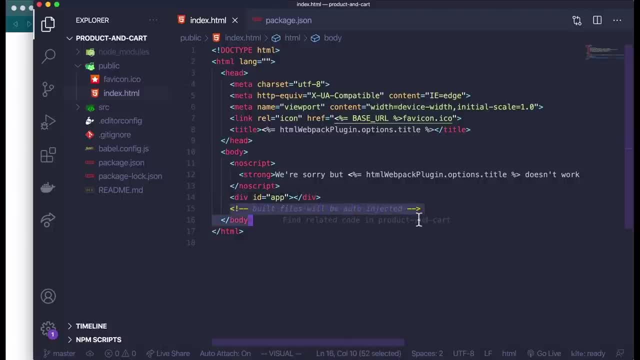 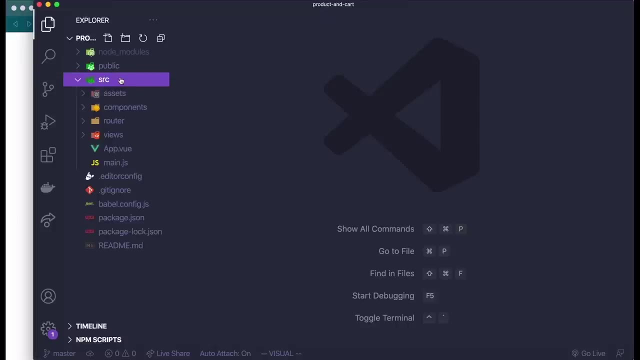 to transpile our files, and so all of the Javascript and everything will be injected as script tags as well here. but we generally don't have to worry about this indexhtml file in Vue project because, again, most of what we will be doing is in the source folder right here. 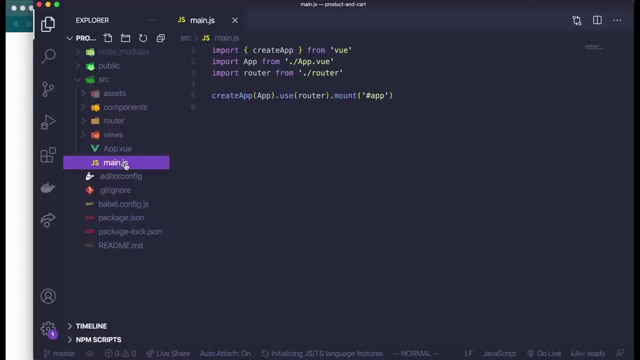 so we have a mainjs file that is always created for us, so this is basically the same thing that we did in the previous application. if you do see Vue 2 code, this file will look a little bit different, but you'll still be able to see the different parts. 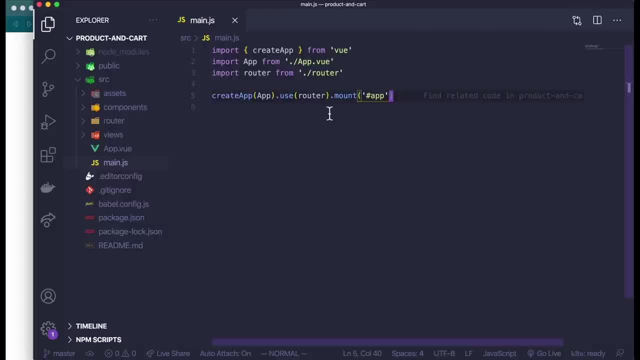 just the organization and syntax is a little bit different. just like before we have to pass in a root component, we chain on any packages that we want to use, in this case the router, and then we mount that to the dom. so inside of the div with id of app. 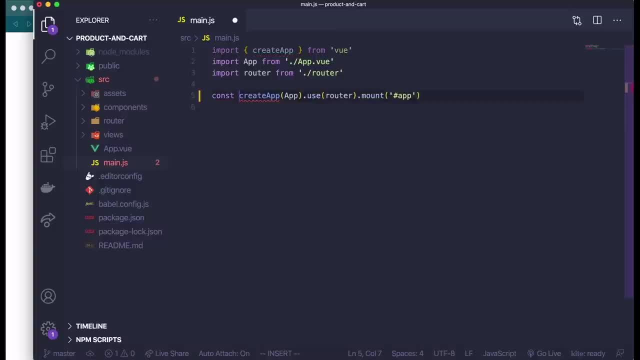 and you could also rewrite this as const app and then appuseRouter and then appmount. that's a bit easier to parse through as you add more packages. now, when we are looking at this initial page, where does all of this come from? let's take a look. 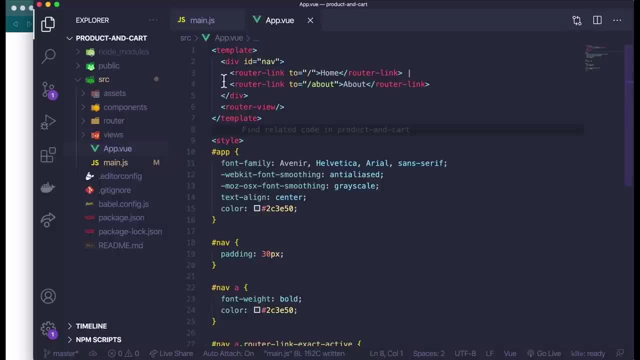 so we have our main component app, but you'll notice in app there's no real content here. all it is is a div. this is basically the top navigation. now, where did this router link come from? this is a custom component, actually, and if you look at our main js when we use 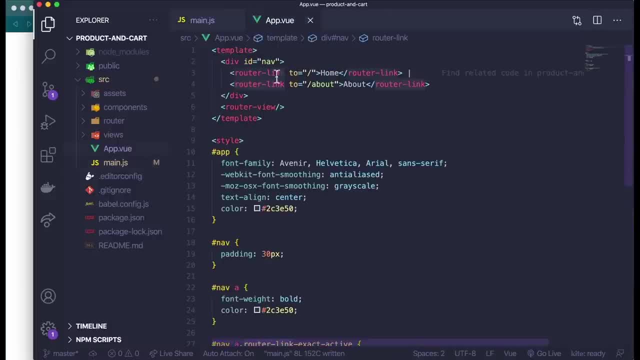 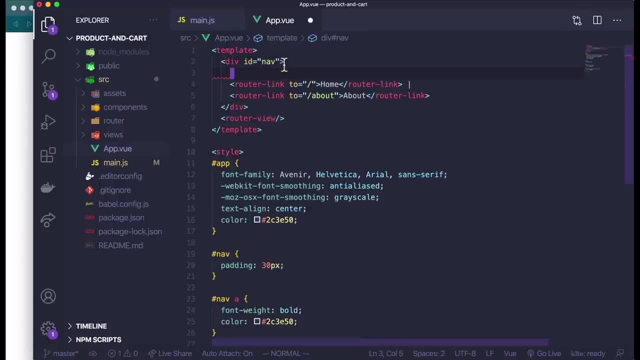 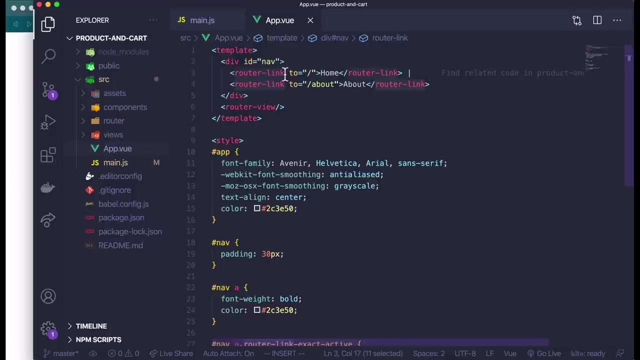 appuseRouter, we are actually given some components like router link as well as router view. now, router link is actually a substitution for using the anchor tag to link to another page, except router link is made by view router specifically for single page application routing, where our javascript. 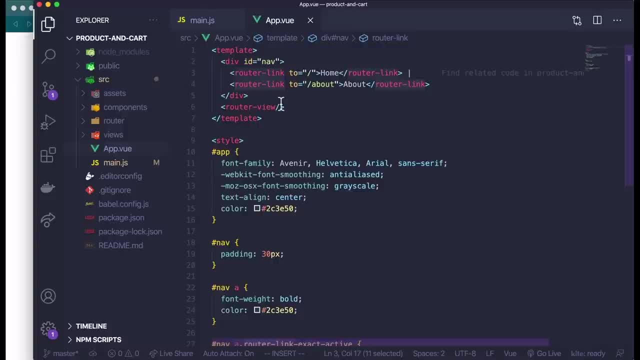 handles the routing instead of linking to a separate html page. of course, we only have one html page and all of our static content is injected into that one page, and the router handles the route, making it appear as though you've navigated to another page, while really it's just showing. 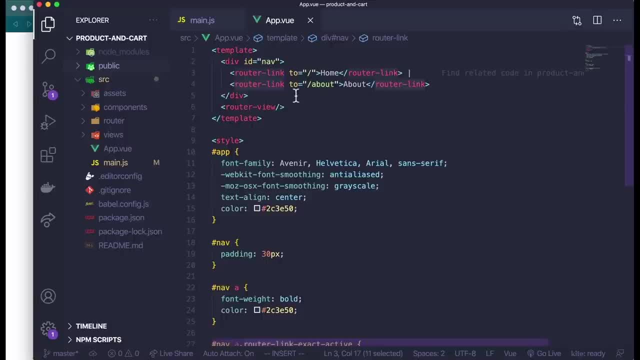 and hiding different elements on the dom. so we have these two router links, and then what does router view do? so router view is actually our page content and our router will handle replacing this router view tag with whatever component we tell it to in our routes file that we are. 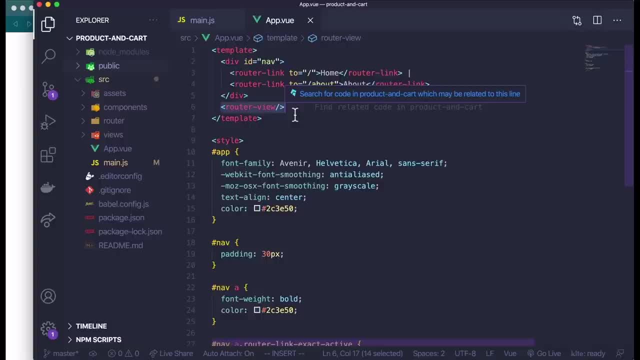 about to look at. so router view is just a temporary placeholder for whatever we put on the page and you'll see, as we navigate to different pages- those home and about links at the top of this file. those will stay no matter what page we navigate to. but all of the 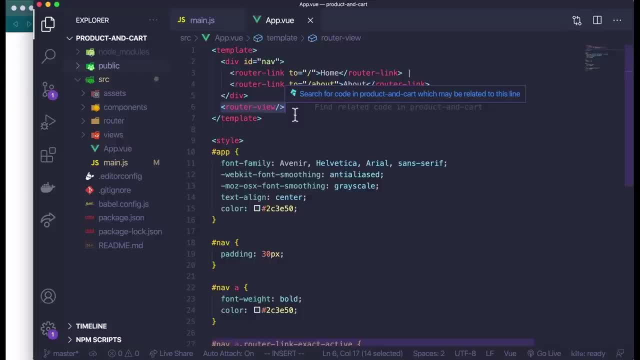 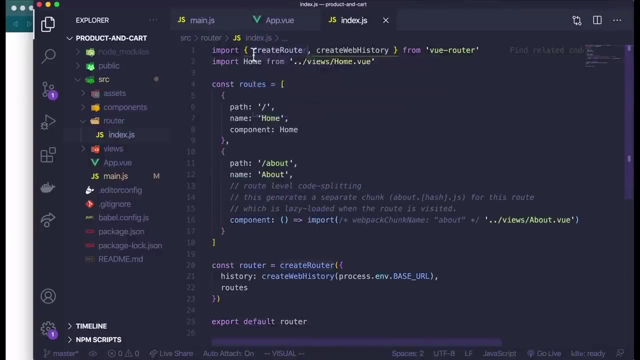 content below. it will change because those are the components getting injected into this router view area. if we look into our router indexjs file here we can see that we are using the view router api to create a router. and when we create a router here we are passing in two things. 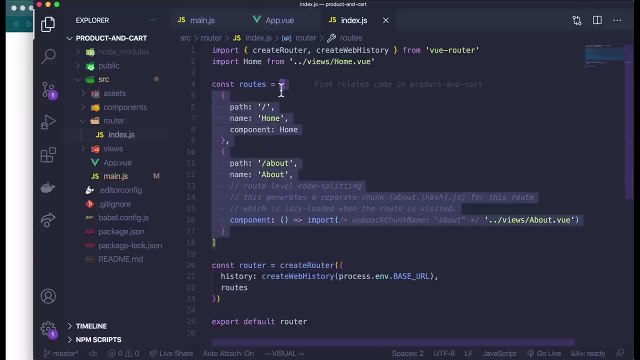 so the routes, which is an array of all our routes that we have in the application and then history mode. it set this up for us because we chose to use that, and view is handling all of that under the hood. but let's talk about the routes here. 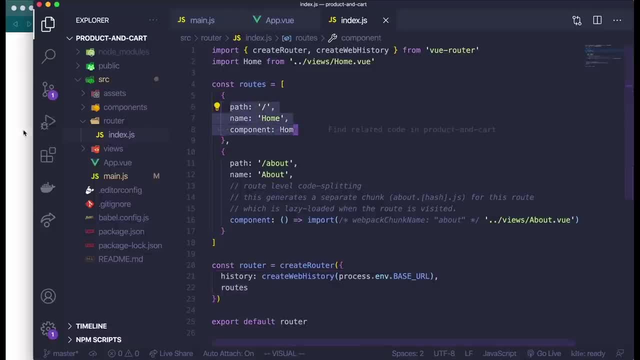 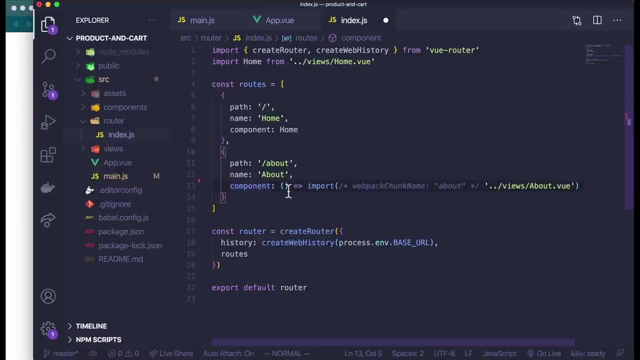 so we have the default home route, which is this page, and then we also have the about page, which is found at this route. now you don't have to worry about code splitting and lazy loading and all of that other stuff. those are more advanced routing concepts, so I'm going to get rid of. 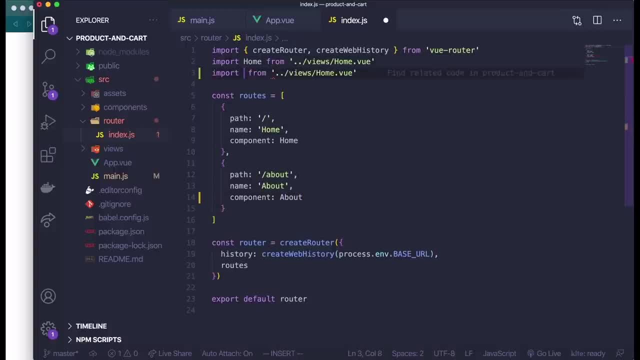 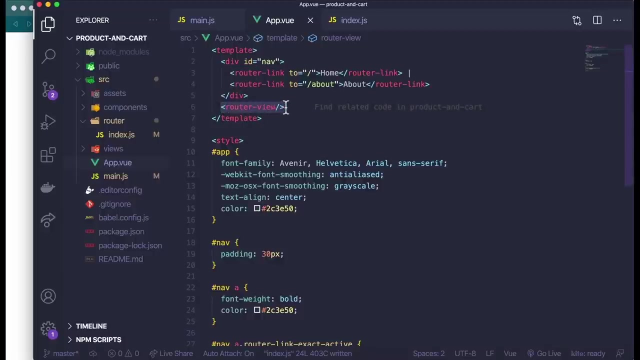 that line and then just import the about component just like the home component. now you basically define routes here and instead of importing the components that you want to show on a page into your appview, you just use a router view tag here and then you import any of your. 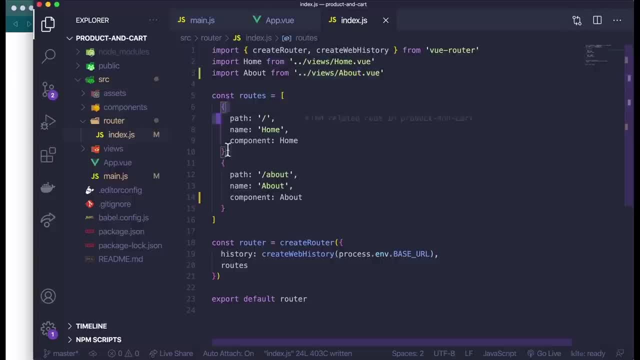 view components like home and about, into this file you define the path where that component can be found at the name of that component- now the name is mostly used for routing- and then you tell it which component will be found at that path, so at the home path. 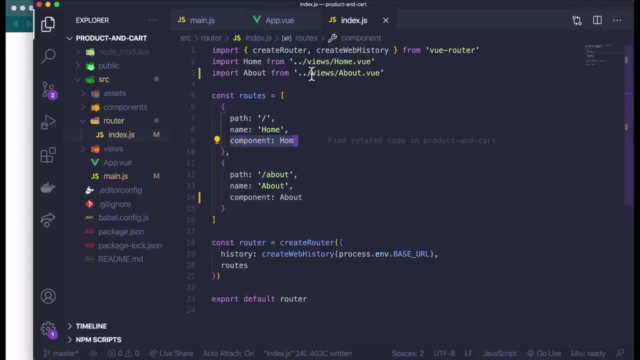 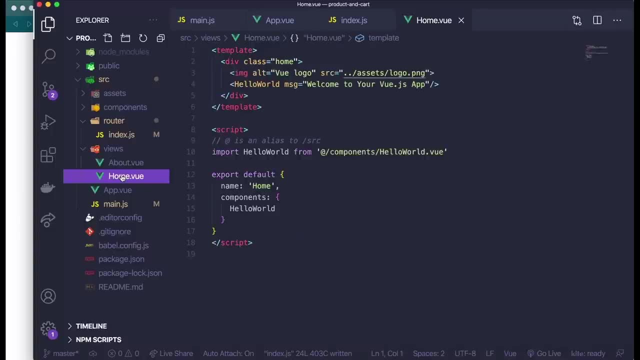 we're going to find the home component. now, where is the home component? you can see that it is in views, slash home. so let's go in here and we can see that this is the component. it has an image, which is the view logo on top, and then it also. 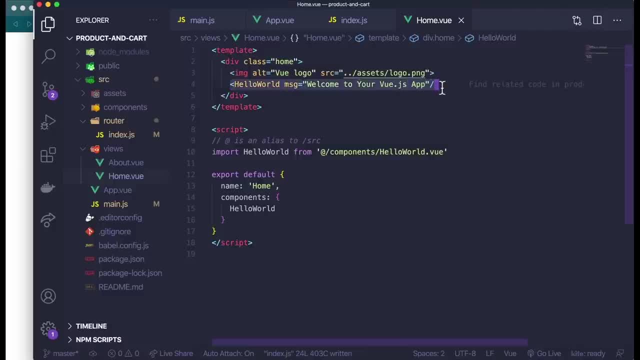 imports another component into itself. now this component is not in the views folder, it's in the components directory. now why is it in the components directory instead of just one folder for all view files? basically, in front end applications, files are usually split up between views or pages, so 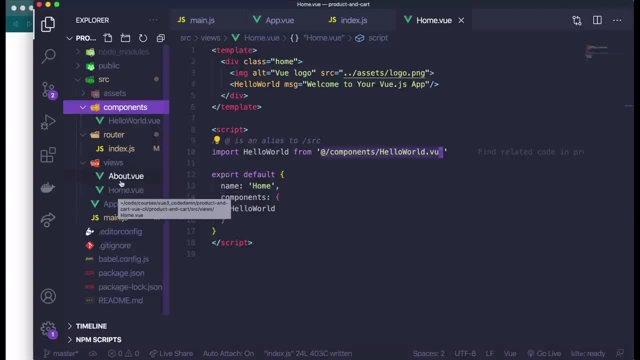 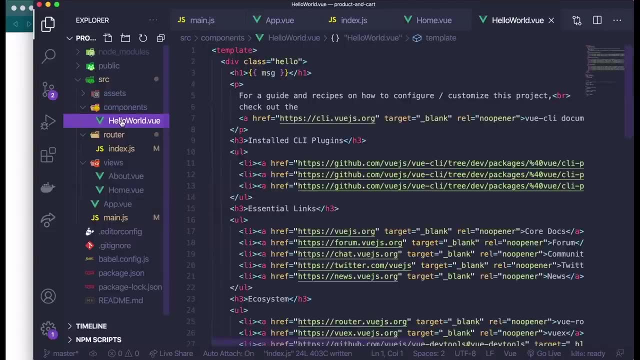 basically anything in this views folder will be connected to the router, so they will have their own routes. they'll be their own pages. anything in the components folder are things that are imported into other components. they're meant to be parts of pages or reusable components that you use throughout. 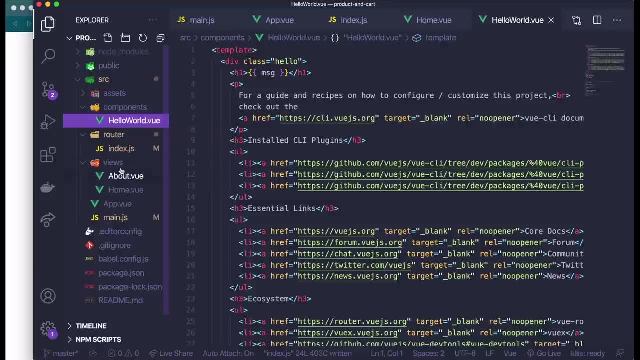 your application. basically anything in the views folder is connected to the router. and if it's not connected to the router and just imported into another component, then put it in the components folder and you'll see at the home route there's a view image at the top. 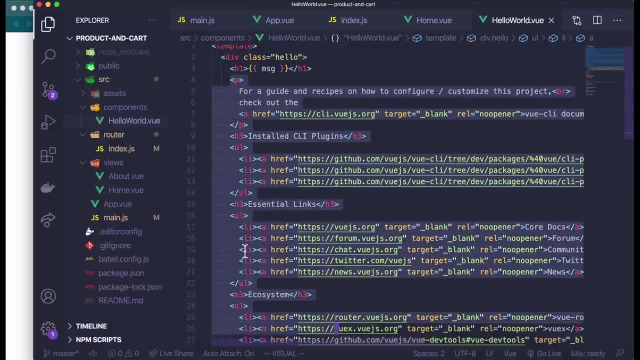 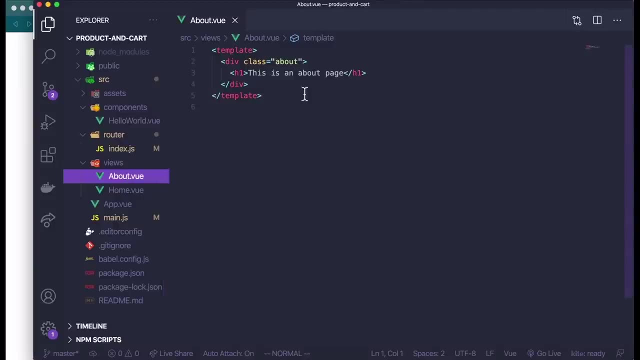 and then there are all of these links here and that's exactly what we see in the home route. now, if we go to the about page, it's not importing any other components or doing anything fancy. there's only this h1, so a header with that text. 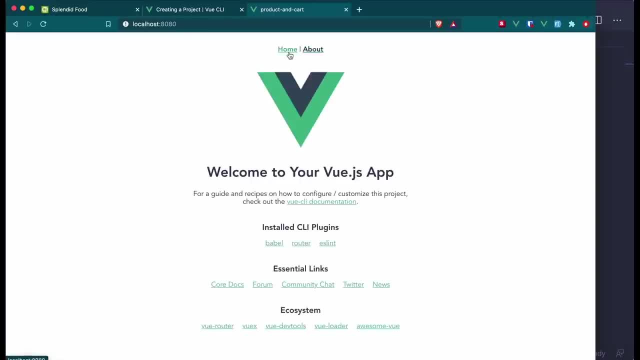 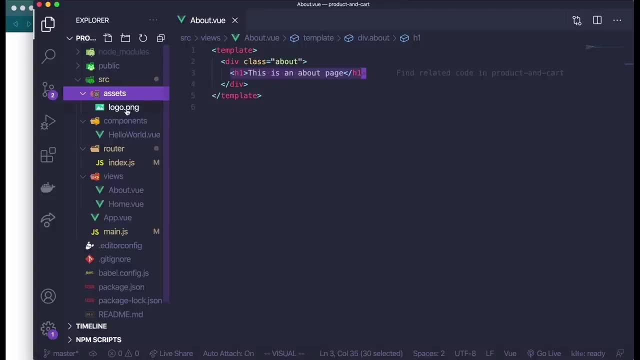 which is what we see when we go to the about page assets, of course, are a place for usually css images- anything like that, to live. sometimes you will see other folders created here in view projects, but these are the basic ones. the only one that we are going to add later is the. 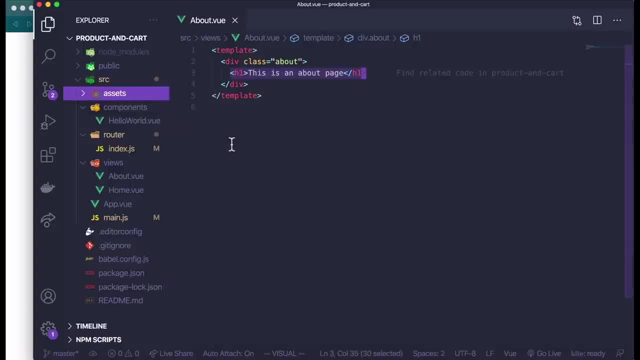 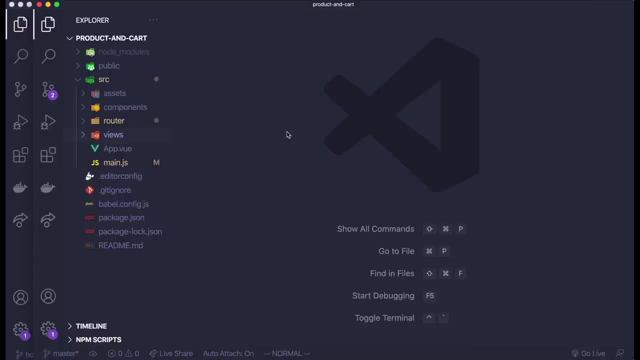 store folder, and we'll talk about that in a few videos. in the next video we are going to start transferring our content over from our old static application into our view application. let's start moving things over one by one, starting with the home page. I'm going to go. 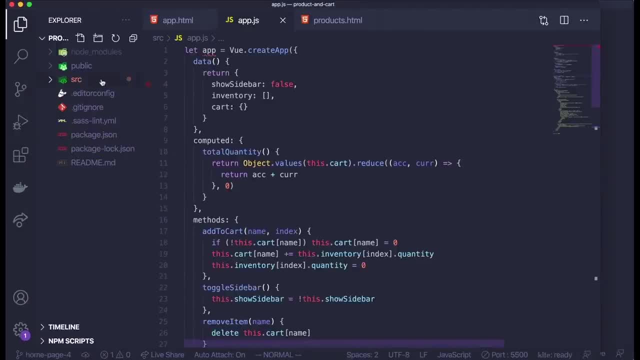 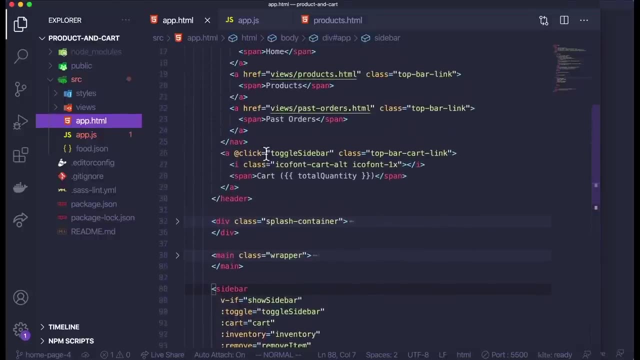 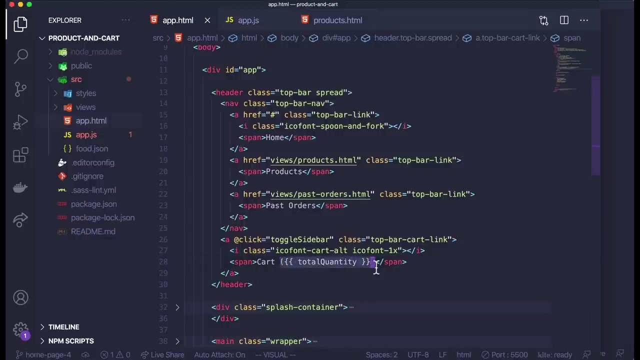 over to my original code here, go to source and then go into my apphtml here. the first thing that I need to grab is this header: now. I do have some javascript functionality in here, and I'll handle hooking that up in a minute, but let me just copy paste. 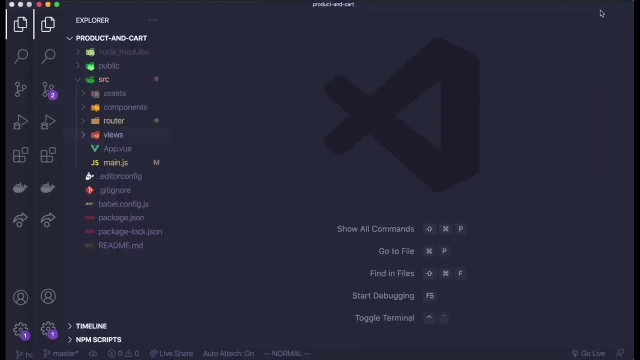 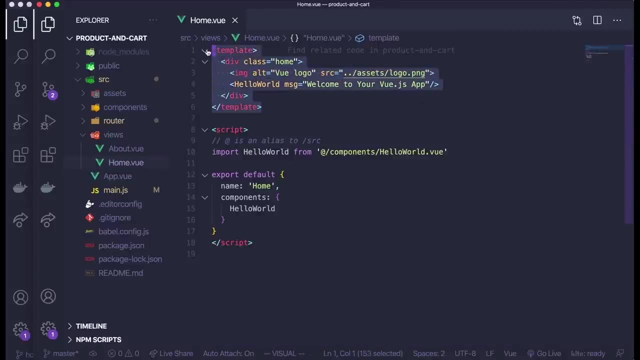 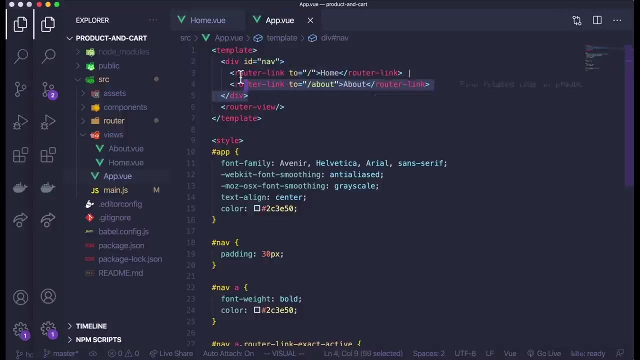 for right now and move this over to a new file. now I'm going to need it on this home page here, but since this header is actually my app-wide navigation, I am actually going to want to replace the navigation here so that I can use this and see this on any page. 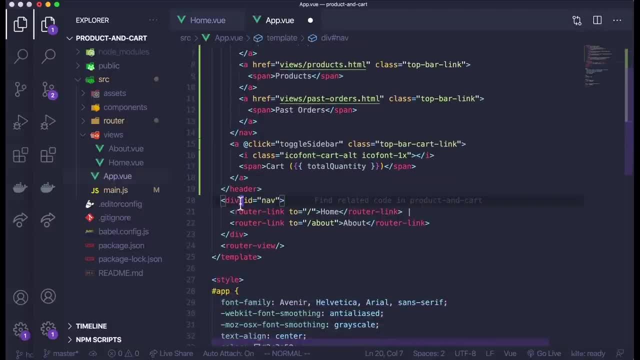 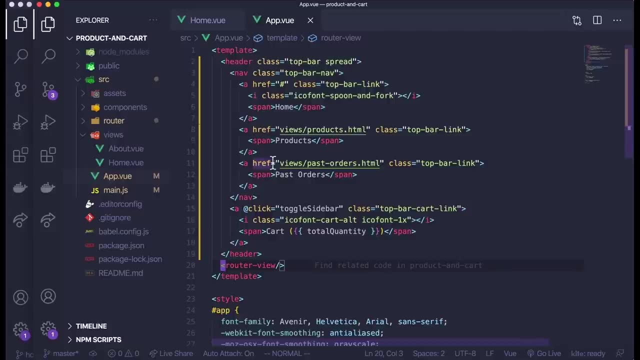 and for right now, I'm going to get rid of these. now there's a bit of clean up that I need to do here, because these anchors tags need to be changed to the view router router link tags, and now I need an actual route. so instead of pointing to, 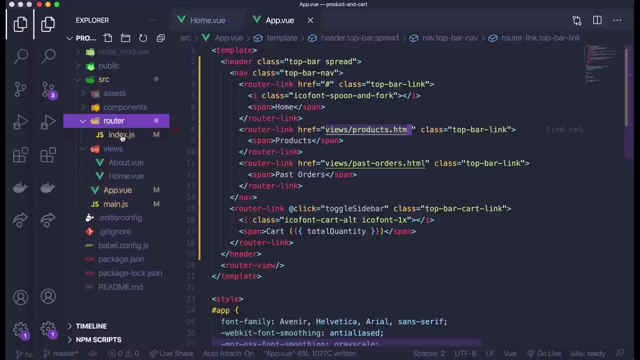 an html file. I am going to give it a route that will be in my router here, linked to a component. so I have this productshtml here. what I'm going to do is change that to slash products. of course, this can't be an href. this will be 2. 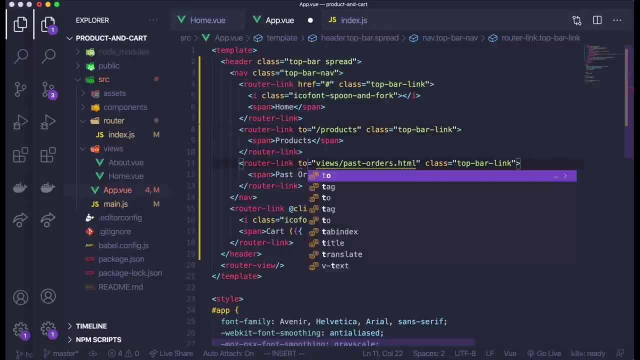 since that's expected by the router link. also, I need to change this and I can just call this route past orders. get rid of the html and, here as well, change this to 2, and this should just be a forward slash. I am not going to worry. 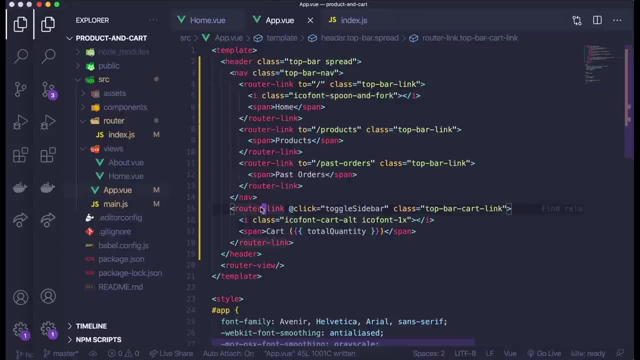 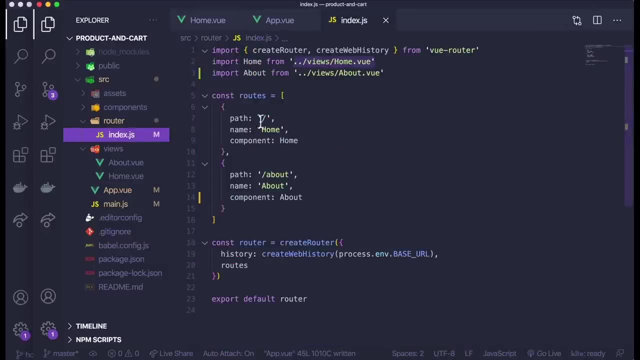 about this yet this last router link at the bottom. I'm going to just comment that out for right now and basically I need to create these three components that are linked to the routes. now I already have the home route here that is linked to the home component. 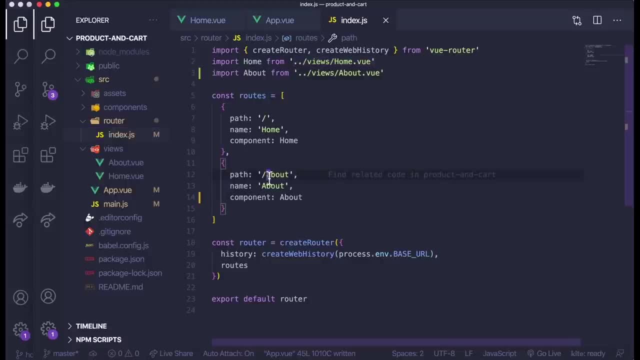 I'm actually going to get rid of about and I'm going to change this to products. I'm going to have to create a new component and now let me delete about from here and let me create a new file. I'll call this products view. now, this is. 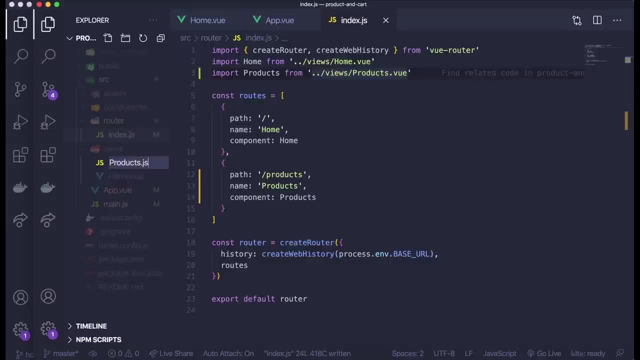 a little bit different. instead of calling this just a regular javascript file with the extension js, view has a custom file extension, which is view. all of these view files are parsed by the view and webpack setup that the view cli sets up for us. so, using these view files, 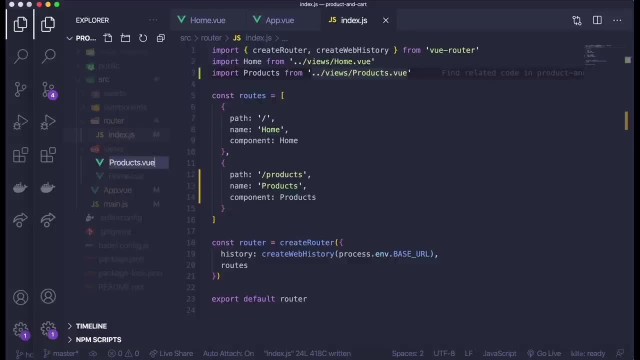 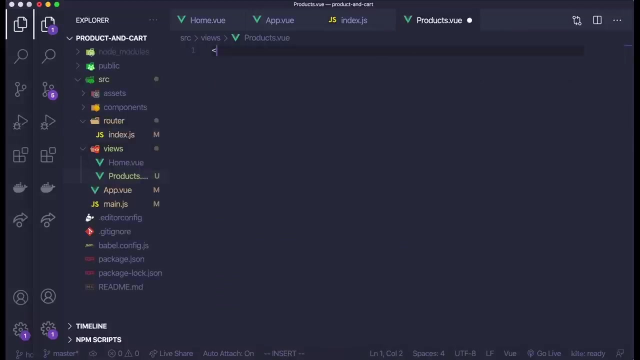 we can put our html template, our javascript and even our css all in the same file that gets parsed and all put together and bundled by the tools that view cli sets up for us. now I have a new file. I'm going to create a template in here. 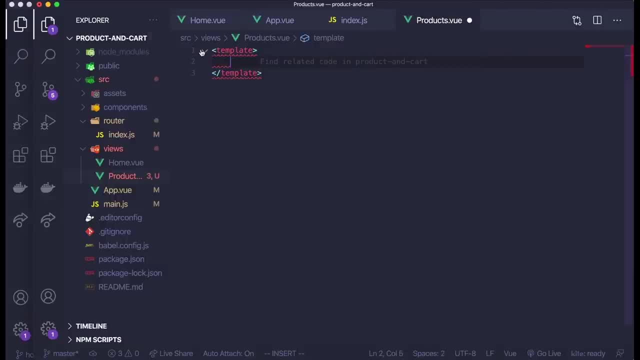 and I have four spaces. I'm going to switch to using two spaces for tab spacing and I'm just going to put h1 products for right now. alright, before we get too far, let's see how this looks. and we do have a products page and a home page. 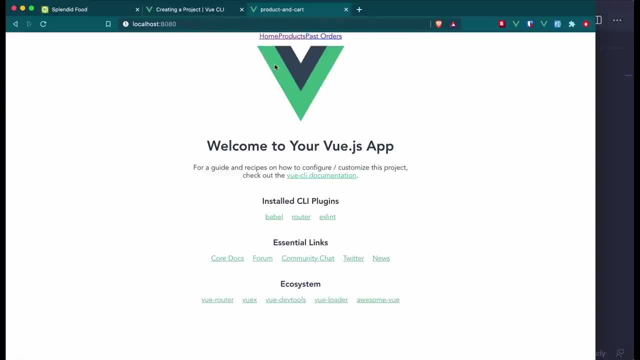 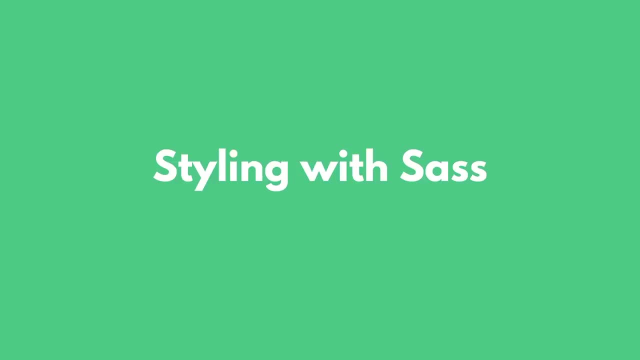 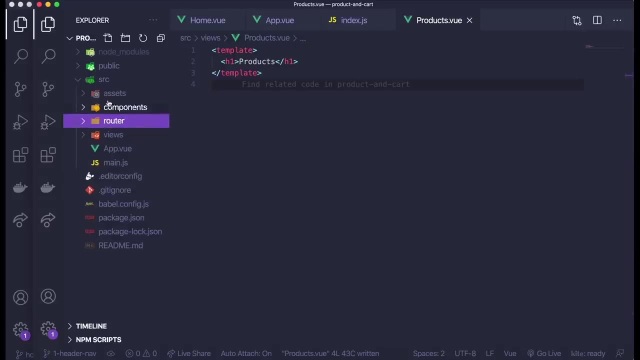 now, but of course, this is completely unstyled. let's pause here and start to bring over some of the styles in the next video. let's start to move our styles over. now. our styles are going to live inside of this assets folder and I can go ahead and create a folder. 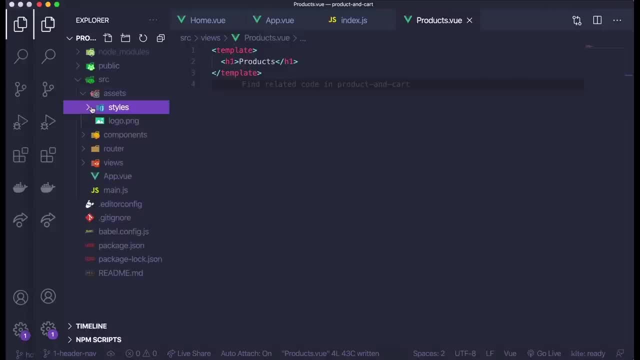 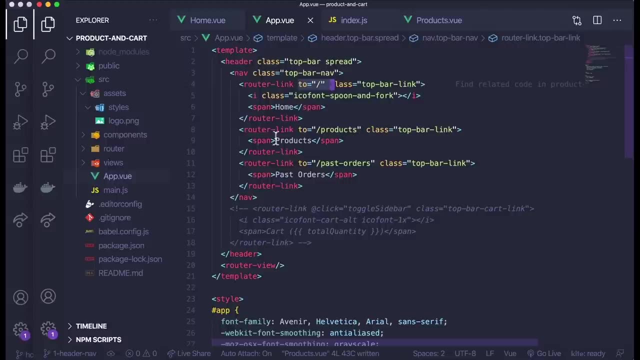 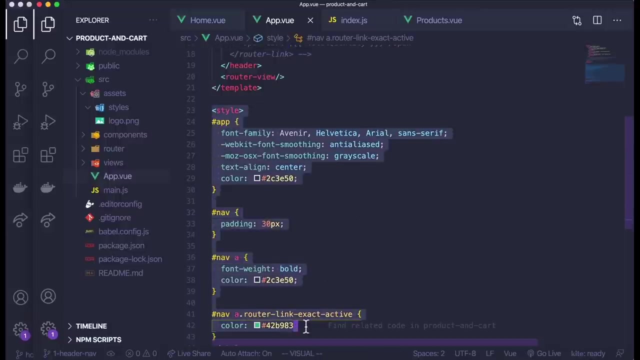 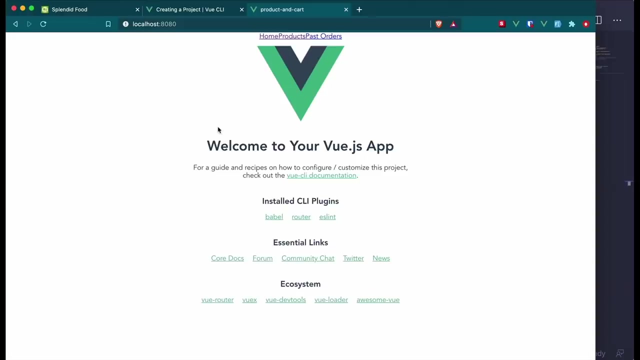 inside of there called styles. now how do I use styles in my project? if you come to this app component here, you will notice that there is a style tag at the bottom of the component and these are what is providing custom styles for the application. if I look in my browser, 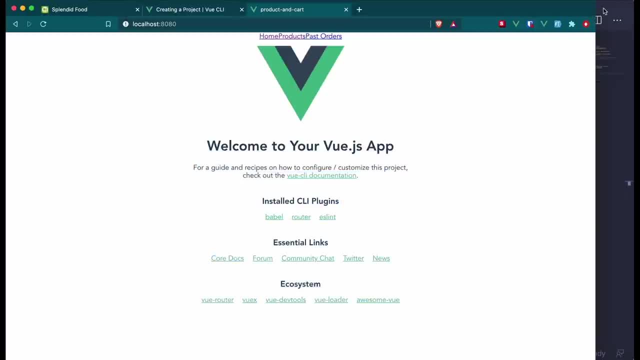 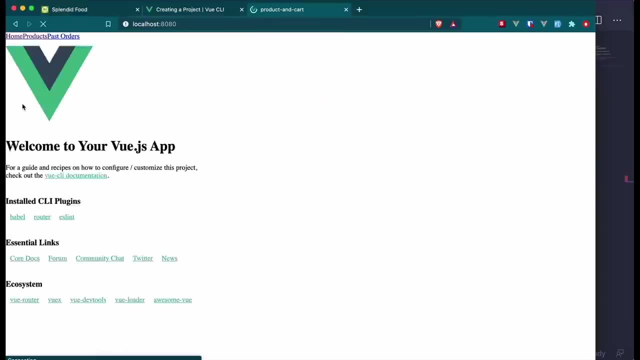 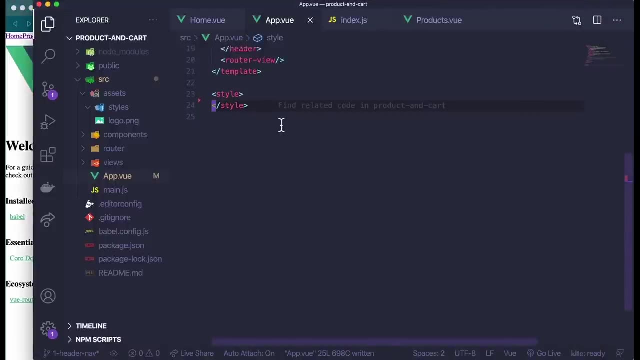 this is what is styling and centering the elements. if I get rid of these styles, this is what it looks like without any of those custom styles. in any view component, you can add styles directly inside of that component. so if I wanted to do something like change all, 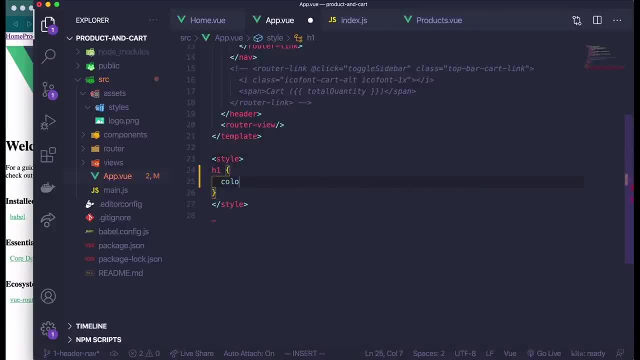 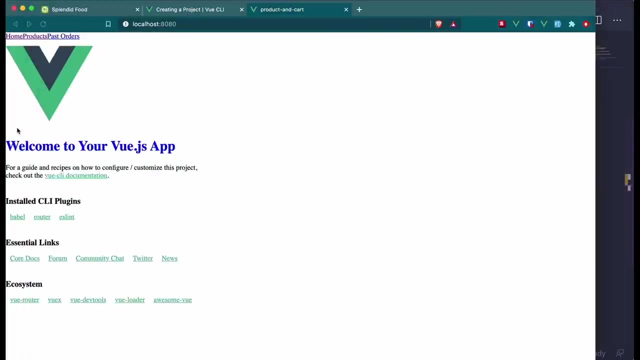 h1 tags to the color of blue and you will notice. this is just plain CSS here that you can write inside of these view files. now, if I go here, you can see that this is an h1 tag and it is changed to being blue also on the products tag. 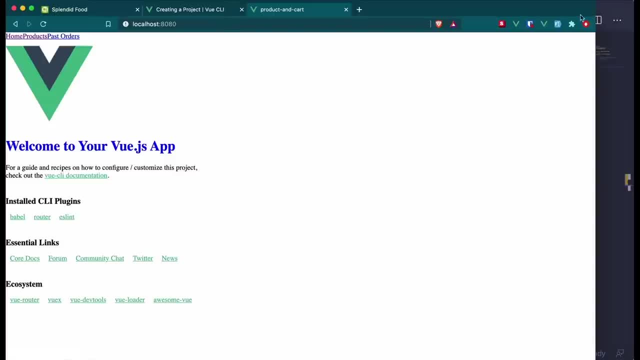 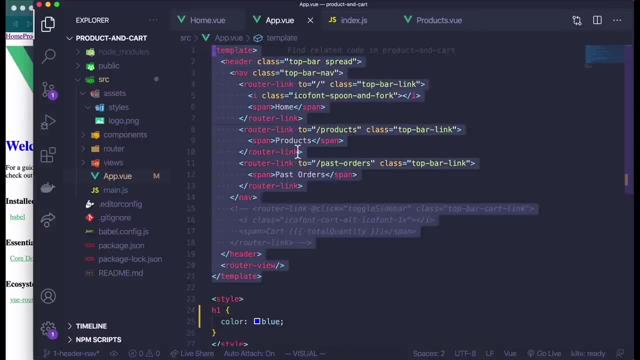 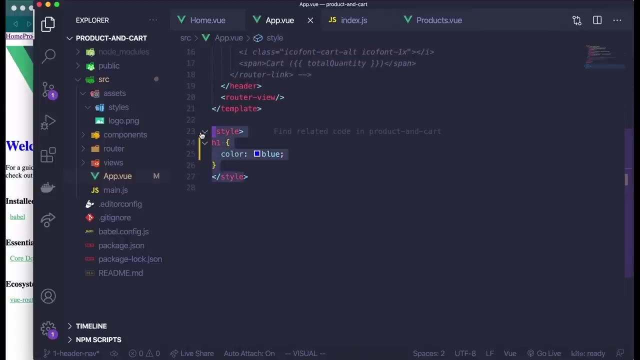 that is blue as well, because that is another h1. now, if I look at this, though, those h1 elements are nowhere to be found in this component. those are actually in other components, but by default the style tag globally affects anything in the application. so if I put a style tag here, 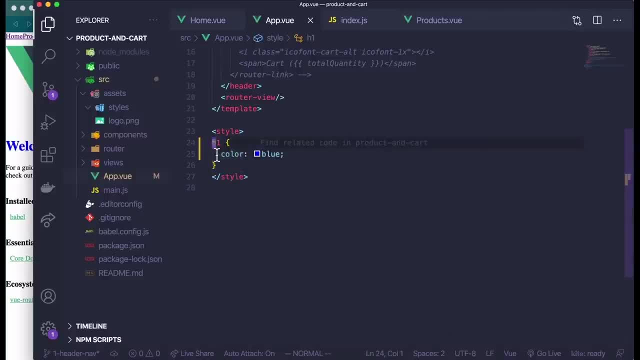 even though it is in the appview file. anywhere in my application that has an h1 tag can be affected by this. now, this is generally not good practice, because if you want to globally change a style, you should put that in a separate style sheet, so in some other css file. 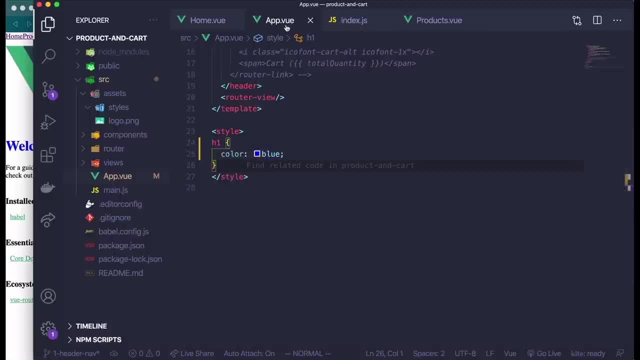 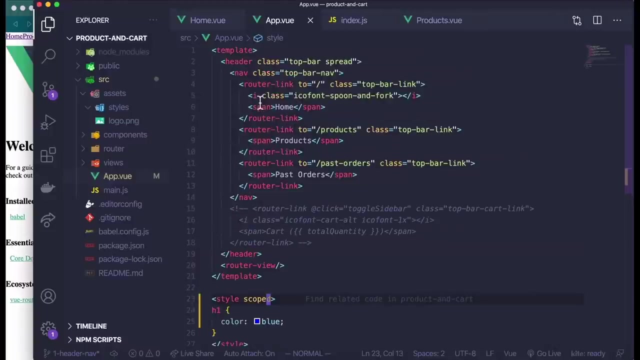 here, if I am putting styles inside of my appview file generally, what I intend to do is only let it affect the appview file, so it won't change styles in any other component. it will only affect whatever is in my template in this file and that is why I use the scope keyword. 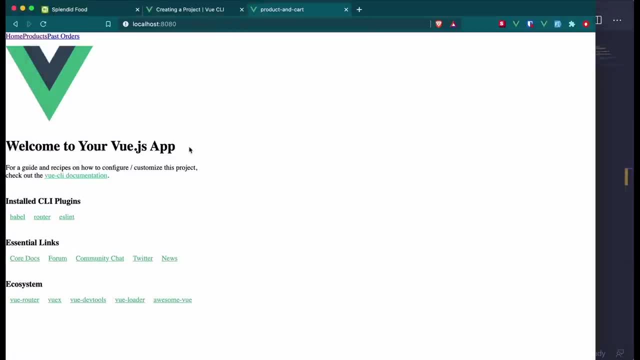 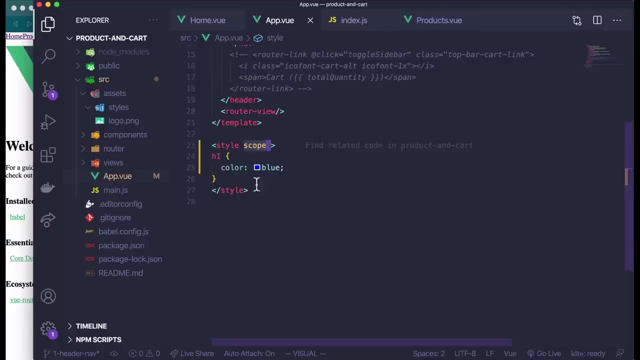 here now, now that I have added the scope keyword, so you can see that the text changed back to black, because now I have scoped this, it is only affecting styles within this view component, not in other components throughout the application. now, if I wanted to add an external style sheet, 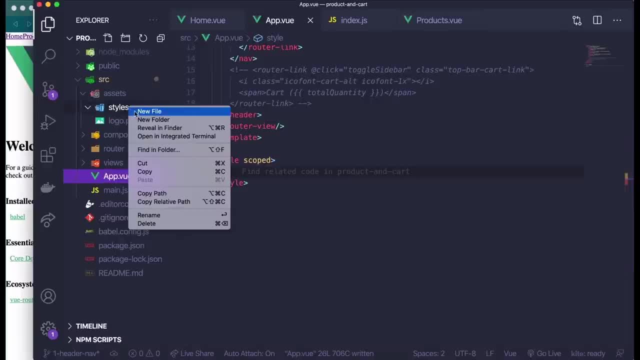 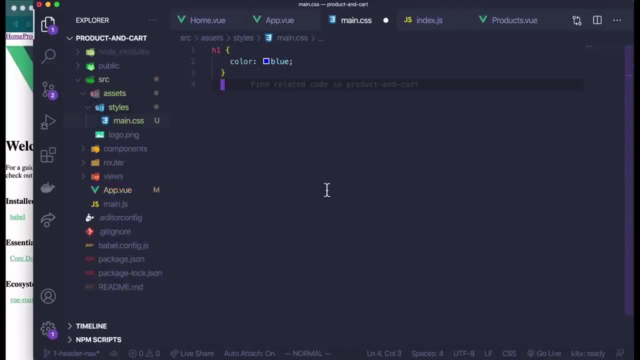 let me just go ahead and create a temporary one here. I will call this maincss and let me paste in my last style and I will change the color. this will not affect my application yet, because I have to import the css file now instead of importing this into one of my html files. 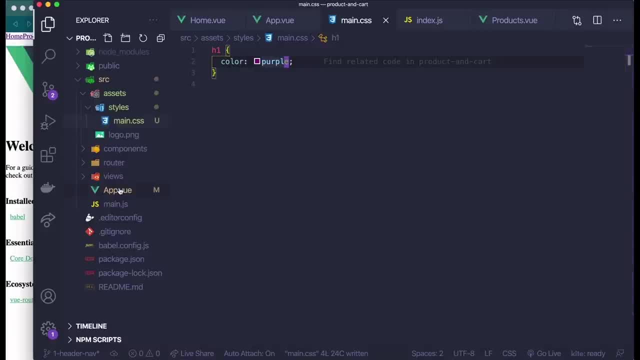 what view does is allow me to import it directly into my javascript. so generally, that would be this mainjs file. what I can do is import from assets styles and then that maincss and the view. cli set up webpack for me in such a way that I can import styles. 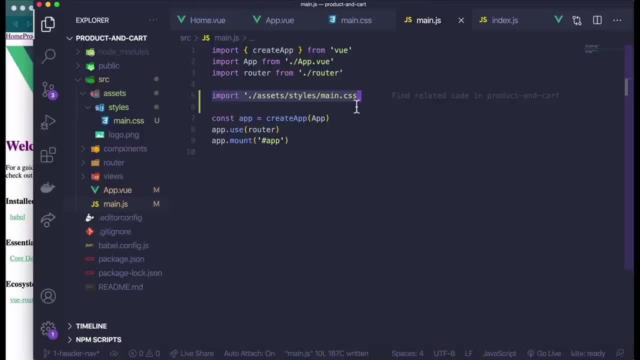 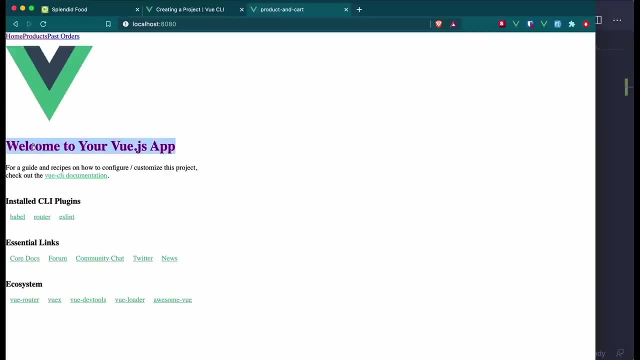 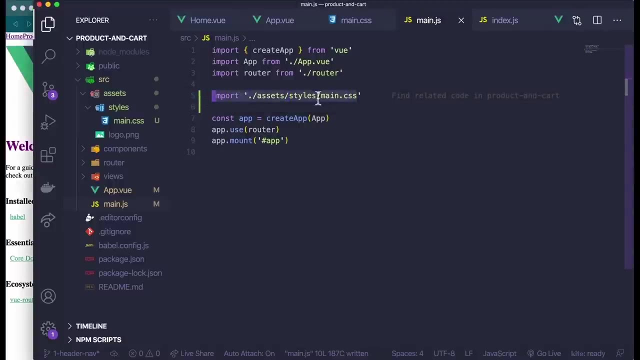 directly into my javascript and it is all handled by the tooling. so now if I go back to my browser it is a little bit darker, but you can tell that this is purple now because I am importing it globally into my project from this maincss file. those are the 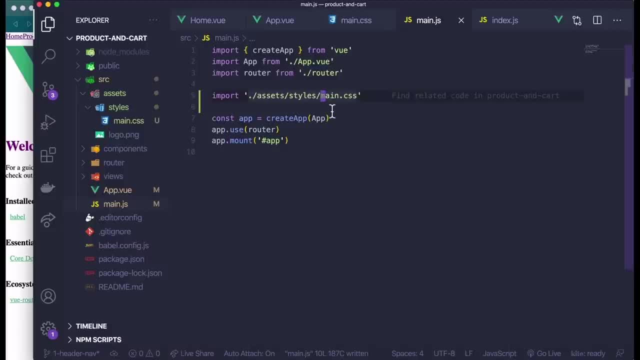 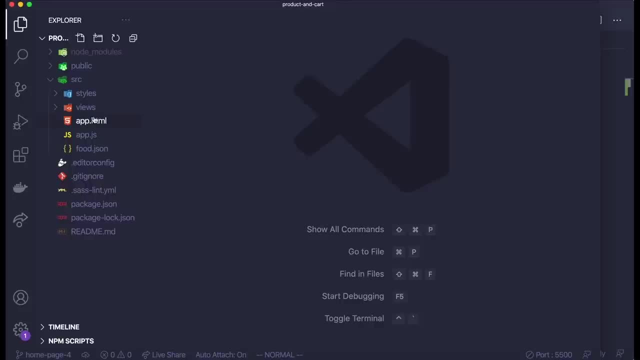 basics of how you import styles into an application. now, if I come back to my original static application with our html files that we were using, if I come to styles here, you can see that these aren't just css files. they are sas files for the most part. 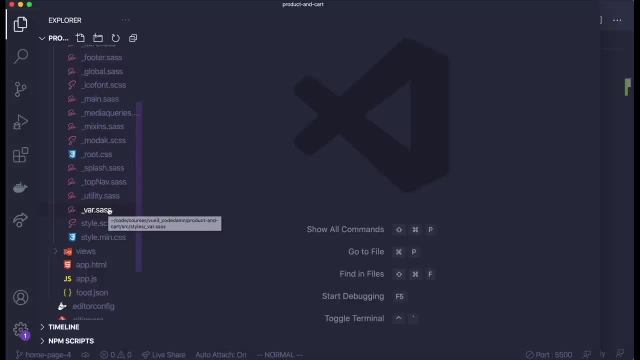 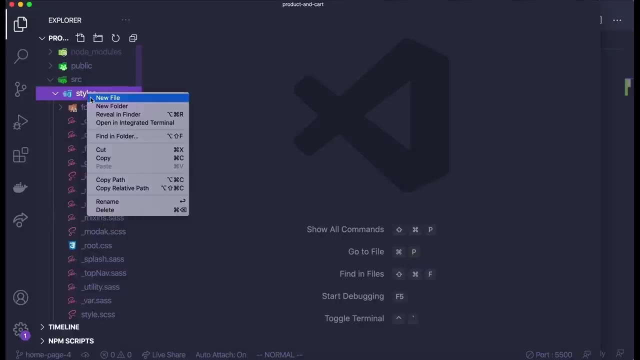 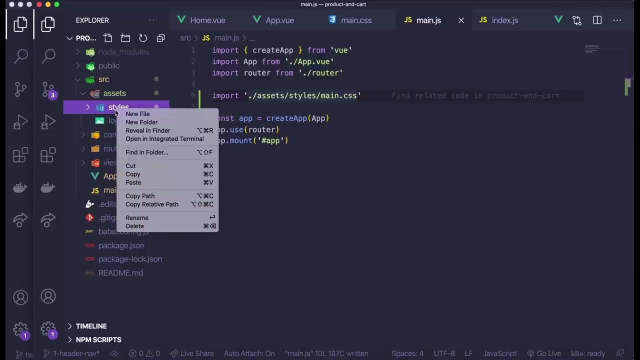 so how do I get these into my project if they aren't standard css files? so view also has built in ways of handling this. let me copy these styles and I am going to delete this styles folder here and I am going to paste. so I pasted in. 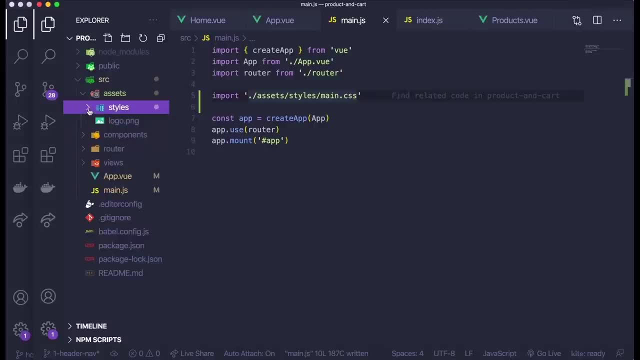 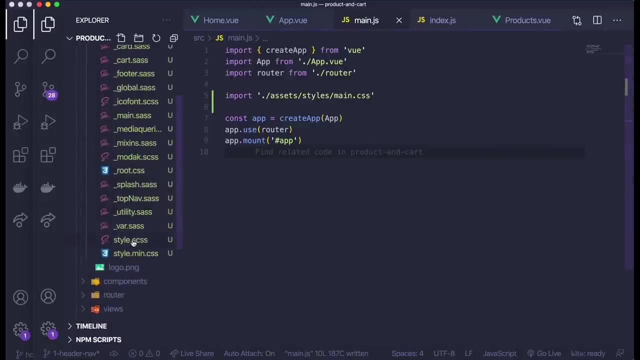 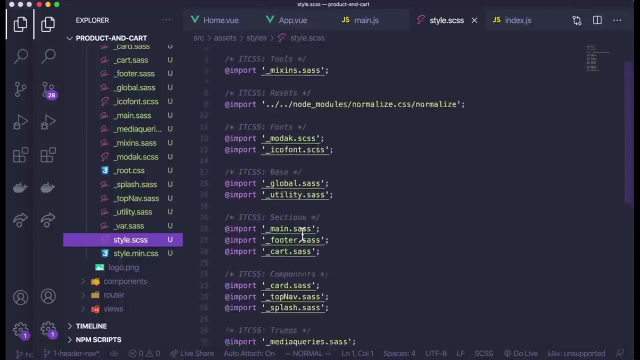 this styles folder from my other project. and now if I look in this folder, there is one file called stylescss, which is a sas file, and this imports all of the rest of the files here, all of my other sas files. now it is this file. 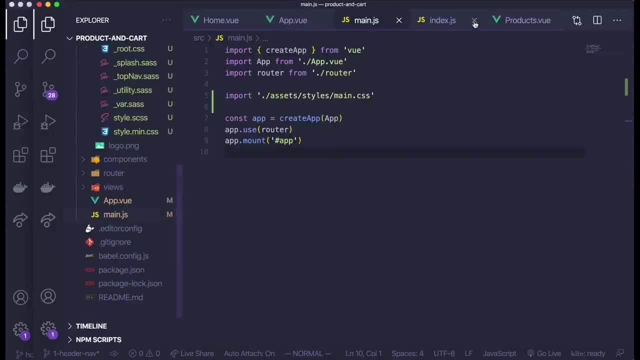 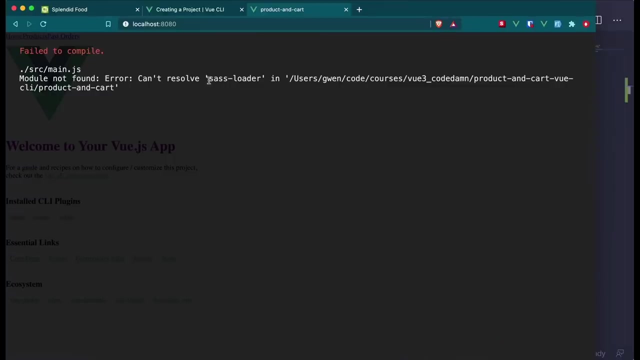 that I really want to import into my project to get all of my styles. I am going to comment this out and now I will import that sas file directly from assets styles: stylescss, stylescss. I will save that and now you can see that it is giving me an error. 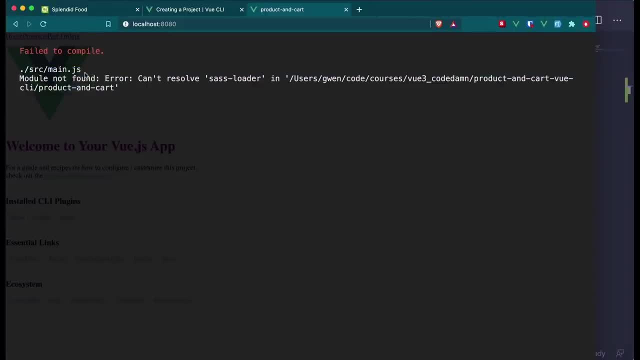 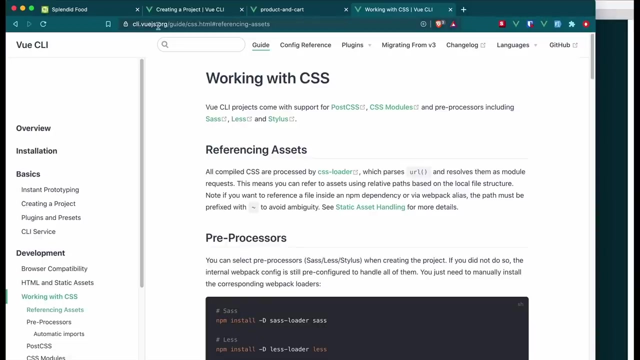 saying: can't resolve sasloader. so it is trying to load those sas files but since they aren't regular css, we have to add another module to be able to import those files. and that is like it says: sasloader. if we look in the view cli, 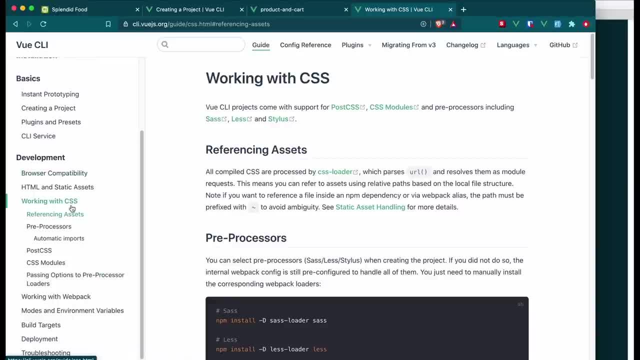 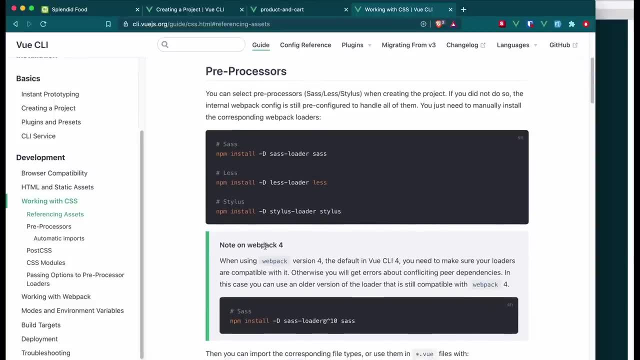 documentation and go to working with css under development. we can see that it has this section on preprocessors. now, as it mentions, we can select our preprocessor when we are creating the project, meaning when we ran that first view- create project name- that command would take us through. 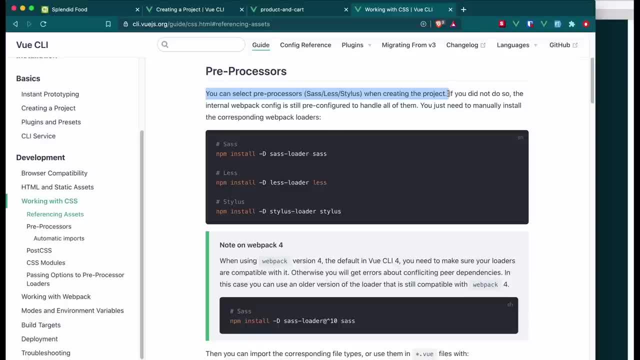 setting up sas automatically. now, since we did not choose sas back then when we were setting it up. there are ways of adding these packages, which you can do through this command: npm install, and then installing the sasloader and also the sas package. now, if I scroll down a little bit, 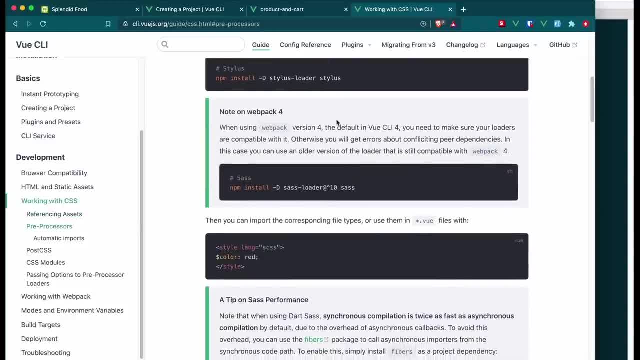 it is giving me this note about webpack 4, which is what I am using in view cli, for I have to make sure I have a compatible version of these loaders, so I am going to go ahead and grab this npm install command where I can install sasloader. 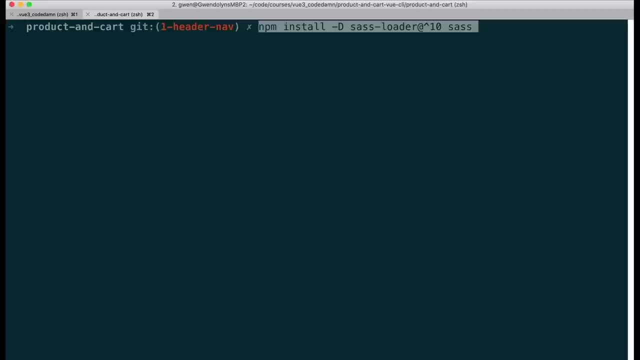 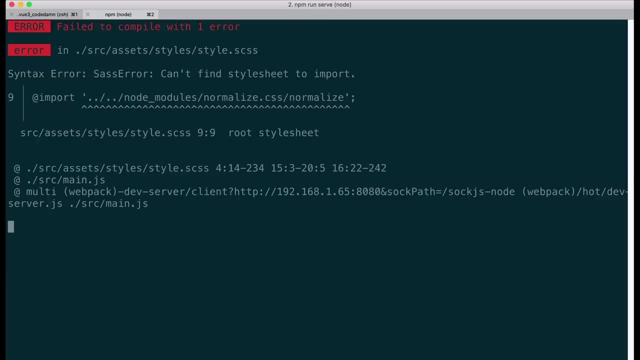 add a specific version and also sas, and it installed those packages for me. now I should be able to run my server once again at npm run serve. now it is complaining that I don't have one specific css module because I haven't installed it in my node modules. 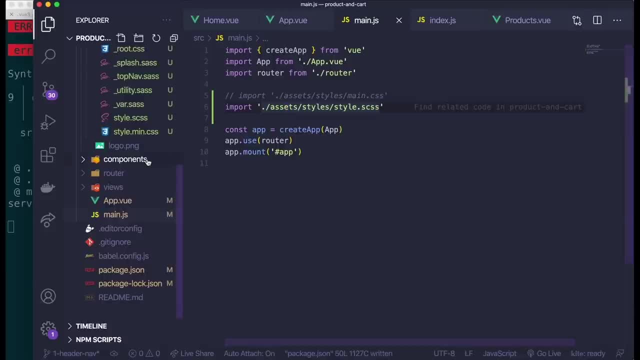 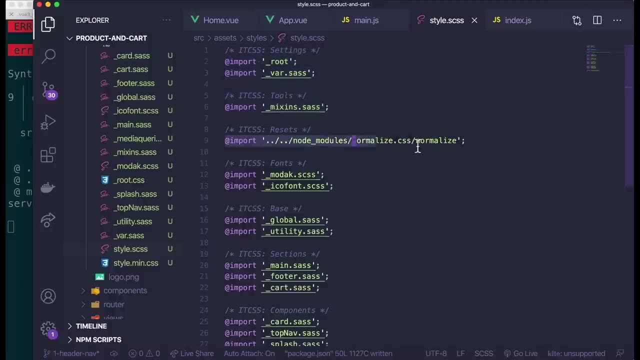 but that is actually a good sign, because that means that it is reading through the rest of my file here. it is reading through this, getting to this line and saying, hey, I can't find that file. so I am just going to comment that out for right now. 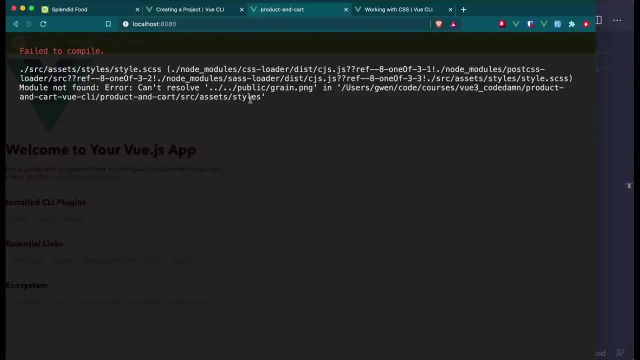 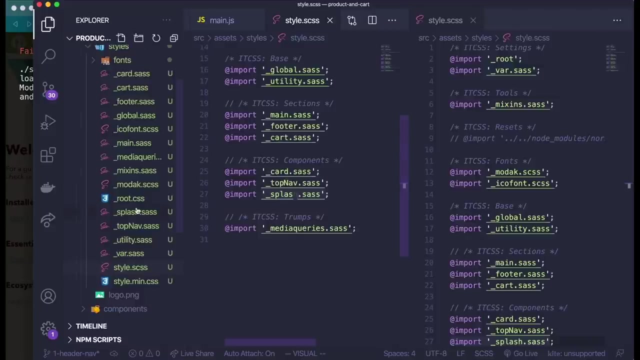 and now we have one more error here, and that is it is looking for images that it can't find right now. let's go ahead and resolve those. and they are coming from this file. so if I go to splash dot sas now, you will notice the syntax. 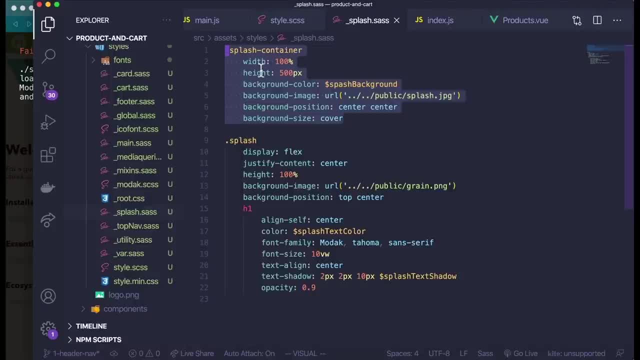 is a little bit different here. you can basically think of it as just an indented syntax without curly braces. either way, you can see that the attributes are the same here. so I have background image. it is looking for this image and again there is a background image. 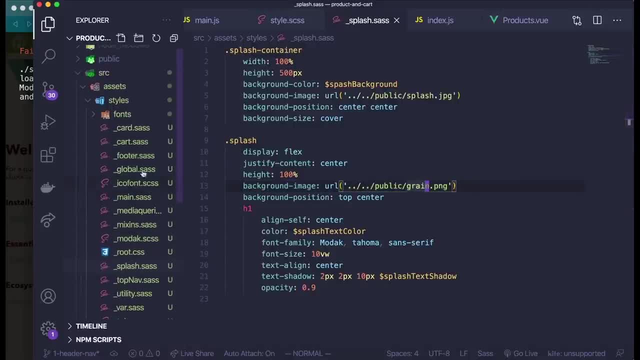 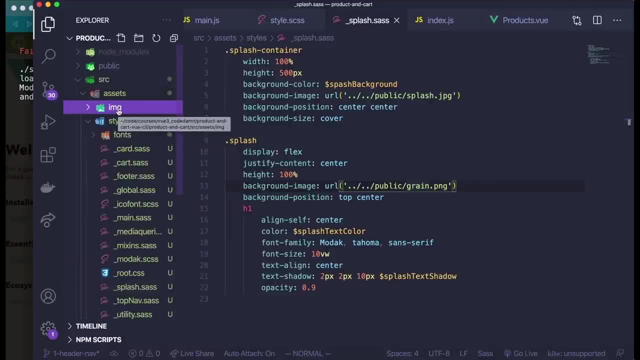 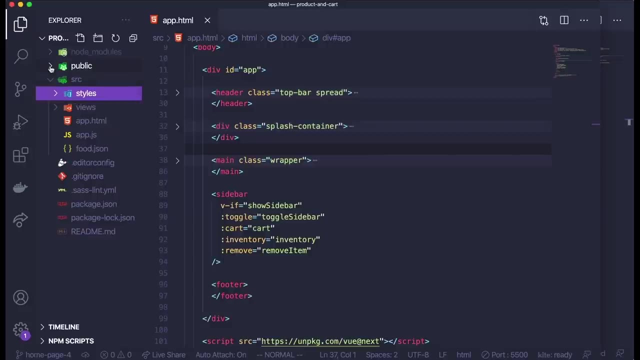 which is looking for this grain image. so I am going to create an images folder here, an img folder, and put those two images inside of the img folder and then update this path. so back in my old application- they were in my public directory- I have grain and splash. 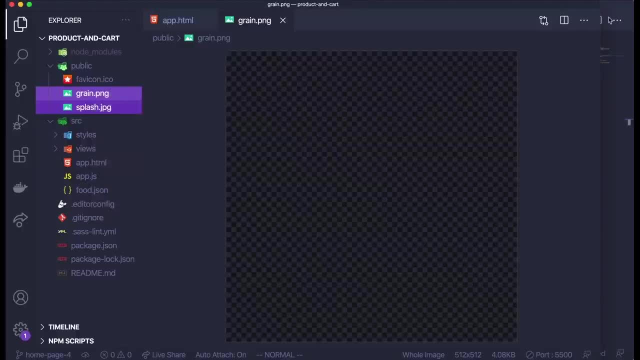 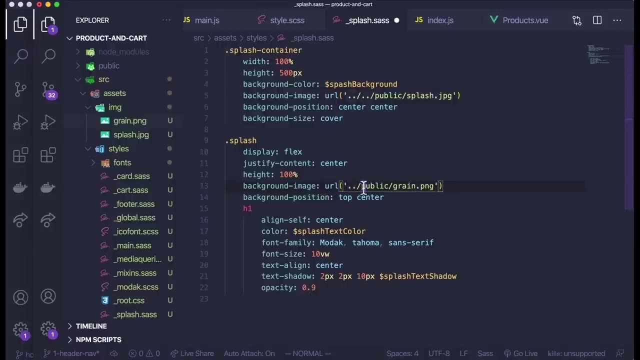 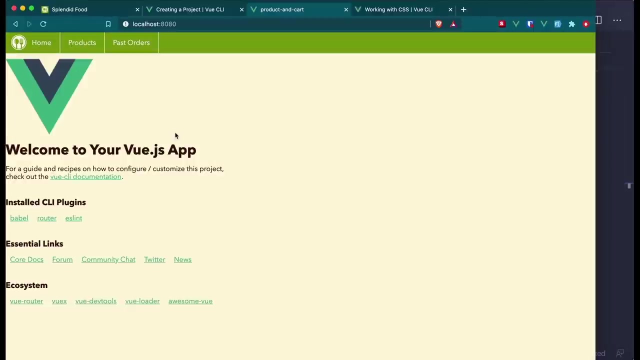 I am going to copy those and paste them here, and I should be able to reference the relative path here. close this file and you can see I have the styles for my main application in here. now let me do one more thing and get rid of this boilerplate. 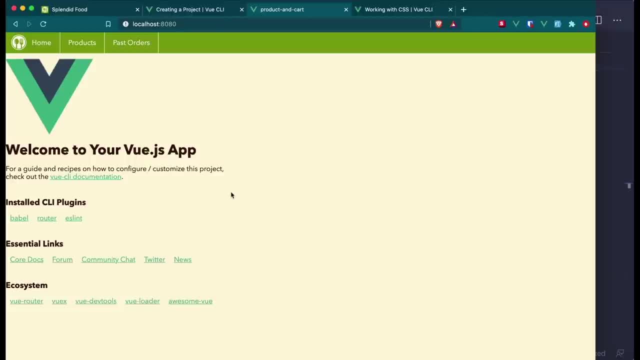 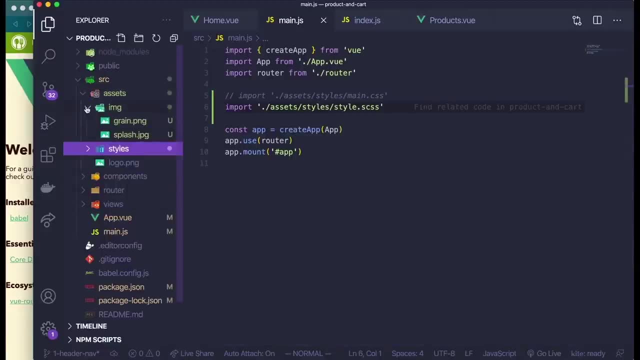 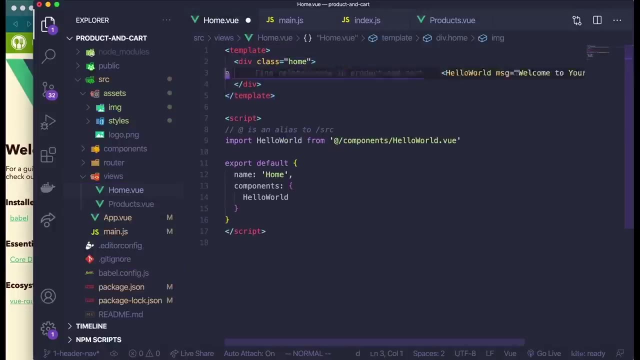 here so I can be ready to put my own content there. so let me get out of here and go to source, slash, views and home. I will get rid of this image. I will also get rid of that component. I am just going to put home here for now. 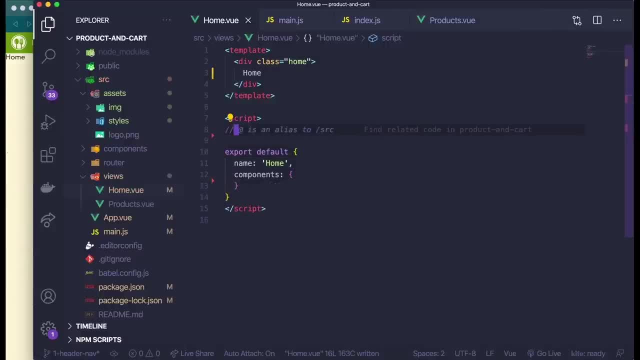 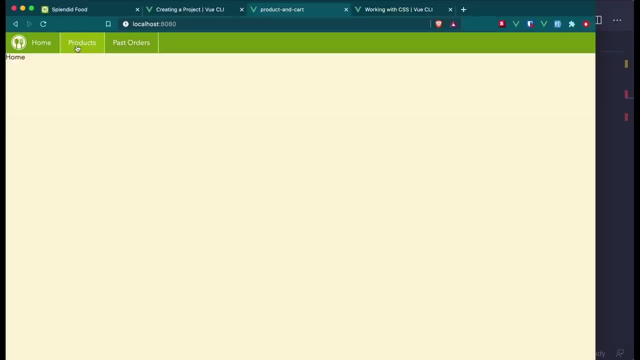 and get rid of the component everywhere. now, if I go back to this page, you can see that it is ready to add my own custom content, and I can see the products page it navigates as well. one more thing I will go ahead and do is add a past orders. 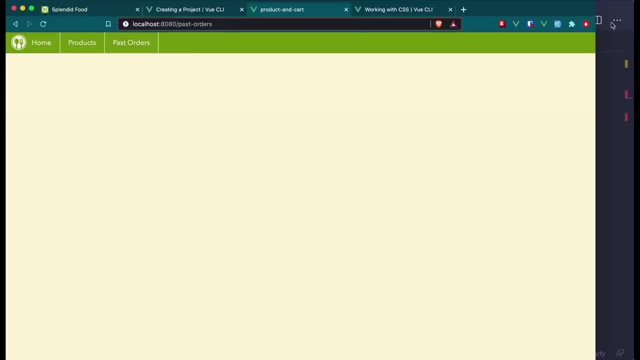 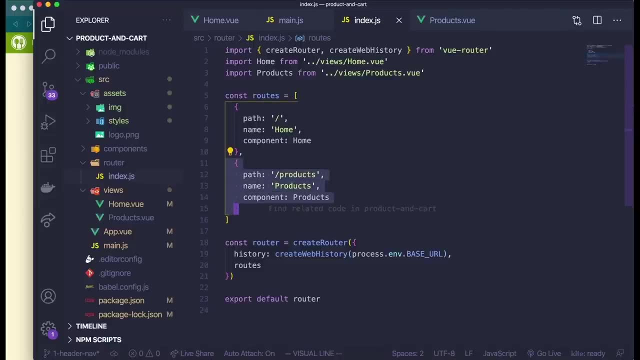 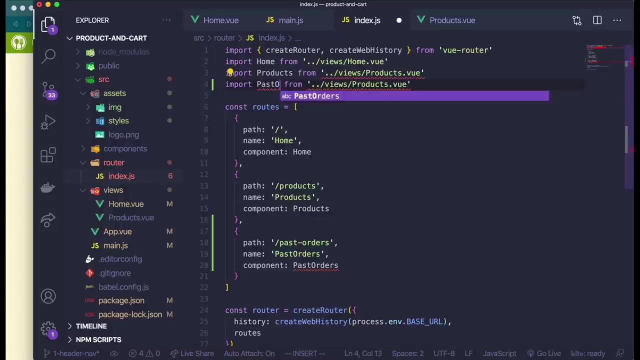 page to the router at this route, and all I will have to do is basically copy the products route. this will be past orders. I can call it past orders, past orders. now I need to create this component. it is connected to my router, so I am going to. 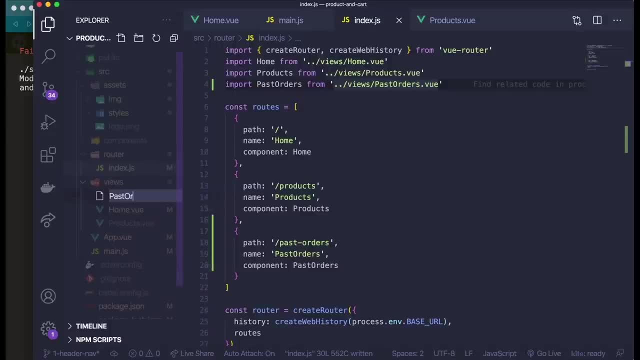 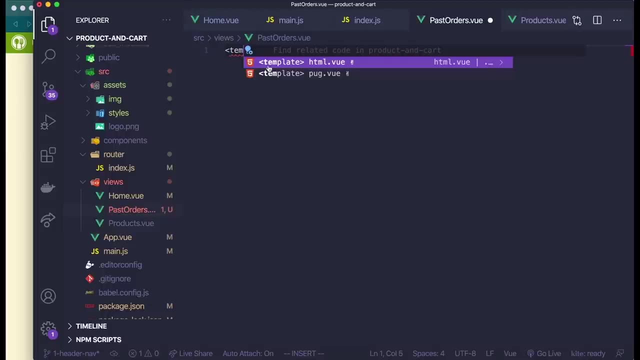 create it in the views folder, call it past orders dot view, and I have a shortcut snippet here. I will show you how to use this in a second. but if I click enter, it just created the template tag for me and I am going to put in each one in here. 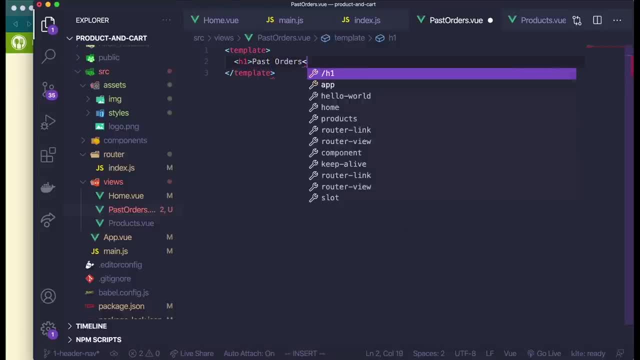 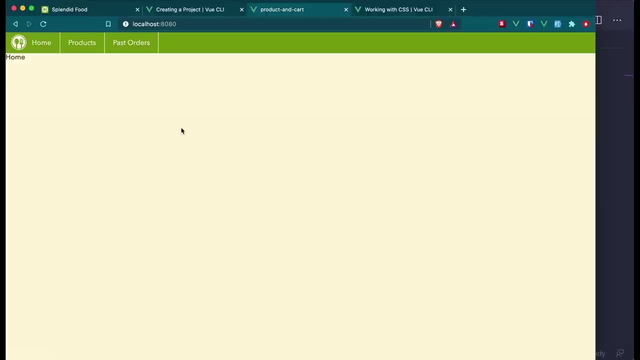 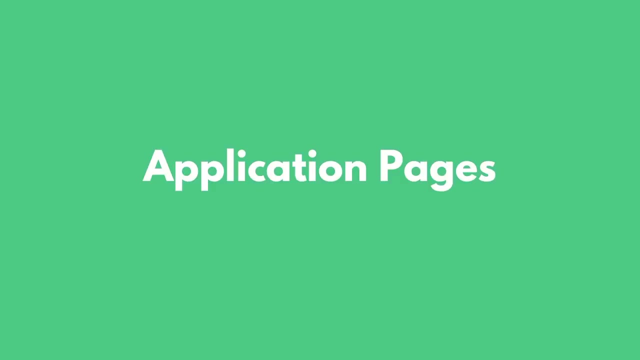 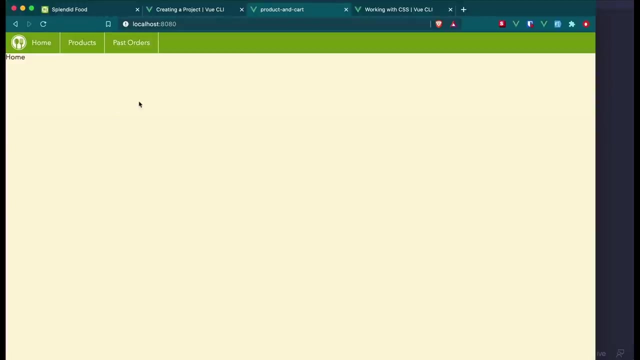 it says past orders and now I have this page working, so all three pages are there. in the next video, I will be putting content on these pages and then hooking them up to javascript to be functional. now let's work on putting actual content on this home page. 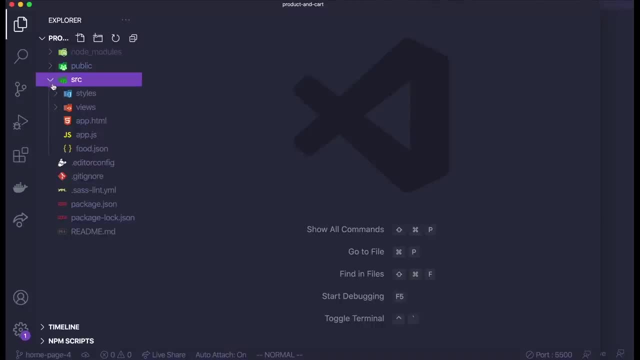 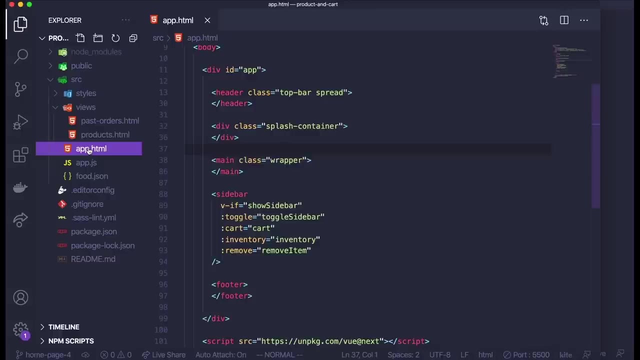 I am in the original application. now let me go to source. inside of views. here I have my pages. actually, the main page is still in app dot html, so I am going to go ahead and grab these two container elements here, the div and the main container. copy those. 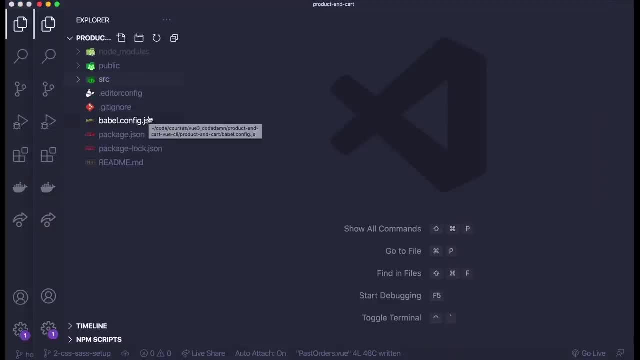 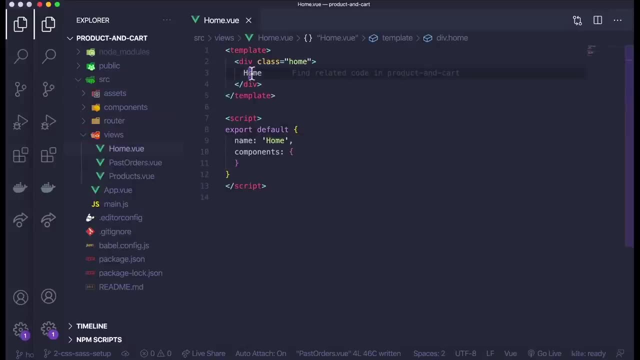 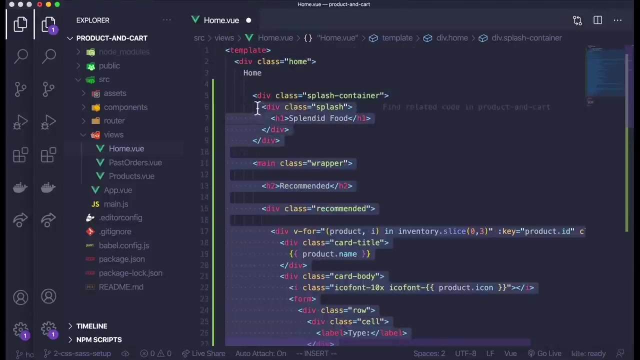 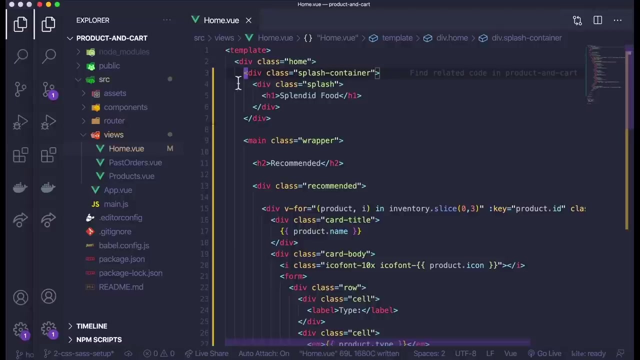 go over to my new code, my view cli project, and here I can come to my home page and just paste that in here. alright, now I will take this just the indentation, get rid of that old word. and now I have my splash container and also my main container. 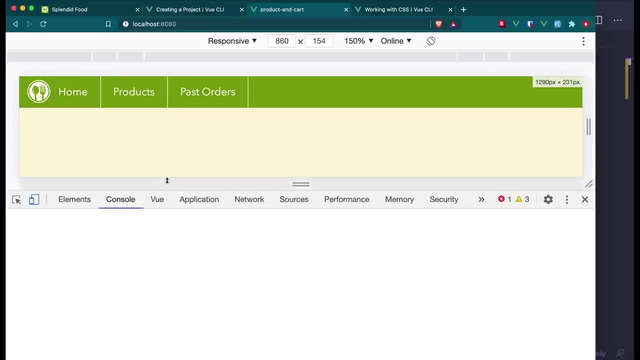 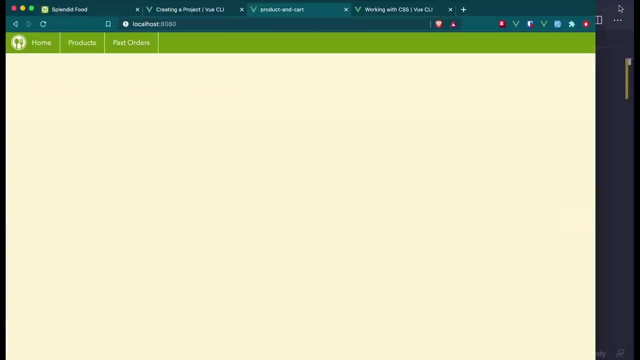 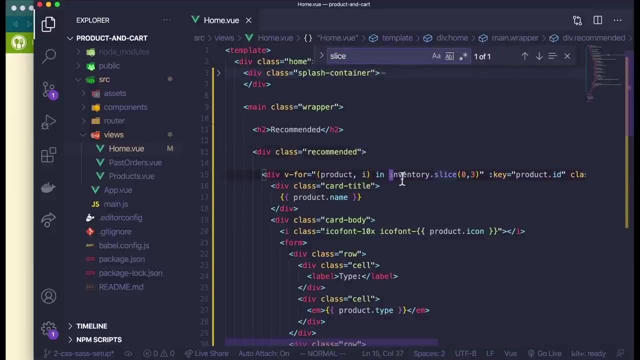 and nothing is showing up on the page. so if I look in the dev tools it says cannot read property slice of undefined and I can search for where that is being used and inventory dot slice. so of course it is broken right now because I don't have any. 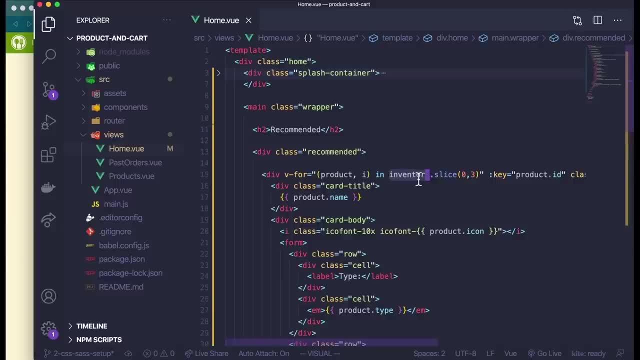 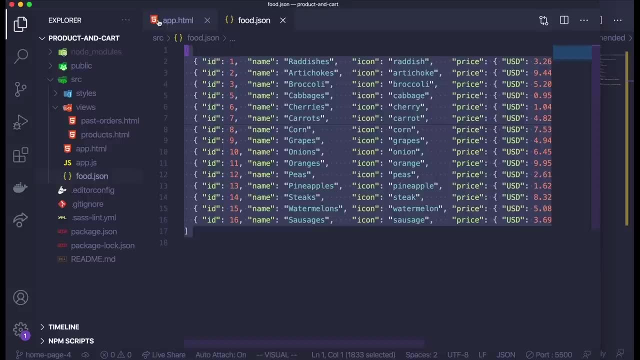 inventory. so let me grab that from my original code base. if I go here I can see in food dot json. this file is really where I have my inventory items. so I am going to copy this file. copy, go over here and inside of source. I am just going to paste that. 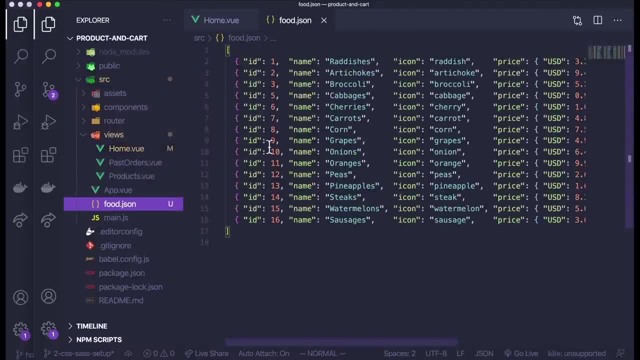 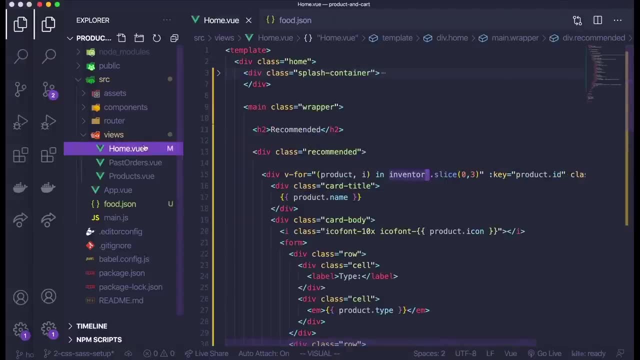 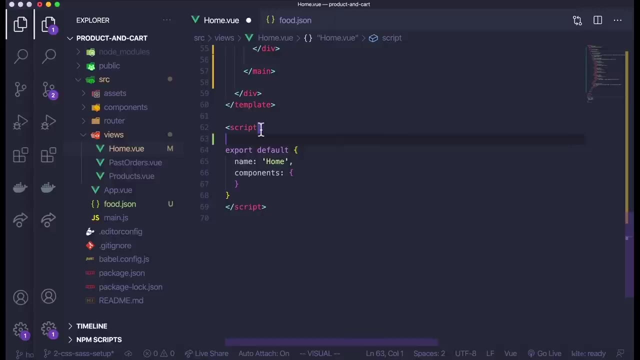 file and now I need to import this into my view js. so if I want this right now in my home component, I need to import it at the bottom here. so let me import my data. so import food from. go up a directory food dot json. let's set it equal to. 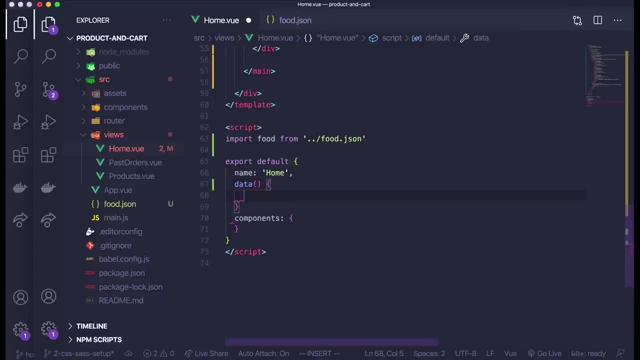 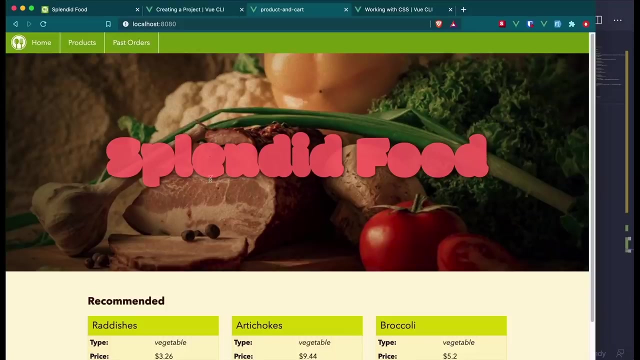 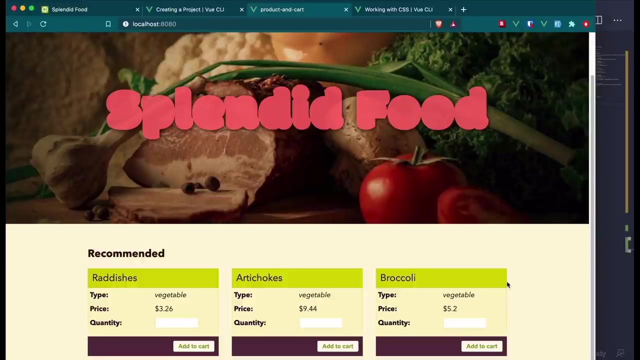 a data variable, so data, and then I can return and then I can set inventory equal to food. ok, let's try this out. and now we see the banner displays just fine, and we can see our recommended product section at the bottom, which is already displaying real data. 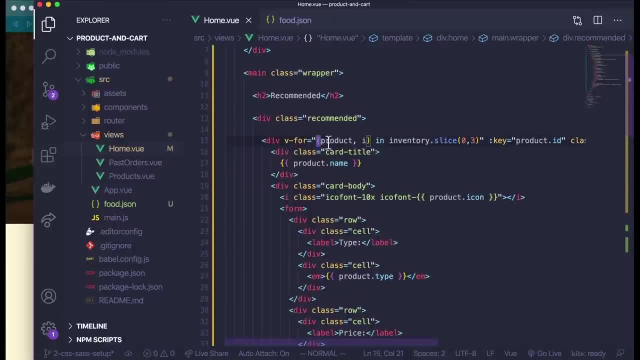 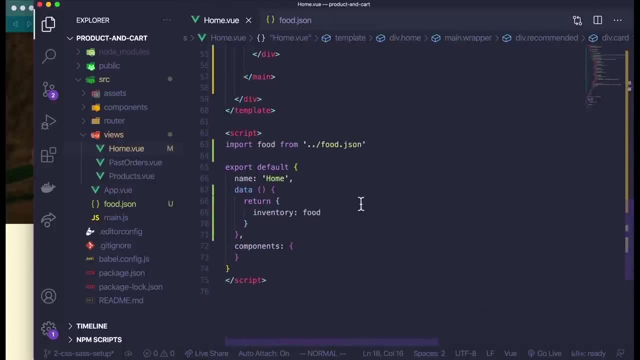 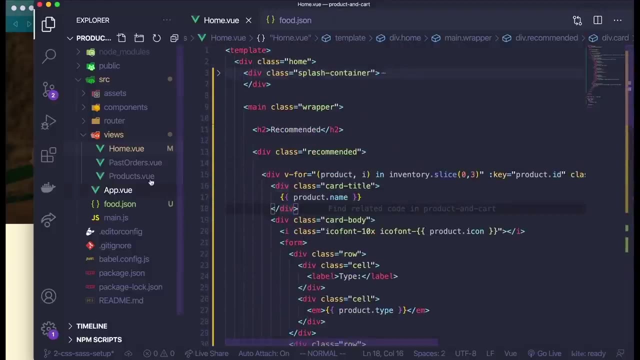 because we already set this up and this is basically the same logic as with the other app, but we've only rewritten this in a component structure. now let's pull in the other pages really quick. so we have past orders and also products. let's go to products. 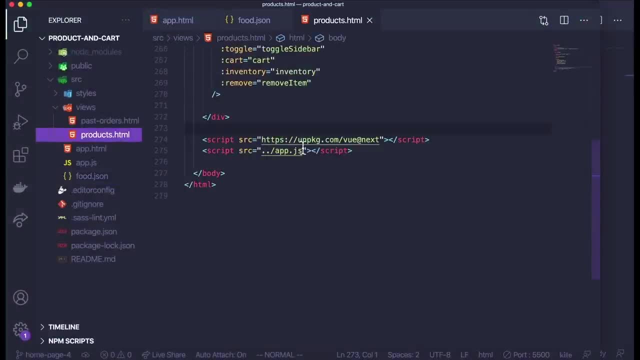 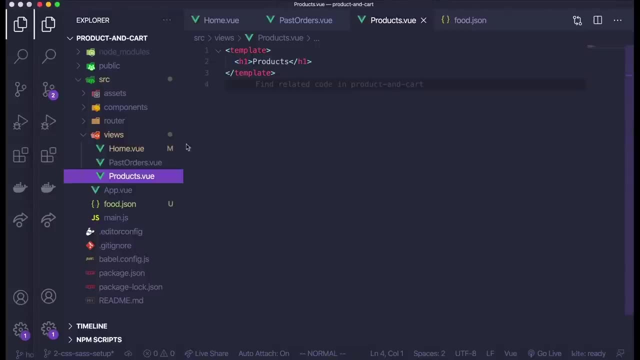 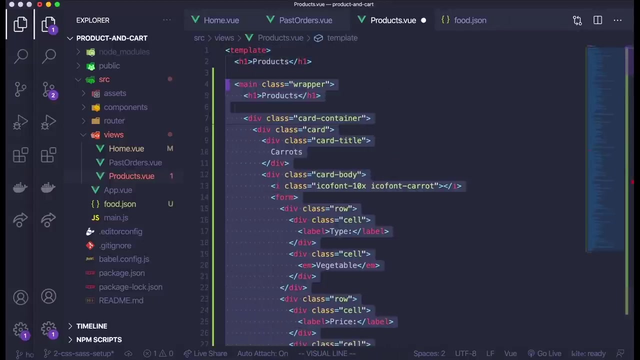 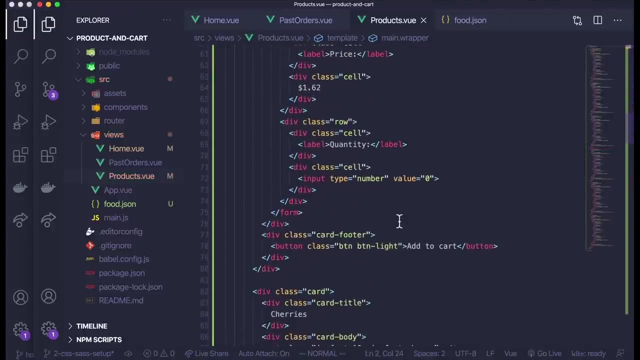 and if I go to the products page, I can just grab this main section here, go back over to my code and then paste that in. now this page should work as it is because if I look at all of the code here, we never made that dynamic, so that's something that we will have to. 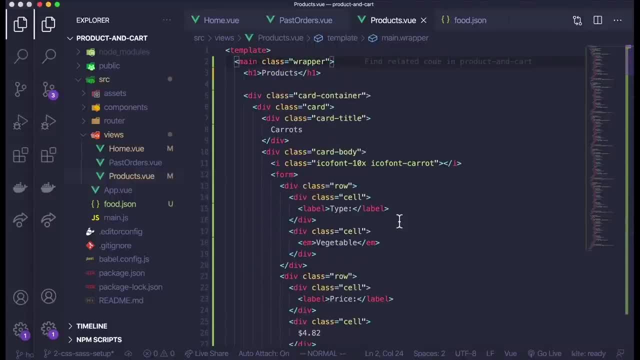 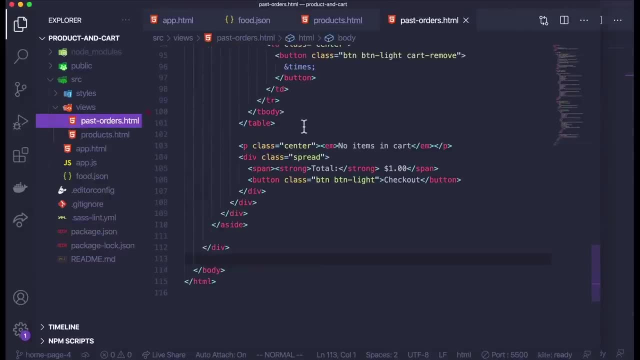 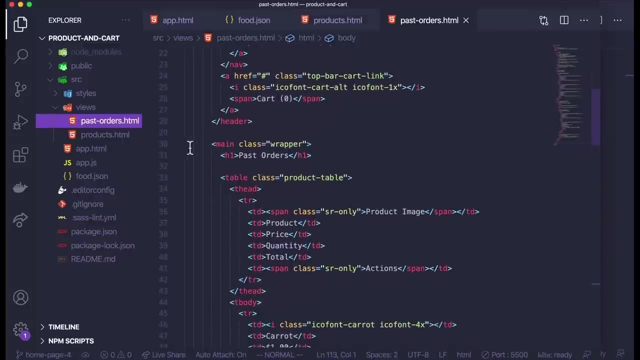 change later. but this is all hard coded. let me grab the past orders page real quick and then we can take a look at it in the browser. so if I go to past orders, let me fold this main section. I'm gonna copy this and go over here to my code. 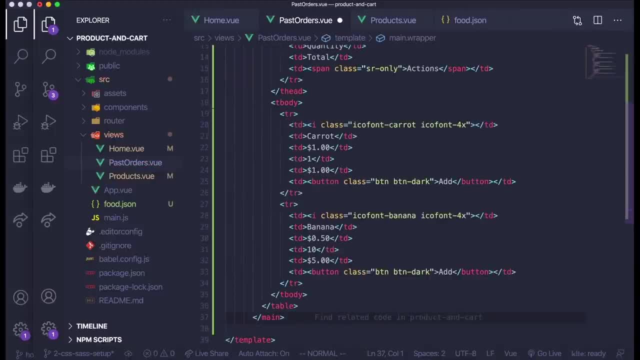 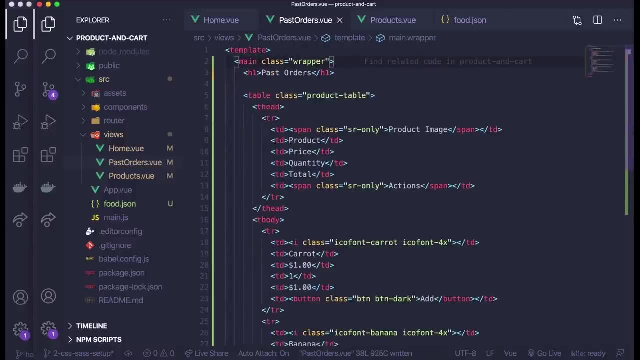 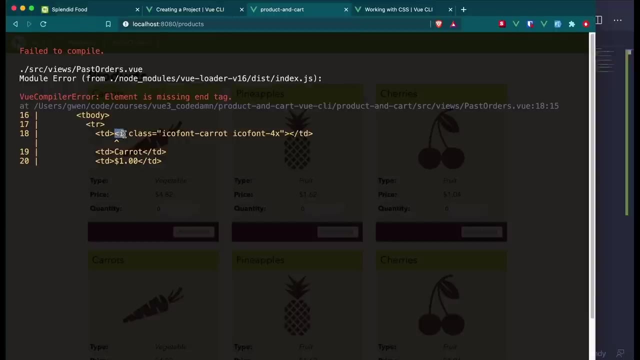 paste that. and now let's take a look at these pages. ok, so our past orders page has an error and it's complaining that this I tag, which was used for icons generally, that it doesn't have a closing tag, meaning it's not explicitly self closing, and 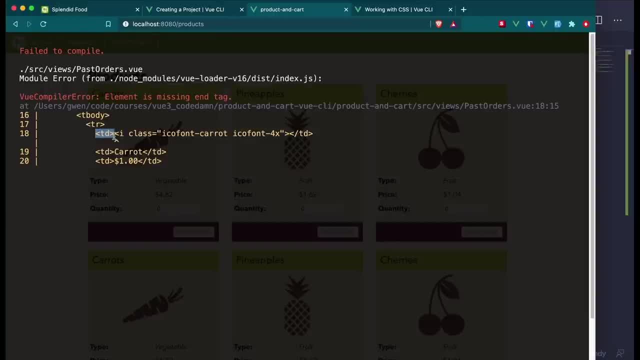 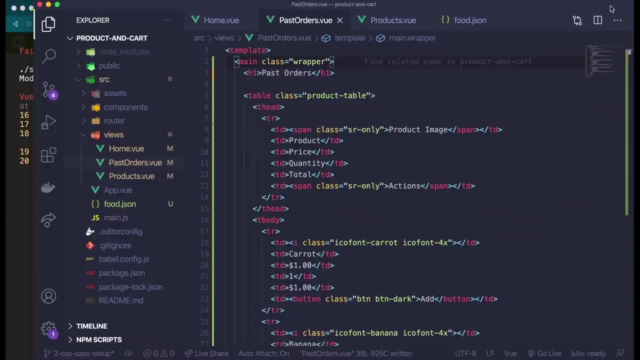 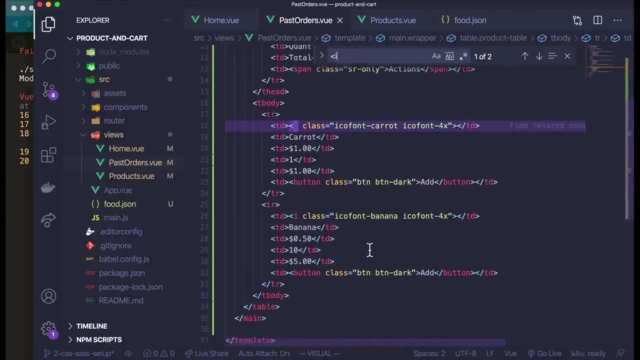 I'm not explicitly closing it either, like this td tag here has a closing td tag there, so I will have to fix that. that's just how view templates work. so let me search for I and seems like it's only in two places, which is good. all I have to do to. 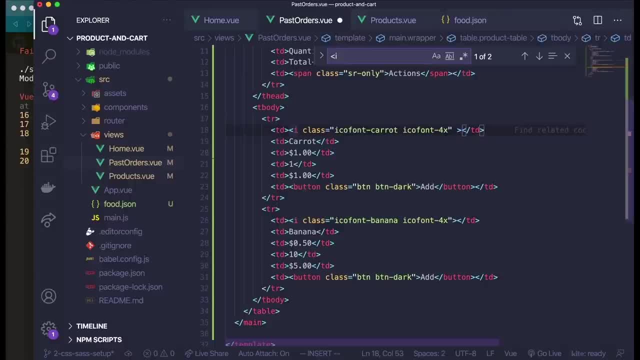 fix. that is, either I could do a closing tag- things like img and I- and certain tags don't really have closing tags, so all I have to do is make them self closing, since you're never going to nest anything in side of this tag in general. so I'm just adding the forward slash. 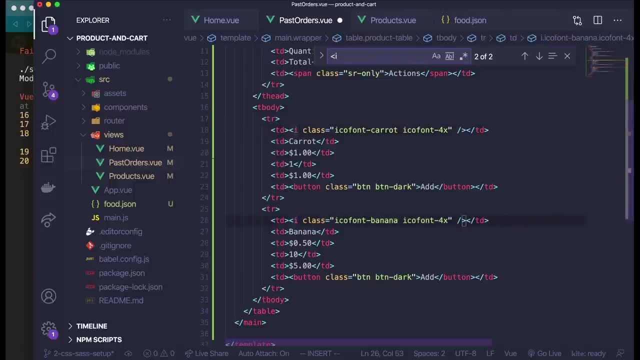 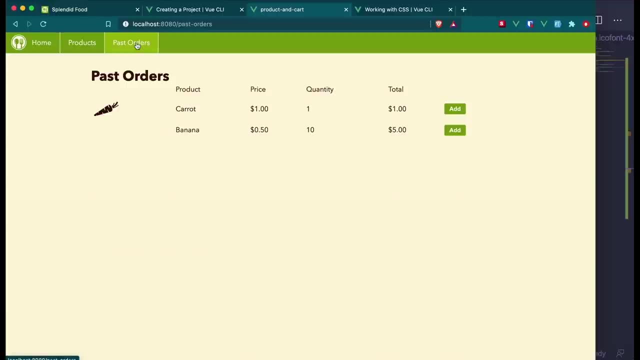 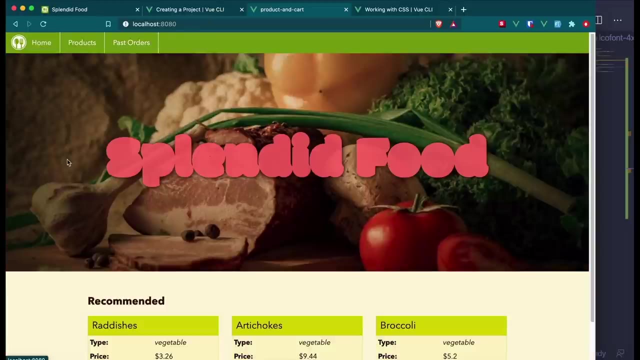 at the end, and I will do that with this I as well, and that fixed my error. and now here's the products page and the past orders page as well. this is kind of a table view of previous orders. now, what about the sidebar? let's add that logic back in in the next. 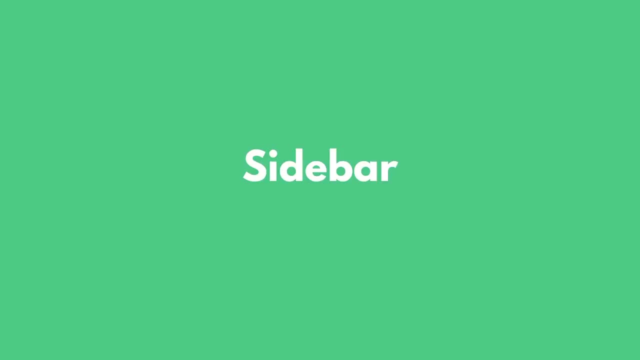 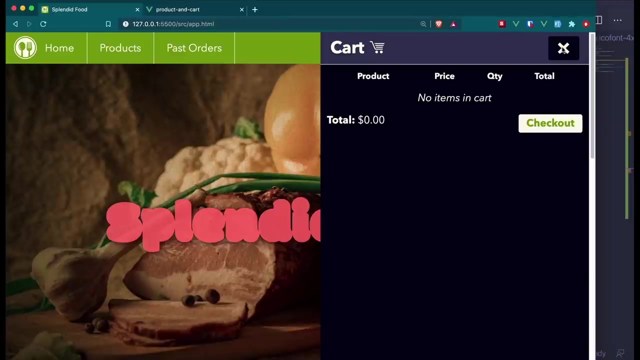 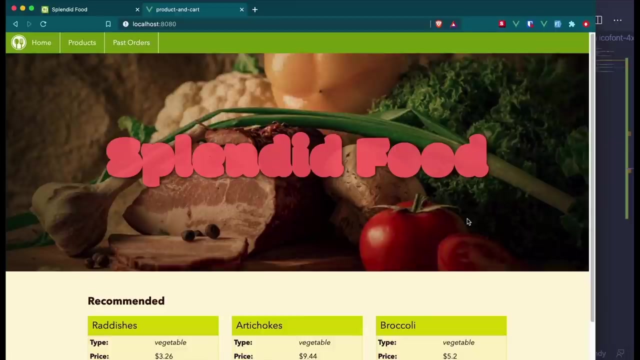 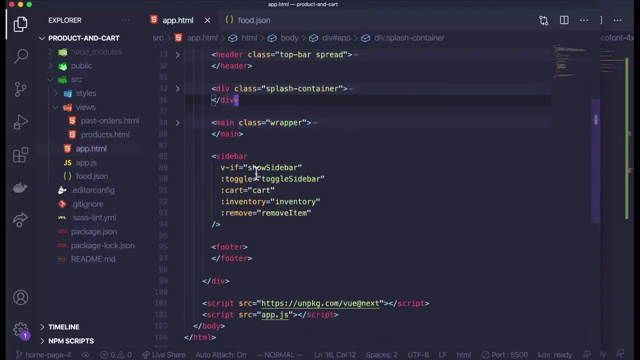 video. in our original application we had this sidebar on the right to display our cart in this video. we're going to move that over to our new viewcli application, so I'm in the original code base here. if I go to any of my files I can see there. 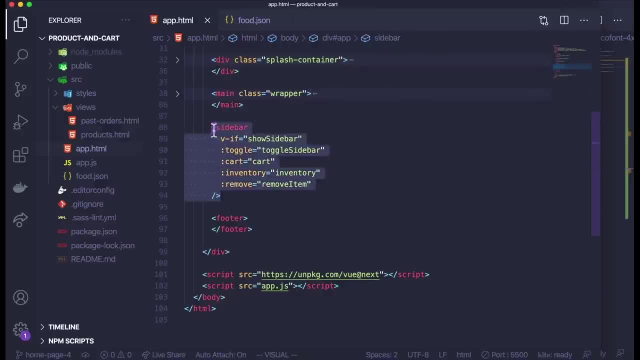 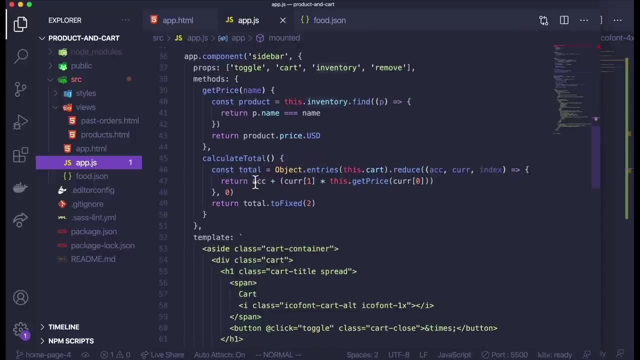 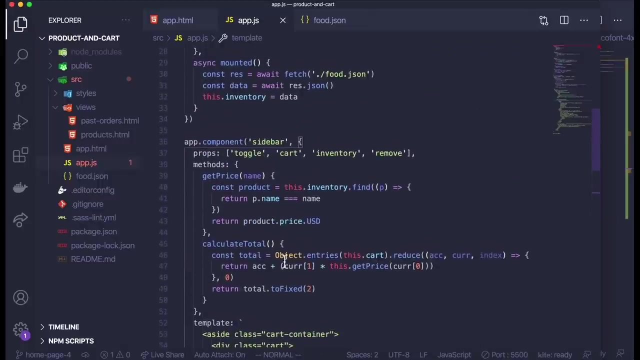 is a sidebar component, which is a custom view component that I define in my appjs file, this sidebar component that I register and I can basically use it globally throughout my application. now, of course, this is just regular view code, so I could absolutely do the same thing. 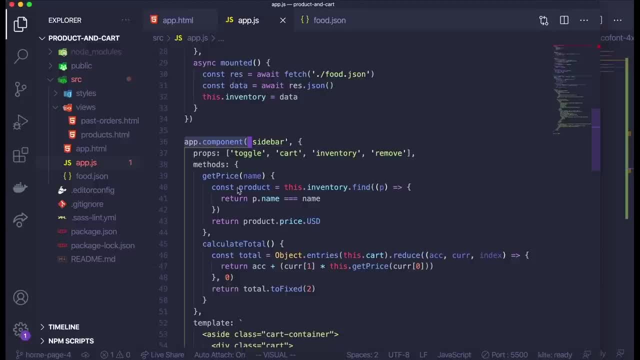 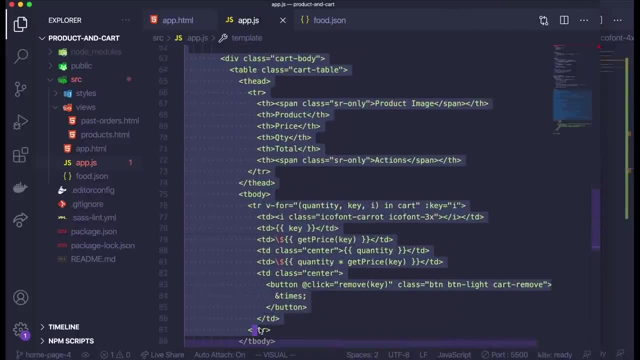 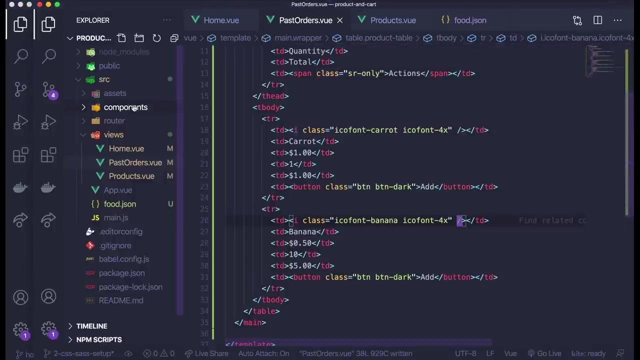 in my new application. but there are other ways that I can now create reusable components, so I'm actually going to put it in my components folder instead. I'm going to copy all of that. let me go to components. I have this old hello world component. I'm going to 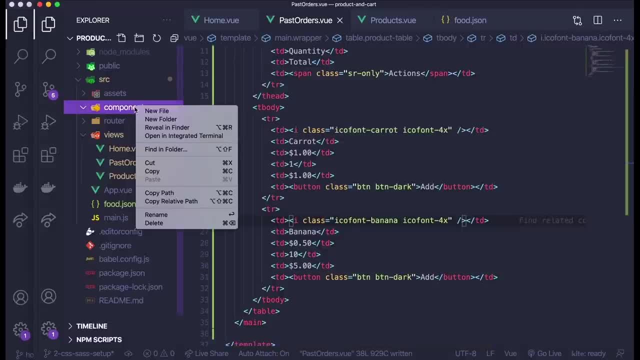 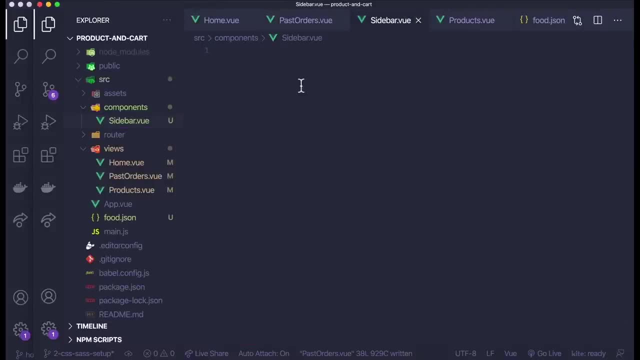 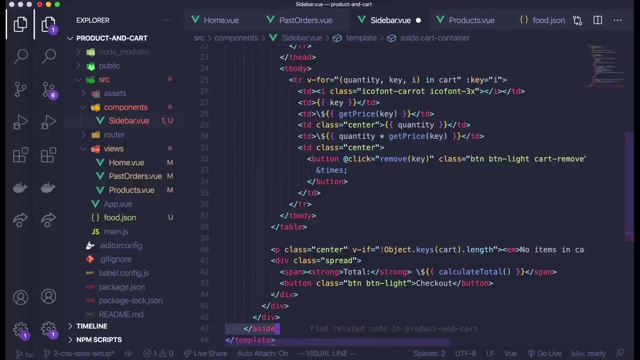 delete it because I don't need it anymore, and then I'm going to create a new file here and call this sidebarview in here. of course, I need the template and I'm going to paste all of that code and this is basically all of the cart logic. now there are a few. 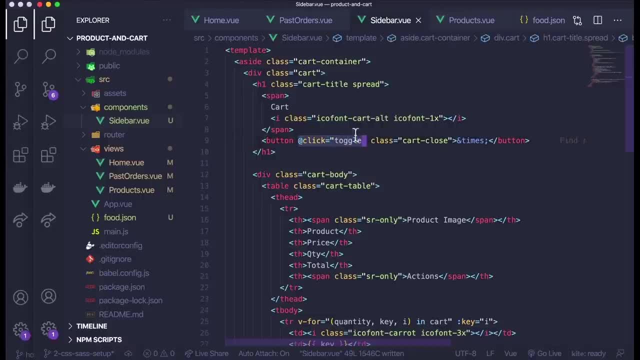 things I will need to add. pass in a dynamic toggle here when the button is clicked. so let me go ahead and set that up now. the first thing I need to do is import this sidebar component into my application, and it's going to be globally available across all my pages. 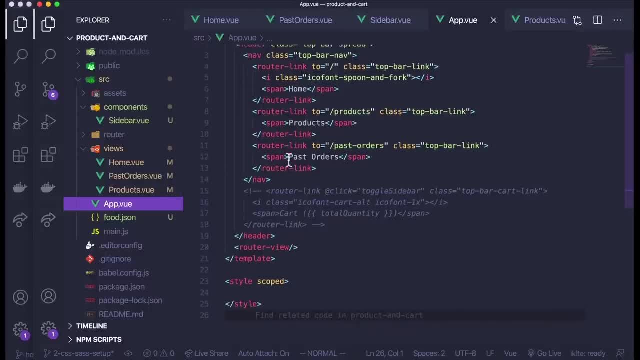 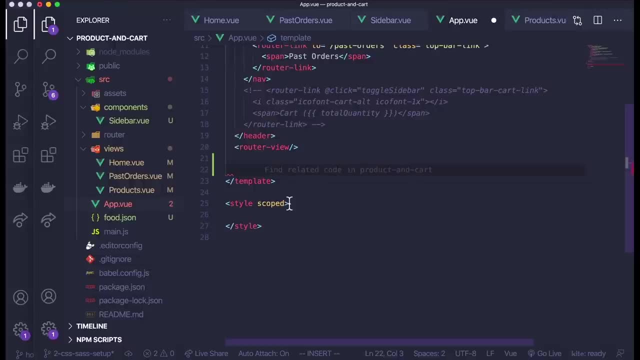 so I'm going to import it into my appview file and I'll do it below. actually I'll do it at the bottom. here I'm going to put sidebar. it has to be, of course, self closing here and also the convention is to capitalize custom components. 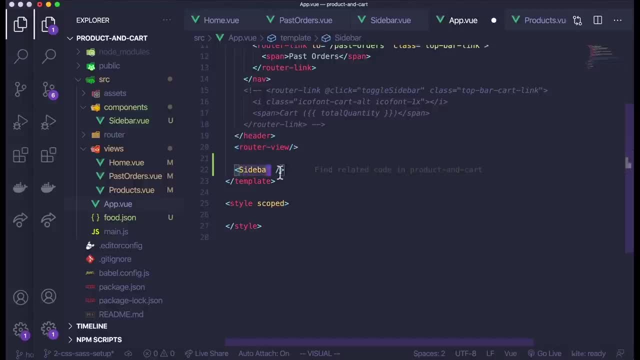 so you can easily see them and see they're even highlighted differently than anything that is lower case, that I've pulled in from a library or that is just standard HTML. I'm going to get rid of my style tag here and add a script tag, and now I can. 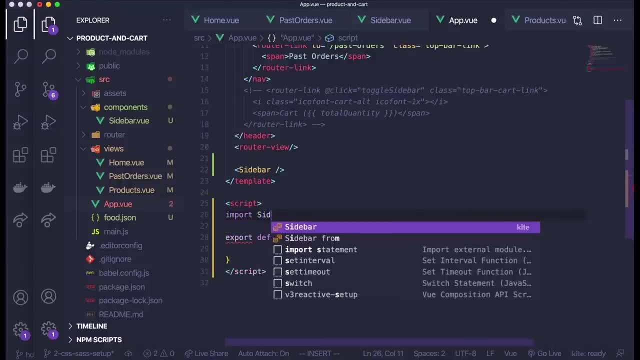 import that component. so I'm going to import sidebar from dot slash components- slash sidebar- dot view. now another way of writing this and what you'll a lot of times see in view applications. instead here you'll see an at sign. now this is a shortcut kind of a. 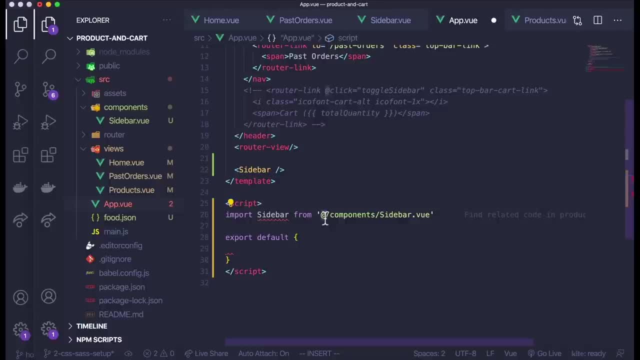 reference to the source folder. so that way, anywhere in my application, no matter how many files deep my components are, I don't have to do anything like dot, dot, slash, dot, dot, slash, dot, dot, etc. I can always reference the source folder with an at symbol, so it will be source slash components. 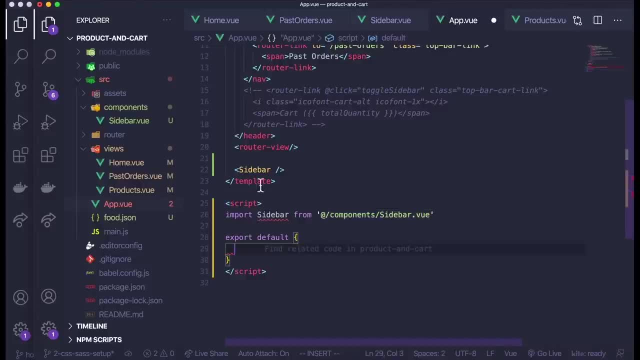 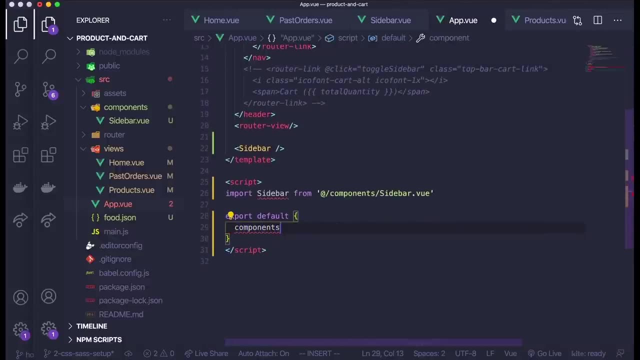 slash sidebar dot view. now, any component that I import into another component, I need to register it and tell my view application I'm going to be using this component and I can do that by setting a component object on this default options object in view and I can set the sidebar component. 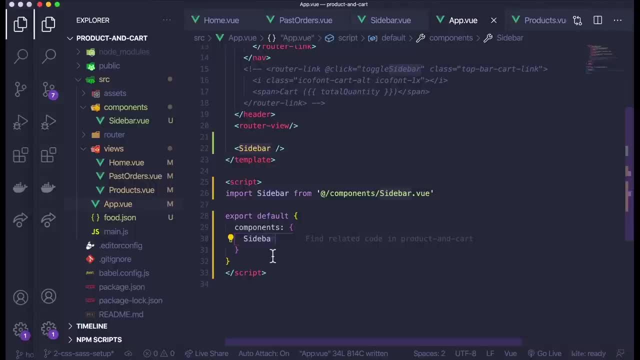 here. registering it here or including it in a list of components here just means that I can use it up here in my template. so how this works, basically this whole object- here it's called the options object- and any kind of javascript functions or data will get set on. 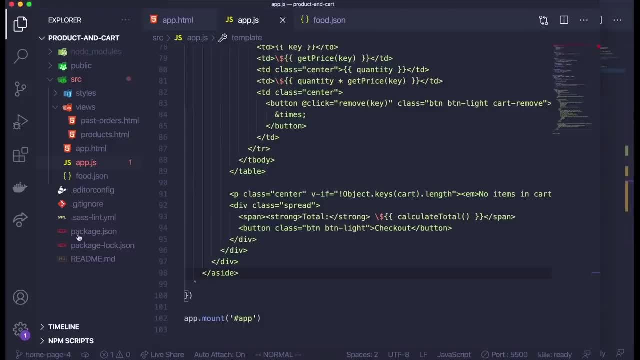 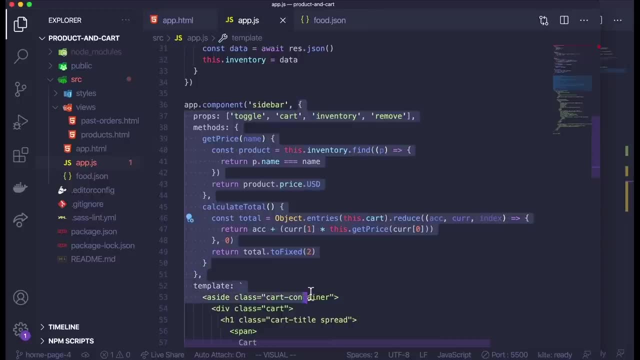 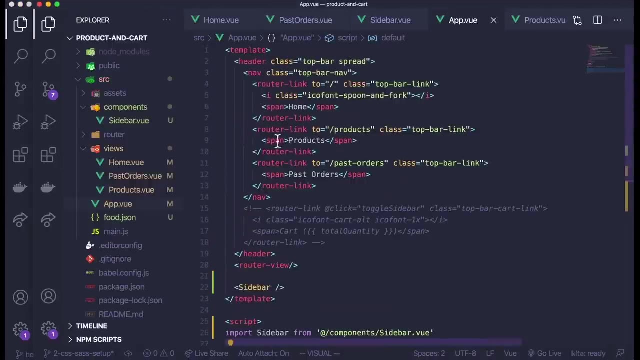 this object. I just want to point out that this is the exact same as the options object you used in custom components like this one, except the template in our dot view file is just included at the top up here inside of this template. and if we look at this, 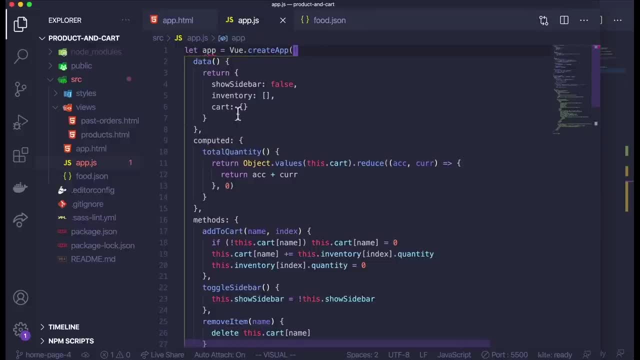 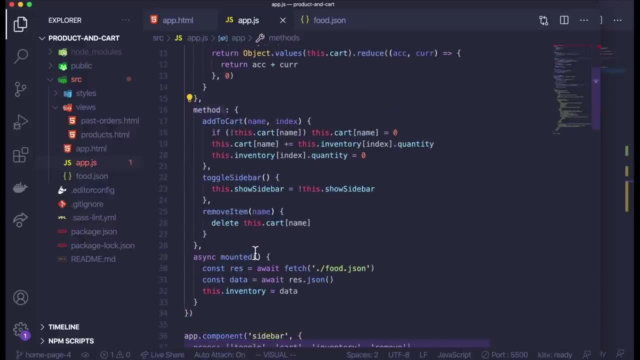 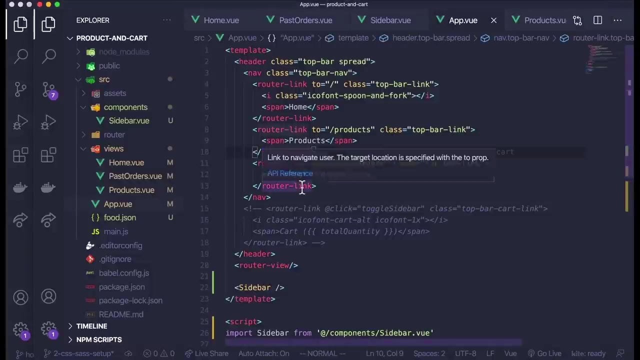 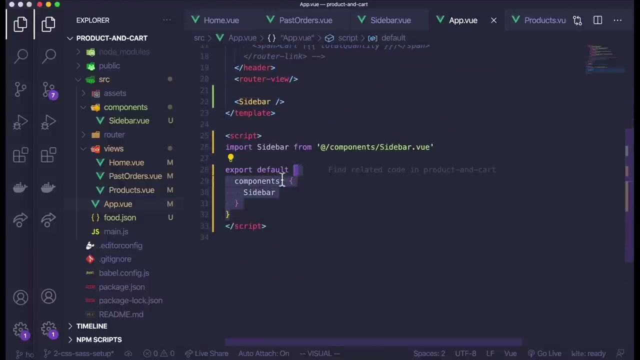 main app component here. everything inside this object, all of this data, computed methods, all of this stuff is the options object, but here we have it to be used globally and when we create a view CLI application, we basically get one template and one options object per component that we 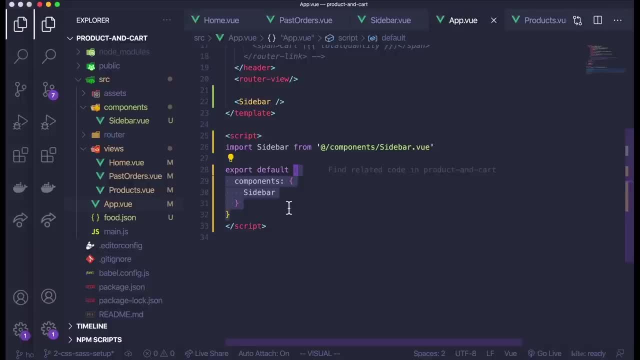 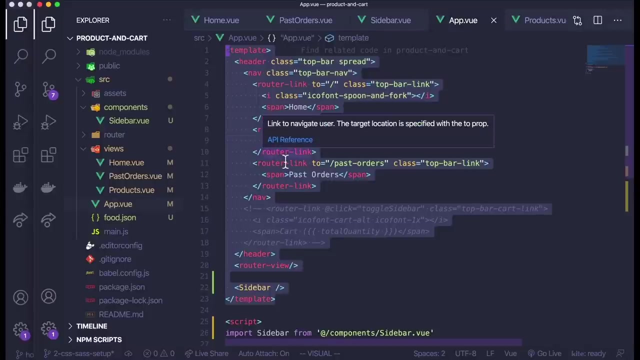 use to define everything on. now, the thing about this is that each component only knows about the javascript inside the options object of that component. so if I create a function here, I can only use it up here and in no other component, unless I explicitly pass it into that component to be used. 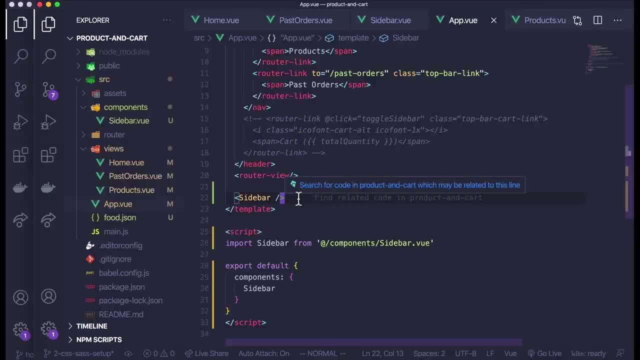 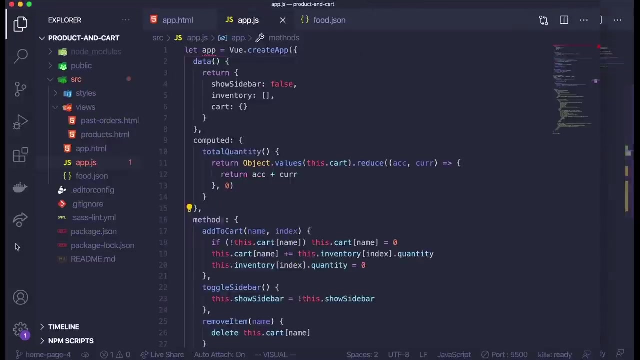 just the same way that we passed data and functions around two different components when we were building the static application, and here we're going to need to do that again because sidebar requires certain things to be passed in now. if we look here, we can see that first. 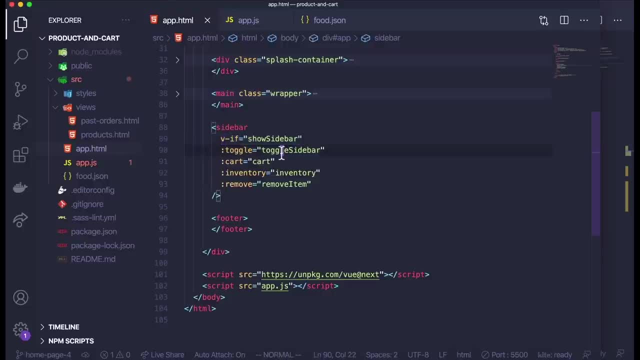 there is a vif boolean. there's a function to toggle the sidebar when it's clicked, or when the button is clicked to open or close it. there's also a cart object for what is currently inside the cart. there are all of our inventory items, and then there is a 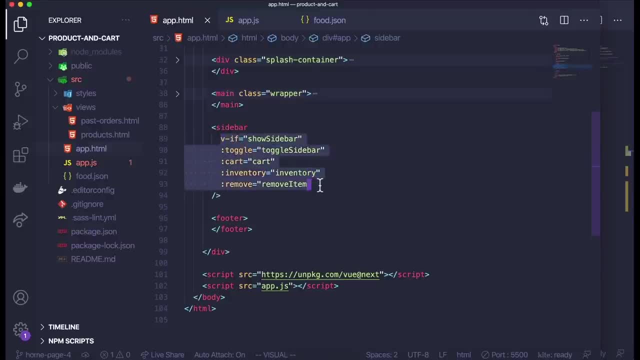 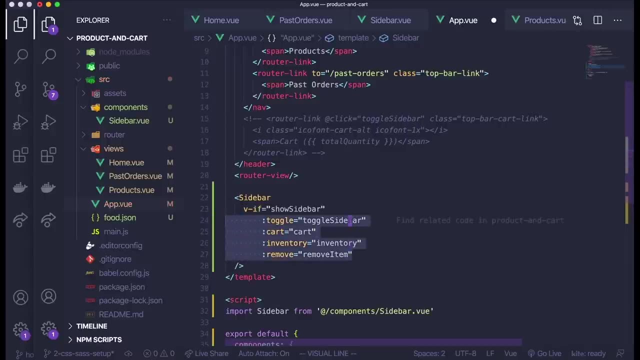 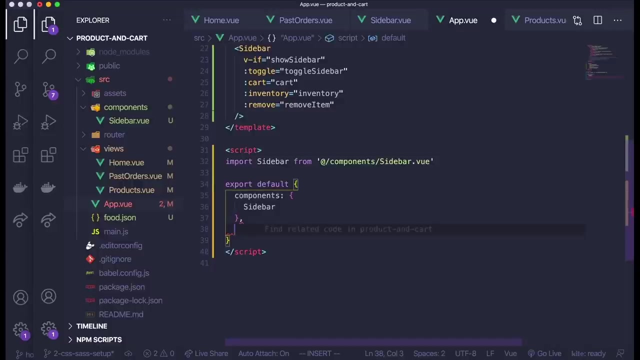 remove item function. so I'm going to copy all of these things and paste them over here, and now I need to define these properties. first thing is vif. I need to create a show sidebar data property here, and I'm going to set this default as true. 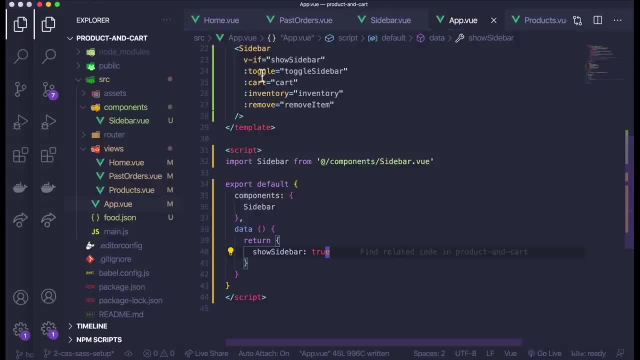 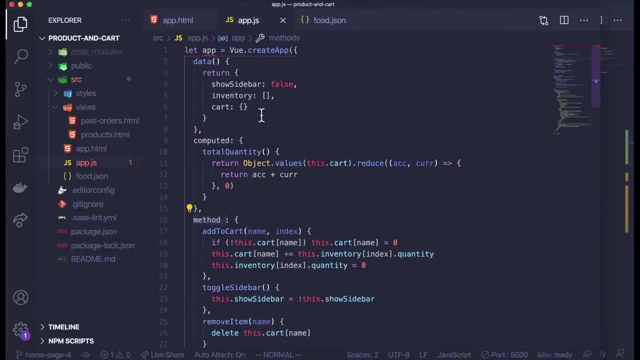 for right now so I can see the sidebar. now I need a toggle sidebar function. now, where does this come from? it has to come from my app component up here, because I'm passing it in basically from app to the sidebar component. so here's my toggle sidebar. 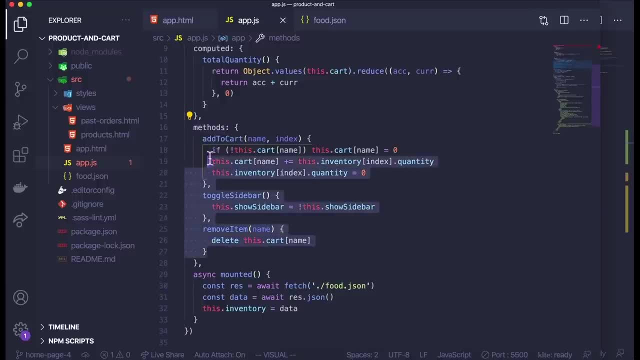 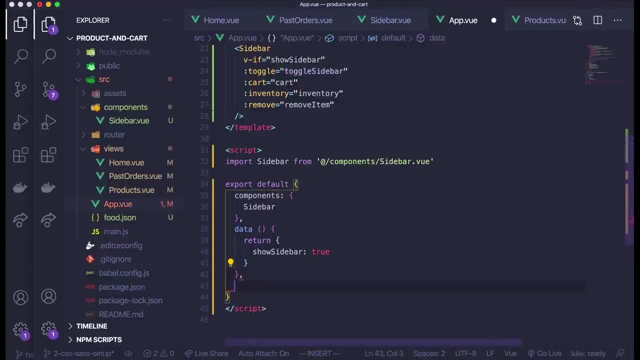 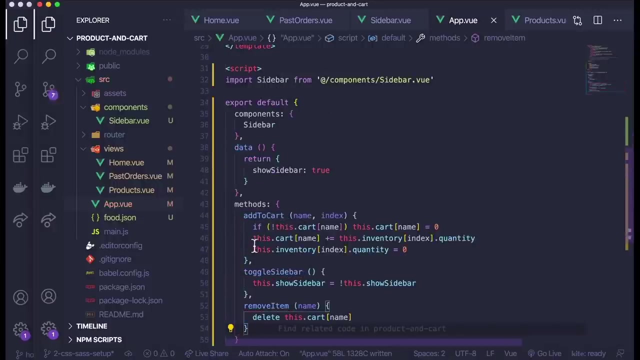 function and I'm just going to grab all of these functions right now and I'll create that methods object and I pasted in all of my methods here. now here's another tricky part, because I want to reference inventory here, but unfortunately I only have it in my 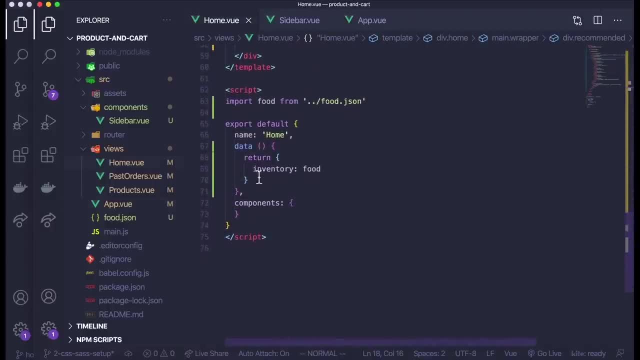 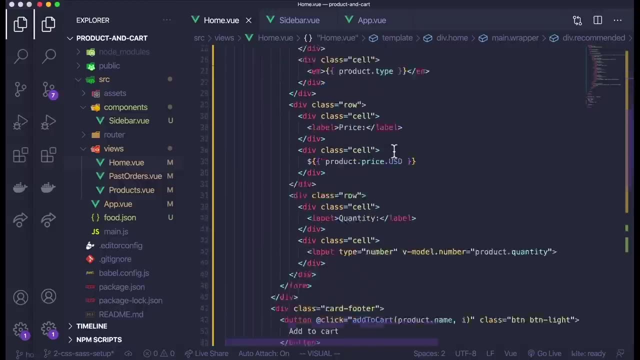 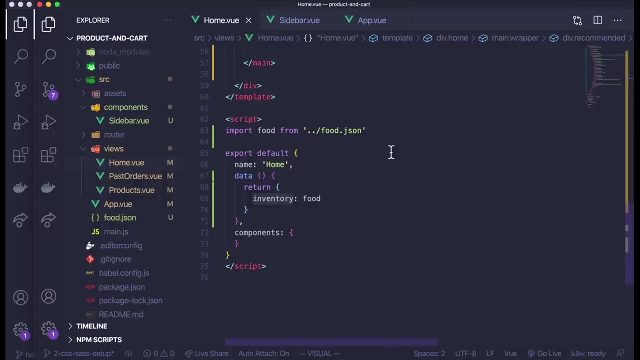 home component which I just kind of quickly put there to fix my issue of basically inventory being undefined. so I'm going to have to restructure my application so I'm not importing inventory separately into each component. so let me actually take this import and I'm going. 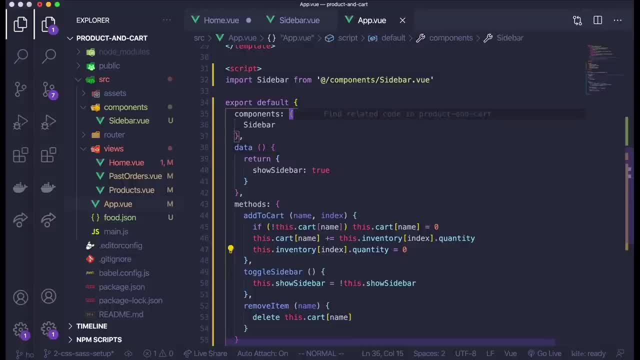 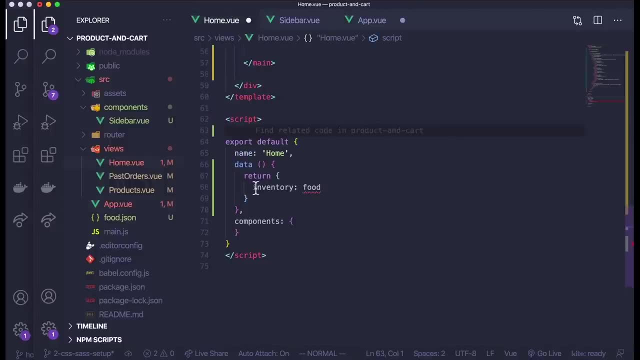 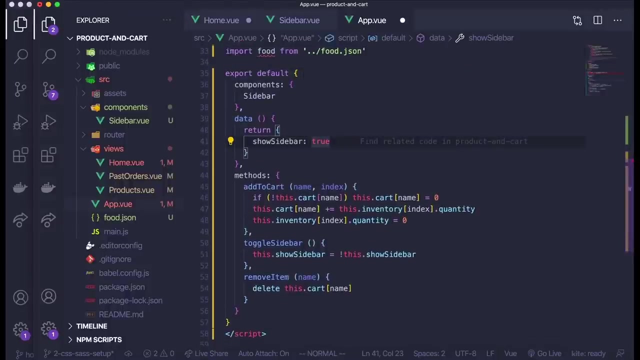 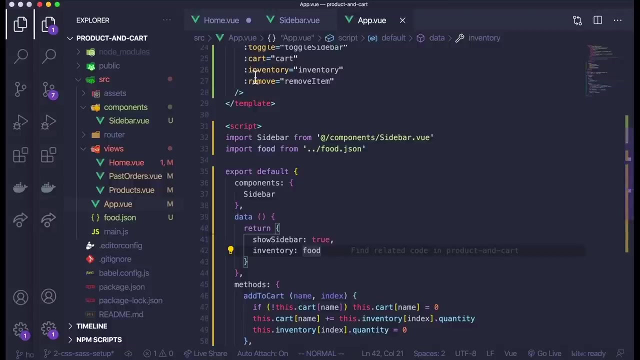 to just import inventory into my appview component. so I'm importing it here and then my logic here. so inventory food and I'm going to add that to that as well. so inventory is food. now I need to get it to my home component, but it's not really a registered 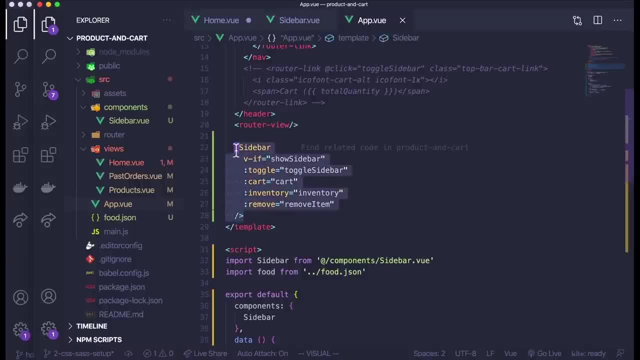 component on this page like sidebar. I can easily pass elements into sidebar as props because it's a registered component right here. but home is a little bit different because the router is dynamically putting the home component there. so how do I pass props through the router then to whatever? 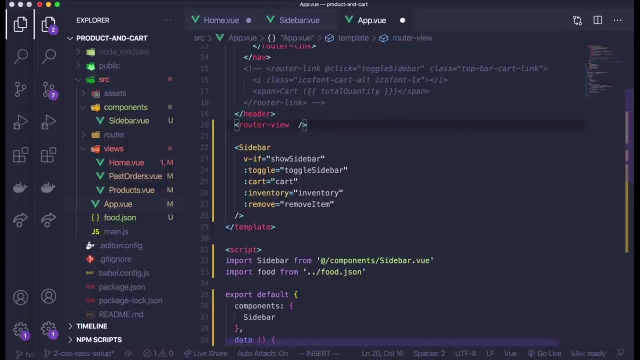 component the router loads. what we're going to do is pass in inventory into basically any router view component. so I'm going to pass in the inventory variable and of course I need to vbind this to make it actually look for a variable and not consider it to. 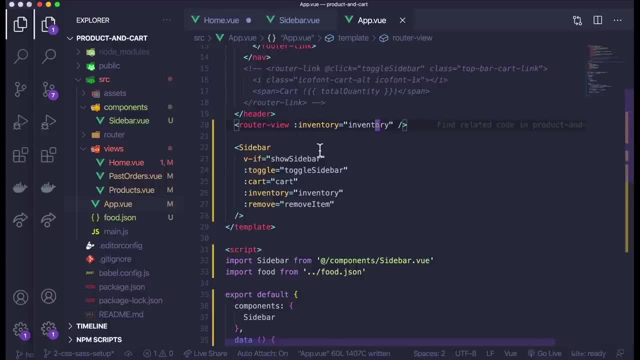 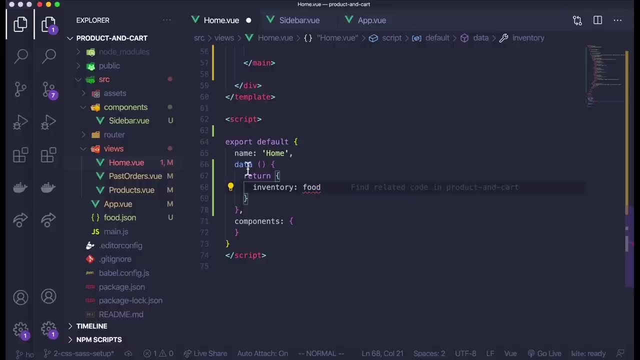 just be a string here. so now I'm passing in inventory and I need to accept that in the child component. so instead of data here I'm actually going to have to use props, just as I did before, and have a props object, or I'll just do it as an array. 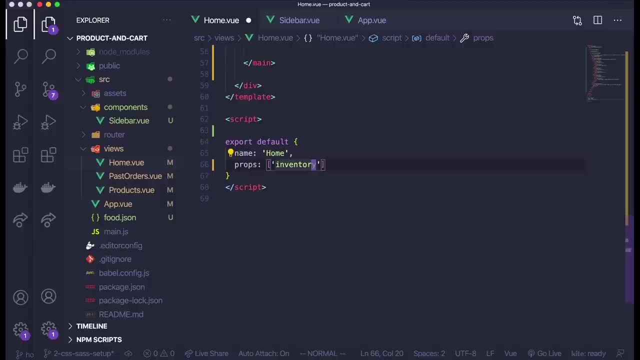 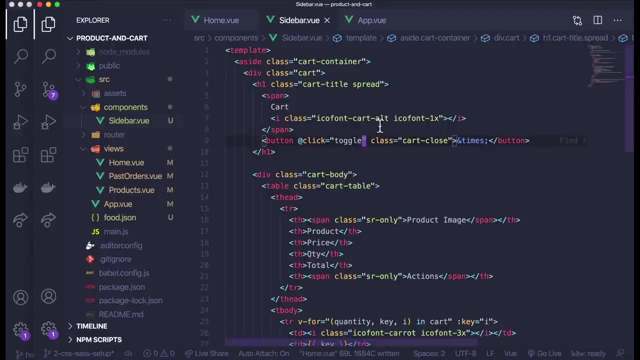 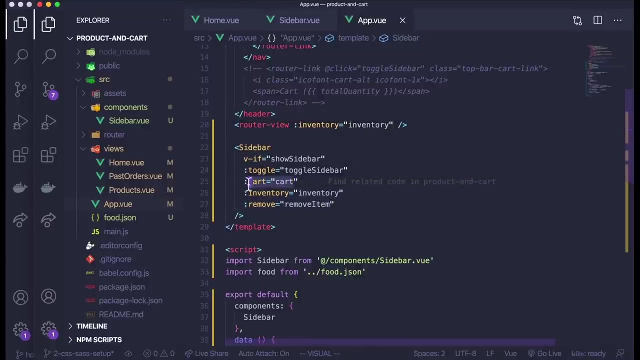 actually- and I have to call it inventory- there are a few more broken elements that I will have to fix here that the sidebar is expecting. I have my inventory and remove item and I really just need my cart at this point. now, if I look in the original version, 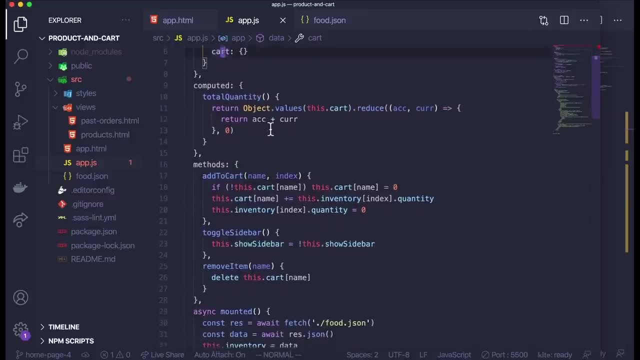 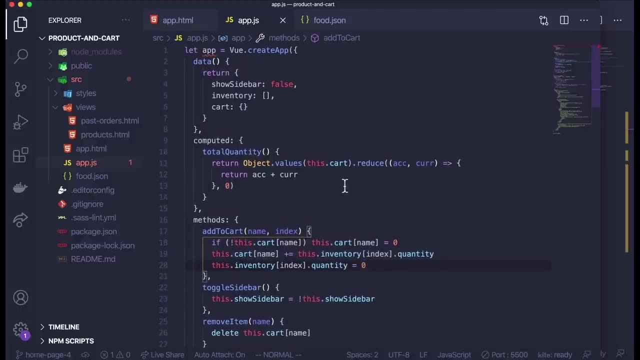 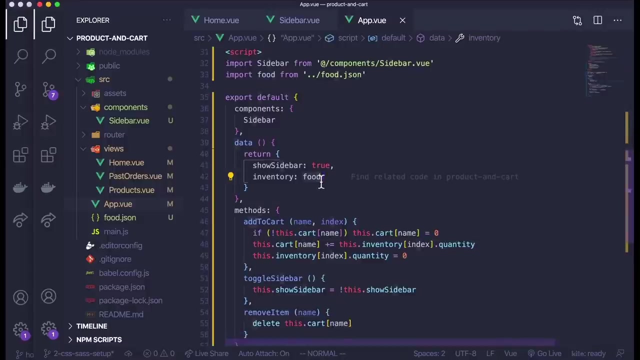 I can see the cart is just an empty object and then things can be dynamically added to the cart. but we're going to worry about dynamically adding things in a minute, but first I'll just set it to an empty object. so let me go to data here. 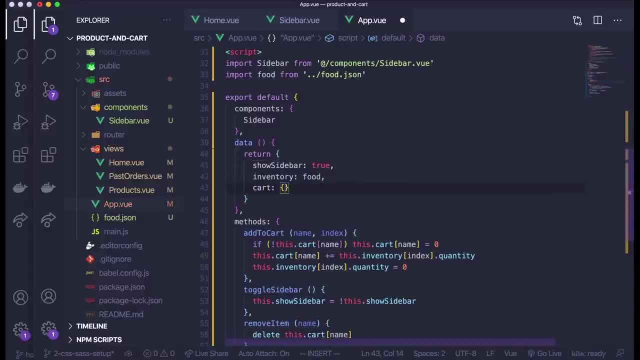 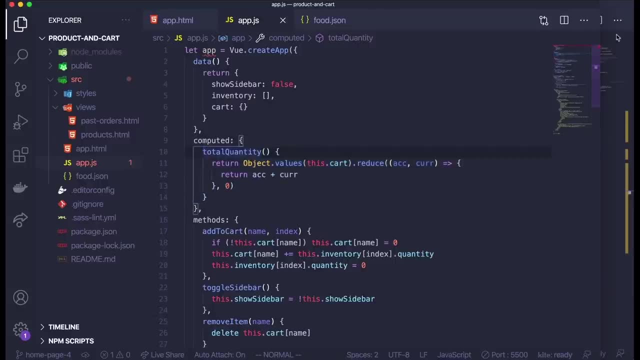 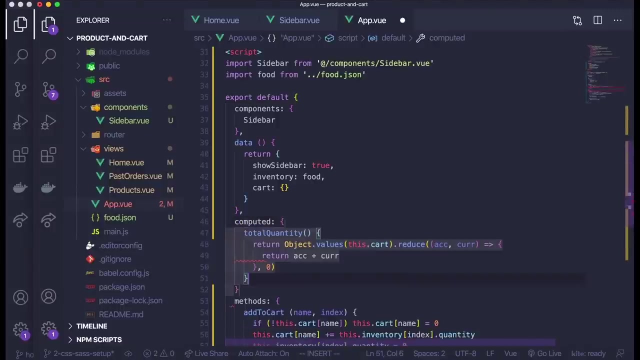 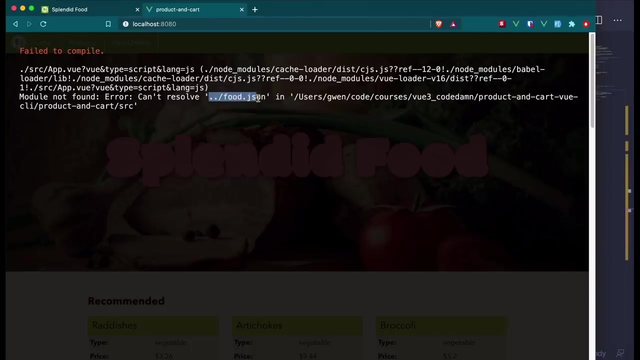 and set cart to an empty object really quick. let's go ahead and grab this computed property as well, because we will need it. so I'll come down here and put computed and let's check this out in the browser. so it's complaining right now that it can't find this json. 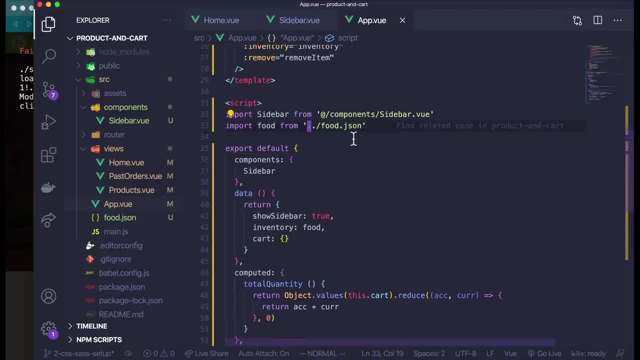 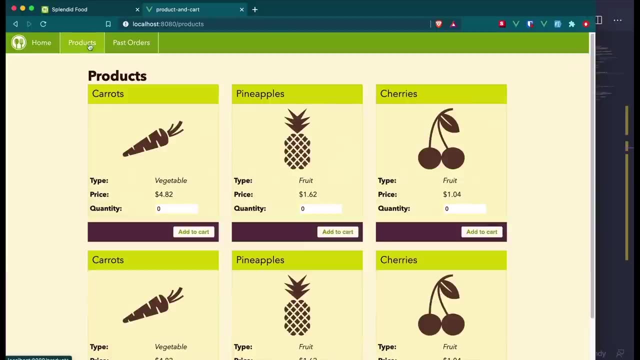 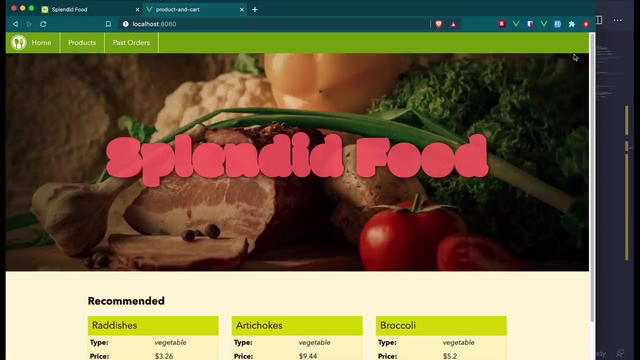 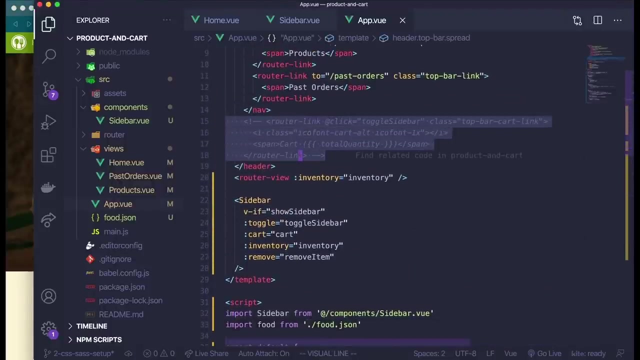 file and that's because we are importing it from the wrong place. and yay, the app is running. products passed orders, everything seems to be working okay. however, we don't have the sidebar yet, so let me go ahead and uncomment this code here, so we have toggle sidebar. 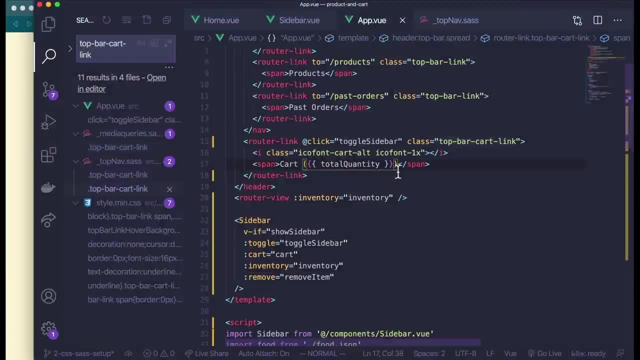 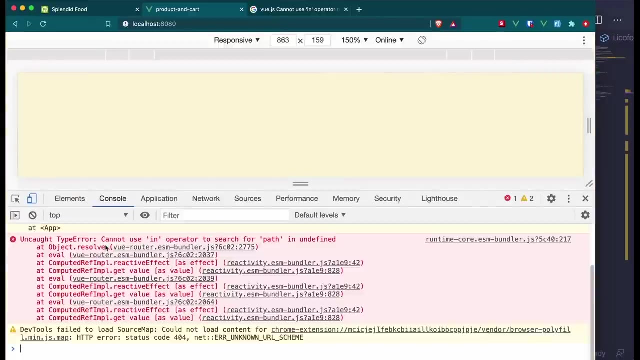 and also showing the quantity and the button here. so here I should be able to see the button that we had before in our previous application. alright, when I come here and refresh, nothing shows up. so we have some kind of an issue. it says uncaught type error can't find path of. 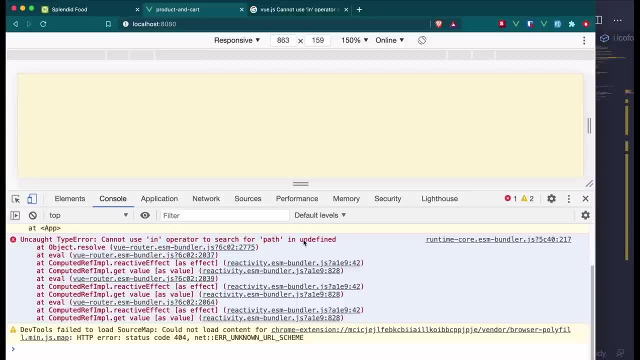 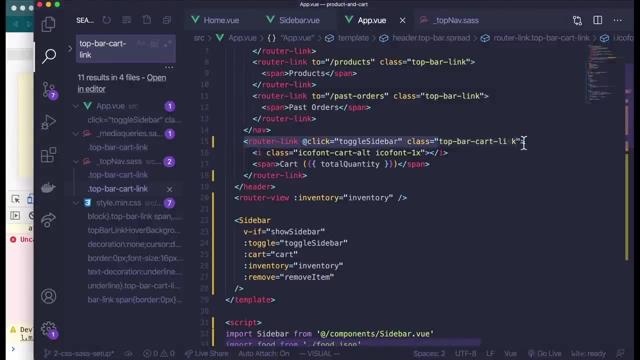 undefined, so the path. this is referring to the router. so I think it's giving us an error in the router link because we are not properly using the router link. so let me just change this to a div. we basically aren't telling it to route anywhere, we are just 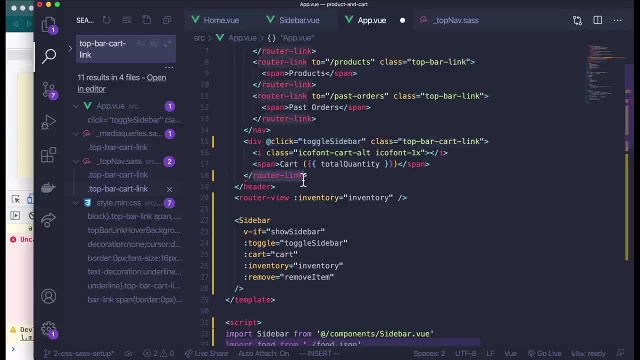 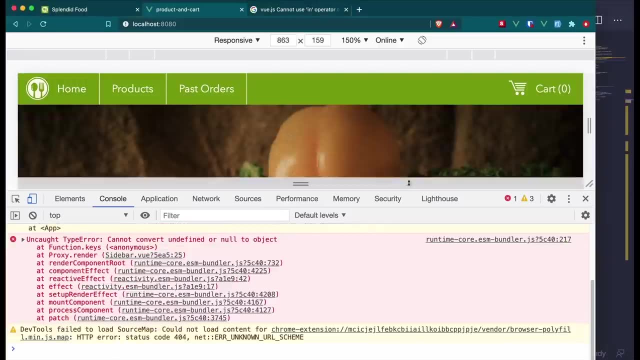 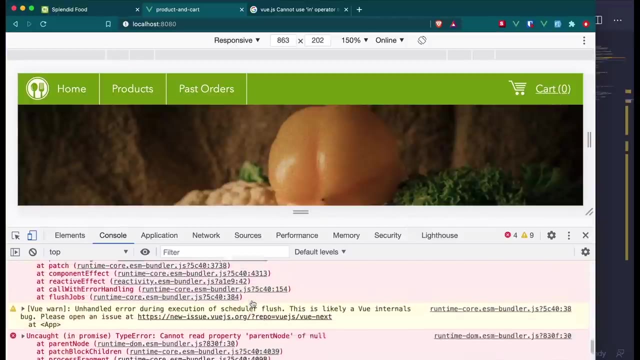 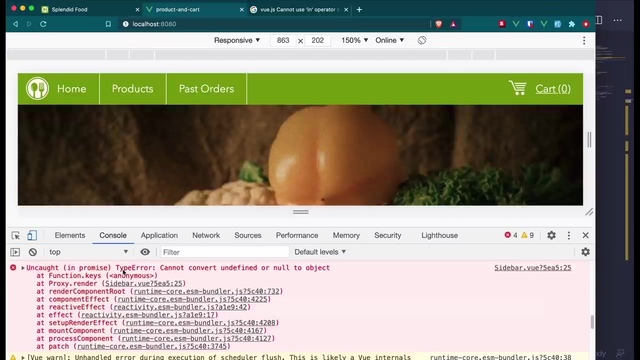 using it as a clickable element, so we might as well be using something else. and now it is working, except I can't click on the cart button. that's not working yet, but everything else is working. let me scroll up to see my original error here. so it says cannot. 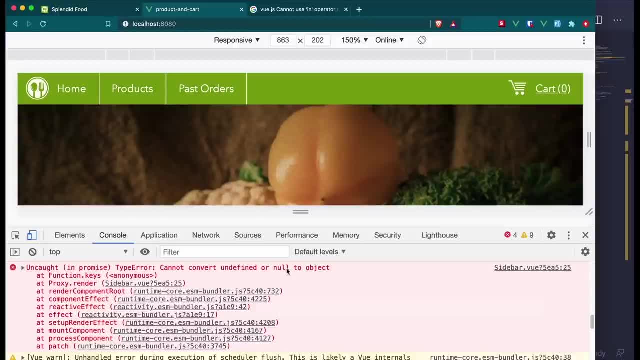 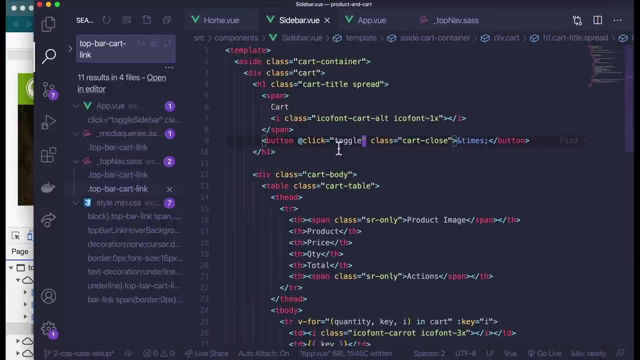 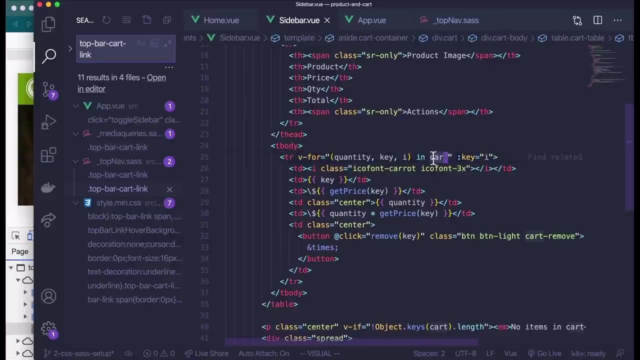 convert undefined or null to an object and this loop is basically inside of my sidebar component, so it's complaining about this line here. line 25: I'm trying to loop through a cart object, get the quantity and key as well as the index and basically it's. 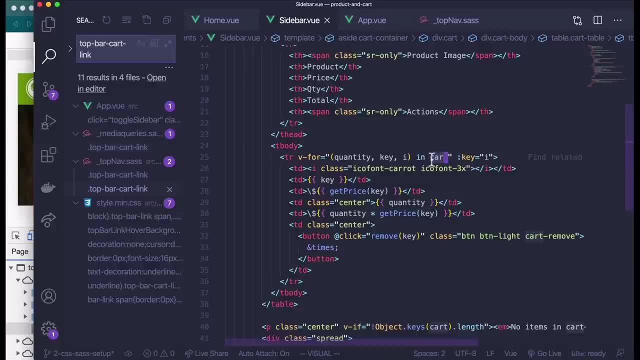 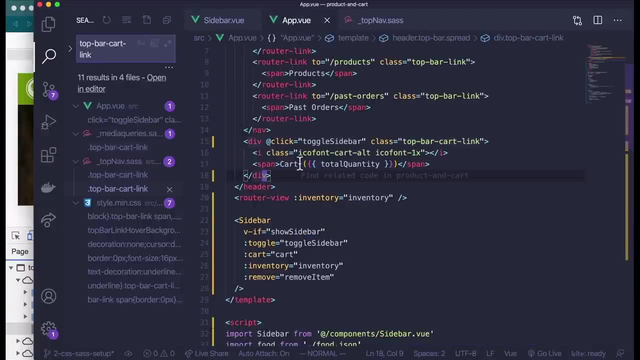 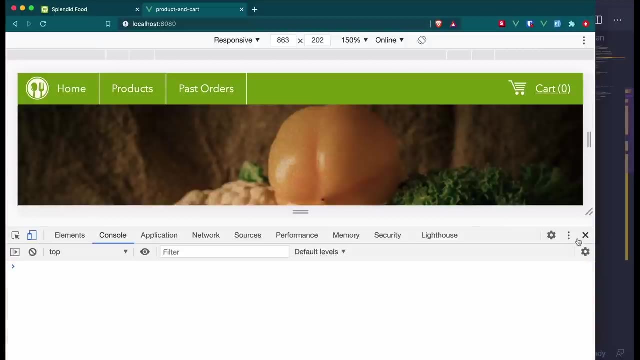 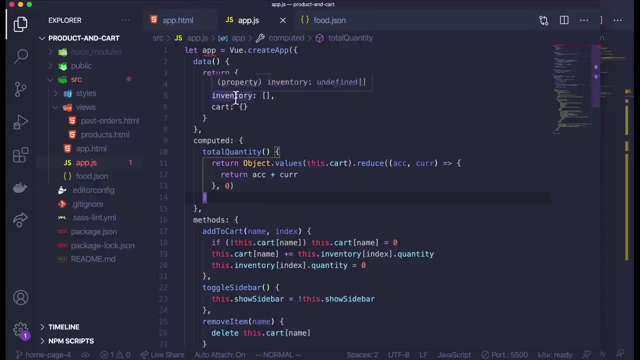 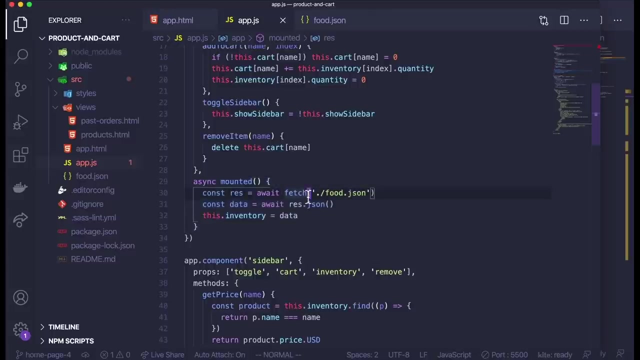 saying that cart must be undefined value. so let me take a look in my app. here it's not opening. so let me actually take a look at the original code and inside of my appjs I have all of this code moved over, except this mounted here. but I don't need that anymore. 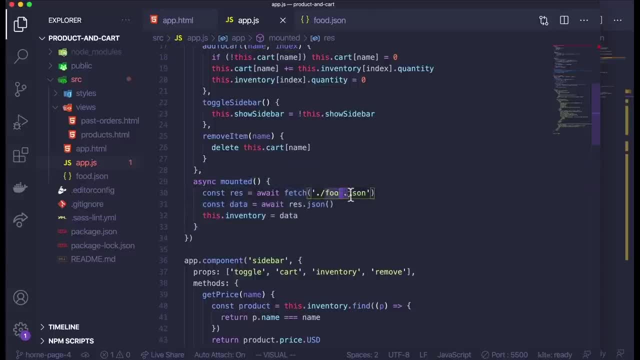 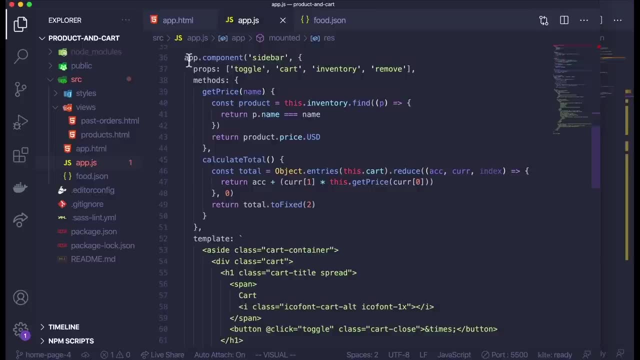 because I can now directly import the JSON file. I don't need to fetch it. so here's my sidebar component. and actually I didn't copy over any of the methods here and I'm also forgetting to add in the props, so let me go ahead and do that. 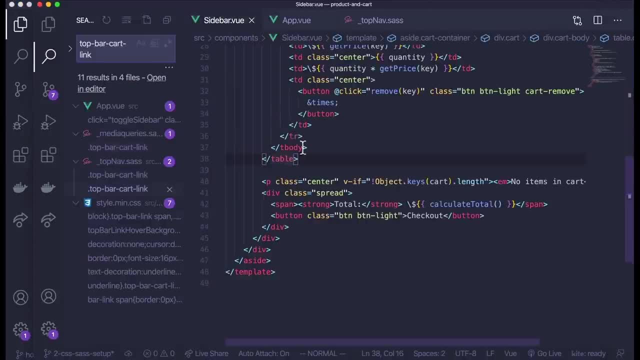 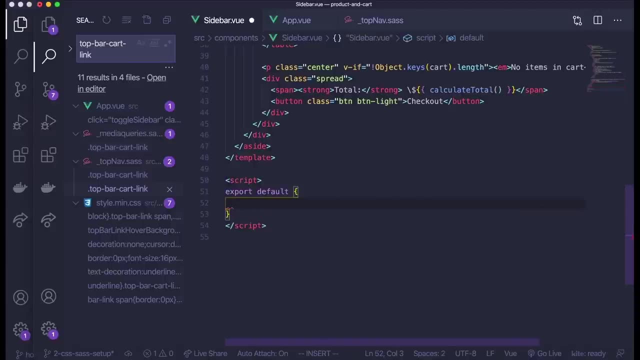 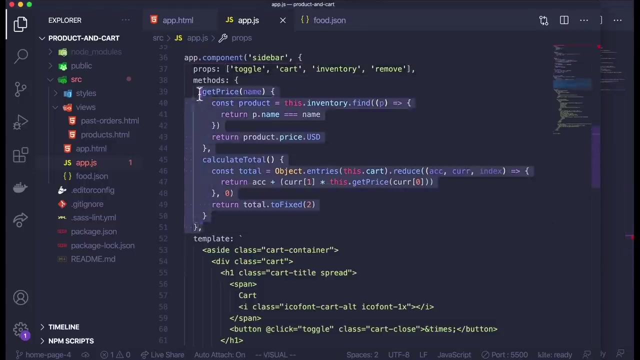 just copy this, go back here to sidebar. and I do need to script tag at the bottom here. so I'm going to add a script tag, paste in the props, and then I also want the methods from here, so I'm going to grab those as well. now calculate: 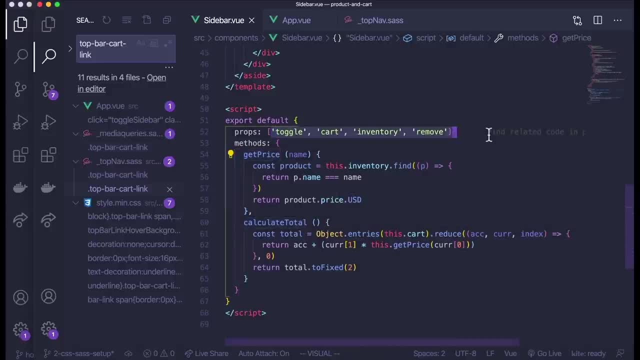 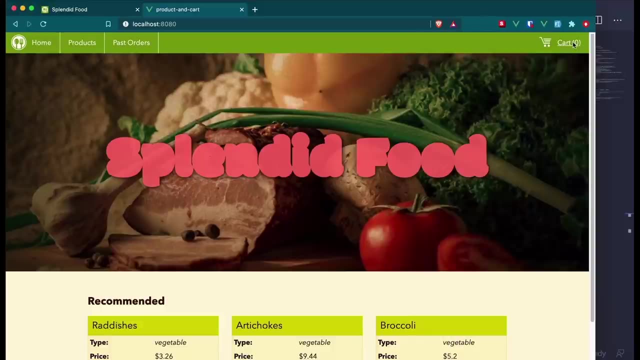 total and get price are defined, and then I also have all of the props here, so let's see if this works. yay, and the toggle is perfectly working. of course, it's starting off as open. if I refresh, it just automatically opens, so let me change that in. 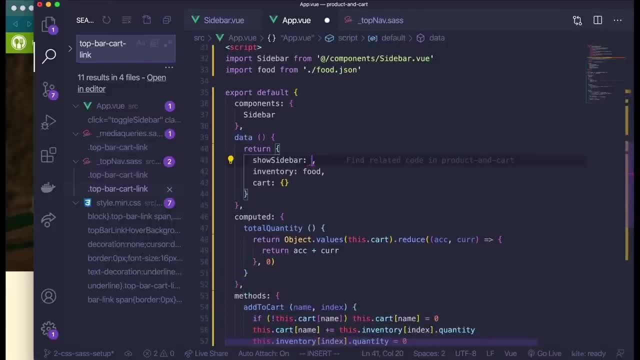 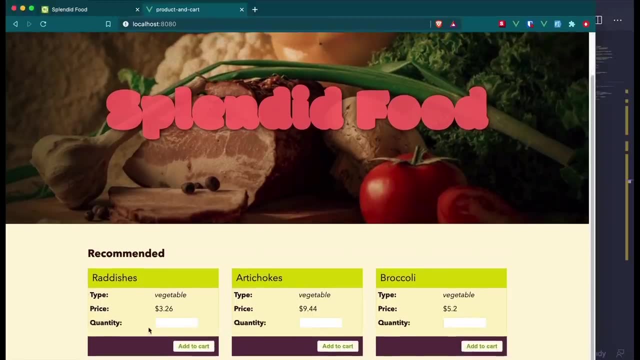 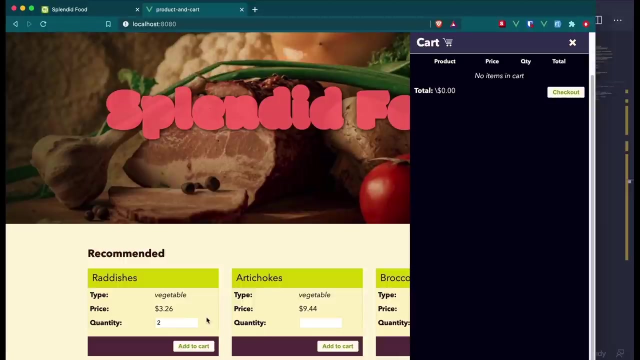 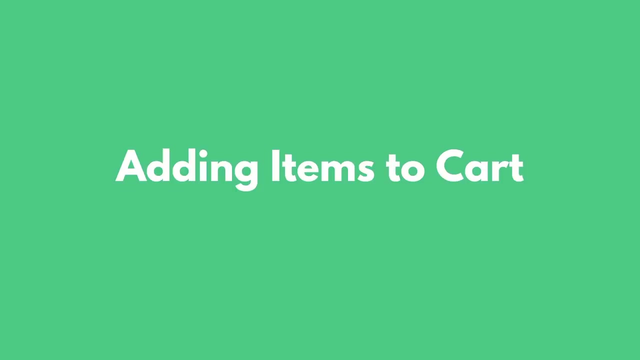 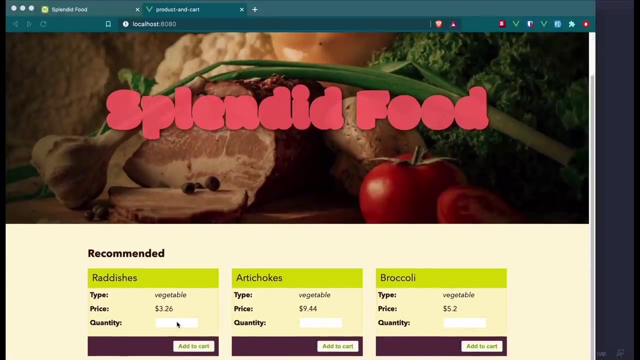 appview, I'll come here and say show sidebar is false. alright, let me see if we can use this. so it's not dynamically adding items to the cart yet, so we will fix that in the next video. in this video we are going to hook up the add to cart functionality. 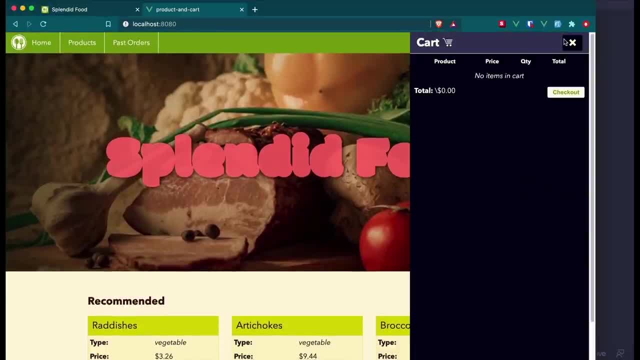 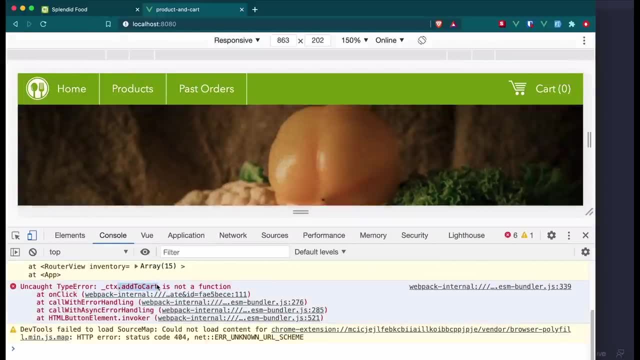 so that when we add to cart here it will show up in the sidebar. if I look in the terminal right now, you can see that this add to cart it's saying it's not a function. so I'm getting an error when I click this add to cart. 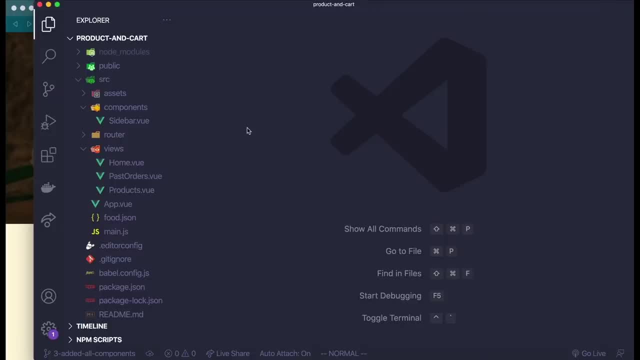 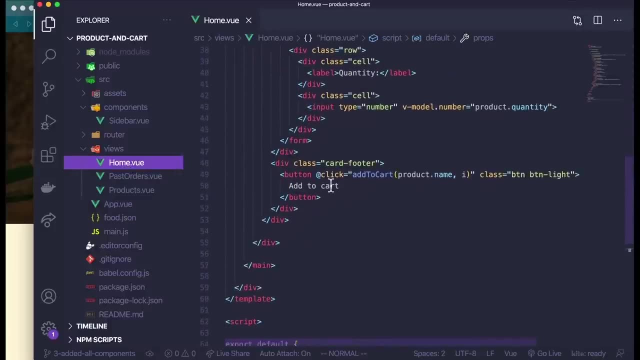 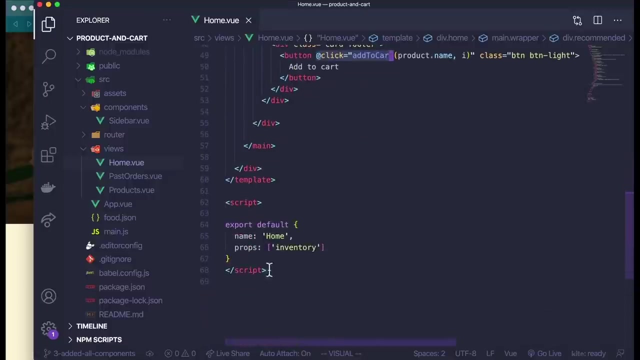 button. now I can see why I'm getting that, because that is in my home page component and if I go down here I can see this add to cart function that I'm calling when I click that button is not defined anywhere in this component. where is that function defined? 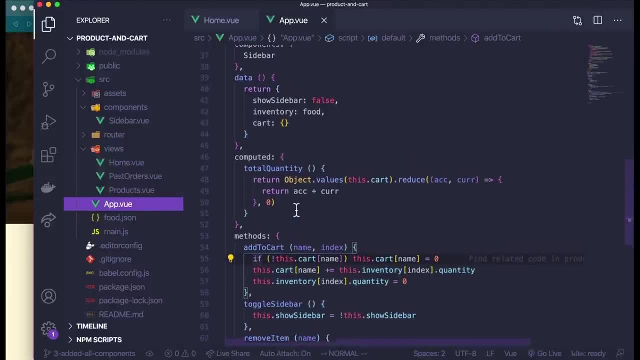 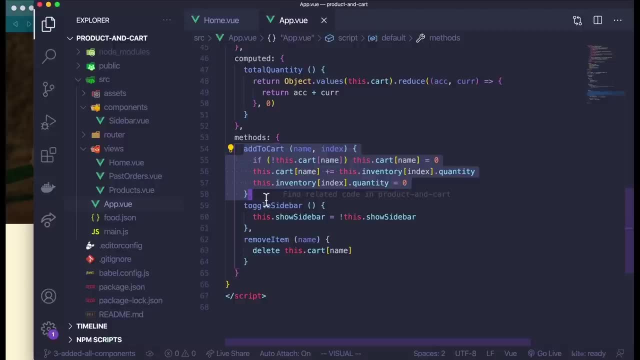 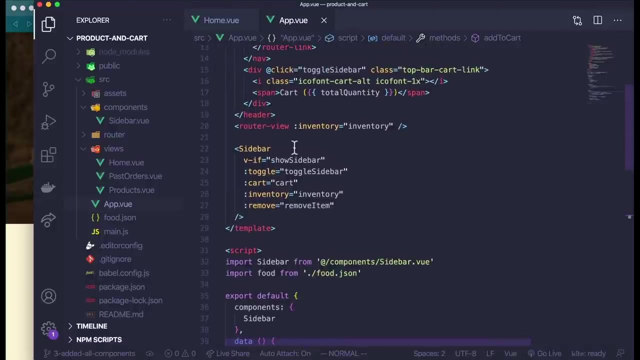 it is in the appview file. so if I go to my methods I can see I have an add to cart method right here. I basically need to pass this function into my home page for my home page to be able to use. so I'm going to also pass. 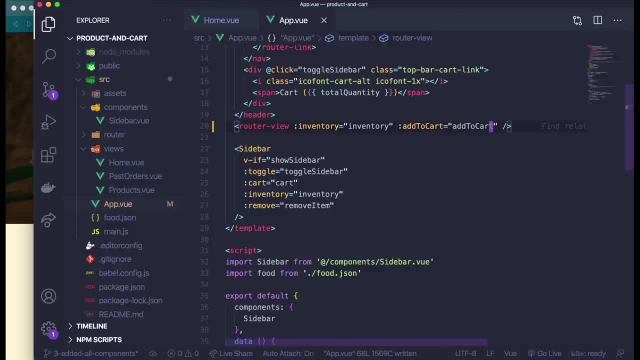 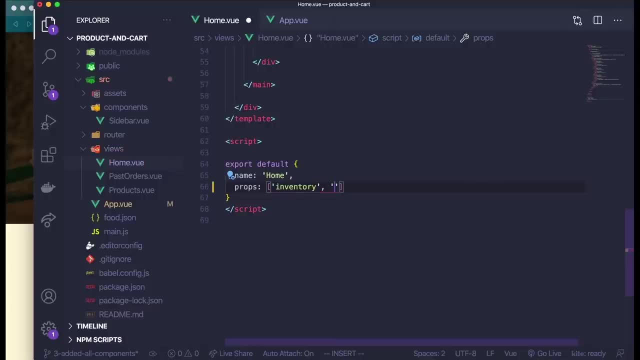 that through the router, as I did before and then in my home page. I can also receive that as a prop. add that onto the props list. add to cart. so I should have access to the function that I passed into this home component now through the router view. 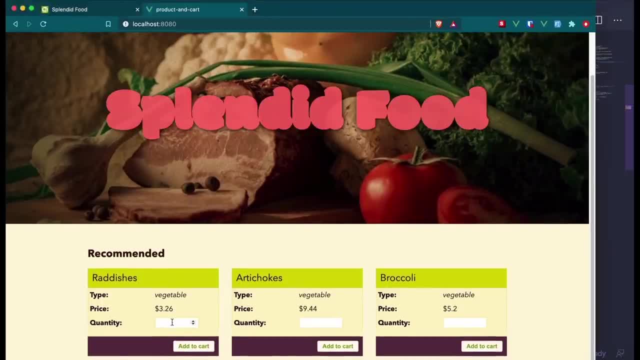 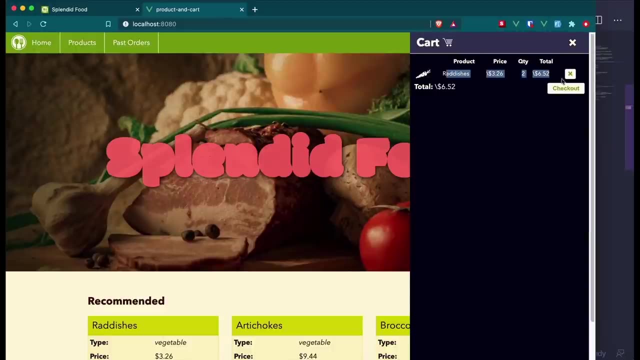 and let me refresh and see if this works. add to cart and you can see that the function is working, because the quantity changed down to zero. the cart says two items and if I open it, it does indeed list two items here. now why are there forward slashes here? 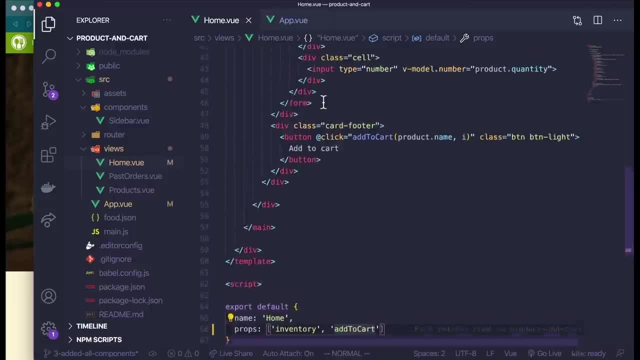 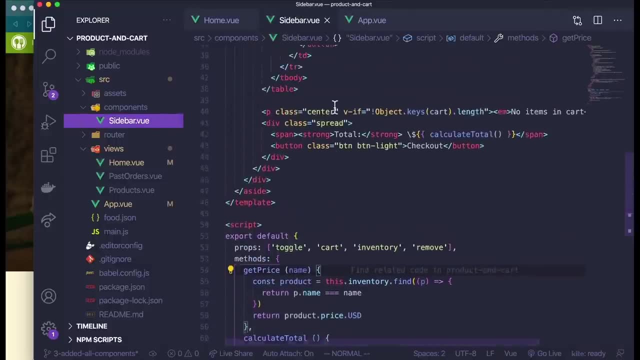 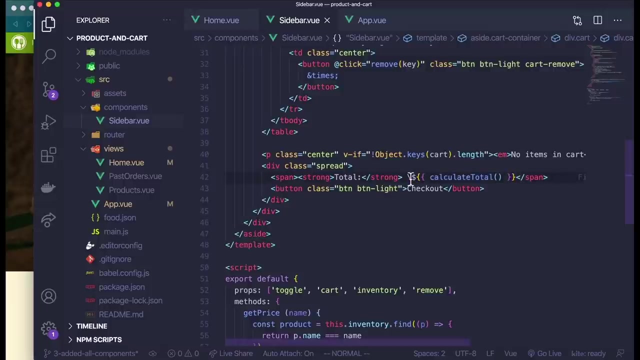 we can actually see in the home page that in regular javascript this is actually in the sidebar component- that in order to put a dollar sign before the variable, we needed to escape it. but we don't have to do that in a vuejs application because it's no longer in a. 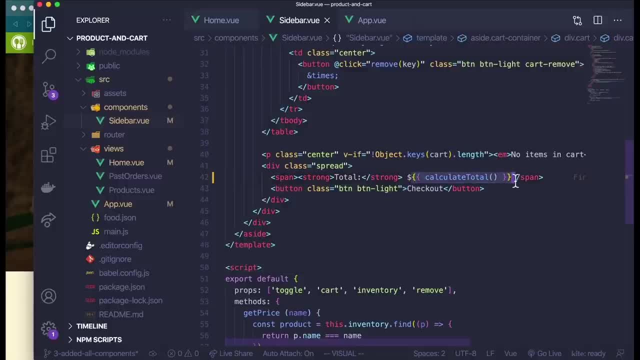 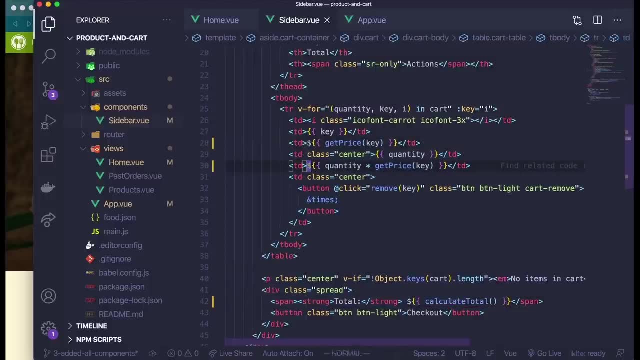 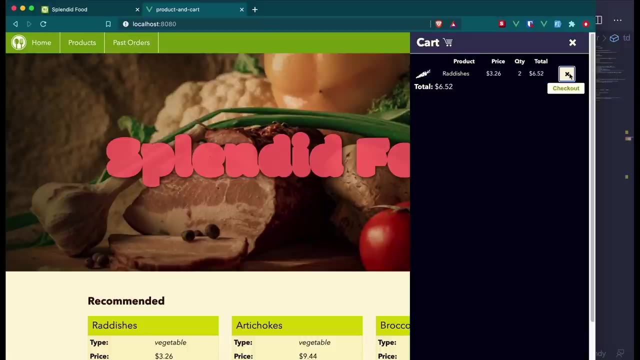 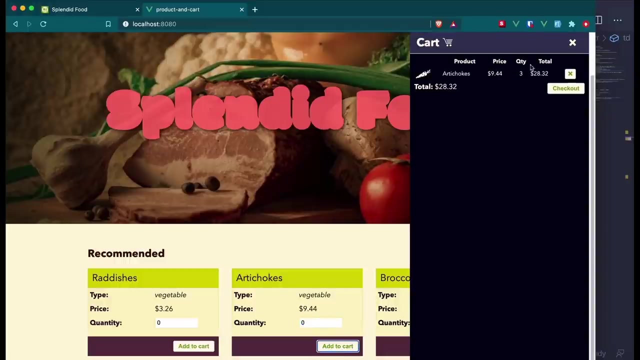 regular javascript file. it's in our vuejs template so I can get rid of all of these escaping characters and now that looks much better. now, if I want to delete this, it deletes. no longer have any items in the cart. I can add a couple items and I get items in the cart. 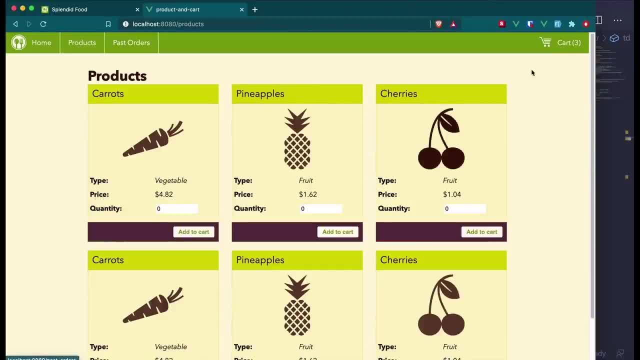 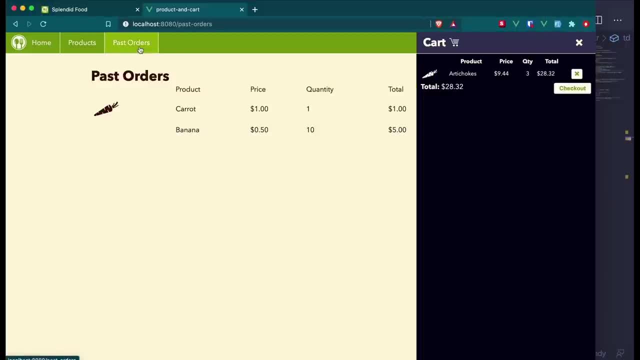 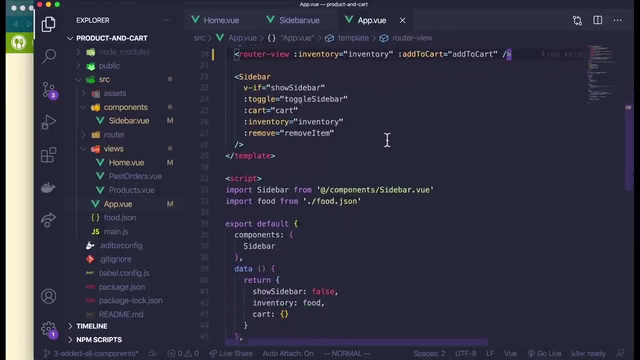 if I go to another page, the cart should still work because that is a shared component that I can see across any page. in this example application, this type of data sharing works pretty well. we can keep all of our variables in a parent component, so in this case in our appvue. 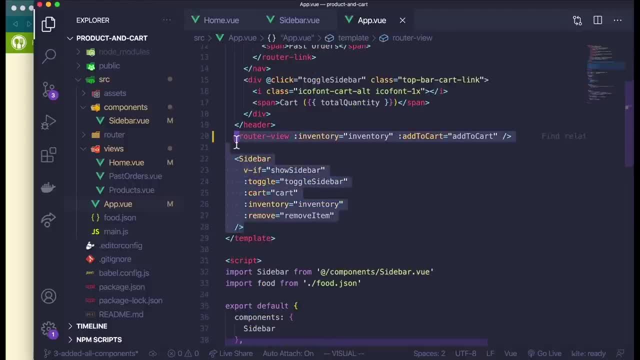 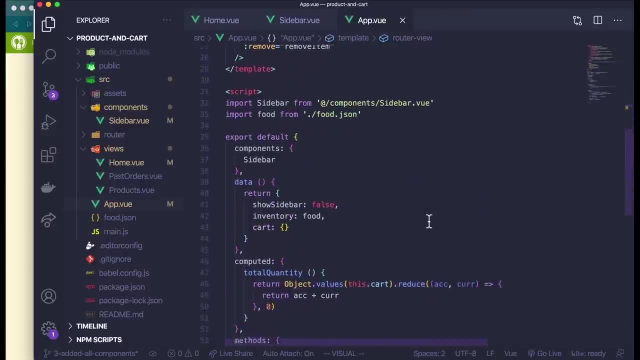 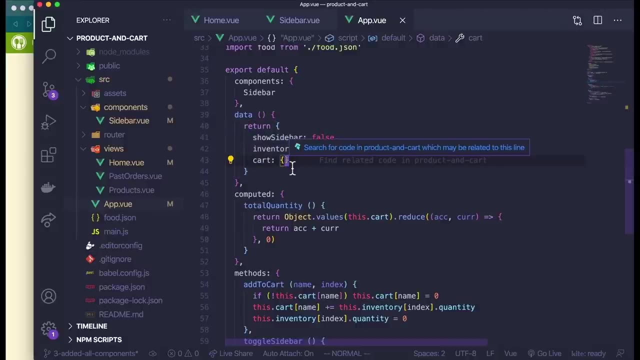 component. we pass functions and variables down to children and then children can call functions like add to cart that will then update the state of the parent component. now, in more complicated applications, we would need something a little bit more robust for state management and being able to share all of this data. 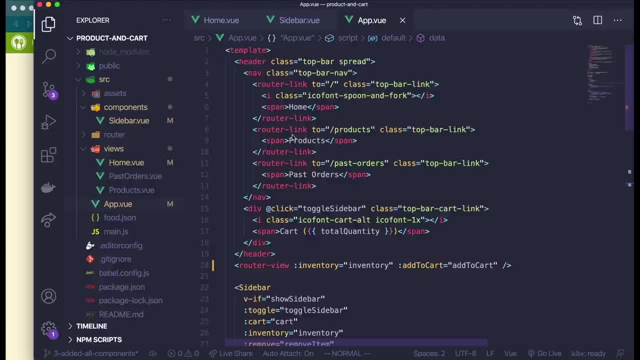 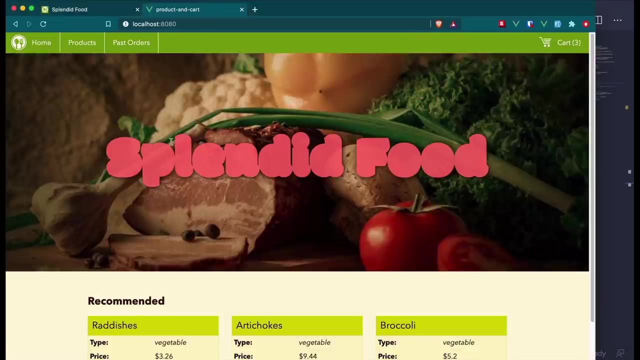 throughout our application and we will talk about that in a future series where we cover vue x, which is vuejs's default state management library. but for right now we are going to leave the application as it is and work on it in future series and lessons. so we have the home. 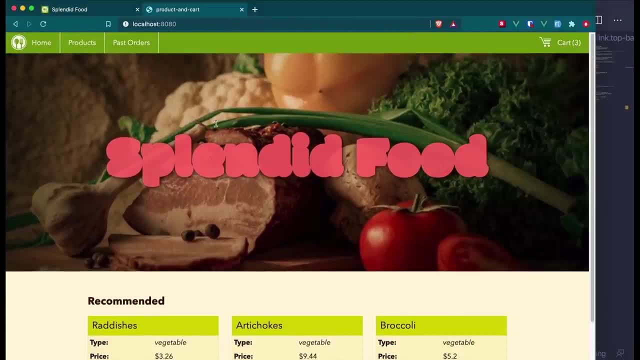 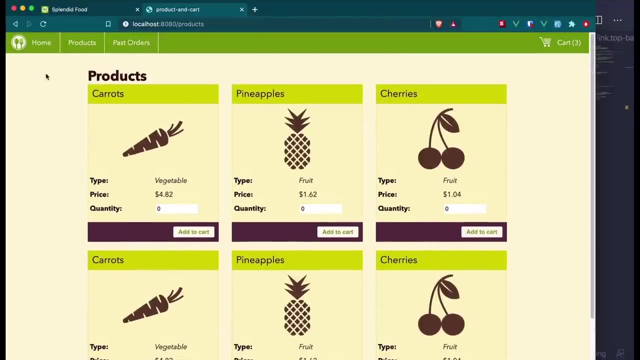 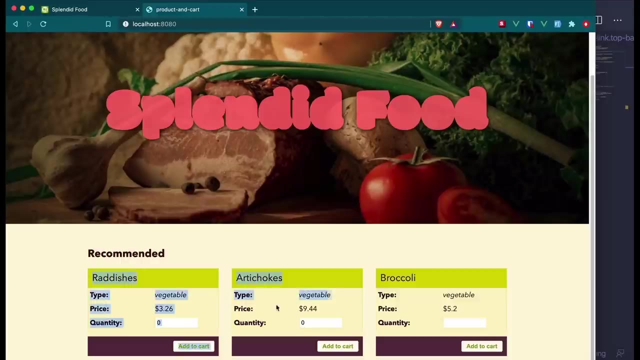 page, the cart sidebar. now we really need to hook up some of the information on this page. so the products page- and it's really exactly the same as the products section here on the home page. we have all of the same kind of cards. we have all of the same kind of. 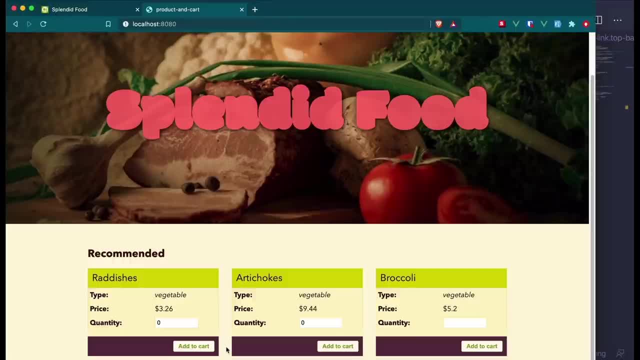 information. so since we have the same thing pretty much in multiple places of the application, it makes sense to pull out all of this UI that makes up these cards into its own component, and then we can share it across the application and on any page that we want. 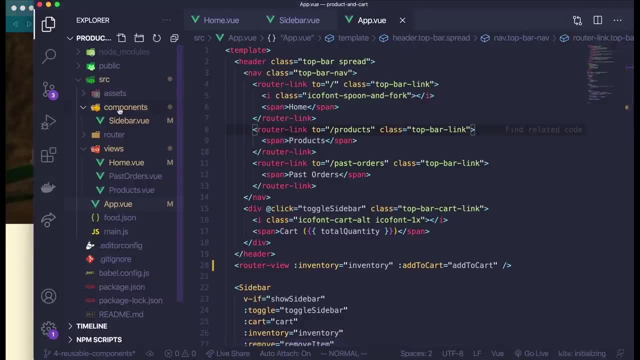 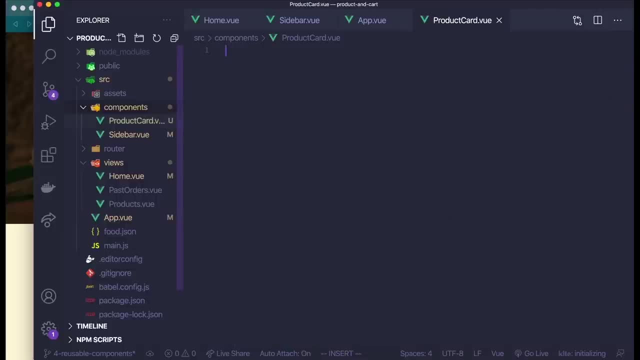 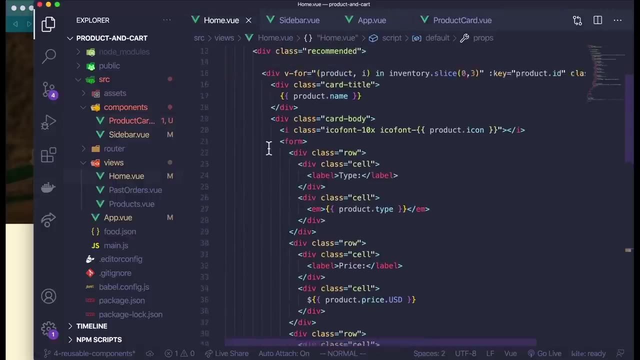 so let's go ahead and create a card component. now in components here I'm going to create a new file called productcardview. I'll start with a template and now I'm going to go to my home page and I can see there's a for loop here. that is: 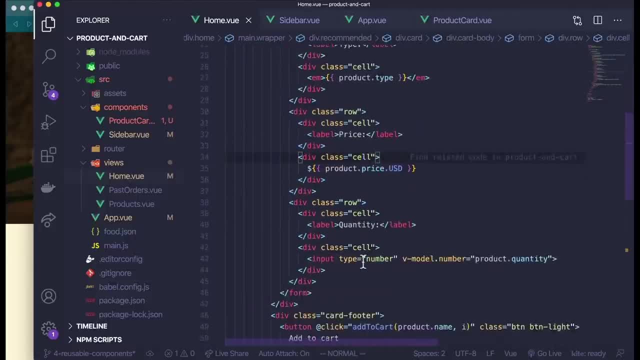 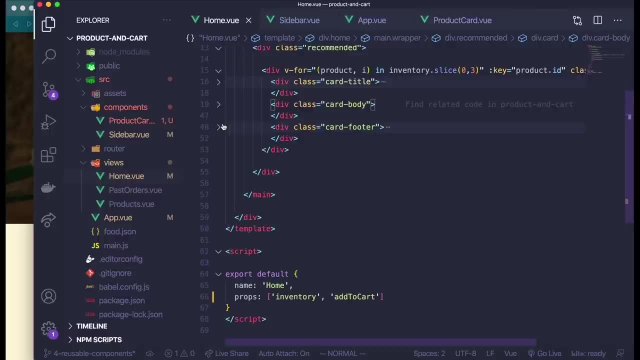 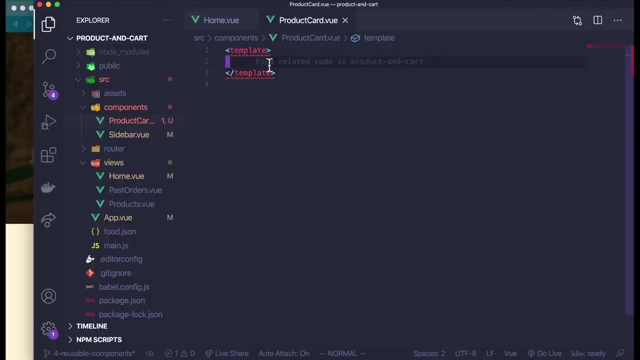 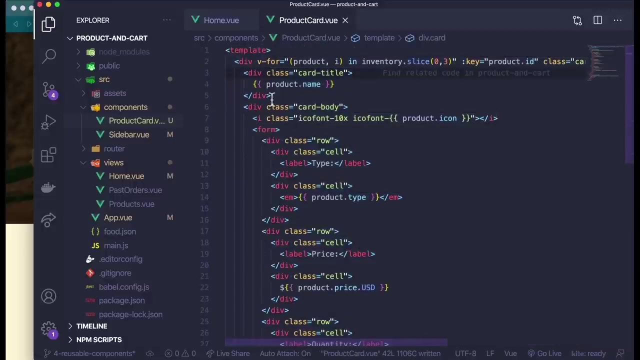 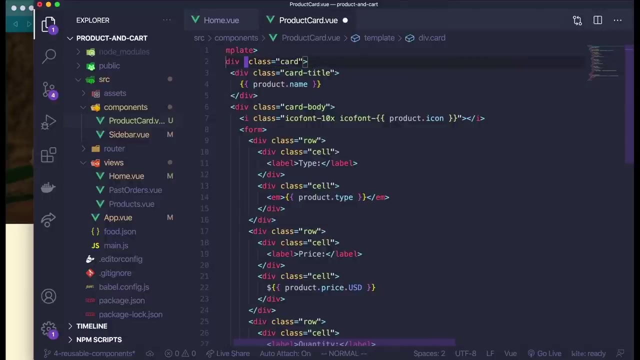 looping through and displaying all of the cards. so I'm going to grab this whole card here and paste it in my product card file, product card file. product card file. now, this is just an individual card, so I don't need a for loop in here. let me get rid of this logic. 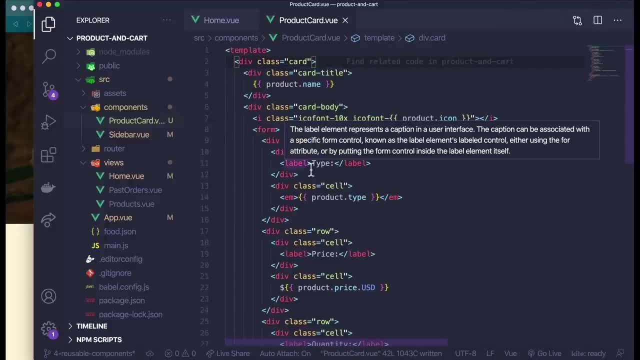 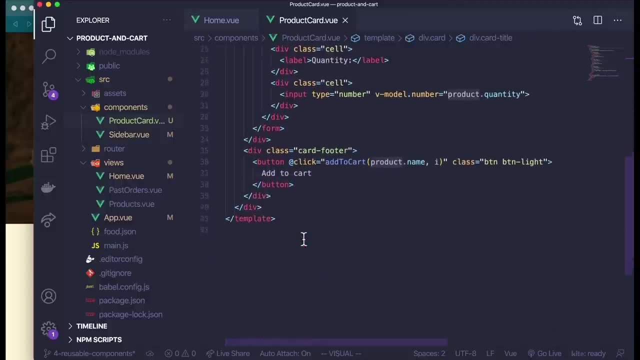 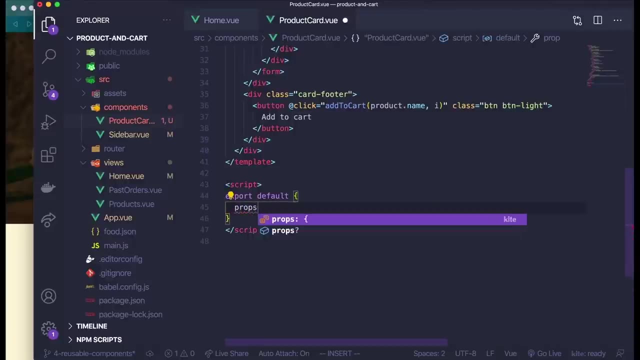 and this will just be one card. now I will need the product information for this card to display correctly, so I'm going to have to accept that as a prop in my component. so let me create a script tag. I'll create props here, just an array of props. 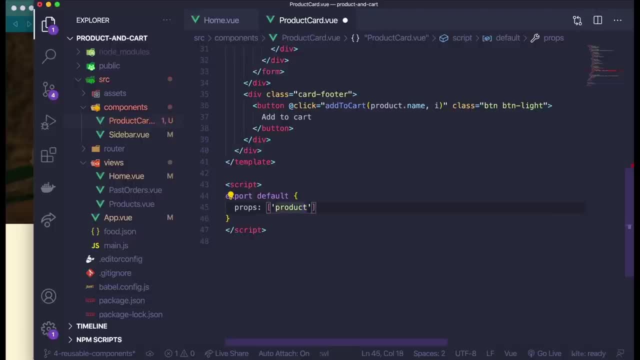 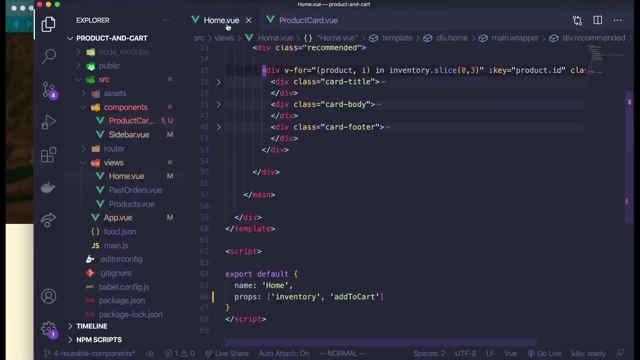 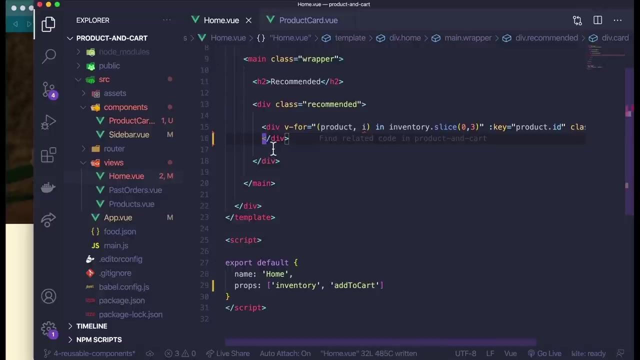 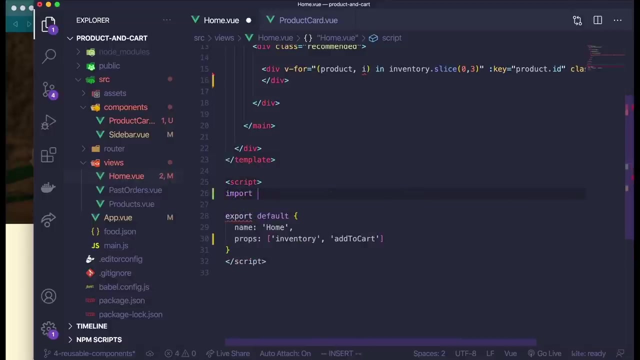 and I'm going to say product. so I accept the product props into my component and now I can use it in my template. now I can remove all of this logic from here and the only thing I need is actually to import that component, to import product card from. 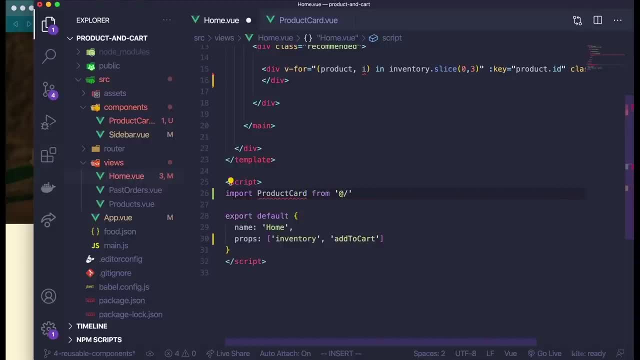 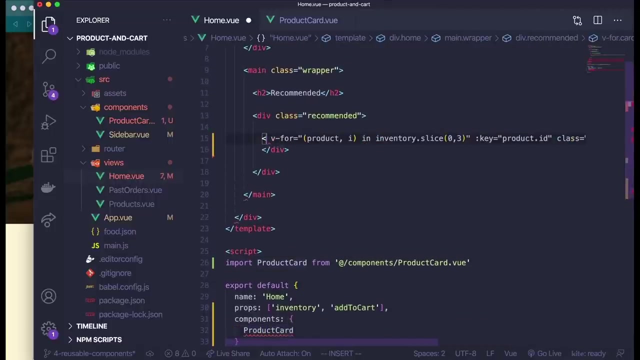 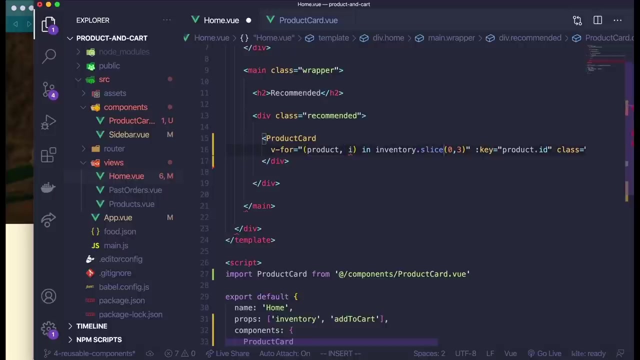 I'm going to use my source folder shortcut, slash components and slash product card dot view, and now I need to register this as a component so I can use it. and now in my code up here I'm going to use product card. I'll clean up the lines. 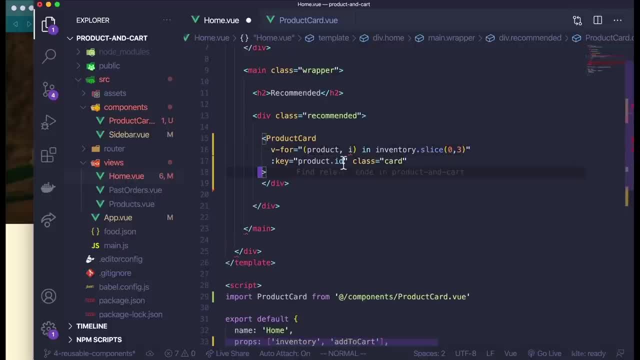 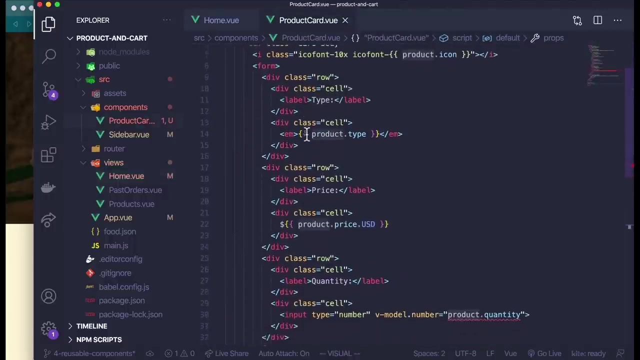 a little bit here and I need to make this self closing because all tags in view templates need to either be self closing or having a closing tag. now I am no longer using this index here. I'm going to see in my product if I'm using the index anywhere. 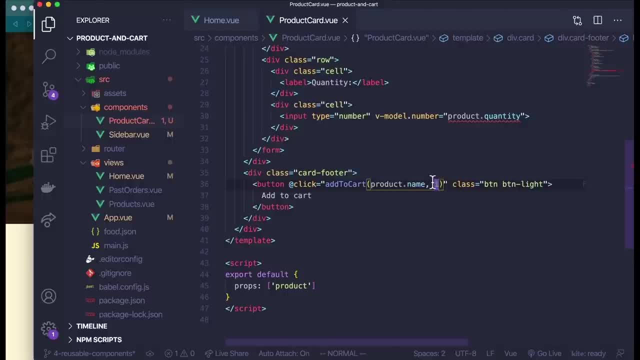 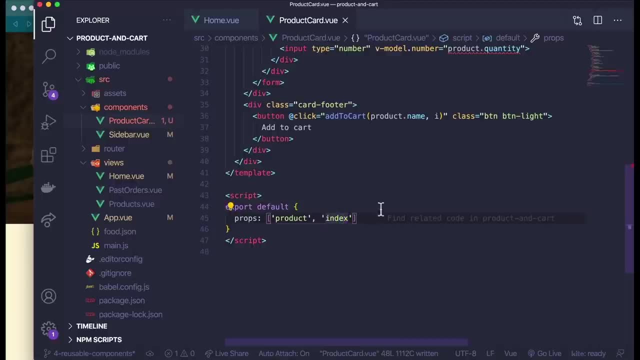 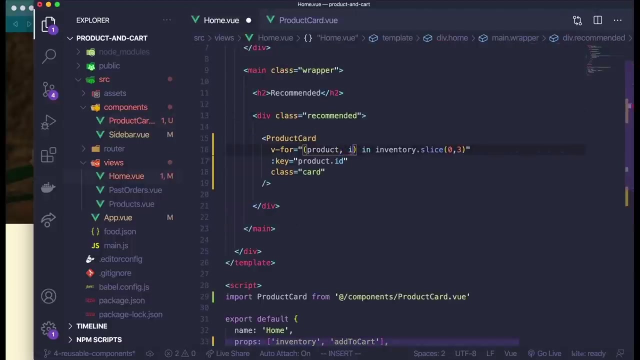 and I am indeed passing in the index, so I will need to accept the index as a prop as well. let me change this to index so it's a little bit more clear, and I will get index here and I'm going to pass that in here and 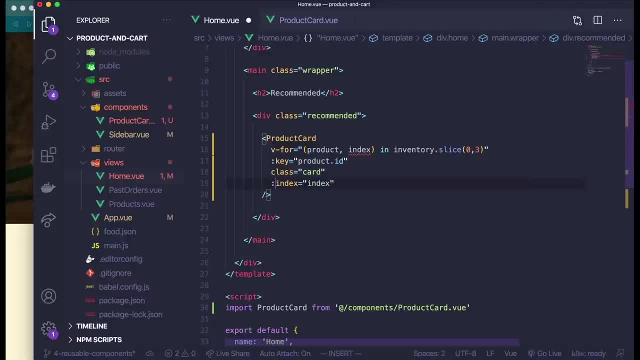 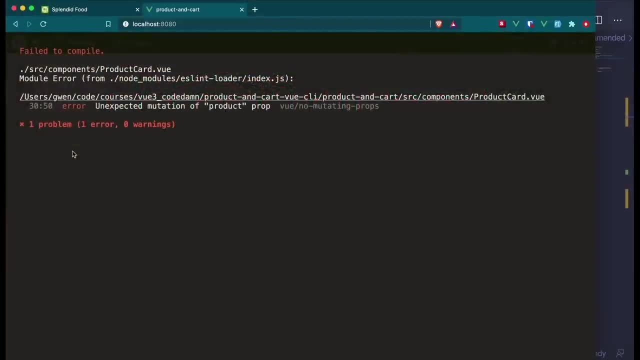 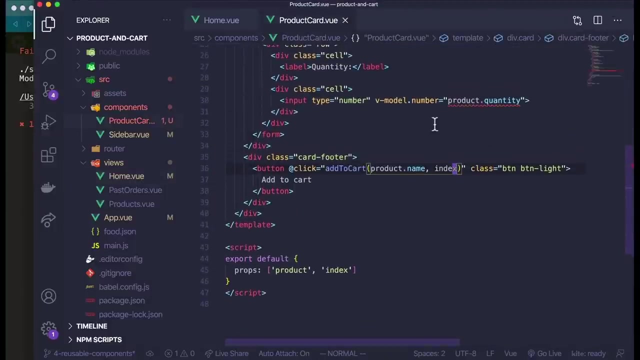 of course index is a variable, not a string, so I'll have to vbind that, and that should work here. let's see if this works. and we are getting an error here now, that is because product is now a prop and of course we cannot mutate props from the parent component. 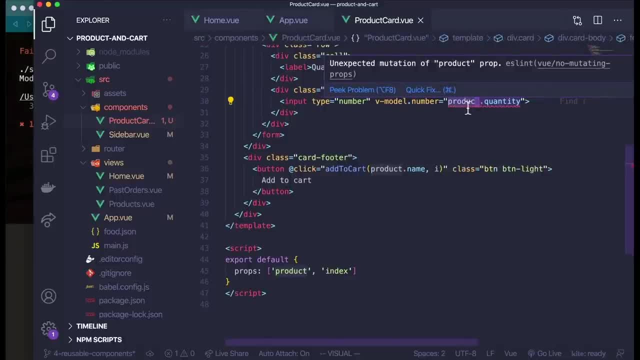 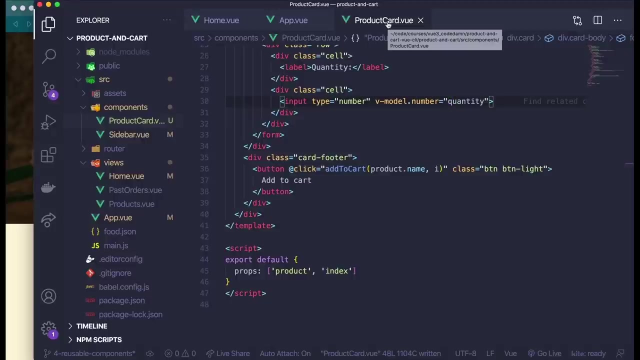 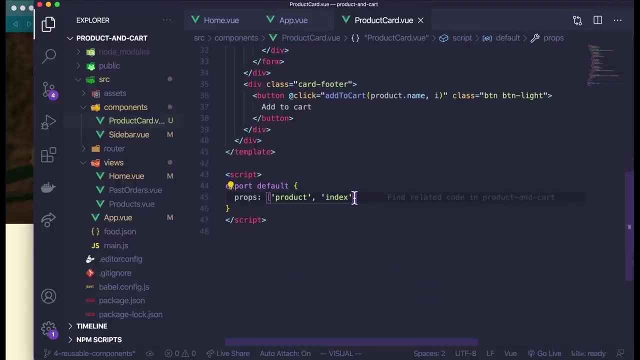 so we can actually fix this by not mapping to the product prop at all. we are actually going to create a local variable inside of this product component. so each component, each time we use the product card component, it will have its own local variable. and we can do that by adding. 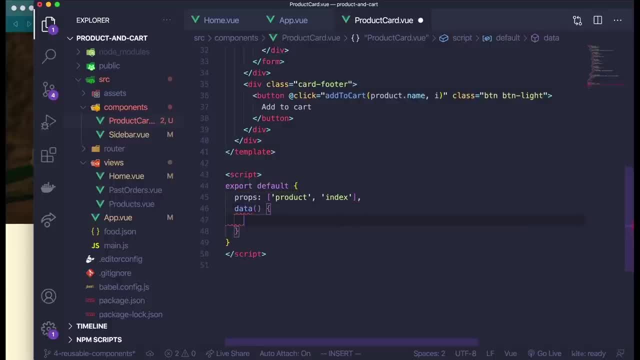 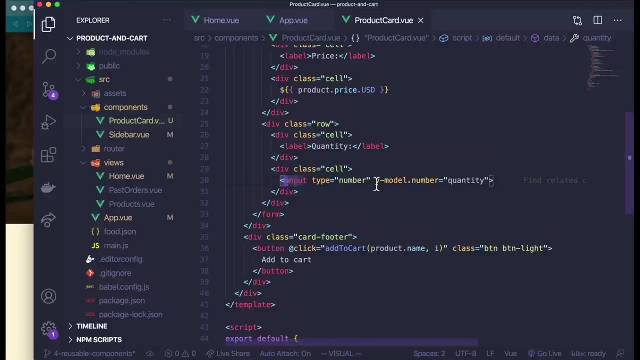 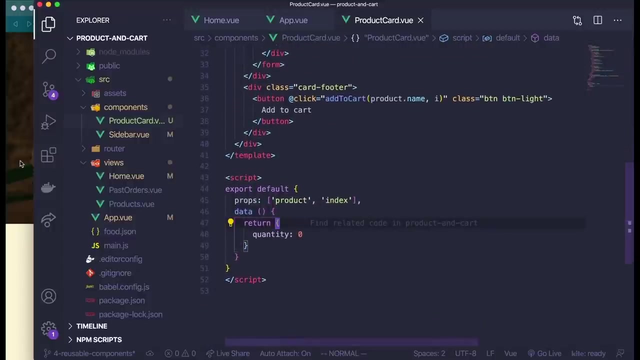 a data prop here and in the method we need return returns it object and now we can simply map quantity because each card only has one input box. so we'll just map it internally in the card and we can check that this works. I'm not sure why it only has two cards right now. 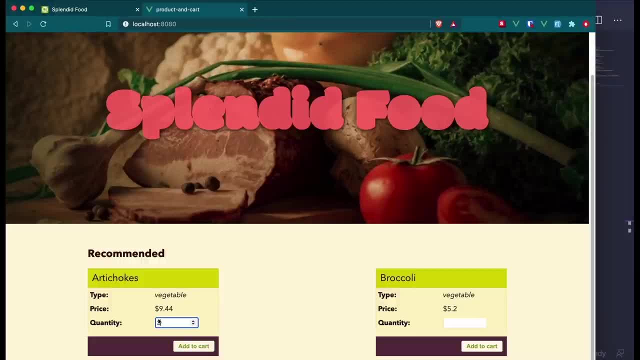 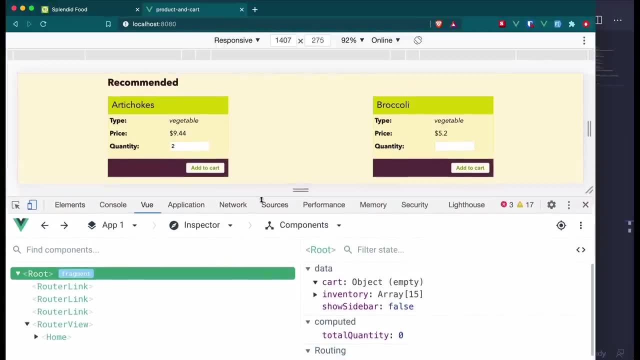 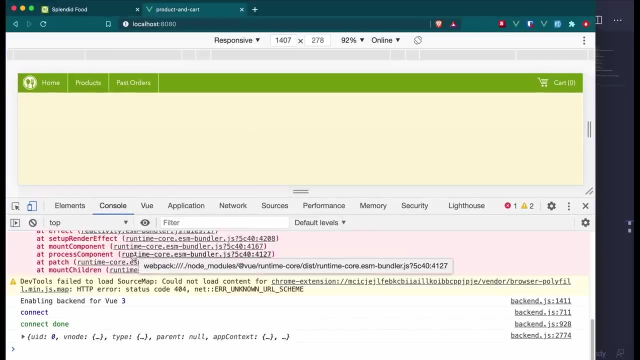 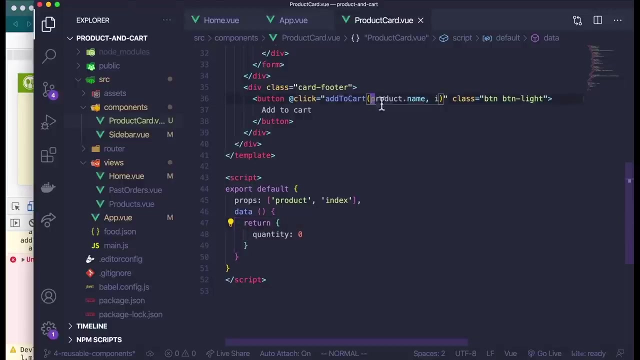 but let's try this. so I press the number 2 and I can look in my Vuejs dev tools and I'm getting an error here and it says I can't read property name of undefined, so productname. yes, I believe I have forgotten to pass. 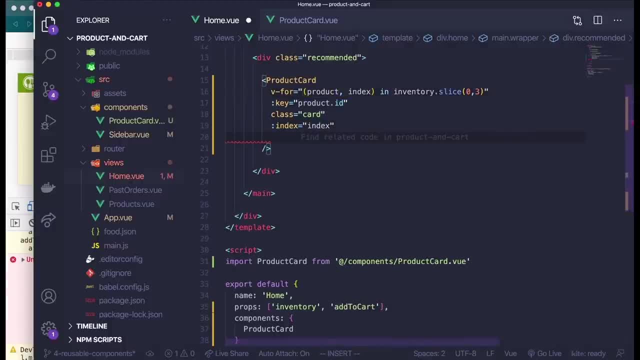 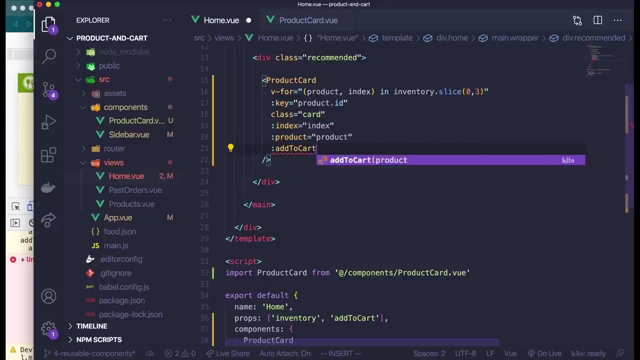 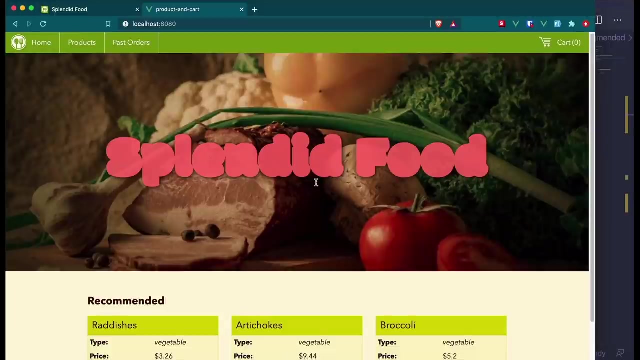 in the correct props here, so let me add those I need to pass in product equals. and then, while I'm here, let me also add the add to cart function equals add to cart. there we go, and now let's check if the page loads and the page 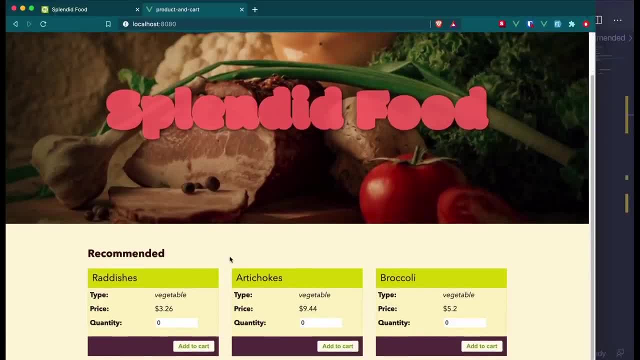 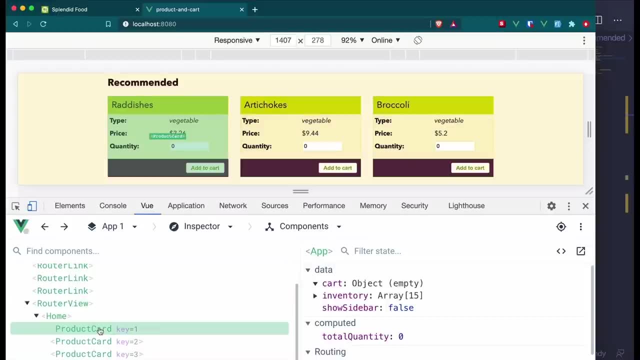 is loading alright. so now we have all of the cards loading and let me just look in my Vuejs dev tools. I can see all of my product card components. so let me just take a look if I change this to 2, and I can see the quantity. 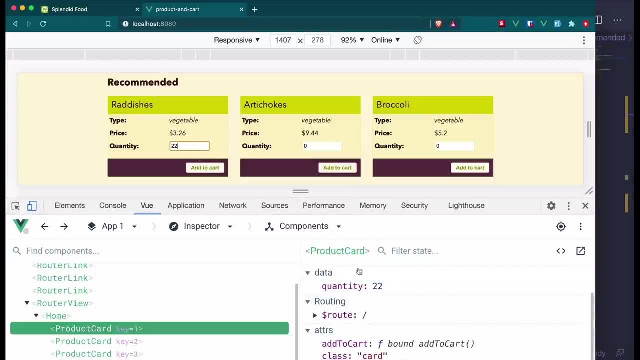 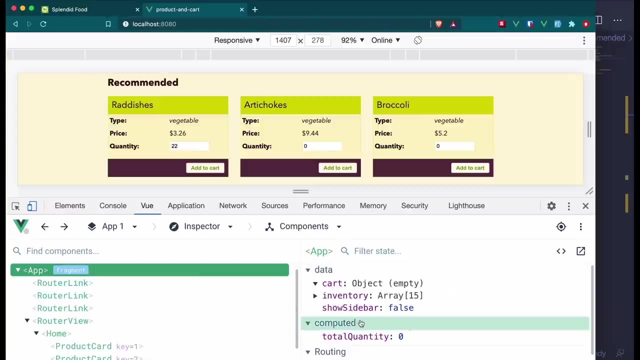 is 2. if I change it to 22, it's now 22. alright, so that is mapping correctly. now I need to get this quantity, the value, up through the home component to the app component, where I am actually performing the function of adding it to the cart. 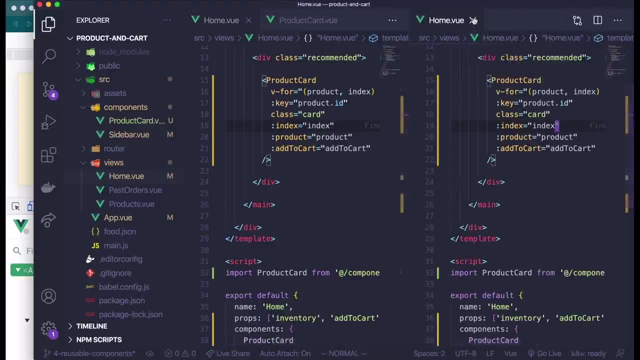 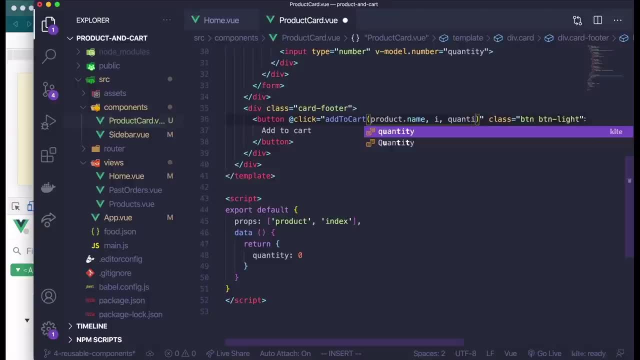 so what I'm going to do for right now, I'm just going to pass in a third parameter and I will pass in quantity. and now let's take a look at our function, our add to cart function in the app component. so we are adding items onto the cart. 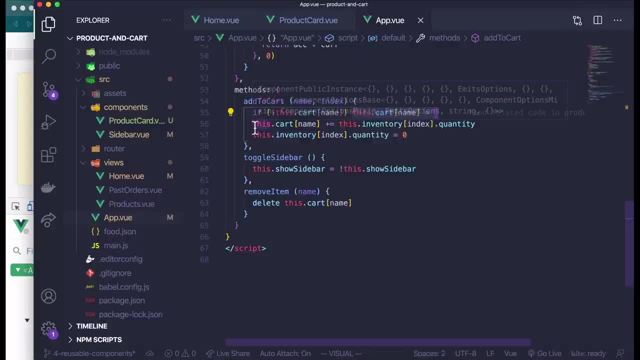 if they're not already there, and then we are basically incrementing the number here. so, now that we have that third parameter being passed in, which is the quantity, all we have to do is change this line to be plus equals quantity, which is now getting passed in. 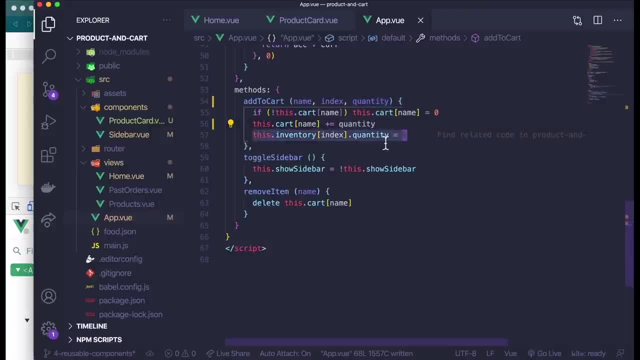 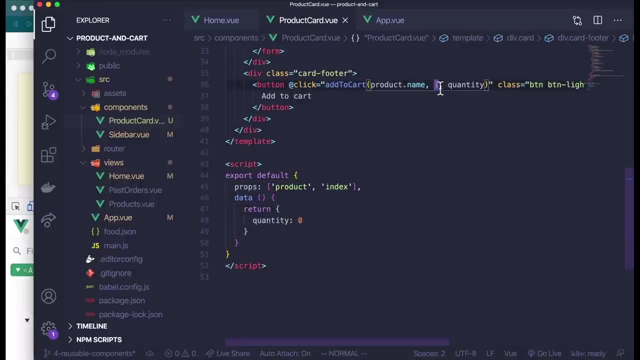 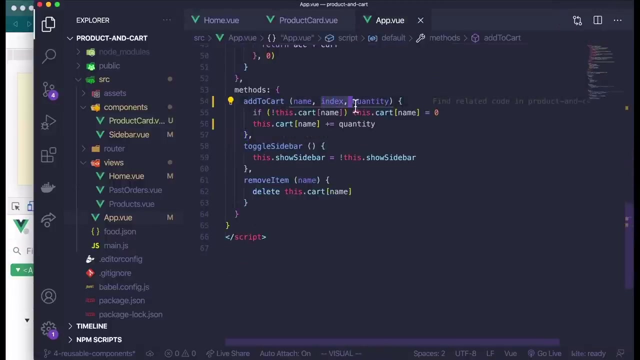 and then, of course, we don't need this line because we are no longer mapping to a nested quantity, rather, we have the quantity variable right here. this also means that we don't need to pass up the index anymore, so we can remove that from this function. we only need the name. 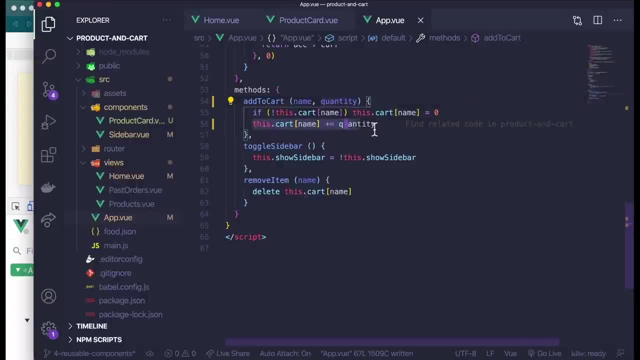 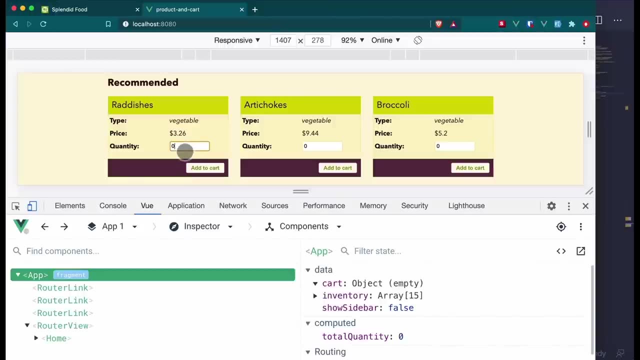 and the quantity, basically so that we can add it to the cart. let's check and see if this works. if I come here, the number still maps to the component. now if I click add to cart, it is not in my cart. let's see if we got an error. 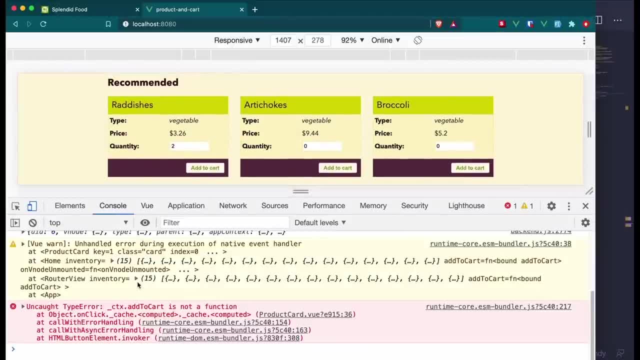 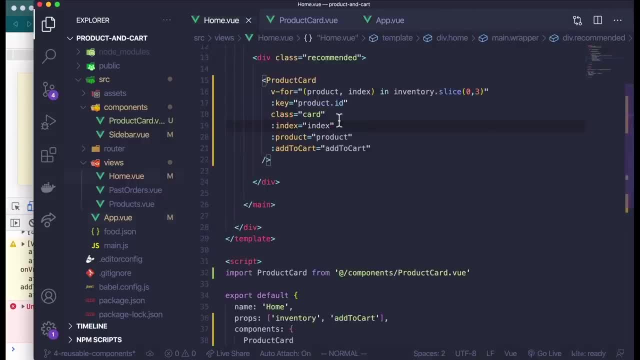 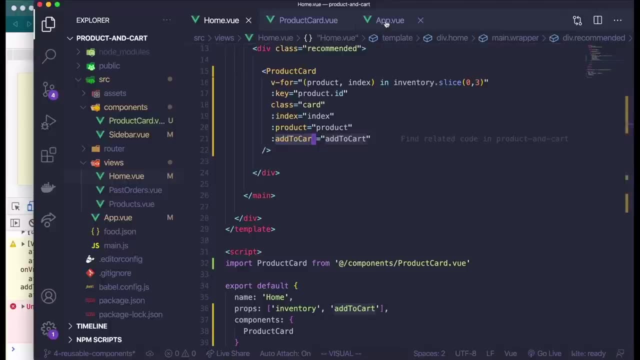 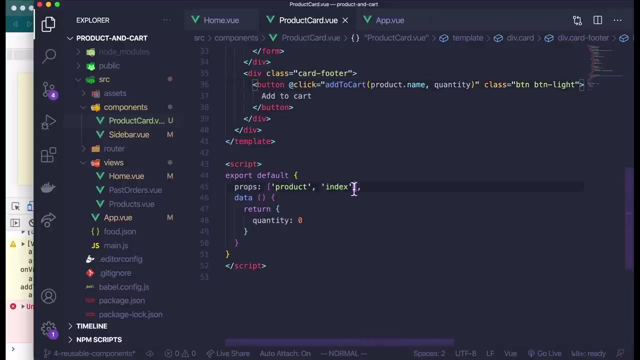 add to cart is not a function. let me look inside of my home dot view. I have add to cart that I am getting from the parent component and I'm going to remove it, so from the app component. I'm passing that in to the product card and I should have it. 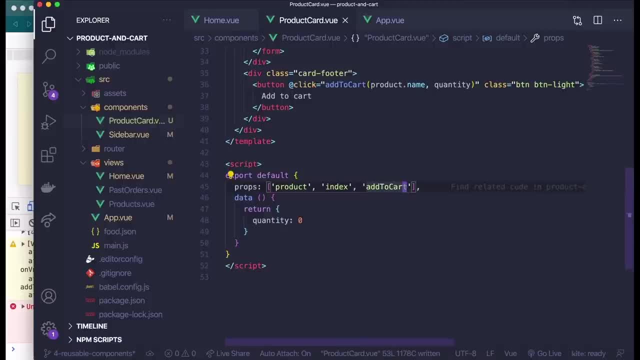 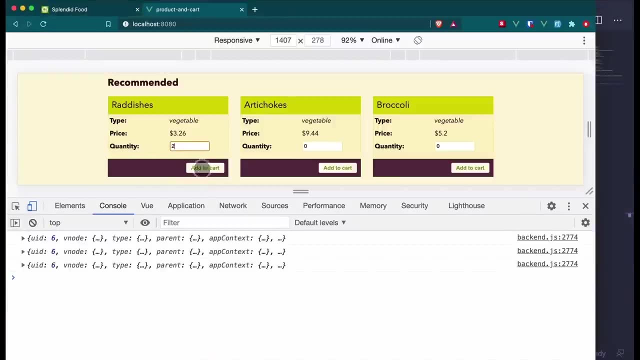 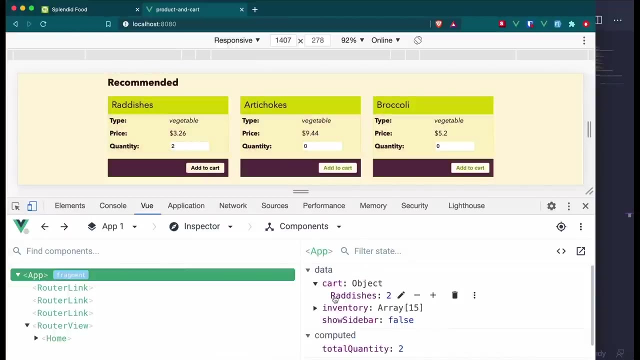 oh right, I didn't accept it as a prop inside of the product card, so now let's see if this works. let me refresh and go into my view: dev tools, and now I can see it's properly working here. if I want to add 10 artichokes. 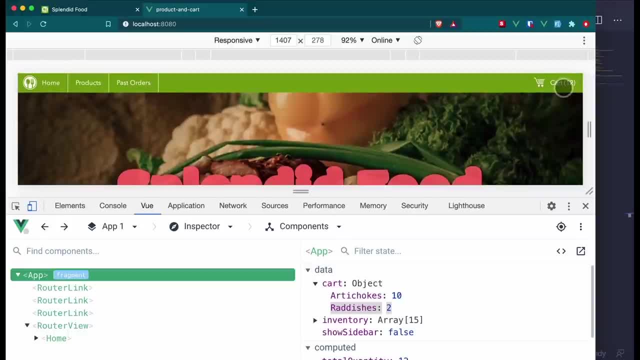 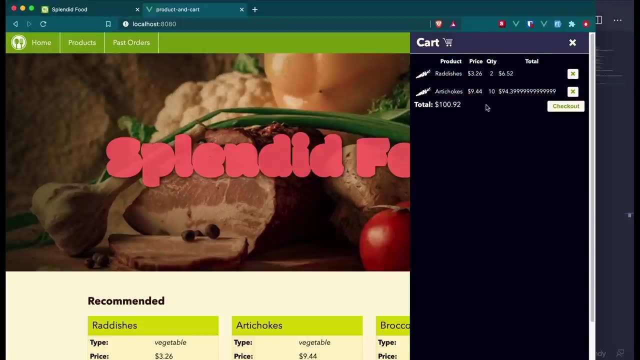 and I have 2 radishes and I have 12 items in the cart. now my rounding functionality isn't properly working, as you can see, but it is properly adding and displaying the quantity and the total in the cart. but I don't just want this functionality on the home page. 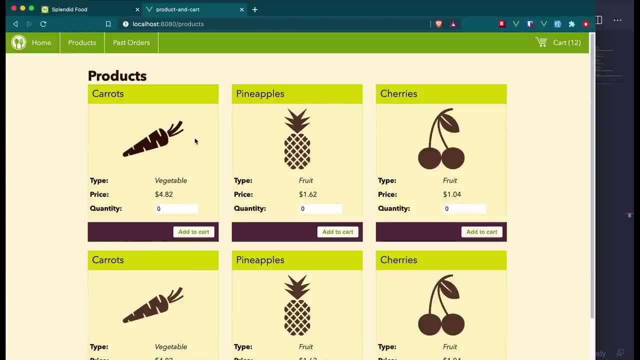 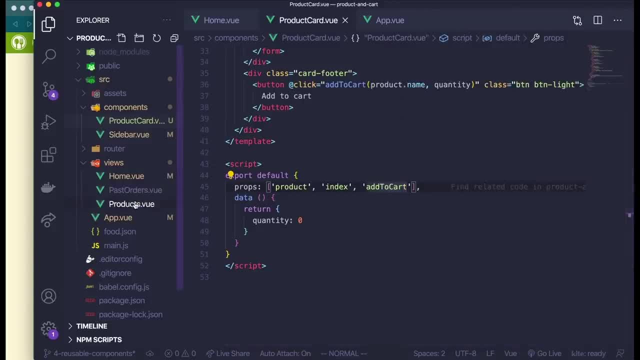 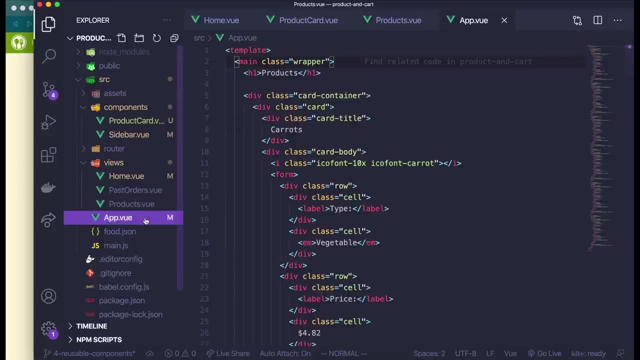 I also want it on the products page, so let me import those components into the products page now. so if I come to my products dot view file, I actually have access to inventory already in here because, if you remember, in my app dot view I am passing inventory. 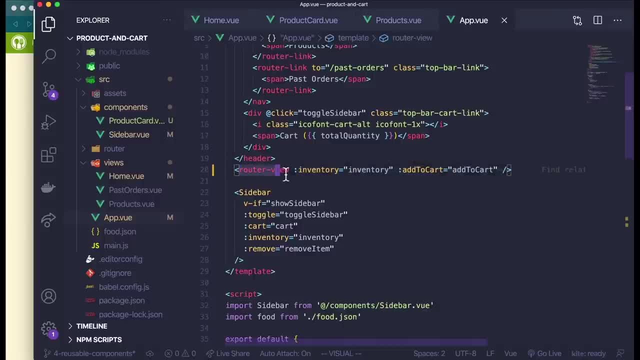 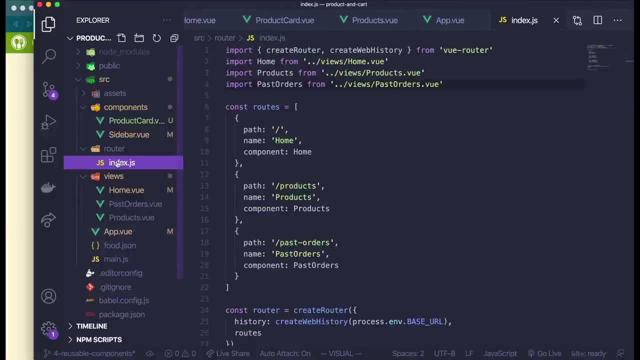 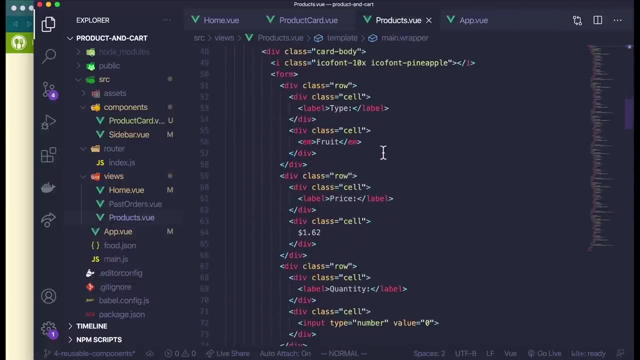 and the add to cart function into anything displayed by the router view, which is basically any of our pages here: home, past orders or products. they are all connected to our router, so let's accept those props in the products page to start with. first let me fold up all of these cards. 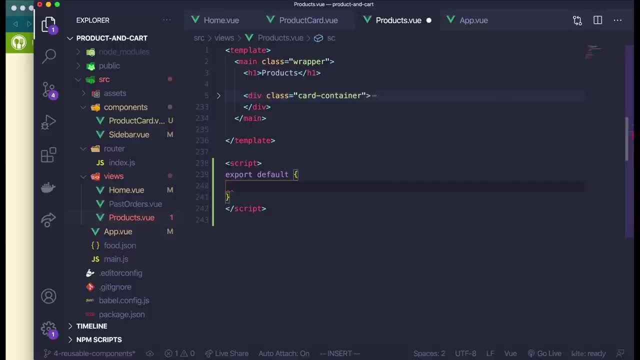 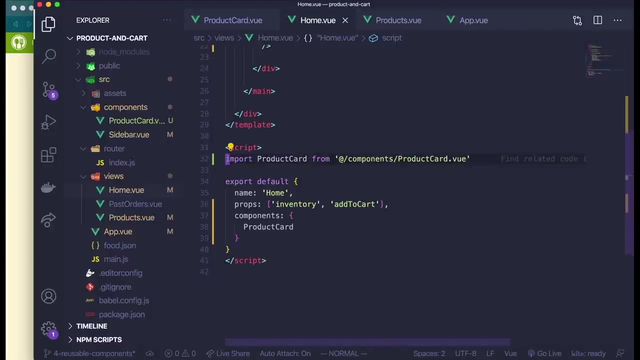 get them out of the way. so let me do a script, tag props and I'm going to accept inventory and add to cart. and one more thing I need to do is import this product card. so I'm going to go to the home component and just copy this import. 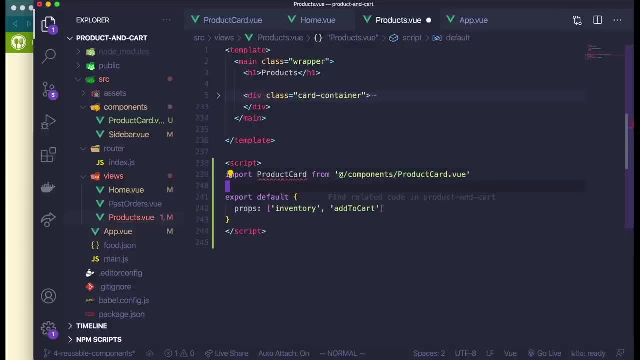 and paste it into product or into the products page. and now I need to define this as a component here, product card, and this should be components, not component. and I also have one more error here, which this should be a capital P. and now, if I see, if I highlight this, 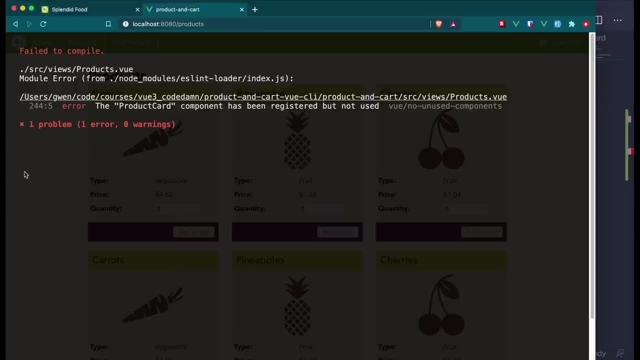 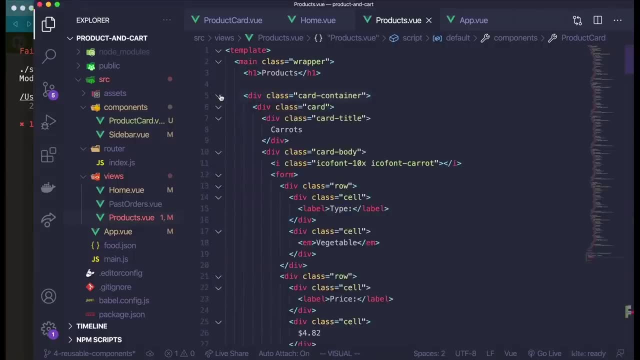 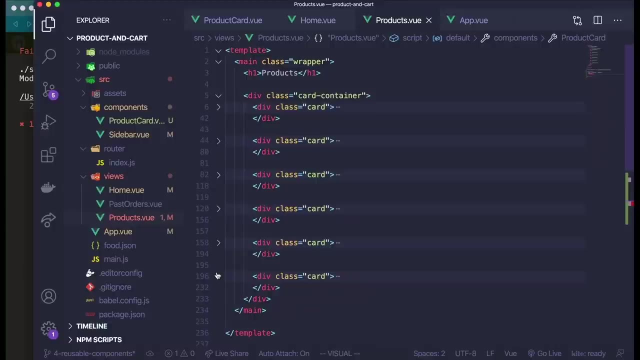 all of these highlight. let me take a look at what this error is here. the product card component has been registered but not used, so let's fix that. so I basically have all of these cards here for the different items that show up on the page I'm actually going to just delete. 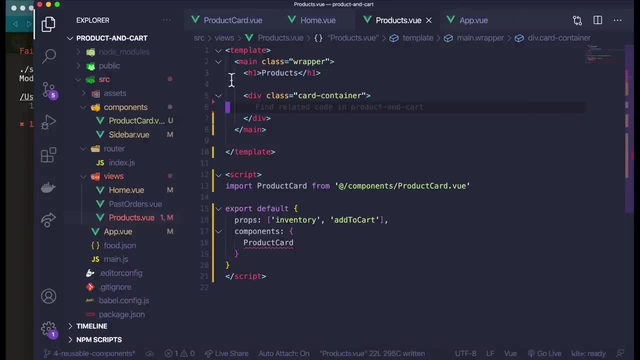 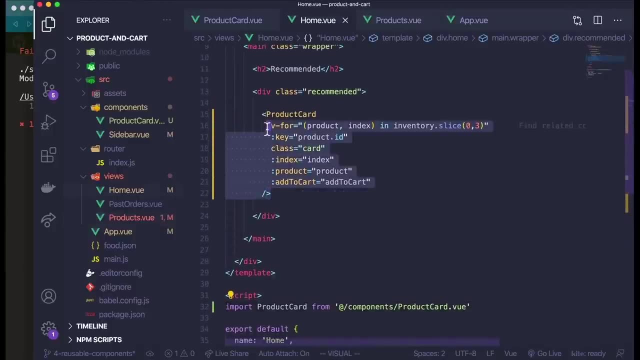 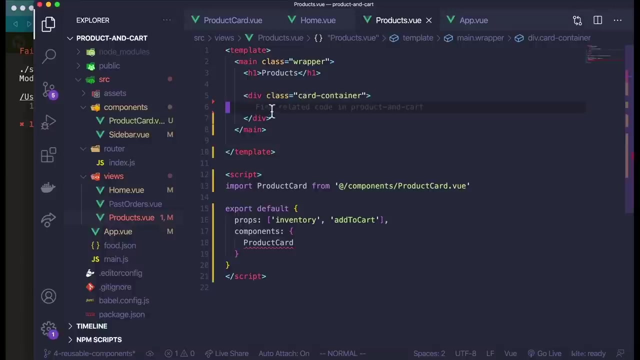 all of these right now and instead I'm going to add the product card, so if I go to home I can take a look at my product card that I'm actually using inside the template and I'm just going to copy that and paste it here. but instead of 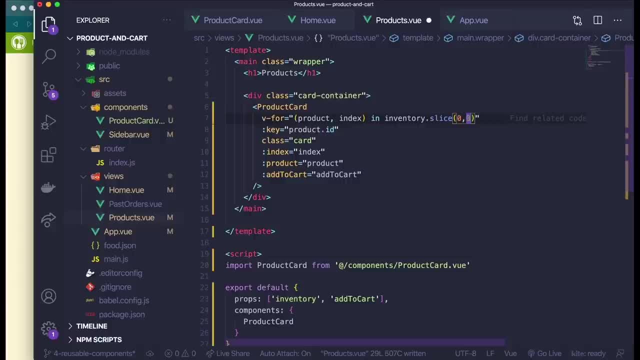 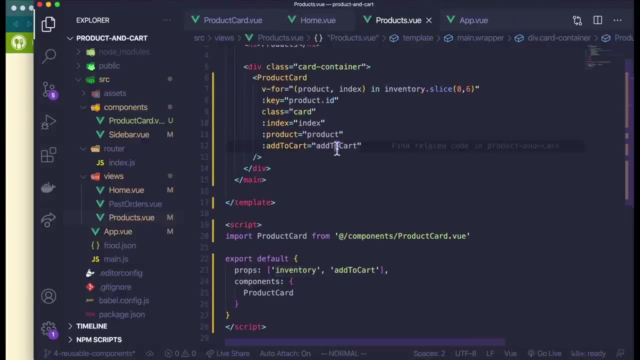 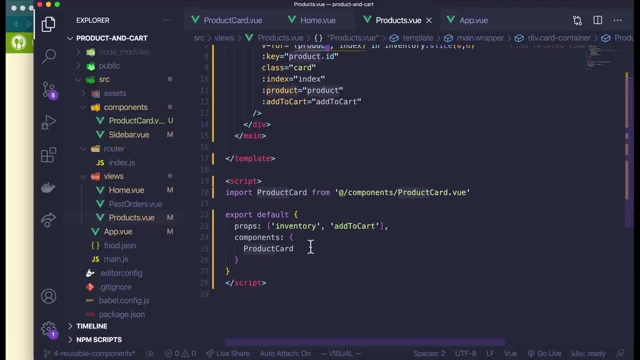 slicing at three here. let me just do the first six elements instead now, because we already have inventory being passed in, as well as the add to cart function. of course, inside the loop we're taking care of the product variable. there's really no other state that we have locally. 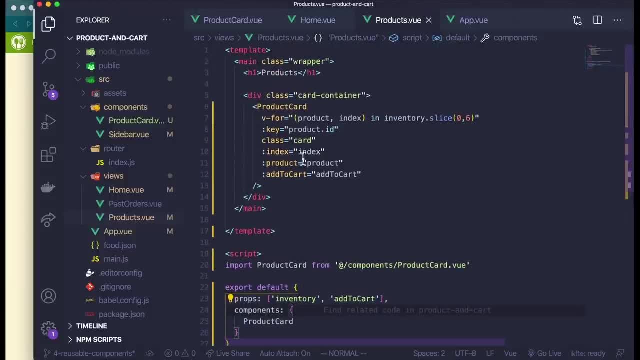 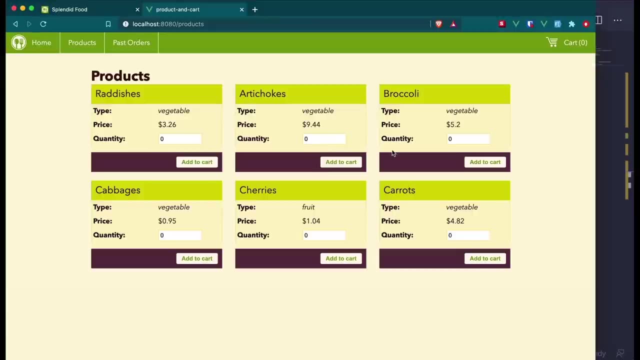 on the products component, so this should pretty much work out of the box for us. let's check here and we can see that it does indeed loop through and display all of the cards on the products page. now let me add a couple of these items to the cart here. 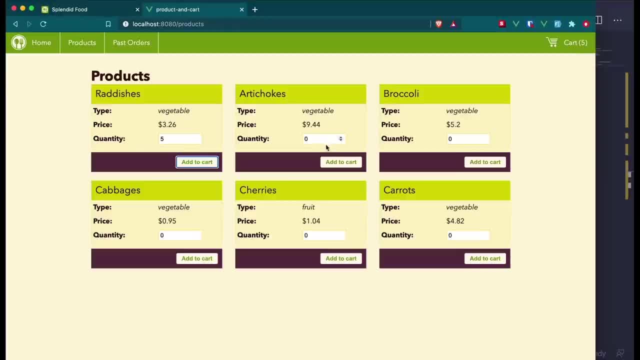 and you can see the cart just updated with five. if I add a few artichokes, let's add some cherries and some cabbage carrots, everything right. we have seventeen items in the cart now and we can see that it added all of these items now, if I 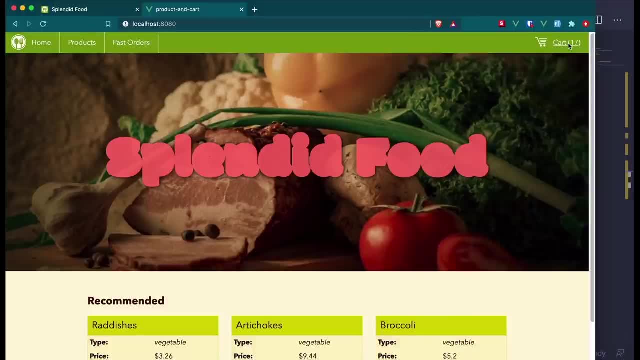 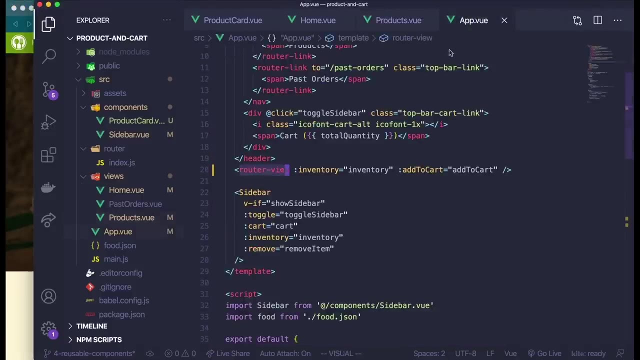 go to the home page, I can still see seventeen items in the cart because we moved to a single page application. all of our routing is handled by the Vuejs javascript and we are actually sharing state between components. so all of the state for our cart lives in the app component. 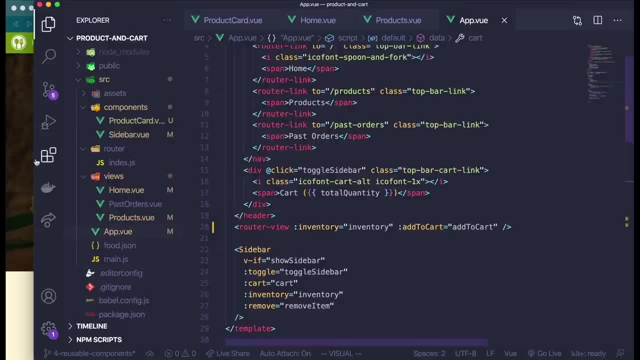 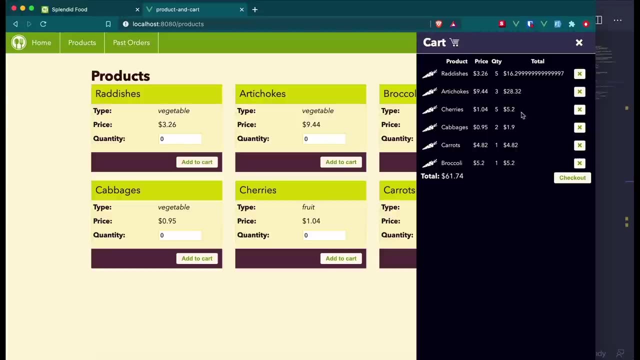 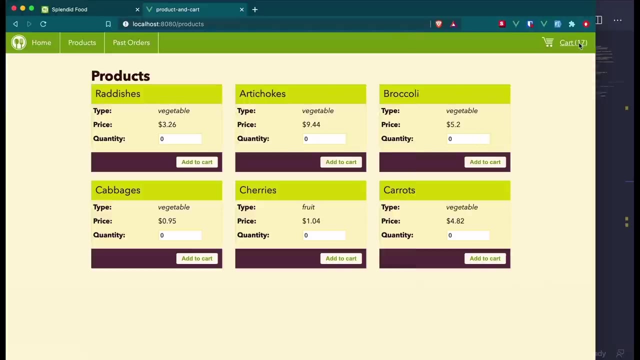 which is the parent component of all the other pages: the home page, the product page- and that's why all of the items in the cart, all of the data that we save here in our application, it stays, no matter what page we navigate to, and even though this is displayed, 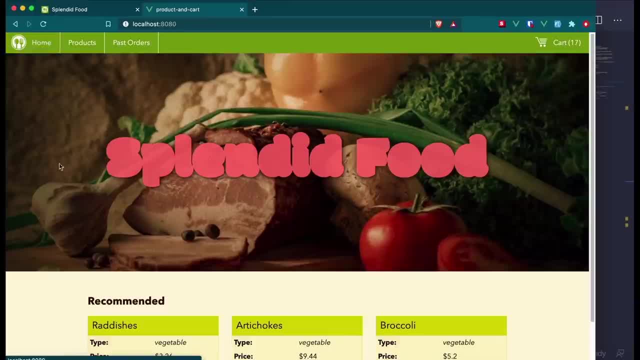 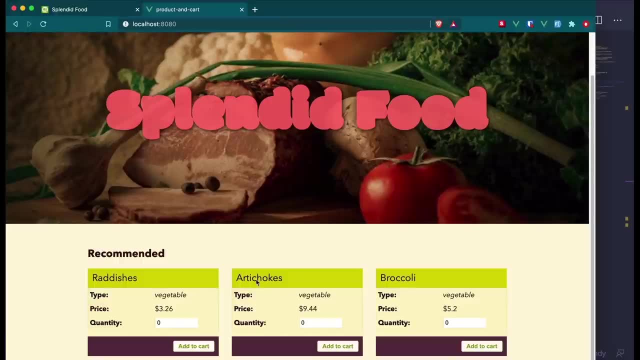 or this card is on multiple pages. you can see how Vue made it very easy for us to reuse the same code and the same template to loop through and display wherever we wanted on the application, and that's basically how reusable components work in Vuejs, I hope. 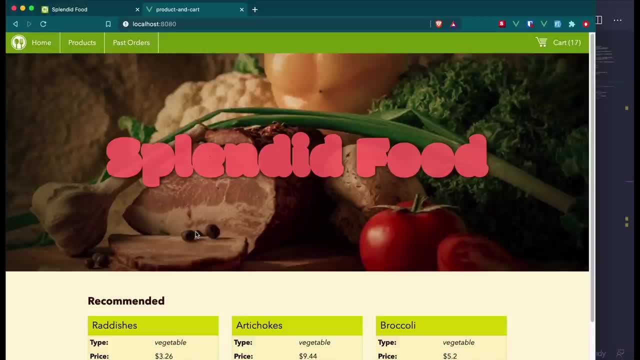 you enjoyed this course and you learned a lot about Vuejs learning it on three different levels. through this course. we started off working in a basic indexhtml file and then we went on to a static site, upgrading it a little bit with some Vuejs, and then we moved on.